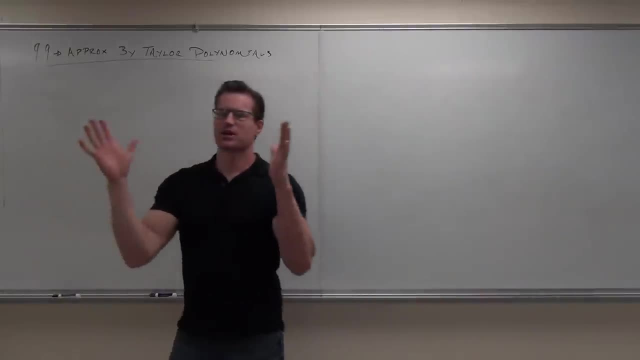 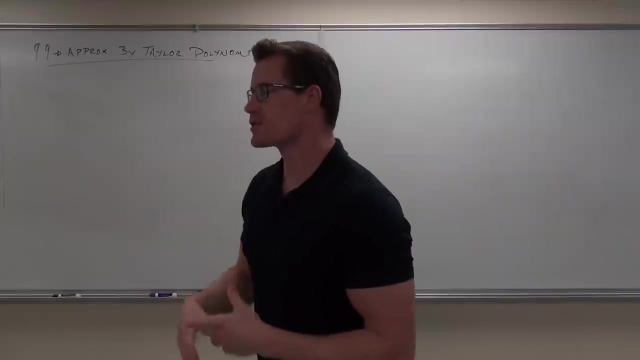 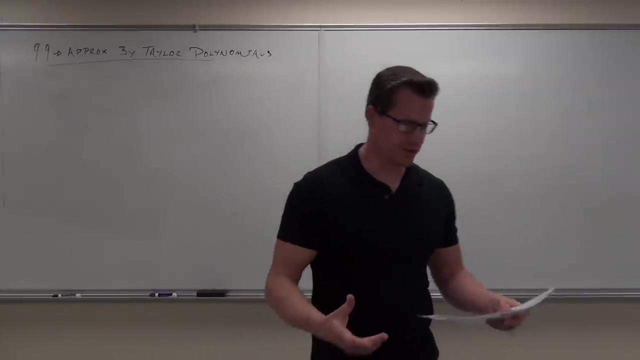 Okay, so the last section we're going to talk about in Chapter 9, the last section we're going to talk about is how to approximate a function using what's called a Taylor Polynomial. Now, these things are based on Taylor Series, so the idea is using a Taylor Polynomial, which is it's just part of a Taylor Series, to closely mimic a function around a certain point for a certain interval. 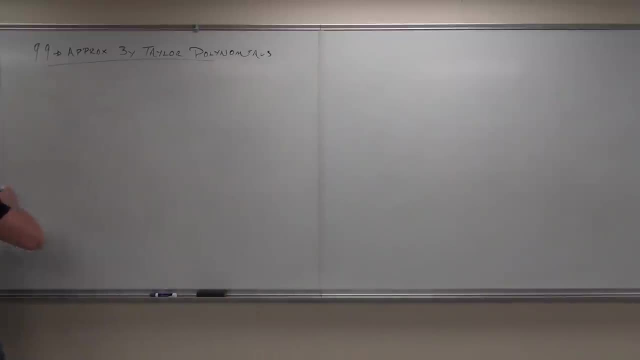 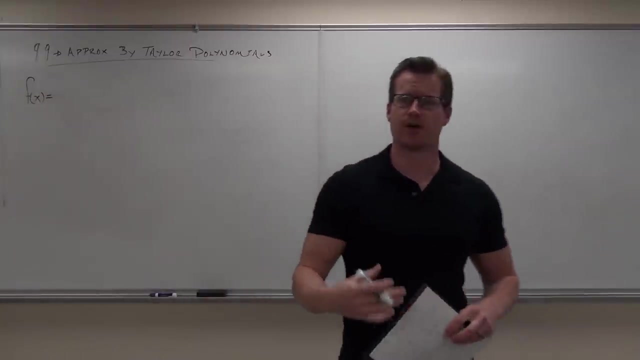 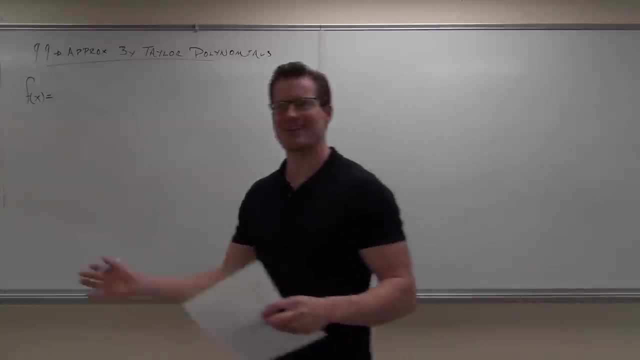 So let me start y'all with this: Given a function, so let's say we have some function. What we know from our last section is that we can represent this function with a Taylor Series. Remember talking about Taylor Series? I hope so. We had spring break here recently, so hopefully that word, that phrase, is in your mind somewhere. 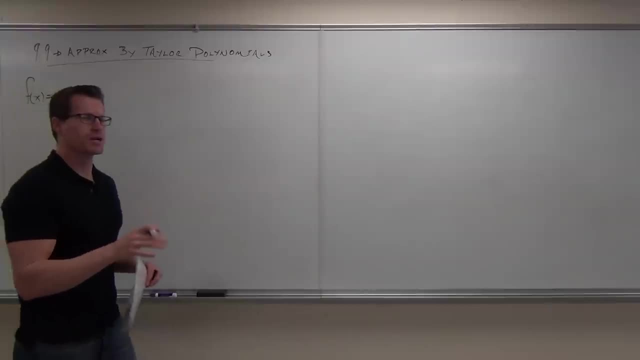 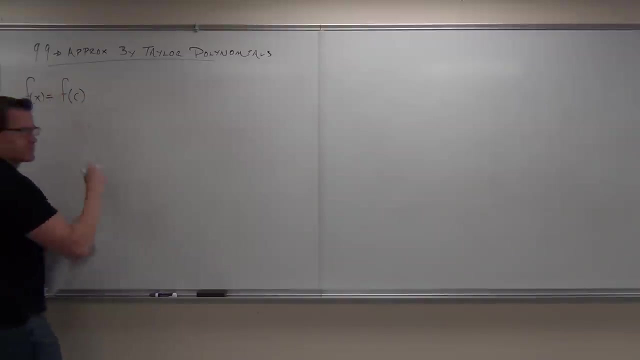 So a Taylor Series does this. It says: hey, if you want to represent your function of x, you can do it. this way, You can start off with your function at some point that we like- We've already said so- at point c equals 1, or c equals whatever I want. So we say: alright, well, the function of f of x can be represented by the function at c plus the first derivative of the function at c, times x minus c. Do you remember doing this? 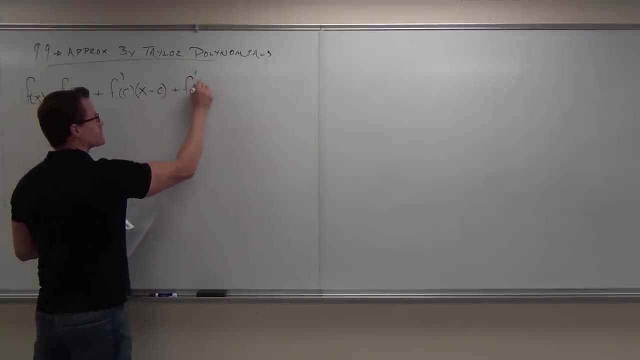 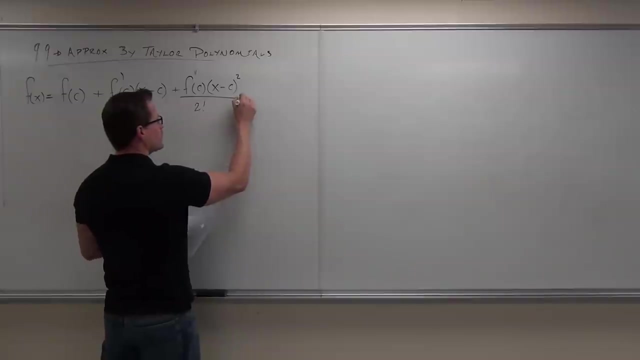 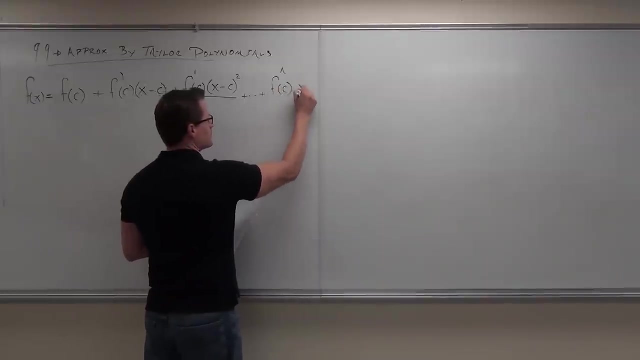 Yes, Plus the second derivative at c, times x minus c to the second, all over 2 factorial plus. and we keep on going until we get to the nth derivative. Thith derivative at c, x minus c to the nth, all over n factorial. 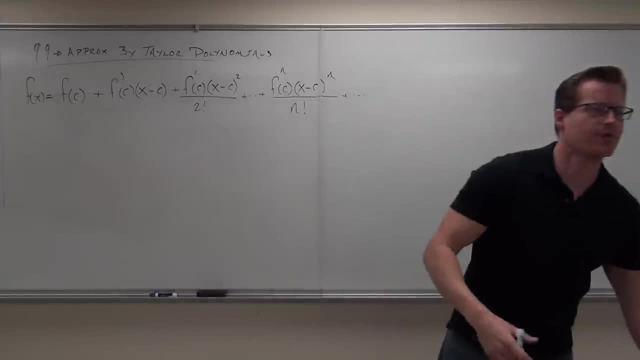 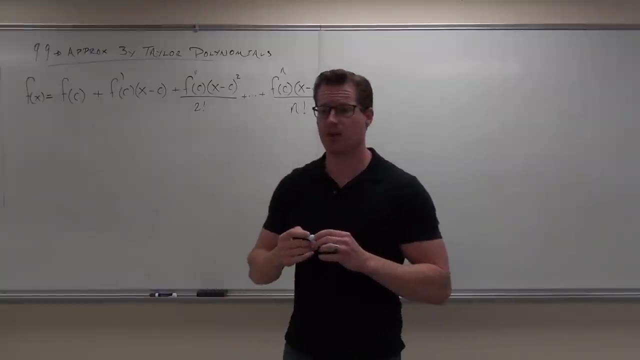 And then this thing keeps on going forever and ever and ever and ever, and that was called a Taylor Series. So show up here if you feel okay with the idea of a Taylor Series. So what we said basically in the last section was: hey, you know what We can represent our function with a Taylor Series or a Maclaurin Series. 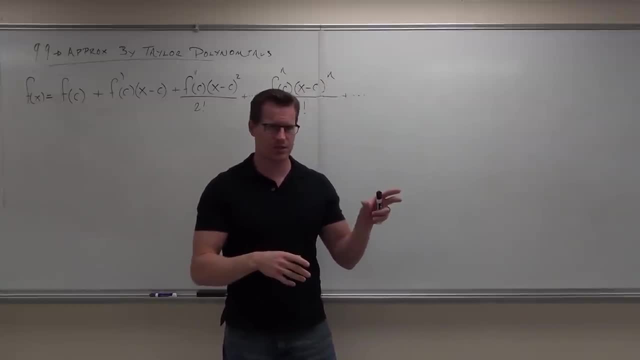 Of course, the only difference between a Taylor Series and a Maclaurin Series is that a Maclaurin Series always has a Taylor Series as a center of what Zero. Very good Taylor series as a center of whatever I want. 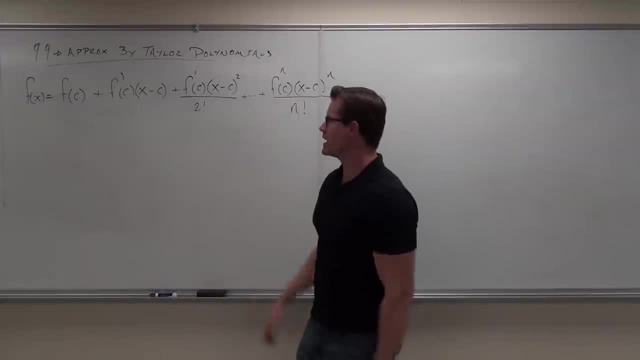 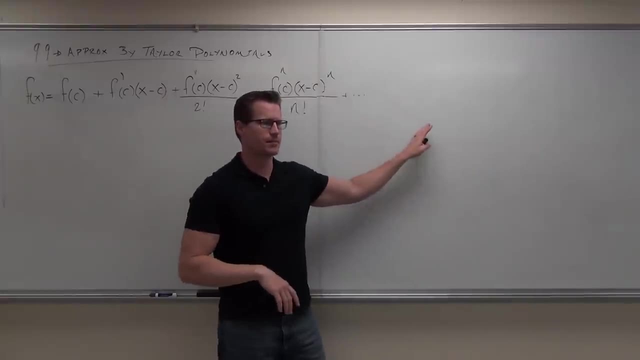 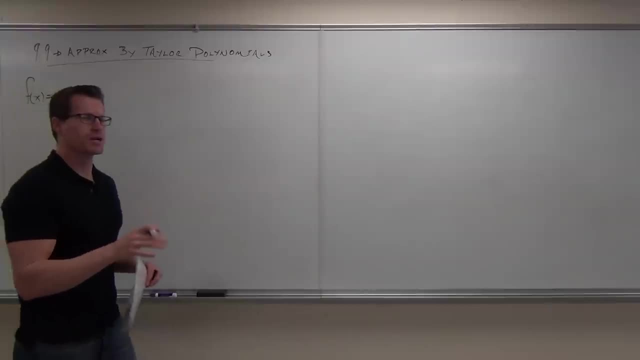 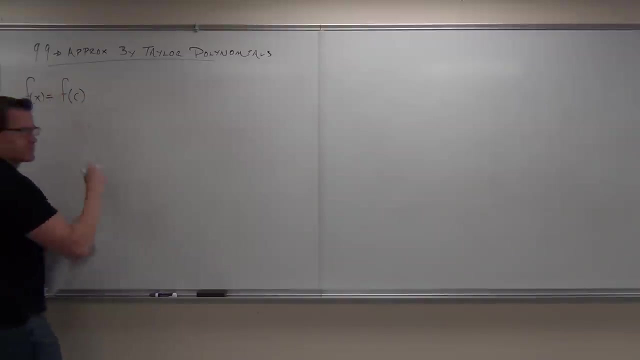 So a Taylor Series does this. It says: hey, if you want to represent your function of x, you can do it. this way, You can start off with your function at some point that we like- We've already said so- at point c equals 1, or c equals whatever I want. So we say: alright, well, the function of f of x can be represented by the function at c plus the first derivative of the function at c, times x minus c. Do you remember doing this? 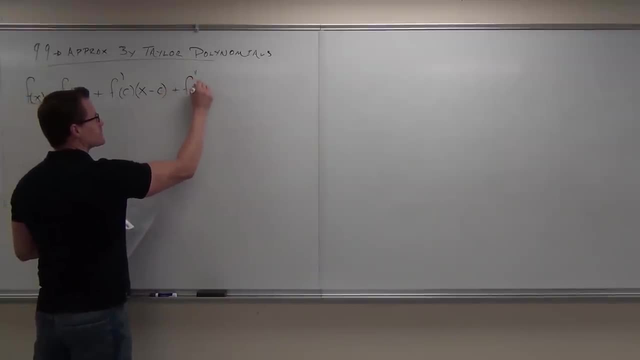 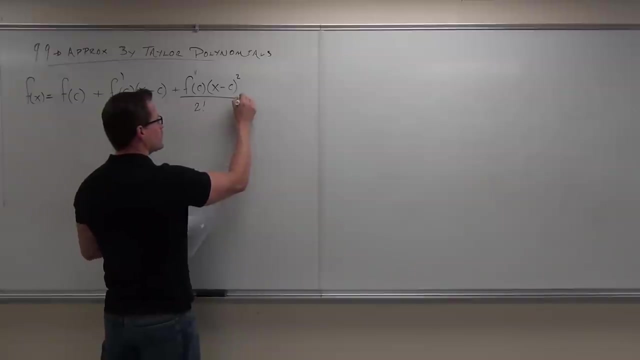 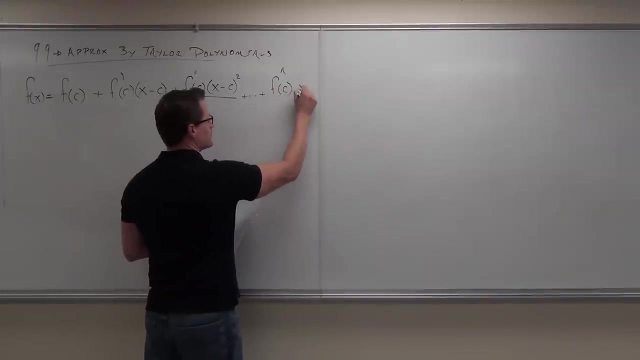 Yes, Plus the second derivative at c, times x minus c to the second, all over 2 factorial plus. and we keep on going until we get to the nth derivative At c, x minus c to the nth, all over n factorial. 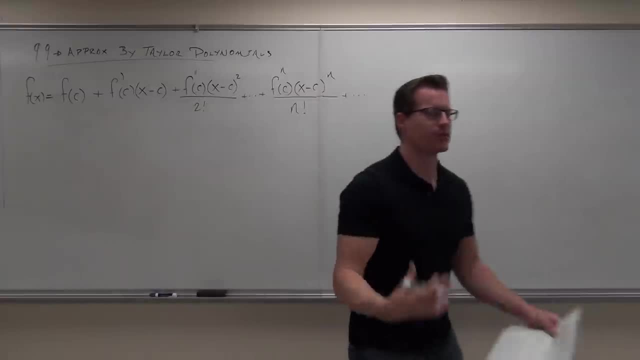 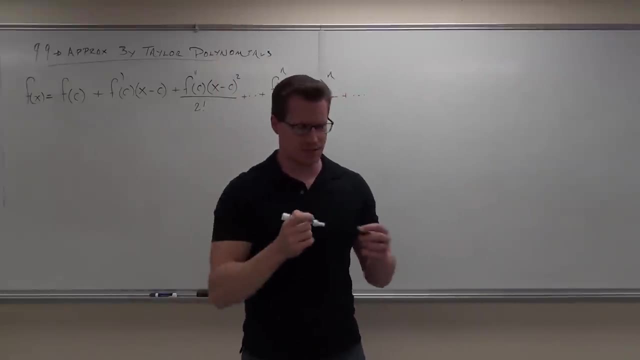 And then this thing keeps on going forever and ever and ever and ever, and that was called a Taylor Series. So show up here with the idea of a Taylor Series. So what we said basically in the last section was: hey, you know what we can represent a function with a Taylor Series or a Maclaurin Series. 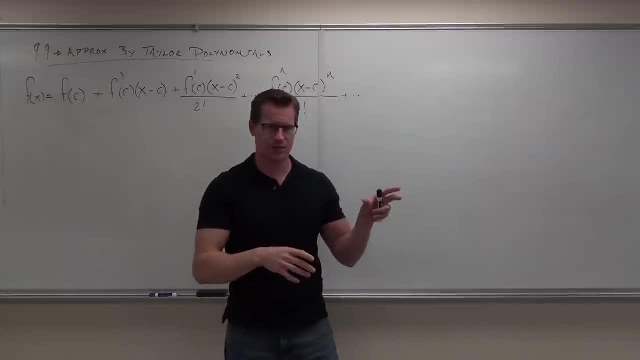 Of course, the only difference between a Taylor Series and a Maclaurin Series is that a Maclaurin Series always has a Taylor Series. So we're going to start with a Taylor Series and a Taylor Series. A Maclaurin Series has a center of what 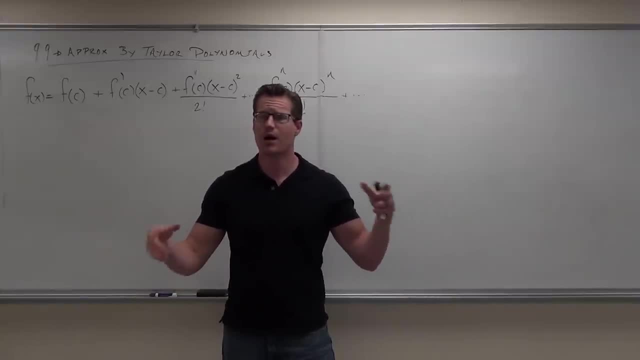 Zero, Very good. A Taylor Series has a center of whatever I want. So a Maclaurin Series is technically a Taylor Series. So this says: hey, you know what we can represent a function with a Taylor Series. 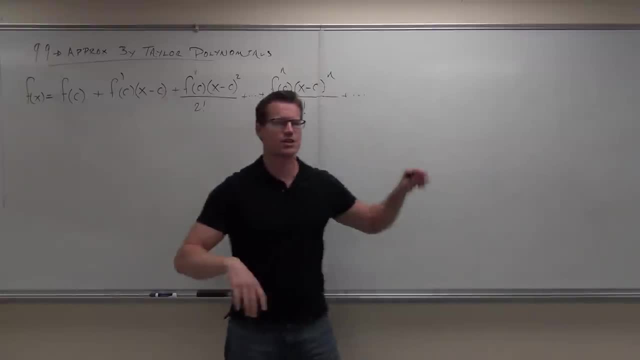 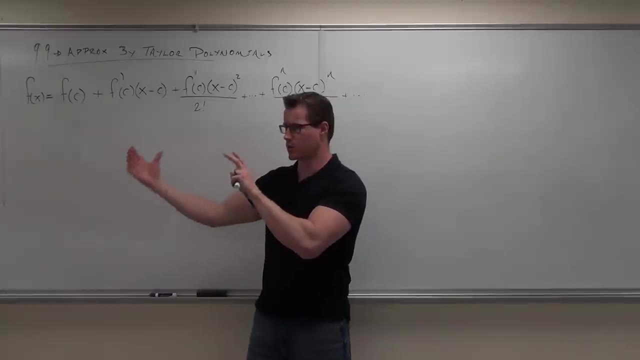 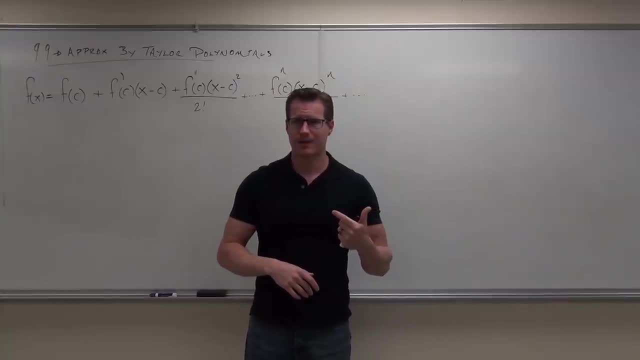 Now here's the idea today. Are you guys ready? Can we ever take a Taylor Series and approximate it forever? Can we do that? Can you just do something forever? Probably not right. You're going to have to end sometime. 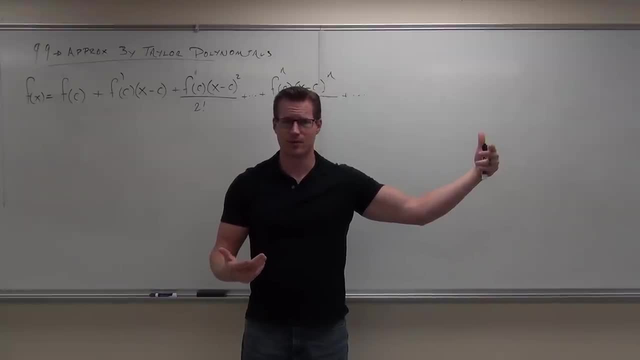 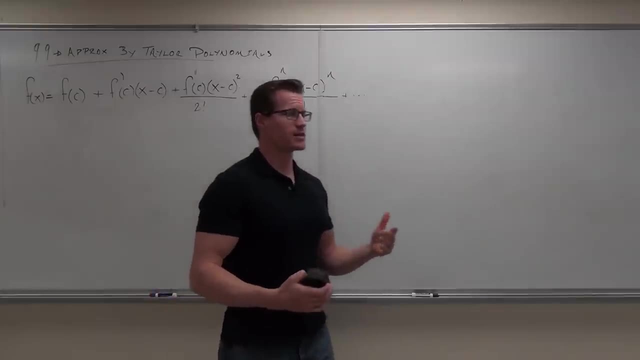 You're going to die, unless you're a vampire, and then you're going to live forever. So you could probably do that, But no, we're not. So here's the idea for today. It says: well, a Taylor Series goes forever. 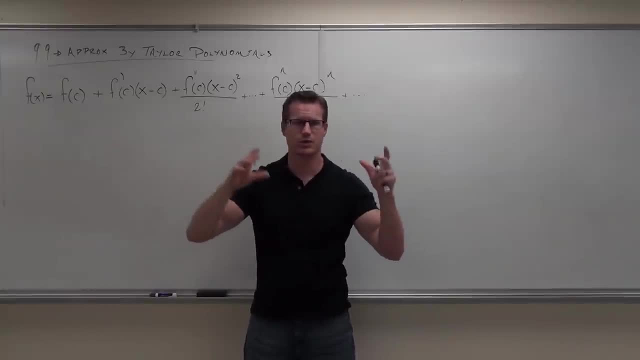 And, since it goes forever, say, okay, it's gonna more closely and closely and closely and closely approximate our function for however far we go. Now here's the idea today. Are you guys ready? Can we ever take a Taylor series and approximate it forever? 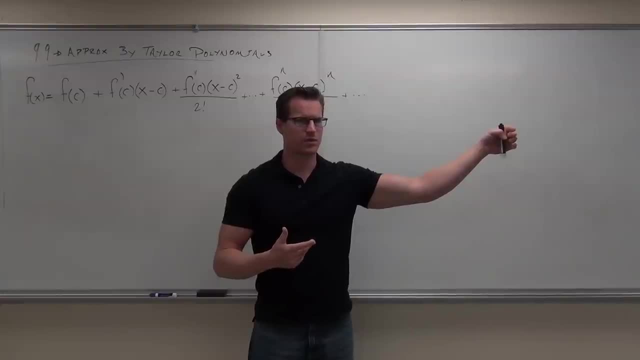 Can we do that? Can you just do something forever? Probably not right. You're gonna have to end sometime, You're gonna die, unless you're a vampire, and then you're gonna live forever. So you could probably- you probably- do that. 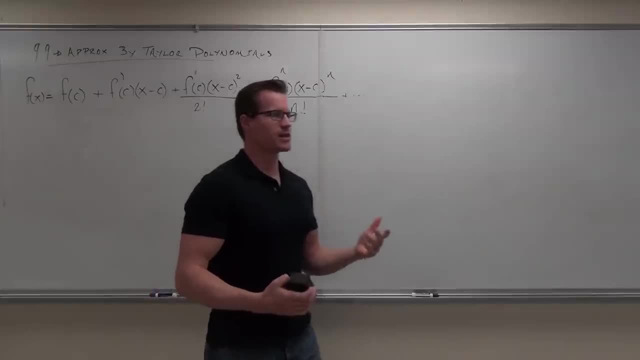 But no, we're not. So here's the idea for today. It says, well, a Taylor series goes forever, A Taylor series goes forever. Let's stop it Right there. Let's stop it at the nth term. So the nth derivative of f. 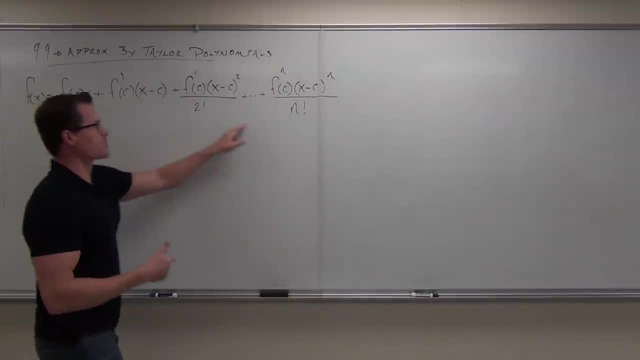 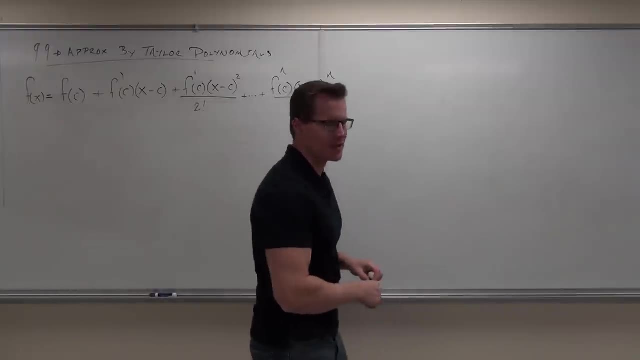 Now here's my question: Is this going to perfectly represent my function? Okay, let me start over Some of you. I lost you. I know that your heads are probably like huh a little bit. You need to wake up right now. 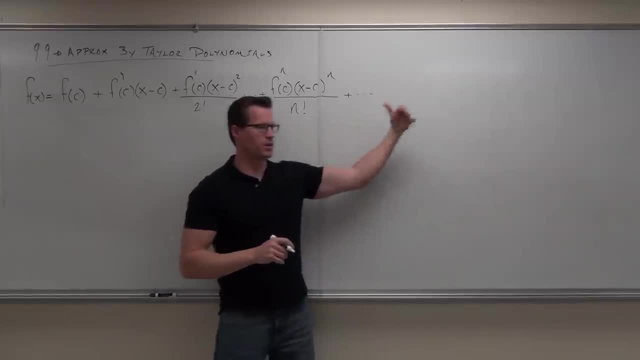 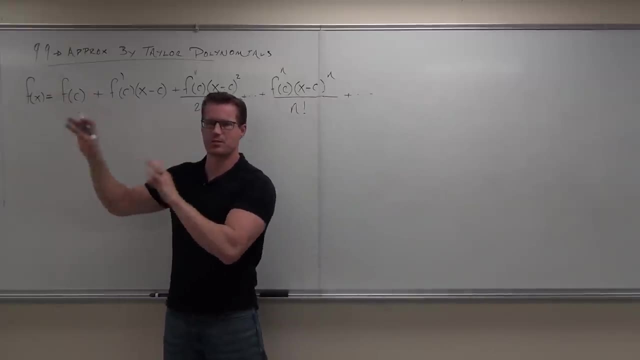 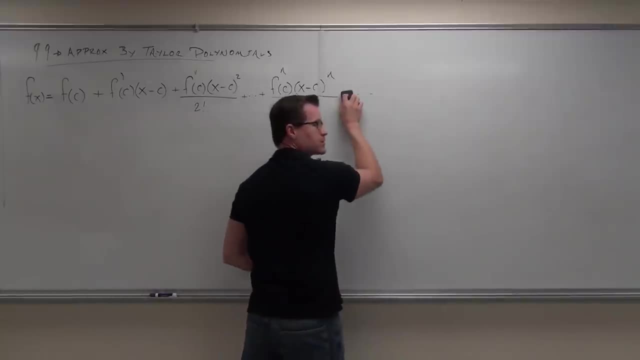 if it goes to infinity. Now, if I stop my Taylor series at a certain point, is it a Taylor series anymore, forever? No, No, it stops at a point. Is that this? whatever we have this expression, we're gonna give it a name in a second. 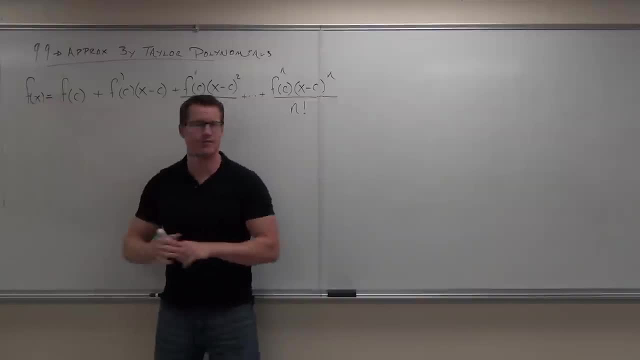 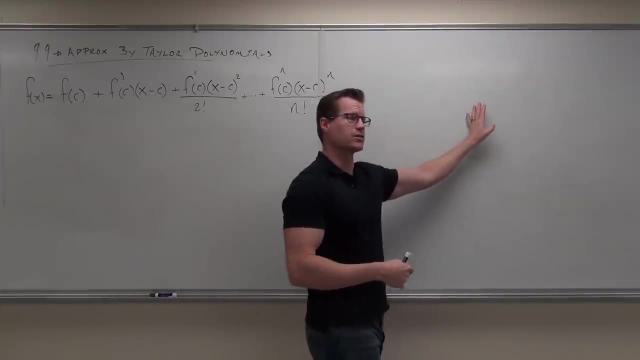 Is this expression going to perfectly represent my function if I stop it after a certain point? No, No. If a Taylor series does represent my function and I don't have the entire Taylor series, then this isn't, then this is not going to perfectly represent this anymore. 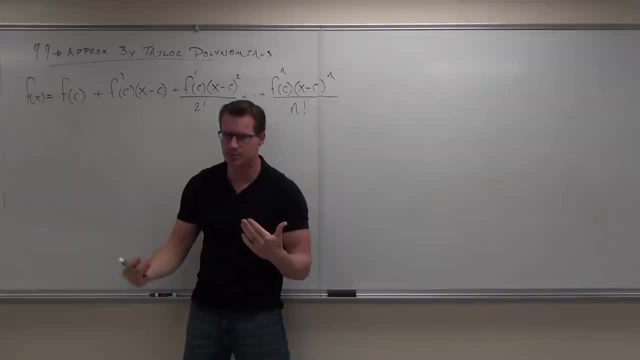 Quick head nod if you understand that idea. I stopped it. It's not the complete thing anymore, So if this is not the complete Taylor series, do you know what I stopped it? I stopped it, that's right. Just making sure you're paying attention, okay. 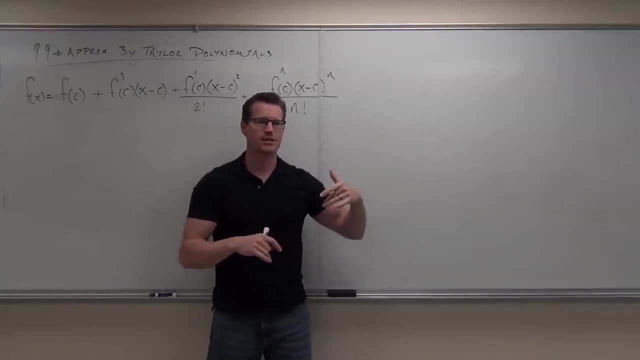 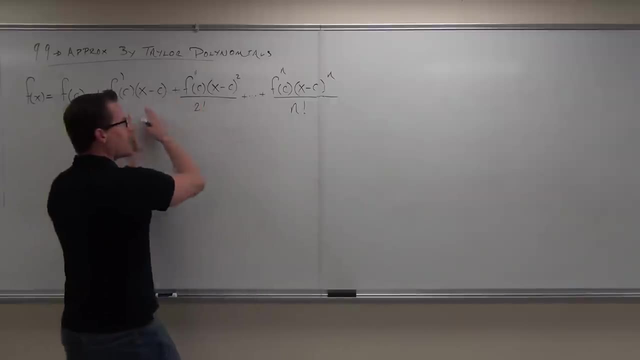 Because I stopped it. it's no longer a Taylor series. But if you notice this, it is a polynomial. Do you guys see it? Mm-hmm, It's a Taylor polynomial. So this thing: when I stop my Taylor series at a certain point, 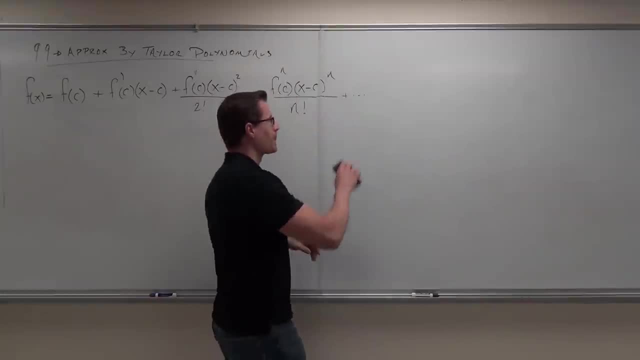 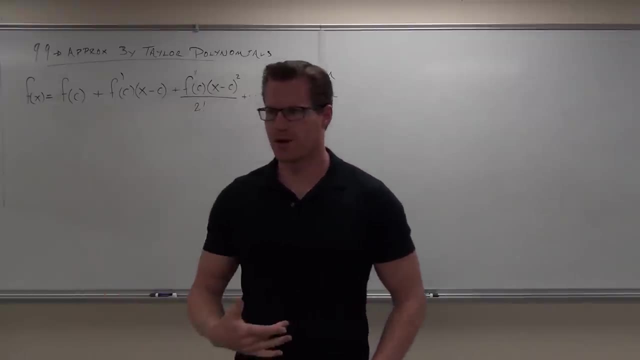 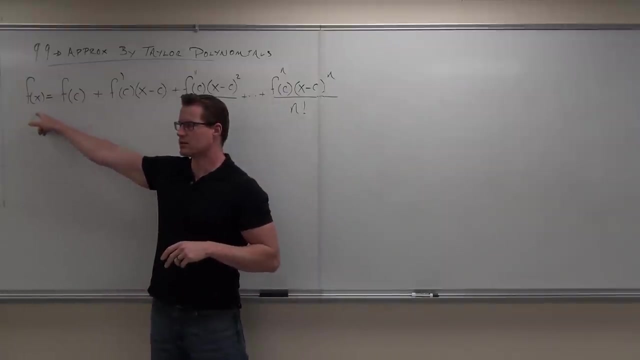 A Taylor Series goes forever. Let's stop it right there. Let's stop it at the nth term. so the nth derivative of f. Now here's my question: Is this going to perfectly represent my function? Okay, let me start over. 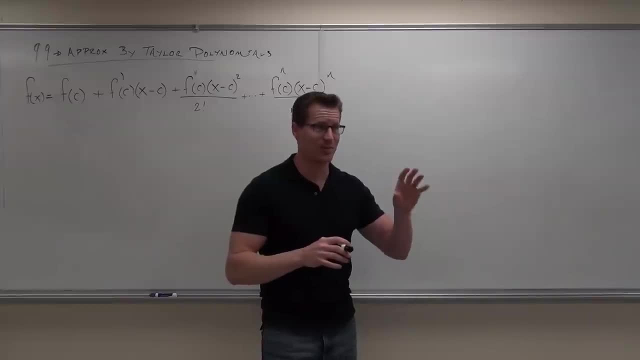 I lost you. I know that your heads are probably like huh a little bit. You need to wake up right now. Do you understand that a Taylor Series goes forever? It goes to this term and it keeps on going and going, and going and going right. 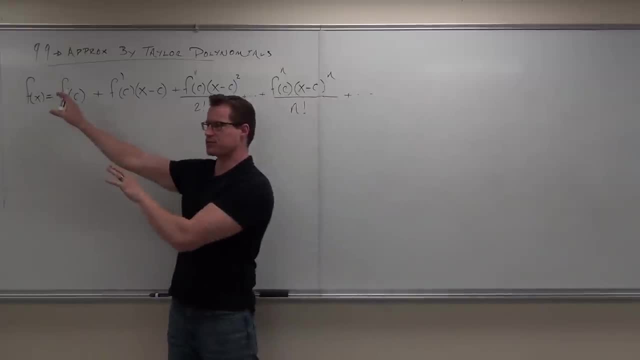 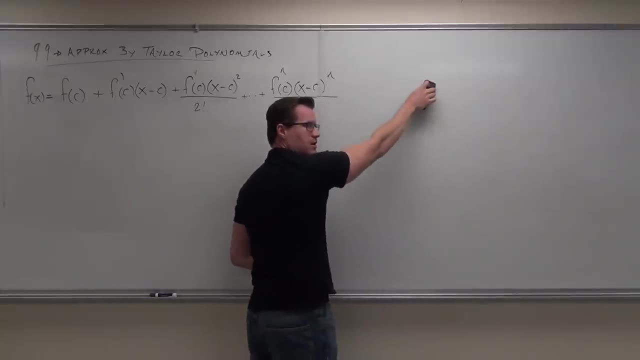 So this would, I'm telling you right now, Would perfectly represent your function. A Taylor Series does represent the function if it goes to infinity. Now, if I stop my Taylor Series at a certain point, is it a Taylor Series anymore, forever. 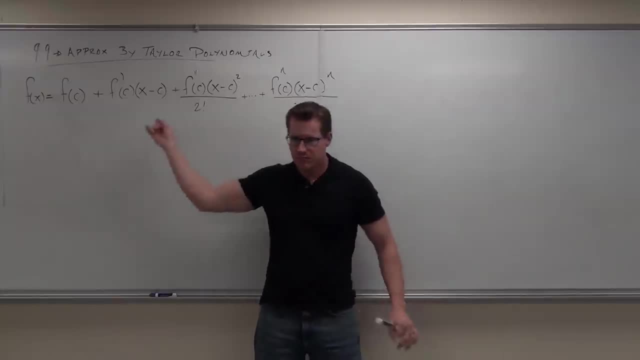 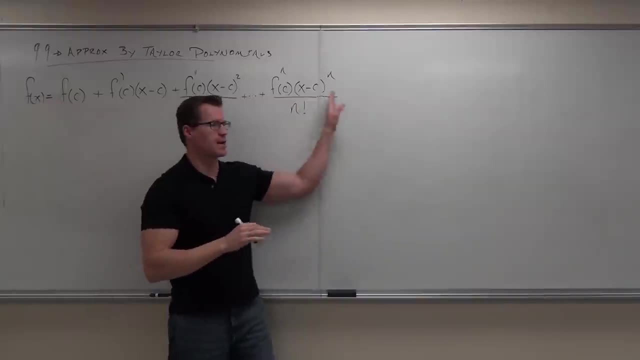 No, No, it stops at a point. Is that this? whatever we have this expression, we're going to give it a name in a second. Is this expression going to perfectly represent my function if I stop it after a certain point? 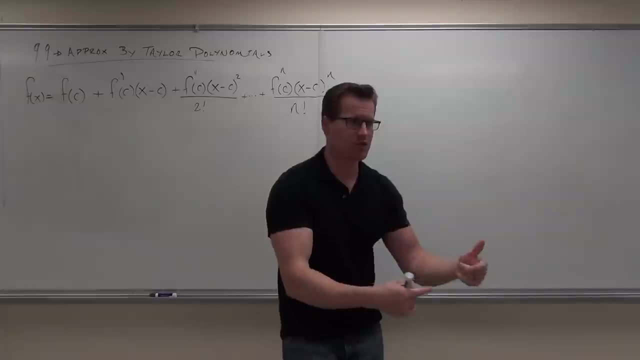 No, No. If a Taylor Series does represent my function and I don't have the entire Taylor Series, then this is not going to perfectly represent this anymore. Quick head nod if you understand that idea. I've stopped it. It's not the complete thing anymore. 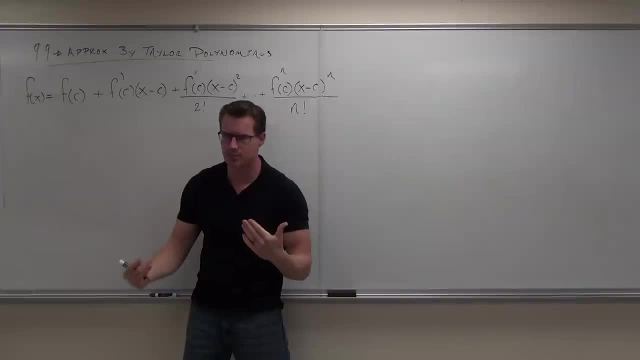 So if this is not the complete Taylor Series, do you know what I stopped it? I stopped it, That's right. Just making sure you're paying attention, okay, Because I stopped it. it's no longer a Taylor Series. 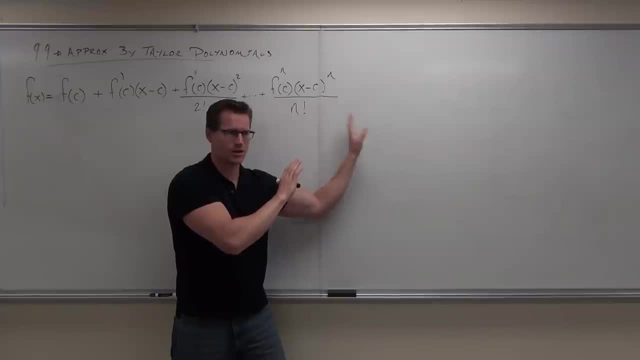 But if you notice this, it is a polynomial. Do you guys see it? Uh-huh, It's a Taylor polynomial. So this thing, when I stop my Taylor Series, it stops at a point. I stop at a point. 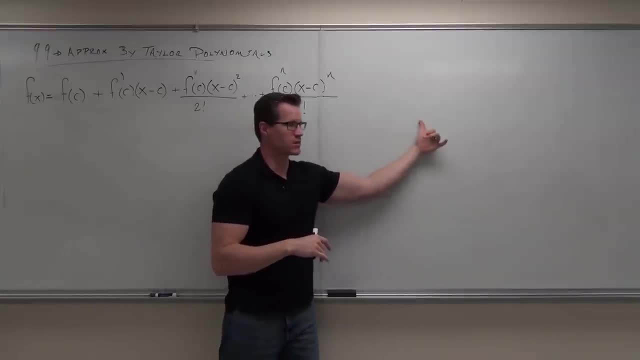 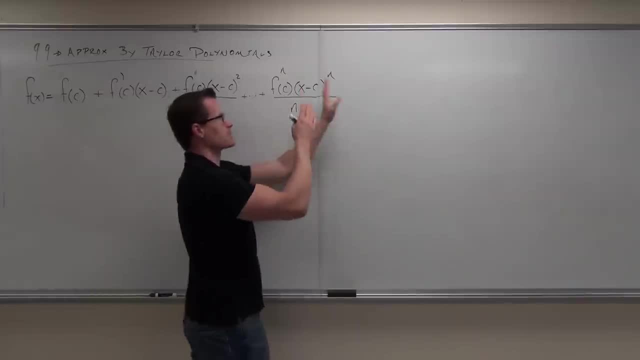 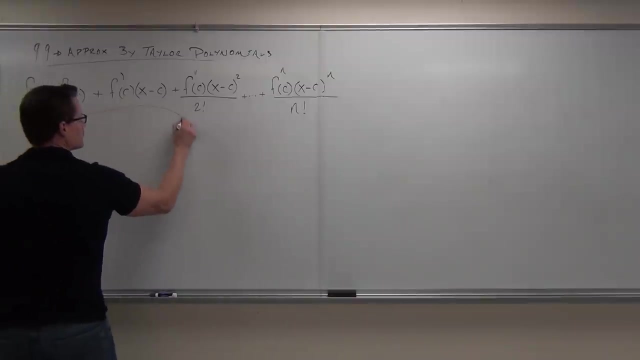 Uh-huh, It's a Taylor Polynomial. So this thing, when I stop my Taylor Series at a certain point, what I end up getting is a Taylor Polynomial of the nth degree. So this is the nth degree Taylor Polynomial. Showfans, are you okay with the terminology here? 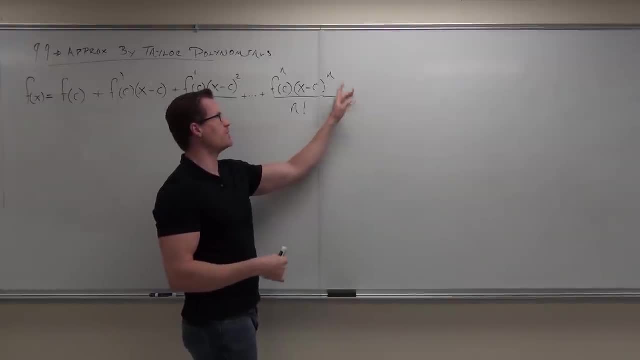 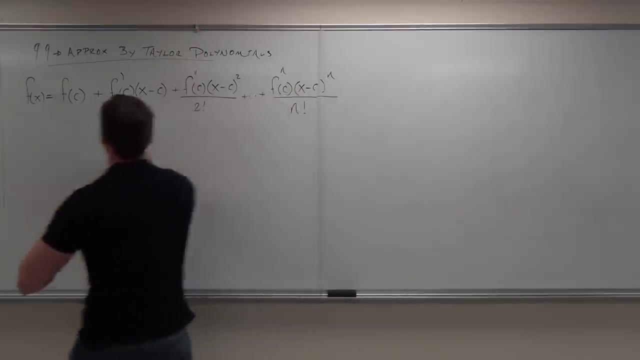 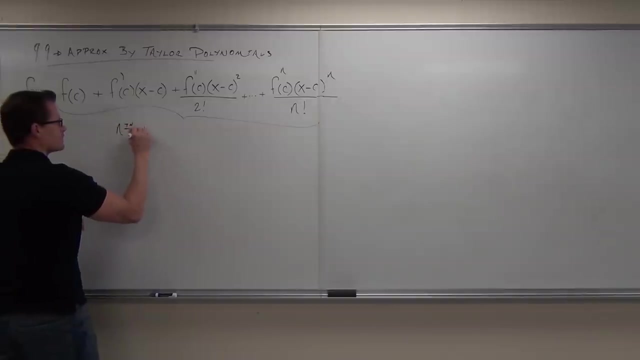 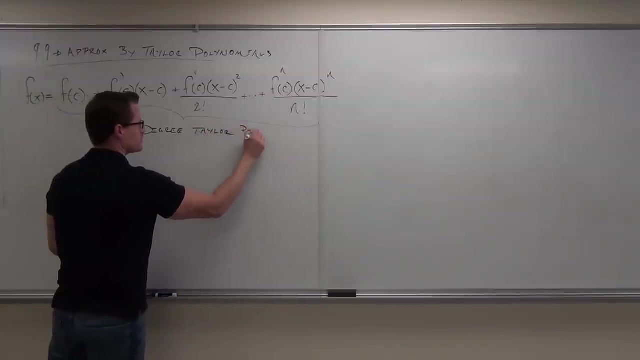 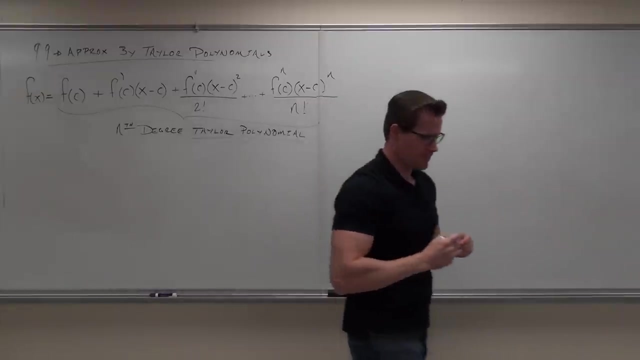 what I end up getting is a Taylor polynomial of the nth degree. So this is a nth degree Taylor polynomial. I'll show if you guys feel okay with the terminology here. So this right here is my nth degree Taylor polynomial. Now here's the issue. 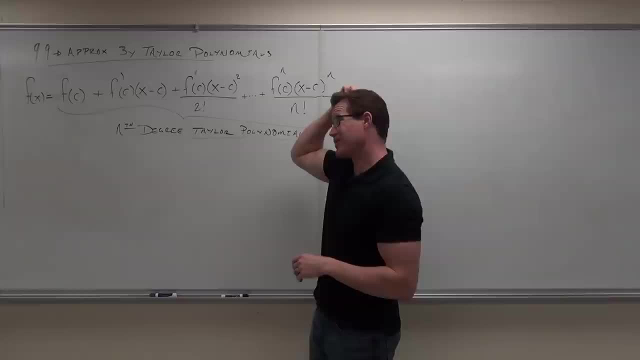 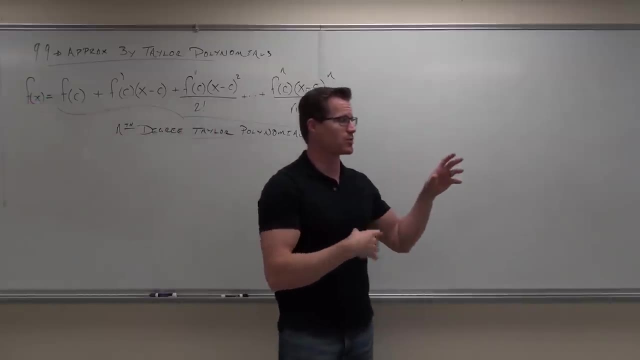 We just talked about it and said: well, you know what Mr Leonard said, that if I had a Taylor series, yeah, it'd perfectly represent my function. But I don't have it anymore. I cut it short. Now I've got a Taylor polynomial. 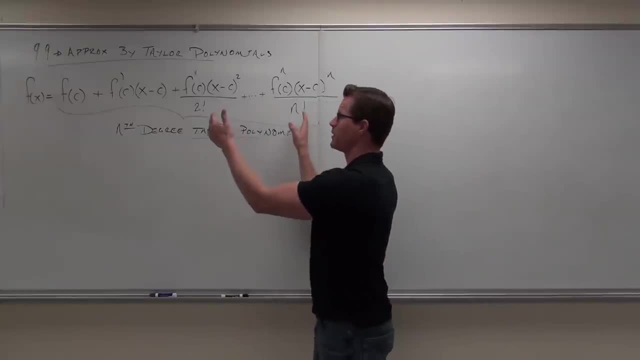 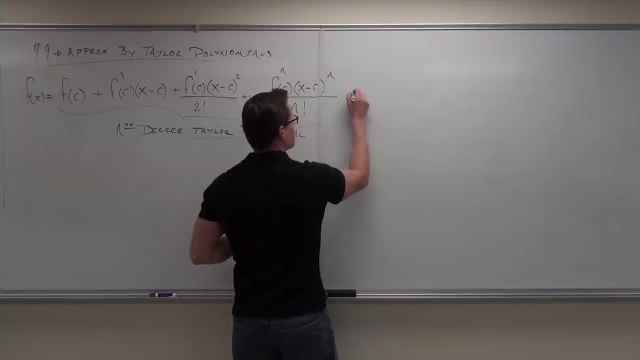 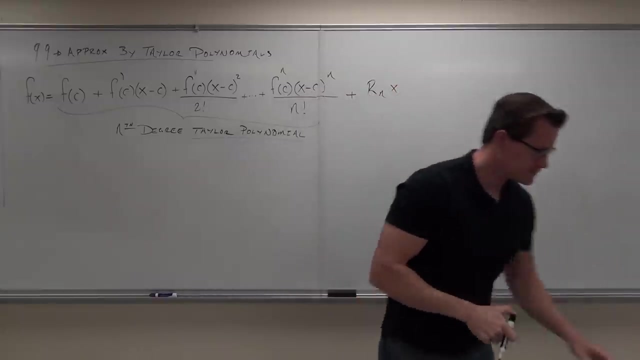 Well, the problem is there's going to be some difference between my Taylor polynomial and my function itself. Does that make sense to you? So, basically, I've got this little extra. I've got this little extra. OK, Over here. 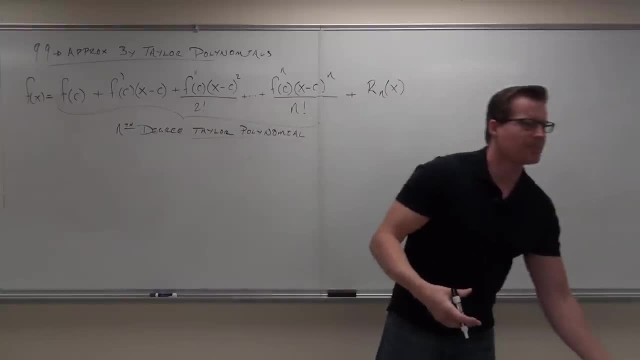 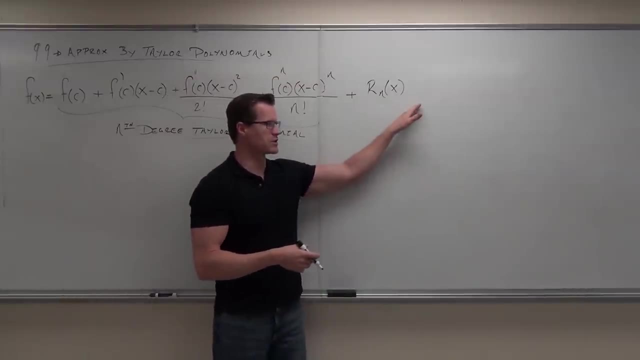 Over here. This little extra would be the. it's called the remainder of your Taylor polynomial. It really represents the rest of your Taylor series. that would make this thing valid. Does that make sense to you? So it goes OK. so imagine this. 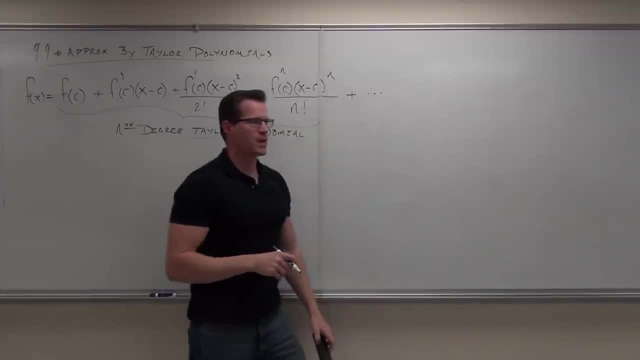 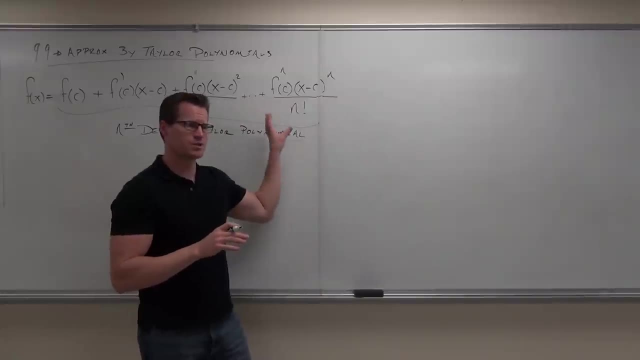 I'm going to start over from the beginning. My Taylor series goes forever And we say: wait a minute, Let's cut it short. I no longer have a Taylor series. This thing no longer perfectly represents my function. We call it a Taylor polynomial. 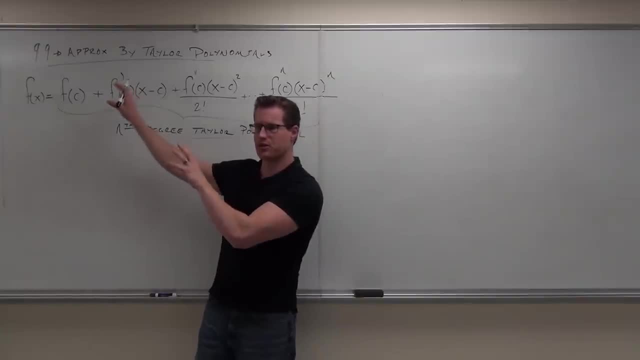 Now, a Taylor polynomial is not going to exactly represent your function, But it's going to be a pretty close approximation. In fact, if I just have this little remainder, this little extra, what we can say is that the Taylor polynomial plus this little extra. 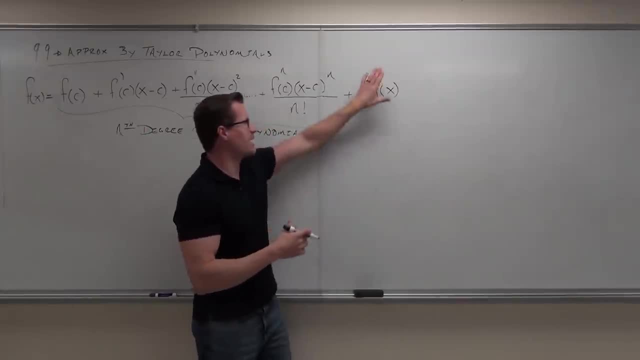 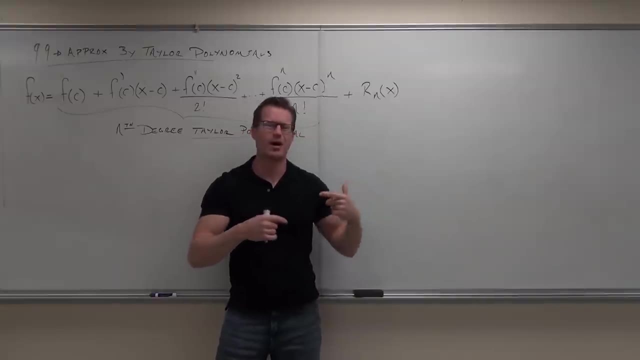 would make your function. So it's basically saying: hey, this thing's just missing a little piece, This little piece that's your error, That's how close you can get to represent your function by your Taylor polynomial, This little extra piece that remainder. 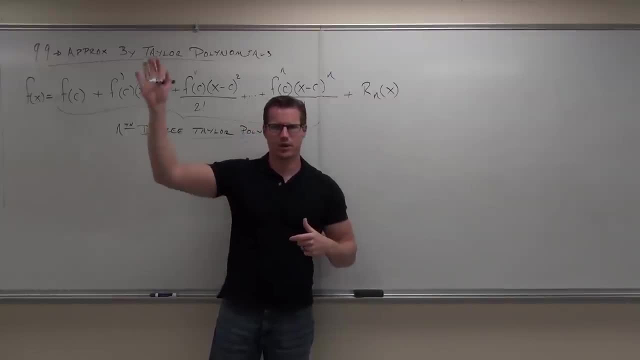 of your Taylor polynomial. that's your error right there. So you guys feel OK with the idea. So is it an entire Taylor series anymore? No, We cut it short, We got a Taylor polynomial. We say, hey, you know what? 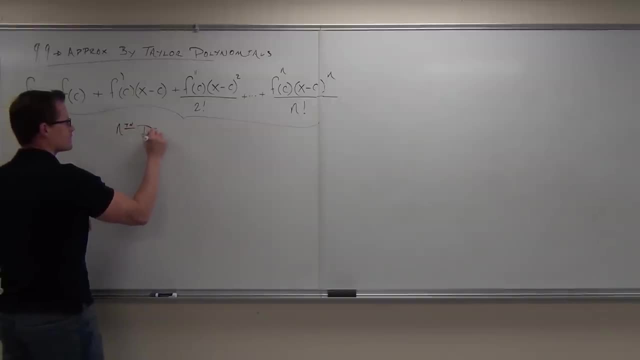 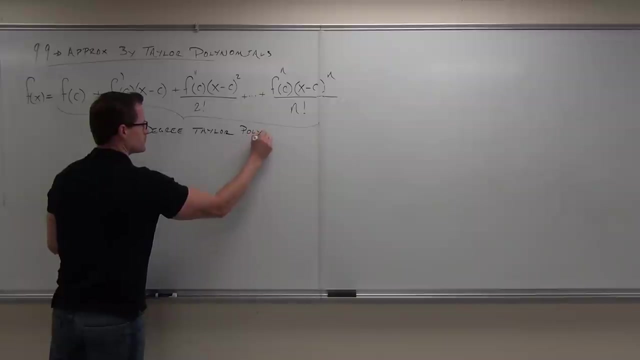 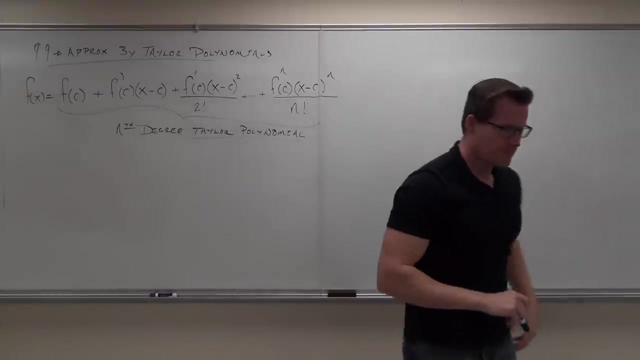 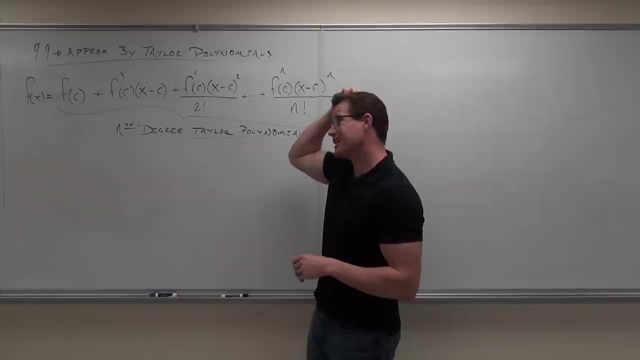 So this right here is my nth degree Taylor Polynomialreath: Tha d, e, f. Now here's the issue. We just talked about it and said- well, you know what Mr Leonard said, that if I had a Taylor series, yeah, it'd perfectly represent my function. 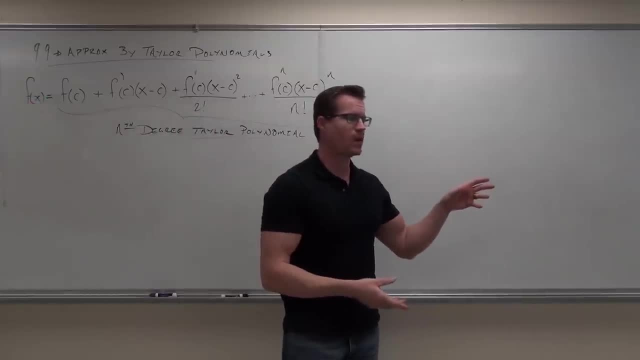 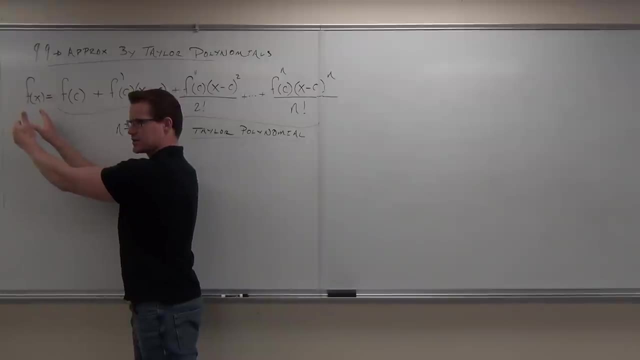 But I don't have it anymore. I cut it short. Now I've got a Taylor polynomial. Well, the problem is, there's going to be some difference between my Taylor polynomial and my function itself. Does that make sense to you? So, basically, I've got this little extra. 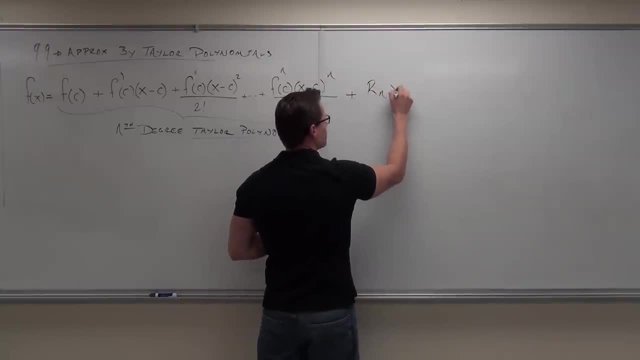 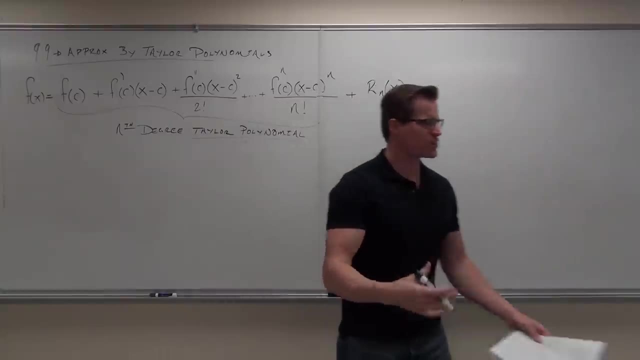 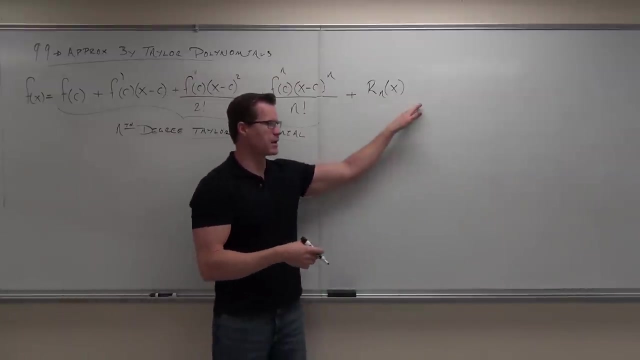 I've got this little extra over here. This little extra would be the. it's called the remainder of your Taylor polynomial. It really represents the rest of your Taylor series. It would make this thing valid. Does that make sense to you? So it goes okay. so imagine this. 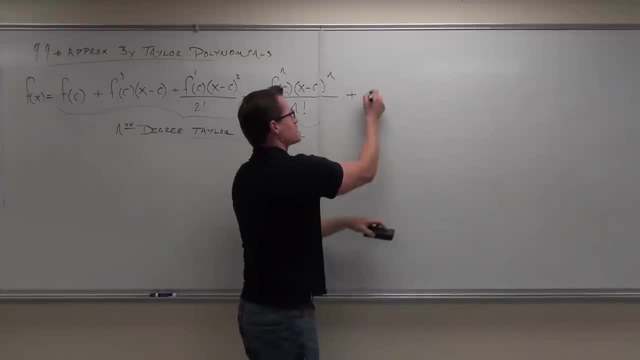 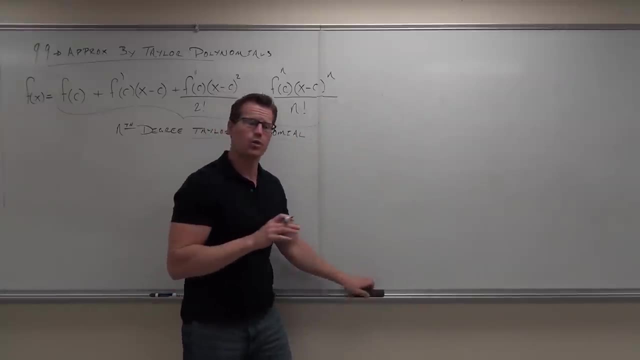 I'm going to start over from the beginning. My Taylor series goes forever And we say: wait a minute, Let's cut it short. I no longer have a Taylor series. This thing no longer perfectly represents my function. We call it a Taylor polynomial. 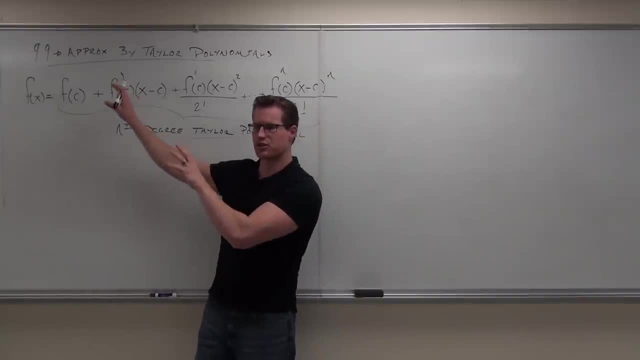 Now, a Taylor polynomial is not going to exactly represent your function, but it's going to be a pretty close approximation. In fact, if I just have this little remainder, this little extra, Okay, What we can say is that the Taylor polynomial plus this little extra would make your function. 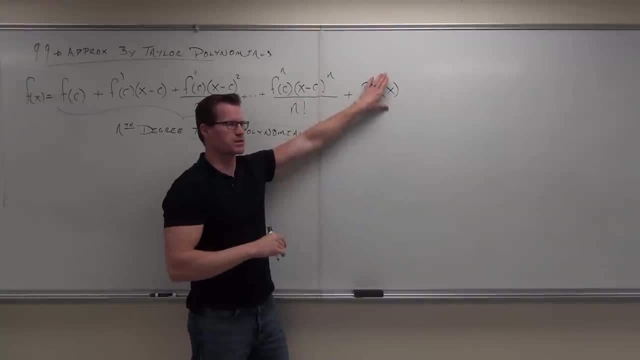 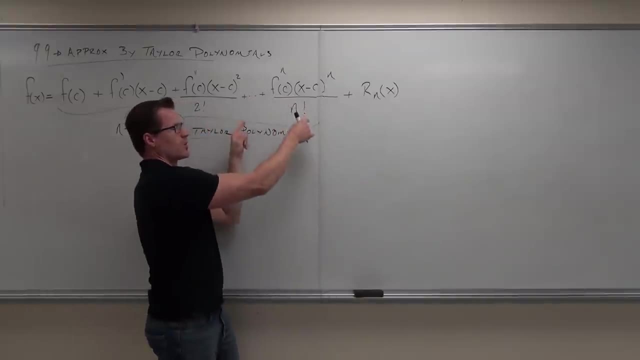 So it's basically saying: hey, this thing's just missing a little piece. This little piece, that's your error, That's how closely, or how close you can get to represent your Taylor polynomial, sorry, as representing your function by your Taylor polynomial. 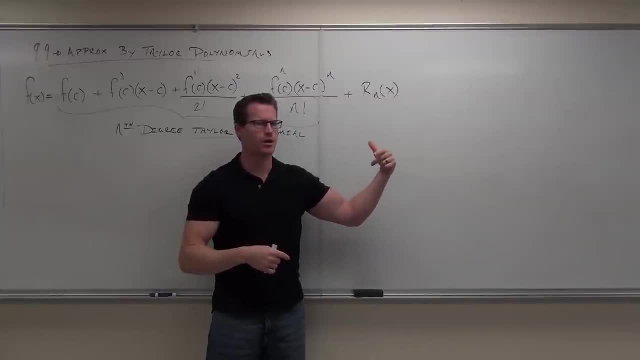 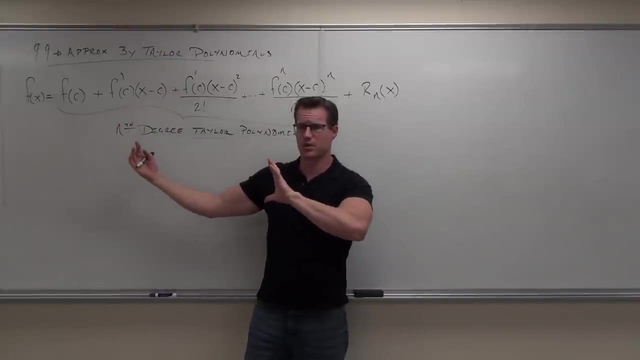 This little extra piece, that remainder of your Taylor polynomial. that's your error right there. So, if you guys feel okay with the idea, So is it an entire Taylor series? No, we cut it short, We got a Taylor polynomial. We say, hey, you know what that Taylor polynomial? it's pretty close to this thing, but it's not. 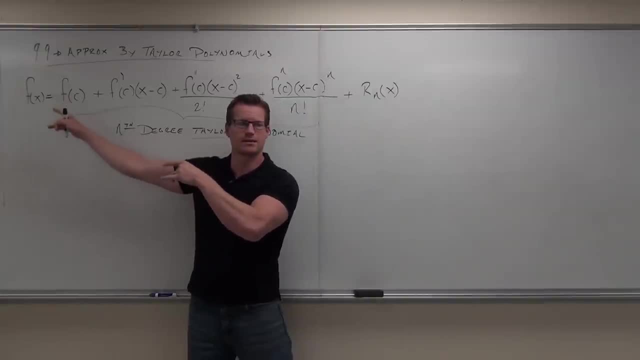 That Taylor polynomial. it's pretty close to this thing, But it's not exactly the same thing as their function. We add a little bit of error, saying it's not exactly the same, but that little piece right there, that remainder is the error. 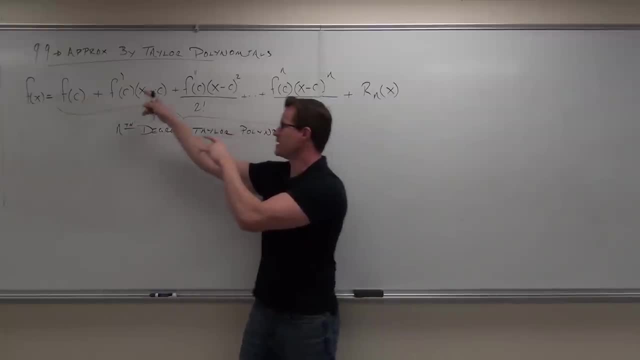 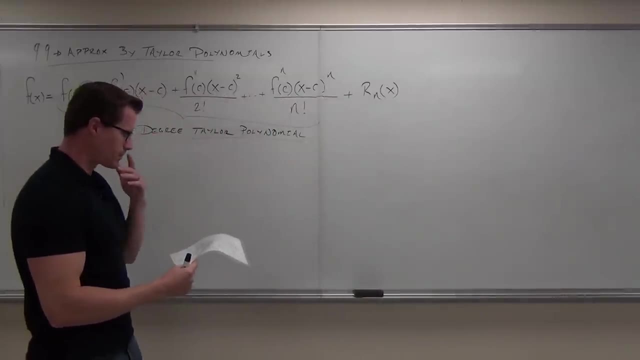 That's how close you can make your function by representing it with a Taylor polynomial. Now what I'd like to do is tell you explicitly what this error is. So it says- and I don't know if you need me to write this down- 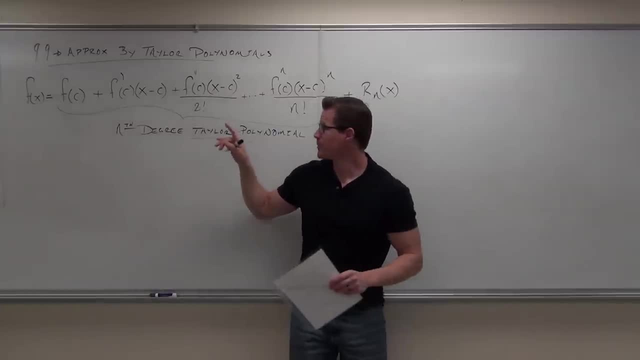 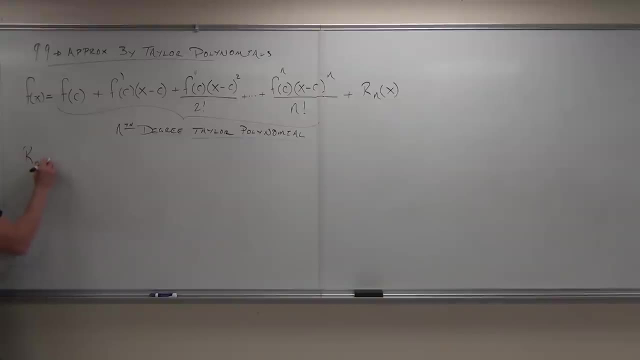 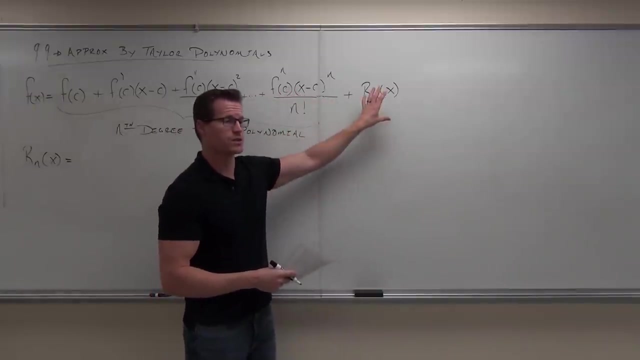 for you. but this says that your function can be represented by a Taylor polynomial, this nth degree Taylor polynomial plus some sort of an error. Now here's our error. Let's look a little more closely at this. If we were to just continue my Taylor series? 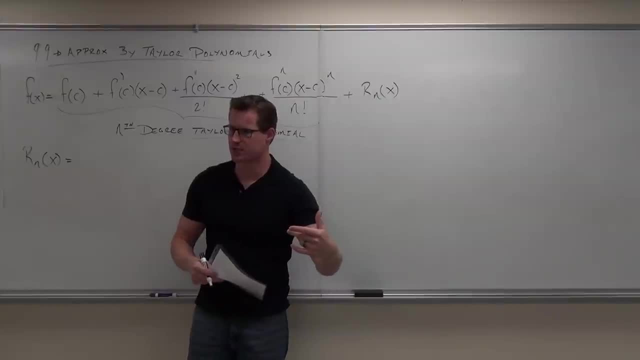 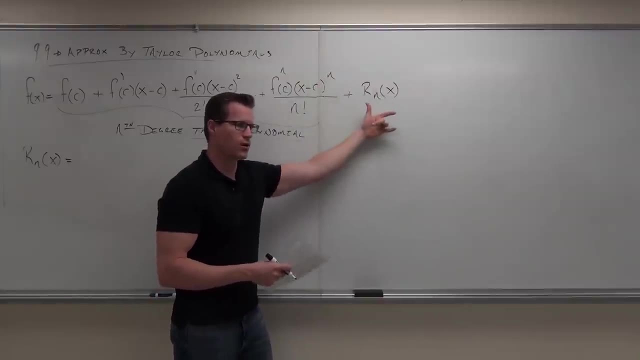 Now keep in mind this is no longer a Taylor series. OK, We have cut it short. Does that make sense to you? We've cut it short, So this is now a Taylor polynomial. and the error? The error, though, if you just continued this. 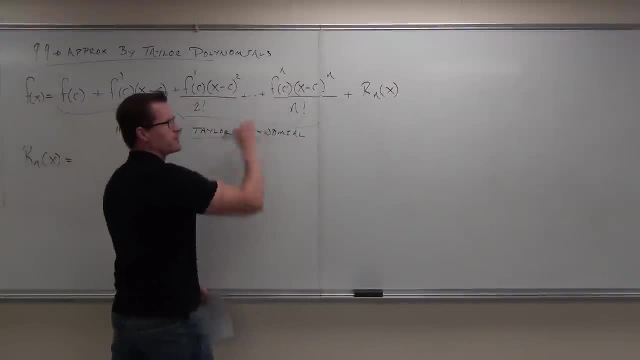 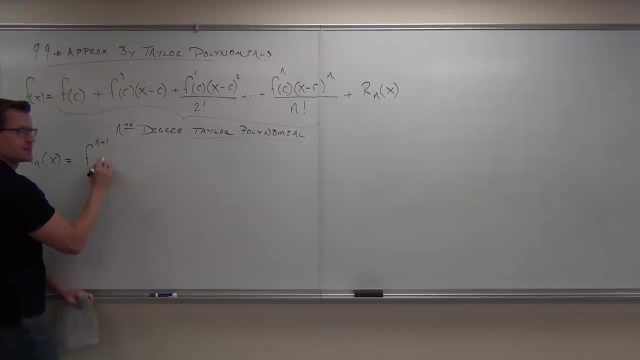 this would be well, what would the next derivative be? That's the n plus 1.. Yep, the n plus 1 derivative at 6 and 3.. Now, that's where we're going to make a little change here. 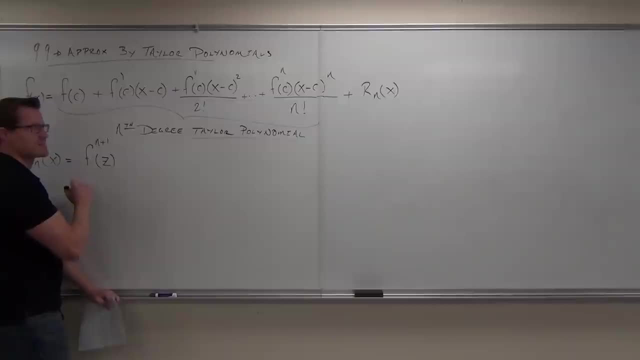 We're going to say it's at z, And I'll tell you why in a second. So keep in mind that's a z, not a c, x minus c to the. what power is that going to be? n plus 1.. 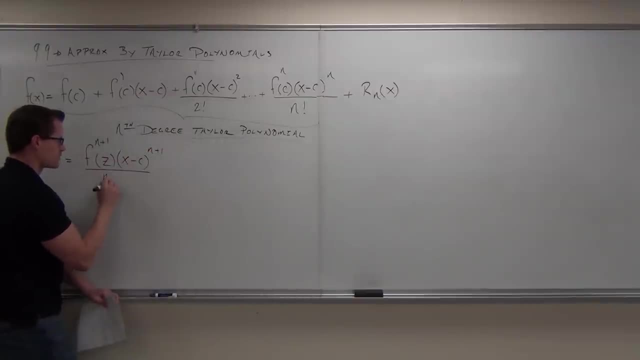 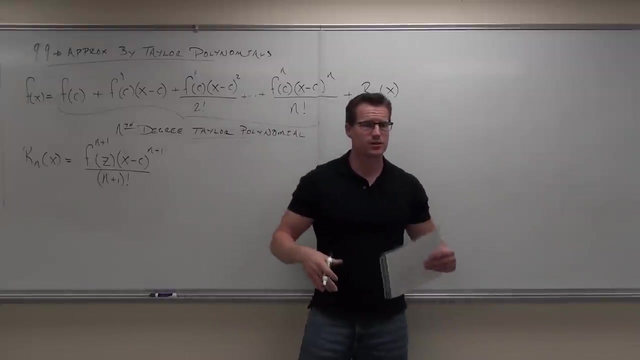 Very good All over, what everybody n plus 1. Perfect, This is the rest. So this is going to represent the rest of our Taylor series, which we kind of cut off. So we're saying, hey, you know what? 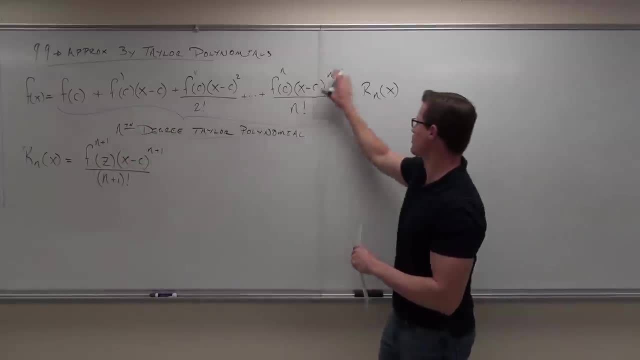 That is the remainder We're going to get if I cut off my Taylor series. you know I have my Taylor polynomial And then I'm going to have this little extra. The rest of my Taylor series is represented by this piece. 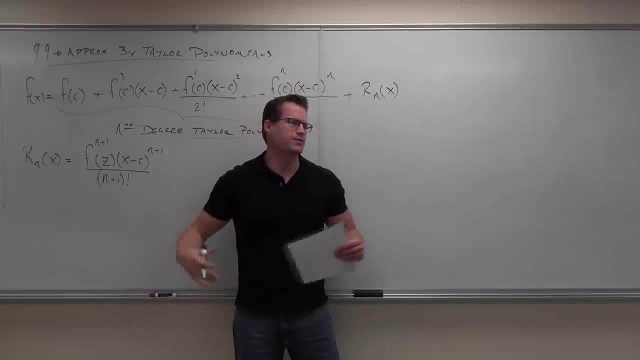 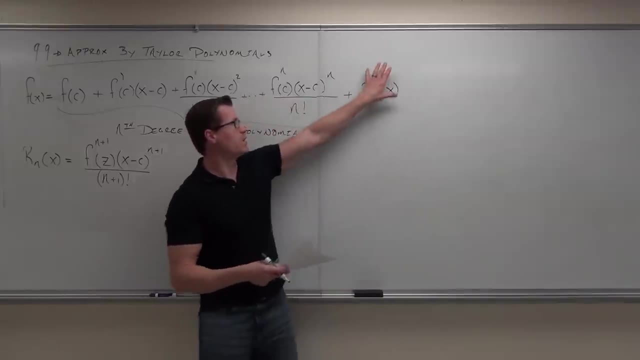 I'm not going to prove it. You can look up the proof if you want to. You can take my word for it right now that we can do this. The logic behind it is that if you cut a Taylor series short, it no longer perfectly represents your function. 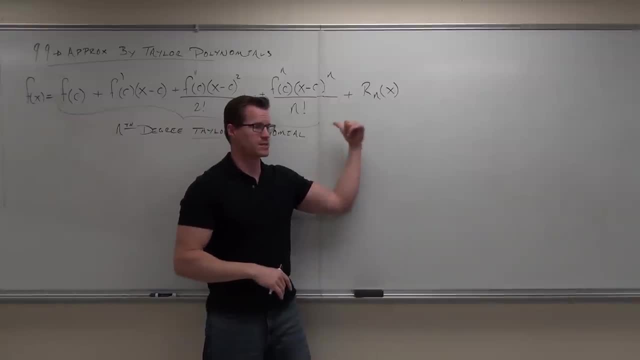 exactly the same thing as their function. We add a little bit of error, saying it's not exactly the same, but that little piece right there, that remainder, is the error. That's how close you can make your function by representing it with a Taylor polynomial. 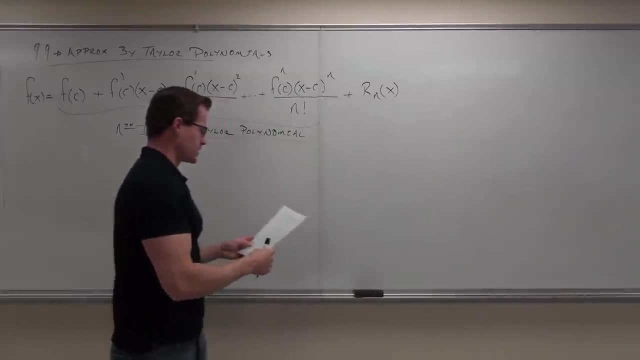 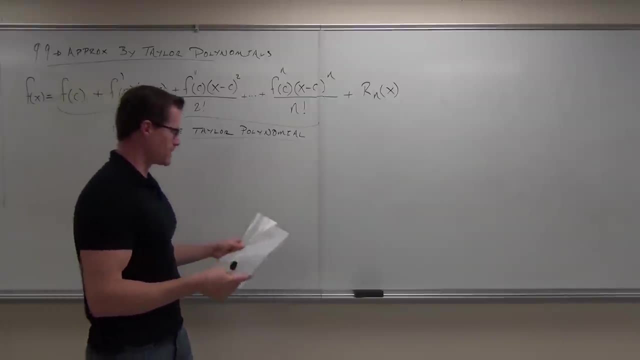 Now what I'd like to do is tell you explicitly what this error is. So it says: I don't know. It says I don't know if you need me to write this down for you, but this says that your function can be represented by a Taylor polynomial, this nth degree Taylor polynomial plus some. 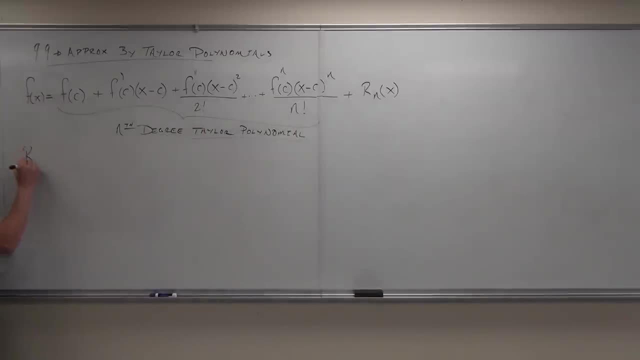 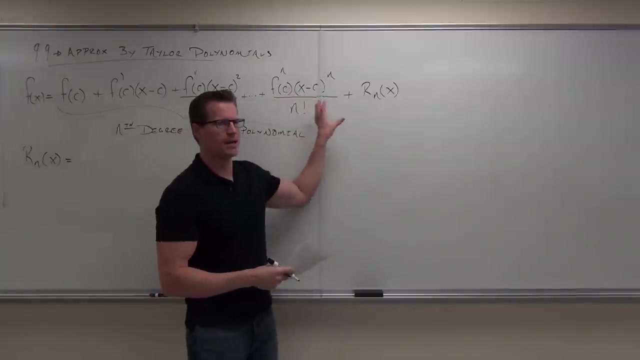 sort of an error. Now, here's our error. Let's look a little more closely at this. If we were to just continue my Taylor series now? keep in mind, this is no longer a Taylor series. okay, We have cut it short. 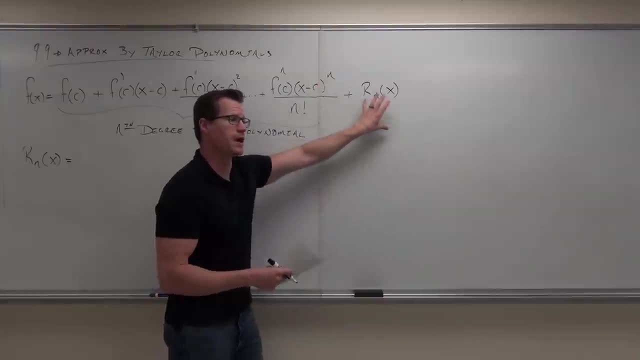 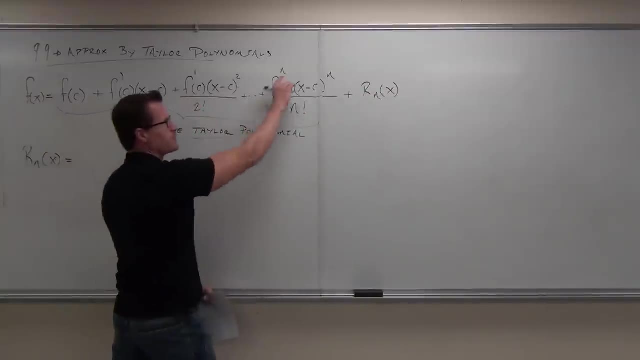 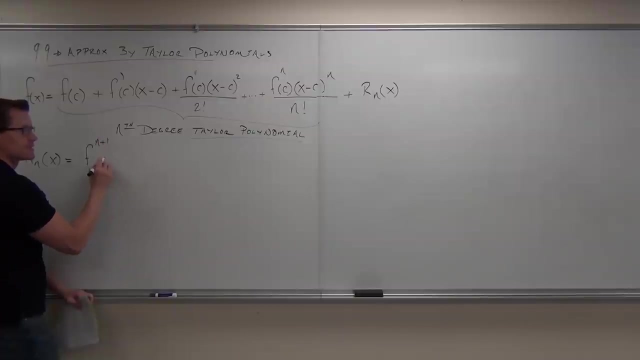 Does that make sense to you? We've cut it short, So this is now a Taylor polynomial, and the error The error, though. If you just continued this, this would be well. what would the next derivative be? Yep, the n plus 1 derivative at. 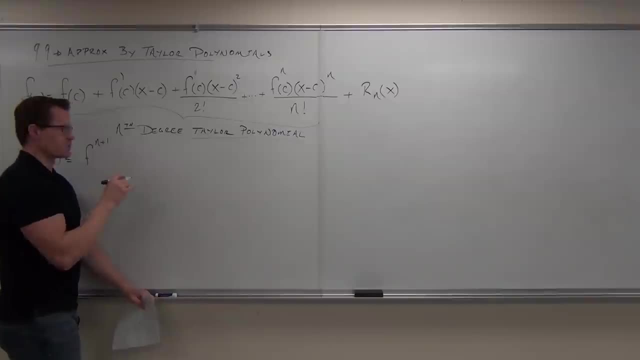 C. Now that's where we're going to make a little change here. We're going to say it's at z, And I'll tell you why in a second. so keep in mind that's a z, not a c. 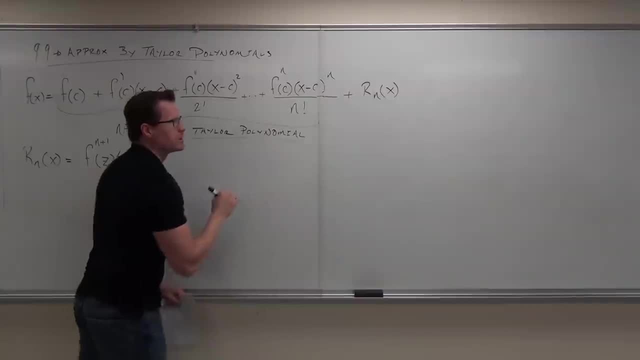 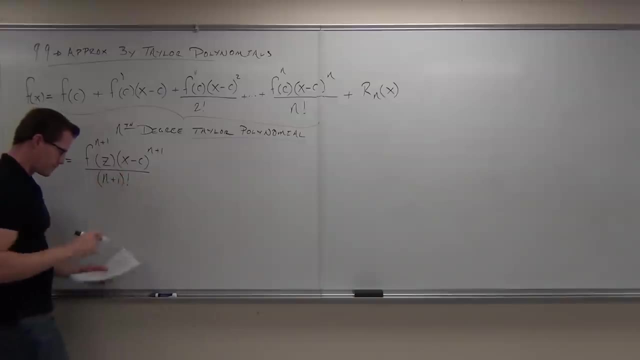 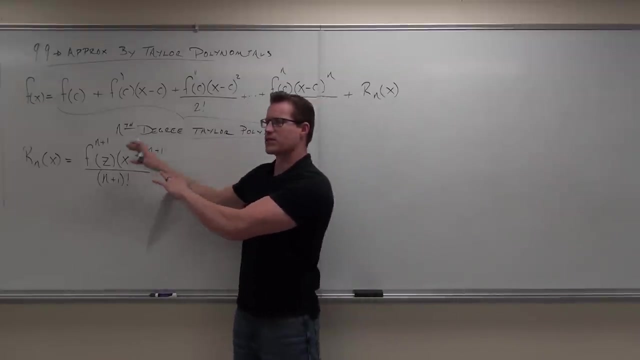 X minus c to the. what power is that going to be? N plus 1.. Very good, All over what everybody? N plus 1.. Yeah, perfect, This is the rest. So this is the. this is going to represent the rest of our Taylor series, which we kind. 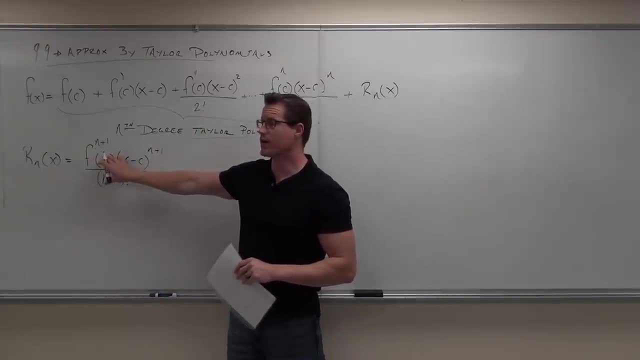 of cut off. So we're saying, hey, you know what That is the remainder that we're going to get if I cut off my Taylor series. you know, I have my Taylor polynomial and then I'm going to have this little extra. 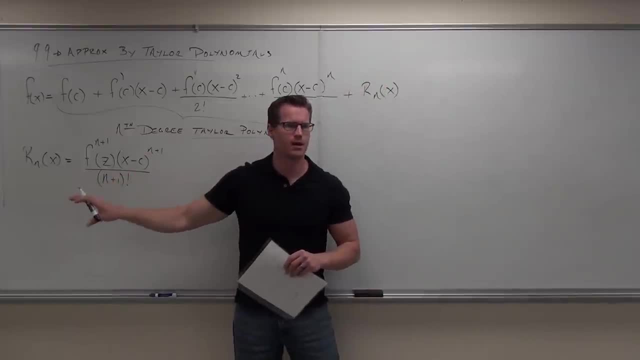 The rest of my Taylor series is represented by this piece. I'm not going to prove it. You can look up the proof if you want to. you know- kind of take my word for it right now- that we can do this. The logic behind it is that if you cut a Taylor series short, it no longer perfectly represents. 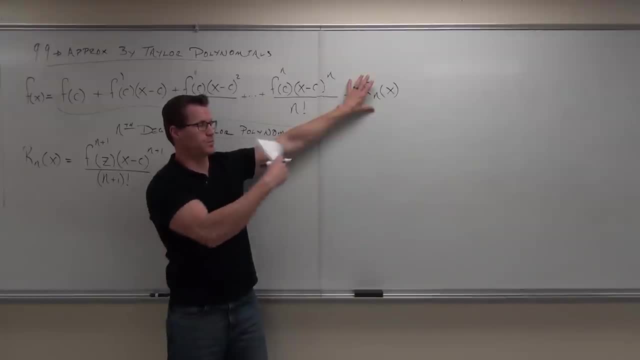 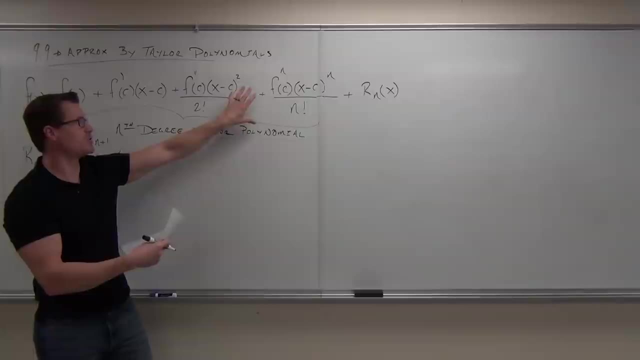 your function A Taylor series would. So we call that place where you cut it off. That's the end of our Taylor polynomial. Now there's going to be some difference between the Taylor polynomial and your function. We say, if I add a little bit to it, then I can make it exactly the same, exactly the. 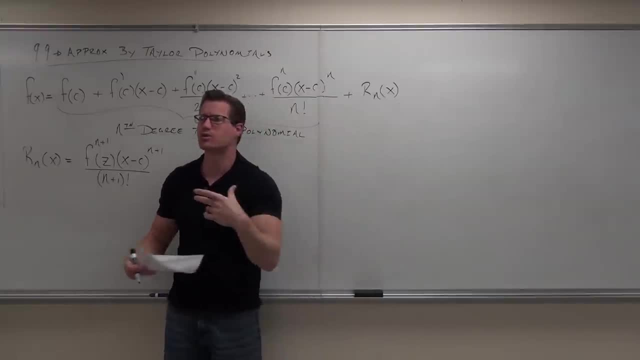 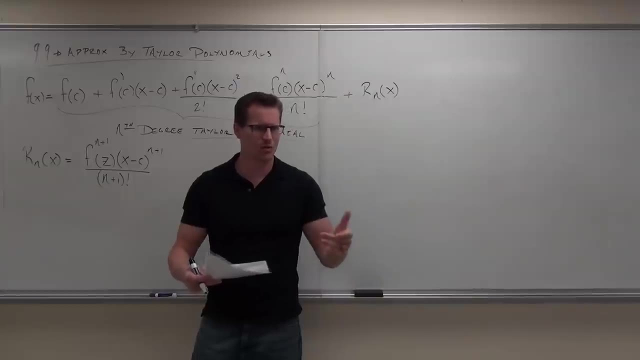 same. That's your error. We you're going to use this a little bit to approximate how close, to say how close our approximation is to our actual function. Have I made sense of this at all for you? It's going to make a little more sense when we go through an example too. 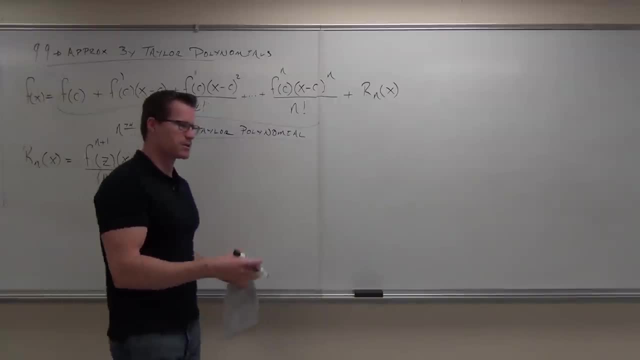 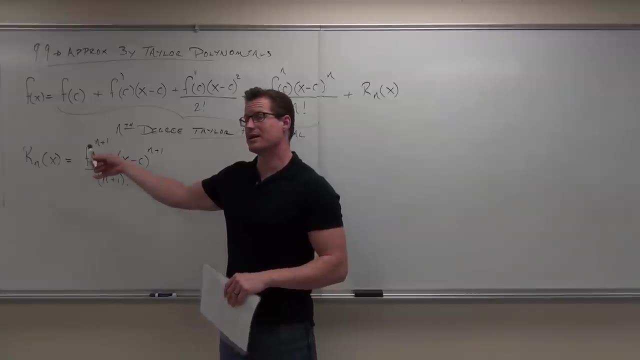 So basically, we're taking part of a Taylor series. as an approximation, Now let's talk about the z, That z right there, that z is some number between c, c, the points you're using, and x, the points you're trying to approximate. 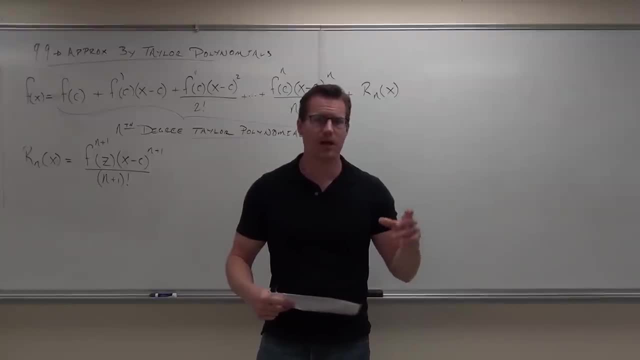 We get to pick what z is, and we're going to do this in a minute- Z You're going to pick z. You get the largest error. Are you listening? You don't want to underestimate your error. You want to overestimate it. if that's the case, 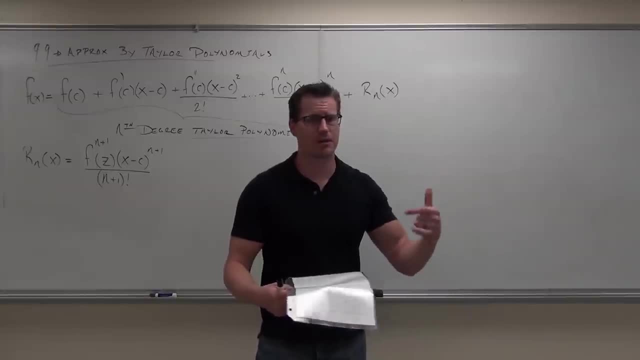 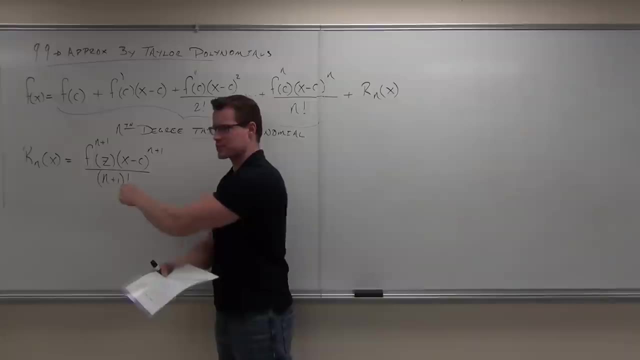 You don't want to underestimate it. So we get to pick z- Z is some point between c and x- between the points you're using and the points you're trying to approximate. And let me illustrate that right now with an example. Are you guys ready for an example? 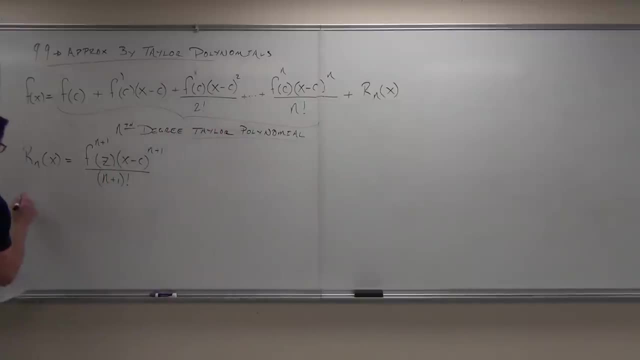 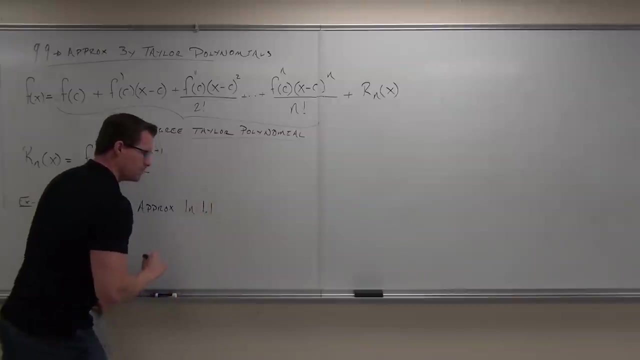 Okay, So here's what we're going to do. Let's say we've got a function, Our function is ln, x, And what we're going to do is we're going to approximate ln of 1.1.. Now, if you're thinking, wait a minute, didn't we just kind of do this in the last section? 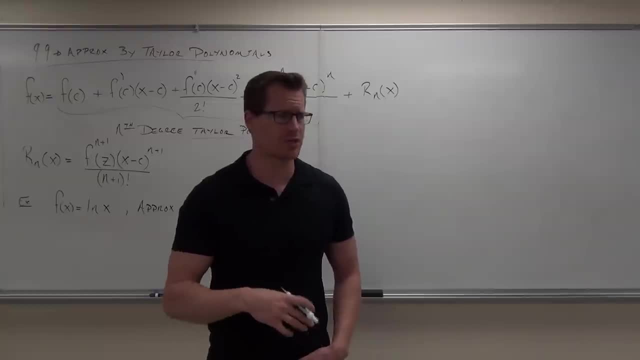 Didn't we have these Taylor series where we could approximate and find out end points, all this stuff for interval? Well, we did that right. Well, but that took a long time correct. This is kind of like a shortcut. This is saying, well, let's approximate, but maybe we don't have to find the entire Taylor. 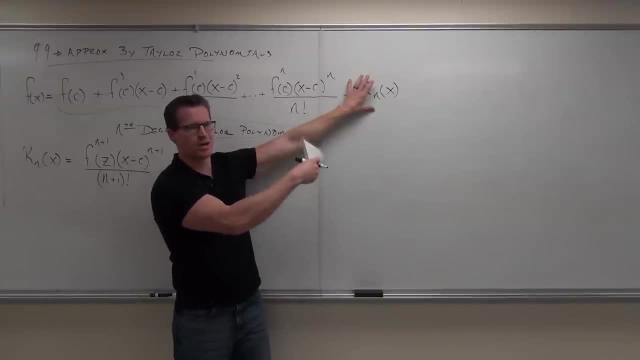 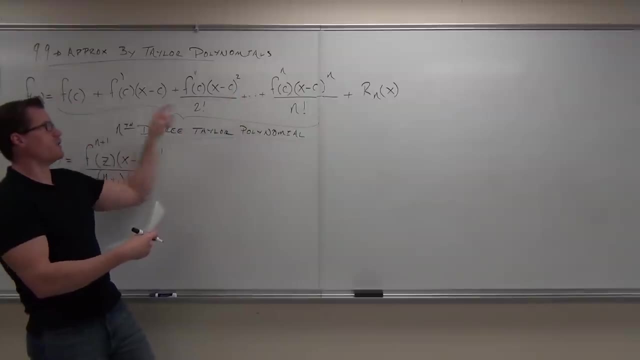 A Taylor series would. So we call that place where you cut it off. That's the end of our Taylor polynomial. Now there's going to be some difference between the Taylor polynomial and your function. We say, if I add a little bit to it, 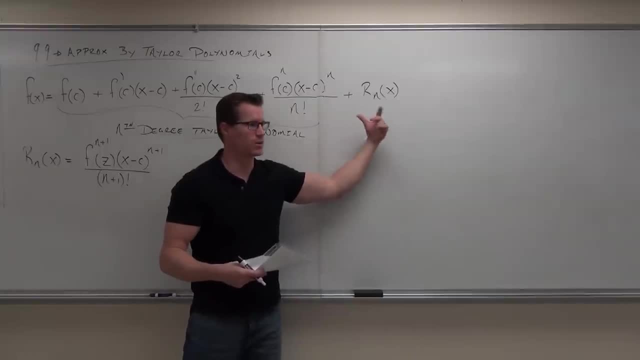 then I can make it exactly the same. exactly the same. That's your error. We are going to use this a little bit to say how close our approximation is to our actual function. Have I made sense of this at all for you? It's going to make a little more sense when we go through an example too. 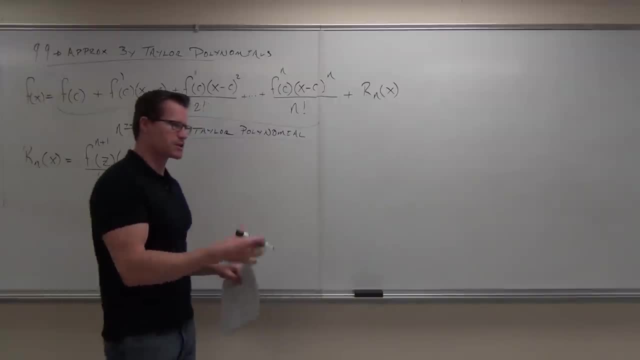 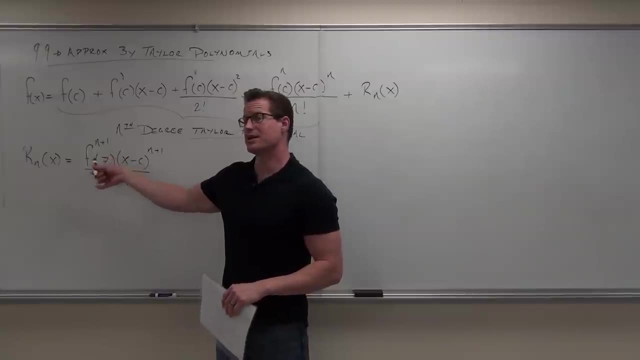 So basically, we're taking part of a Taylor series as an approximation, Now let's talk about the z, That z right there. That z is some number between c, c, the points you're using, and x, the points you're trying to approximate. 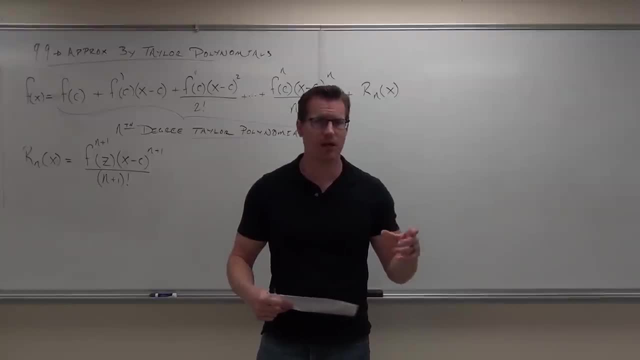 We get to pick what z is, and we're going to do this in a minute z. you're going to pick z so that you get the largest error. Are you listening? You don't want to underestimate your error. You want to overestimate it. if that's the case, 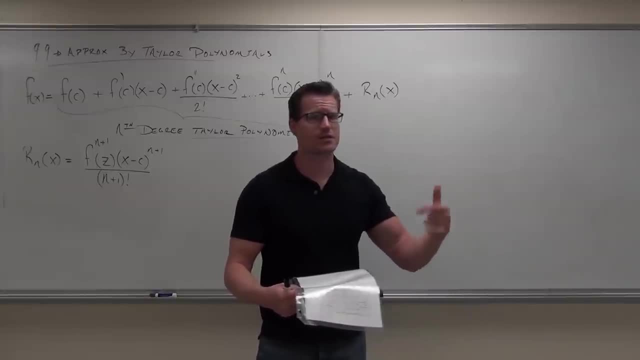 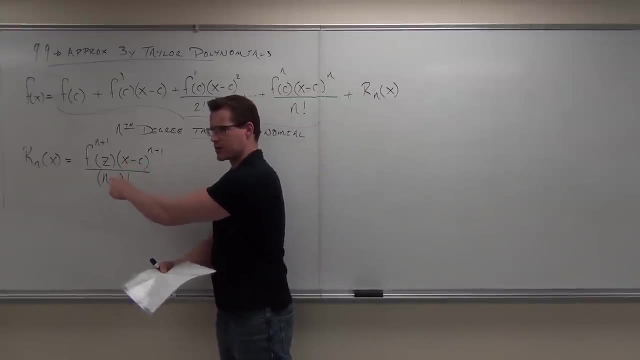 You don't want to underestimate it. So we get to pick z- z is some point between c, c and x- between the points you're using and the points you're trying to approximate. And let me illustrate that right now with an example. 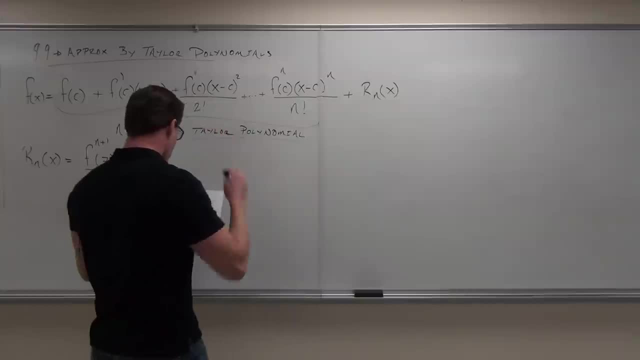 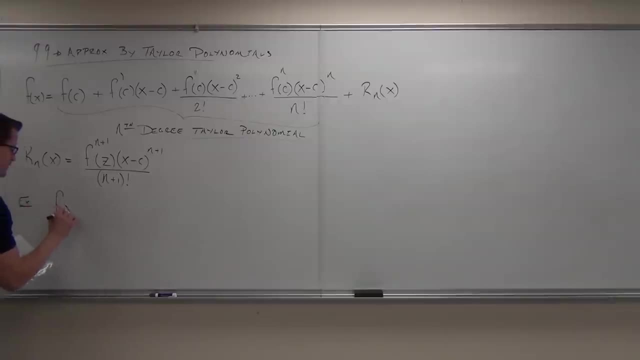 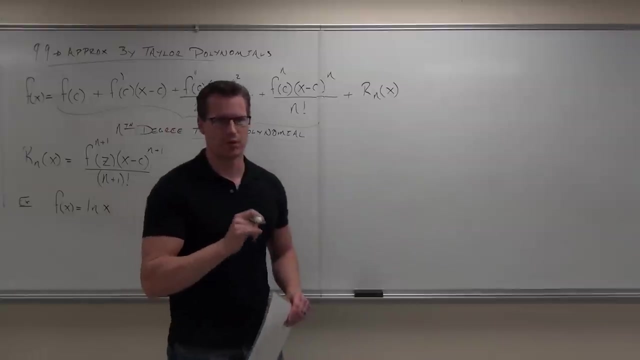 Are you guys ready for an example? Mm-hmm. OK, So here's what we're going to do. Let's say we've got a function, Our function is ln x, And what we're going to do is we're going to approximate ln of 1.1.. 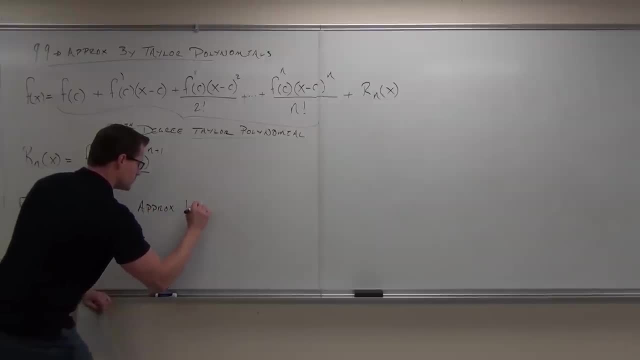 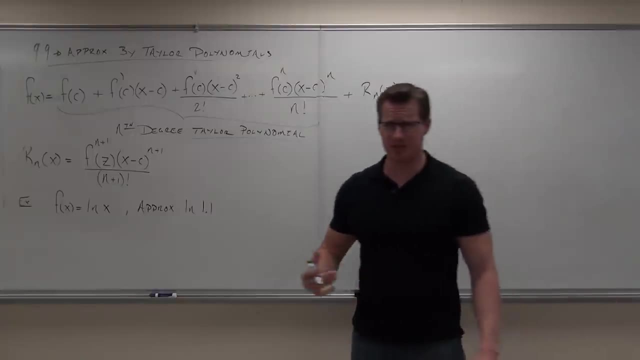 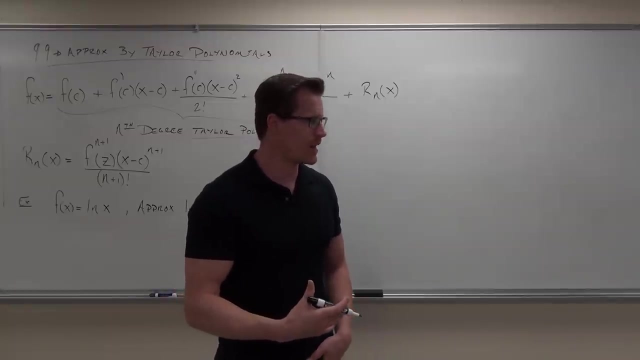 OK, Now if you're thinking, wait a minute, Didn't we just kind of do this in the last section? Didn't we have these Taylor series where we could approximate and find out endpoints, all this stuff for interval? Well, we did that, right. 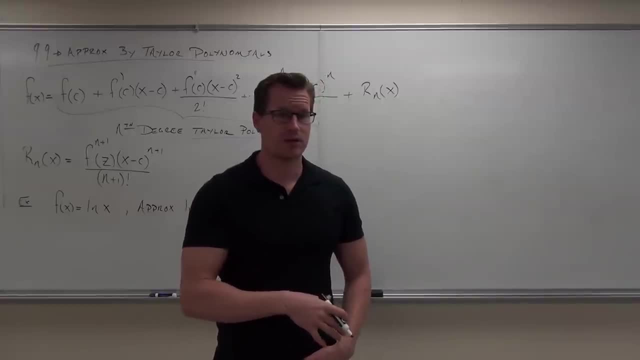 Well, but that took a long time correct. Yes, This is kind of like a shortcut. This is saying: well, let's approximate, But maybe we don't have to find the entire Taylor series or Maclaurin series or whatever. 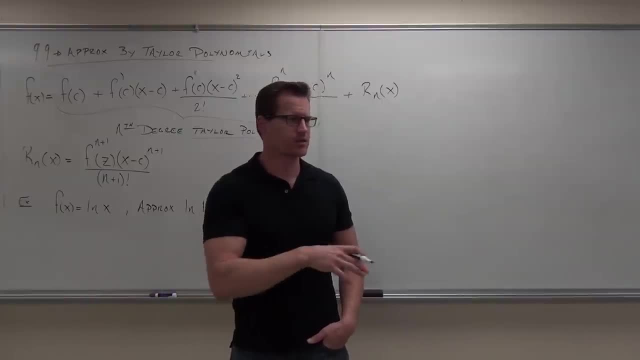 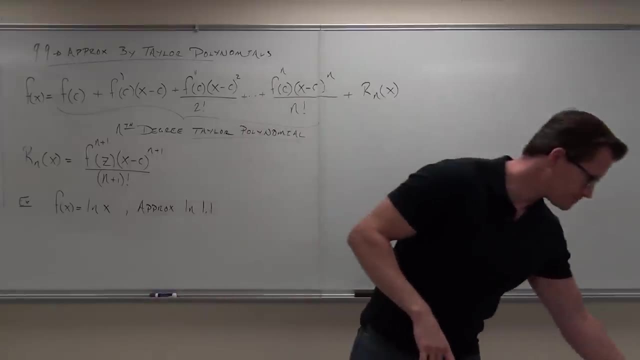 series or Maclaurin series or whatever. Let's go ahead and let's do an approximation really, really fast. And that's what this is for. Taylor polynomial says: let's approximate this quickly. Here's how we're going to go about doing it. 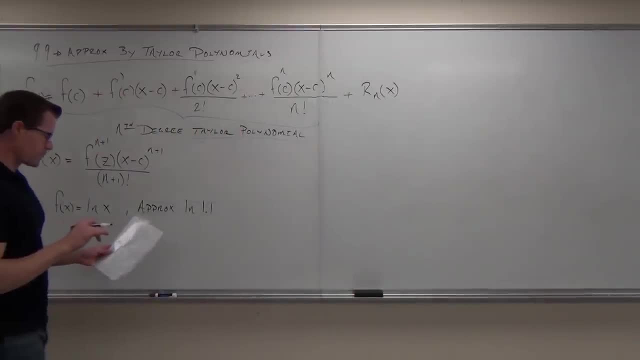 So our idea is we're going to find a Taylor polynomial at something that's close to this and then we're going to approximate it And then use it to approximate. So our idea: we want to find a Taylor polynomial at some point close. 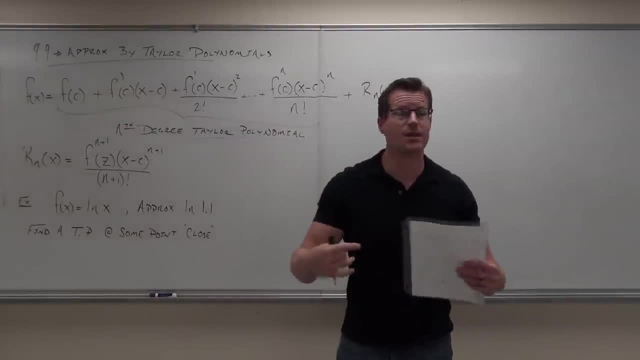 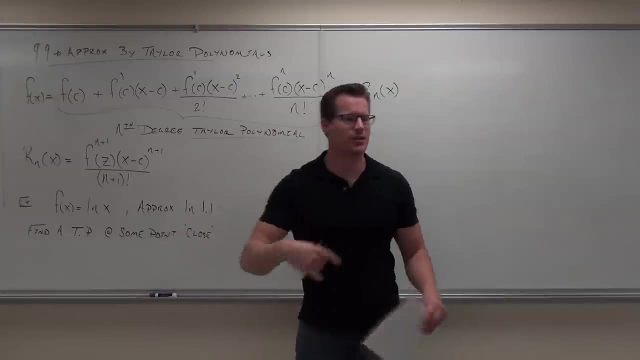 Now let's pick a good point that's really close to the number we're trying to approximate. What number are we trying to approximate here? 1.1., 1.1.. Give me a number that's close to 1.1, that would be easier to work with. 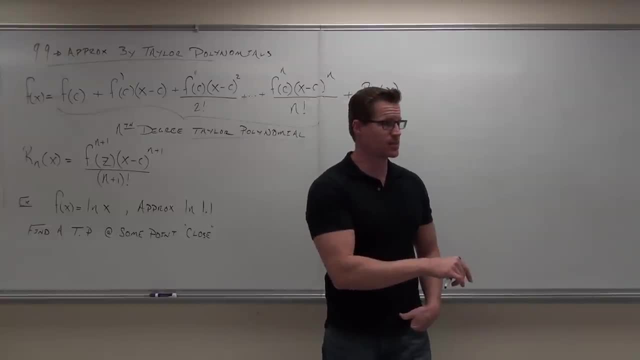 1. OK, That right there. that is your c. Does that make sense? Your x in this case is 1.1.. Look at f of x. Your x is 1.1.. Do you guys get that? So your x is 1.1.. 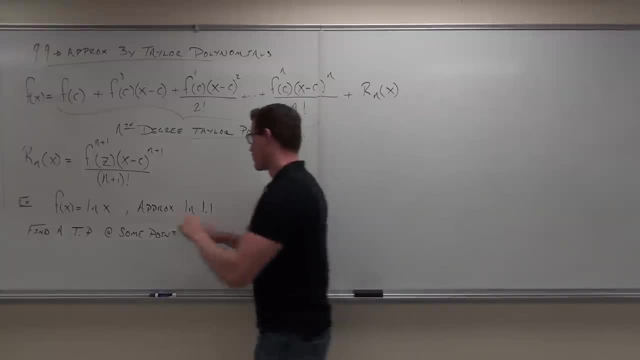 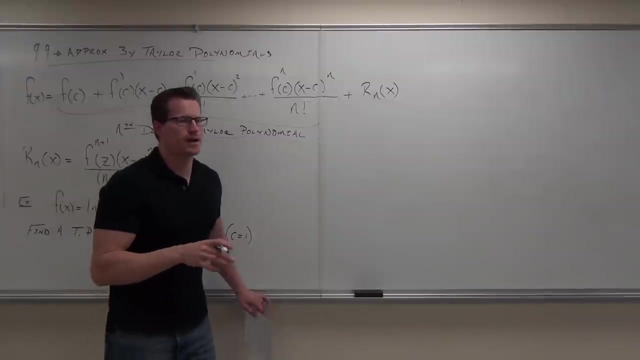 Your c is going to be 1.. So we're going to find the Taylor polynomial at some point close. Let's say c equals 1. 1. 1. 1. 1. 0.. The l values are not growing, they're just not growing together. 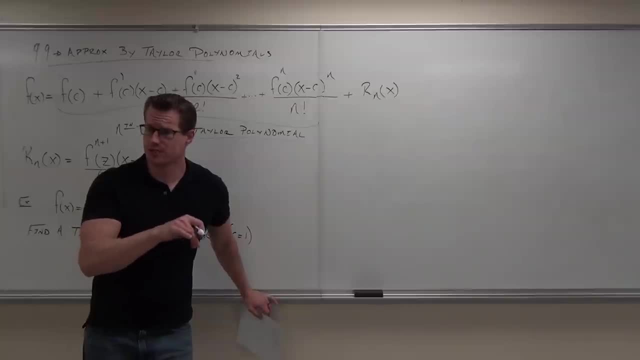 So we want to use x equal to 1.1.. The l values on either x and y just, or 1 and all the less than 1, they're going to break. So in this case we wanted to pledge x equals 1.1.. 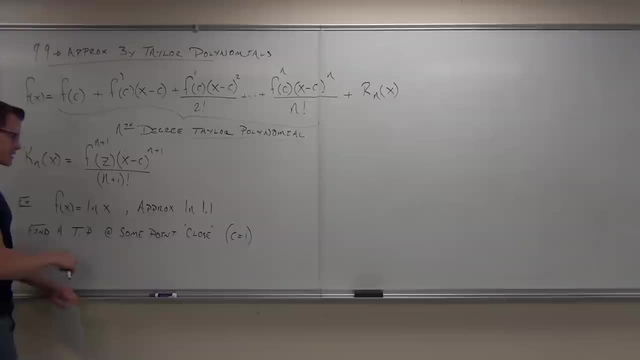 So if we want to take this, and we yeah, a 2 and 1's equal to 1, plus that To get this to the 7.5. Right, You with me, And let's pick the fourth degree, because I'm pretty sure. 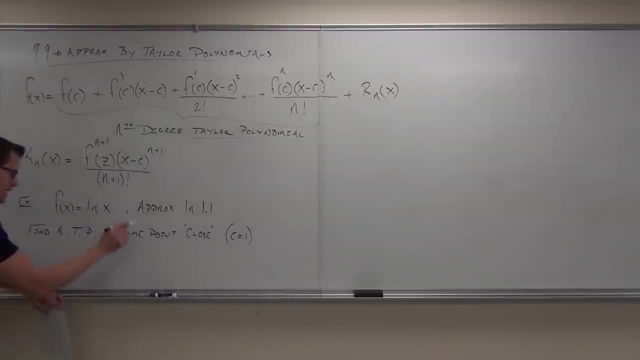 at that point we're going to have an approximation. that's fairly good. So find some Taylor polynomial that's close at some point. that's close equals 1, and then we're going to use a fourth degree Taylor polynomial to do this. 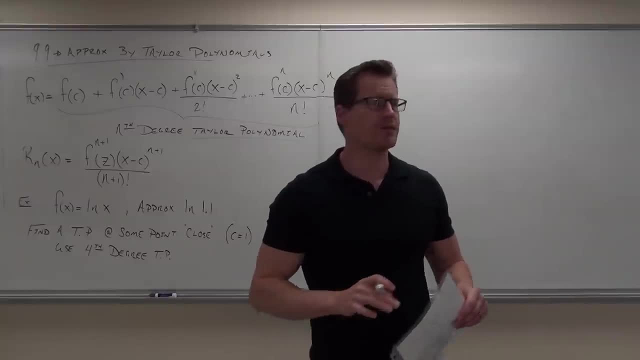 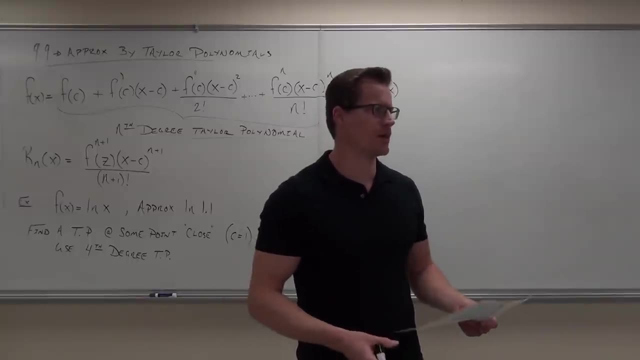 The rest of it is honestly pretty easy. There is no pattern to find. Remember the patterns that you guys just had to do in your homework that were kind of hard to find sometimes. You don't have to do that here and that's what's kind. 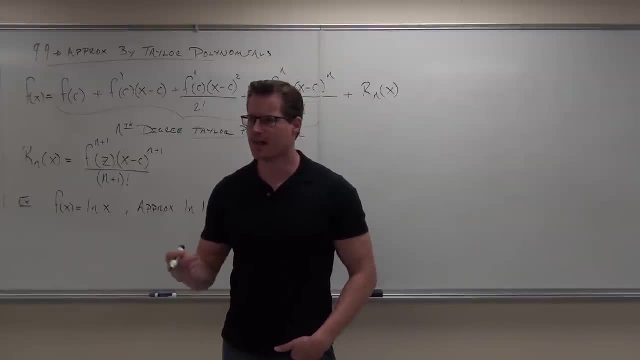 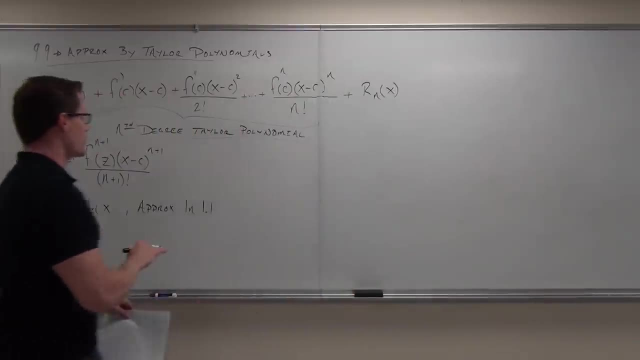 Let's go ahead and let's do an approximation really really fast, OK, And that's what this is for. Taylor polynomial says: let's approximate this quickly. Here's how we're going to go about doing it. So our idea is we're going to find a Taylor polynomial at something that's close to this. 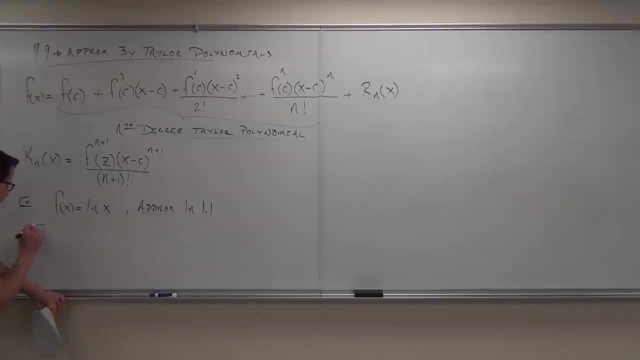 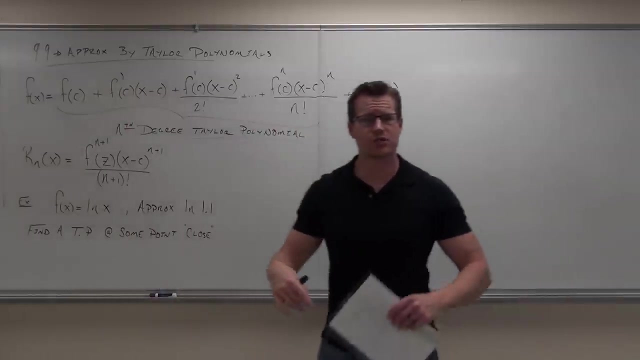 and then use it to approximate. So our idea: we want to find a Taylor polynomial at some point close. Now let's pick a good point that's really close to the number we're trying to approximate. What number are we trying to approximate here? 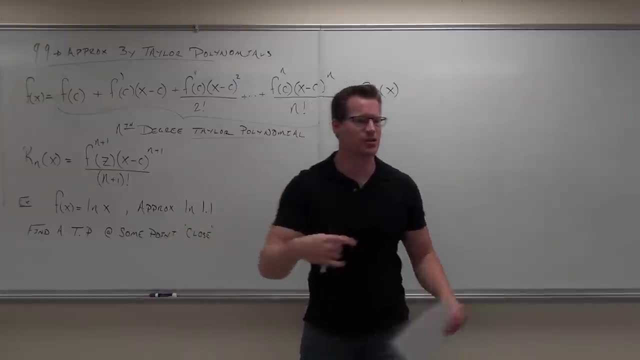 1. Yeah, ln of 1.1.. Give me a number that's close to 1.1, that would be easier to work with 1. OK, That right there. that is your c. Does that make sense? 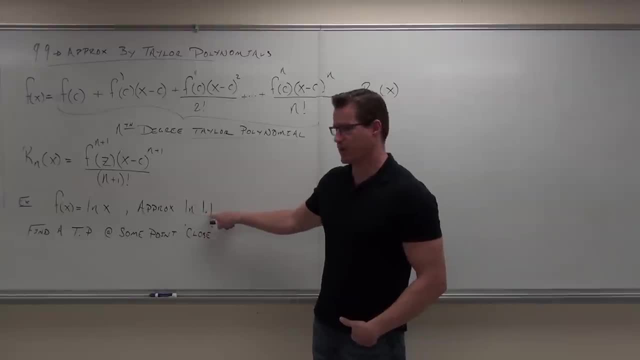 Your x in this case is 1.1.. Look at f of x: Your x is 1.1.. Do you guys get that? So your x is 1.1.. Your c is going to be 1.. So we're going to find the Taylor polynomial at some point close. 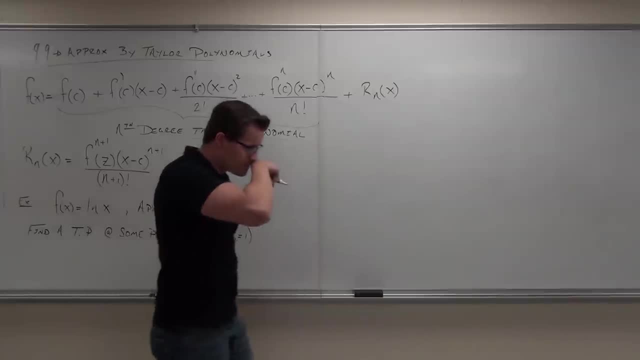 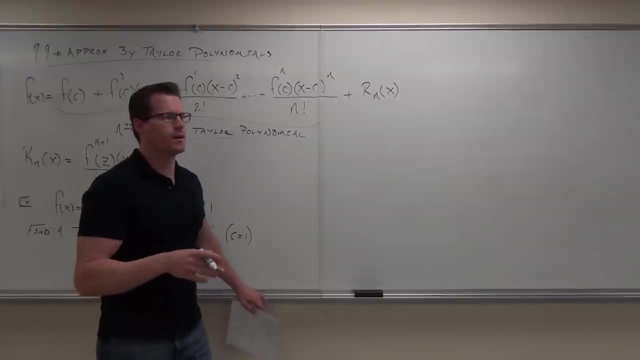 Let's say c equals 1.. And here we're going to use a fourth degree Taylor polynomial because I want to show you how it works. all right, Now I've got to be honest with you. On any test or any homework that you're going to have, they're going to tell you what c to use. 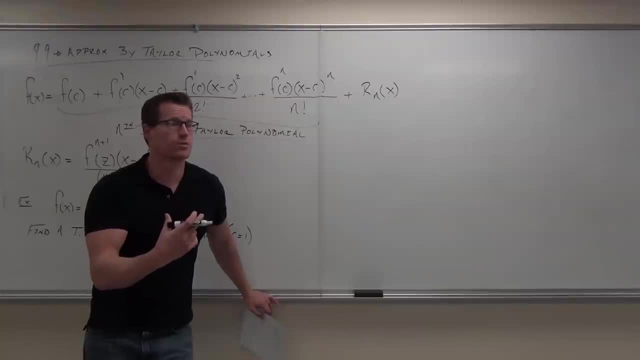 You don't get to pick it And they're going to tell you what range you're going to have And they're going to tell you what degree you're going to use. Does that make sense? So it's not going to be up in the air like this one is. 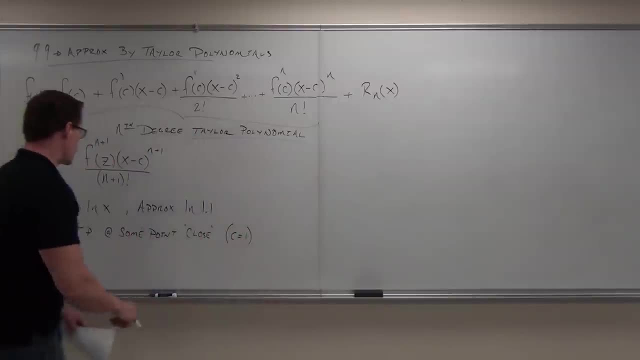 I'm just showing you, like in real life, how you go about it. You go OK. well, I'll tell you what I want to approximate this. Let's use a Taylor polynomial. Let's use it at a point. that's close. 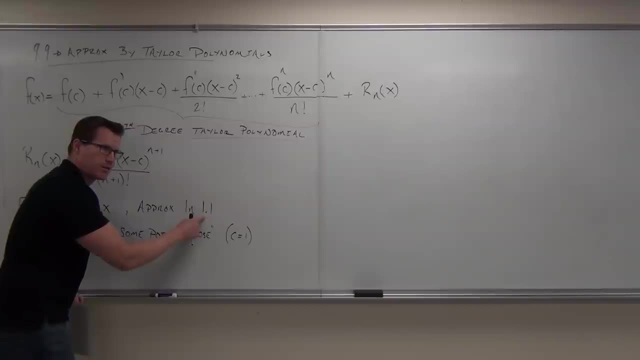 Hey, 1 is pretty close to that. Are you with me? And let's pick the fourth degree, because I'm pretty sure at that point we're going to have an approximation? that's fairly good. So find some Taylor polynomial that's close at some point. that's close. c equals 1.. 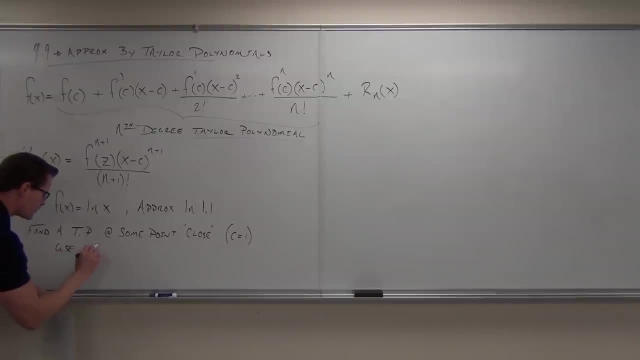 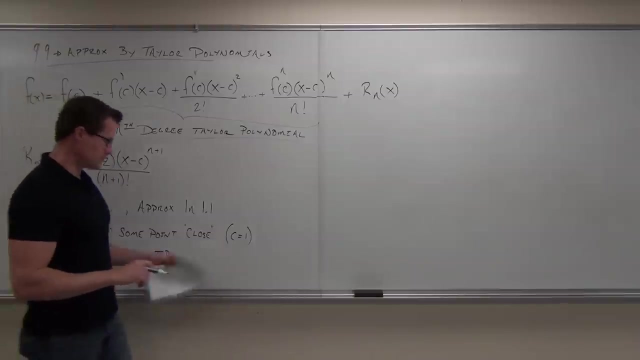 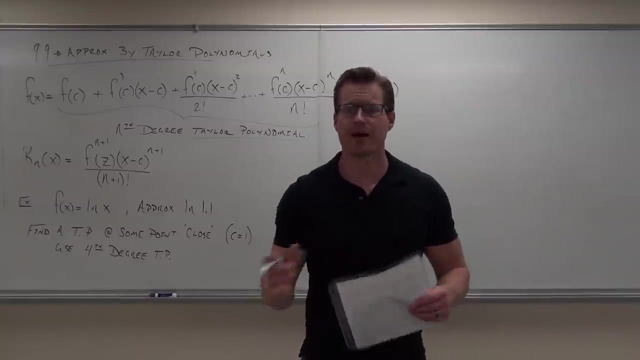 And then we're going to use a fourth Degree Taylor polynomial to do this. The rest of it is honestly pretty easy. There is no pattern to find. Remember the patterns that you guys just had to do in your homework that were kind of hard to find sometimes. 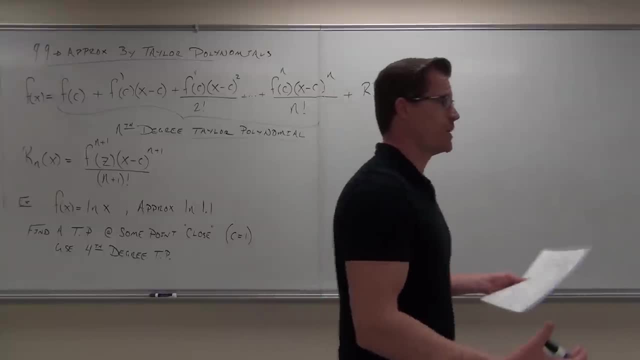 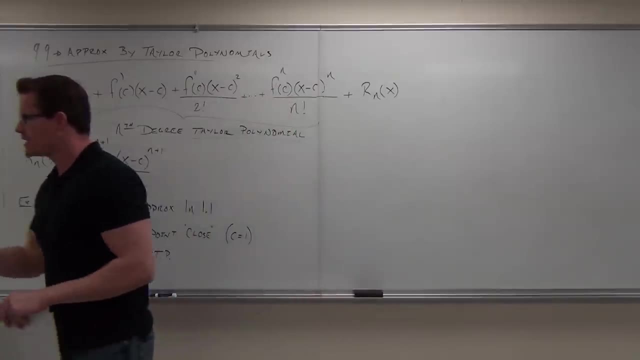 You don't have to do that here, And that's what's kind of nice about this. There is no pattern. All we're going to do is start, like you would do a Taylor series, but then you're just going to stop. So we start with: OK, can you do a Taylor series from this? 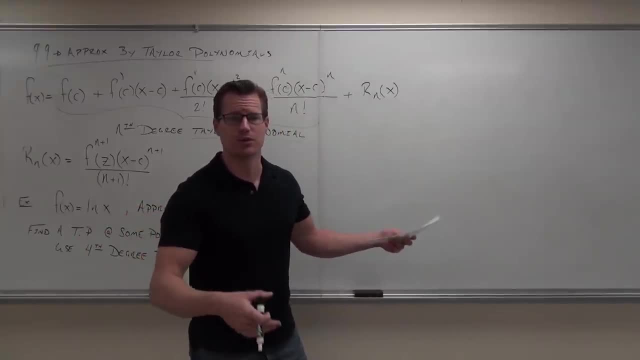 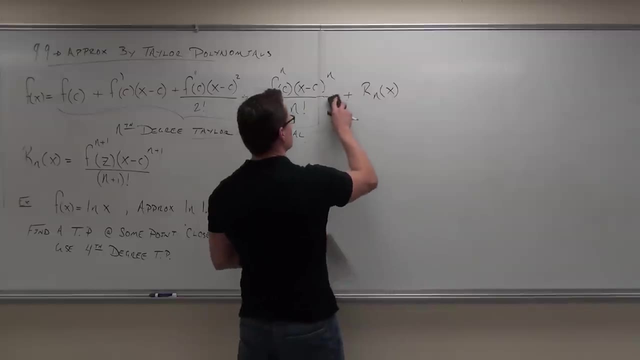 Sure you could. What's the first thing you did when finding a Taylor series? What would you do All those derivatives you had? So we're going to start with. can I erase this here? This is right my way. Well, let's start with f of x. 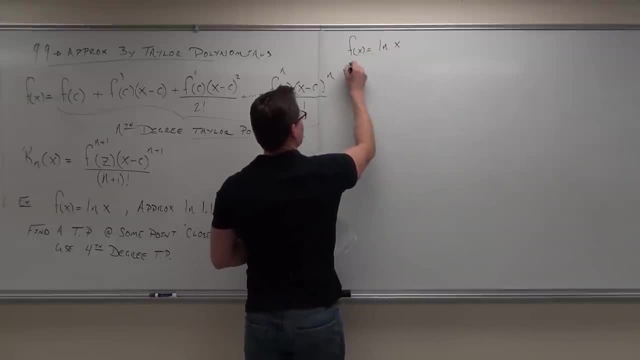 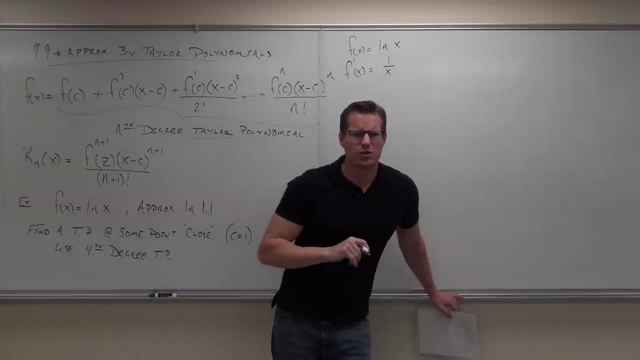 What's f of x? How about f prime of x? Good, Do we need to keep going? Yes, What degree? Taylor polynomial did it say 4 and 4.. How many derivatives you got to go to 4 and 4.. 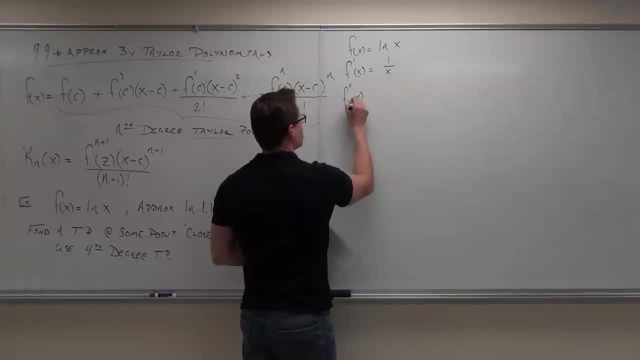 You're kind of close, We'll get there. Second derivative is Minus 1 over x. Good, How about third derivative: Negative 2 over x. Say it again: Positive 2 over x. I'm going to assume you said 2 over x, cubed. 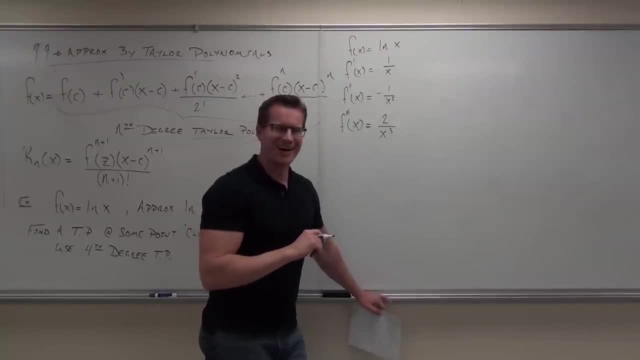 Let's get our brains working today. I love that one. How about the fourth derivative? Negative: 6 over x is 4.. OK, Are you guys with me on this one? We know derivatives. yeah, All right, Just to make sure. 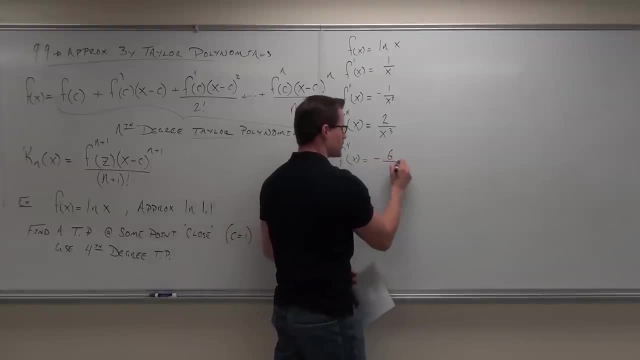 Just to make sure, I know spring break takes a lot out of our minds. sometimes It does mine. I'll tell you that. So stop drinking, all of you. Just so you know I appreciate it. Thank you, Thank you. 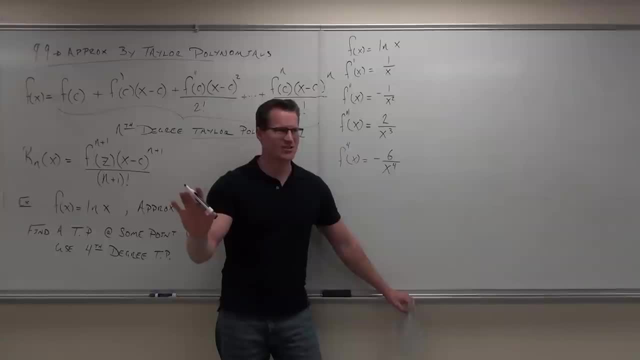 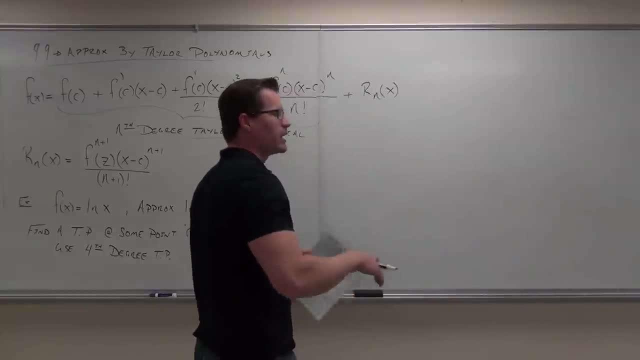 of nice about this. There is no pattern. All we're going to do is start like you would do a Taylor series, but then you're just going to stop. So we start with: okay, can you do a Taylor series from this? 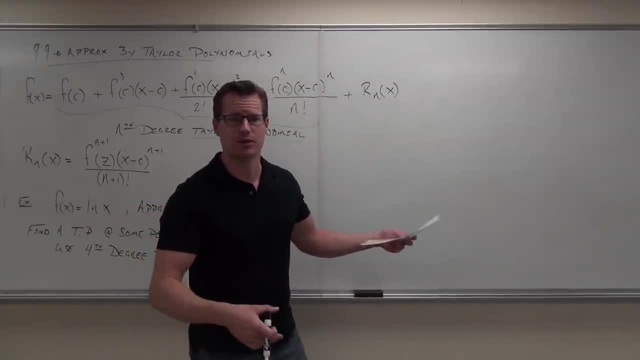 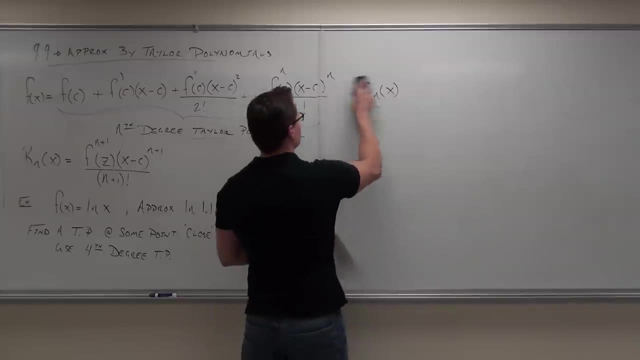 Sure you could. What's the first thing you did when finding a Taylor series? What would you do All those derivatives you had? So we're going to start with. can I erase this here? this is right my way. Well, Let's start with f of x. 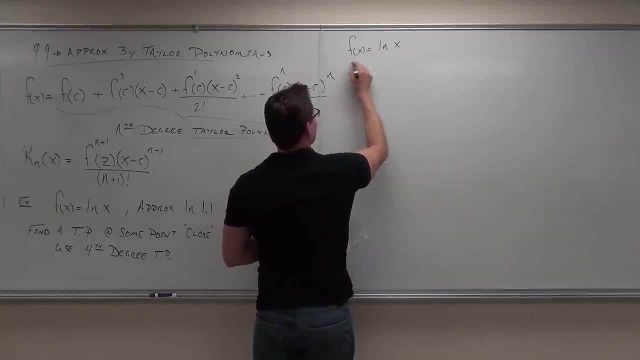 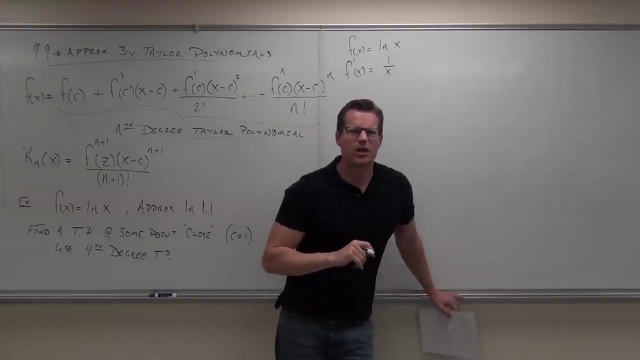 What's f of x, L and y? How about f? prime of x, One over x? Good, Do we need to keep going? Yes, What degree? Taylor polynomial did it say? Fourth, So what derivative do you got to go to? 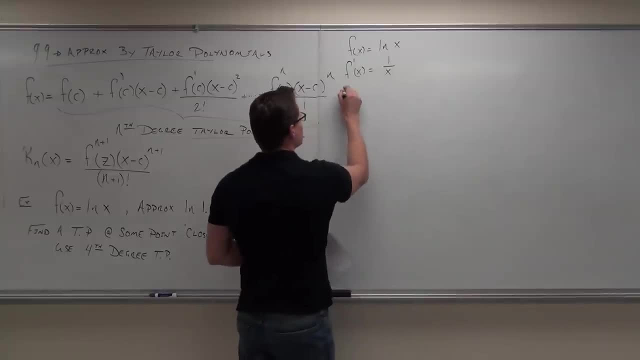 Fourth, Fourth. You're kind of close, We'll get there. Second derivative is: Minus one over x, Minus one over x. Good, How about third derivative, Negative, two over. Say it again, Positive, Positive. I'm going to assume you said two over x, cubed. 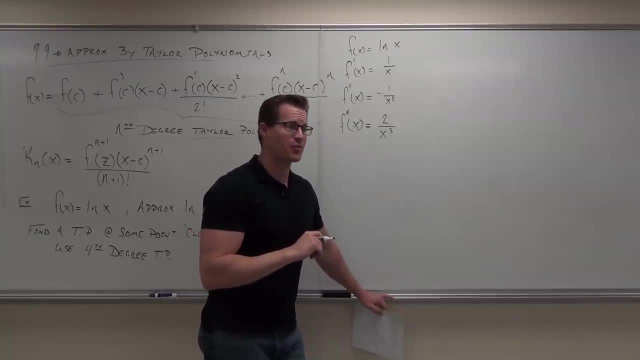 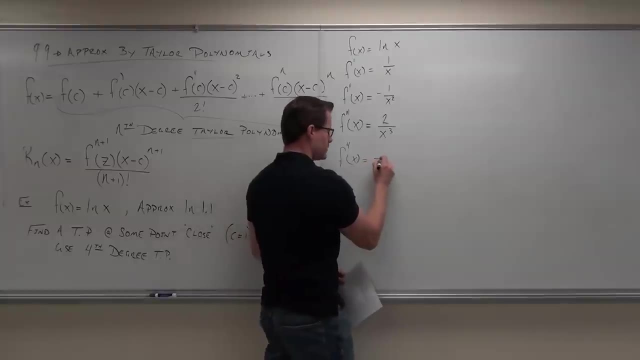 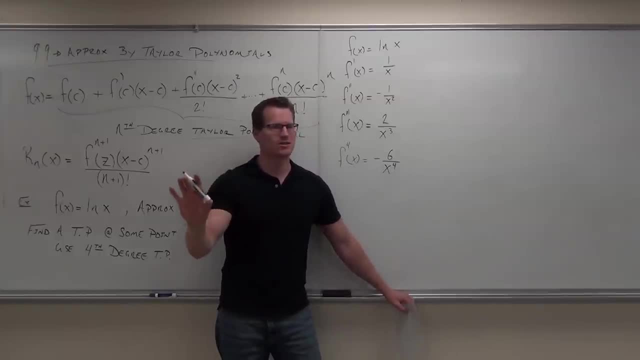 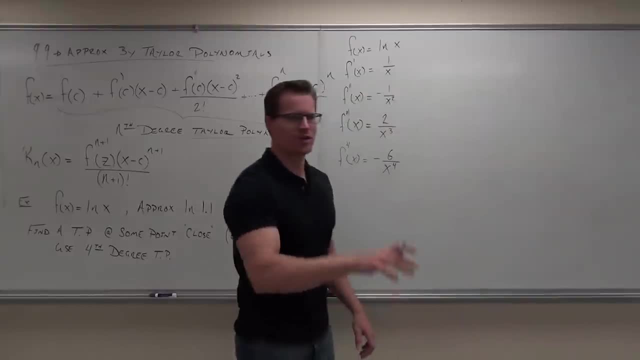 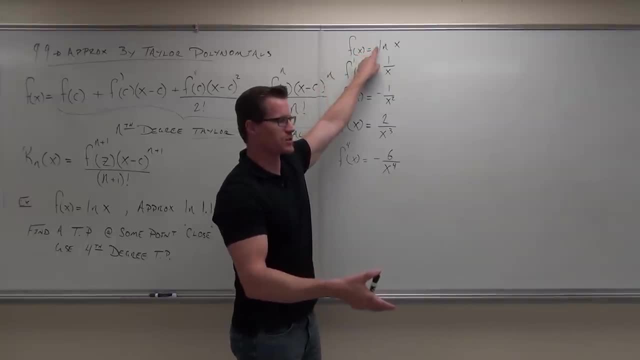 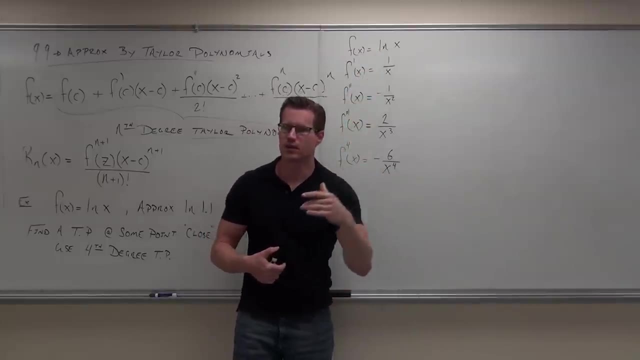 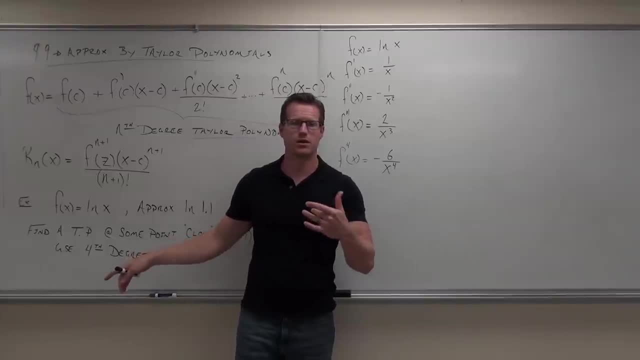 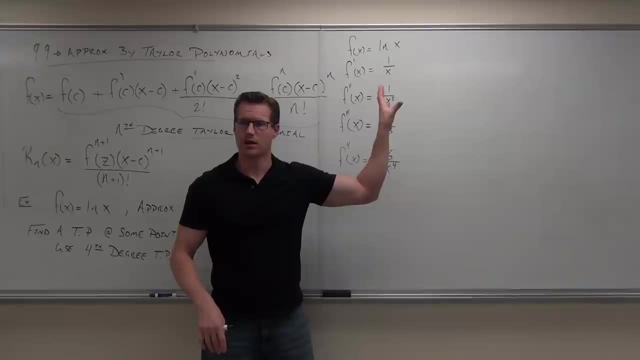 Four, Four, Four, Four. It's a degree four. Now here's the thing. Do you understand that? with a degree four, I erased it, but the next term was my error. right, Yeah, Look up here. The next term was my error. 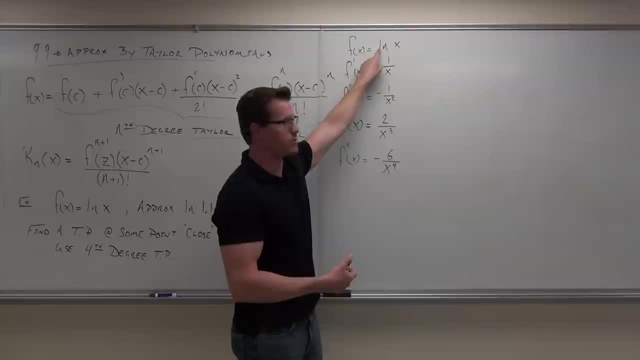 We do the function, We do a derivative, then a second derivative, then a third derivative, then a fourth, And with a Taylor series we keep going And we'd find a pattern for this. So if you'll be OK with that one, 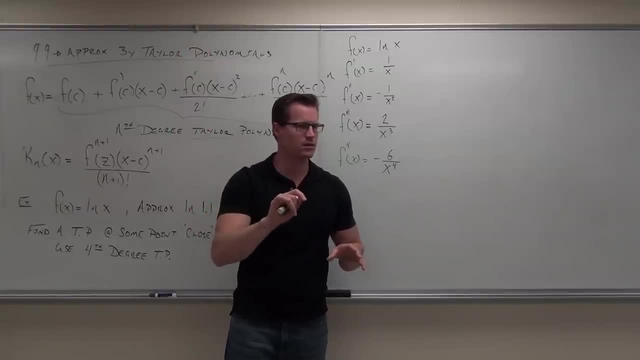 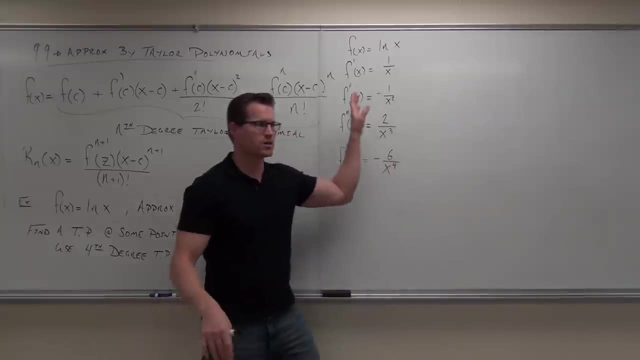 Now we stopped at the derivative of 4.. Why did we do that? Because 4 is a degree 4.. So it's a degree 4.. Now here's the thing. Do you understand that? with the degree 4, I erased it, but the next term was my error. 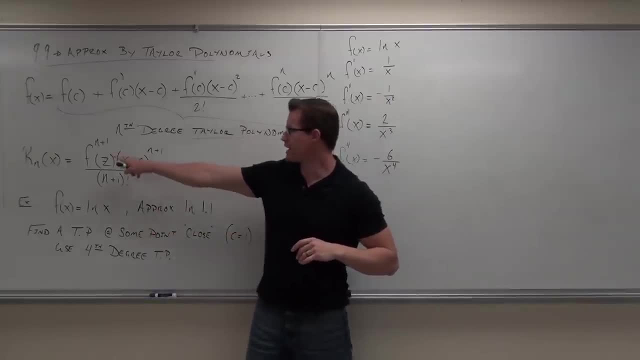 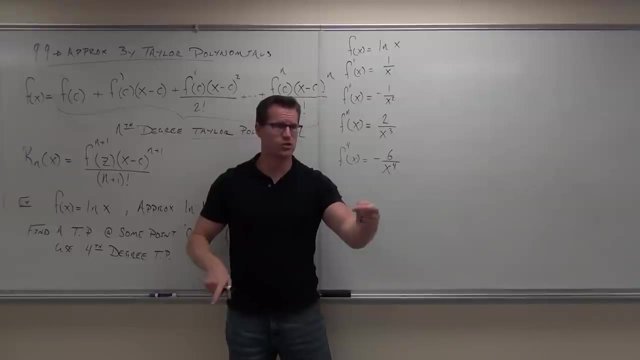 Look up here. The next term is my error. If I have a degree four, what's this one going to be? Find your next derivative, because you're going to use it for your error, So I'm going to leave this. This is all we need for my polynomial, okay. 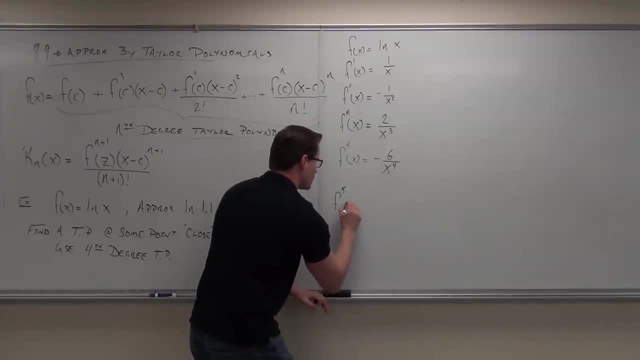 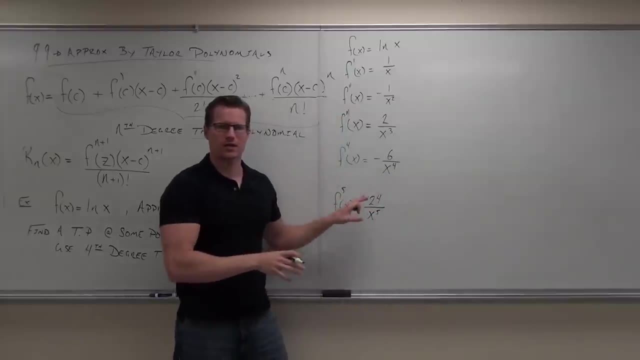 For my error. I'm going to go. okay, I need one more. Just hang on to this in the back of your head, because we're not going to use it right now. We're going to use it in just a little bit. 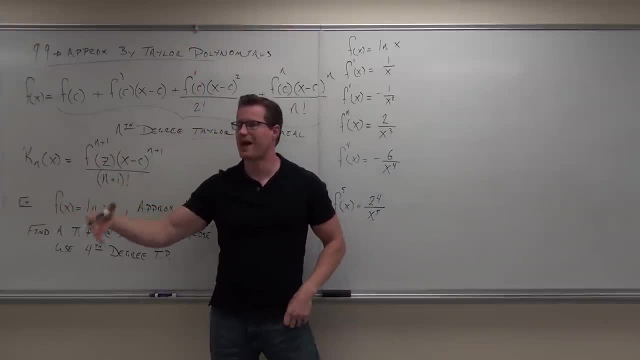 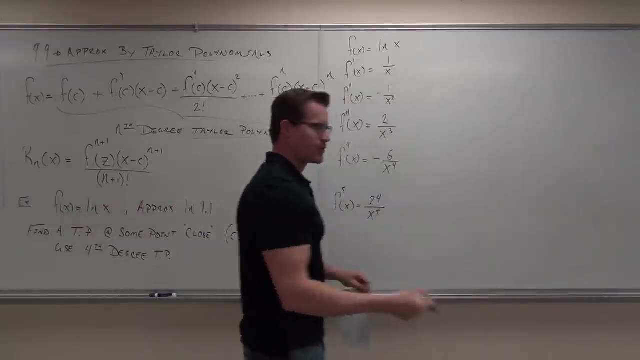 Do you understand why we're finding the next derivative past our degree? that I've told you What's it for Error? That's exactly right Now, the next thing we did with the Taylor series. you say, all right, well, cool. 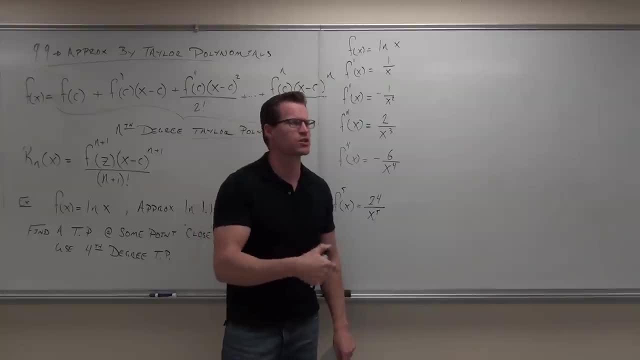 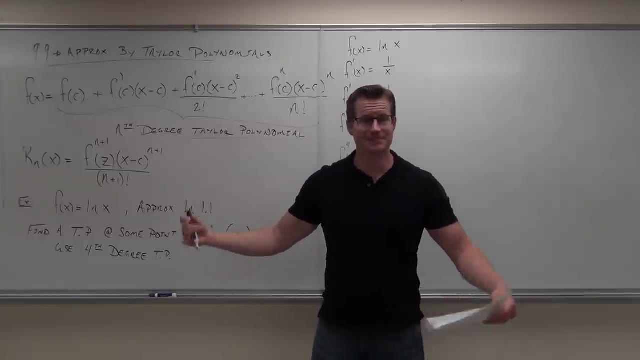 What do we do now With the Taylor series? what did you do? You plugged in c. Oh, very good. Do we have a c? What's our c? y1. c? So if we plug in, c equals 1, then we have f of 1.. 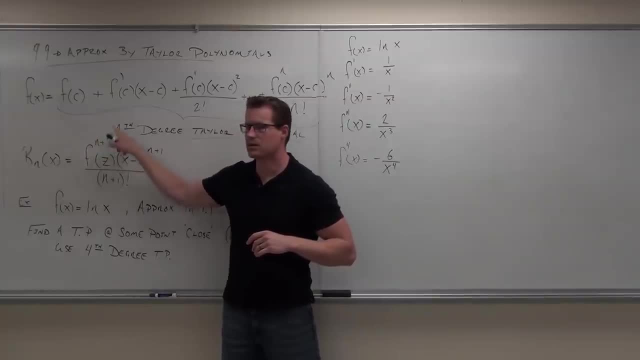 If I have a degree four, what's this one going to be Five, Five. Find your next derivative, because you're going to use it for your error, So I'm going to leave this. This is all we need for my polynomial, OK. 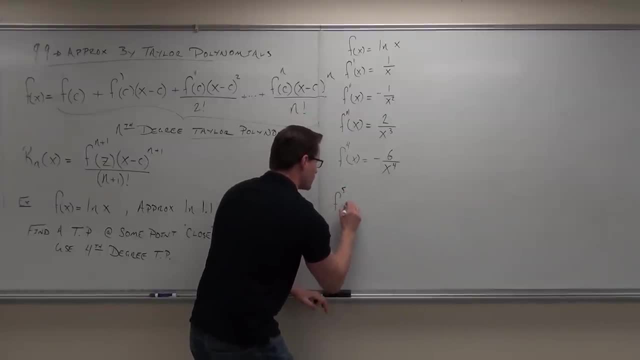 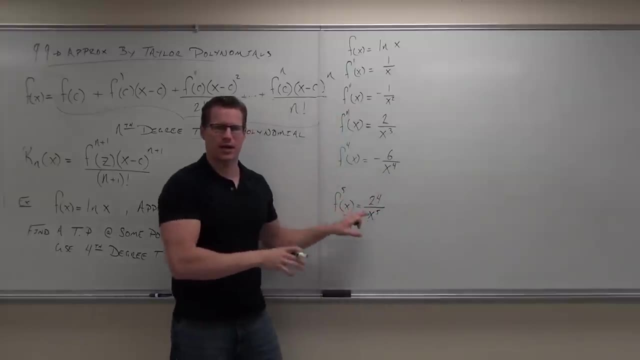 For my error. I'm going to go. OK, I need one more. Just hang on to this in the back of your head, because we're not going to use it right now. We're going to use it in just a little bit. 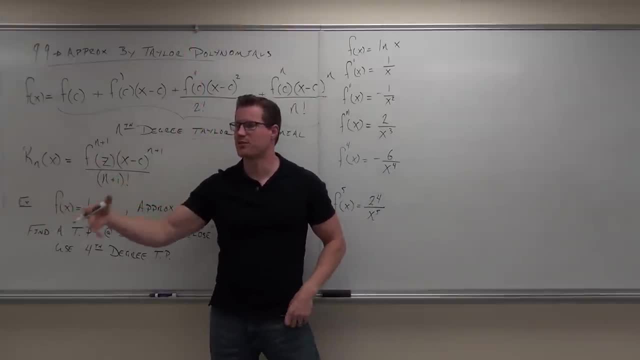 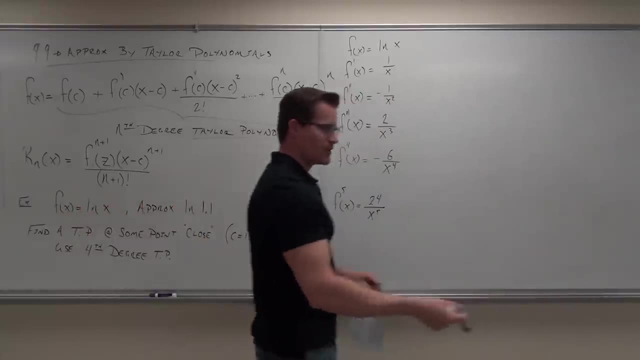 So if you guys are OK with that so far, OK, do you understand why we're finding the next derivative past our degree that I've told you? Error, What's it for? Error? That's exactly right Now. the next thing we did with the Taylor series. we said: 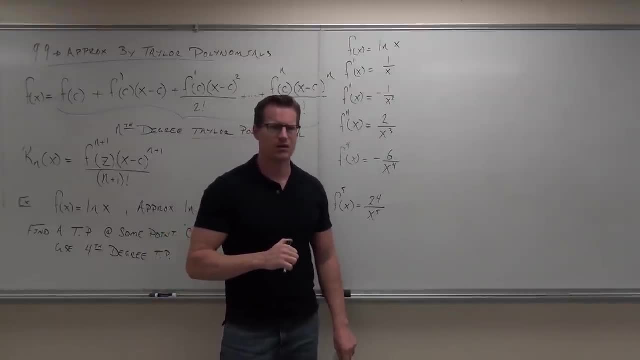 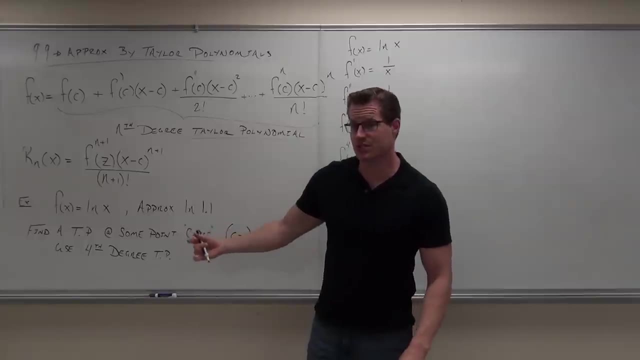 all right, well cool. What do we do now With a Taylor series? What did you do? You plugged in c. You plugged in c. Oh, very good. Do we have a c? What's our c? y1.. 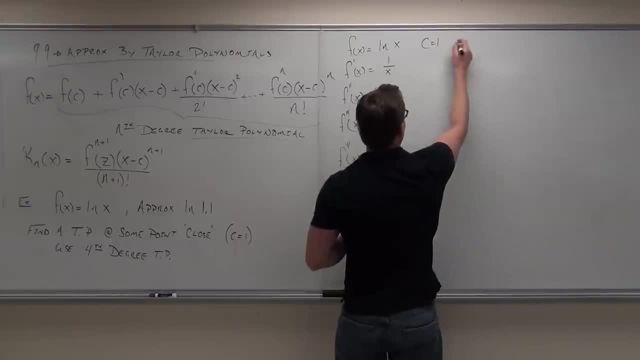 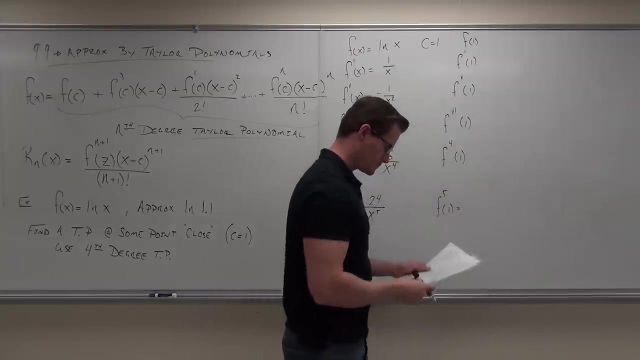 c. So if we plug in c equals 1, then we have f of 1.. And we have f prime of 1, and so forth and so on, And we're even going to do it down here. So let's plug that in. 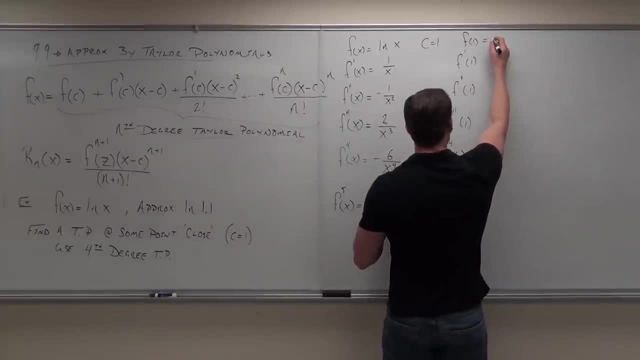 Let's see what we get. How much is f of 1,, please 0.. How about f prime of 1?? What are you going to get? 1.. How about f double prime of 1?? 1. Triple prime. 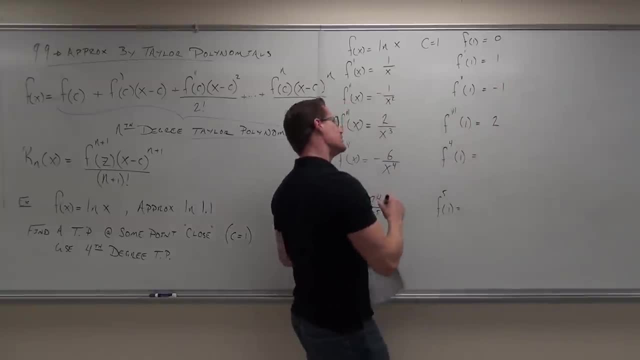 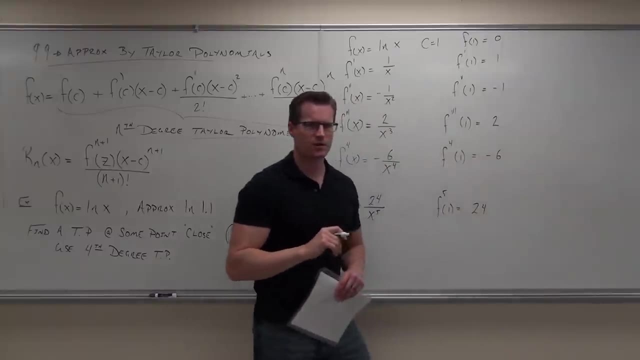 2. What Drupal prime 6. And 4. 4. Perfect, Yeah, Y'all still OK with that so far? Yeah, Now don't make it harder than it is. You're not looking for a pattern here. 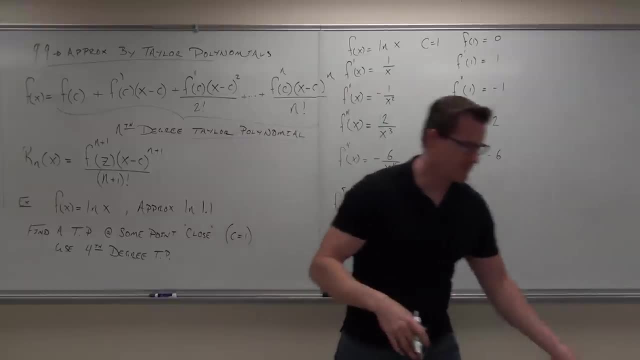 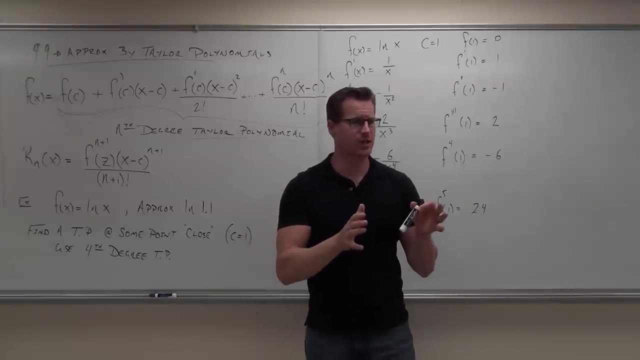 I don't care about the pattern, What we're doing. remember the very beginning of when I explained this. I said: what we're doing here is we're taking part of a Taylor series That's called Taylor polynomial. We're taking part of a Taylor series, our Taylor polynomial. 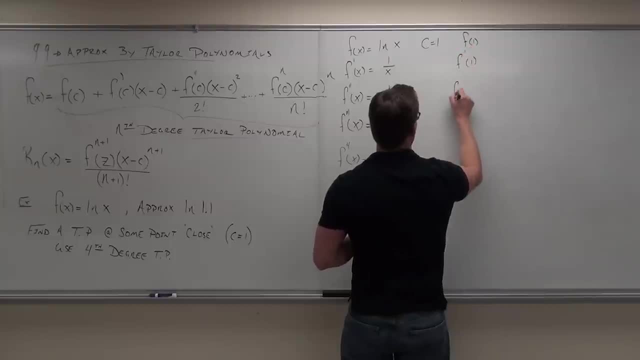 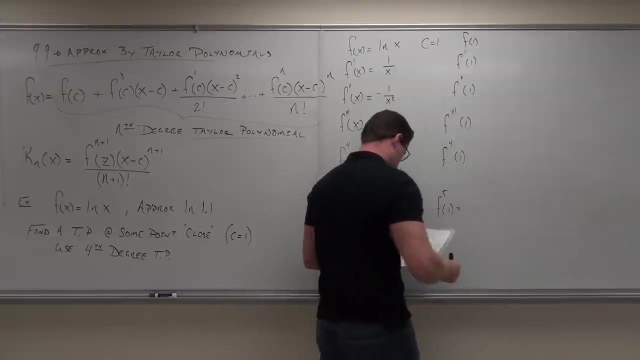 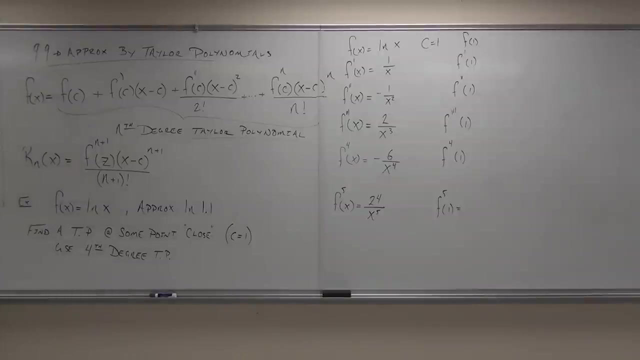 And we have f prime of 1.. And so forth And so on, And we're even going to do it down here. So let's plug that in. Let's see what we get. How much is f of 1, please? 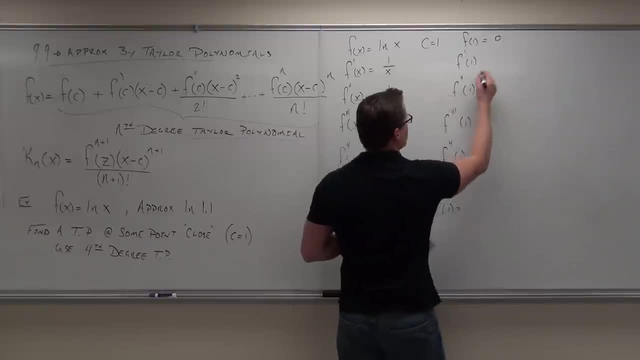 0.. 0., 0., 2.. And then we're gonna get what F prime of 1, where are you going to get 1.. How about f double prime of 1? слов What Druple prime. 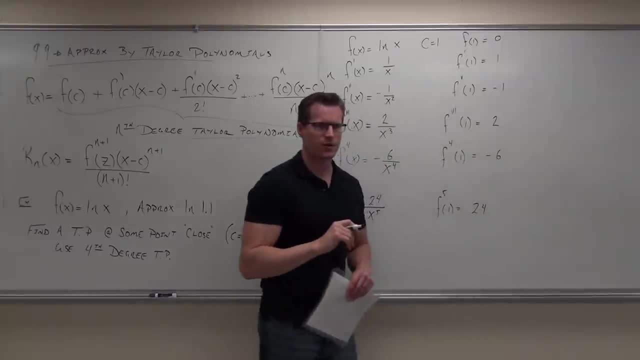 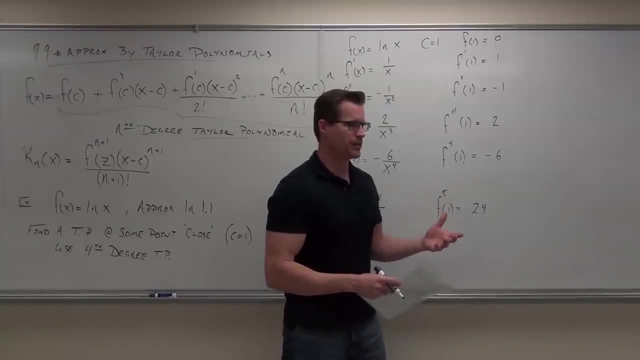 And Y'all still OK without zero CHARLOTTE. Now, don't make it harder than it is. You're not looking for a pattern here. I don't care about the pattern, What we're doing. remember that the very beginning of when I explained this, I said what we're. 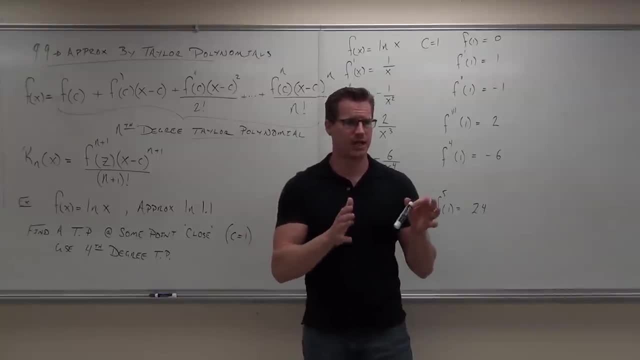 we're doing here is we're taking part of a Taylor series That's called Taylor polynomial. We're taking part of a Taylor series, our Taylor polynomial, to represent or approximate our function. It's going to be an approximation. We don't have to find the whole series. You 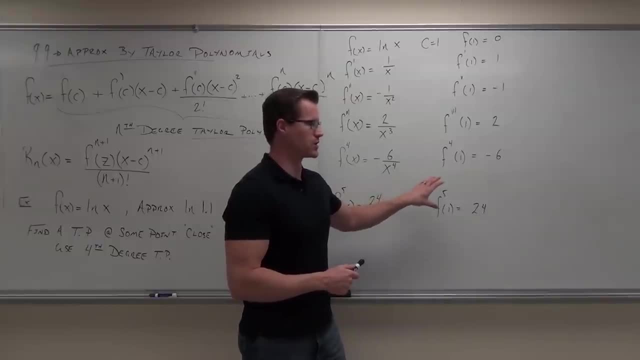 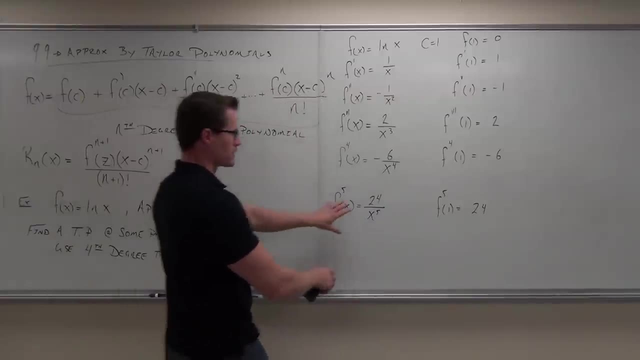 stop right here and then you start building your polynomial. So here's what we're going to do at this point. Are there any questions on you know what? I'll do it down here because I want to make sure you see all this together. So, from right here, after we found our derivatives. 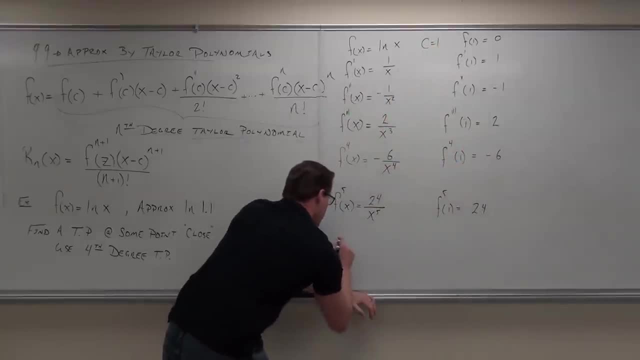 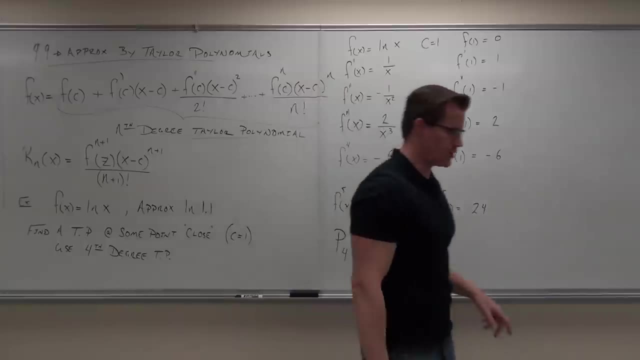 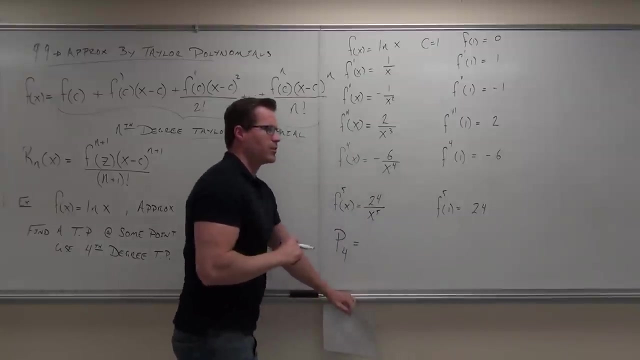 after we plugged in our c, we're going to go ahead and do our fourth degree Taylor polynomial. This right here stands for your fourth degree Taylor polynomial. Now I'm hoping that you remember what Taylor polynomials are, because they are based right off of the Taylor series. 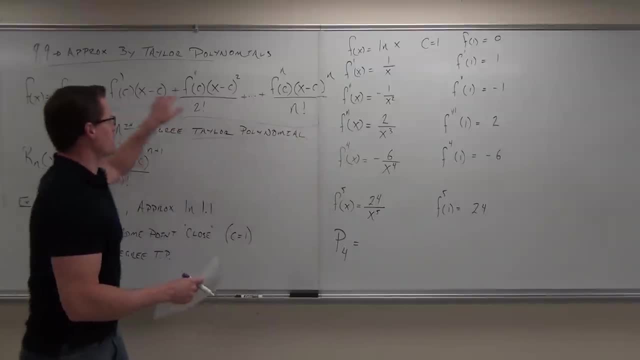 So, basically, we just got to get rid of this Taylor polynomial and we're going to get rid of this Taylor polynomial. So we're going to get rid of this Taylor polynomial and then we're going to take this stuff and plug it into here. That's all we're going to do. 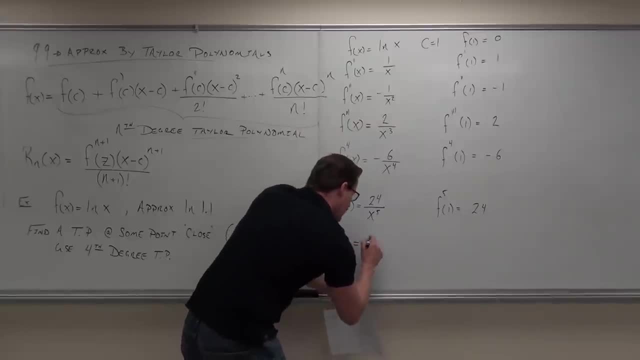 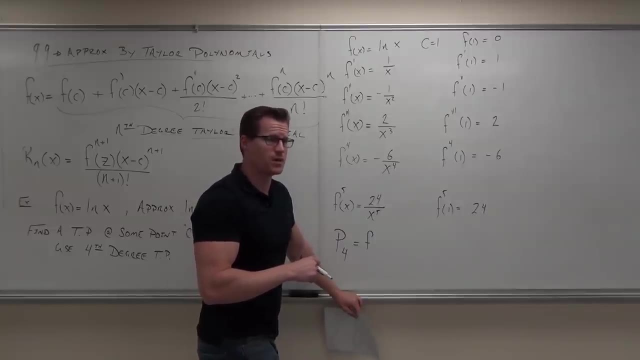 So a Taylor polynomial would look like this. It would be. it would start with f of c. But what is our c? in our case, One f of c would be One. Yeah, f of c. f of one would be zero, So we'd have f of one. Are you guys with me on this? 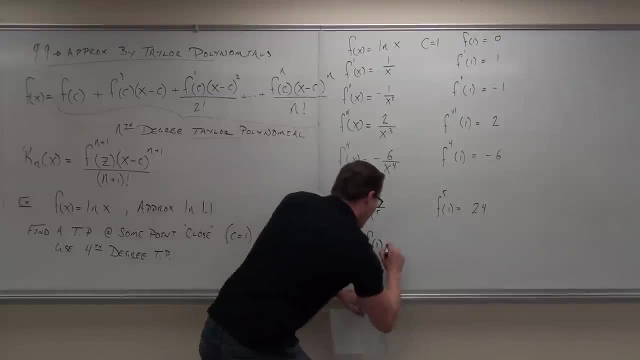 Are you sure you're with me? I don't want to lose you right now. right, We've been doing this for a while now. Plus, what's the next one? Prime of c, Okay, f, prime of one, And then you would have. 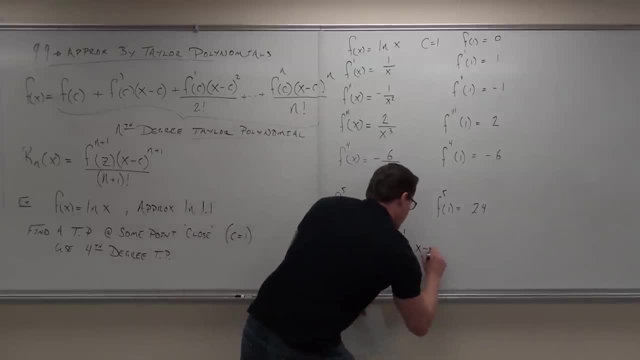 X minus One. You're right, It's x minus c, but in our case our c is one. Are you okay with that one? Mm-hmm, Okay, what's the next one? Double prime of one. And then you would have. 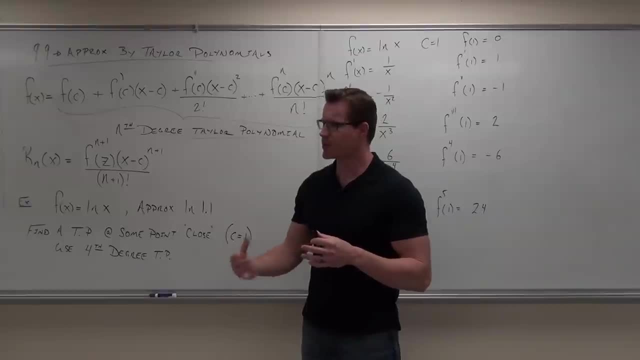 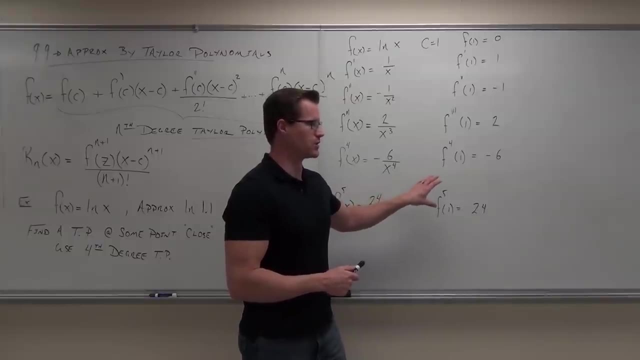 to represent or approximate our function. It's going to be an approximation. We don't have to find the whole series. You stop right here And then you start building your polynomial. So here's what we're going to do at this point. 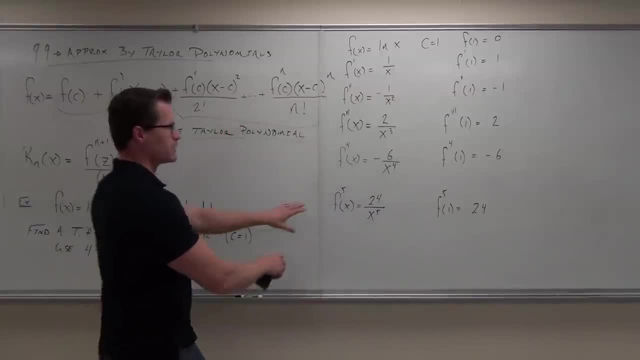 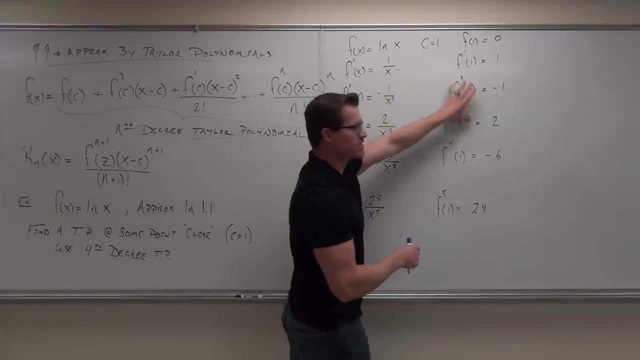 Are there any questions on You know what? I'll do it down here because I want to make sure you see all this together. So, from right here, after we've found our derivatives, after we've plugged in our c, we're going to go ahead and do our fourth degree Taylor polynomial. 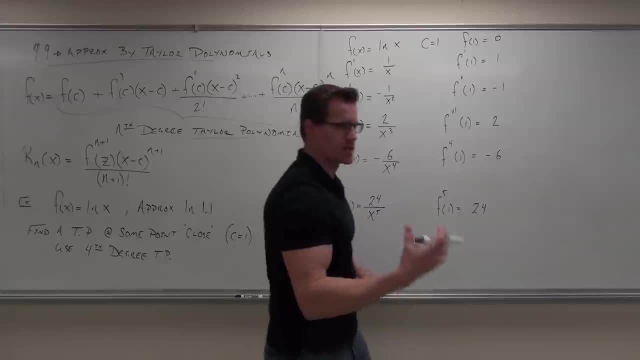 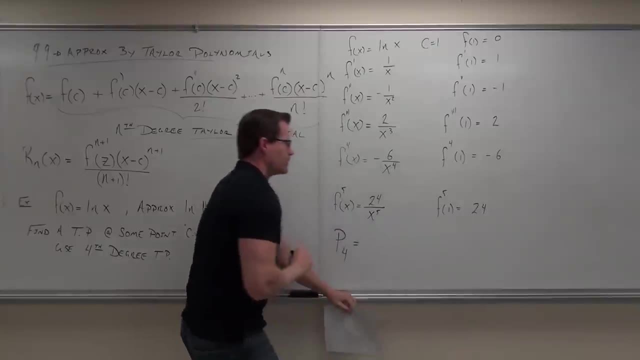 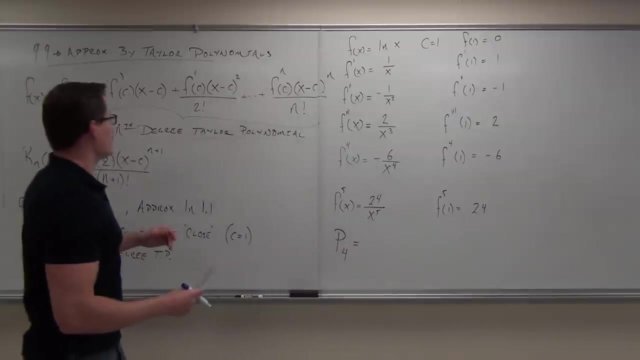 This right here stands for your fourth degree, Taylor polynomial. Now I'm hoping that you remember what Taylor polynomials are, because they are based right off of the Taylor series. So basically, we just got to take this stuff and plug it into here. 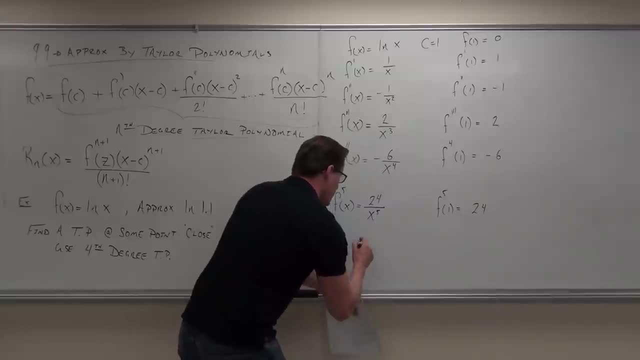 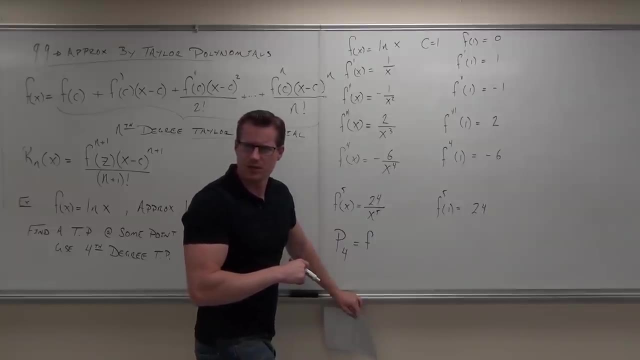 That's all we got to do. So a Taylor polynomial would look like this: It would be: it'd start with f of c. But what is our c? in our case? 1. f of c would be 1. Yeah. 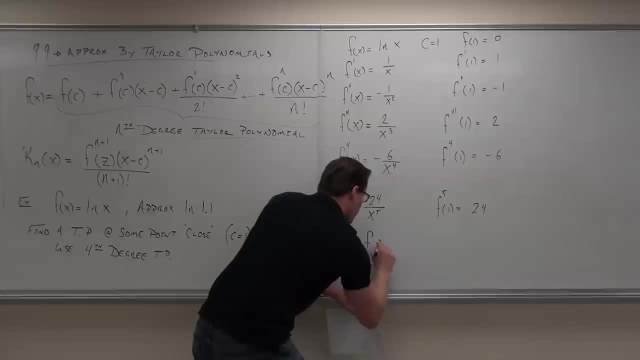 f of c would. f of 1 would be 0. So we'd have f of 1. 1. Are you guys with me on this? Are you sure you're with me? I don't want to lose you right now, right. 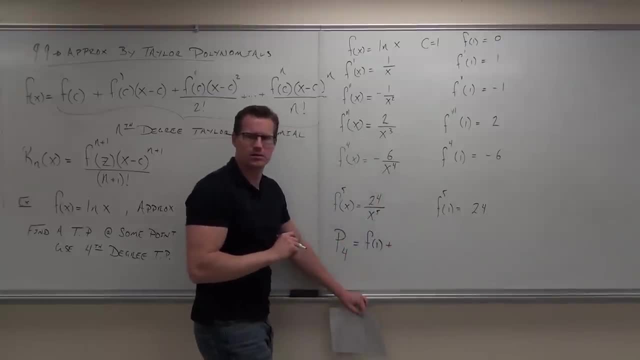 We've been doing this for a while now. Plus what's the next one? f prime of c. Okay, f prime of 1. And then you would have x minus x minus 1.. You're right, It's x minus c, but in our case our c is 1.. 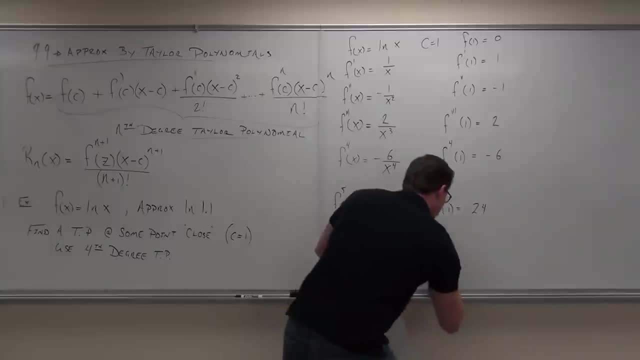 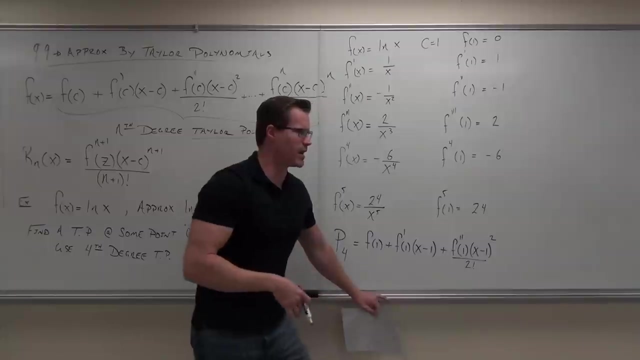 Are you okay with that one? Mm-hmm. Okay, what's the next one? f, double prime of 1.. And then you would have x minus 1 squared, squared Over. Yeah, it's 2 factorial. I'm going to change that to 2 in just a second, but just so we have the pattern here. 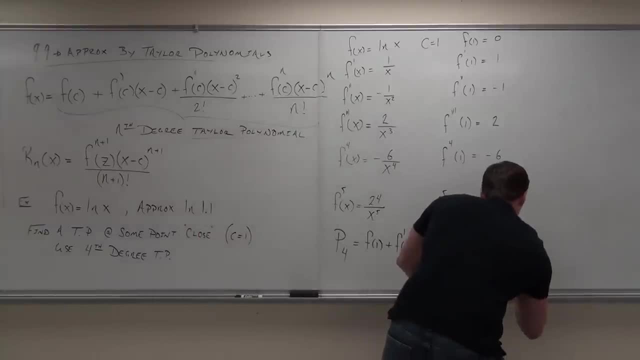 Keep on going. What next? Triple prime of 1.. x minus c to the Third. So we're going to have x minus 1 to the third, All over 3 factorial Plus. keep on going. What is it? 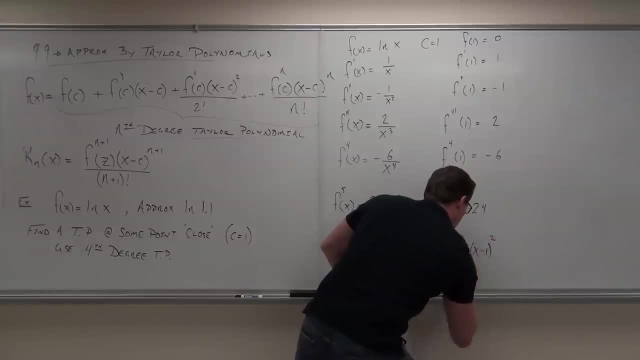 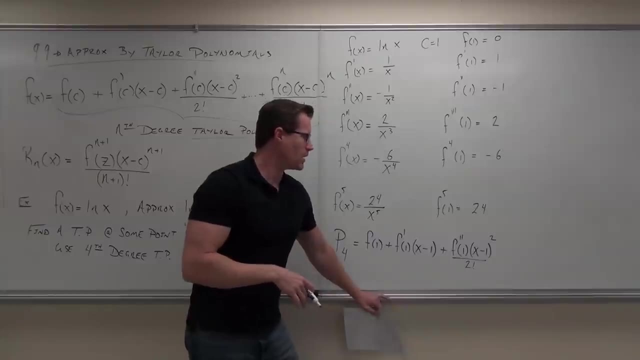 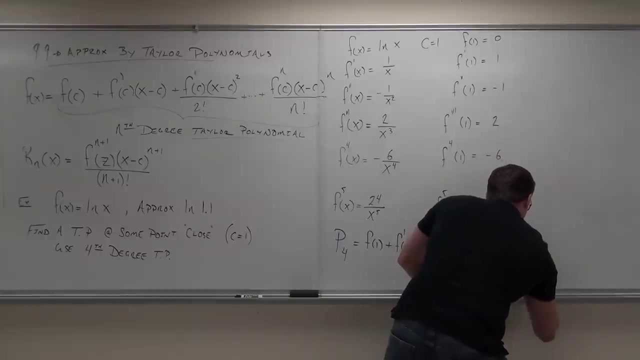 Over. Yeah, it's two factorial. I'm going to change that to two in just a second, but just so we have the pattern here. Keep on going. What next? Triple prime of one X minus c to the Third. 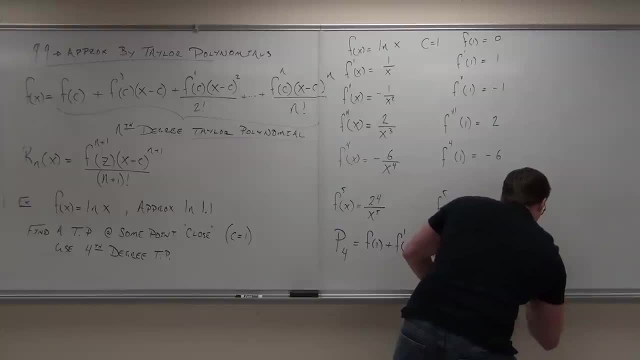 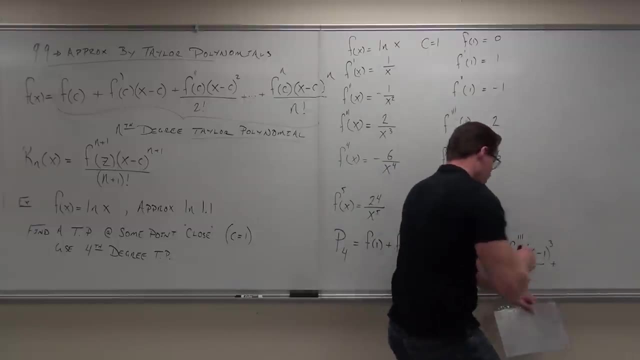 So we're going to have x minus one to the third, All over three factorial Plus. keep on going. What is it? F? triple prime of one? Oh, yeah, the triple prime F factorial of one. Yeah, F, yeah. 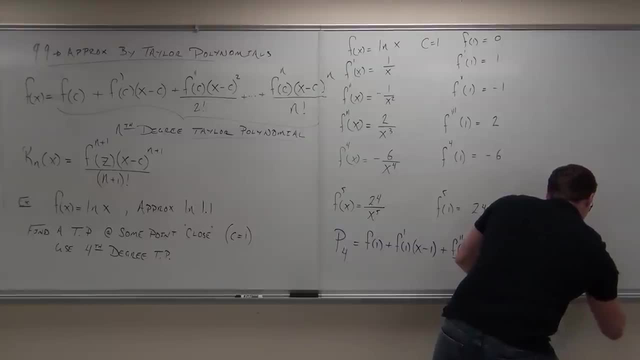 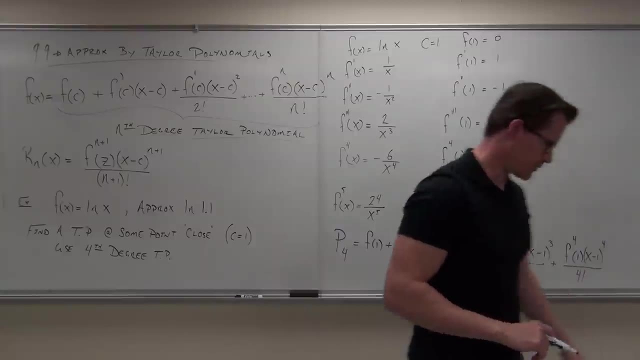 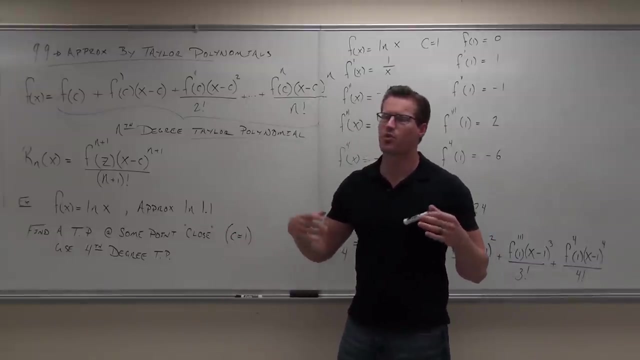 That's it, That's it, That's it. Yeah, Okay, let's see if we're all okay with that one so far. I want to really make sure. So we start off. basically, a Taylor polynomial is just part of a Taylor series, So we're. 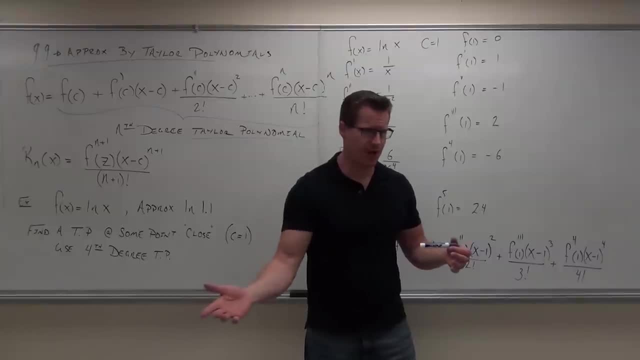 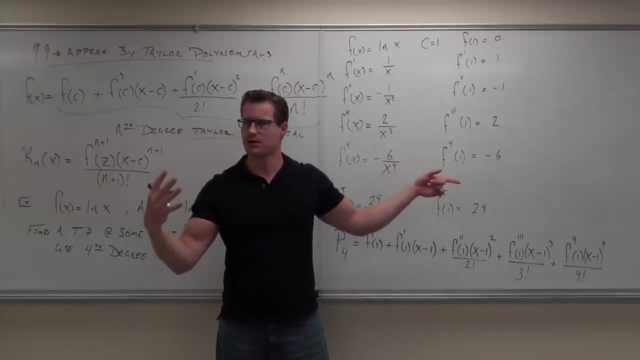 practically doing the same thing, but it's easier. It's easier because you don't need to find a pattern. All you got to do is, hey, find out whatever derivative that you need. So if I say degree four, you're going to find out the fourth derivative. yeah, Plus one. 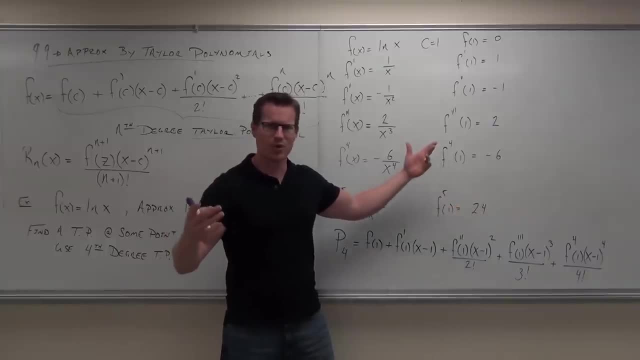 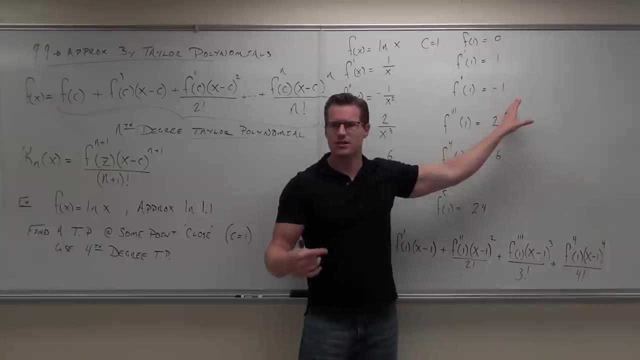 The plus one is for your error, Quick hit. if you're okay with that one, Plug in the point, No problem, You're going to have the C. I've told you what it is here Generally it's going to be given to you. So plug in your C, Not a problem. Do you see that this? 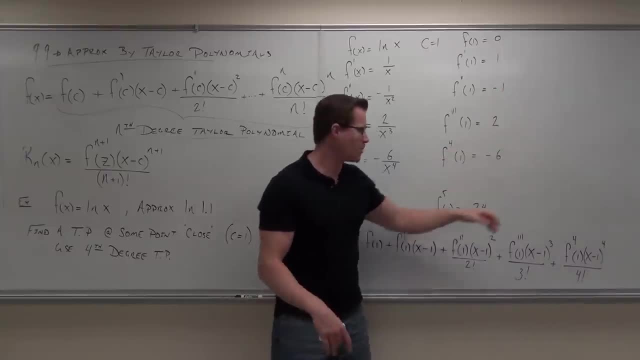 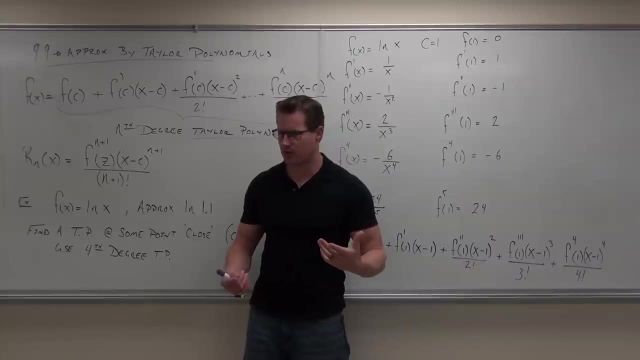 is exactly the same as the Taylor series. so far. Find these points, No problem. Now make up your Taylor polynomial. A Taylor polynomial don't need a pattern, because it stops at a certain degree, It's finite, It does not go forever. So if I say, find the tenth degree, 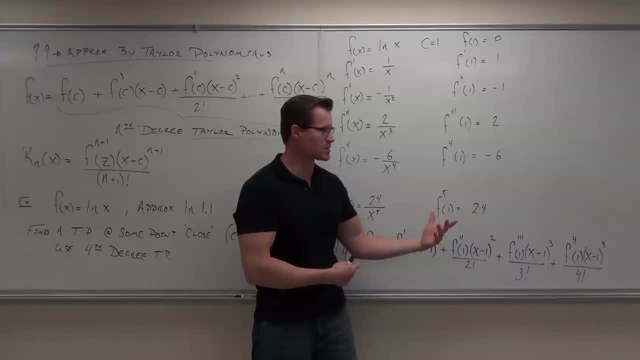 yeah, that sucks, but at least you're going to be able to do it and stop somewhere. Does that make sense? Mm-hmm, It does not need to go to infinity. So if I say fourth degree, you do well, here's. 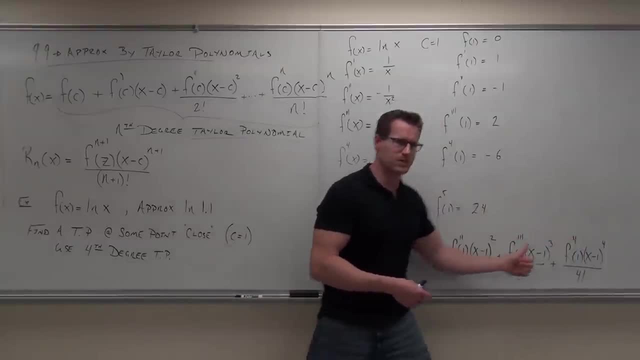 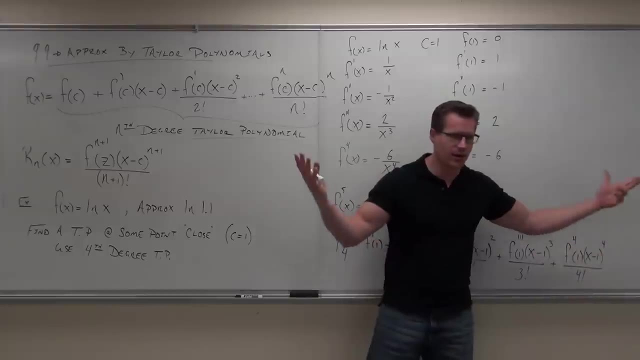 the zero degree. One, two, three. Let's stop at four. Fourth degree, Taylor polynomial says we stop at the fourth derivative. It's a degree four polynomial. You see the degree four I'm talking about. That's what it is, Making sense. so 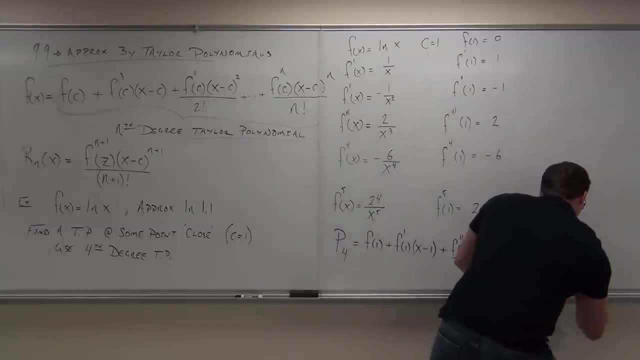 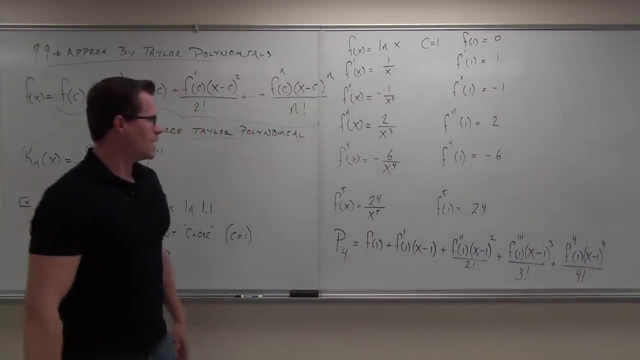 f, triple prime of 1.. Oh, we have the triple prime f, triple prime of 1.. Yeah, f, yeah, Okay, let's see if we're all okay with that one so far. I want to really make sure. 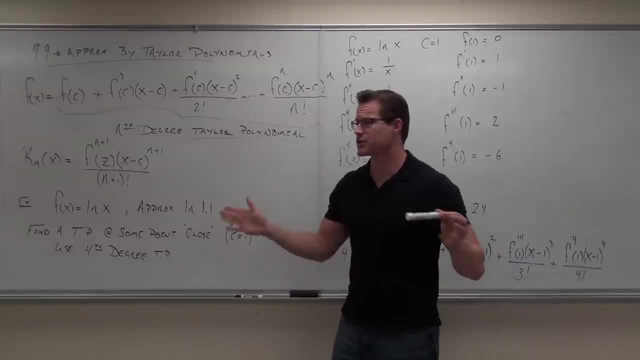 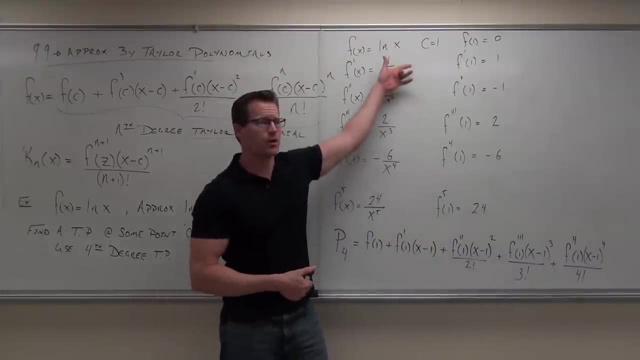 So we start off. basically, a Taylor polynomial is just part of a Taylor series, So we're practically doing the same thing, but it's easier. It's easier because you don't need to find a pattern. All you've got to do is, hey, find out whatever derivative that you need. 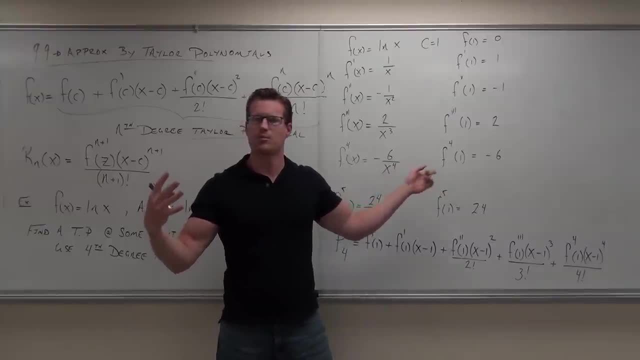 So if I say degree 4, you're going to find out the fourth derivative: Yeah Plus 1.. The plus 1 is for your error, Quick handout. if you're okay with that one, Plug in the point, No problem. 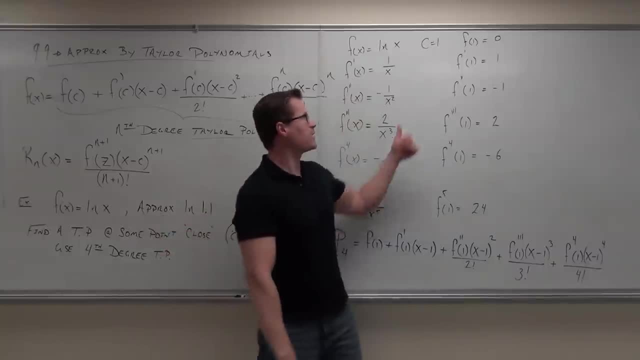 You're going to have the c. I've told you what it is here Generally. it's going to be given to you, So plug in your c, Not a problem. Do you see that? this is exactly the same as the Taylor series so far? 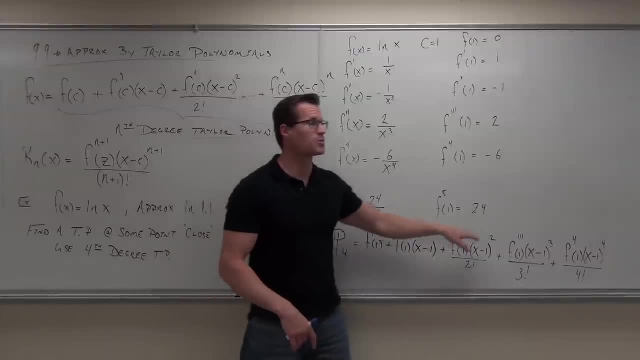 Find these points, No problem. Now make up your Taylor polynomial. A Taylor polynomial don't need a pattern, because it stops at a certain degree, It's finite, It does not go forever. So if I say, find the tenth degree, yeah, that sucks. 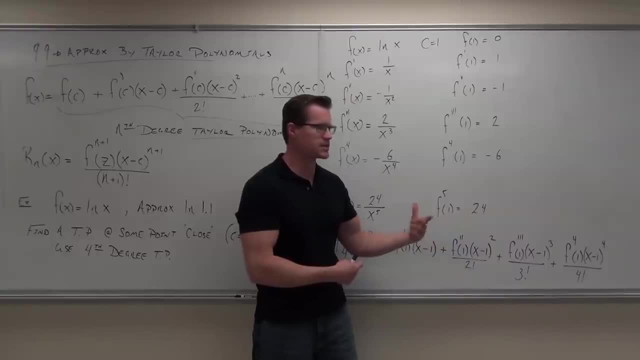 But at least you're going to be able to do it and stop somewhere. Does that make sense? It does not need to go to infinity. So if I say, fourth degree, do. well. here's the zero degree: 1,, 2,, 3.. 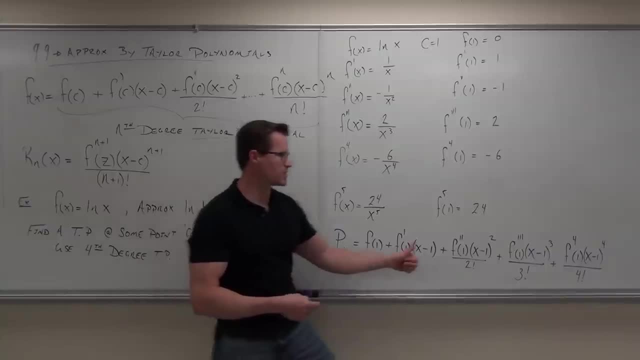 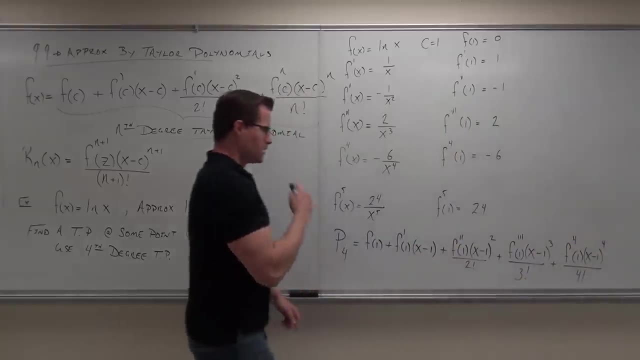 Let's stop at 4.. Fourth degree: Taylor polynomial says we stop at the fourth derivative. It's a degree 4 polynomial. You see the degree 4 I'm talking about. That's what it is Making sense so far. Now you might want to simplify it. 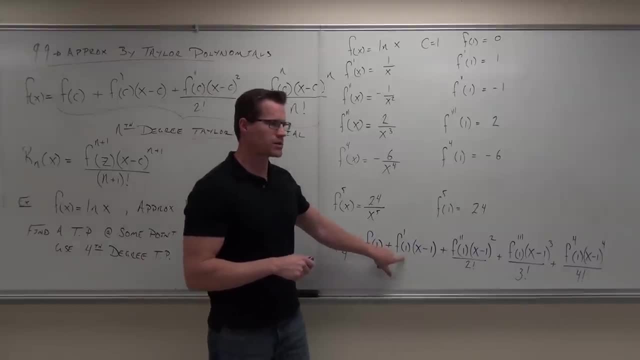 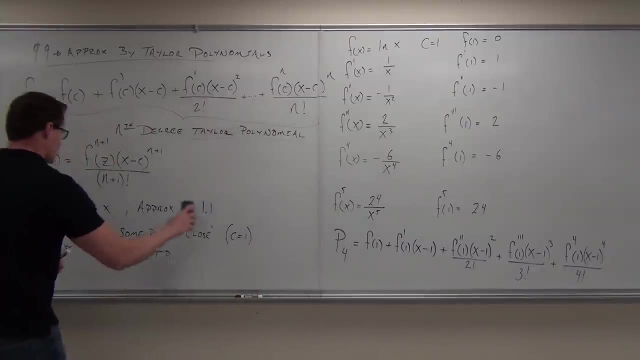 Do we know what f of 1 is? Yeah, Do we know what f of 1 is? Yes, We know what all those things are. Plug in those numbers. So let's do that. I'm going to leave this here. 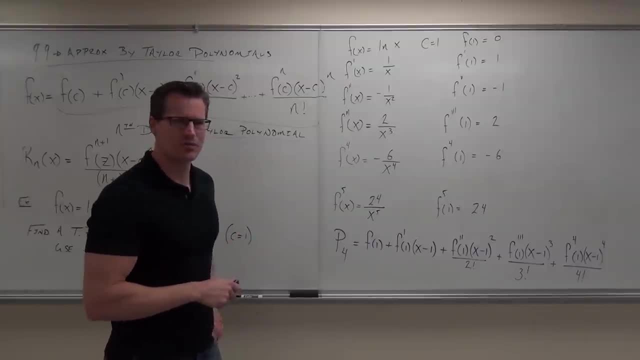 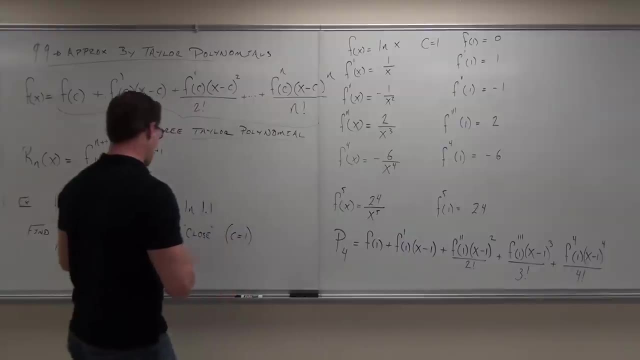 far Mm-hmm. Now you might want to simplify it. Do we know what f of one is? Yes, And f prime of one is Yes. We know what all those things are. Plug in those numbers. So let's do that. I'm going. 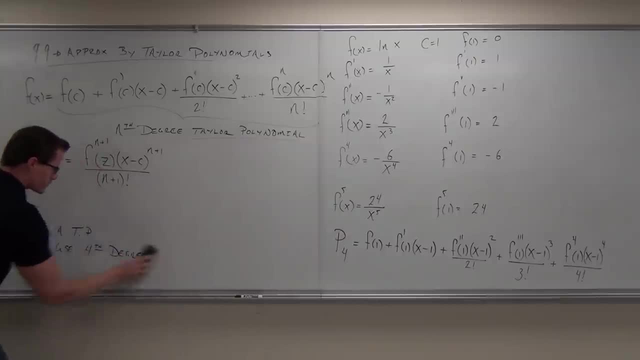 I'm going to work down here for a second. Unfortunately, these boards are quite small, So the fourth degree Taylor polynomial is what's the first thing we're going to start with? Zero, Zero, Yeah, And then what? 1.. 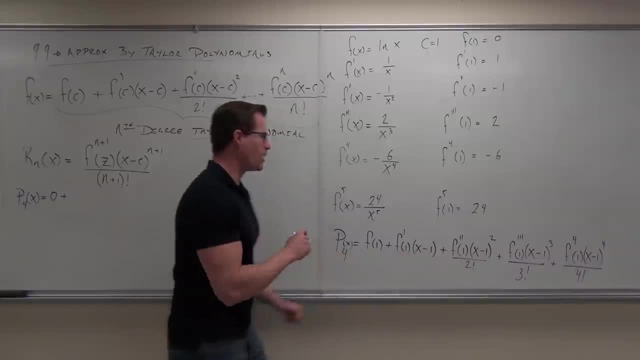 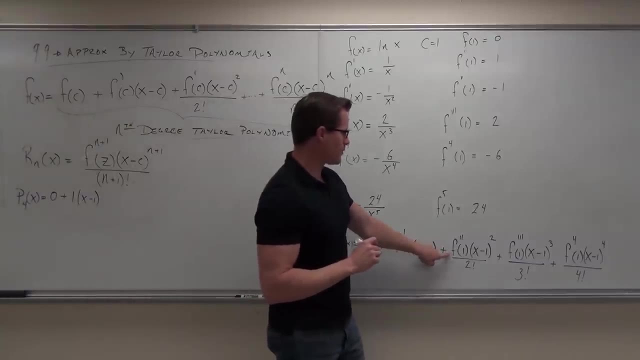 Yes. So if it says f prime of 1 is 1, then right here we have 1.. So what's our first f prime of 1.. Mm-hmm, And then we're going to go: OK, now let's add to it f double prime of 1.. 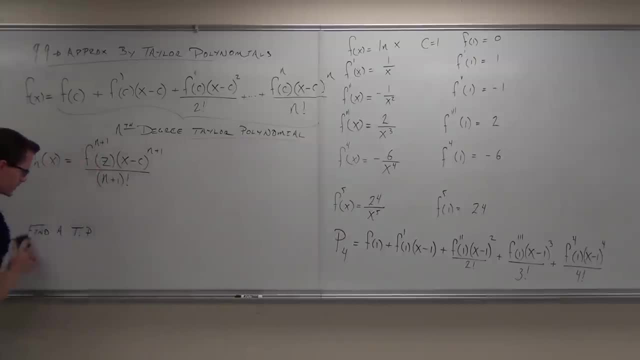 to leave this here. I'm going to work this out. I'm going to write it down here for a second. Unfortunately, these boards are quite small, So the fourth degree Taylor polynomial is what's the first thing we're going to start? 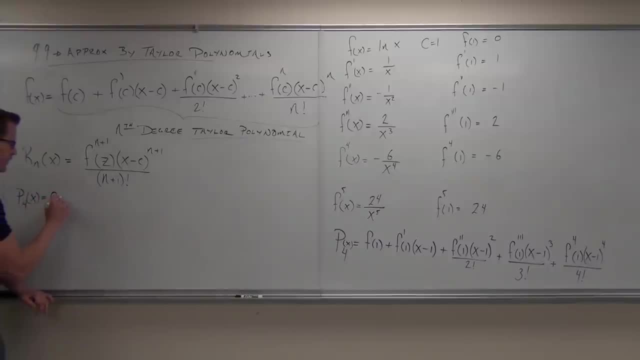 with One Zero, Zero, Yeah. And then what One, Yes? So if it says f prime of one is one, then right here we have one. So what's our first F prime of one? Mm-hmm. 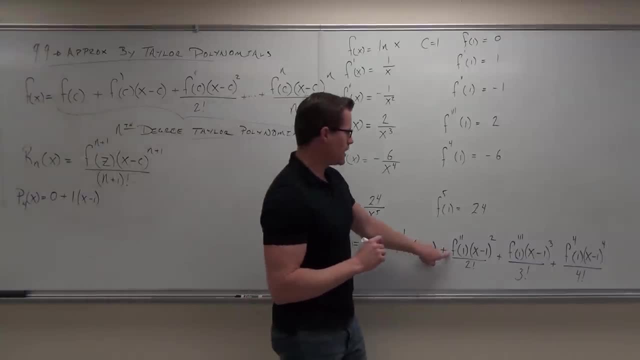 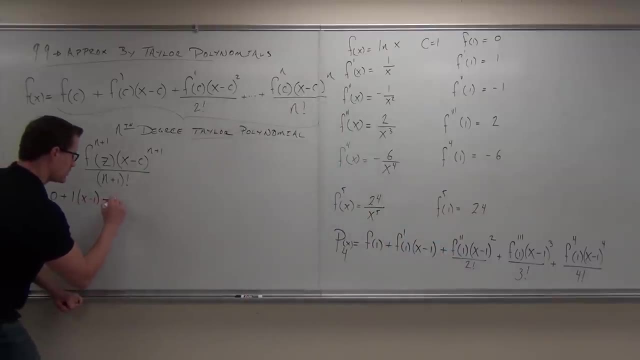 And then we're going to go: okay, now let's add to it f double prime of one. What's f double prime of one Negative one? Oh, okay, So we're going to have minus x, minus one squared over two. factorial is simply: 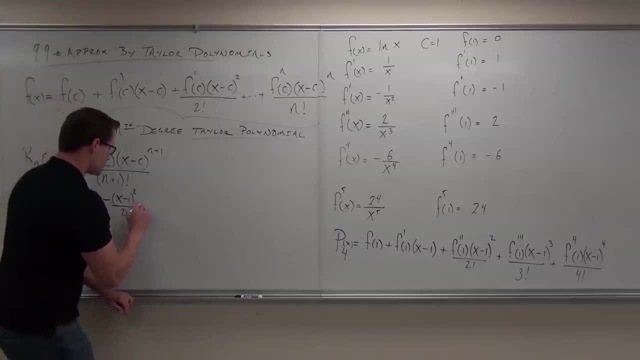 two: Okay, we can do that. What's after that? Two: Yeah, let's do f triple prime. F triple prime is two, but it's still a plus. So plus two Times x minus one, X minus one to the. 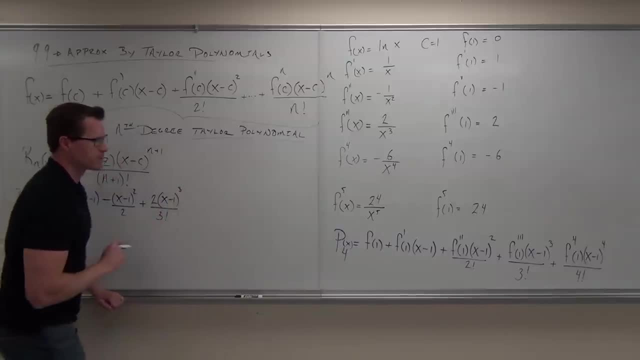 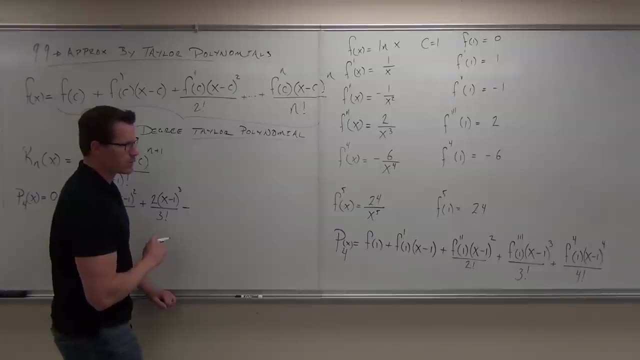 Over two, Over two: factorial Perfect. Okay, and then where are we at now? Minus, Minus. Why are we having a minus here? Negative six, Negative six. So we're going to have minus six x minus one to the fourth over four: factorial Do. 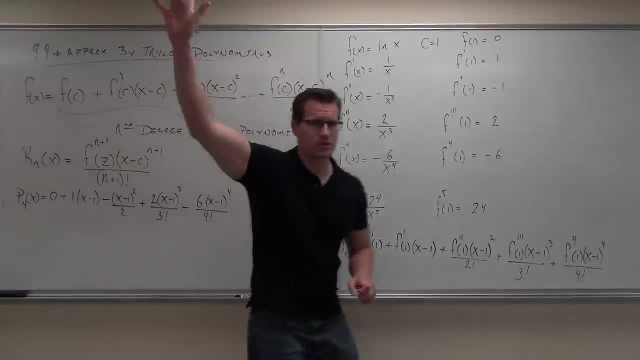 we go any further than that right there? No, Okay, should we be okay with that so far? So all we've done: we've taken these numbers, we've plugged them into their appropriate spots in our fourth degree Taylor polynomial. this is exactly what we have. 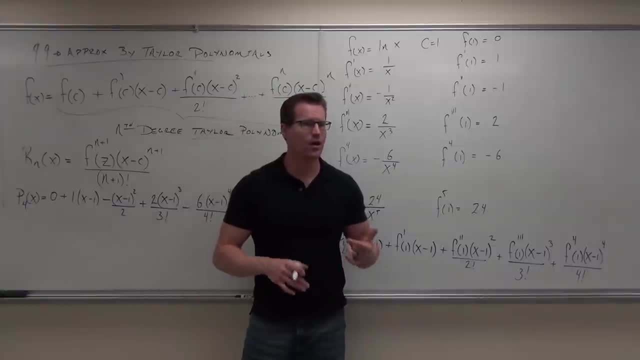 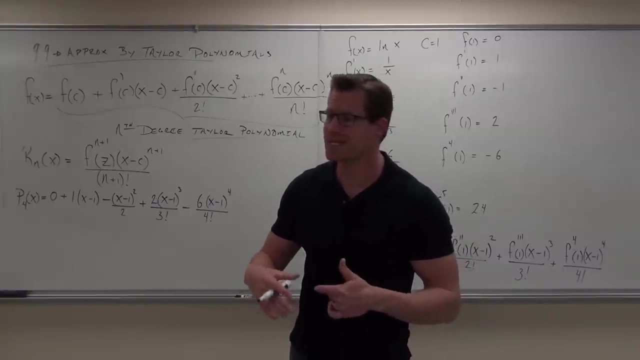 Okay, We're going to simplify this stuff, make it easy. Remember. what we're doing here is we're going to use this Taylor polynomial as an approximation. What that means is that we want it to be easy to plug a number into, So let's do it. So, if we make this easier, 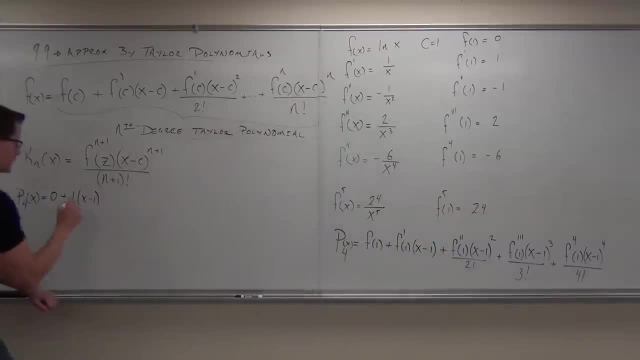 What's f double prime of 1? Negative 1.. OK, So we're going to have minus x minus 1 squared over 2, factorial is simply 2.. OK, We can do that. What's after that? 2.? 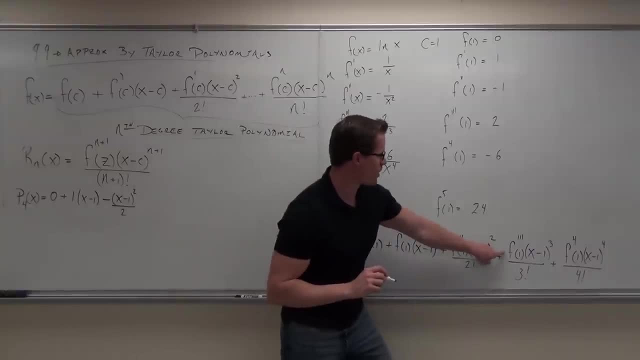 Yeah, Let's do f triple prime. f triple prime is 2, but it's still a plus. So plus 2 times x minus 1.. x minus 1 to the Over, 2. Over 2. Perfect OK. 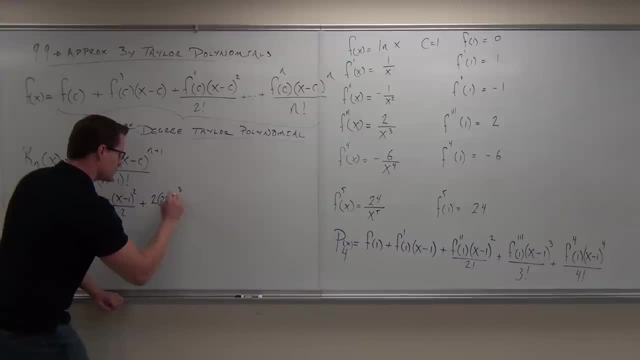 And then where are we at now? Minus, Minus. Why are we having a minus here? Negative 6.. Negative 6.. So we're going to have minus 6x, minus 1 to the fourth over 4 factorial. 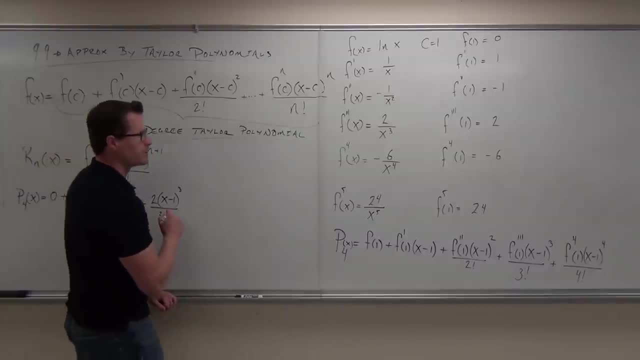 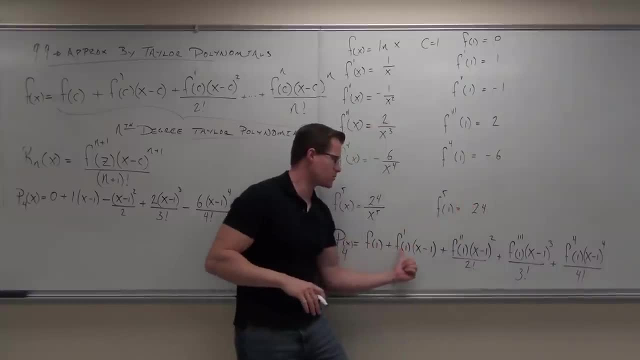 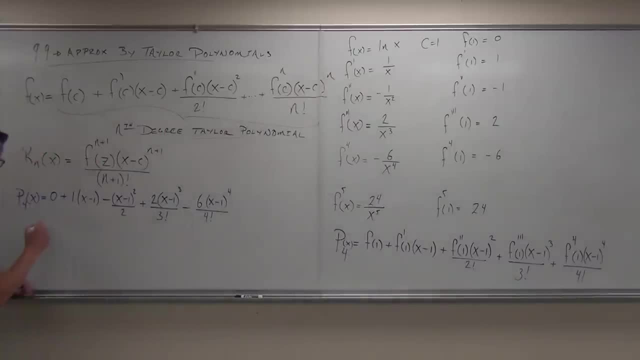 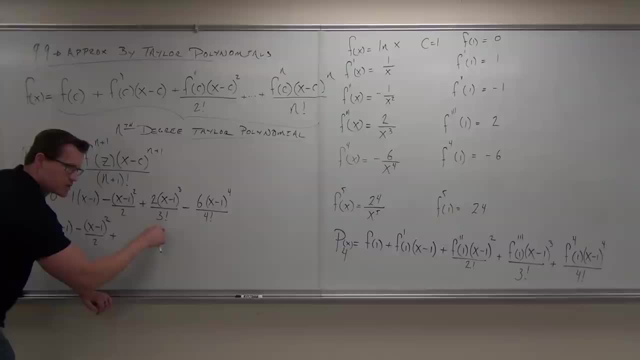 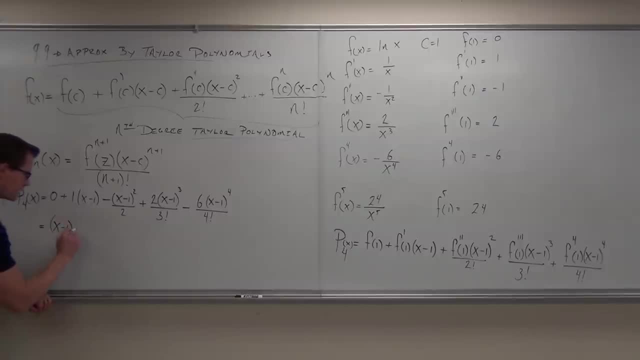 zero's gone, we get x minus one. we get minus x minus one. squared over two, we get plus. do you see that this is going to be three times two times one? Mm-hmm, So our twos are going to simplify, I'm going to get. 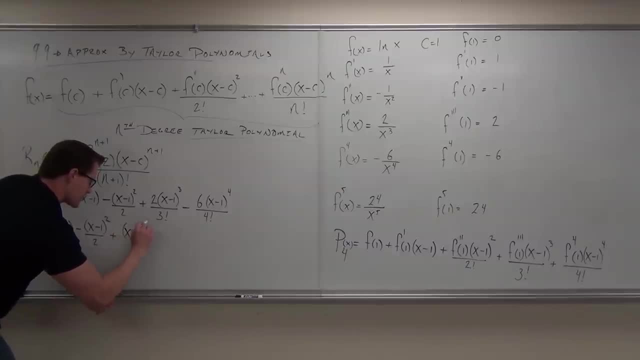 Three, Three X minus one. to the third, over three minus. do you see that this is four times three times two and this is three times two, Mm-hmm Four. Do I keep going? No, No, Taylor, polynomial. stop at whatever degree I say, whatever degree the problem says. 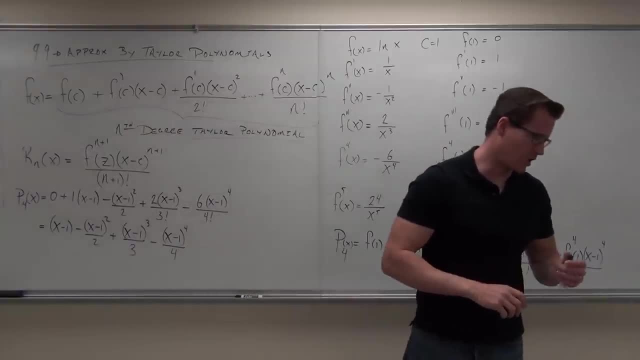 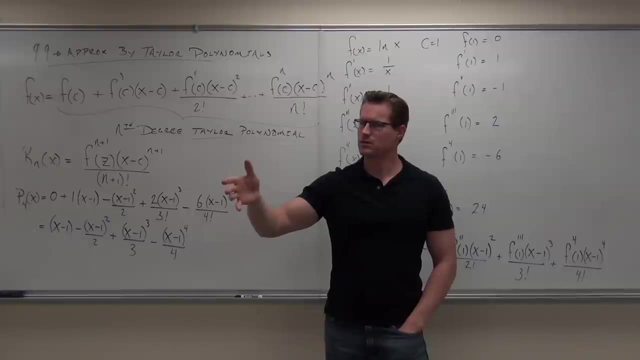 What I want to know is show of hands. if that one makes sense to you. so far, Okay. so Taylor polynomial, Okay. so yes, no, Yes, You see where all the things come from. Mm-hmm. So now here's the plan. If this is the fourth degree, Taylor polynomial, basically. 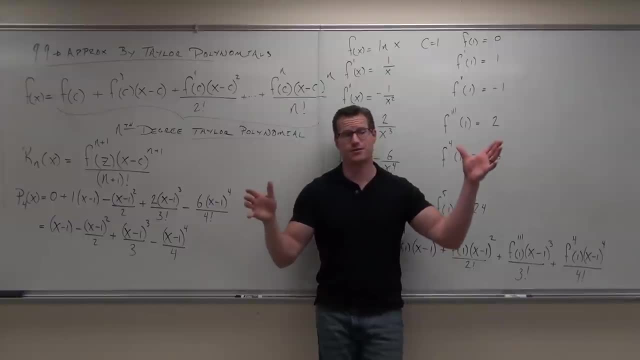 it says we've stopped our Taylor series after five terms. The first one is no derivative, so after five terms we've stopped. You got me: Yes, This is going to be an approximation. Now how good. We're going to determine that. 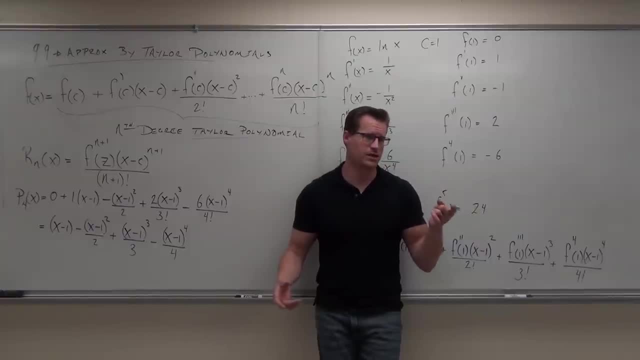 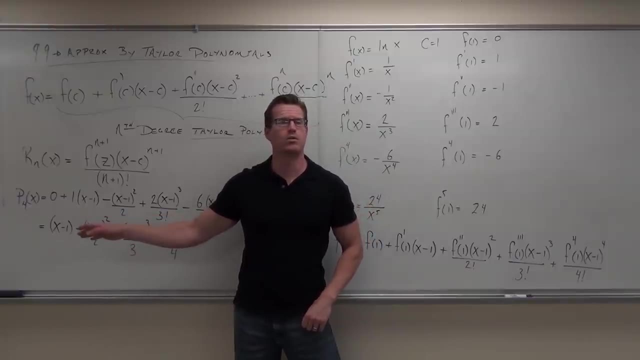 in a minute but you can't approximate it. Notice what it says. It says we base this on something that's really close to the number we're trying to approximate. Our c was one That's really close to 1.1.. So if I wanted to approximate ln of 1.1, here's what it. 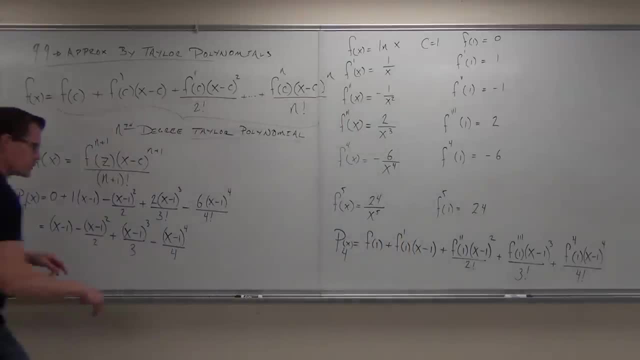 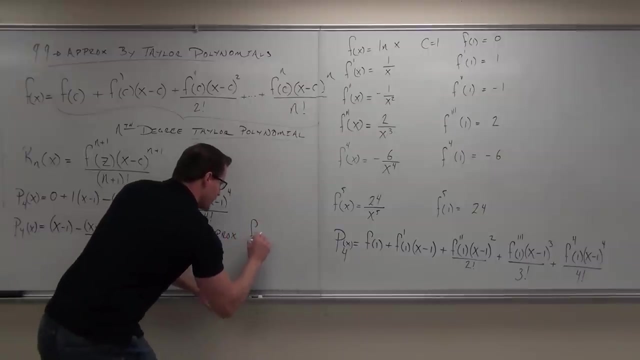 says? It says that this Taylor polynomial, this degree four Taylor polynomial, represents or approximates. this thing approximates: f of x equals ln x around f of x. Now, what does that mean? It means that f of x is equal to f of x, minus f of x, minus f of x. 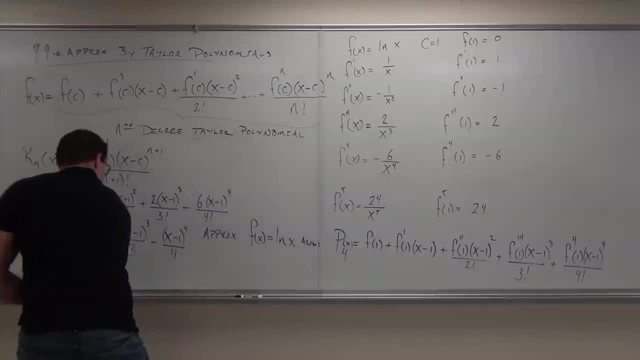 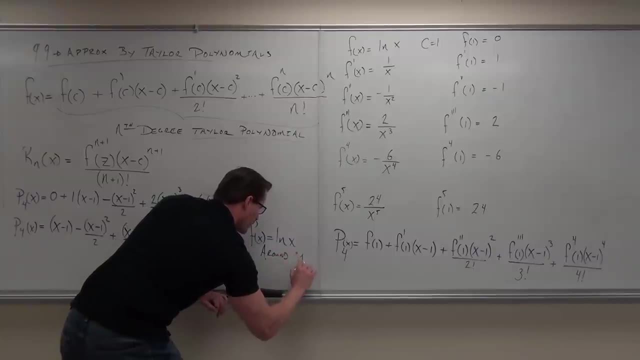 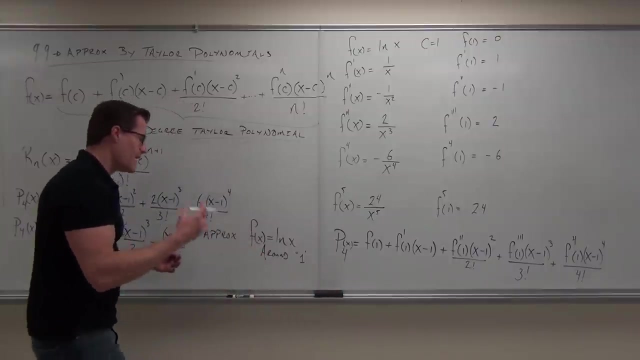 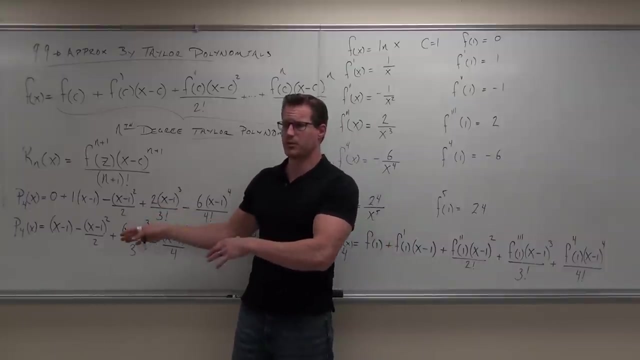 Okay, So if we want to approximate ln of 1.1, all we need to do is plug in 1.1 to our Taylor polynomial. Does that make sense? Yes, I'll say that one more time. What we've done so far is say: hey, you know what we've got. 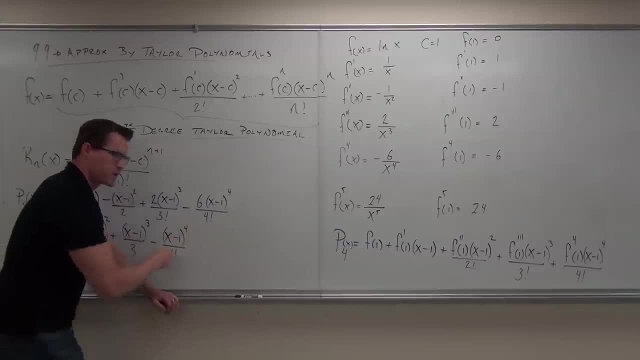 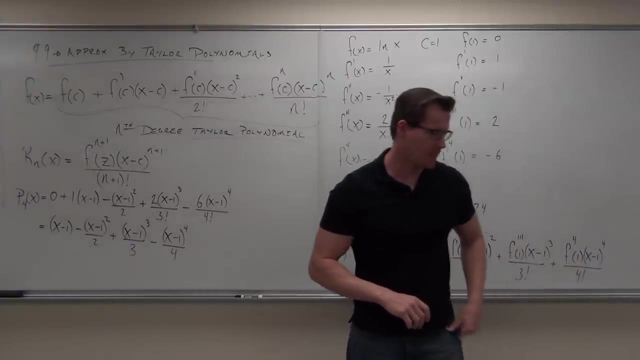 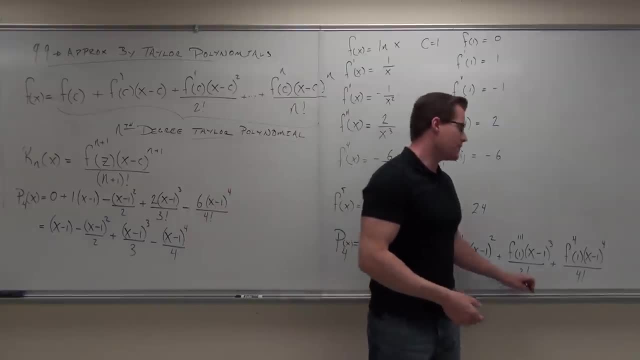 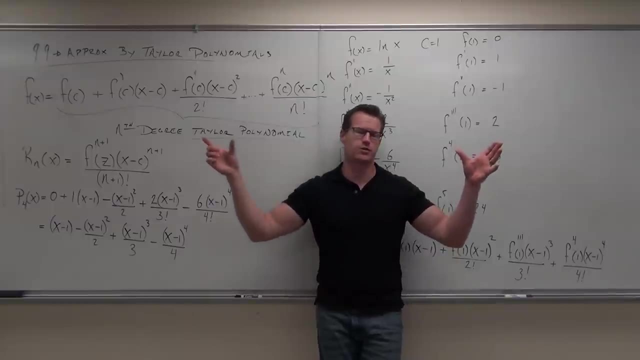 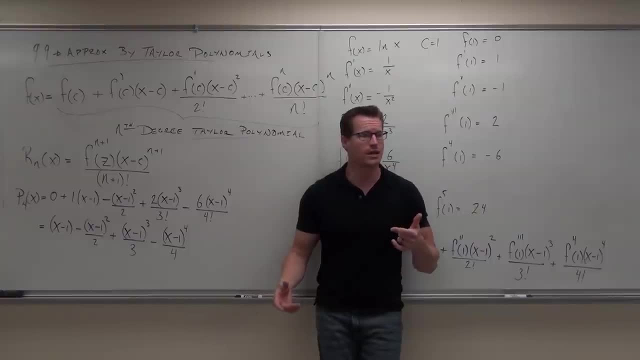 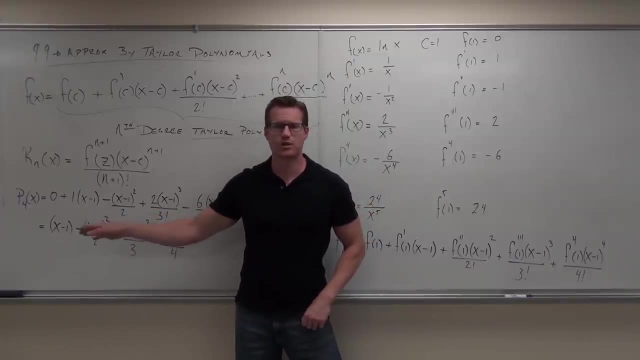 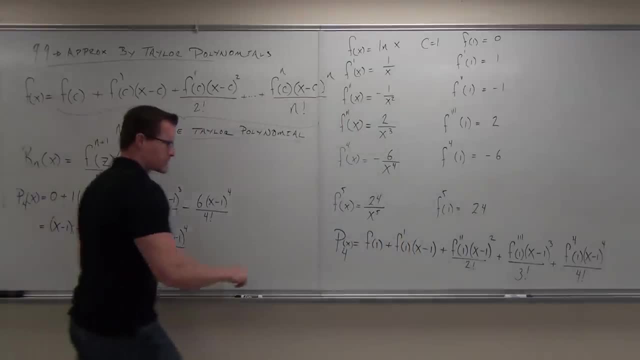 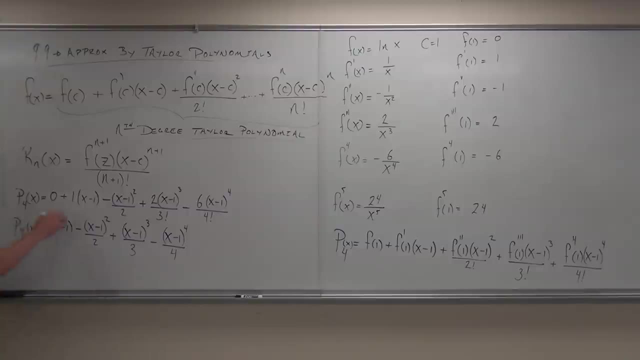 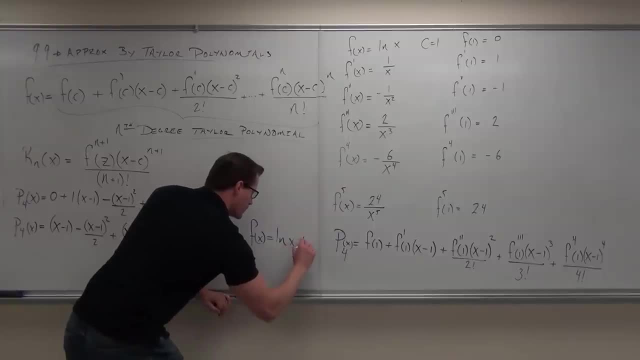 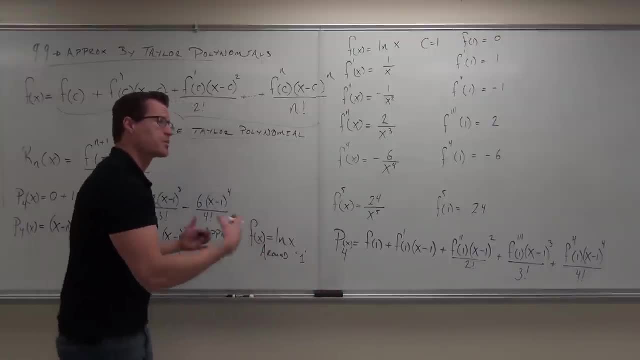 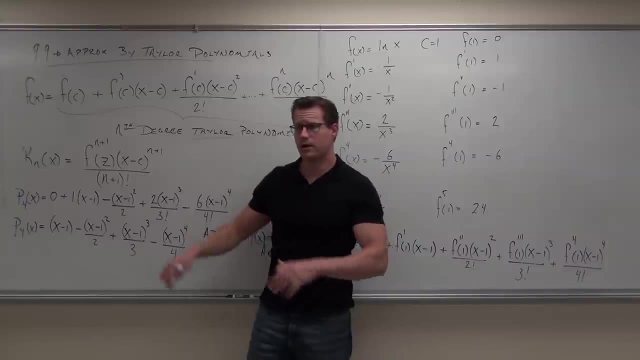 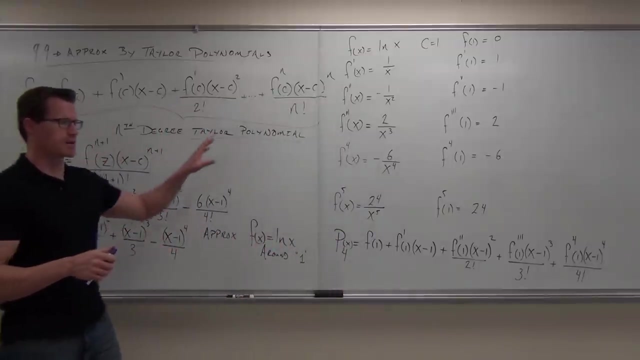 Minus, Minus, Minus, Minus. approximate ln of 1.1, all we need to do is plug in 1.1 to our Taylor polynomial. Does that make sense? I'll say that one more time. What we've done so far is say: hey, you know what? 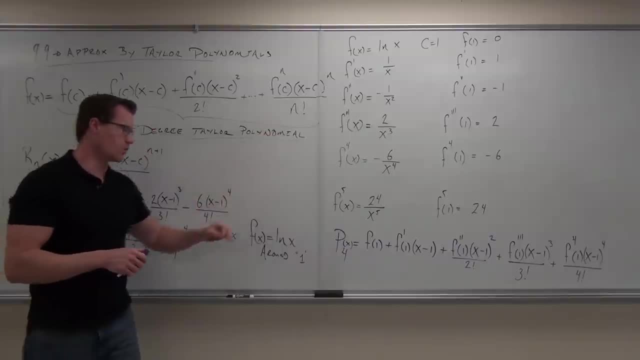 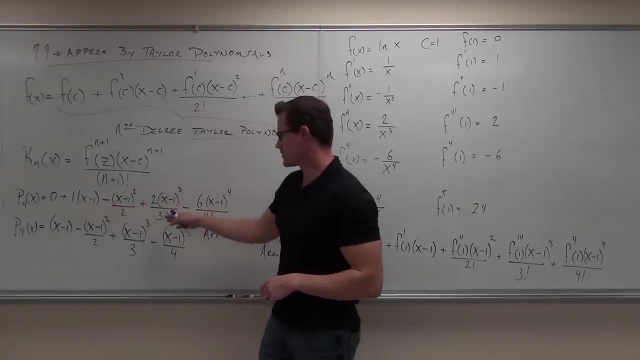 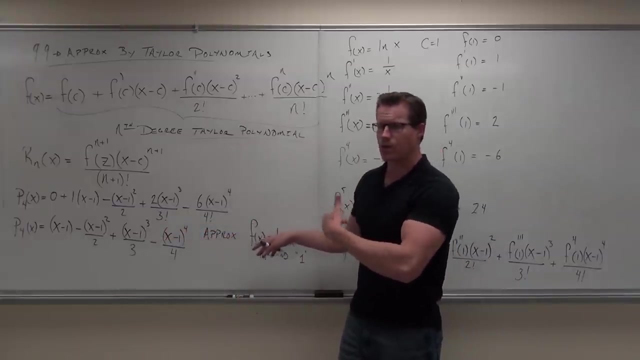 we've got a Taylor series, let's cut it off. That's gonna be an approximation. So this cut off Taylor series at the fourth derivative says that our fourth degree Taylor polynomial is going to approximate the function where we got that thing from around a certain point. 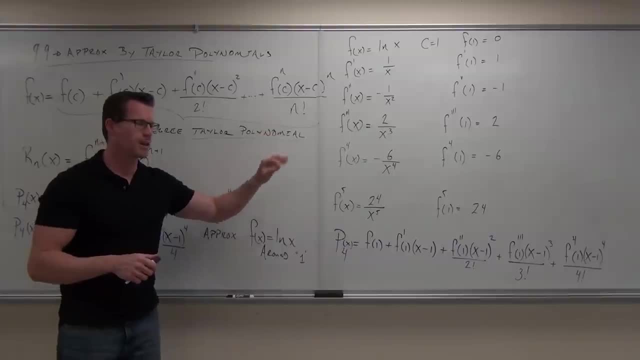 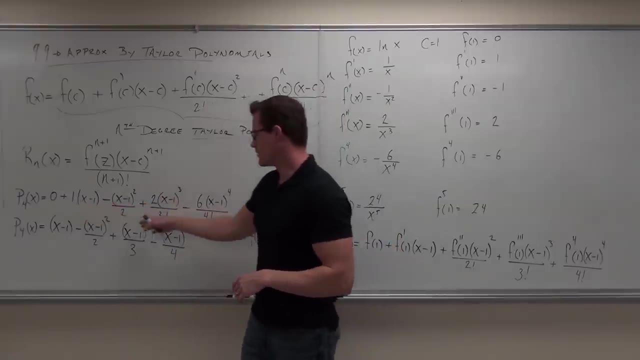 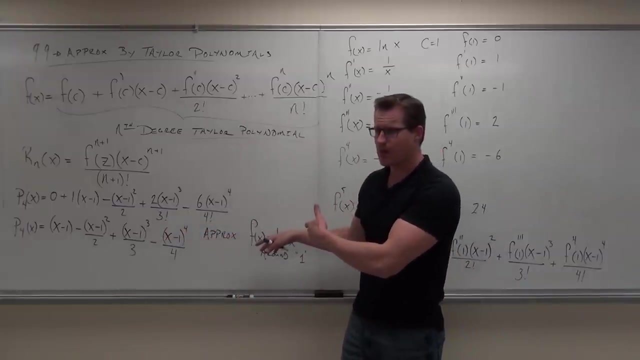 a Taylor series, Let's cut it off. That's going to be an approximation. So this cut off Taylor series at the fourth derivative says that our fourth degree Taylor polynomial is going to approximate the function where we got that thing from around a certain point. That certain point that we picked was around. 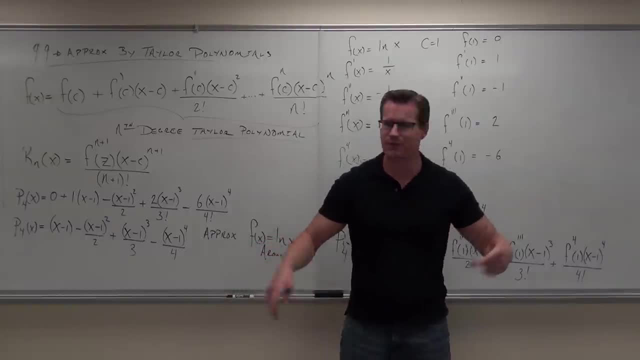 That certain point that we picked was around the point c equals to one. So while we have an x minus one up there, that's our center. Quick head on, if you're all right with that one. So if I wanted to find ln of 1.1,. 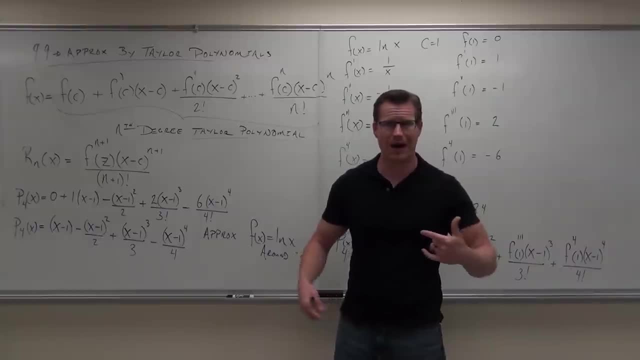 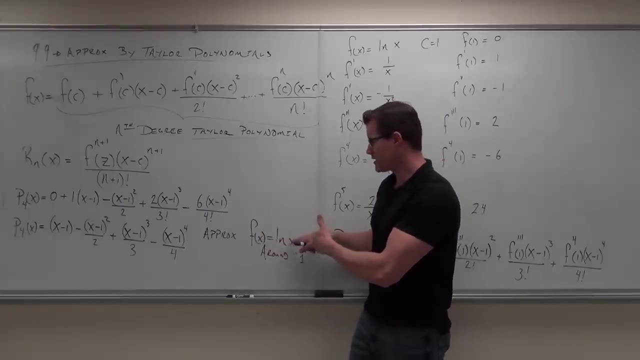 all I have to do is plug in 1.1 for my. if this is f of x equals ln of x, and I want to find out 1.1, this x, that's this x. So if I want to approximate- 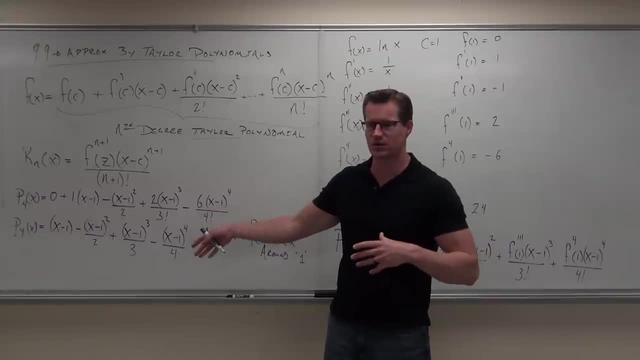 the point c equals to 1.. So while we have an x minus 1 up there, that's our center. Quick head on, if you're all right with that one. So if I wanted to find ln of 1.1, all I have to do is plug in 1.1 for my. yeah, if this. 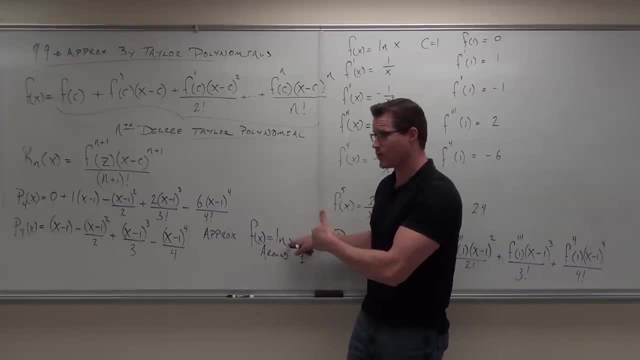 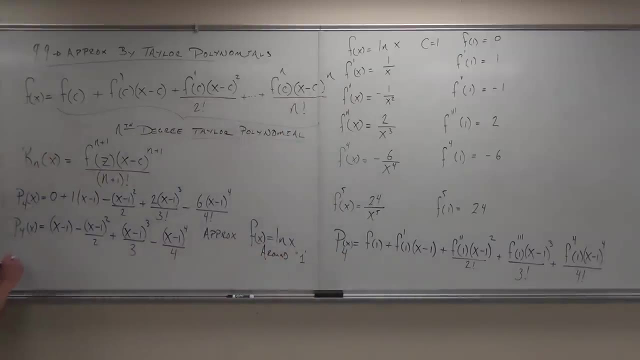 is f of x equals ln of x, and I want to find out 1.1, this x, that's this x. So if I want to approximate ln of 1.1,, all I've got to do is find p, sub 4 of 1.1.. 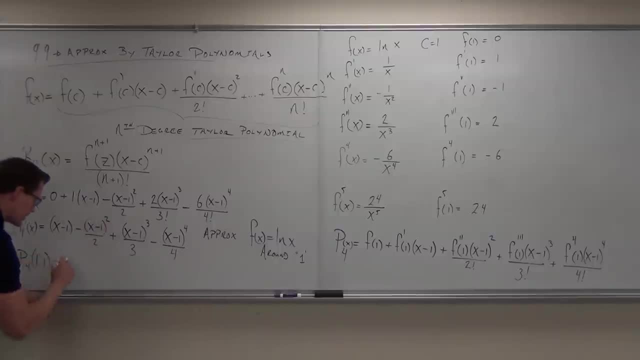 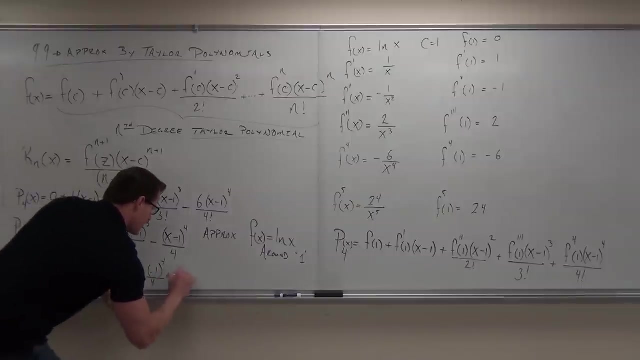 What that ends up being is 0.1 minus 0.1 squared over 2, plus 0.1 to the third over 3, minus 0.1 to the fourth over 4.. Now this is an approximation for f of x. 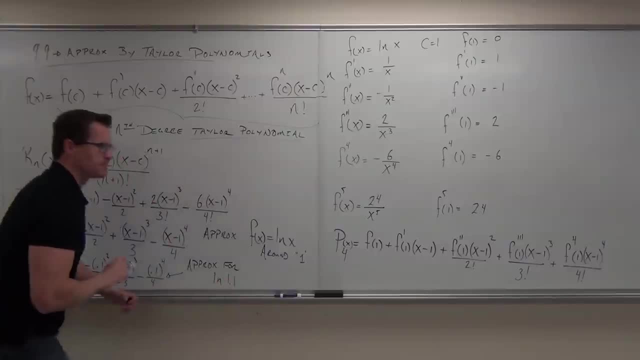 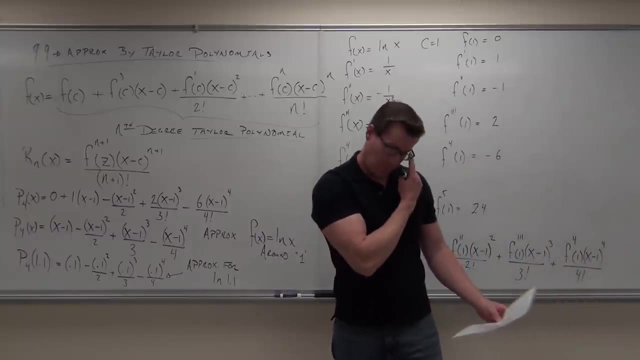 This is an approximation for ln of 1.1.. I've got to make sure that this all makes sense to you because I'm of course your teacher here. So do you guys get the idea that if I cut a Taylor series short for a 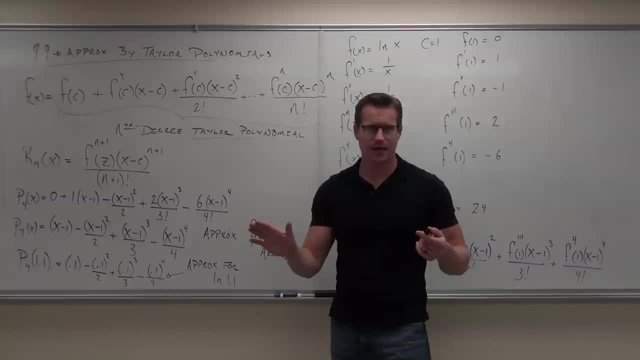 Taylor polynomial. it's an approximation, Mm-hmm. Do you get the idea that if I want it to be close to a certain point, I'm going to have a certain number I'm trying to approximate, then that's what my center's going to become. 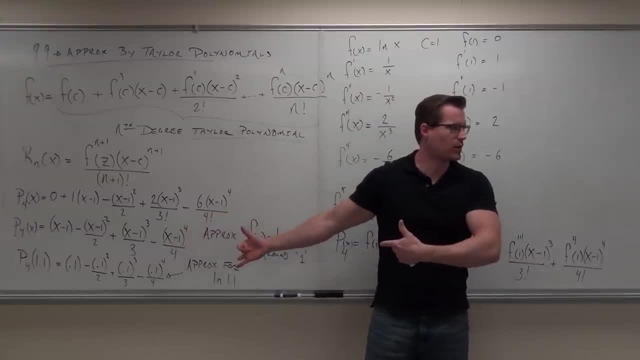 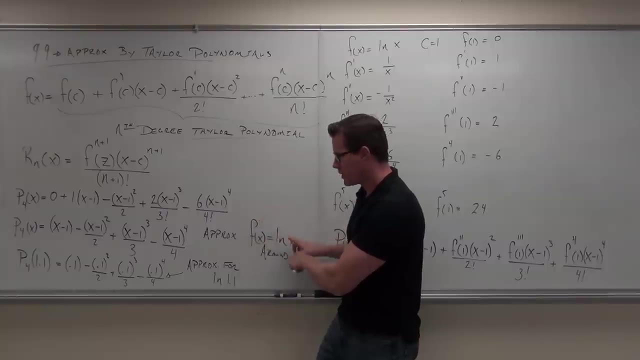 So here our center's 1, because it's really close to 1.1.. All right, Well, do you also understand that if I want to approximate my function, all I have to do is plug in the number into my Taylor polynomial? Do you guys get that idea? 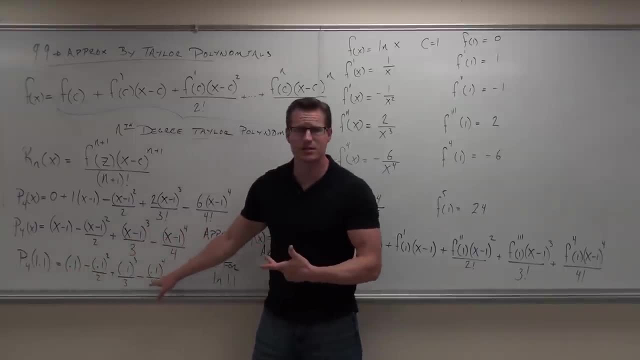 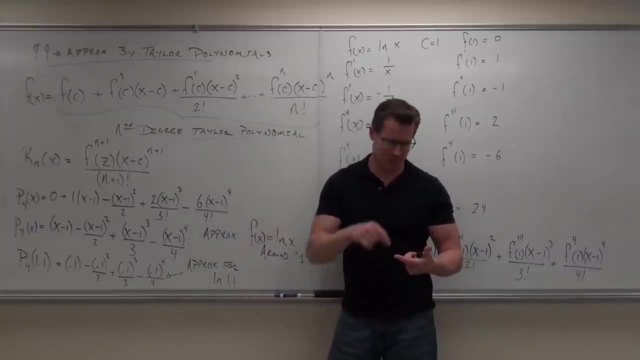 Yes. So if I were to work this out on a calculator, whatever this is, it's going to be pretty darn close to ln of 1.1.. Now we of course have calculators, right, So we let's do 1.1ln. 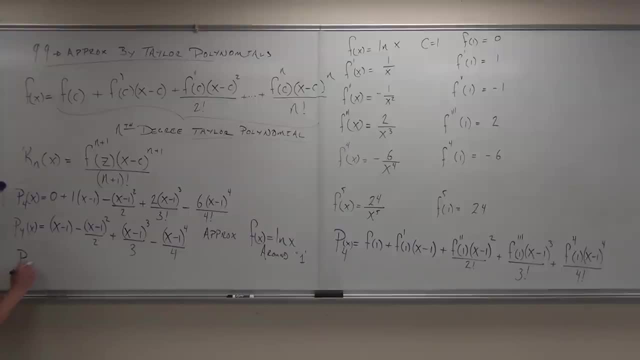 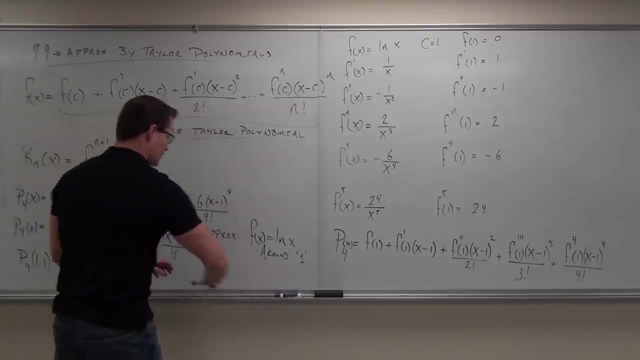 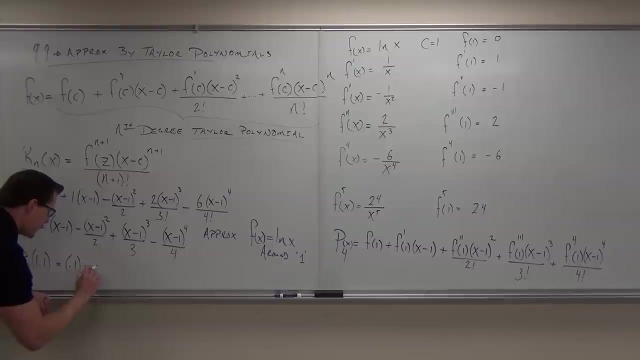 ln of 1.1, all I'm gonna do is find p sub four of 1.1.. What that ends up being is .1 minus .1 squared over two, plus .1 to the third over three, minus .1 to the fourth over four. 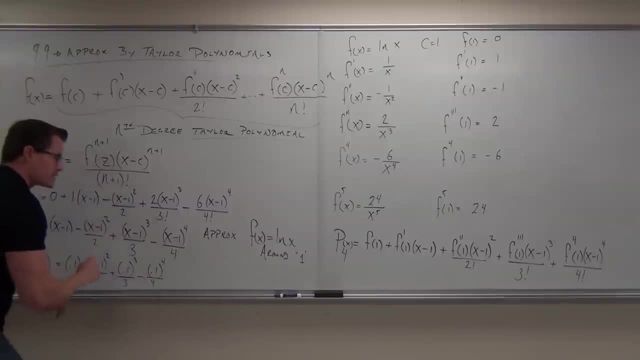 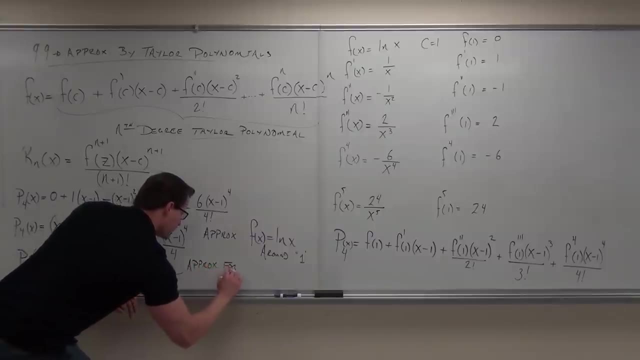 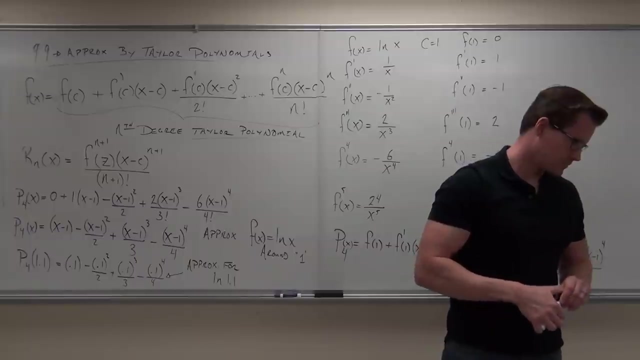 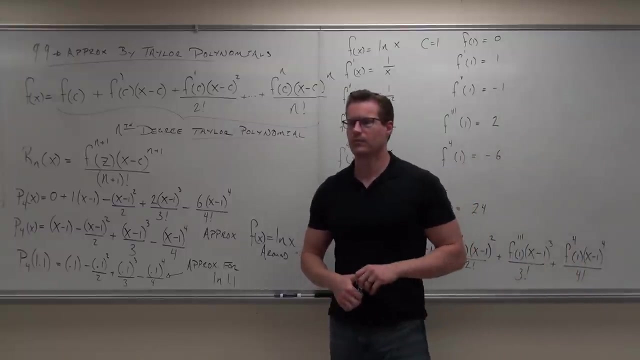 Now, this is an approximation for ln of 1.1.. Now, this is an approximation for ln of 1.1.. I gotta make sure that this all makes sense to you, because I'm, of course, your teacher here. 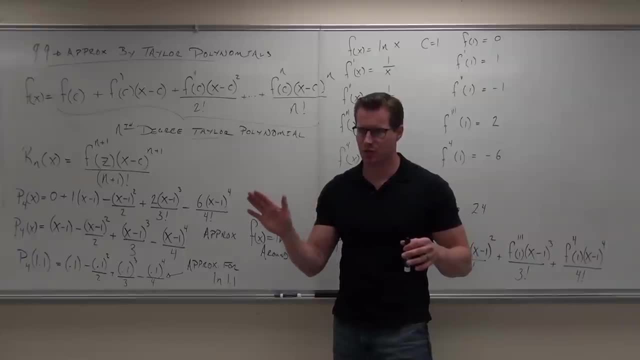 So do you guys get the idea that if I cut a Taylor series short for Taylor polynomial, it's an approximation? Do you get the idea that if I want it to be close to a certain number, I'm trying to approximate? then that's what my center's going to become. 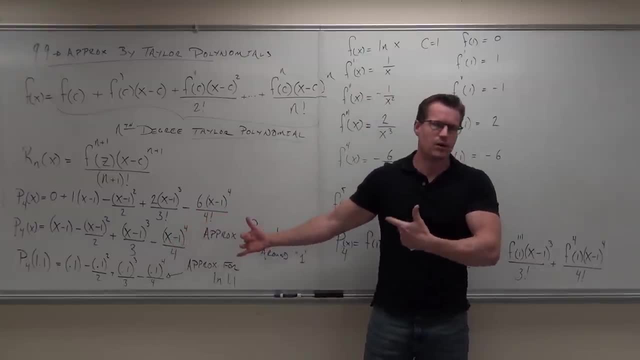 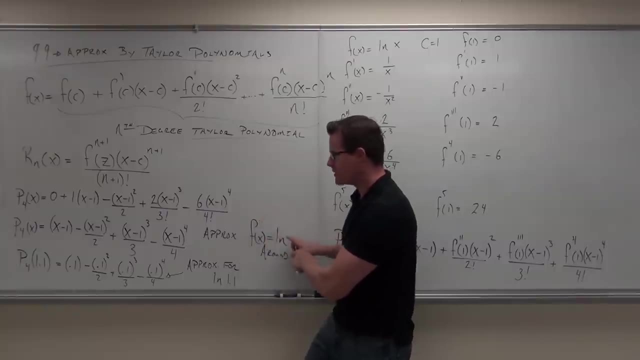 So here our center's one, because it's really close to 1.1.. All right, well, do you also understand that if I want to approximate my function, all I have to do is plug in the number into my Taylor polynomial? 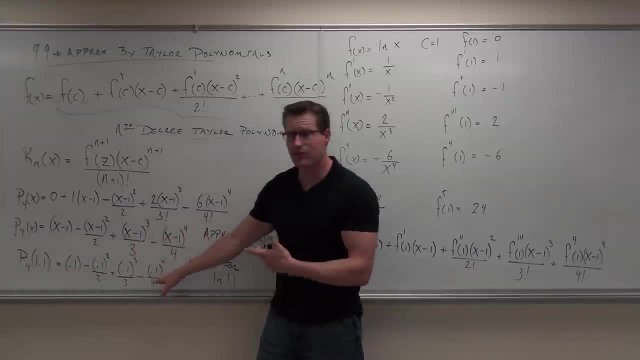 Do you guys get that idea? Yes, So if I were to work this out on the calculator, whatever this is- I'm gonna have to plug in the number into my Taylor polynomial. Do you guys get that idea? Yes, So if I were to work this out on the calculator, whatever this is- 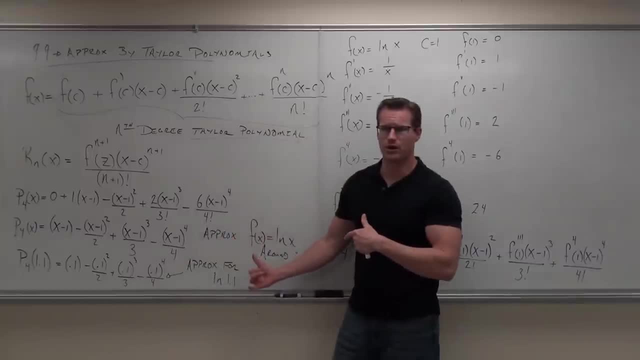 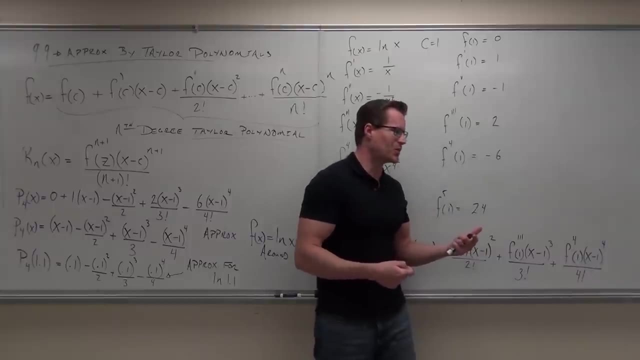 it's going to be pretty darn close to ln of 1.1.. Now we of course have calculators right, So we let's do 1.1 ln, But it's kind of cool that we can also approximate it. 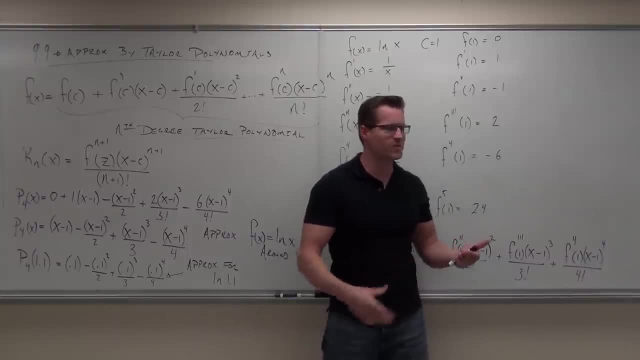 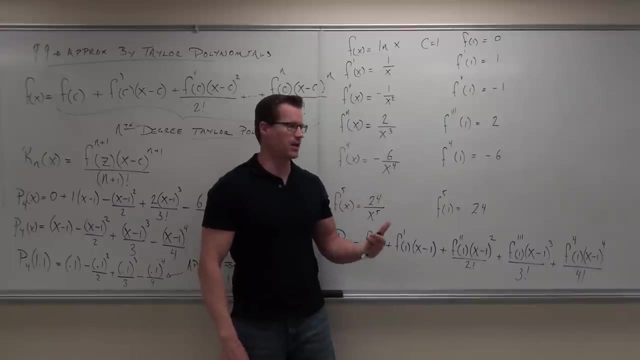 But it's kind of hard. It's kind of cool that we can also approximate it with a Taylor polynomial. Isn't that nice? This has no ln ln whatsoever, It's just based on the derivatives of ln. That's interesting. Now here's the issue that we're going to have with this. 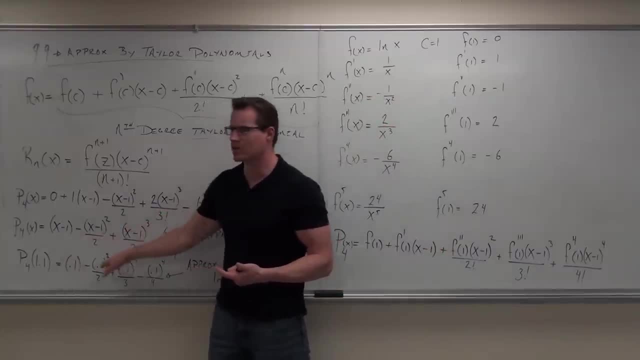 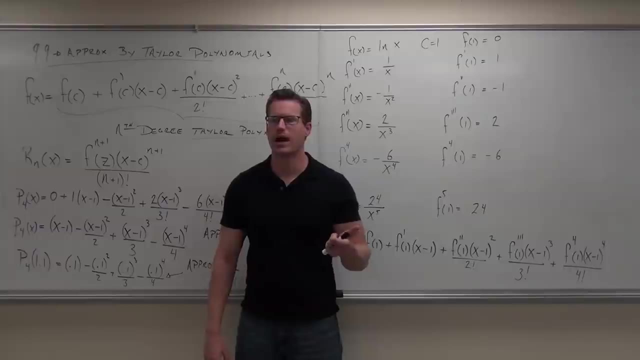 with a Taylor polynomial- Isn't that nice. This has no ln ln whatsoever. It's just based on the derivatives of ln x. That's interesting. Now here's the issue that we're gonna have with this. The issue is: is this an approximation? 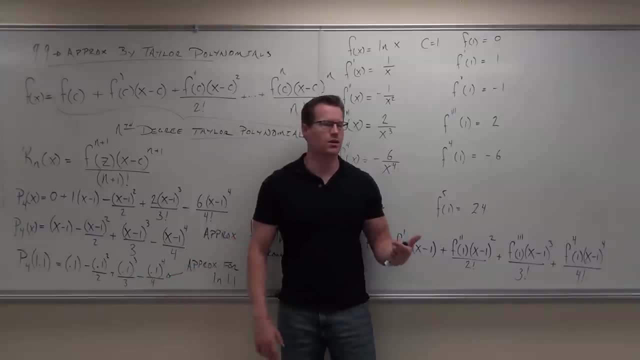 Yeah, How good of an approximation is it. That's where the error is. That's where the error comes in. So here's what we're gonna do next: We're gonna find out the error of this approximation. Are there any questions on any of this? 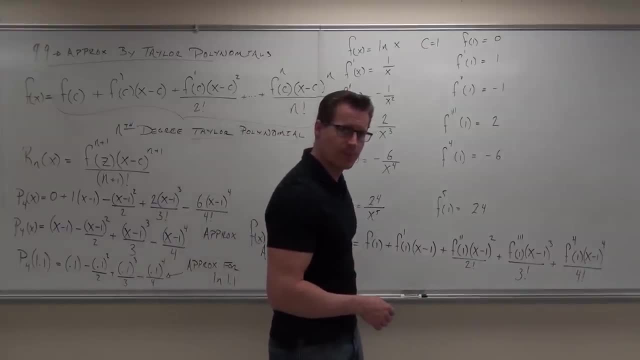 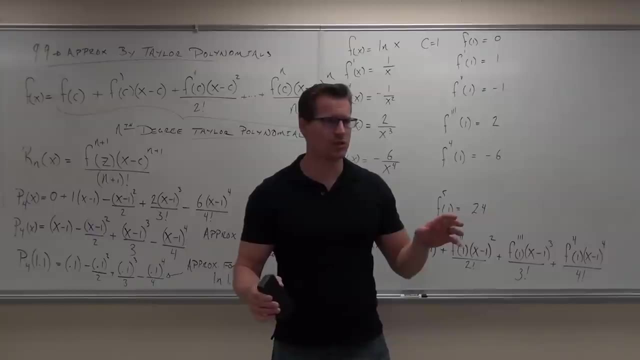 Question: Do you always go to the fourth degree or did you just choose for this one? No, I chose it just for this problem. Hopefully it makes sense to you that the larger degree Taylor polynomial I go to, the more accurate your approximation is. 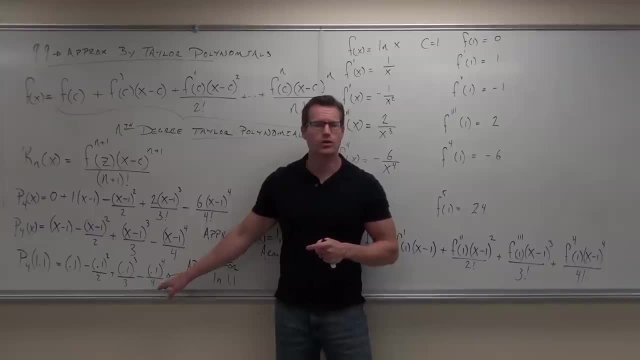 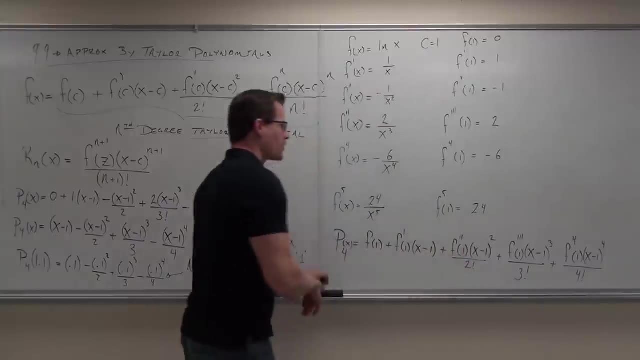 The issue is: is this an approximation? Yeah, How good of an approximation is it? That's where the error comes in. So here's what we're going to do next: We're going to find out the error of this approximation. Are there any questions on any of this question? 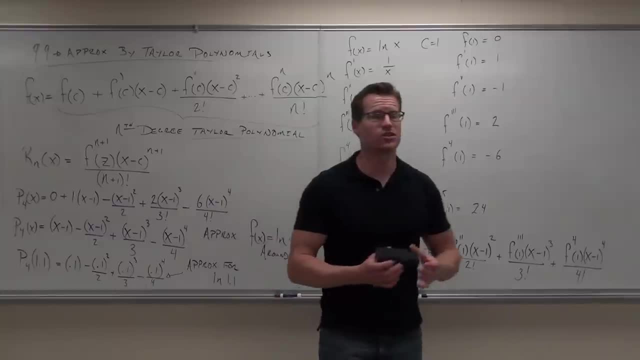 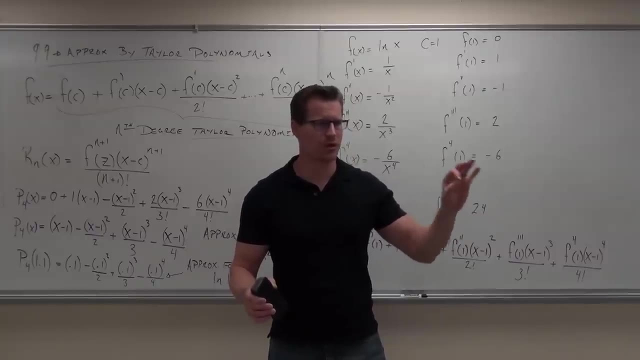 Do you always go to the fourth degree? No, I chose it just for this problem. Hopefully it makes sense to you that the larger degree Taylor polynomial you go to, the more accurate your approximation is. If I did a first degree Taylor polynomial, well, that'd be not so much right. 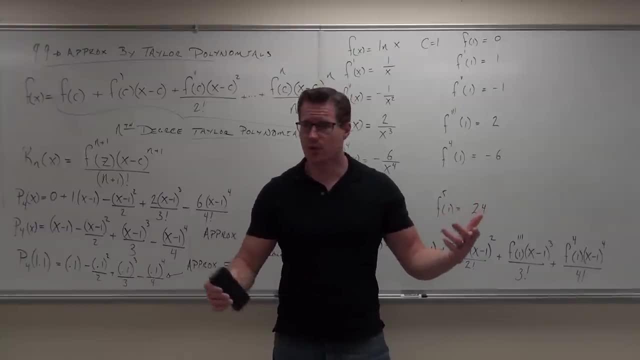 So we're going to use seconds, We're going to use thirds, fourths, whatever. Usually people don't go much past that because it just gets a little tedious, But I picked four just because it came into my head And I wanted to show you the process. 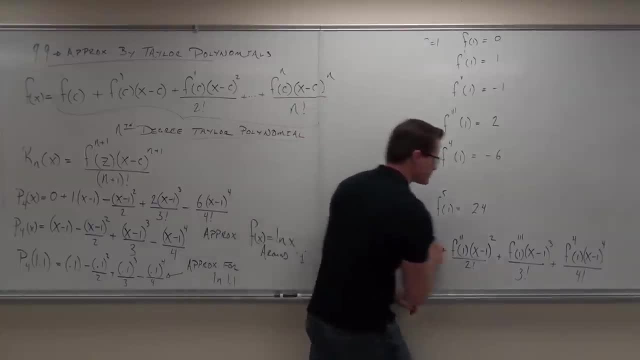 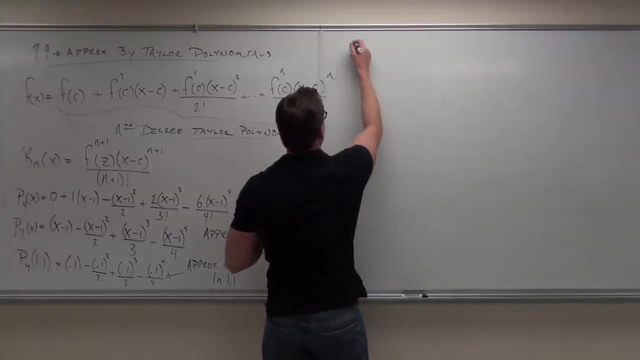 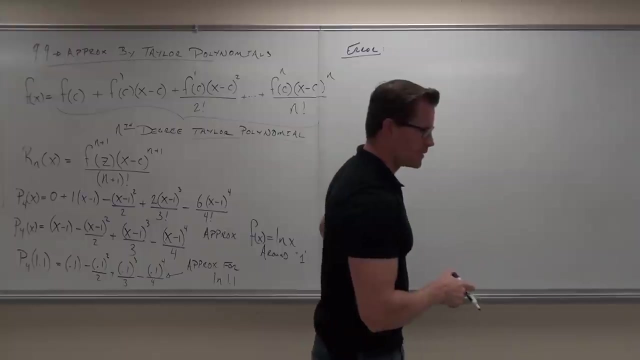 I think if I just did a first degree, you really wouldn't see a lot. Okay, so now for our error. Well, our error. I'm going to start from the beginning on the error. I'm not going to use anything that we've basically done. 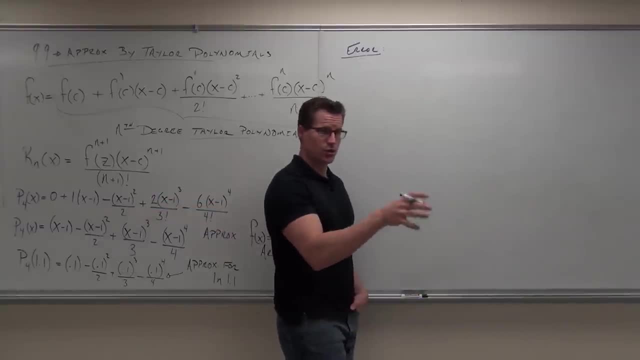 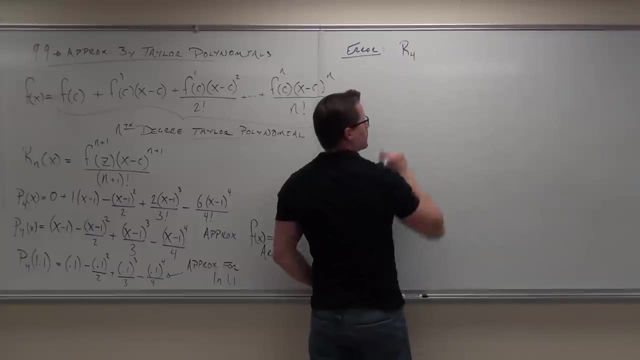 We had it up here, but I'm going to show you from the beginning And you're going to see that you could have just taken what we had right here and gone with it. Our error from a fourth degree Taylor polynomial. that's a remainder. 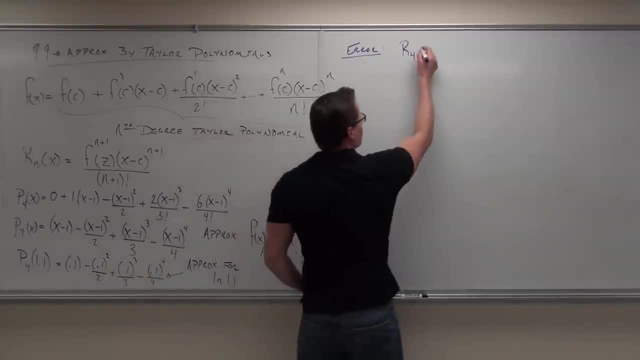 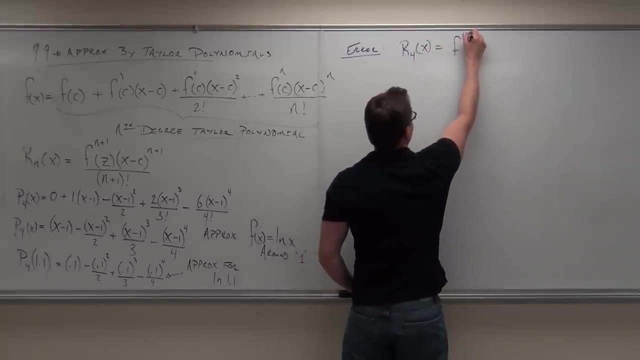 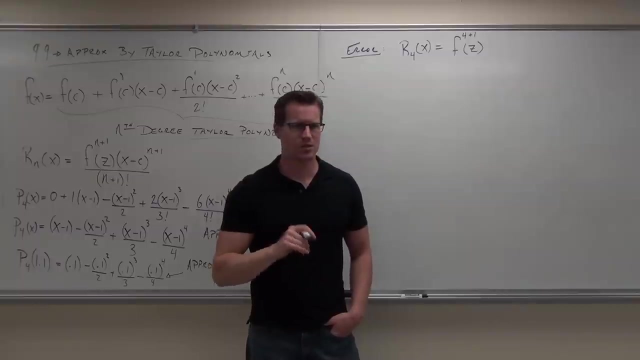 It's called a remainder, So the remainder of a fourth degree Taylor polynomial. Well, what that's going to be is that's going to be the next derivative at some point- z. Did I talk about z before? Yes, Because z is between c and x. 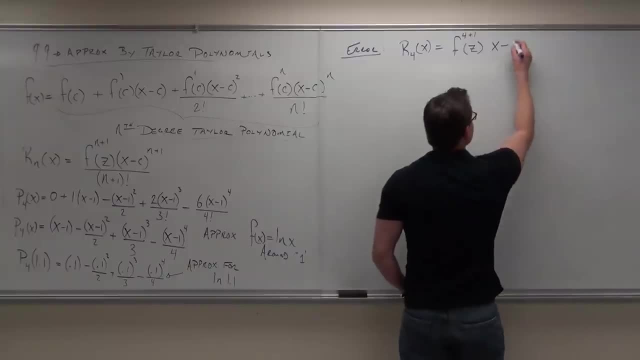 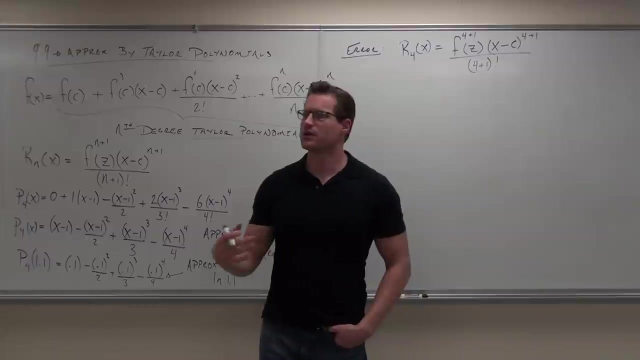 What's our c? We're going to plug that in in a minute Of the next power over the next factorial. Now it's your job to start plugging these things in. So here's what we're going to do. We're going to start simplifying this. 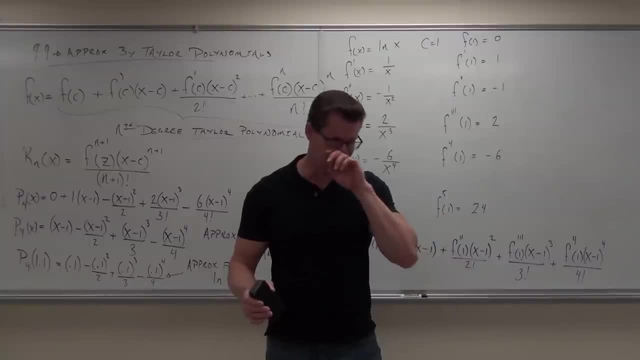 If I did a first degree Taylor polynomial, well, that'd be not so much, right? So, second, third, we're gonna use seconds, we're gonna use thirds, fourths, whatever. Usually people don't go much past that. 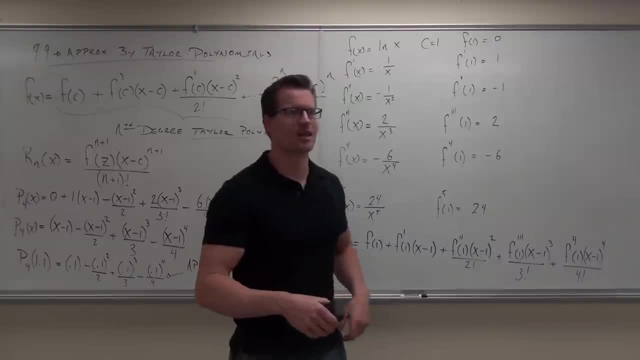 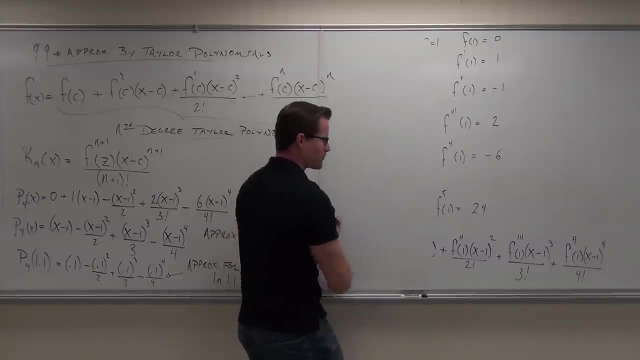 because it just gets a little tedious. But I picked four just because it came into my head okay, And I wanted to show you the process. I think if I just did a first degree it really wouldn't. you wouldn't see a lot. 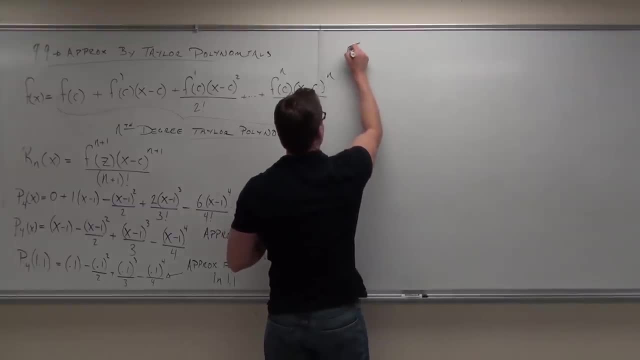 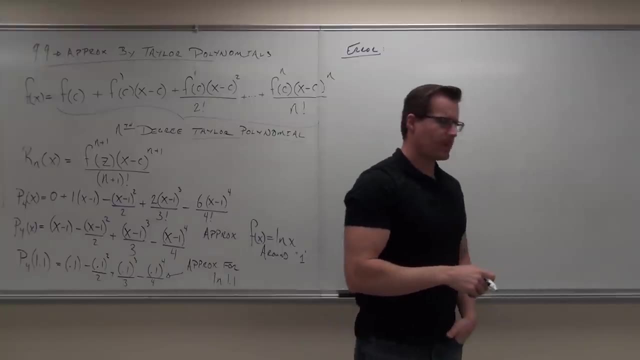 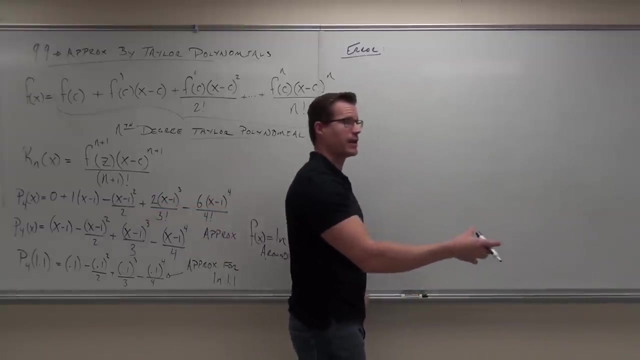 Okay, so now for our error. Well, our error. I'm gonna start from the beginning of the error. I'm not gonna use anything that we've basically done- We had it up here- but I'm gonna show you from the beginning and you're gonna see. 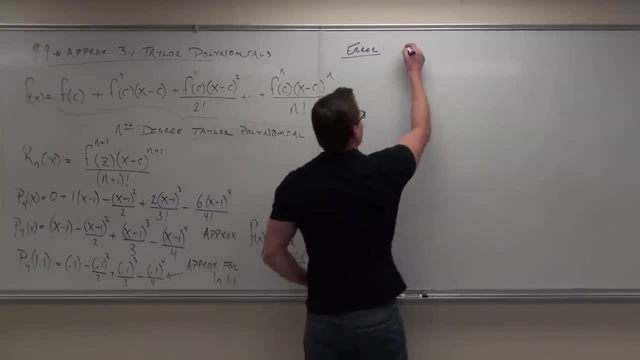 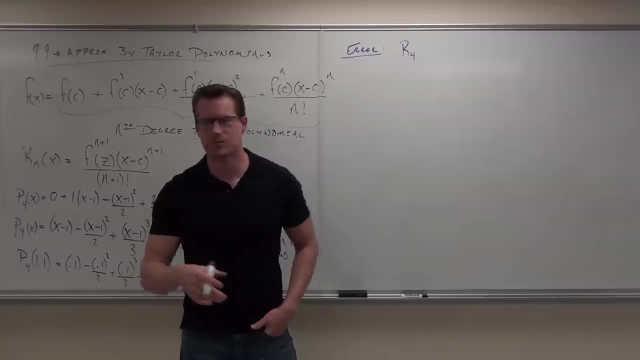 that you could've just taken what we had right here and gone with it. Our error from a fourth degree Taylor polynomial, that's a remainder. it's called a remainder, so the remainder of a fourth degree Taylor polynomial. well, what that's gonna be is that's gonna be. 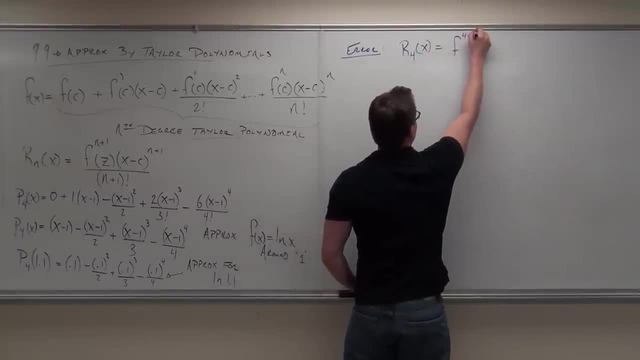 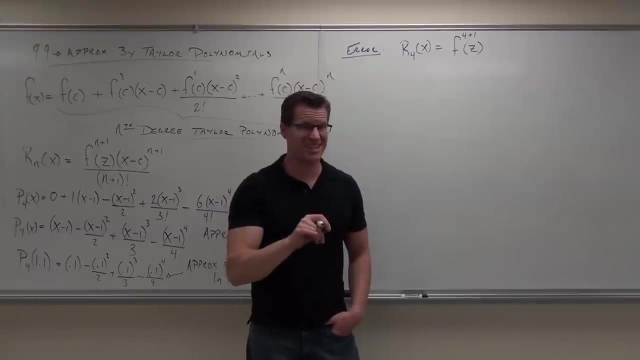 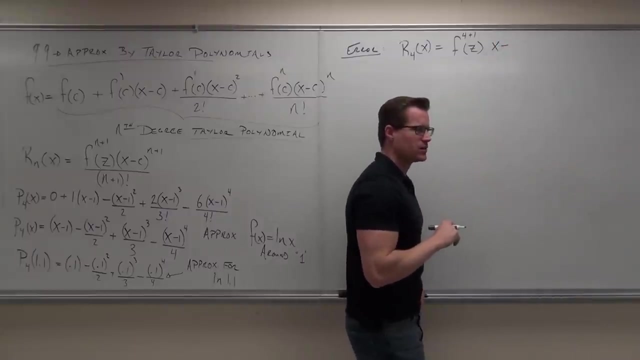 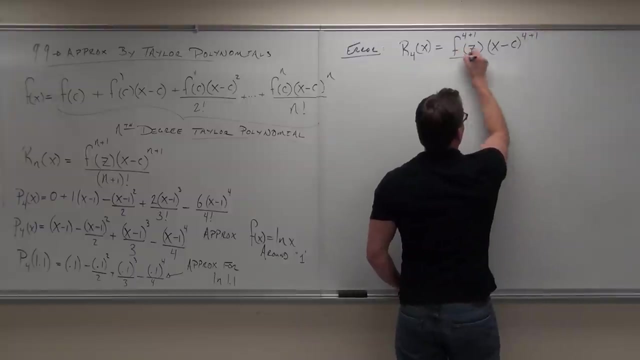 the next derivative at some point, z. did I talk about z before? Yes, Did I talk about how z is between c and x? X? what's our c One? We're gonna play that in a minute Of the next power over the next factorial. 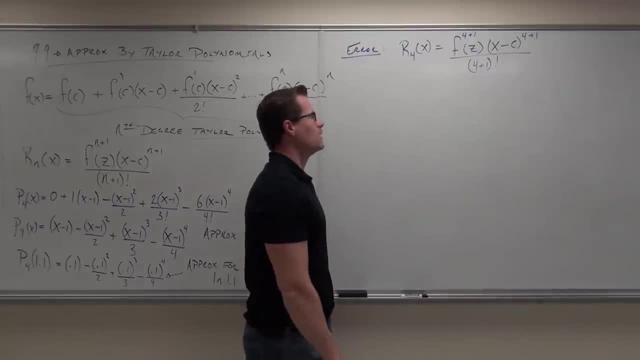 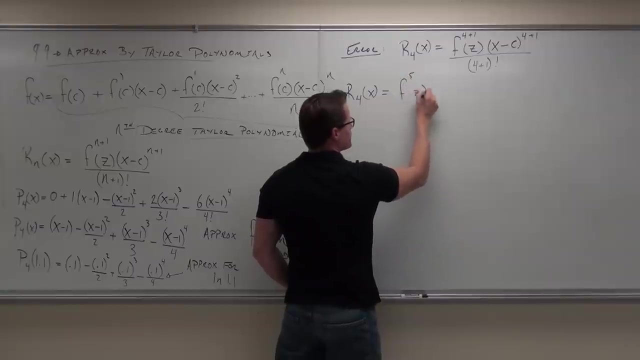 Now it's your job to start plugging these things in. so here's what we're gonna do: We're gonna start simplifying this. So the remainder of the fourth degree Taylor polynomial is the fifth derivative, at z, some point between c and x. 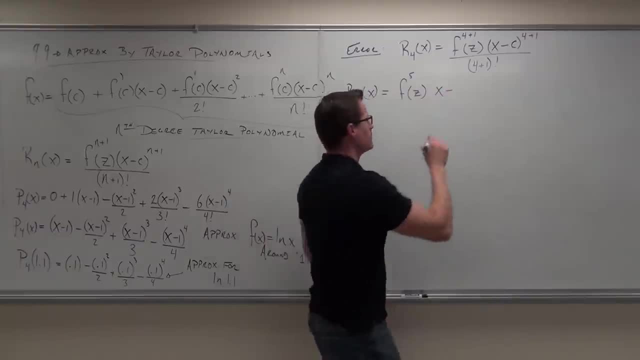 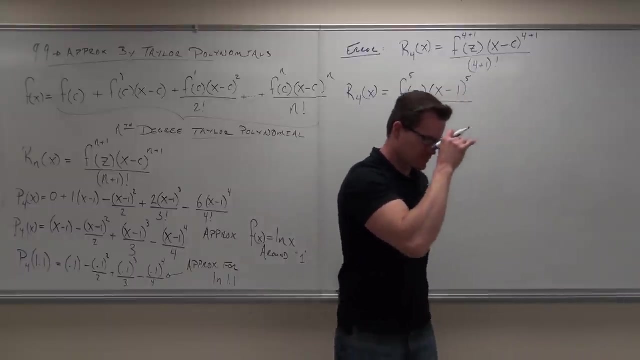 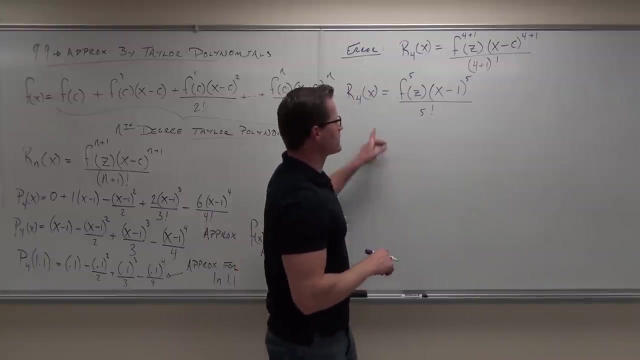 X minus. we already had our c. use the same c. We're gonna start using the fourth derivative at z. Did we Goddamn right what You guys? okay with this one so far? What piece of this do we know? 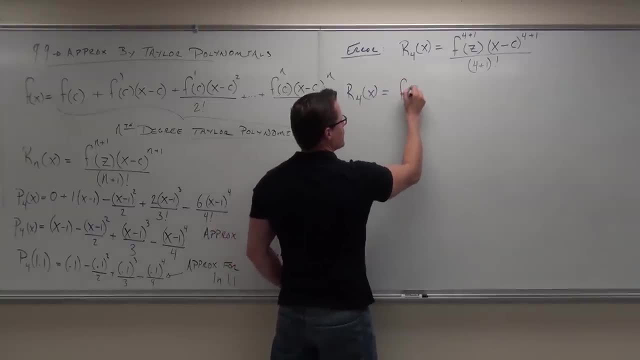 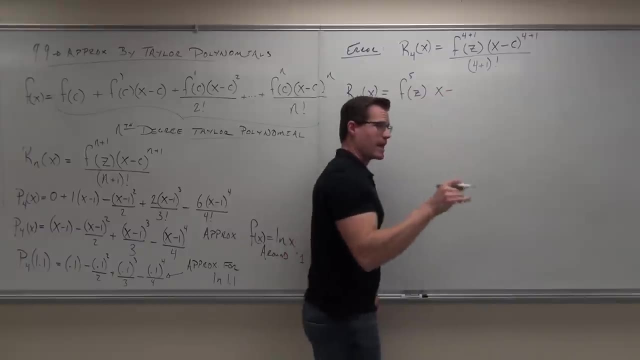 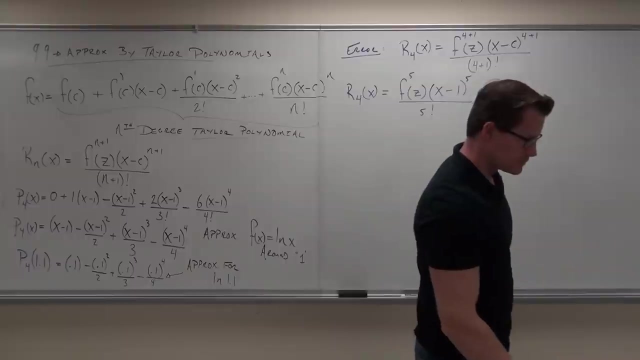 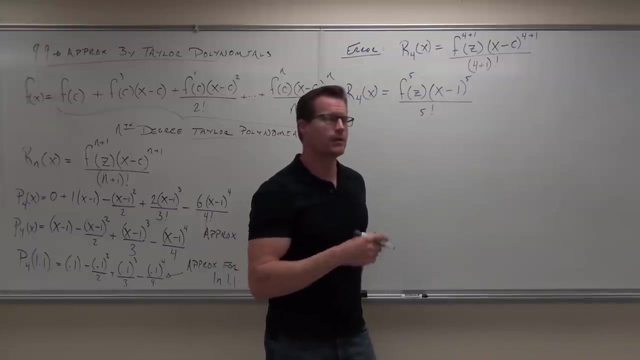 So the remainder of the fourth degree Taylor polynomial is the fifth derivative at z, Some point between c and x, x minus. We already had our c. Use the same c, You guys. OK with this one so far. What piece of this do we know? 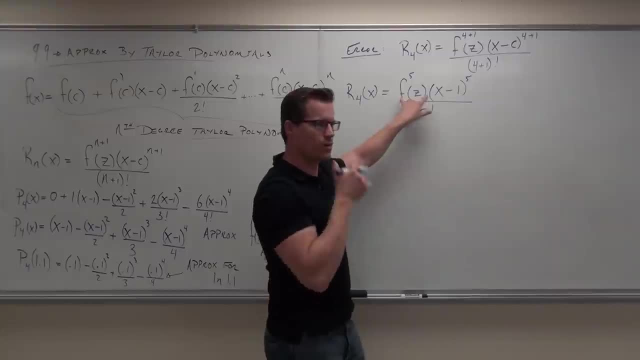 x. OK, We know that one. What about that? Do you know what the? let's start here. Do we know what the fifth derivative of x was? You had that already right, Because I told you to go one more derivative than we already had. 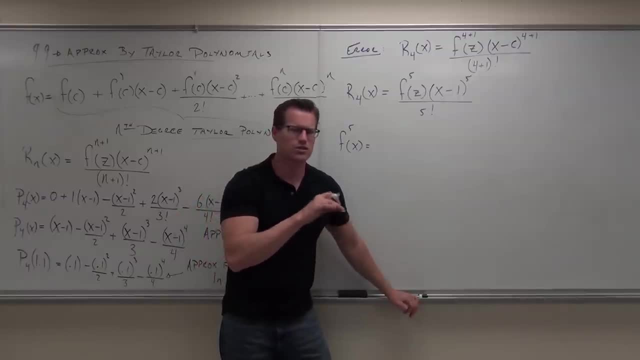 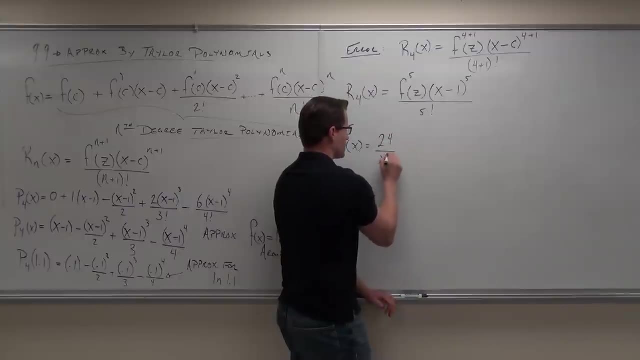 Otherwise you'd have to start from the beginning right now. I don't want to do that. This was, if I don't, 24.. 24 over x to the. The power, The power, The power. OK, You guys, OK with that one. 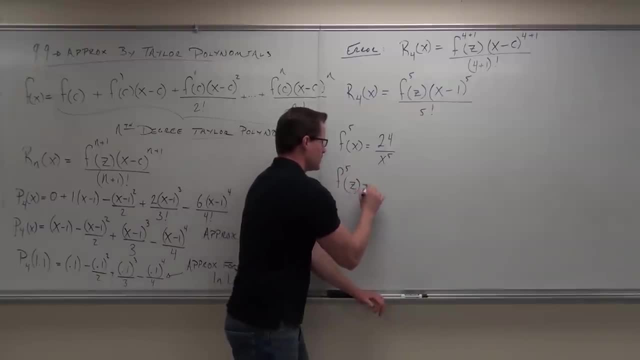 Which means that the fifth derivative of z is simply 24 over z to the fifth. So you guys feel OK with that one. Here's the deal: You get to pick z, You're going to pick z such that you get the largest area. 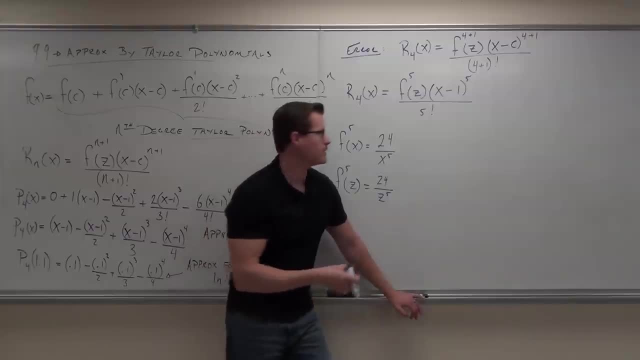 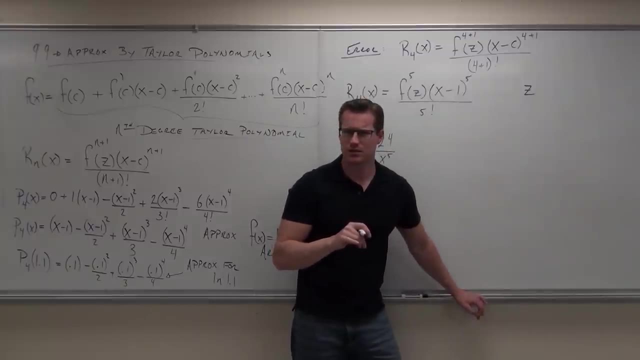 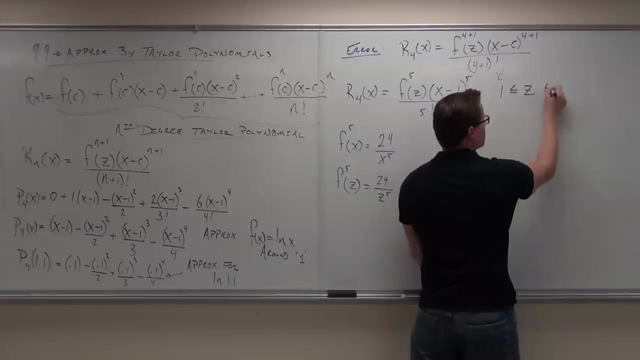 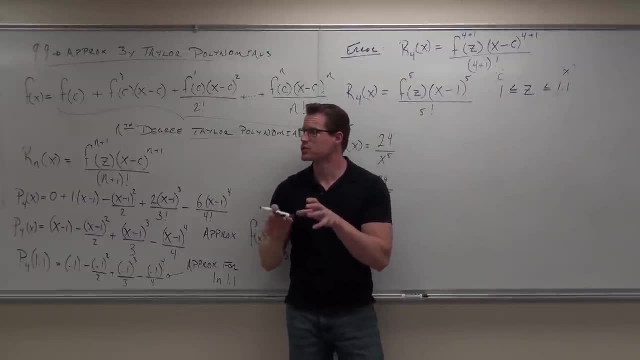 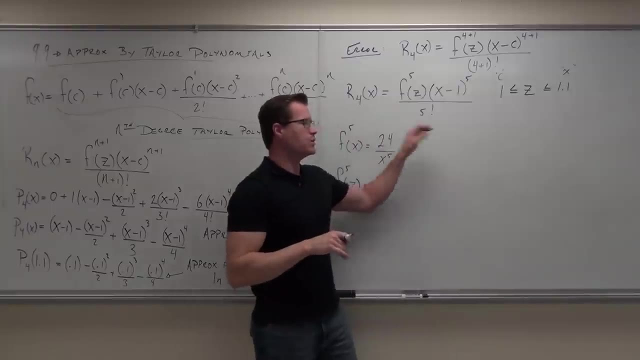 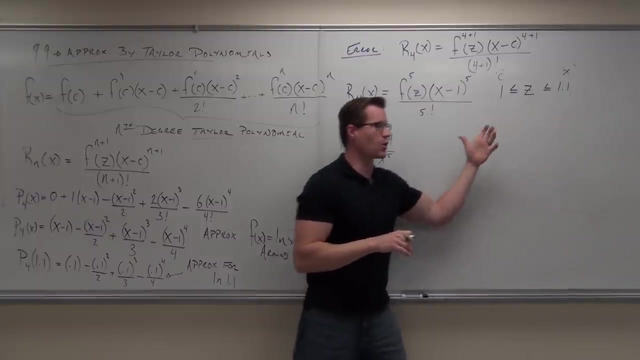 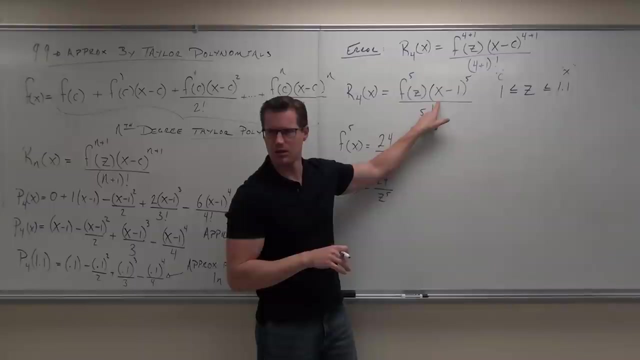 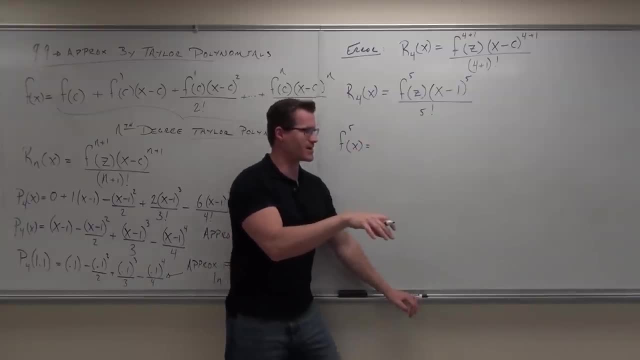 We know that one. what about that? do you know what the? let's just start here. Do we know what the fifth derivative of X was? You had that already right, Because I'd told you We had that already right. 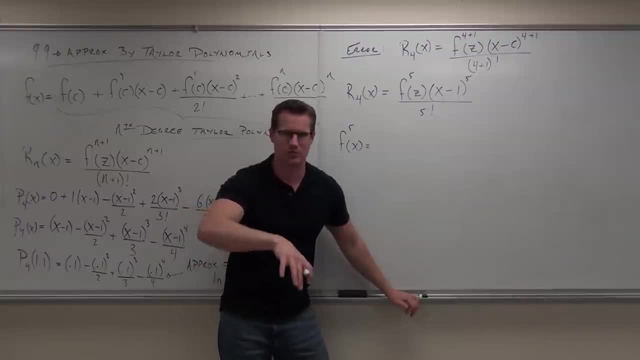 Because I told you to go one more derivative than we already had, otherwise you'd have to start from the beginning right now. I don't want to do that. This was, if I don't, if I'm 24 over, X to the. 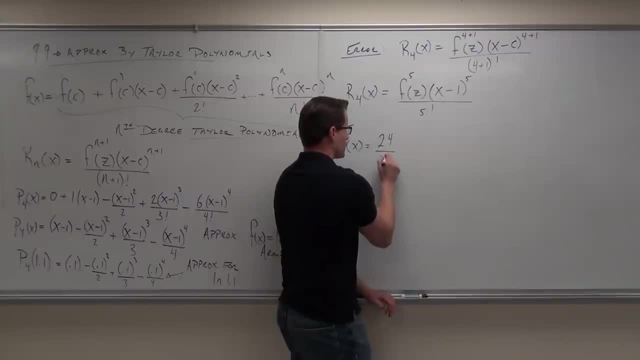 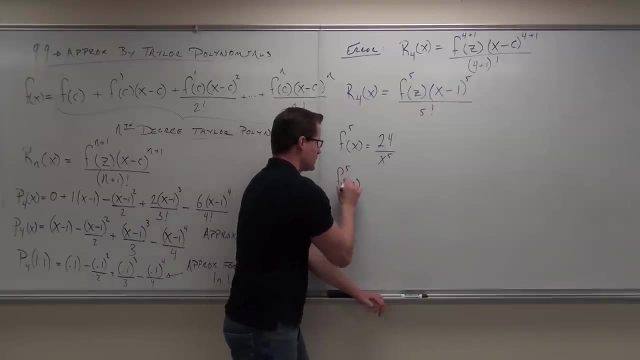 F power. You guys okay with that one, Which means that the fifth derivative of Z is simply 24 over Z to the fifth. So you guys feel okay with that one. There's your deal: You get to pick Z. You're going to pick Z such that you get the largest error. 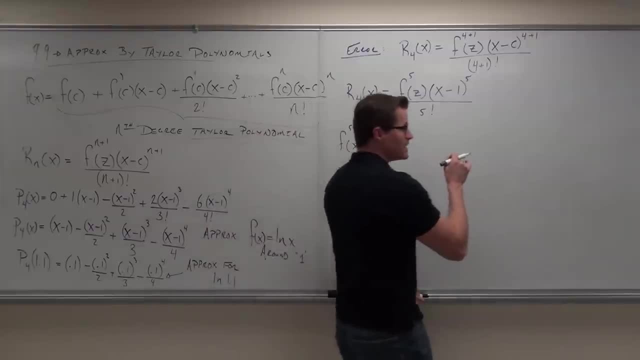 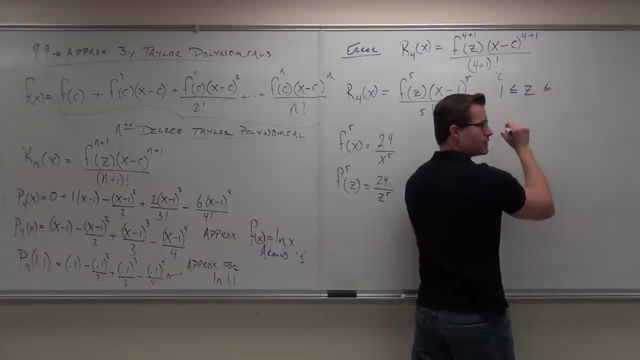 The largest error. Now, keep in mind: Z is a number between. what two numbers did I say One X and Z Is a number between C and X. What's our X, One One. Yes, that's exactly right. 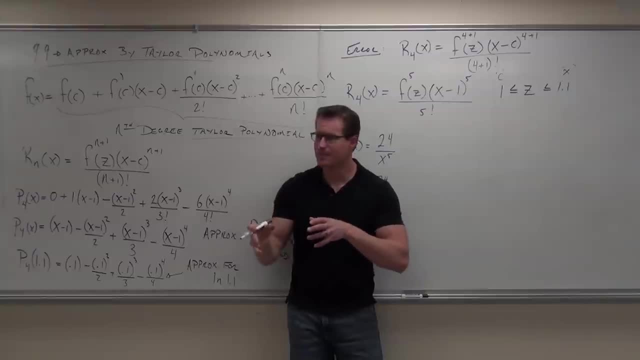 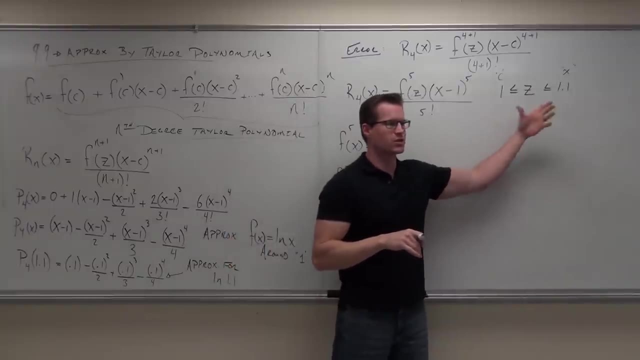 So Z is a number between those two values, C and X. So if you understand that concept, Okay, now here's the deal. You need to pick which one of the. it's usually going to be one of the end points here. 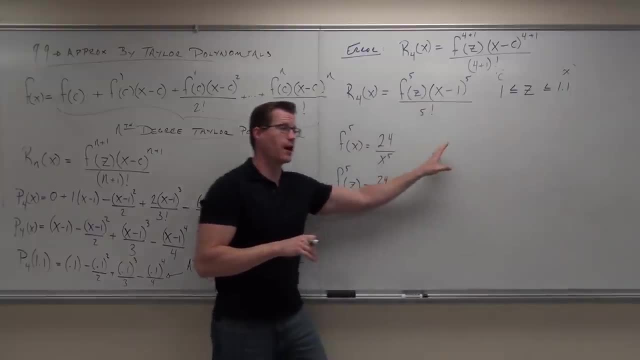 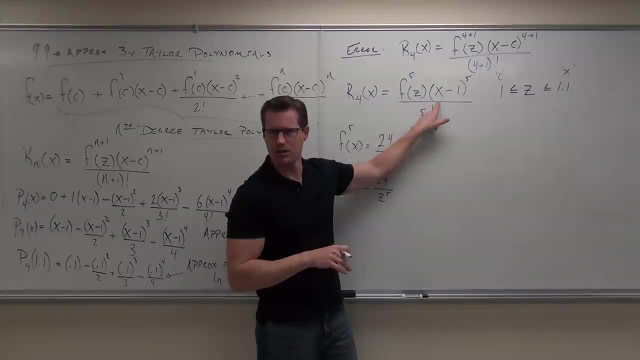 You need to pick which one of these things is going to give the larger value when you plug it into here. This does not change. Okay, this is going to be 1.1.. Do you see what's going to be 1.1?? 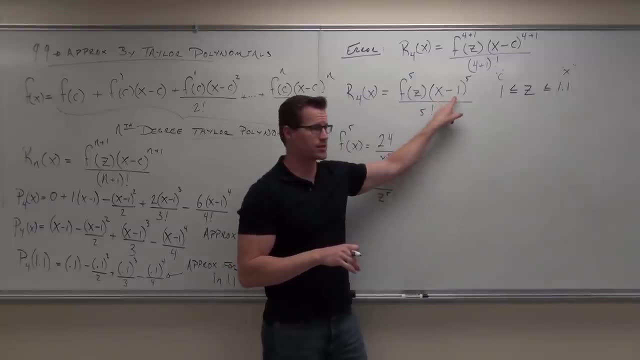 How much is your X? This is going to be 1.1.. This C, it's already there. It's going to be one. Does that make sense to you? So you're going to get .1.. That's not going to change. 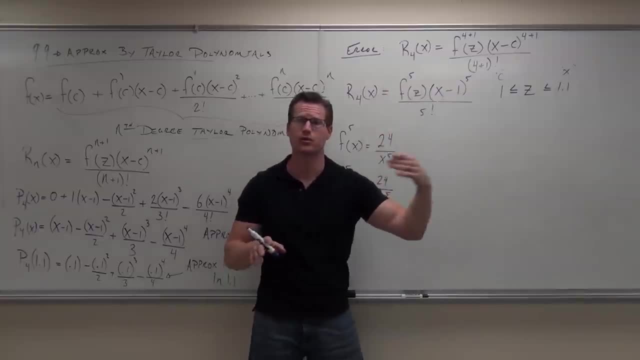 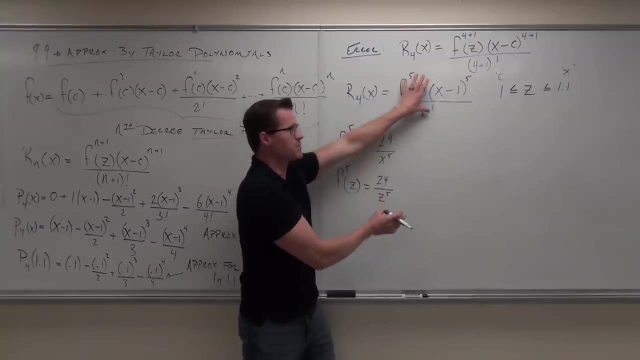 That's not going to change. This is the only thing that has a possibility of changing, because it's in an interval of numbers, So you're going to pick the Z, for which this thing is biggest. Now look here: This is the only thing that can make this bigger or smaller. 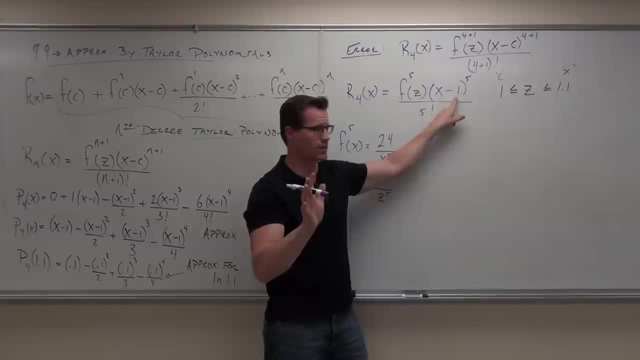 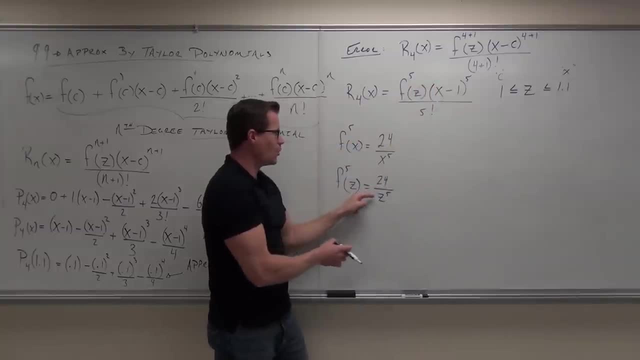 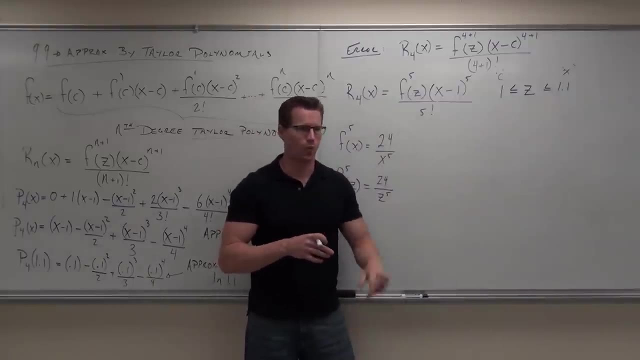 that can make this bigger or smaller. okay, The x is chosen. What would you put here to make this larger? Would you put one point one or would you put one One? You put one. So in our case we're gonna pick: z equals one. 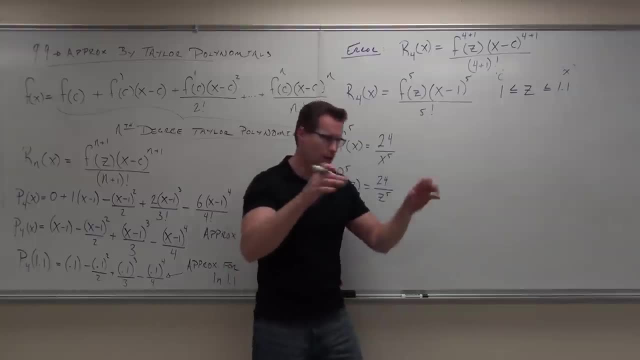 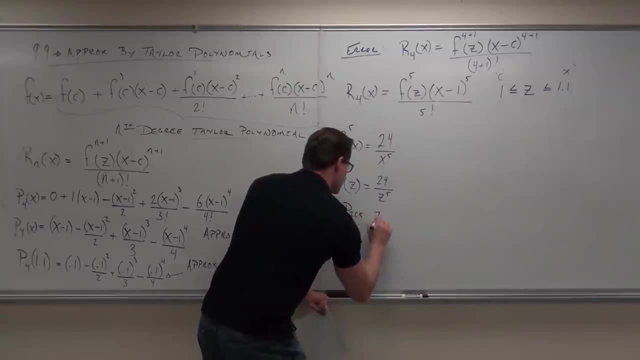 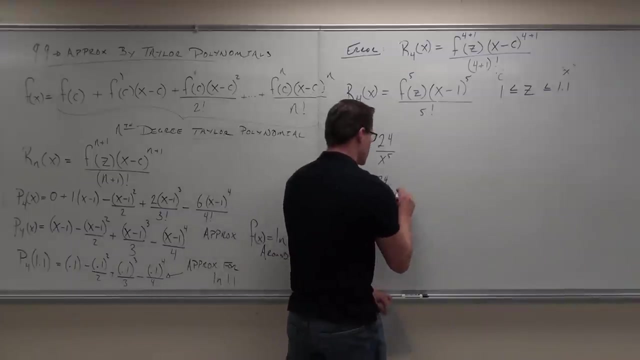 because that's gonna give us the largest error. Quick hint now: if you're okay with that one, Okay, so we're gonna pick z equals one for the biggest error. You don't want to underestimate the error. So in our case, the fifth derivative of f at z. 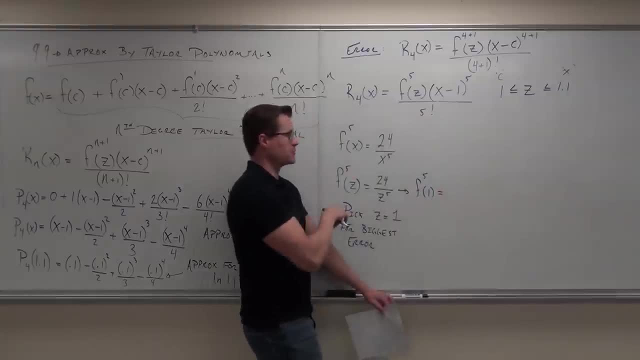 would be the fifth derivative of f at one. What's the fifth derivative of f at one when I plug in one? How much is that gonna be? Say it again: It's 24 over one to the fifth, it's 24.. 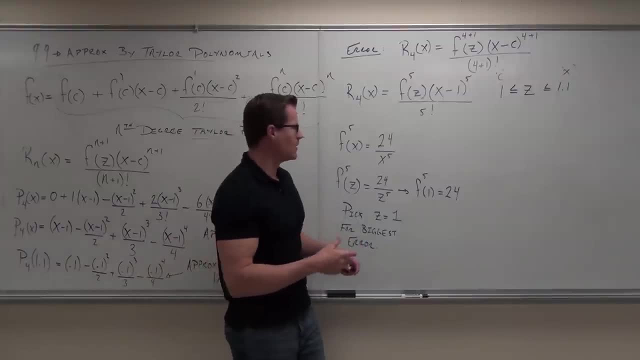 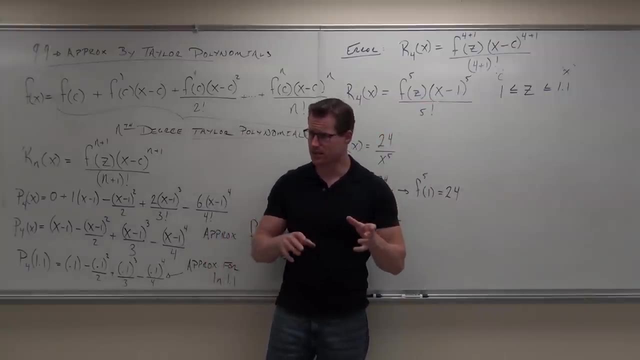 By the way, you're gonna notice something. Some students have an issue with this. You go wait a minute. why did I plug in one here when I'm plugging in one point? one here You can have different values for x and z. 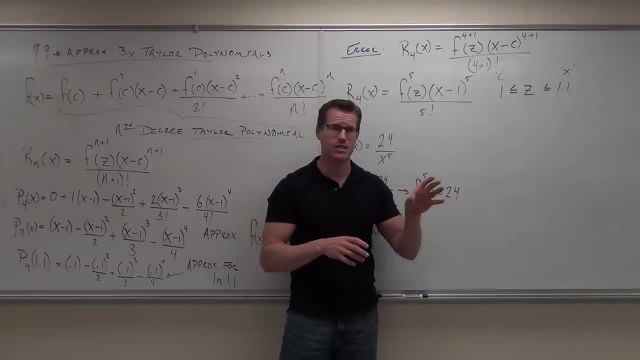 They don't have to be the same. Okay, so sometimes your z will be the same as x, Sometimes your z will be the same as c. Your z just has to be between those numbers and you pick it such that you get the biggest error possible. 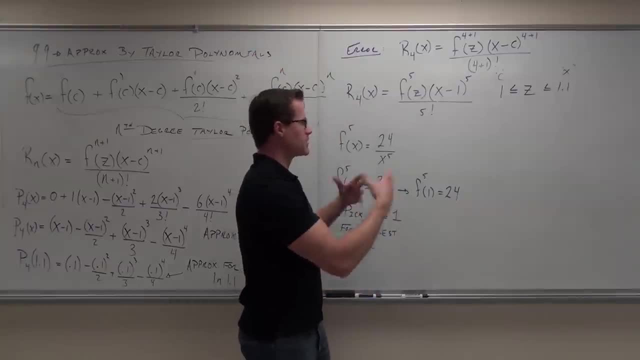 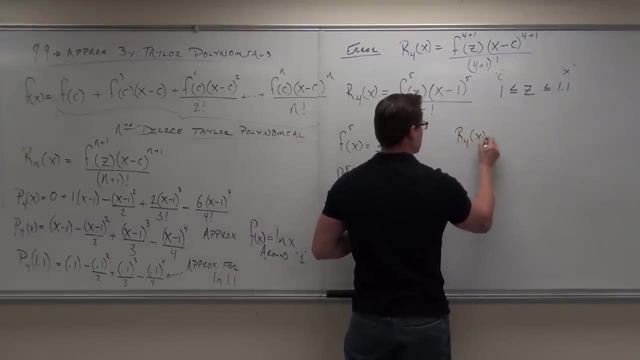 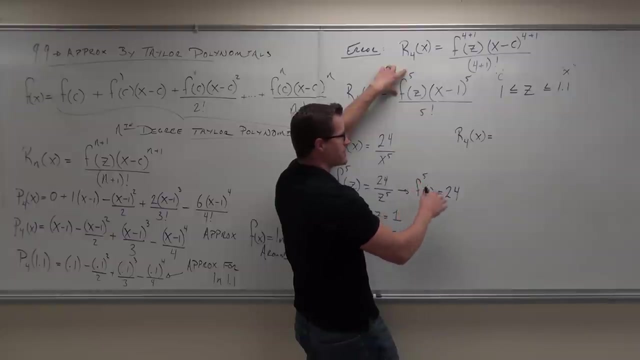 Show of hands. Okay, now here we go. Let's put this all together. So if I know that my error is equal to the fifth derivative of f at z, some point between x and c, and this value of z equals one, gives me my biggest error. 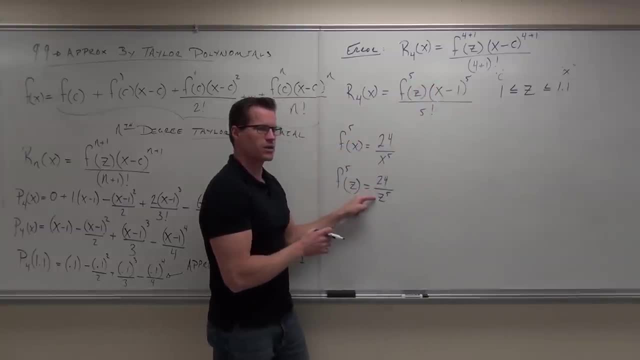 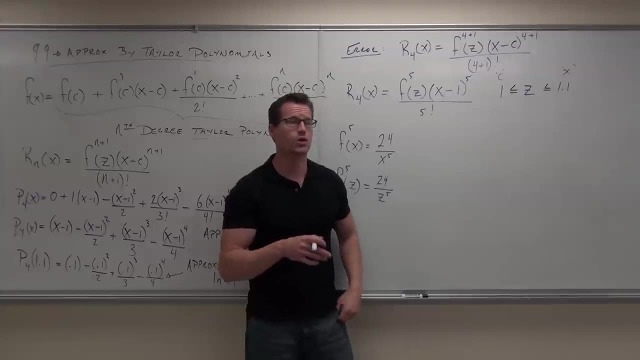 Okay, the X is chosen. What would you put here to make this larger? Would you put 1.1 or would you put one One? You put one. So in our case we're going to pick: Z equals one. 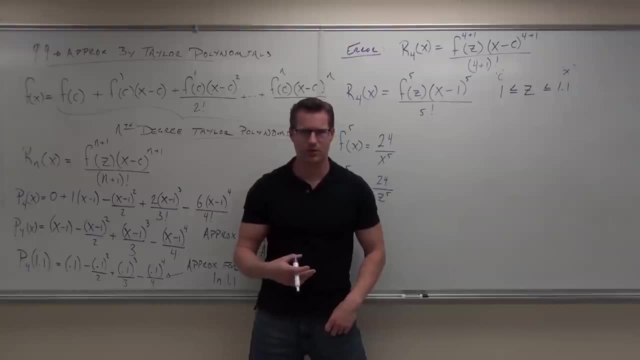 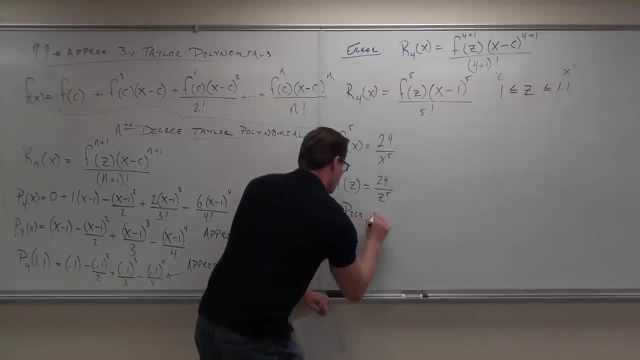 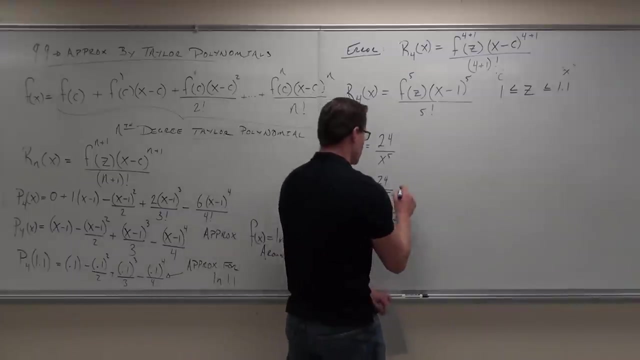 Because that's going to give us the largest error. Quick hit now if you're okay with that one. Okay, so We're going to pick Z equals one for the biggest error. You don't want to underestimate the error. So, in our case, the fifth derivative of Z. 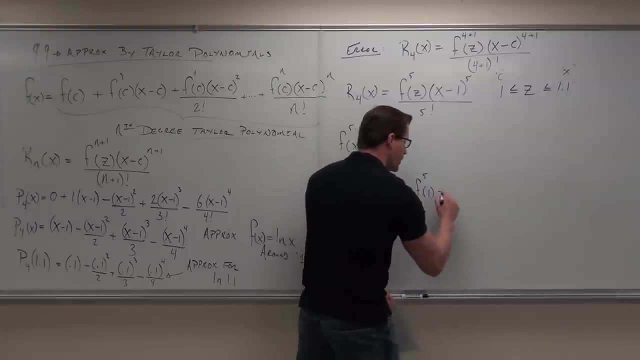 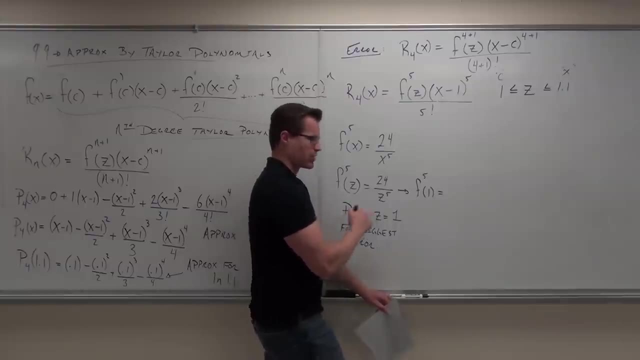 F at Z would be the fifth derivative of F at one. What's the fifth derivative of F at one when I plug in one? How much is that going to be? Say it again: It's 24 over one to the fifth, It's 24.. 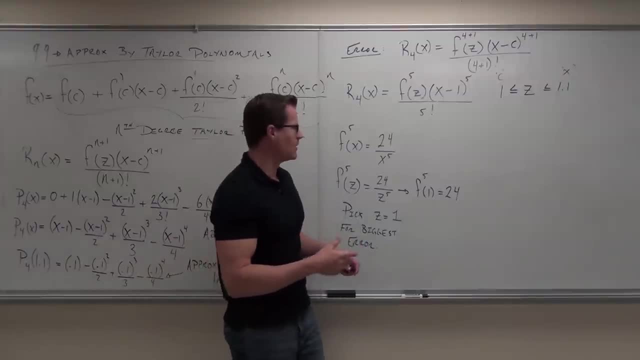 By the way, you're going to notice something. Some students have an issue with this. You go wait a minute. Why did I plug in one here when I'm plugging in 1.1? here You can have different values. 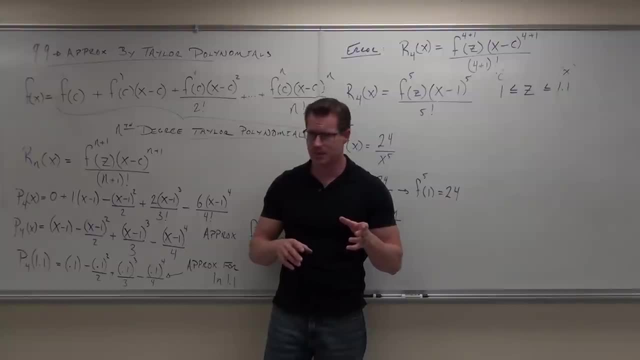 You can have different values for X and Z. They don't have to be the same. Okay, so sometimes your Z will be the same as X. Sometimes your Z will be the same as C. Your Z just has to be between those numbers. 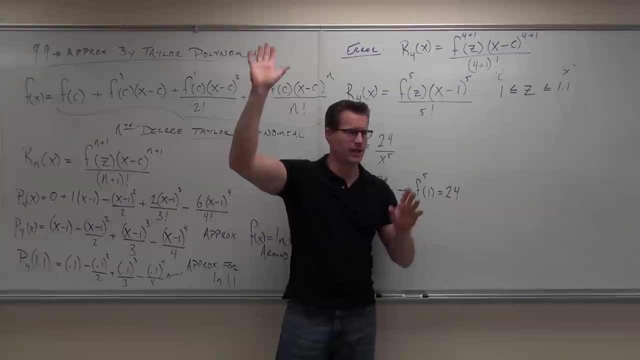 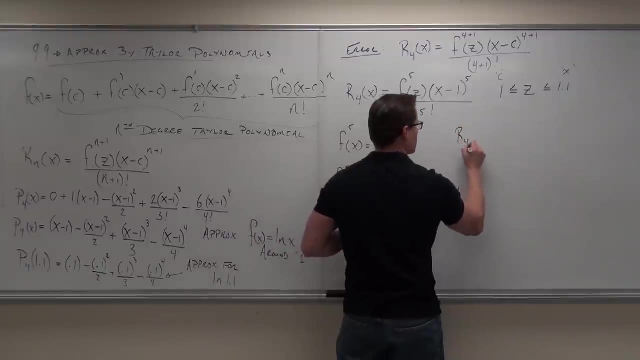 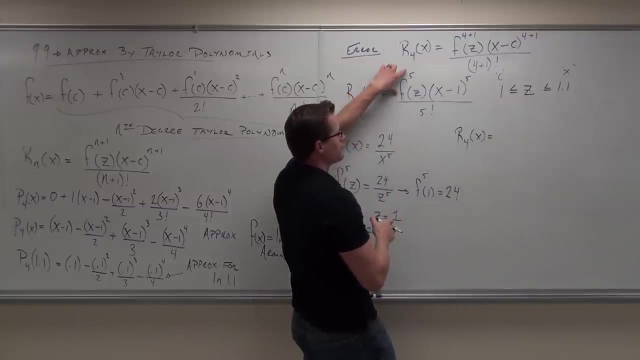 and you pick it such that you get the biggest error possible. Show of hands. Okay, now here we go, Let's put this all together. So, if I know that, my error is equal to the fifth derivative of F at Z. 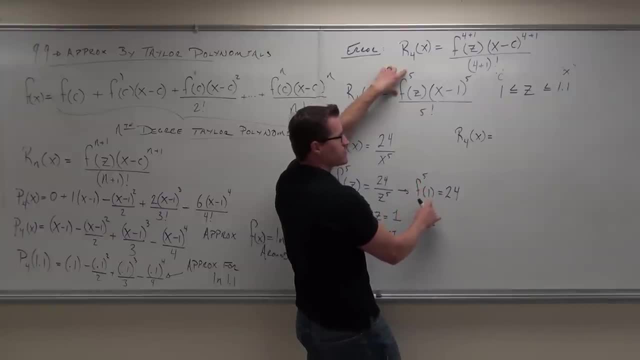 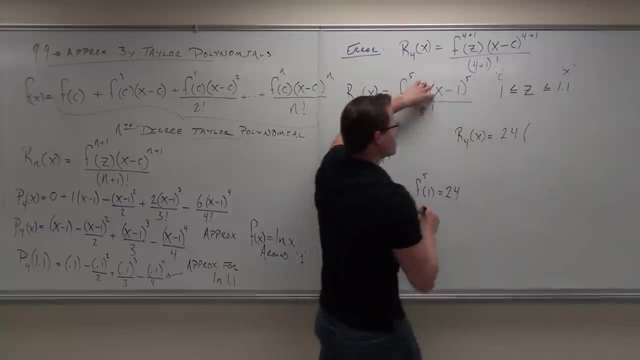 some point between X and C, and this value of Z equals one gives me my biggest error. I'm going to have 24.. This gives me 24.. I'm going to have what's my X? going to be everybody 1.1.. 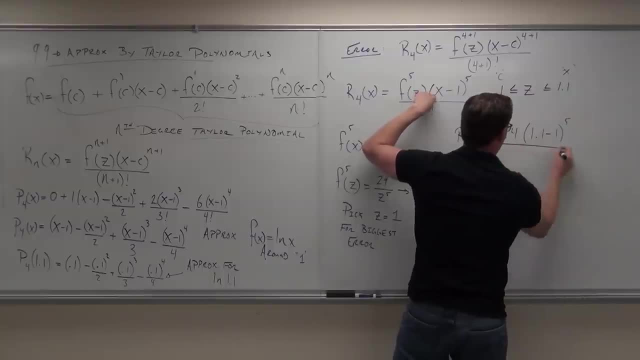 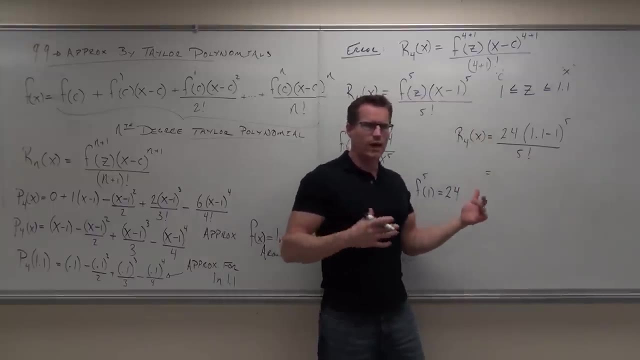 1.1 minus one to the fifth, all over five factorial. So in our case, if you notice this and this works out for this one quite nicely- 24 is four times three times two times one, Five times four times three times two times one. 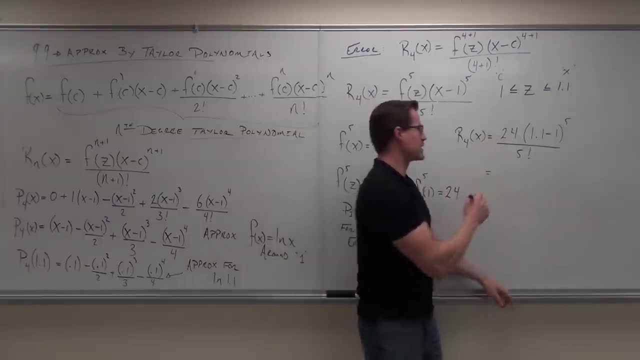 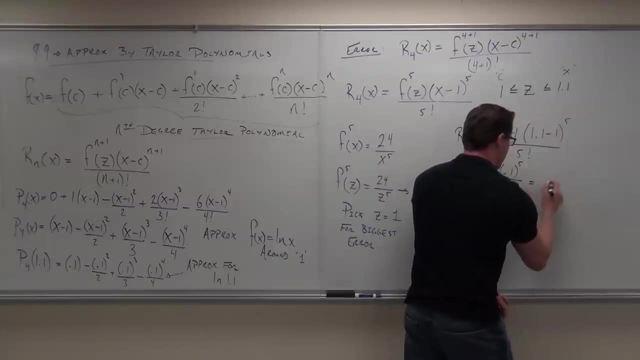 So if I simplify that, I'm just going to get something over five. In fact, I get .1 to the fifth power all over five, And that's equal to someone with a calculator. tell me what that is. .1 to the fifth divided by five. 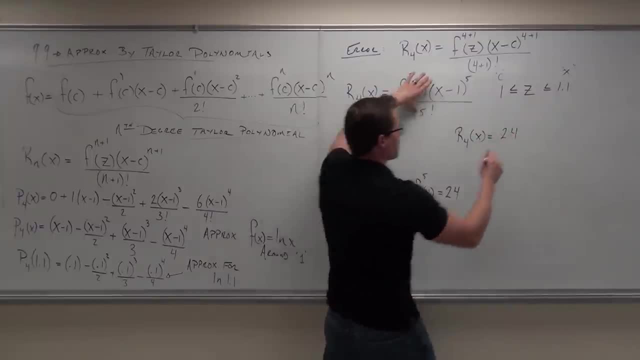 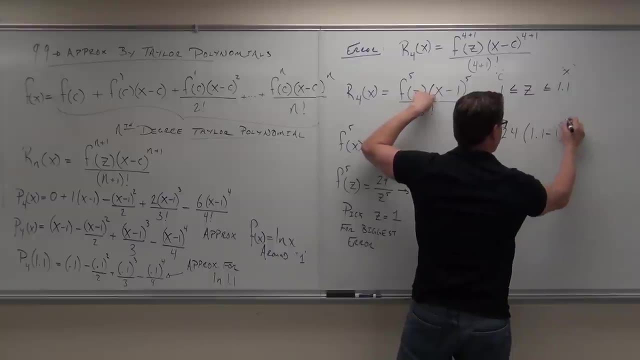 I'm gonna have 24.. This gives me 24.. I'm gonna have what's my x? gonna be everybody. One point one. One point one minus one to the fifth, all over five factorial. So in our case, if you notice this, 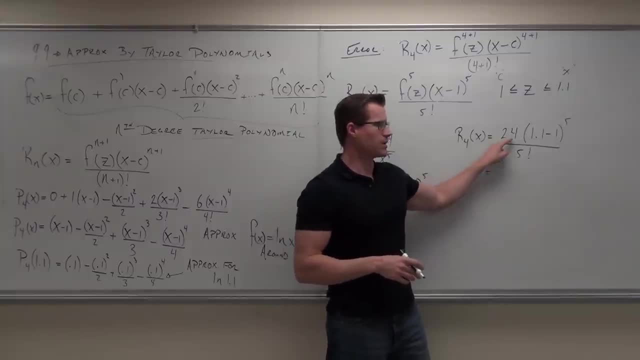 and this works out for this one quite nicely: 24 is four times three times two times one. This is five times four times three times two times one. So if I simplify that, I'm sure you get something over five. In fact I get point one to the fifth power all over five. 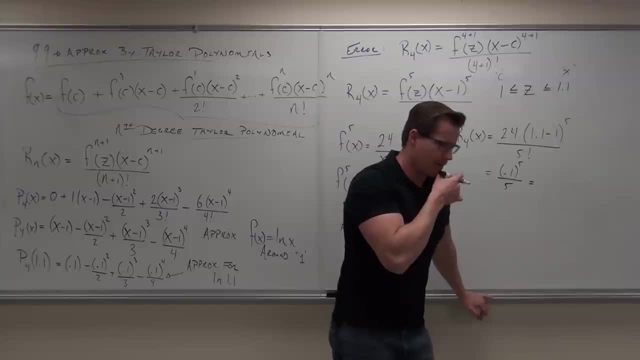 And that's equal to someone with a calculator. tell me what that is. Point one to the fifth divided by five. So point zero, five zeros or something. Don't leave me hanging Two times 10 to the negative sixth. There you go. 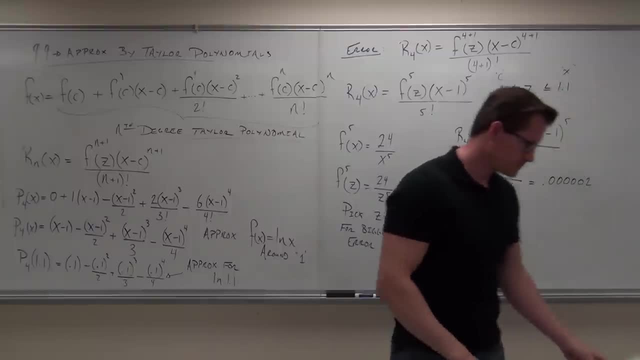 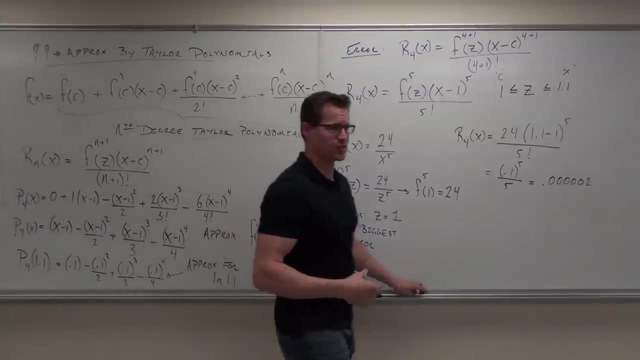 Thank you. Now, I said that this goes fast, and they do go fast. I just had to explain this to you. but this does go quite quickly because all you gotta do is do a few derivatives And then you gotta plug in a number. 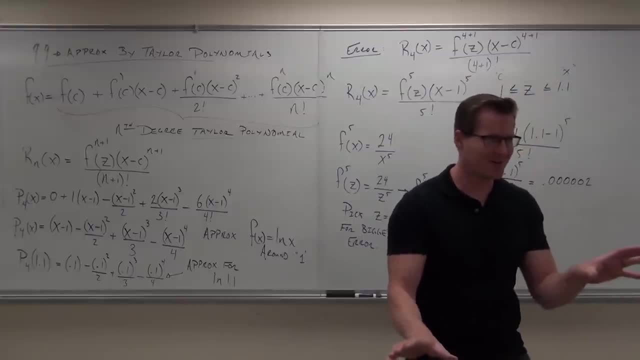 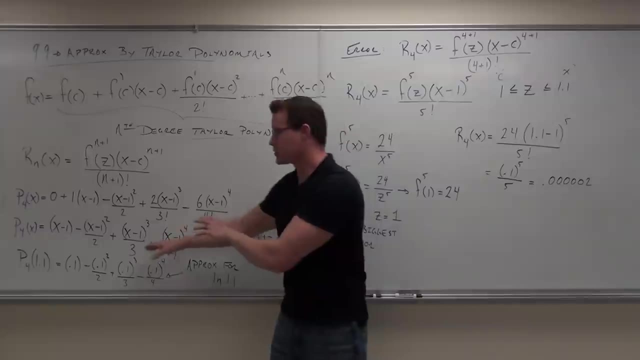 and then you gotta find an error. So here's what we just said. Are you with me? Okay, we cut a Taylor series short. it's called. There is some sort of error associated with that With our Taylor polynomial. all you've got to do is plug. 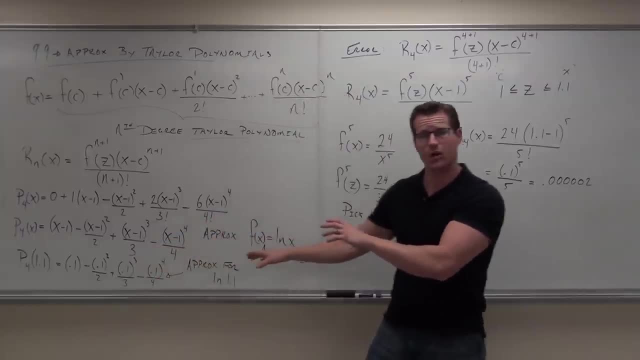 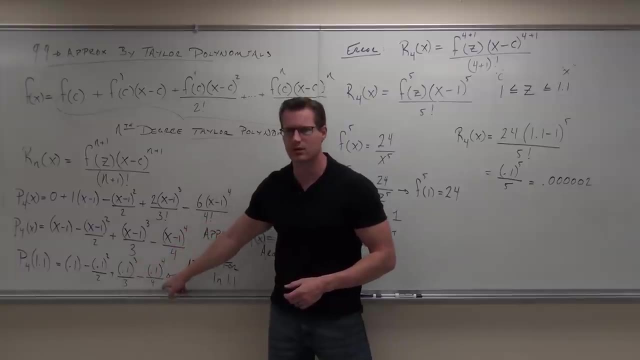 in a number you want to approximate, as long as you base that Taylor polynomial around the number. So in our case we base it around 1 because we're trying to approximate 1.1.. Just plug it in, By the way. has anyone worked this out? 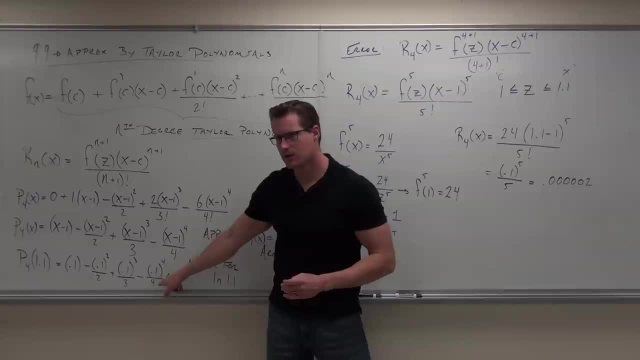 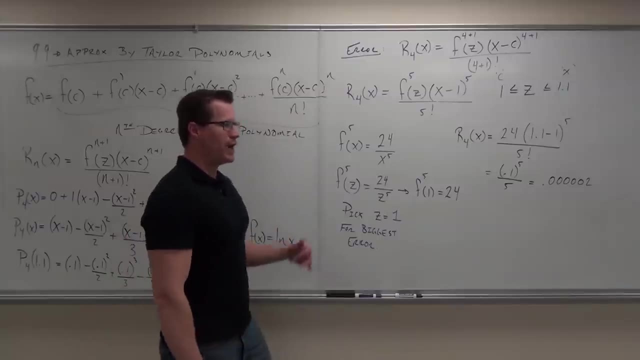 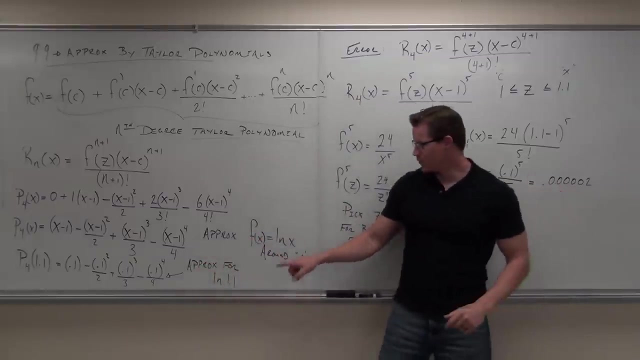 Did you do it? How much is it? 0.095308333.. Assuming you're right, I'm not going to double check you. So assuming that you're right, That approximation is within this number of what this really is for ln 1.1.. 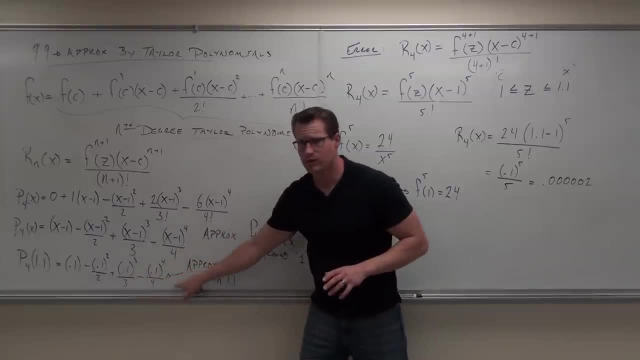 I'll say that one more time: When you work that out, when you work this out and you find it, this is within this distance from what this actually is. So is this an approximation of this? Yes, How close is it? Now we know? 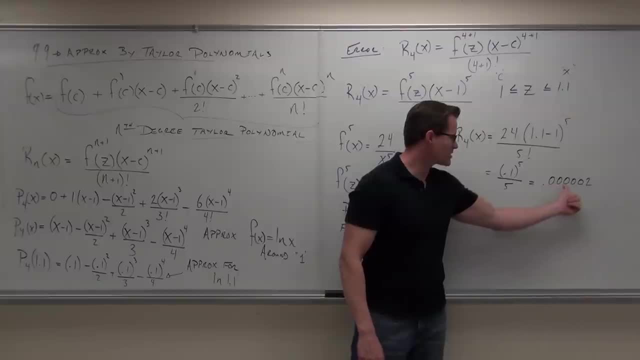 It's within .00010th 100th, 1000th, 10th, 100th, 1000th, 100th, 1000th- within 2 millionths, So it's pretty darn close. 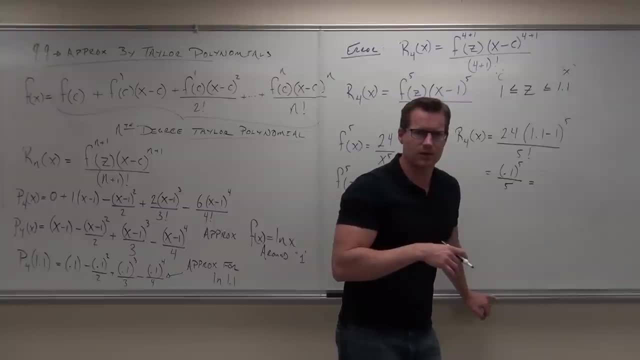 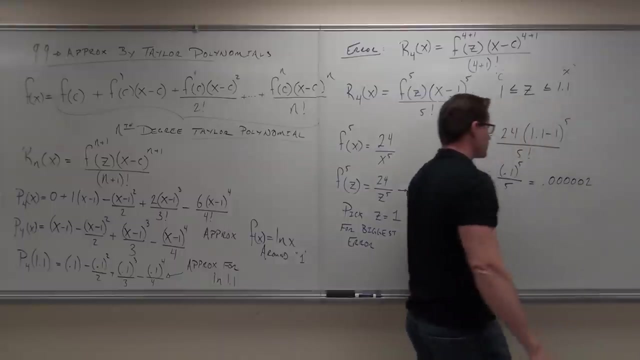 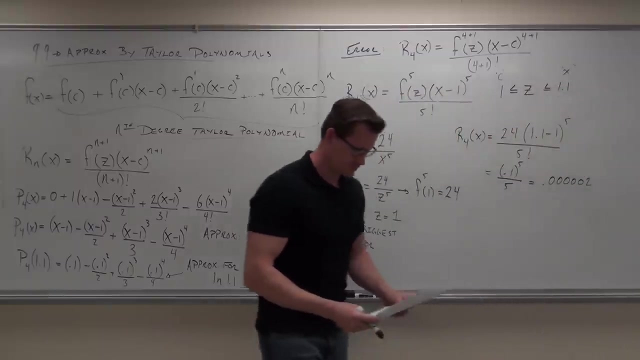 So .50 or something. Don't leave me hanging Three times 10 to the negative six. Well, there's even a six. There you go, Thank you. Now I said this goes fast and they do go fast. I just had to explain this to you. 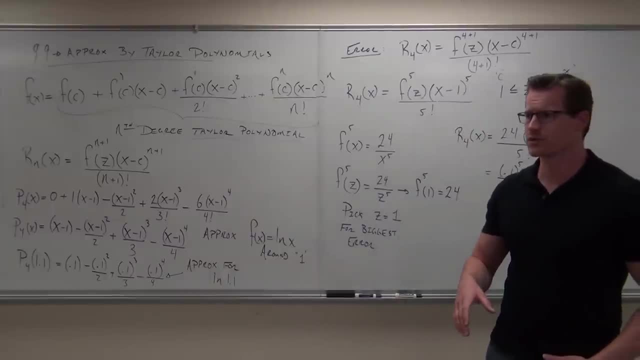 But this does go quite quickly, because all you've got to do is do a few derivatives and then you're going to plug in a number and then you're going to find an error. So here's what we just said. Are you with me? 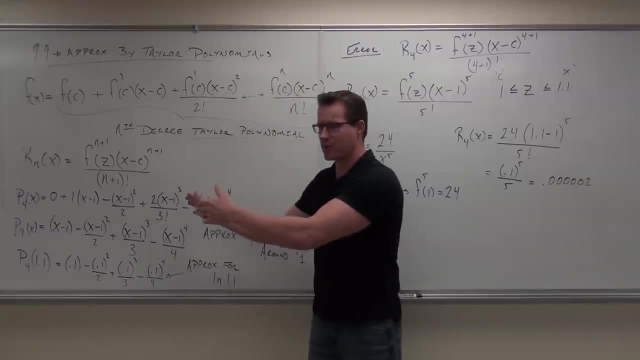 Mm-hmm. We cut a Taylor series short called Taylor polynomial. there is some sort of error associated with that. With our Taylor polynomial, all you've got to do is plug in a number you want to approximate, as long as you base that Taylor polynomial around the number. 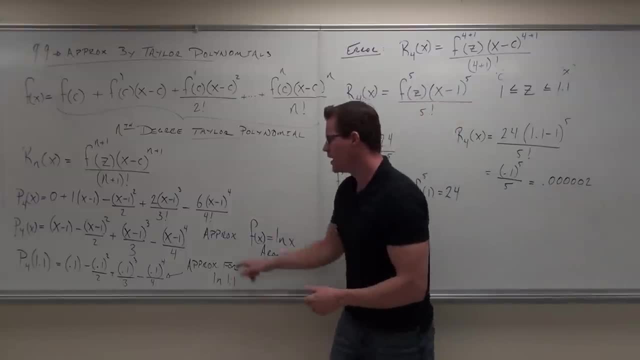 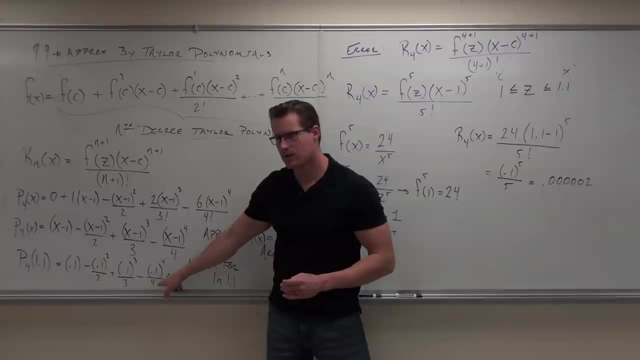 So in our case, we base it around 1 because we're trying to approximate 1.1.. Just plug it in. By the way, has anyone worked this out? Did you do it? How much is it? 0.095308333. 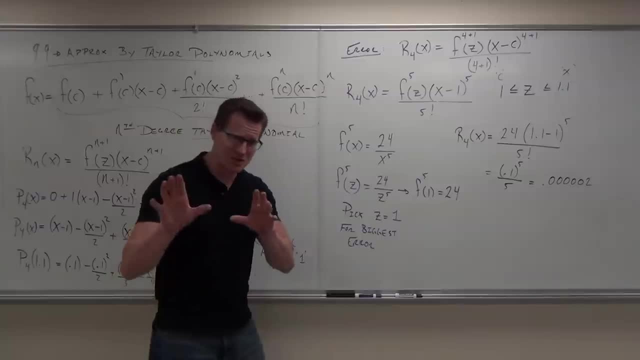 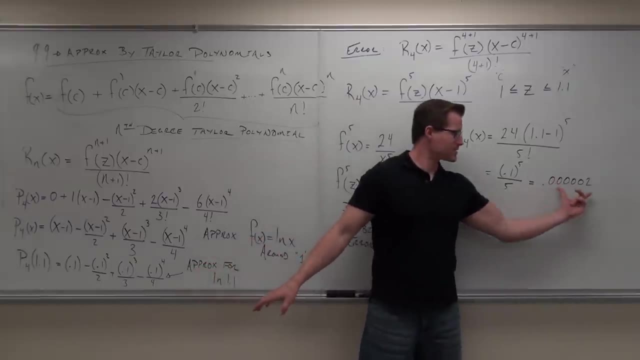 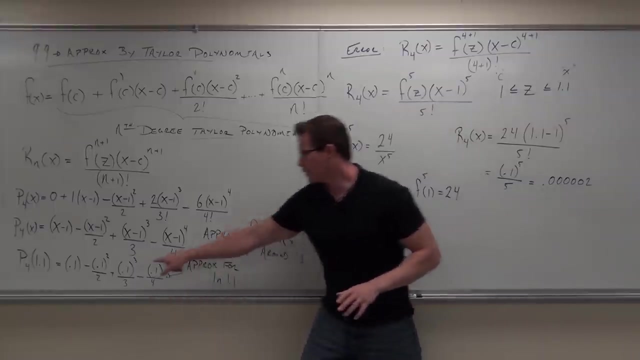 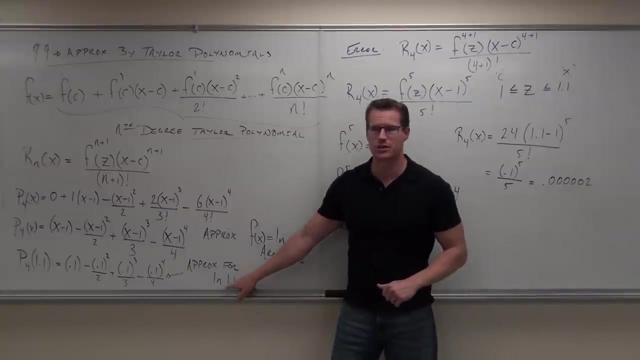 Assuming you're right- I'm not going to double check you- So assuming that you're right, that approximation is within this number of what this really is for ln 1.1.. I'll say that one more time. When you work that out, when you work this out and you find it, this is within this distance from what this actually is. 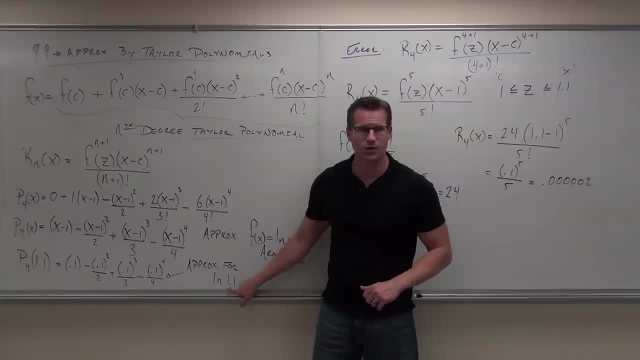 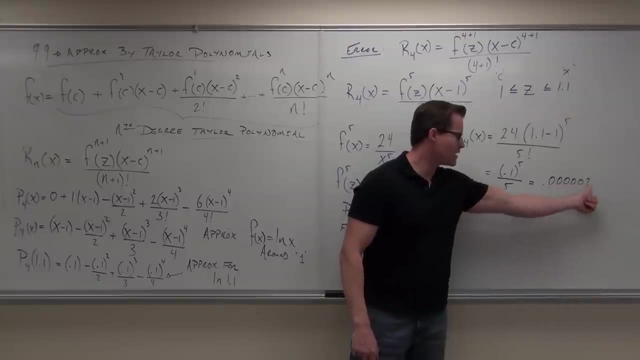 So is this an approximation of this? Yes, How close is it? Now? we know It's within 0.000.. 0.000.. tenths, hundredths, thousandths, ten thousandths, hundred thousandths, within two millionths. 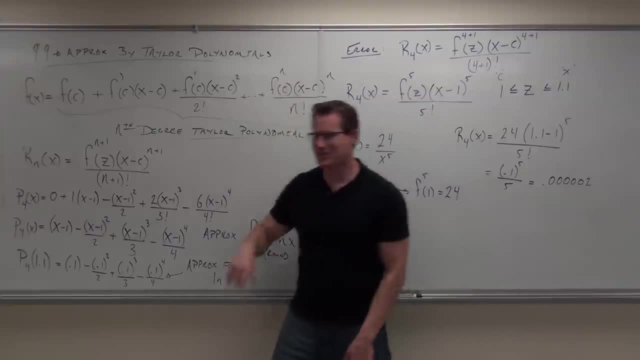 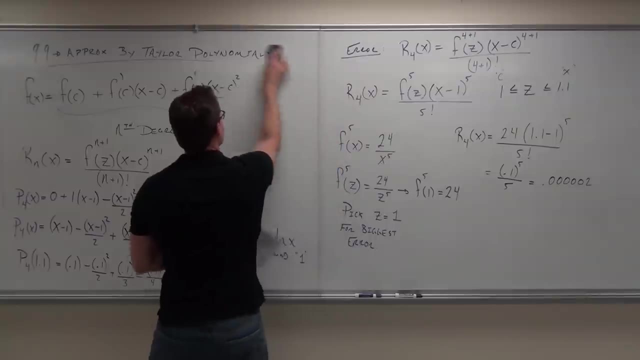 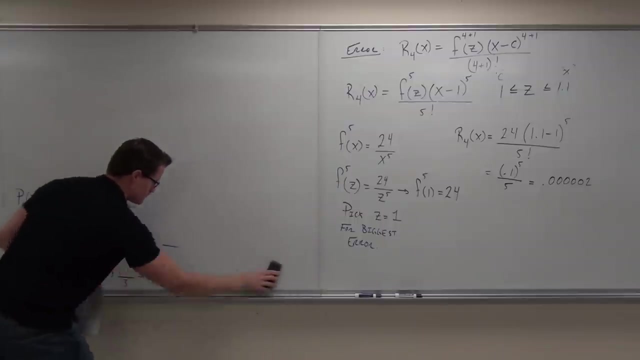 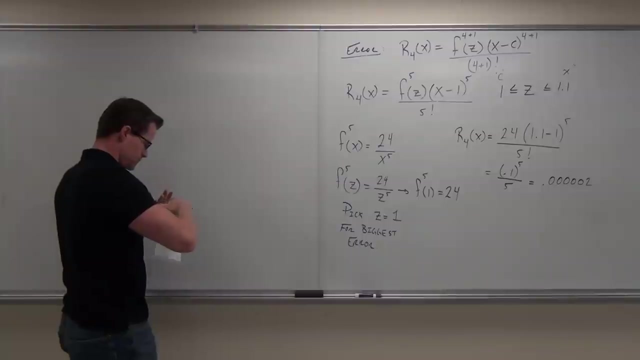 So it's pretty darn close Birds feel okay without that idea. Let's do another example, while this is freshening up our heads right now. It's an interesting idea though, isn't it? Yeah, Imagine if you didn't have calculators, and you had. 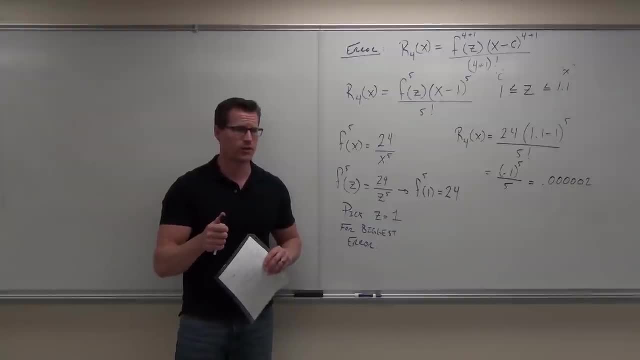 to be extremely close with your value and you didn't know what. ln of 1.1, ln of 1 is easy, it's 0, but ln of 1.1, how are you going to do that without a calculator? 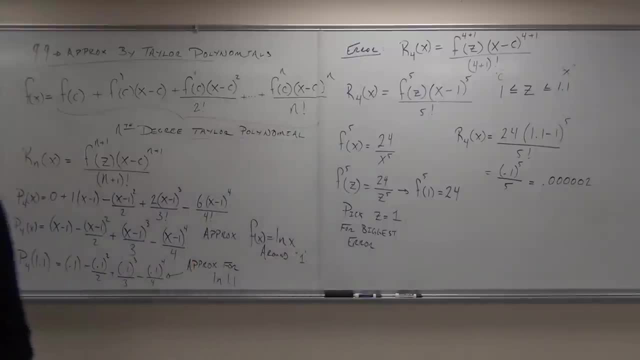 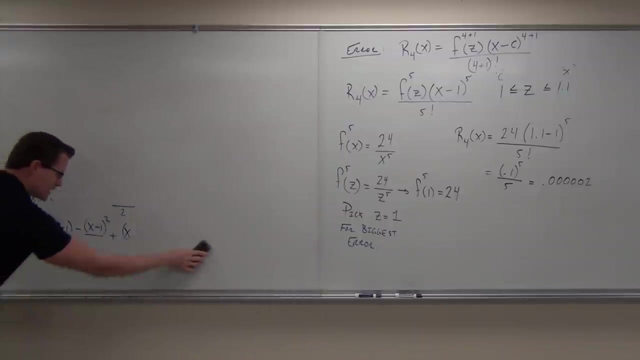 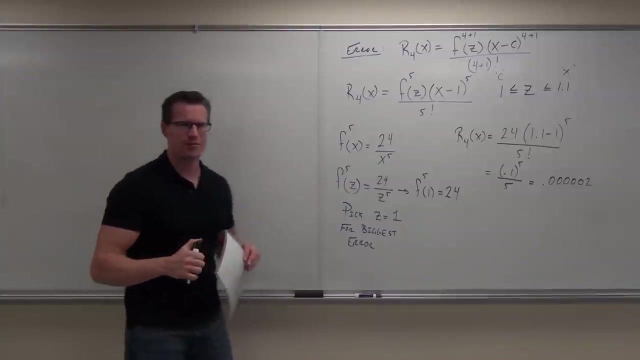 So you'll be okay with that idea. Let's do another example. while this is fresh in our heads right now, It's an interesting idea though, isn't it? Yeah, Imagine if you, If you didn't have calculators and you had to be extremely close with your value. 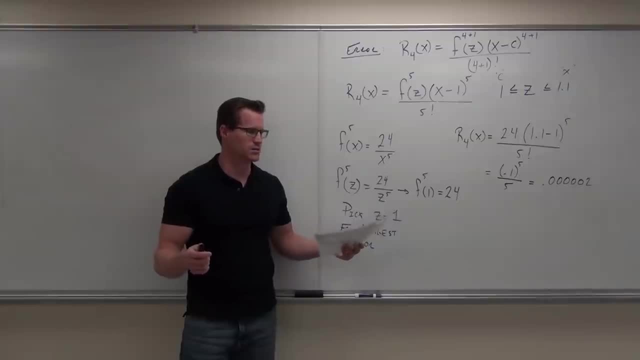 and you didn't know what. ln of 1.1.. ln of 1 is easy, It's 0. But ln of 1.1, how are you going to do that without a calculator? How would you do it? I would probably use Taylor polynomials and just do it to like the 10th degree. 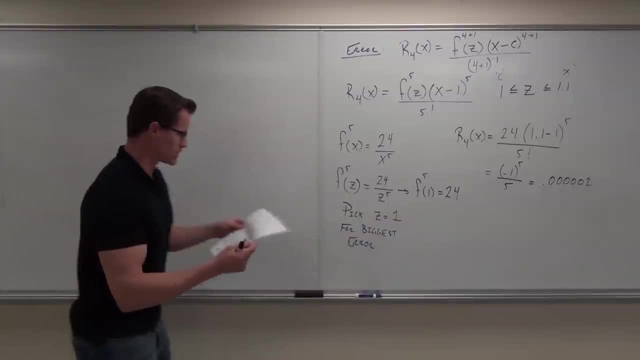 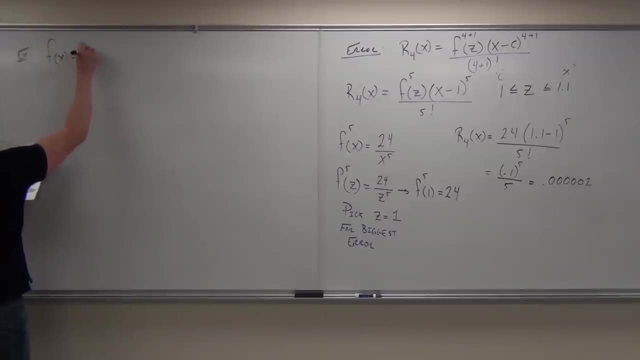 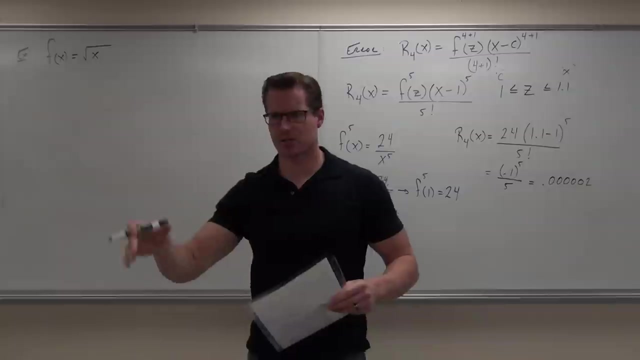 It's going to be super freaking close and you can prove how close it is. That's interesting. Okay, Let's try another one. Let's do the square Square root of x. Here's how your test question is going to look. 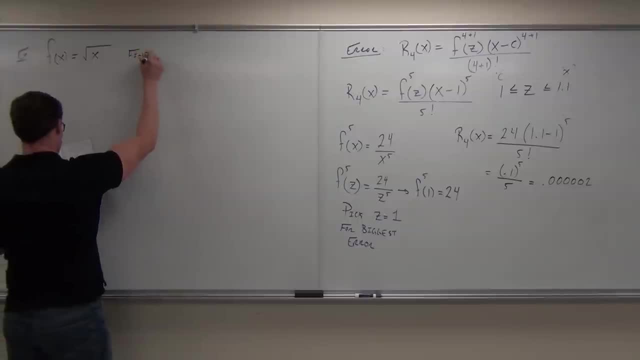 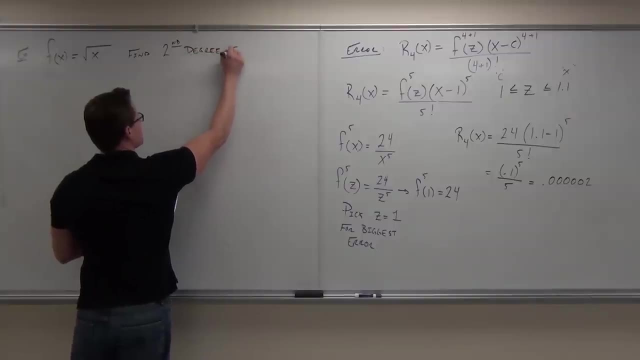 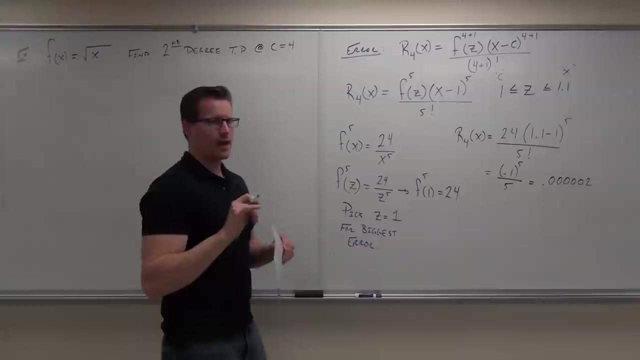 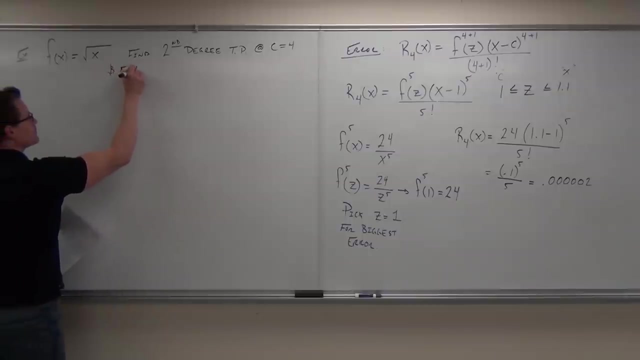 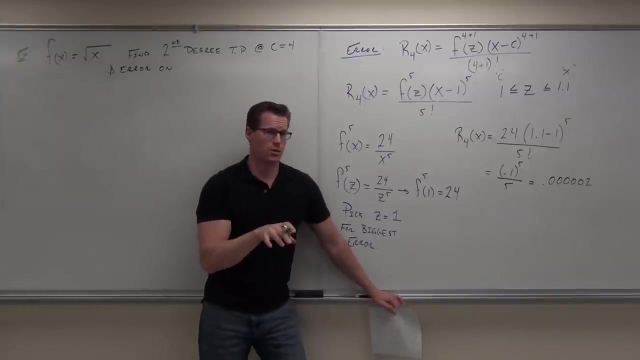 What I want is find the second degree Taylor polynomial at c equals 4.. And I want the error on a given square, On a given interval. By the way, if my c equals 4, do you follow that my interval is probably going to be somewhere around 4?? 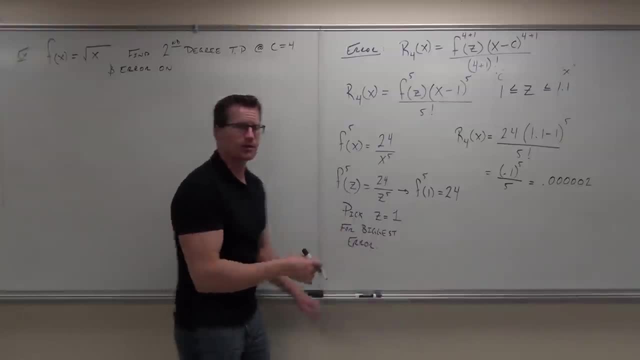 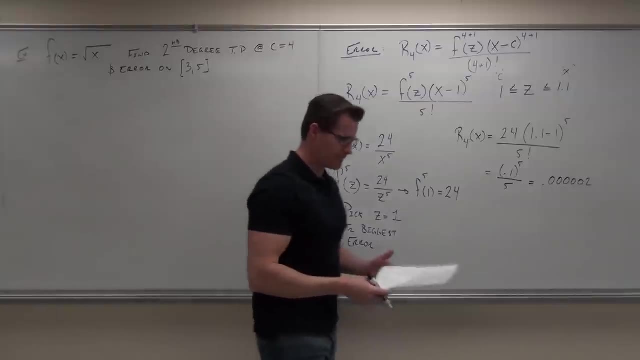 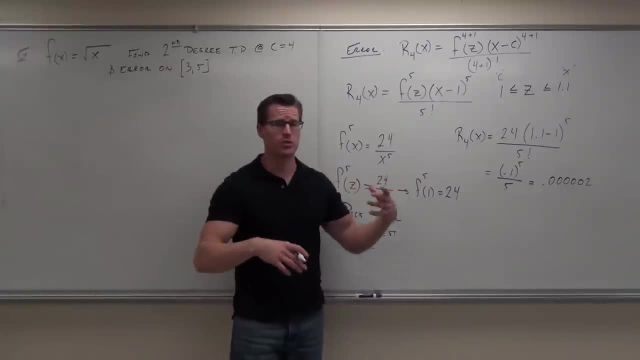 So it's not going to. I kind of made up the last one to give you how you would do this in real life. okay, You pick something close to it and you go for it For us. it says: all right, I'll tell you what I want: a second degree Taylor polynomial. 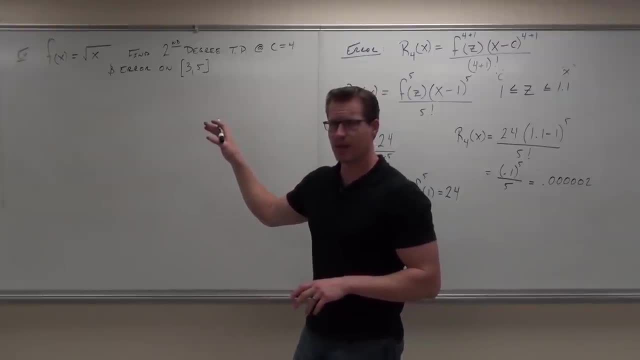 I want you to find this Taylor polynomial: centered at c equals 4.. And I want you to find the error if I approximate something between 3 and 5.. This is what this means. So when you find the error later on, it says: you know what? tell you what? give me any number between 3 and 5 inclusively. 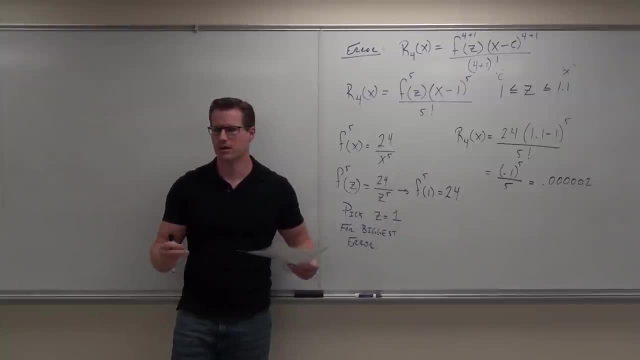 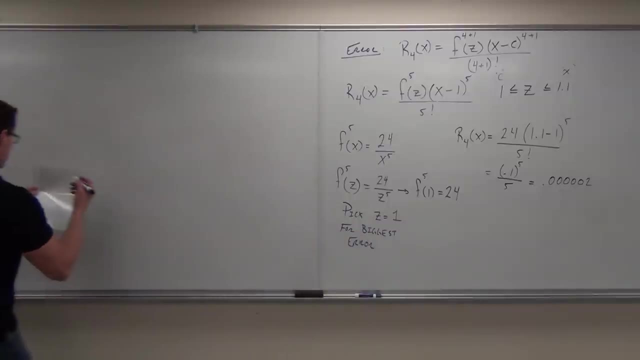 How would you do it? I would probably use Taylor polynomials and just do it to like the 10th degree. it's going to be super freaking close and you can prove how close it is. That's interesting. Okay, let's try another one. 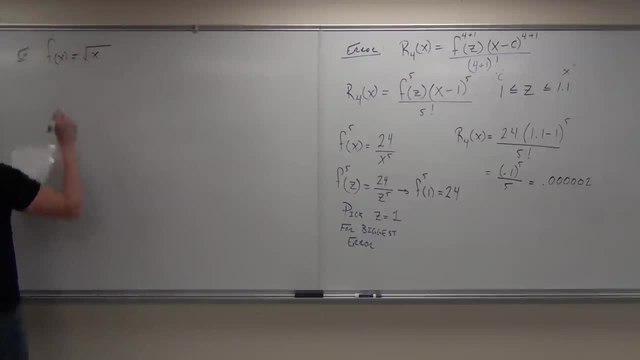 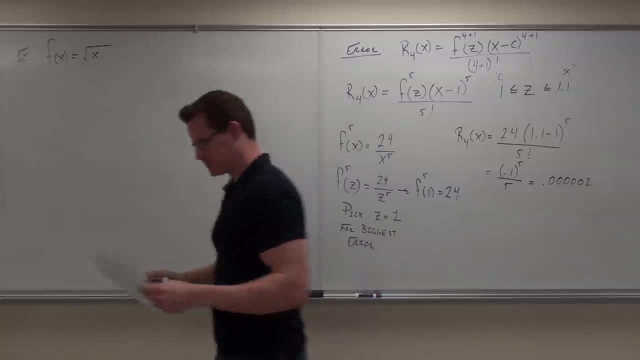 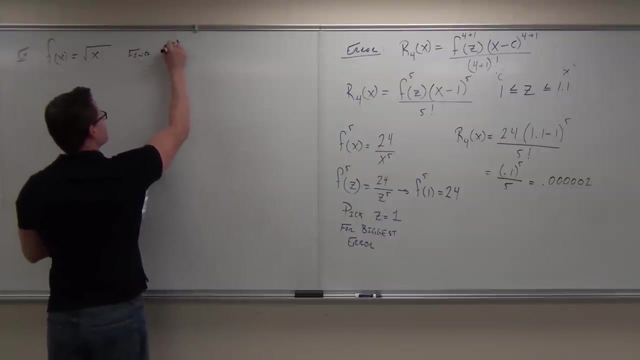 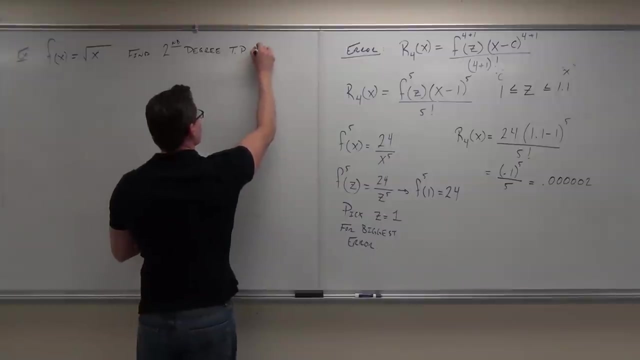 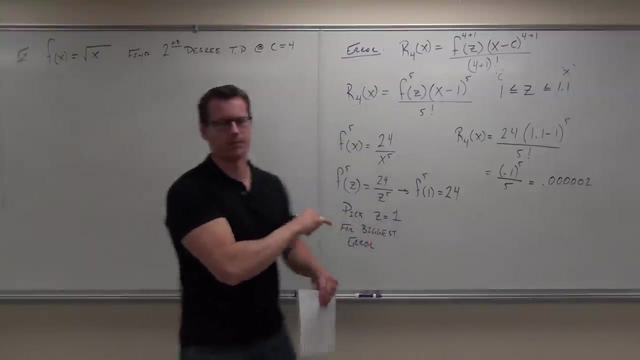 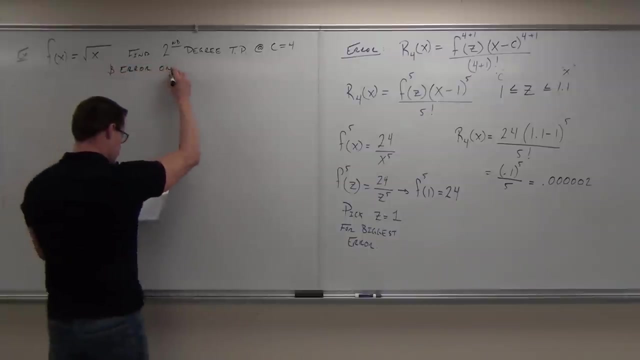 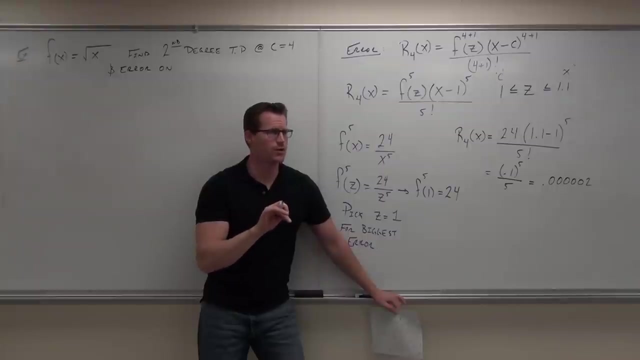 Let's do the square root of x. Here's how your test question is going to look. What I want is find the second degree Taylor polynomial at c. So I want c equals 4 and I want the error on a given interval. By the way, if my c equals 4, do you follow that my interval is probably going? 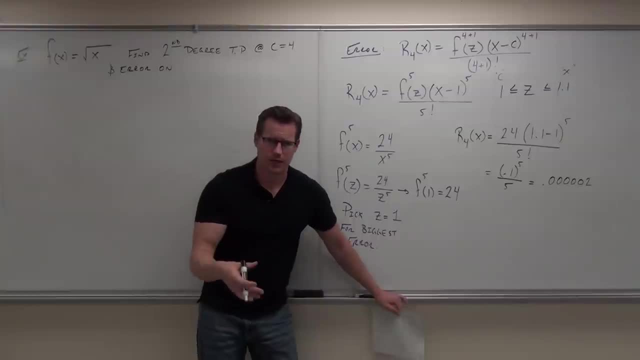 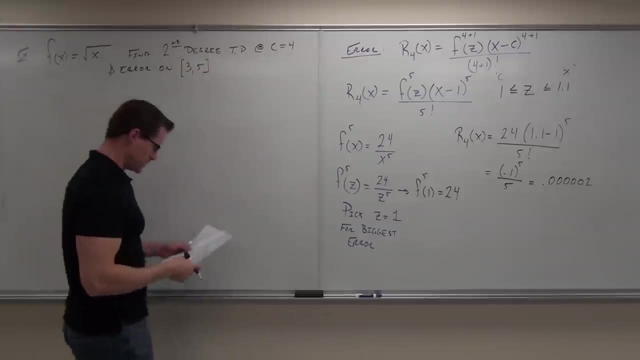 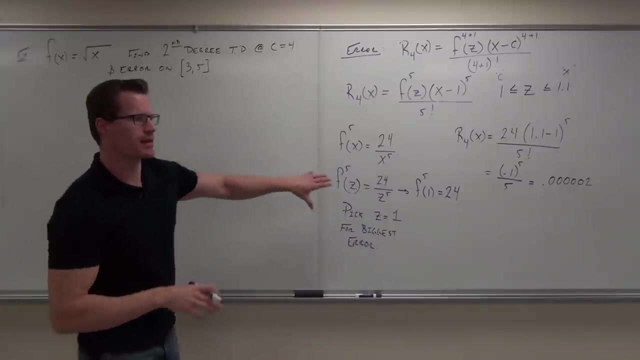 to be somewhere around 4?. Yeah, In our case, right now, it's going to be 3 to 5.. This is how it's going to be worded for you guys, So it's not going to. I kind of made up the last one to give you how you would do this. 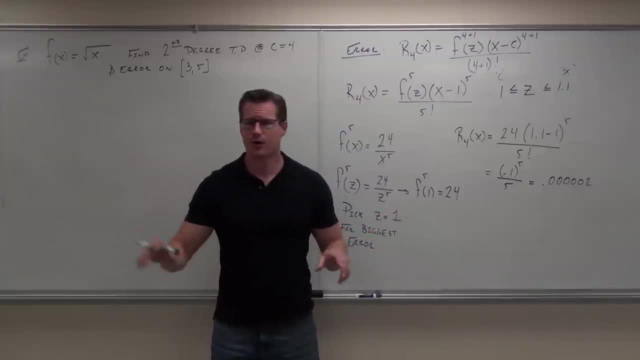 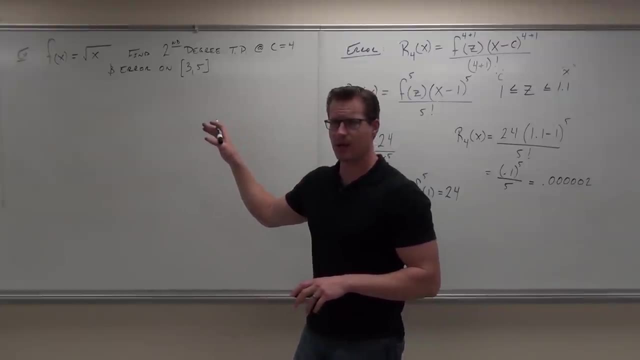 in real life. okay, You pick something close to it and you go for it. For us. it says: all right, I'll tell you what I want: a second degree Taylor polynomial. I want you to find this Taylor polynomial, centered at c equals 4, and I want you. 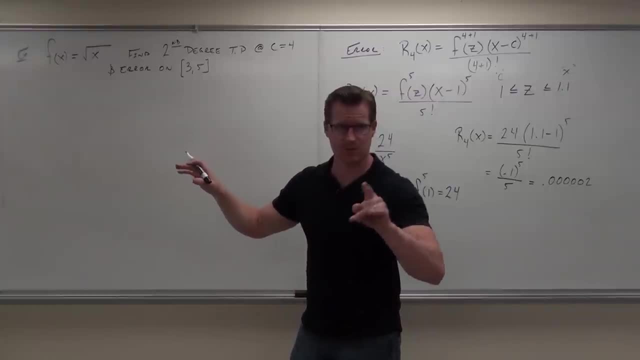 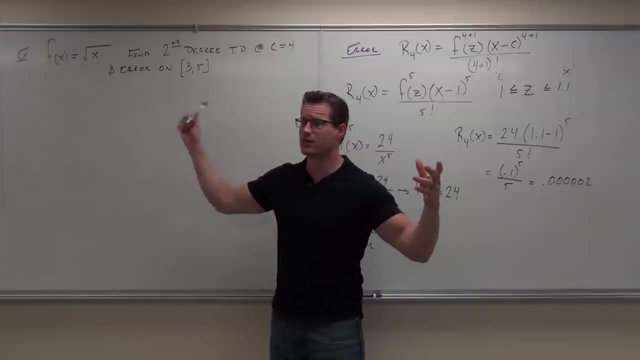 to find the error if I approximate something between 3 and 5.. This is what this means. So when you find the error later on, it says: you know what? tell you what? Give me anything, Any number between 3 and 5 inclusively. plug it into your Taylor polynomial. 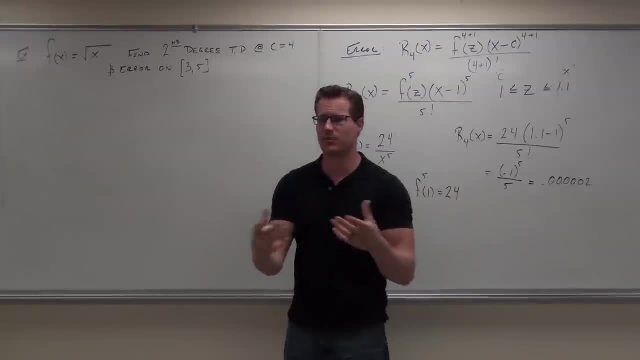 and I guarantee the error is going to be less than blank. Does that make sense to you? So within this interval we have a maximum error. You get it. That's why we pick the number that you think is the biggest error here. 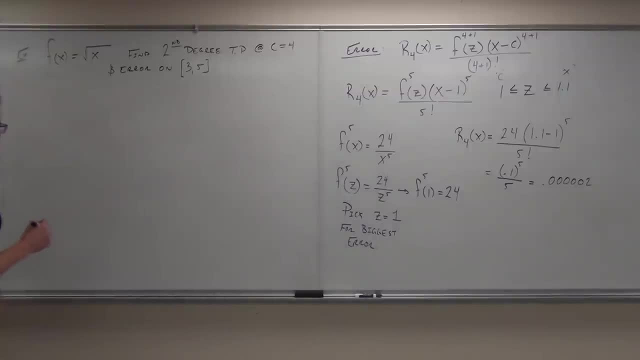 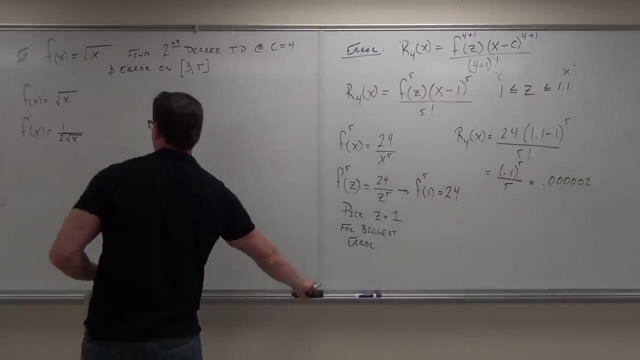 So let's continue. How do we start? Yeah, just like the Taylor series. So we're going to have f of x, We're going to have f prime of x Next, Next, I don't know what effect, Probably going to be a little bit easier, just to ____. 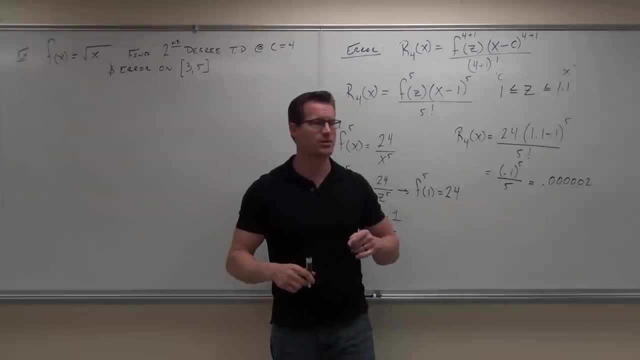 Plug it into your Taylor polynomial And I guarantee the error is going to be less than blank. Does that make sense to you? So within this interval we have a maximum error. You get it. That's why we pick the number that you think is just the biggest error here. 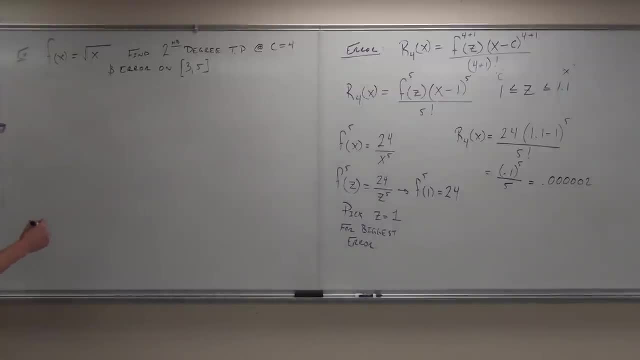 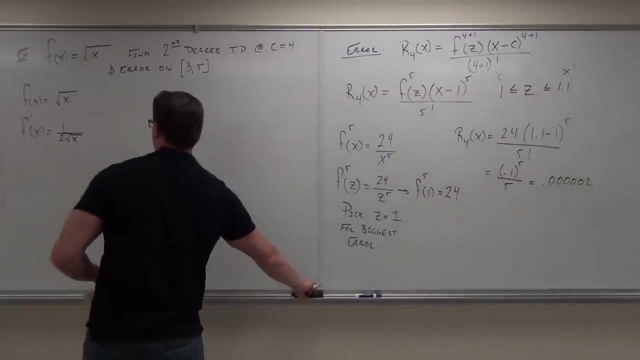 So let's continue. How do we start? Yeah, just like the Taylor series. So we're going to have f of x. We're going to have f prime of x. Second of all, this is going to be f prime of x. 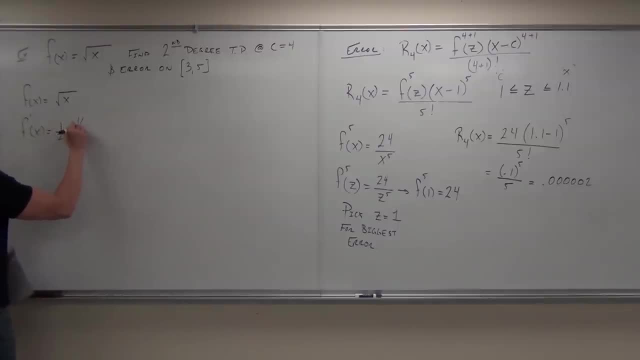 And we're going to have f prime of x, Next one: Oh, Lets see. Okay, That's probably going to be a little bit easier instead of doing What next? Do we need to keep going? Yes, How much is it? 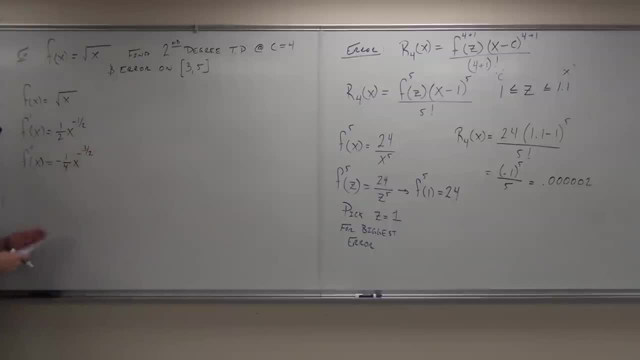 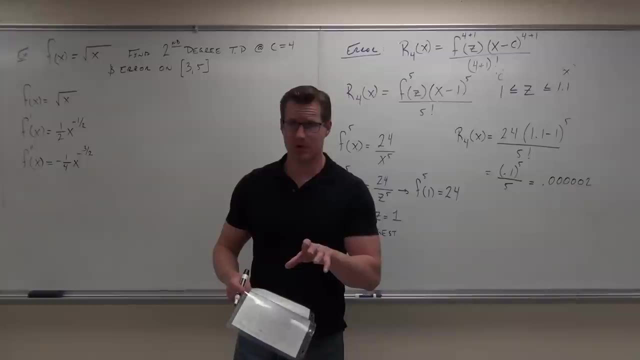 Like two and a half, Uh huh, Yeah, Like. Do I have to keep going? Yes. Do I have to keep going for my Taylor polynomial? No. Do I have to keep going for my error? Yes. Okay, so I'm going to write this down here. 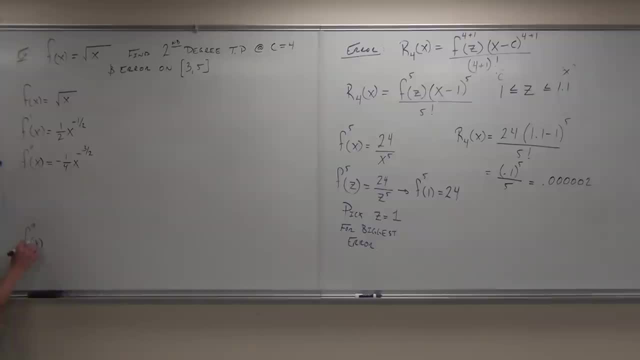 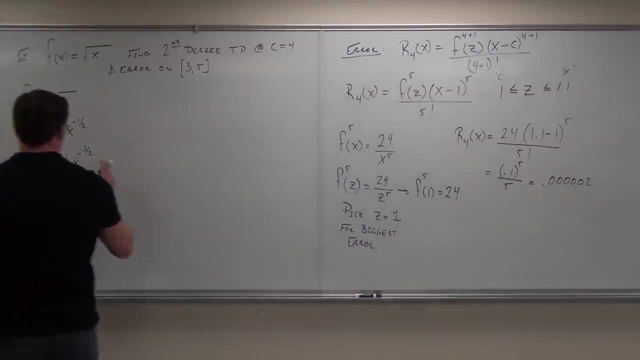 I'm going to leave this one, One, two, three, A third derivative. we go one more derivative than whatever degree I want, because that's going to give us our error. So here we're going to have. what is that positive three-eighths? 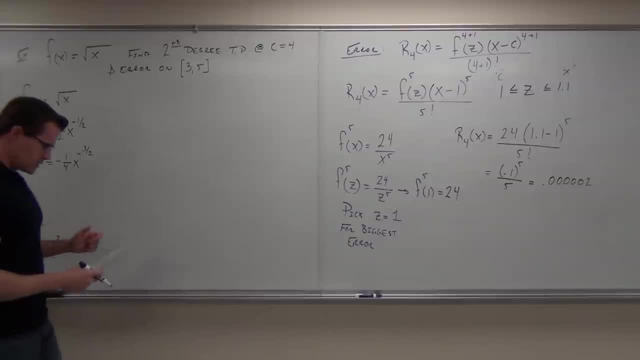 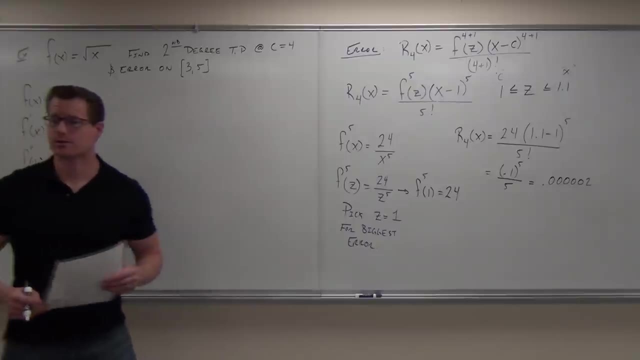 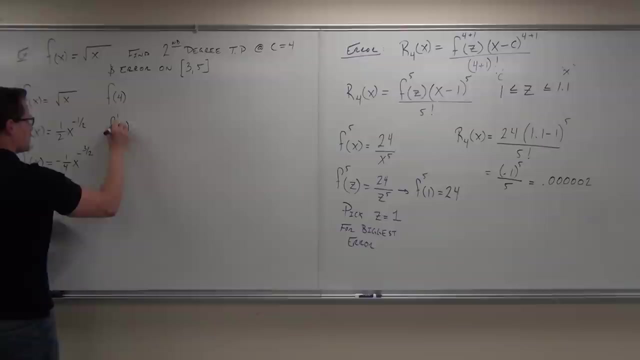 Next to the negative five-halves. alright, that's cool. Now what? What is our c in our case? So what we want is: we want f of four and we want f prime of four, and we want f double prime of four and ultimately we're going to have f triple prime of four and we want. 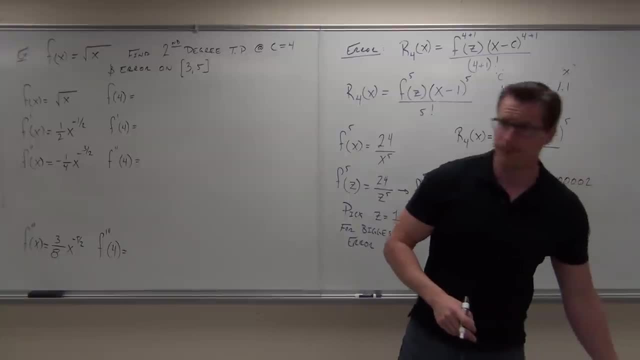 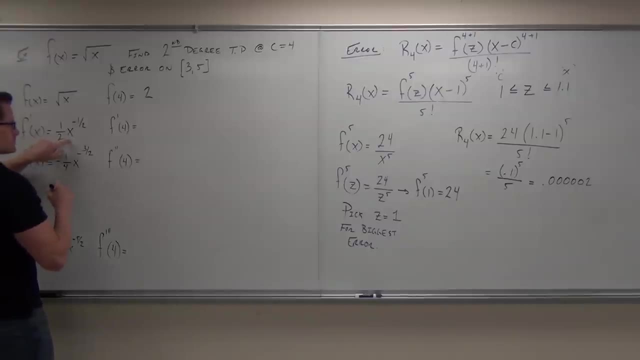 f: Okay, come on. I want your help with this real quick. What do we get? Two, Two, Two, Very good. What's next? One-fourth, One-fourth, You're right. What's next Negative one-third-second. 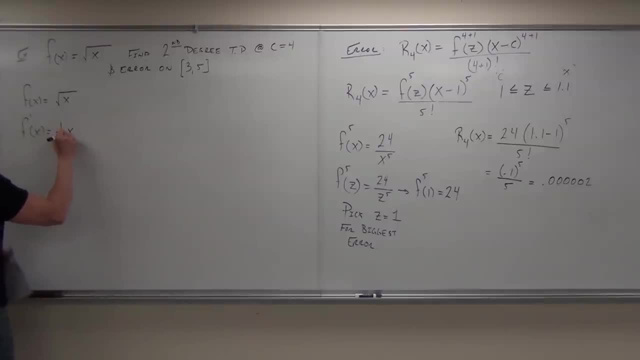 What next? Do we need to keep going? Yes, How much is it? I wasn't thinking about. I didn't think you were going to put that. Sure, You didn't put it in. Do I have to keep going? Yes, 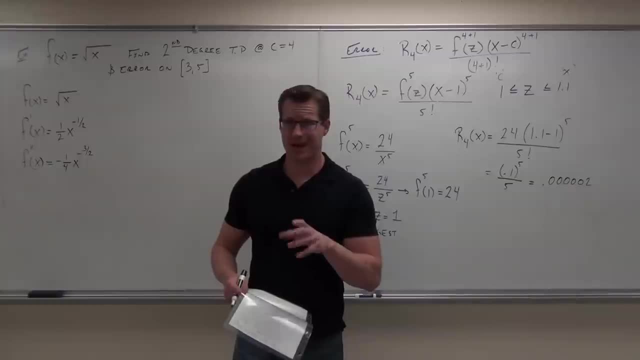 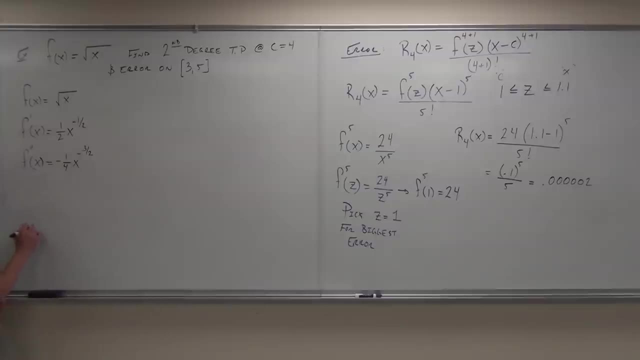 Do I have to keep going for my Taylor polynomial? No, Do I have to keep going for my error? Yes, Okay, so I'm going to write this down here. I'm going to leave this one. one, two, three. 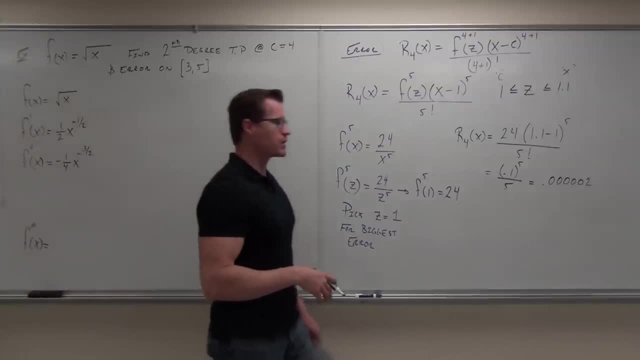 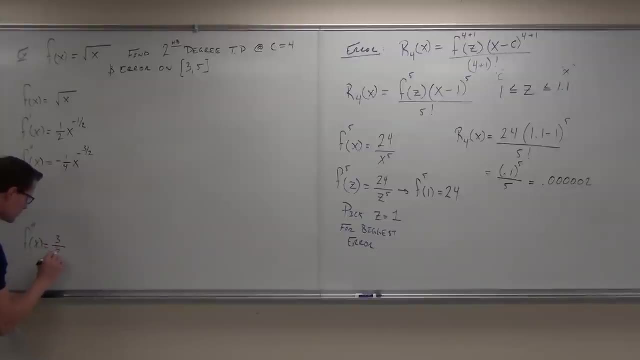 A third derivative. we go one more derivative than whatever degree I want, because that's going to give us our error. So here we're going to have what is that? positive three-eighths X to the negative five-halves- alright, that's cool. 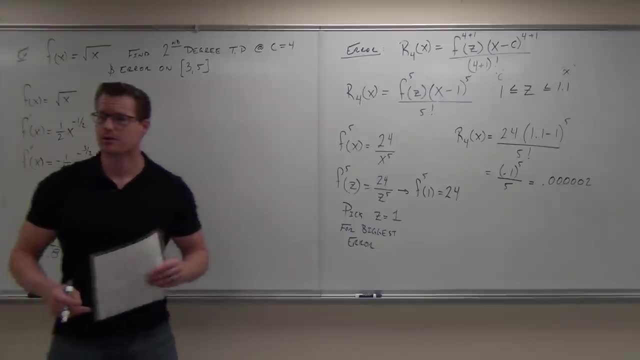 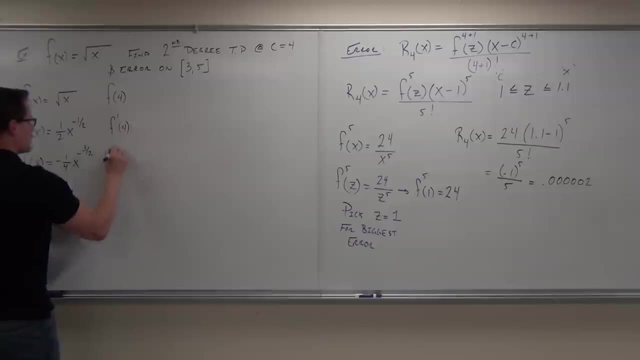 Now what? What is our C in our case? So what we want is we want F of four, and we want F prime of four, and we want F double prime of four and ultimately we're going to have F triple prime of four. 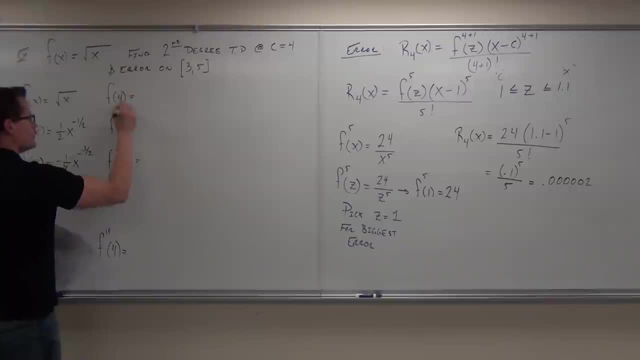 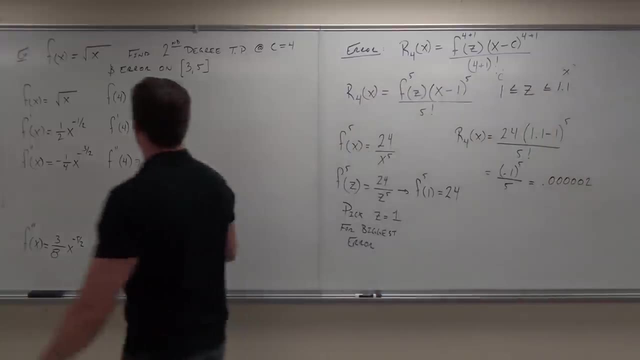 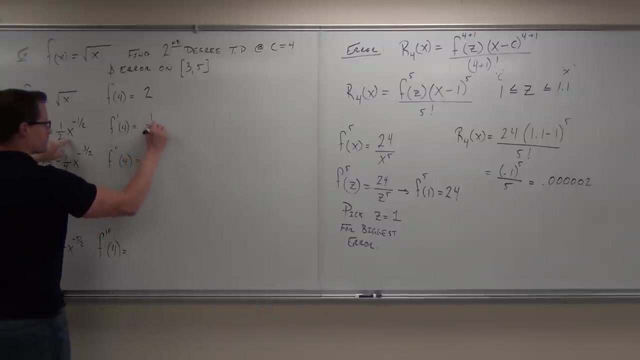 Okay, come on. I want your help with this real quick. what do we get? Two, Two, very good. What's next? One-fourth, One-fourth, you're right. What's next? Negative one-third-second. 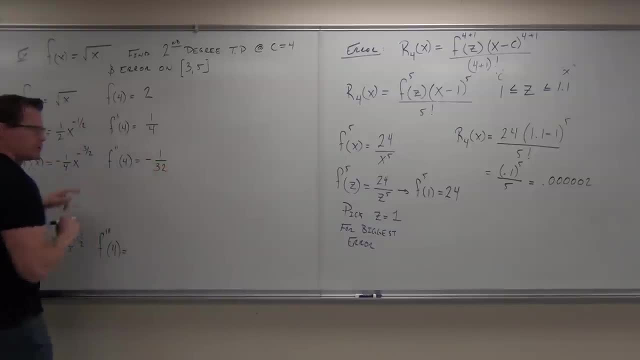 I think so. Do you know how we're doing those ones? This is negative, one-third-second Negative, one-third-second Negative, one over four times square root of four to the third. So you take the square root of four, that's two, to the third power, that's eight. 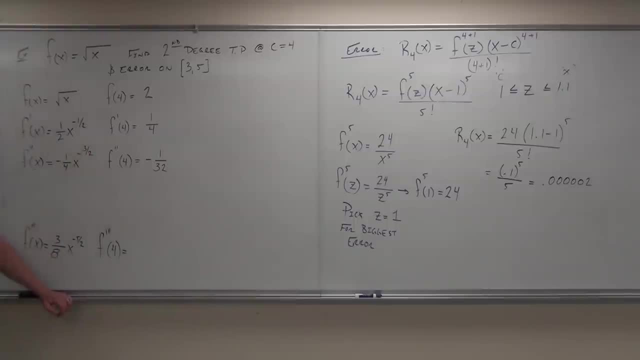 Eight times four is 32, it's negative. negative one over 32.. Let's do this one. So this would be: oh man, is that a little nasty. How much is that? Square root of four is Two to the fifth power. 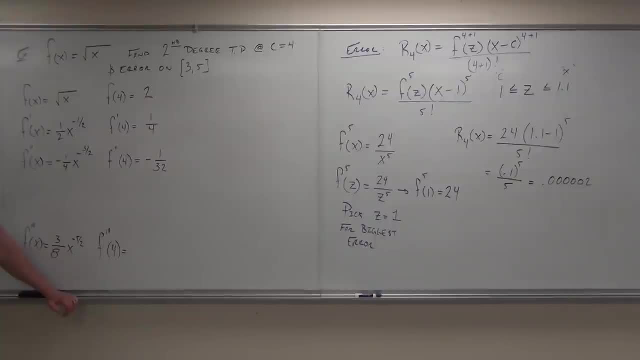 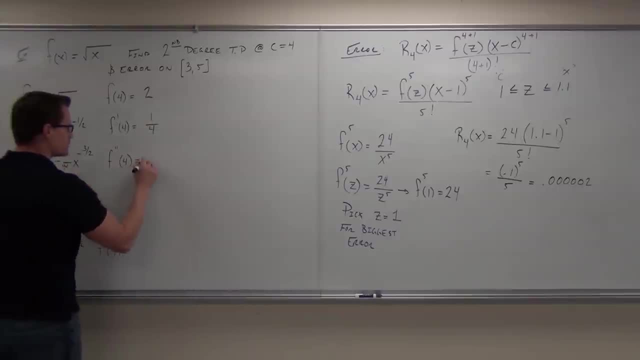 I think so. Do you know how we're doing those ones? This is negative one over four times square root of four to the third. So you take the square root of four to the third, You take the square root of four, That's two, to the third power. 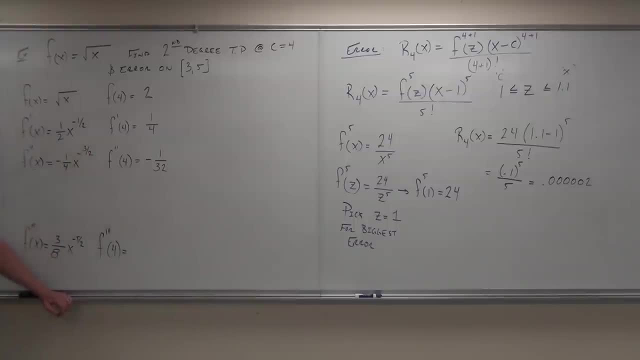 That's eight. Eight times four is thirty-two, It's negative, Negative one over thirty-two. Let's do this one. So this would be: Oh man, Is that a little nasty? How much is that? The square root of four is: 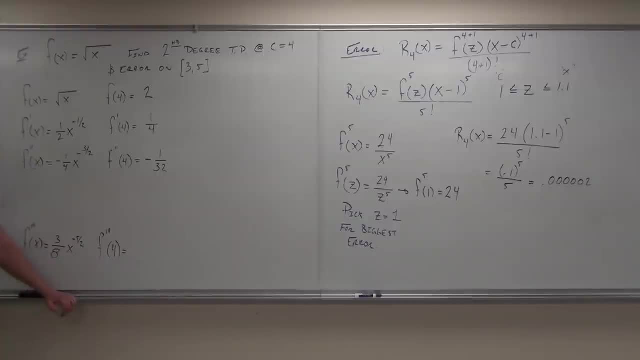 Two to the fifth, Two to the fifth power Times eight. whatever that happens to be, What is it? Are you over two-fifty-six? Two-fifty-six, Dang? Two-fifty-six, Two-fifty-six, Two-fifty-six? 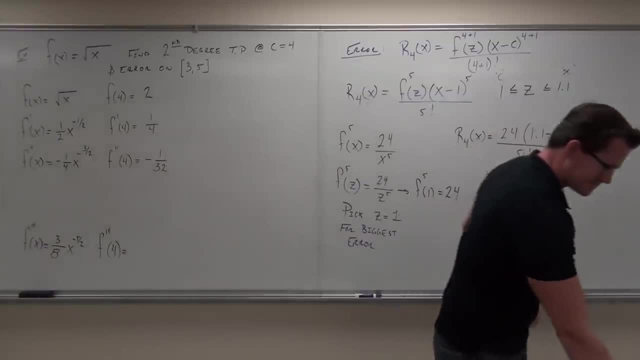 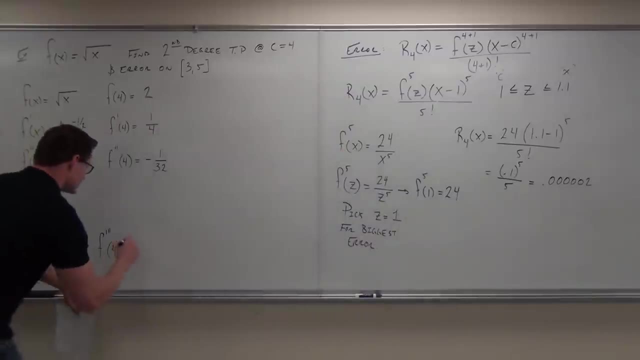 Two-fifty-six, Two-fifty-six, Two-fifty-six, Two-fifty-six? What is it? Are you over? two-fifty-six, Two-fifty-six, Dang, Yeah, Okay, Okay, We'll hang on to that one and remember to make sure real quick. 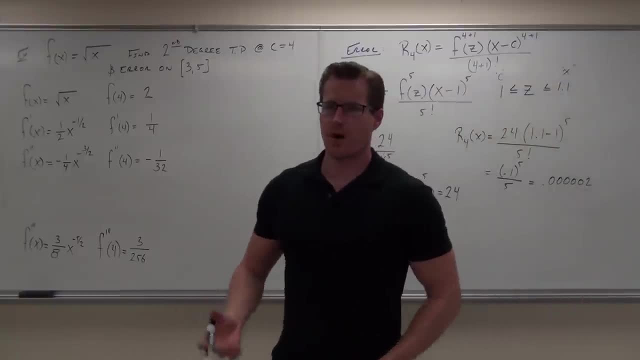 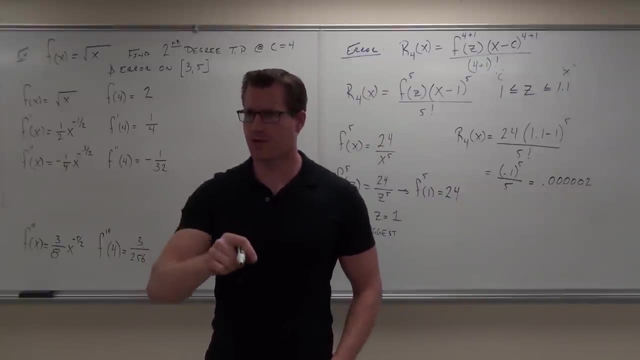 Now, do we need to find a pattern like a Taylor series? No, No, All we're going to do is write out the first. When I say degree two, you're going to have three terms. then You're going to have F, the first derivative of F and the second derivative of F, because 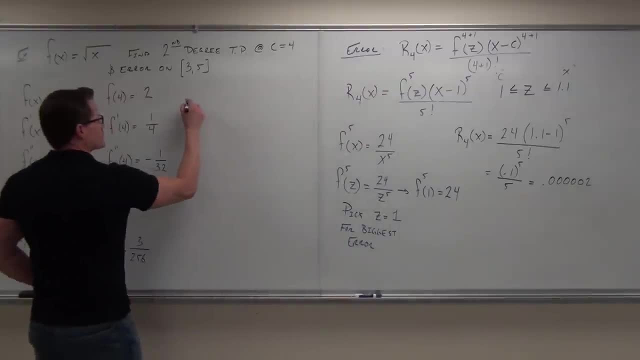 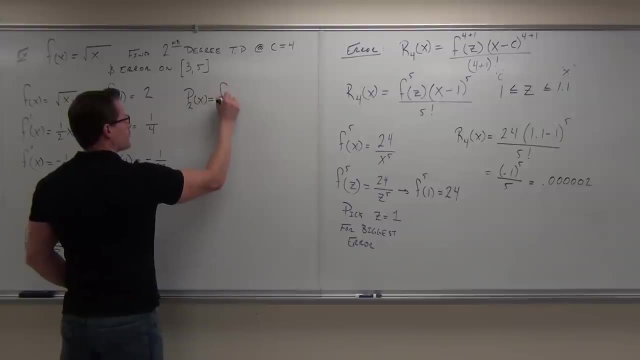 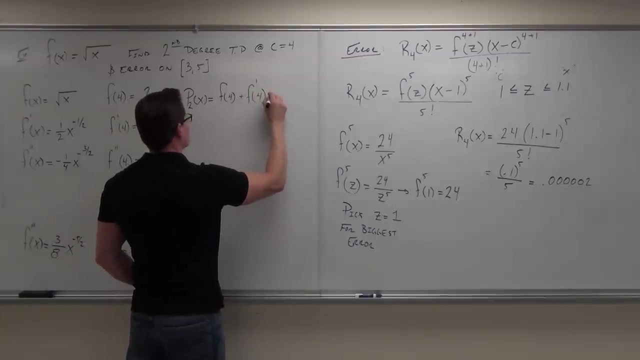 we're in a degree two polynomial, So let's do it. If we do this, our Taylor polynomial- Okay, of a second degree is going to be F of four plus F prime of four Square. I'll make the next one square. 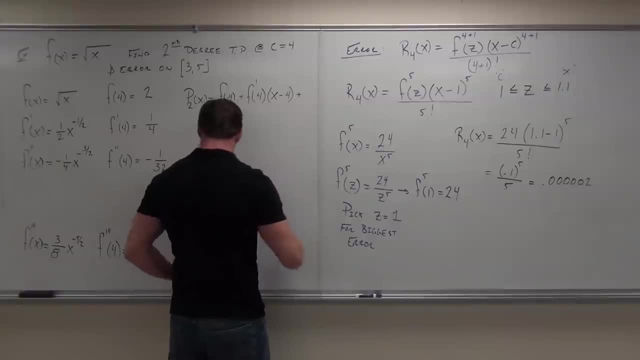 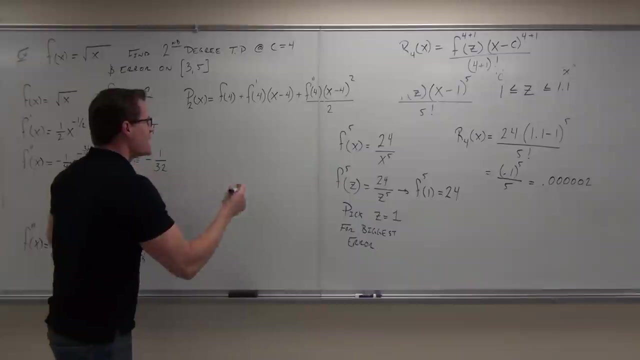 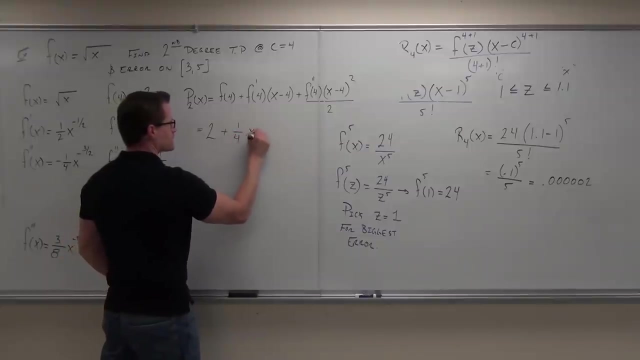 Next one's square. You're right, All over two, All over two. And then we start simplifying it. F of four, okay, that was two plus F. prime of four, that was one-fourth. X minus, four plus, if I wanted. 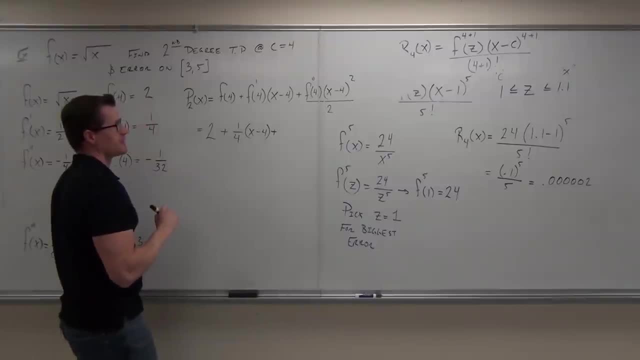 Let's see The second derivative. Oh my gosh, There's going to be a minus Minus one over thirty-two. So what's that going to give us all said and done? One over sixty-four, That's right. 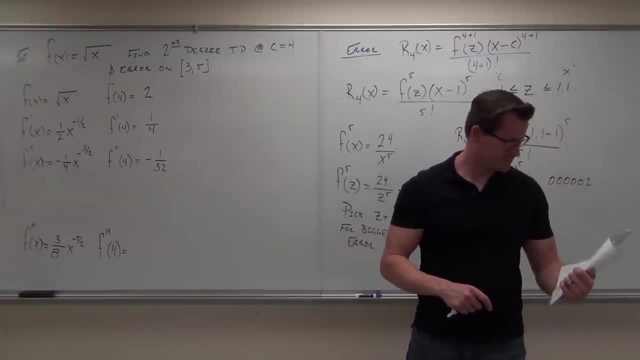 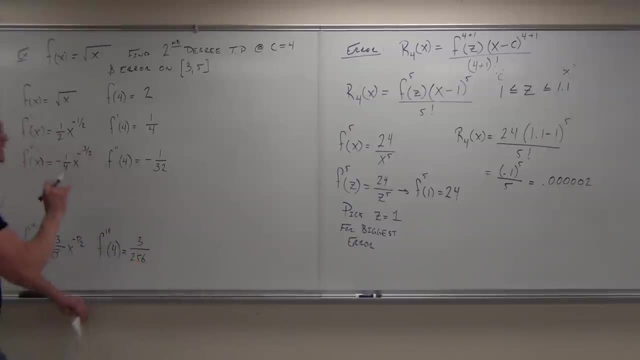 I don't know. I don't know What's that? Three over 256.. 256. Dang yeah, OK. OK, we'll hang on to that one and remember to make sure real quick Now. do we need to find a pattern like a Taylor series? 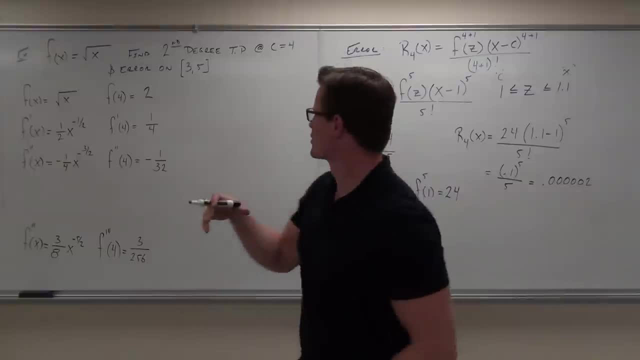 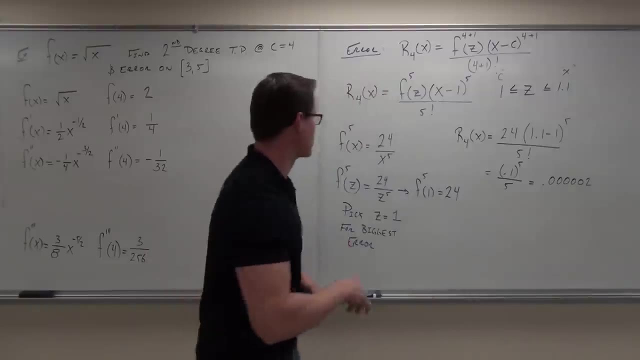 No, All we're going to do is write out the first. when I say degree two, you're going to have three terms. then You're going to have F, the first derivative of F, and the second derivative of F, because we have a degree two polynomial. 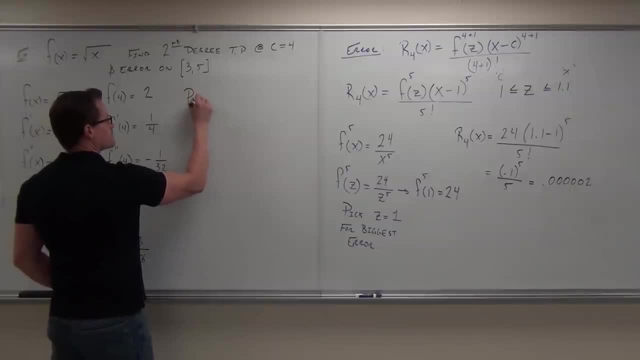 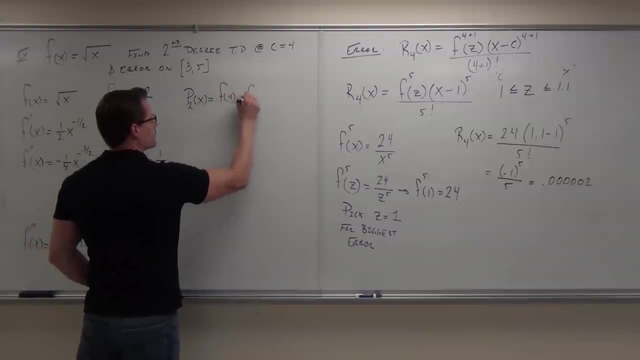 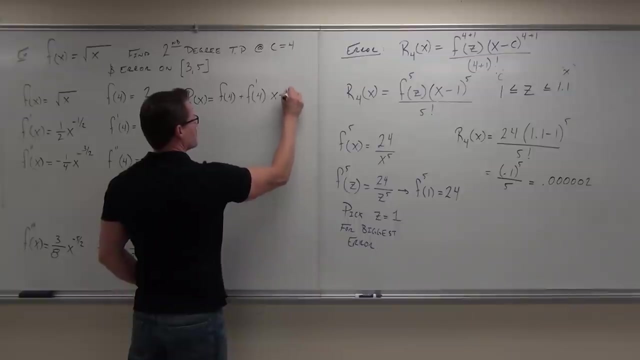 So let's do it. Our Taylor polynomial of a second degree is going to be f of 4 plus f, prime of 4. x minus 4.. Square. I'll make the next one square, The next one's square, You're right. 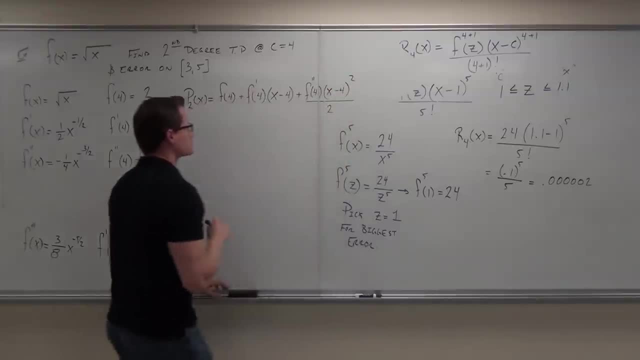 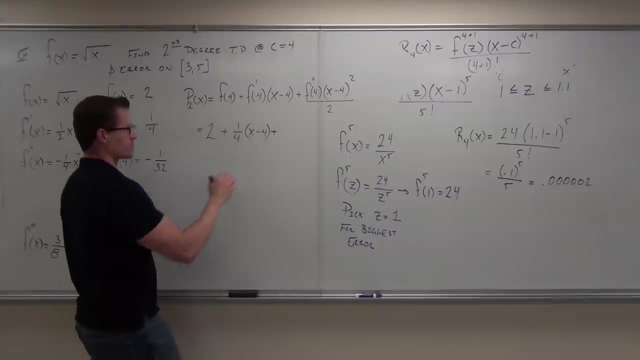 All over 2.. And then we start simplifying it: f of 4,- okay, that was 2, plus f. prime of 4, that was 1 fourth x minus 4.. Plus, if I wanted, let's see the second derivative. oh my gosh, it's going to be a minus. 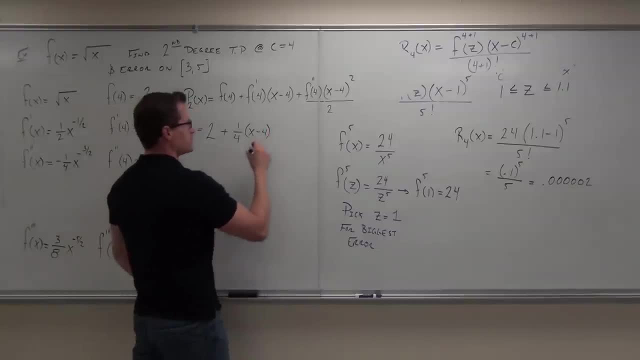 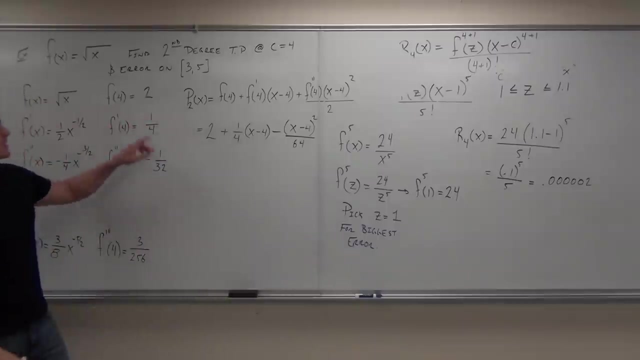 Minus 1 over 32.. So what's that going to give us all said and done? 1 over 64.. That's right, minus 1 over 64.. x minus 4.. Square over 64.. I want to make sure you guys are okay with this. 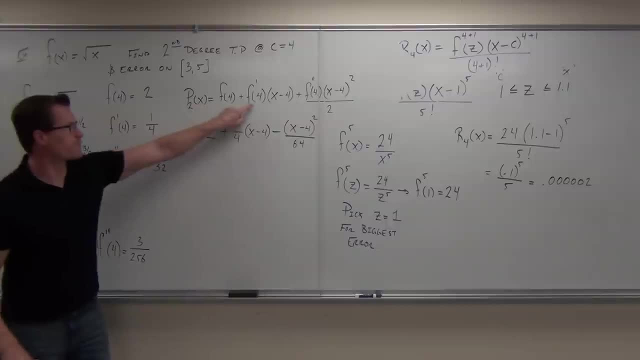 So f of 4 was 2,. no problem, f prime of 4 was 1 fourth. we get 1 fourth x minus 4.. Okay, well, this second derivative of 4 is negative: 1 over 32, are you with me? 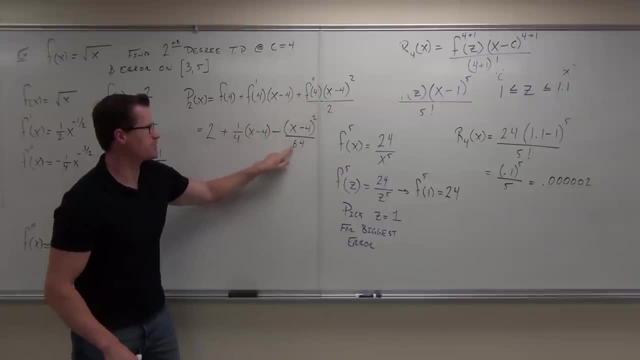 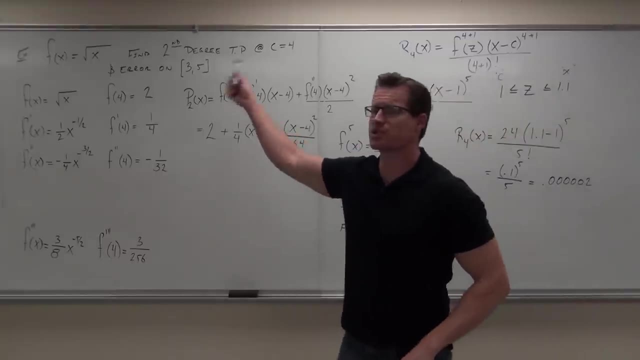 Negative 1 over 32 times 2 is negative 1 over 64, x minus 4 to the second power, not a problem. This answers the first part of the question. Did I tell you to approximate anything? No, All I want. 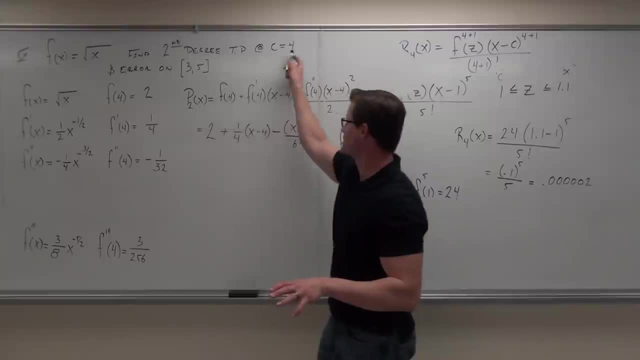 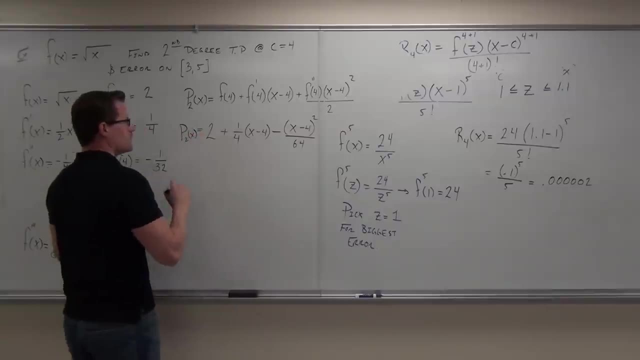 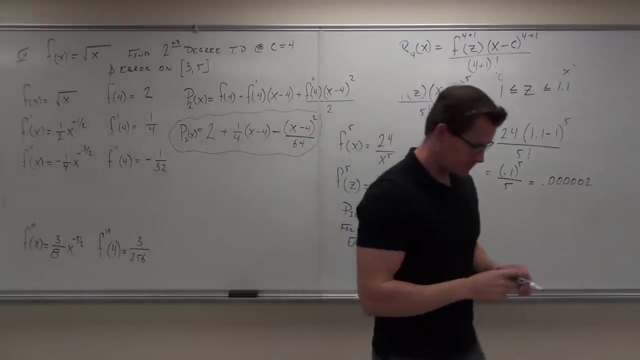 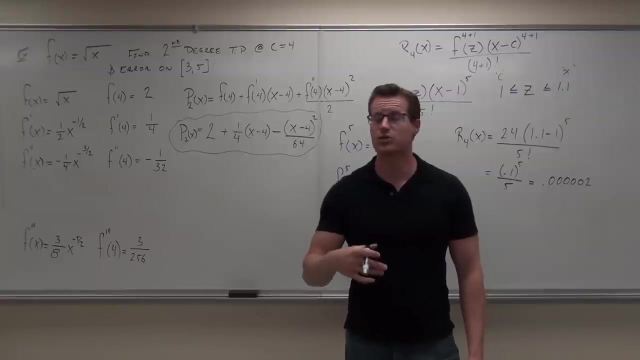 All I wanted was a Taylor polynomial of the second degree at c equals 4.. That's this. This is the Taylor polynomial of the second degree at c equals 4.. You guys are okay with that one Mm-hmm. Now this can be used to represent or to approximate. you say: 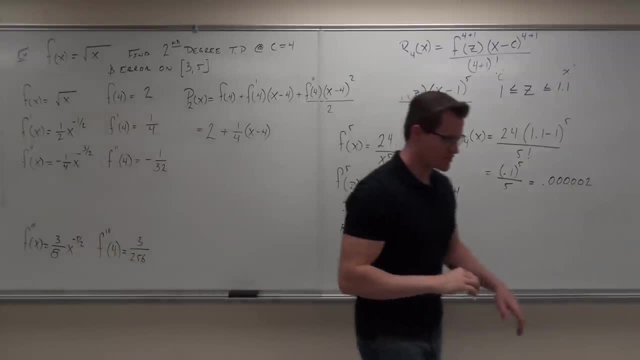 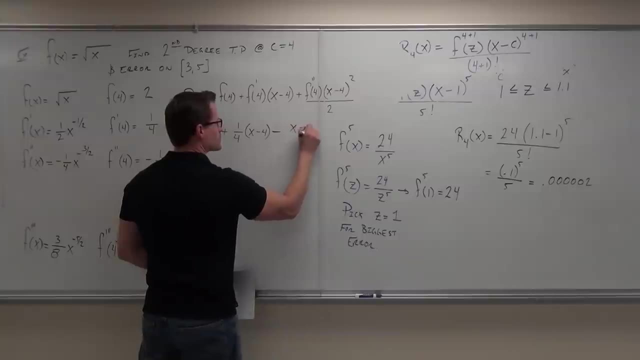 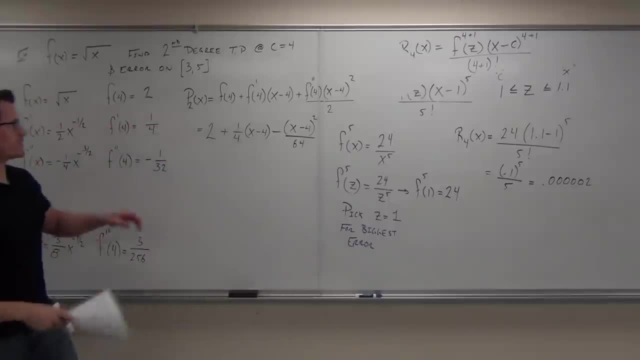 That's right. So this is. this is four squared over sixty-four. I want to make sure you guys are okay with this. So F of four was two, no problem. F prime of four was one-fourth. we get one-fourth X minus four. 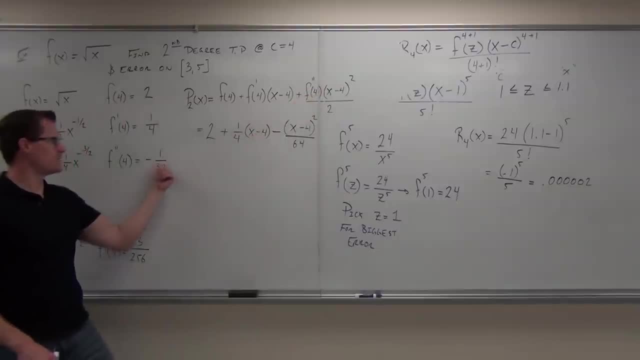 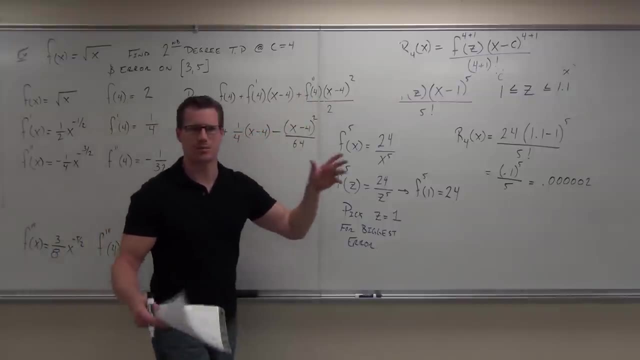 Okay, well, this second derivative of four is negative. one over thirty-two. are you with me? Negative one over thirty-two times two is negative. one over sixty-four. X minus four to the second power. Not a problem, This answers the first part of the question. 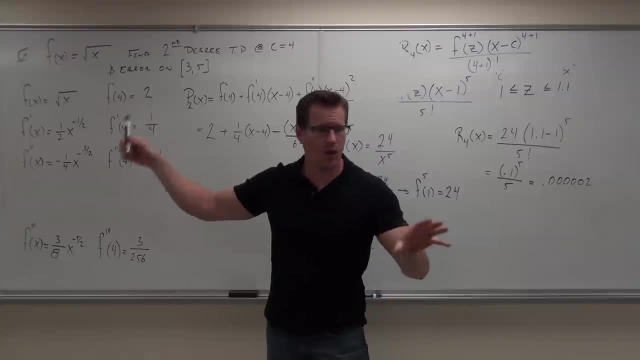 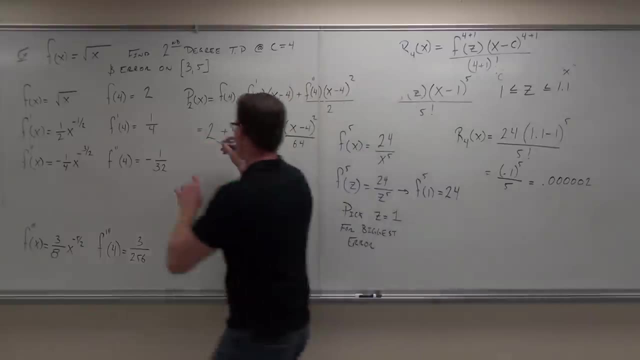 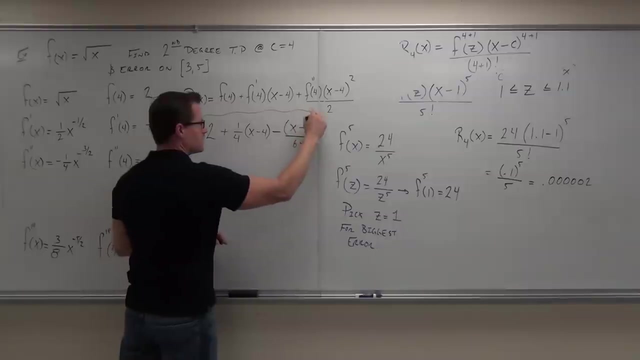 Did I tell you to approximate anything? No, All I wanted was a Taylor polynomial of the second degree at c equals 4.. That's this. This is the Taylor polynomial of the second degree at c equals 4.. You guys okay with that one? 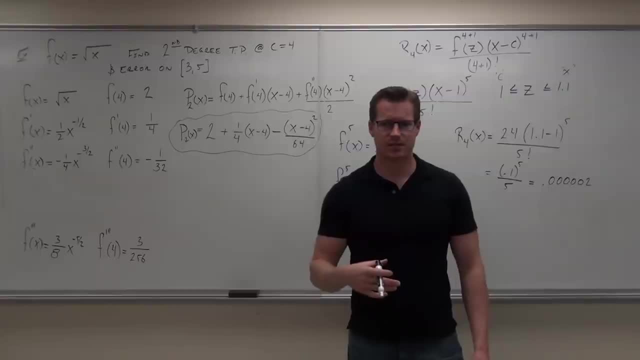 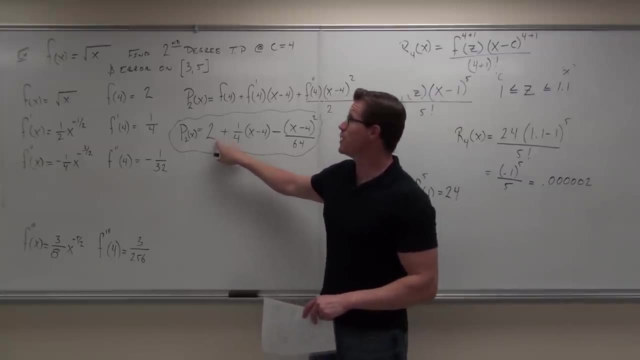 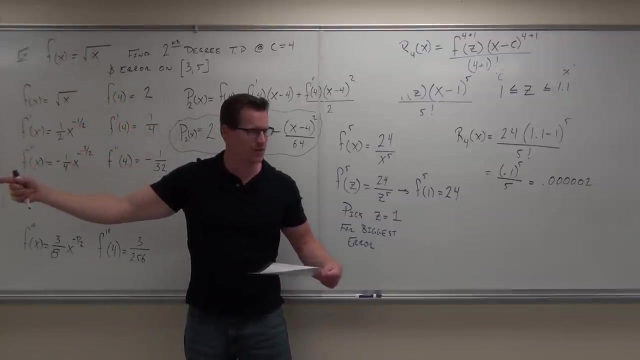 Now this can be used to represent or to approximate. you should say: This can be used. here's the idea here. This Taylor polynomial can be used to approximate this function on anything around 4.. Does that make sense? Do I need to write that down for you? 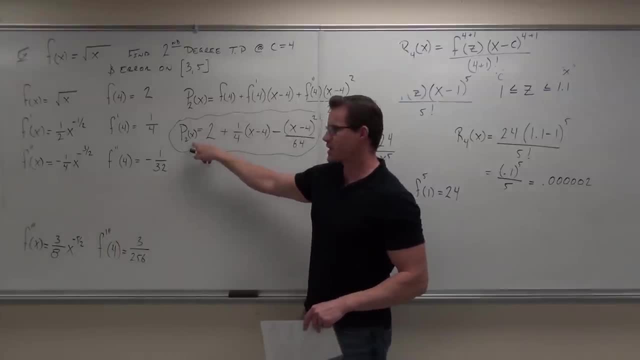 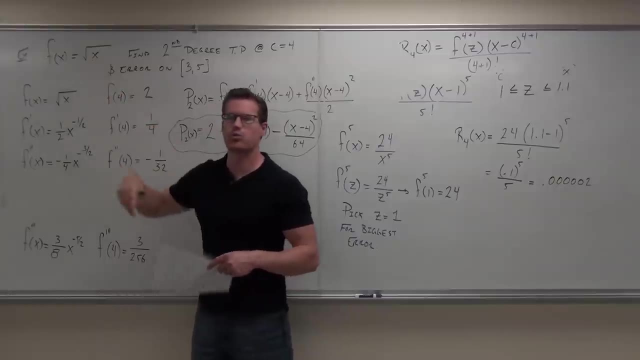 No, Okay, You sure, So you might want to write that down. This Taylor polynomial can be used to represent or approximate this function on anything around 4.. Why around 4?? That's our center. Now what we're going to do is say: 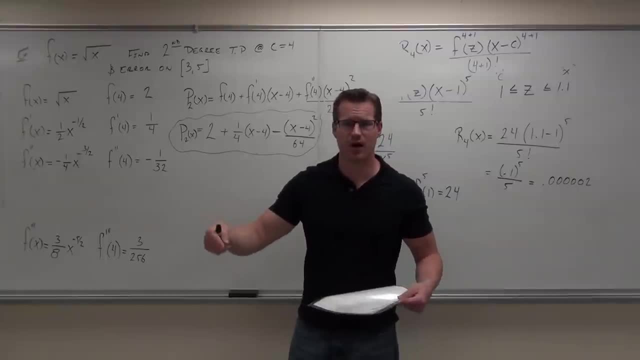 imagine you used it. You used it to represent or approximate a number between 3 and 5.. We're going to find out the largest error after probably the next time we come back, So I'll write this out real quick and then we'll stop here. 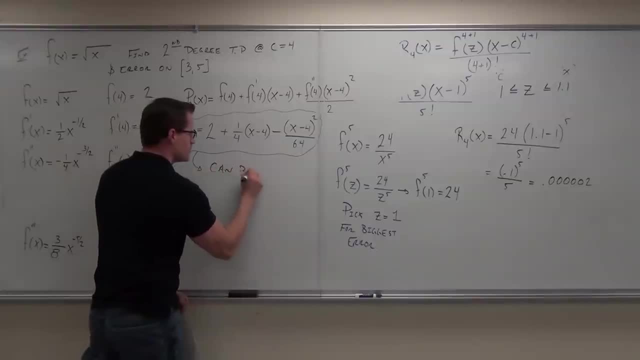 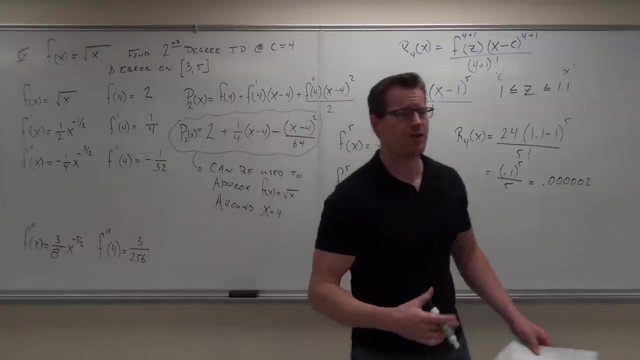 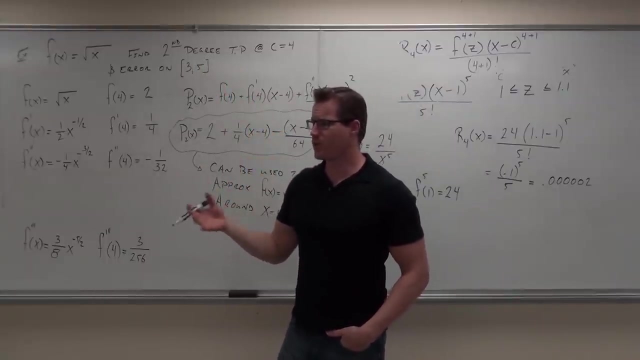 So this can be used to approximate our function around 4.. Okay, The next step is we're going to find the maximum error between numbers, so 4 times between 3 and 5.. So you're going to say this: I want to plug in 3.1, or I want to plug in 4.9,. 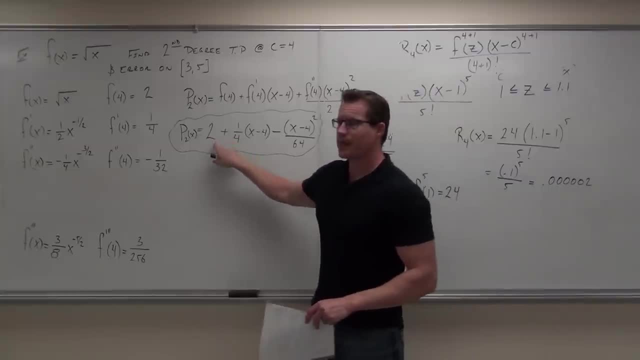 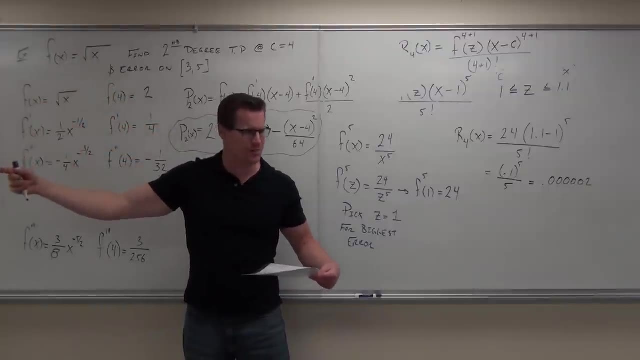 This can be used. here's the idea here. This Taylor polynomial can be used to approximate this function on anything around 4.. Does that make sense to you? Do I need to write that down for you? No, No, Okay, You sure? 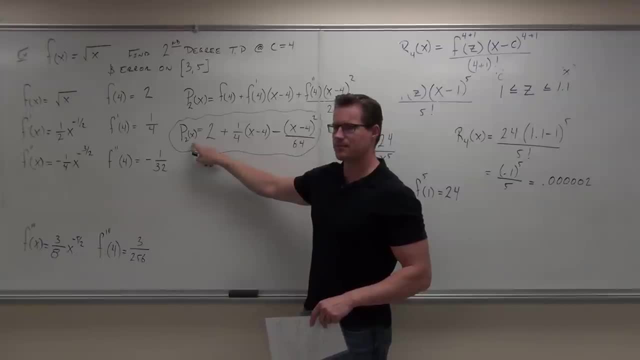 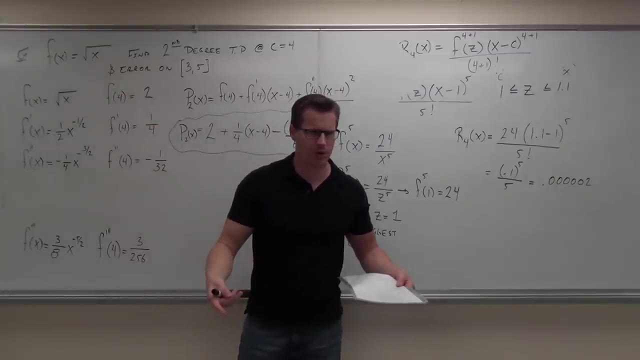 So you might want to write that down. This Taylor polynomial can be used to represent or approximate this function on anything around 4.. Why around 4? It's 4.. That's our center. Now what we're going to do is say: 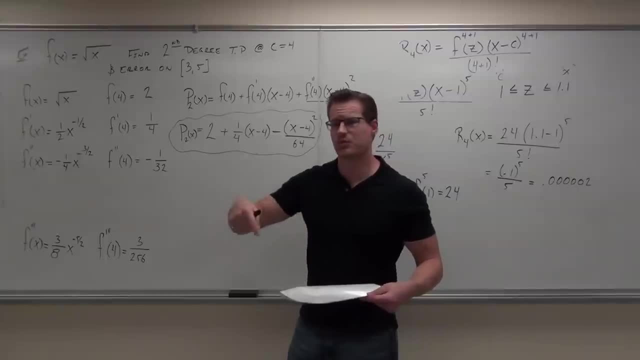 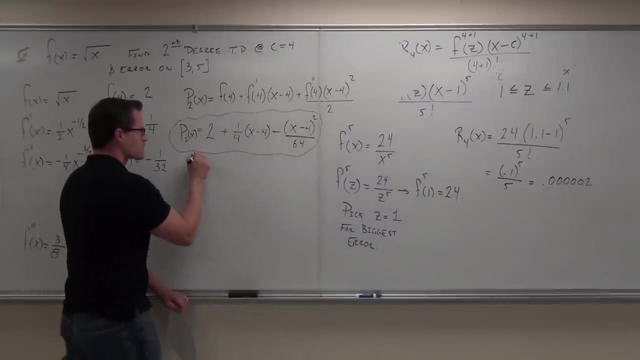 Imagine you used it to represent or approximate a number between 3 and 5.. We're going to find out the largest error after, probably next time we come back, So I'll write this out real quick and then we'll stop here, So this can be used to approximate our function around 4.. 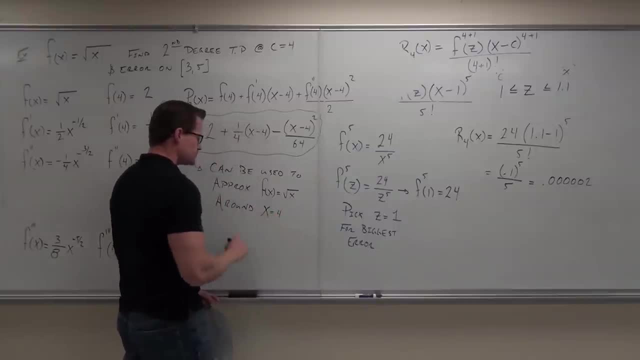 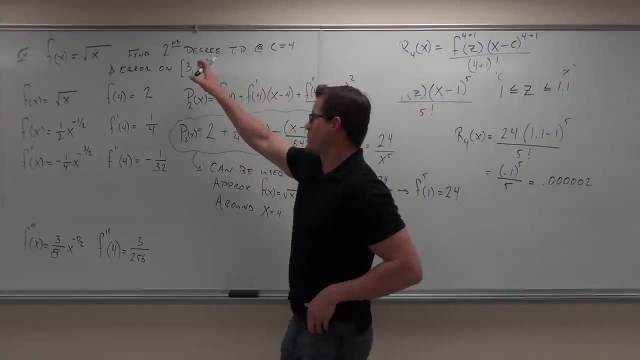 The next step is we're going to find the maximum error between numbers, so 4 times between 3 and 5.. So you're going to say this: I want to plug in 3.1. Or I want to plug in 4.9.. 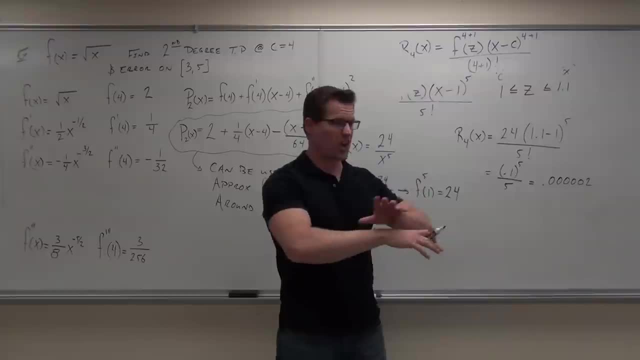 I want to plug in 5.. Whatever I want to plug in 3.. We're going to say, okay, Whatever number you want to plug in between 3 and 5, I'm going to tell you that this Taylor polynomial. 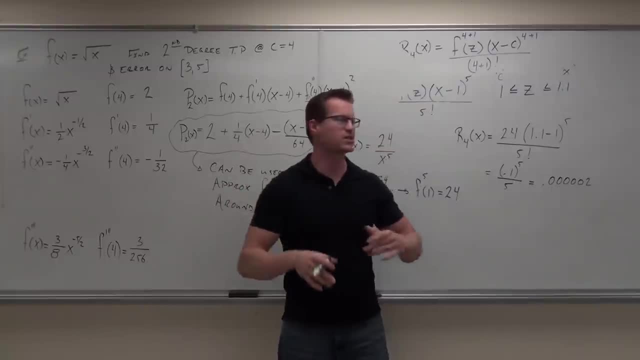 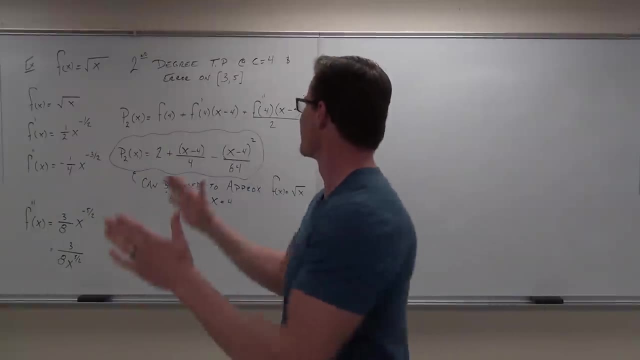 whatever you plug in is going to be within a certain range. It's going to be within a certain error. We'll do that next time. You're going to help me. Okay, So we're finding a Taylor polynomial of functions now. 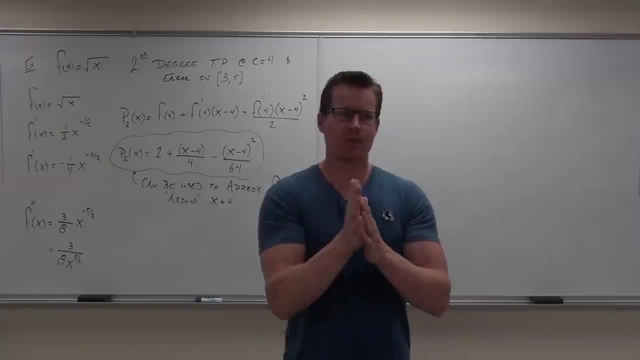 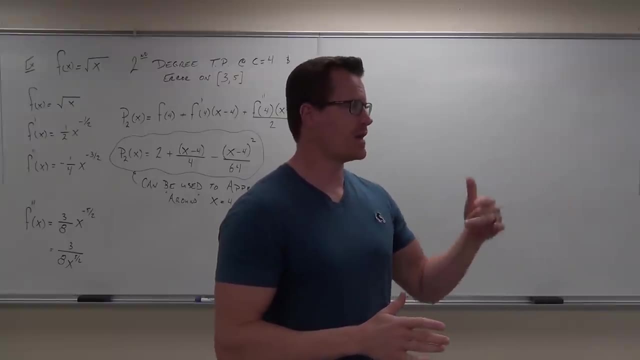 So the Taylor polynomial is part of the Taylor series. We stop at a certain degree. That means, if I want a degree 2, we're going to stop at the second derivative And that now becomes instead of the whole Taylor series, which perfectly represents our function: we're stopping. 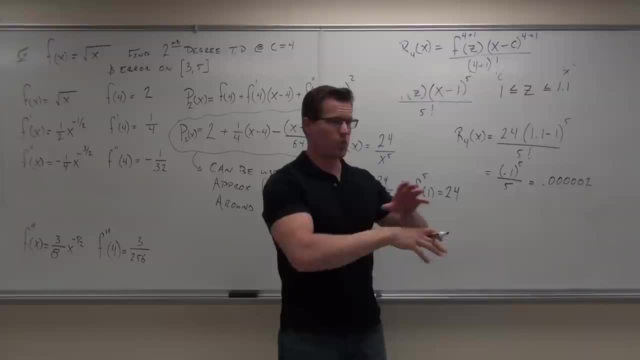 I want to plug in 5, whatever I want to plug in 3.. We're going to say, okay, whatever number you want to plug in between 3 and 5, I'm going to tell you that this Taylor polynomial, whatever you plug in. 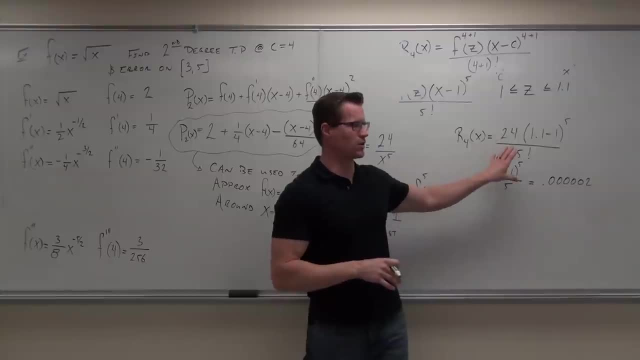 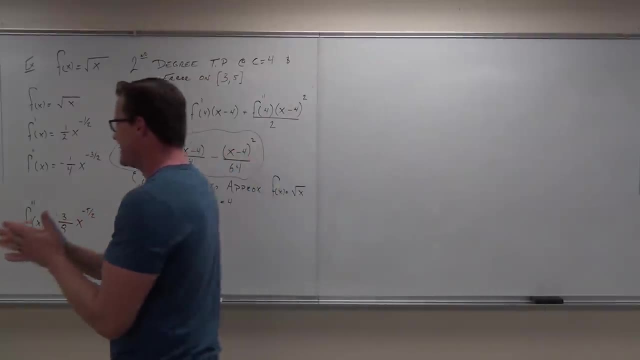 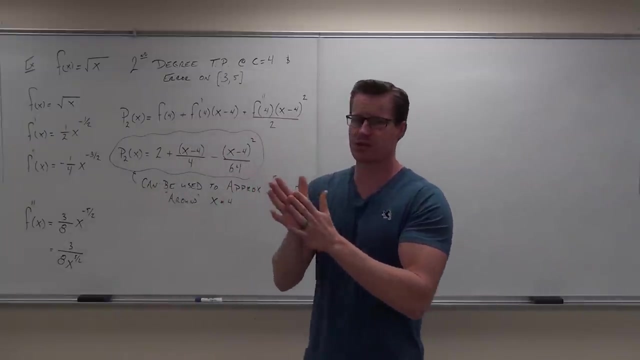 is going to be within a certain range. it's going to be within a certain error. We'll do that next time You're going to help me. Okay, so we're finding a Taylor polynomial of functions now, So the Taylor polynomial is part of the Taylor series. 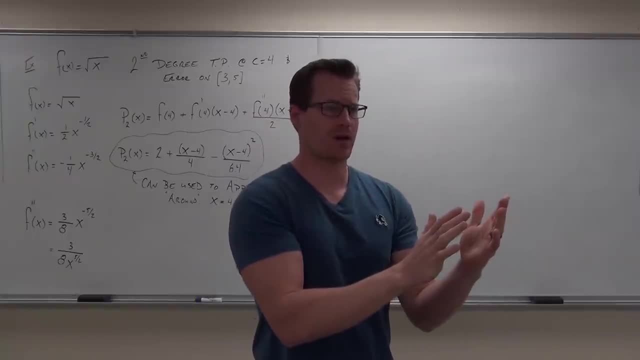 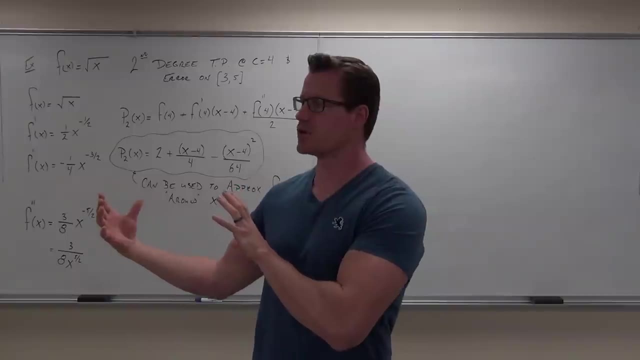 We stop at a certain degree. That means if I want a degree 2, we're going to stop at the second derivative and that now becomes instead of the whole Taylor series, which perfectly represents our function, we're stopping. That means it's an approximation. 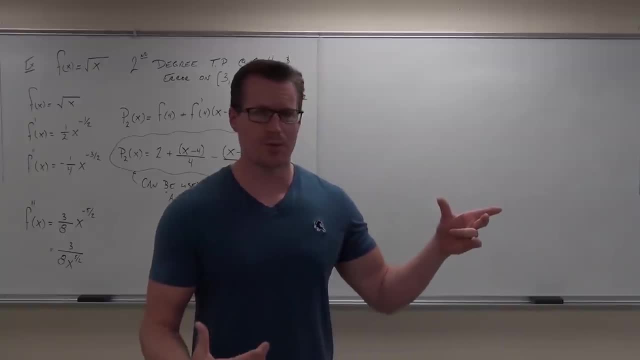 So it's a two-part idea. Find the approximation, the Taylor polynomial, then find the error. The error says: whatever you plug in, it's going to be within a certain range, It's going to be within this amount of what the actual function is at that point. 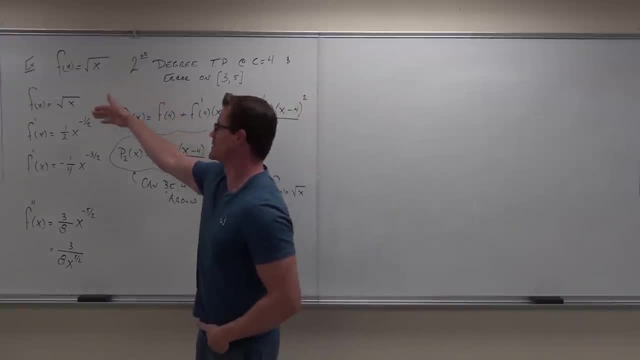 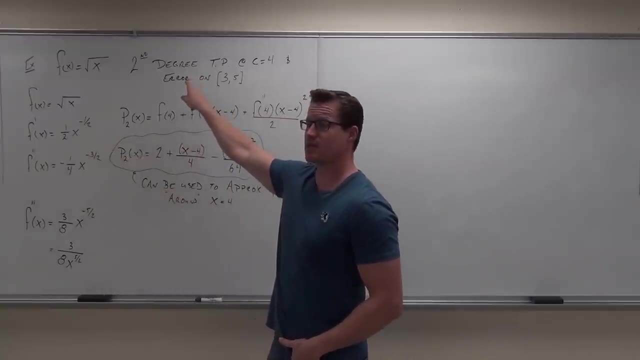 We've made it this far, We've done the Taylor series idea. We said, okay, here's our function: first derivative, second derivative. We always go one more derivative than the degree I'm asking you for, And the reason that we do that is because we use that next derivative in our error. 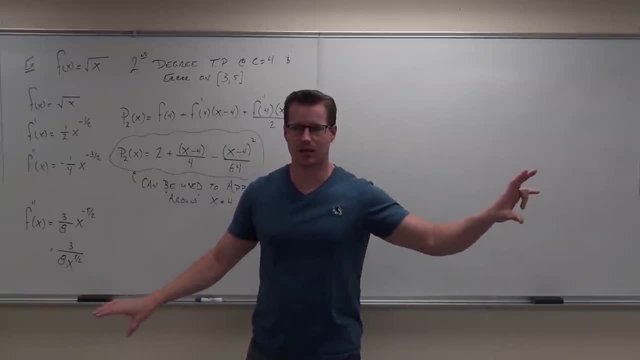 So the error is the next term, basically in a Taylor series. So what we say is: oh, a Taylor polynomial. We're stopping at the second degree. no problem, We have f of 4.. Why do we have a 4?? 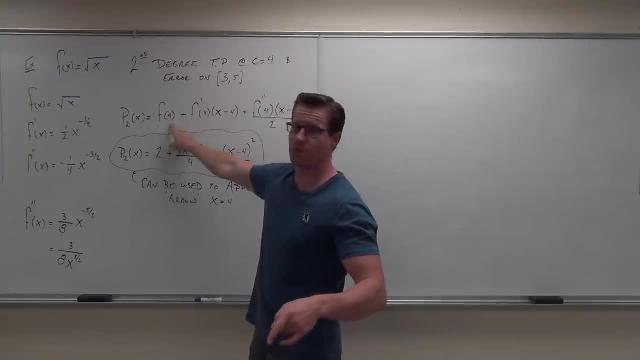 Where's that coming from? The degree of force, Not the degree of 4, but the c, the center of force. So we have 4.. Okay, first derivative of 4,, second derivative of 4,. no problem, Plug those things in, and this is where we got last time. 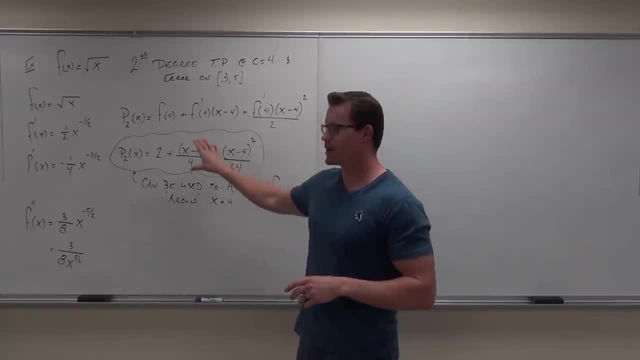 Got it, Yeah. Now what we need to know is that this thing right here, this is a Taylor polynomial of the second degree. what I'm asking you for. We have all of our numbers plugged in, except for our x. That's great. 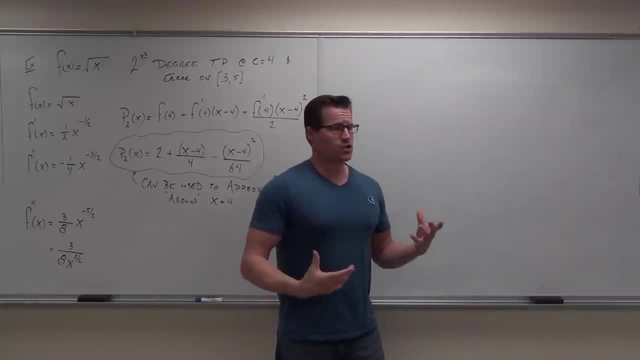 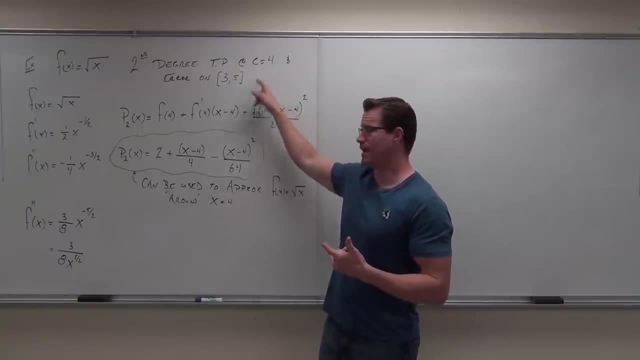 This can be used to represent our function or approximate our function at any number around 4.. Why around 4?? Because that's what I told you to center it at. That's what it is: x minus 4.. So what I said is okay. that can be used to approximate f of x around 4.. 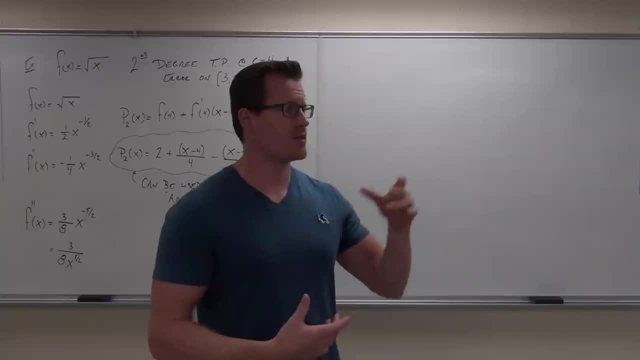 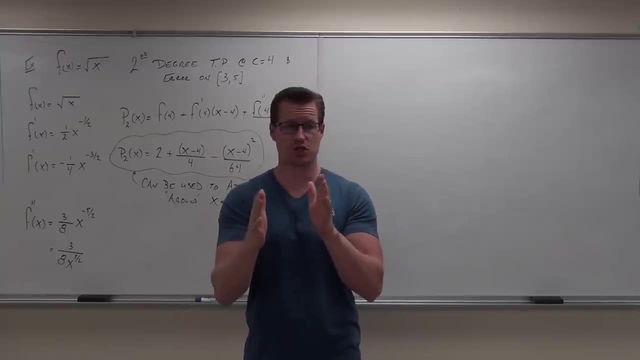 That means it's an approximation. So it's a two-part idea. Find the approximation, The Taylor polynomial, Then find the error. The error says: whatever you plug in, it's going to be within this amount of what the actual function is at that point. 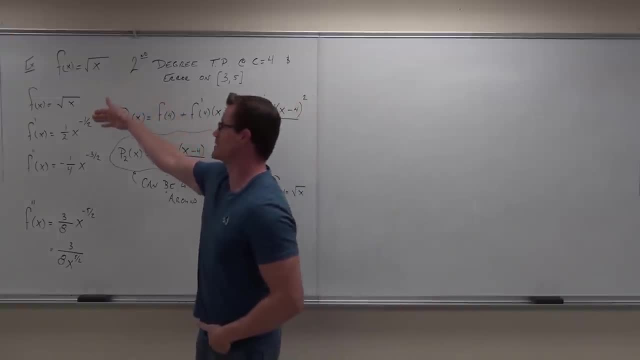 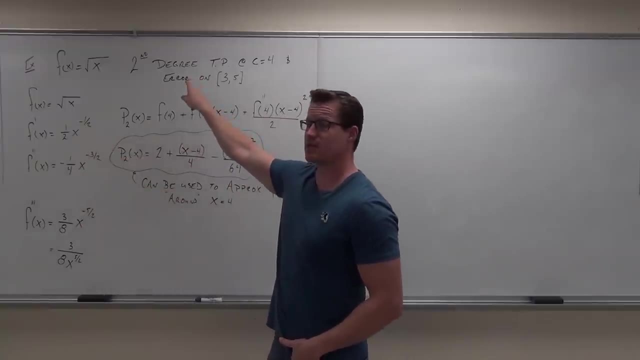 We've made it this far, We've done the Taylor series idea. We said, okay, here's our function: first derivative, second derivative. We always go one more derivative than the degree I'm asking you for, And the reason that we do that is because we use that next derivative in our error. 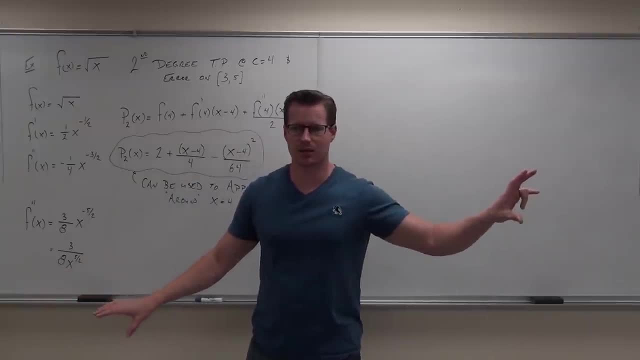 So the error is the next term, basically in a Taylor series. So what we say is: oh, a Taylor polynomial. We're stopping at the second derivative. No problem, We have f of 4.. Why do we have a 4?? 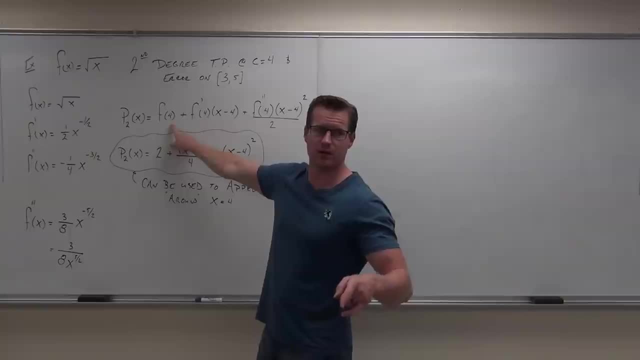 Where's that coming from? Not the degree of 4, but the C, the center of 4.. So we have 4.. Okay, first derivative of 4, second derivative of 4.. No problem, Plug those things in, and this is where we got last time. 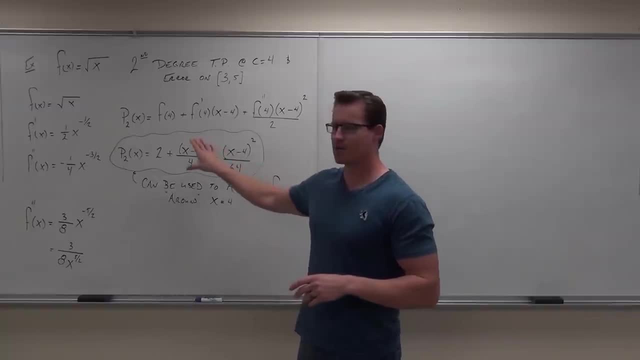 Got it. Now what we need to know is that this thing right here, this is the Taylor polynomial of the second degree. what I'm asking you for. We have all of our numbers plugged in, except for our x. That's great. 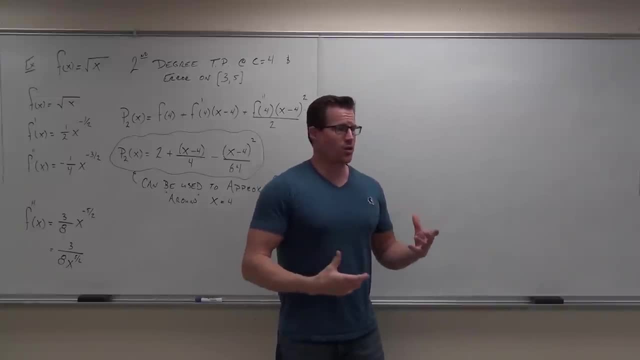 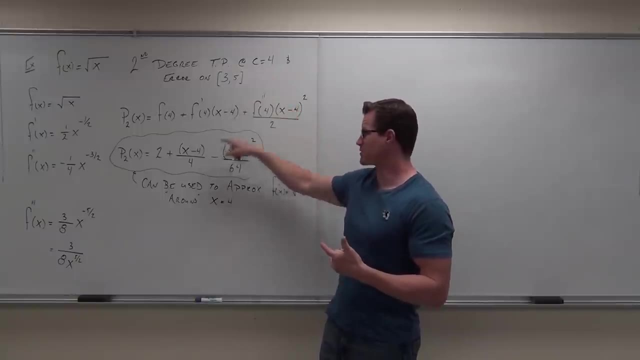 This can be used to represent our function Or approximate our function at any number around 4.. Why around 4?? Because that's what I told you to center it at. That's what it is: x minus 4.. So what I said is okay. that can be used to approximate f of x around 4.. 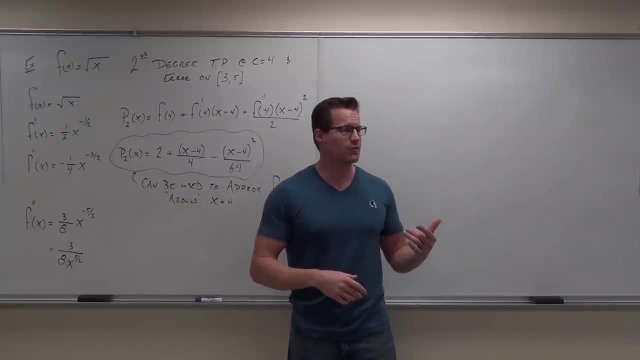 What's the maximum error that we will have if we plug in the numbers from 3 to 5?? So if we plug in like 3.01, if we plug in 4.2 or 5, point whatever, what's the biggest error that we could even get? 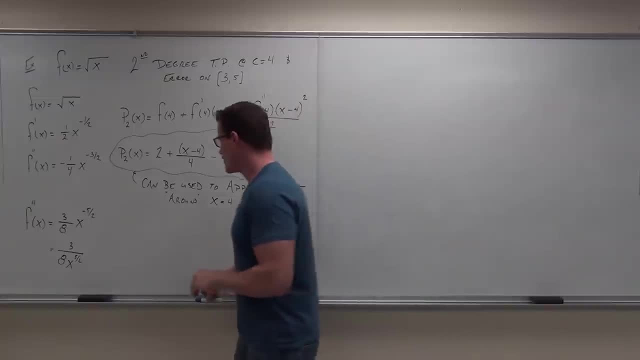 And that's the idea of the next thing that we're going to do, So we don't end with our approximation. This is actually really, really easy to get. All you've got to know how to do is do a few simple derivatives and know the formula. 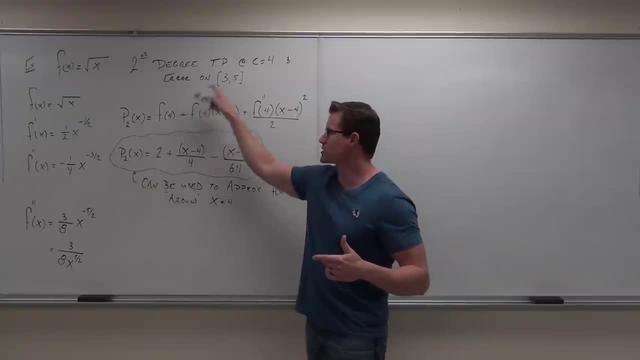 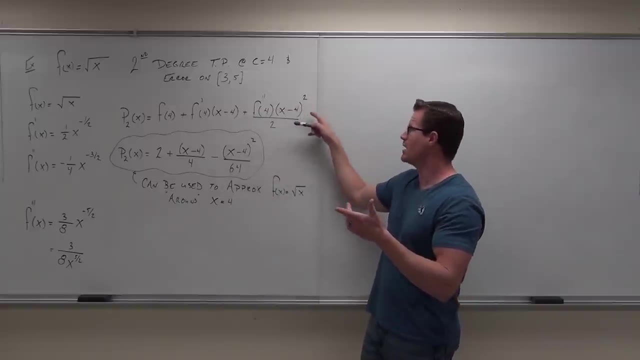 The formula is a piece of cake. It's the function at whatever your center is The first derivative at your center, and then x minus 4.. The second derivative at your center, x minus 4 to the second over 2.. And the next one would be x minus 4 to the third over 3, factorial, and so on, and so on and so on, until you reach the degree I want. 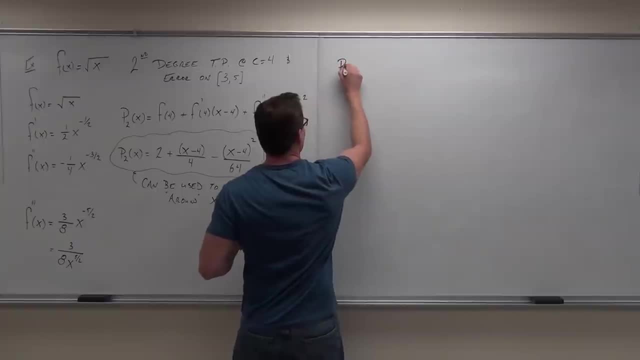 Now the error. the error of the sorry. it should be a. 2. The error of a second degree Taylor polynomial says: alright, you're going to start with the next derivative. So if I have a second degree Taylor polynomial, the error- the remainder of that starts at the third derivative. 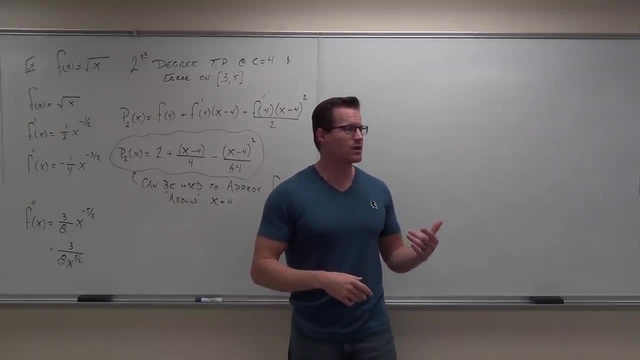 What's the maximum error that we will have if we plug in the numbers from 3 to 5?? So if we plug in like 3.01, if we plug in 4.2 or 5, point whatever, what's the biggest error that we could even get? 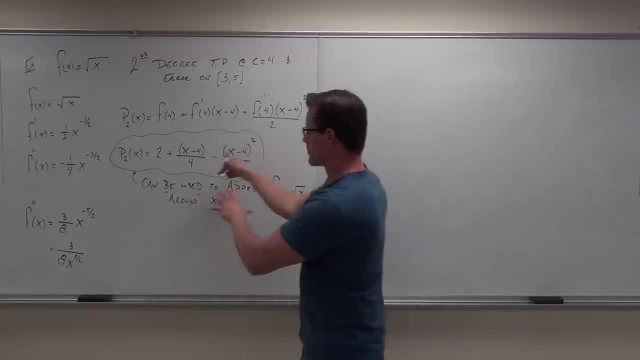 And that's the idea of the next thing that we're going to do, So we don't end with our approximation. This is actually really, really easy to get. All you've got to know how to do is do a few simple derivatives and know the formula. 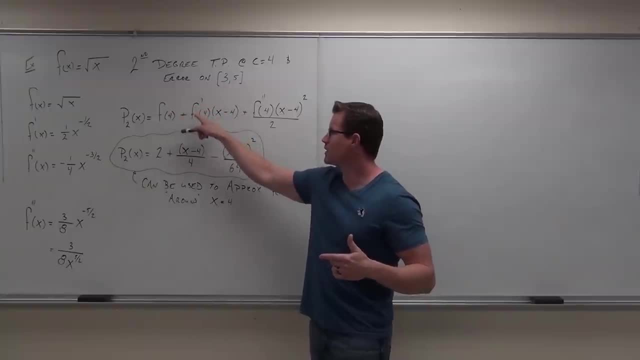 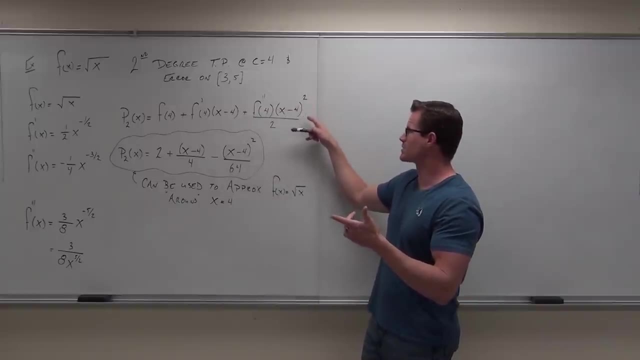 The formula is a piece of cake. It's the function at whatever your center is The first derivative at your center, and then x minus 4.. The second derivative at your center, x minus 4 to the second over 2.. And the next one would be x minus 4 to the third over 3, factorial, and so on, and so on, and so on. 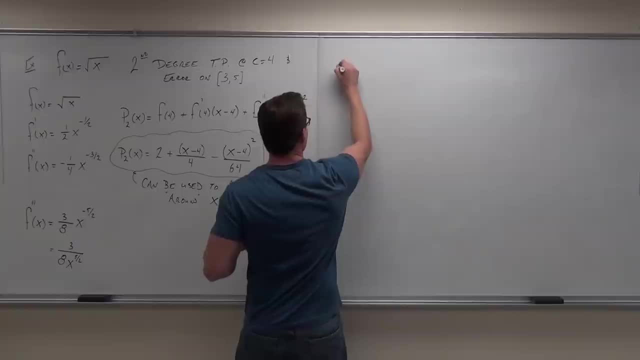 until you reach the degree I want. Now the error of a second degree Taylor polynomial says: all right, you're going to start with the next derivative. So if I have a second degree Taylor polynomial, the error- the remainder of that- starts at the third derivative. 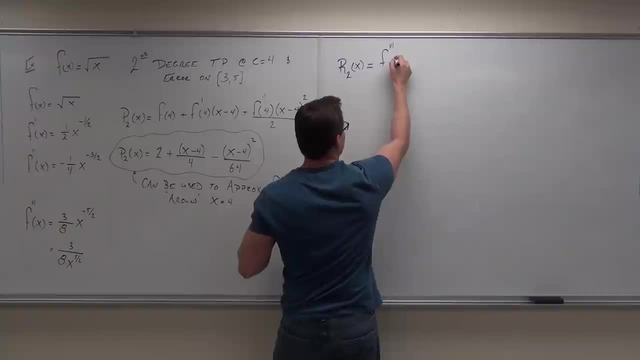 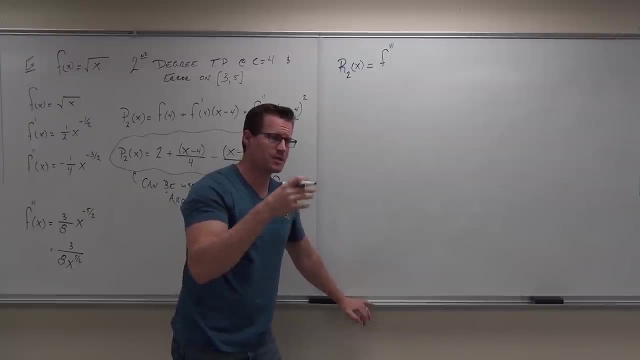 That's why we go ahead and find that, because we're going to be using it. Starts at the third derivative of: is it an x? It's a z. Z is some number between c and x, So between c, the center, and some number that you are approximating. Okay, All right. So that's what we're going to do. All right, Now we're going to start with the next derivative. So if I have a second degree Taylor polynomial, the error- the remainder of that- starts at the third derivative. 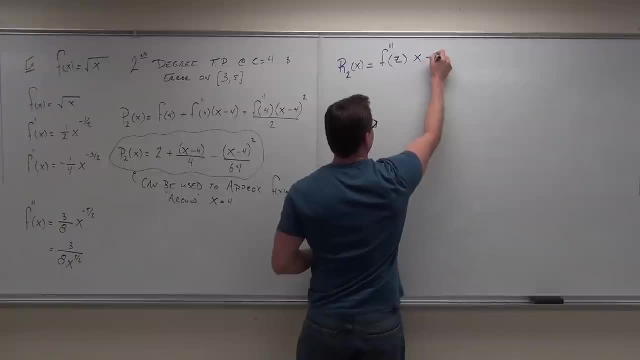 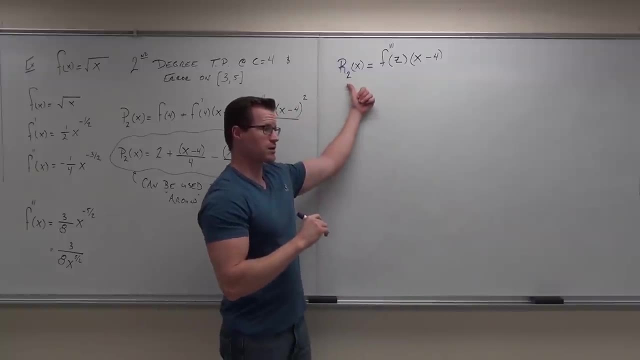 We're going to talk about that in a minute. Then I'm going to have x minus 4, no problem to the Your degree's 2, correct? That means that your remainder's going to have a power of 3 to it. 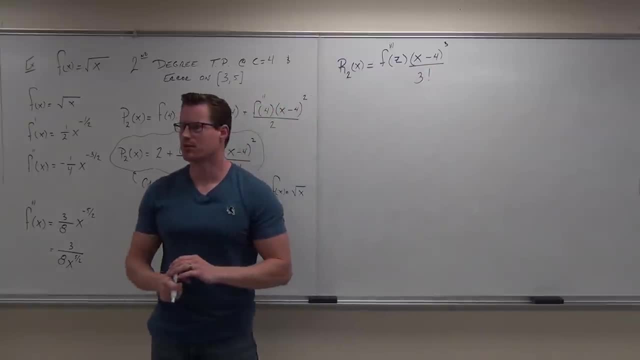 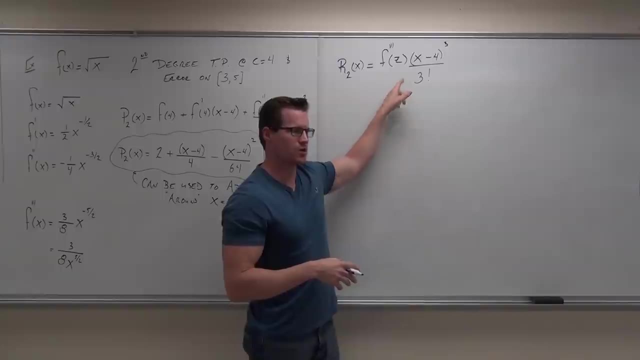 Over 3 factorial. Those things match Quick head note, if you're okay with that so far. Okay, let's go back and look over here, because right now I don't know the number I have to plug in here, So I'm not going to plug in 3.. 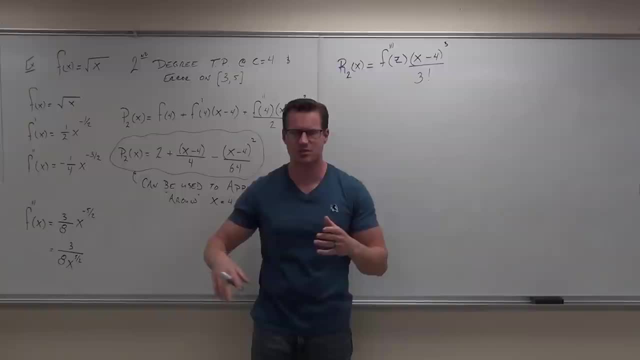 I'm not going to plug in 4.. I'm going to plug in 5.. I think I did that last time just to give you an exercise, but we're not actually going to do that. We're going to be smarter about this, because what we're trying to find out is what the 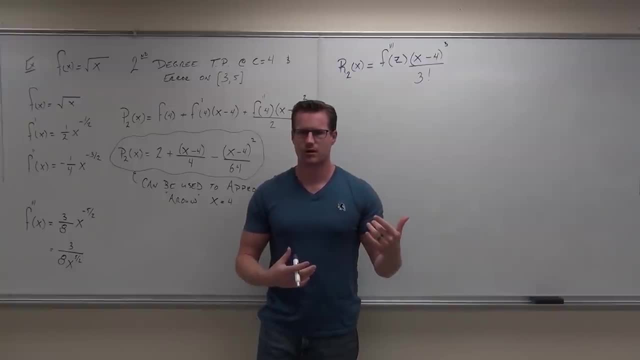 smallest possible error or the largest possible error. Largest- Yeah, the largest, The smallest would be. well, if you plugged in 4, exactly, you'd get the smallest error. But if you plug in anything outside of that, naturally you're going to get an error. 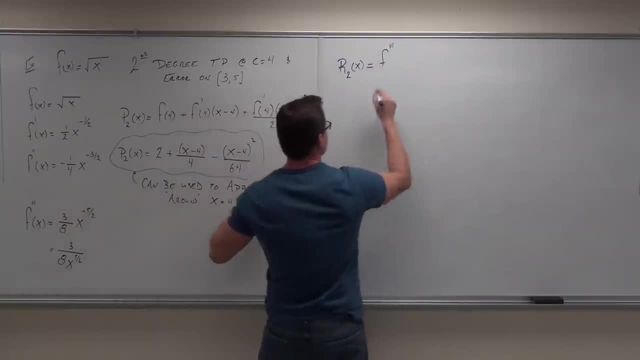 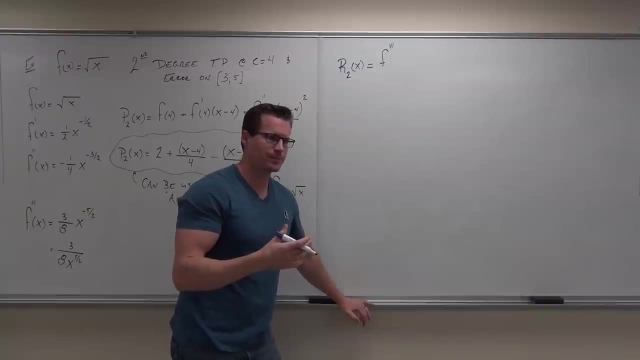 That's why we go ahead and find that, because we're going to be using it. It starts at the third derivative of: is it an x? It's a z. Z is some number between c and x. Okay, So between c, the center, and some number that you are approximating. 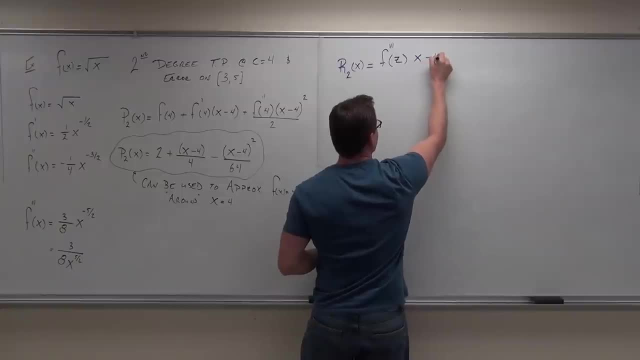 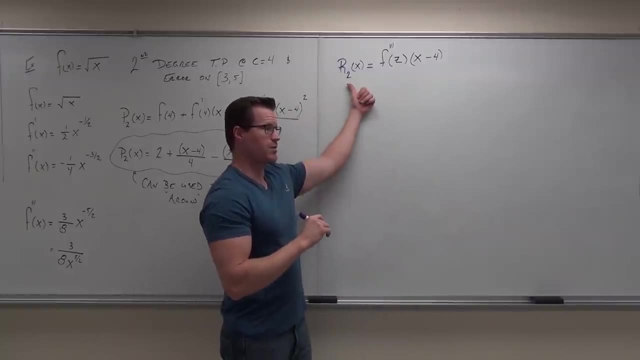 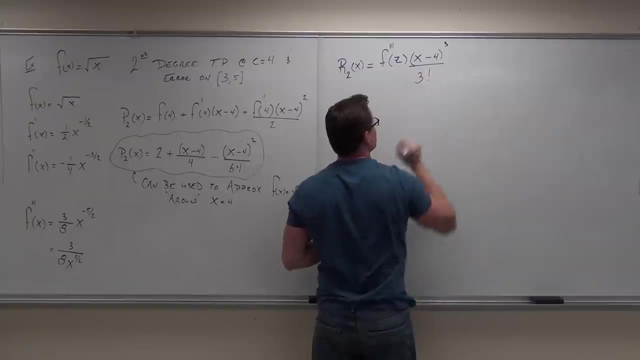 We're going to talk about that in a minute. Then I'm going to have x minus 4, no problem. to the to the. your degree is 2, correct? Yes, That means that your remainder is going to have a power of 3 to it over 3 factorial. 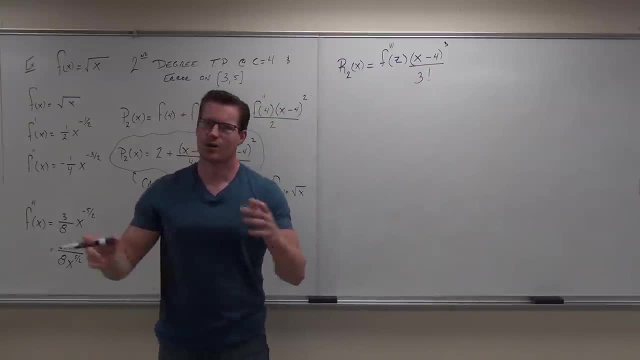 Those things match. Click here now. if you're okay with that so far, Let's go back and look over here, because right now I don't know the number I have to plug in here, So I'm not going to plug in 3.. 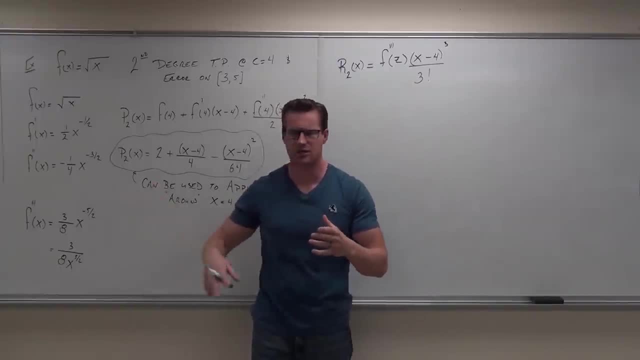 I'm not going to plug in 4.. I'm not going to plug in 5.. I think I did that last time, just to give you an exercise, But we're not actually going to do that. We're going to be smarter about this, because what we're trying to find out is what the smallest possible error or the largest possible error 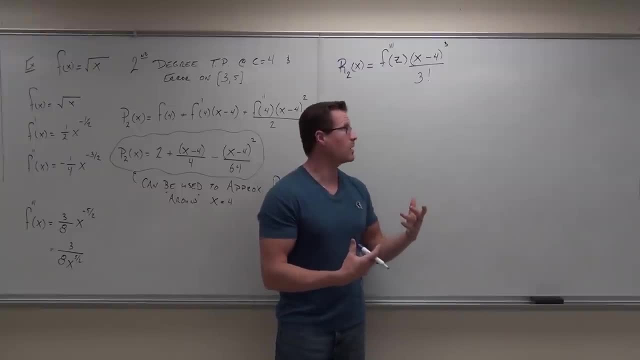 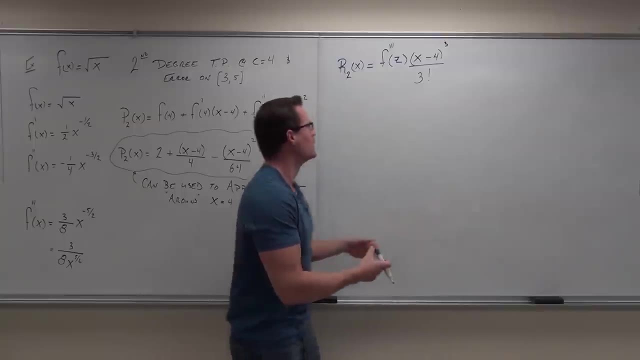 Largest, Yeah, the largest, The smallest would be well, if you plugged in 4 exactly, You'd get the smallest error. But if you plug in anything outside of that, then actually we're going to get an error. So what we're going to do is go back over here and say: all right, if this is our third derivative of f at x. 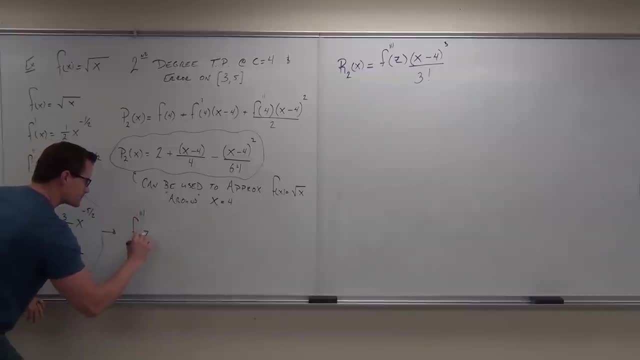 then what that means is our third derivative of f at z would simply be this same thing with a z instead of an x. Does that make sense to you? Hello, you with me, guys? Yes, Okay, so this says all right. well, the only reason why we did this third derivative was now for our error. 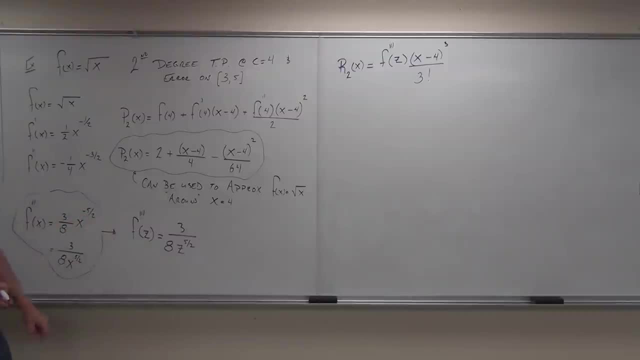 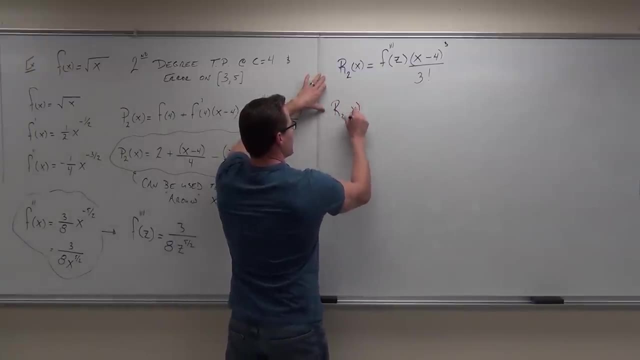 That's why we're using our Taylor polynomial. Well, now let's make a little substitution. So if I know that the third derivative of f at z gives us this thing, then I can translate this to the remainder of the error of the degree 2 Taylor polynomial is: 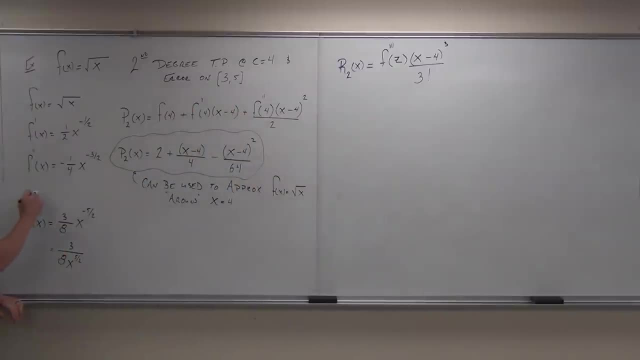 So what we're going to do is go back over here and say, all right, if this is our third derivative of f at x, Now what that means is our third derivative of f at z would simply be the same thing with a z instead of an x. 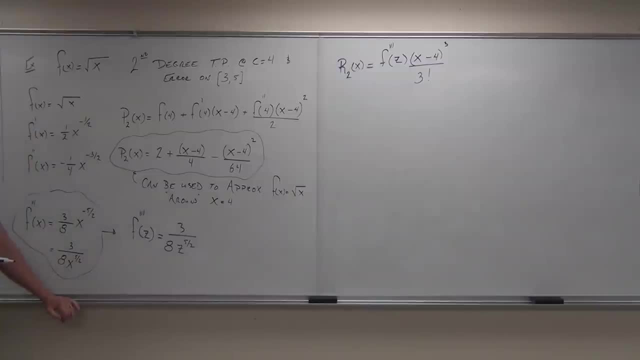 Does that make sense to you? Hello you with me guys? Yes, Okay, so this is all right. well, the only reason why we did this third derivative was now. for error, We didn't use it in our Taylor polynomial. 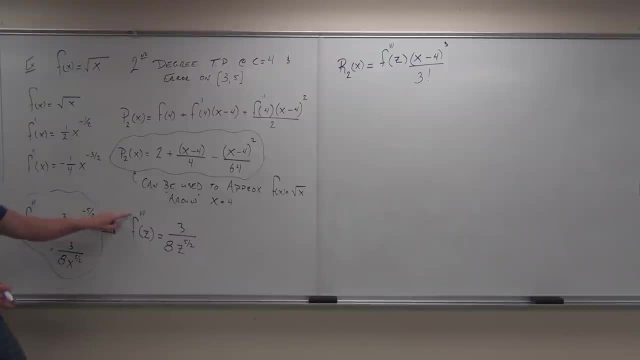 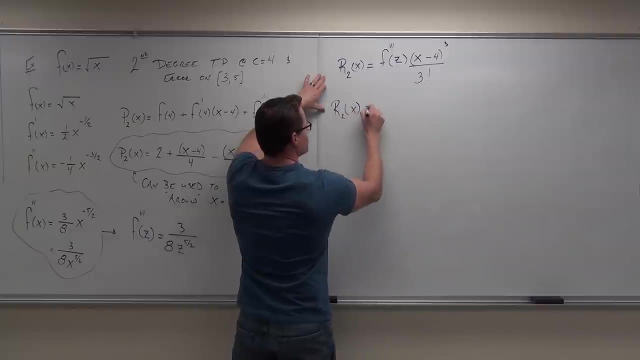 Well, now let's make a little substitution. So if I know that the third derivative of f at z gives us this thing, then I can translate this to the remainder of the error at of the degree 2 polynomial. Taylor polynomial is instead of the third derivative of z. I'm just going to put this. I'm going to put 3. 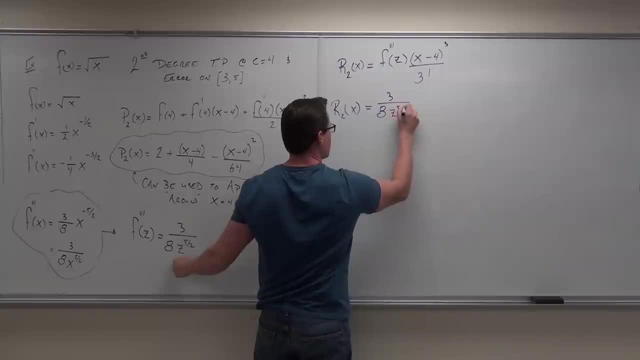 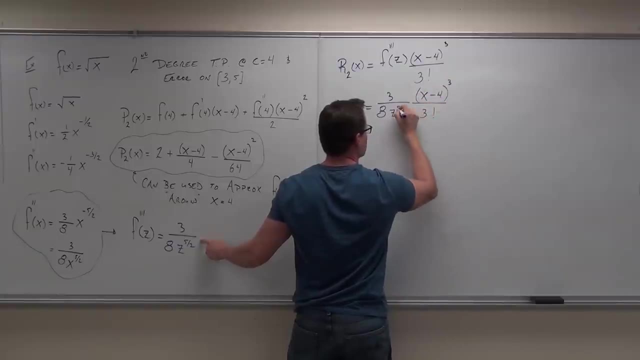 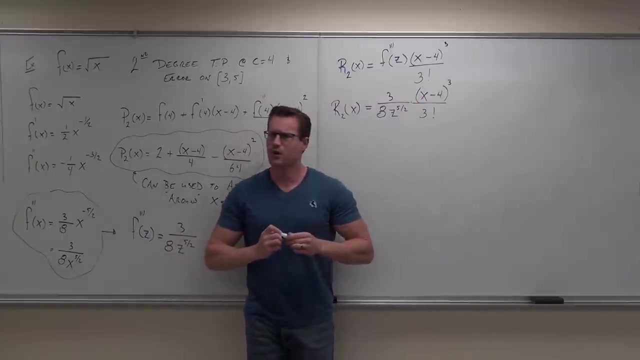 over 8 z to the 5 halves times x minus 4 to the third over 3 factorial. no problem, Quick show of hands if you feel. okay getting that far. show of hands if you do. We already talked about the formula for the error. the remainder: 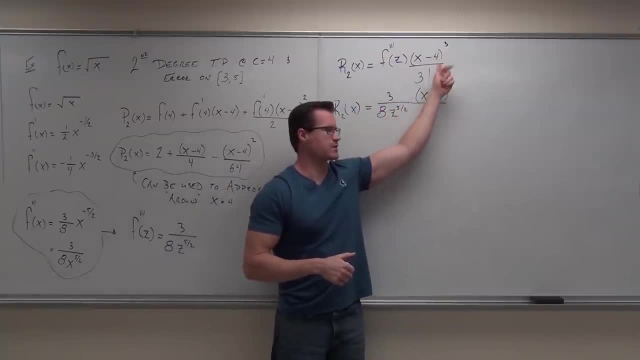 It's just the next derivative, the next degree over the same same thing. Degree matches your, your factorial Cool deal. Well, we've gone ahead and said: well, you know what The degree 3 remainder is going to have? a third derivative of f. 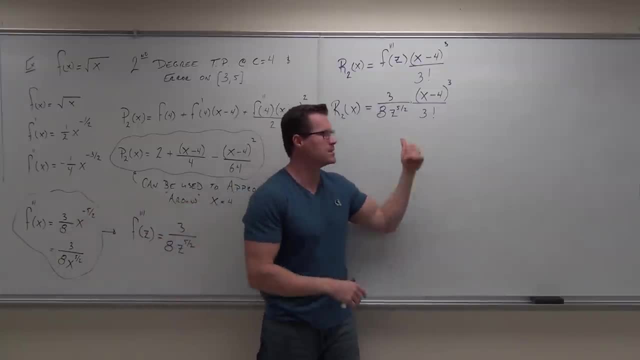 We've already done that. This was an x, You just plug in z, not a big deal. Now is where you do something that's kind of important: to find your, your error, your maximum error. You pick the numbers that are going to make your error the biggest. 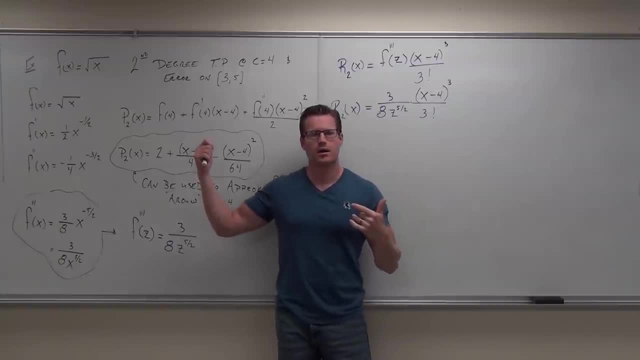 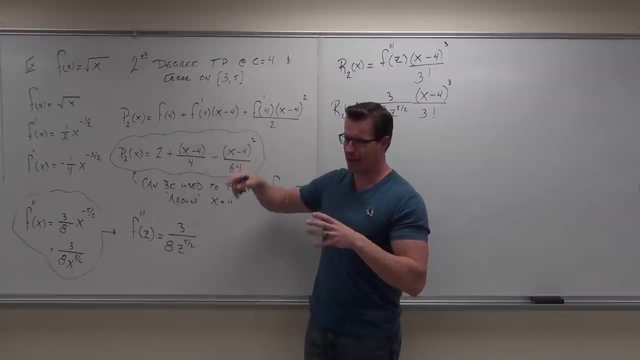 Okay, So look back over here. We have centered at 4, very good, but we're on the interval from 3 to 5.. Now your x is going to be some number between 3 and 5.. You're going to pick the x that gives you the biggest error here. 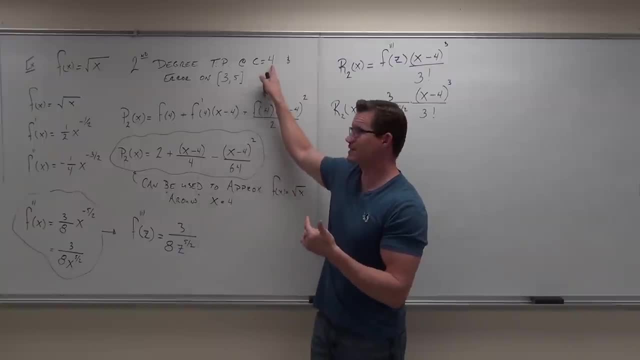 Your z is going to be some number between 4, somewhere in here, somewhere between 4 and your x. Now, keep in mind, your x ranges from 3 to 5. So you can pick x between 3 and 5. And you can pick z. 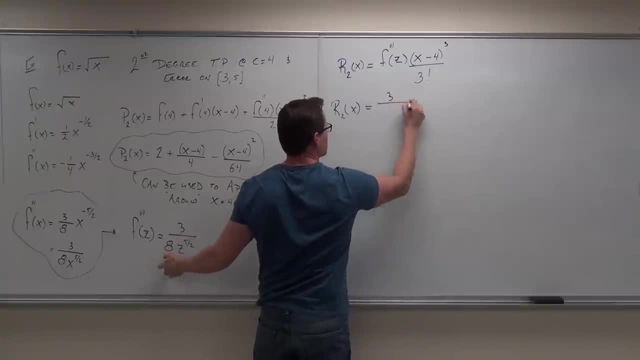 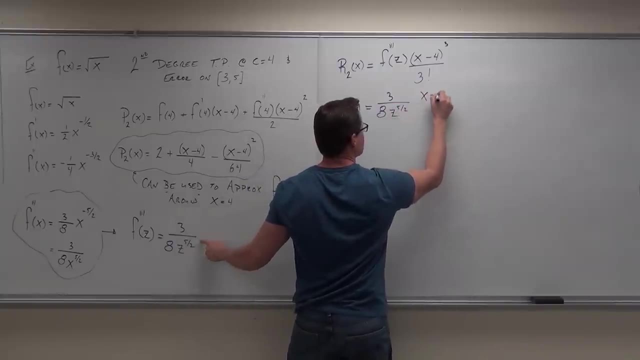 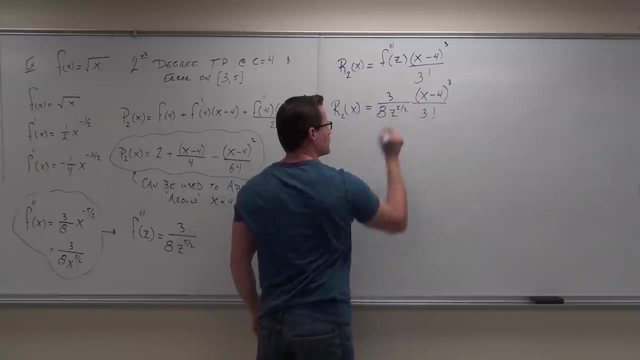 instead of the third derivative of z. I'm just going to put this: I'm going to put 3 over 8, z to the 5 halves times x minus 4 to the third over 3 factorial. No problem, Quick show of hands if you feel. okay getting that far. 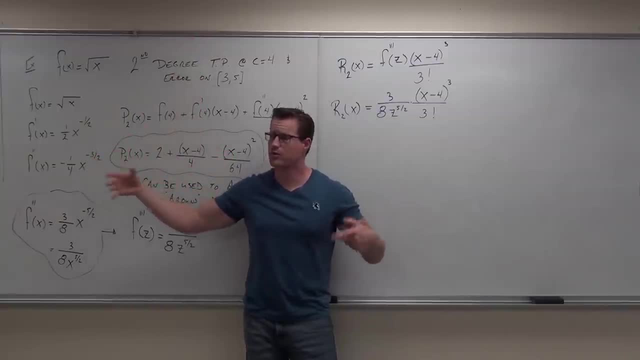 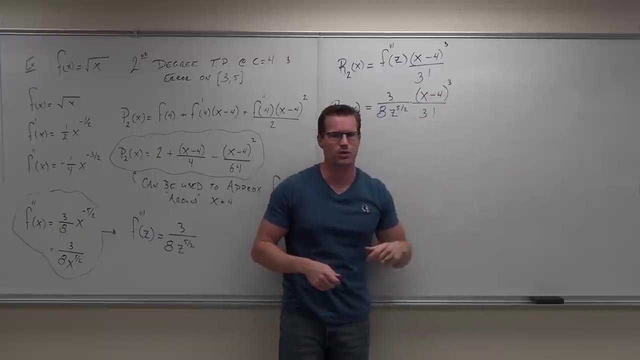 Show of hands if you do. We already talked about the formula for the error. the remainder, It's just the next derivative, the next degree over the same thing. Degree matches your factorial Cool deal. Well, we've gone ahead and said: well, you know what? 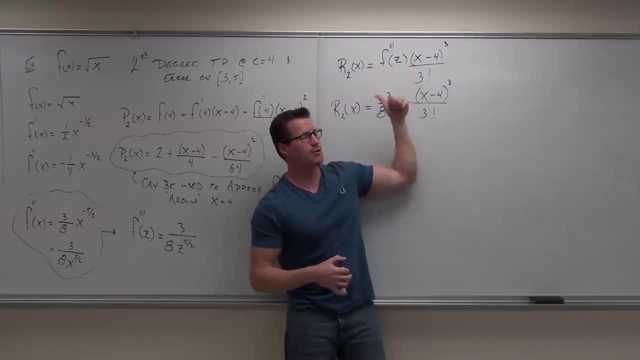 The degree 3 remainder is going to have a third derivative of f. We've already done that. This was an x, You just plug in z, Not a big deal. Now is where you do something that's kind of important: to find your error, your maximum error. 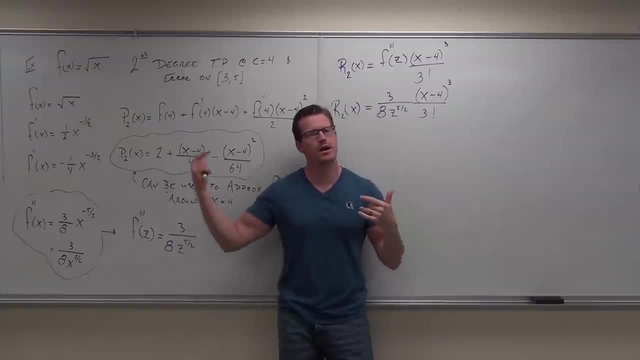 You pick the numbers that are going to make your error the biggest. So look back over. here We have centered at 4.. Very good, But we're on the interval from 3 to 5.. Now your x is going to be some number between 3 and 5.. 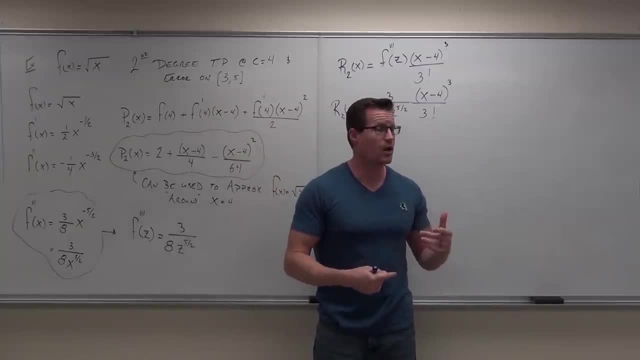 You're going to pick the x. that gives you the biggest error here. Your z is going to be some number between 4.. It's somewhere in here. 4 and your x. Now, keep in mind your x ranges from 3 to 5.. 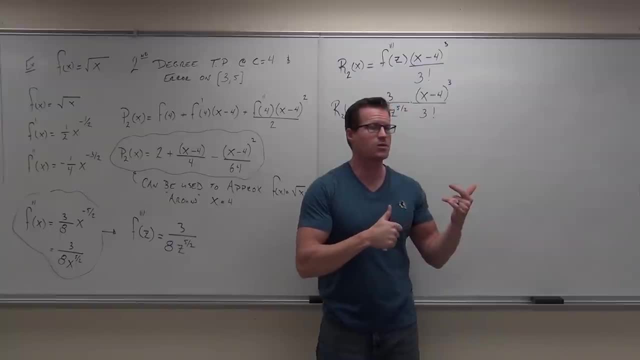 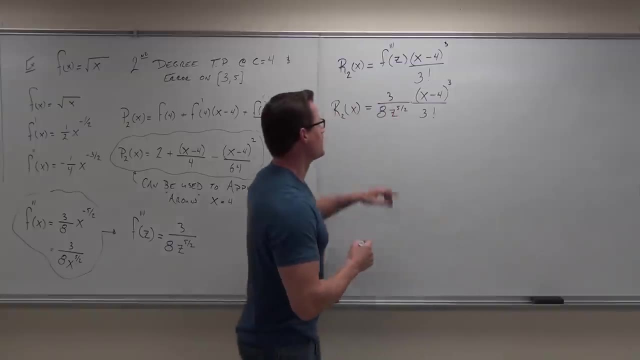 So you can pick x between 3 and 5 and you can pick z between 3 and 5.. Pick them so that your error becomes the biggest. Here's what I mean by that: Your x in order to make this the biggest, because, hey, this is centered at 4, right. 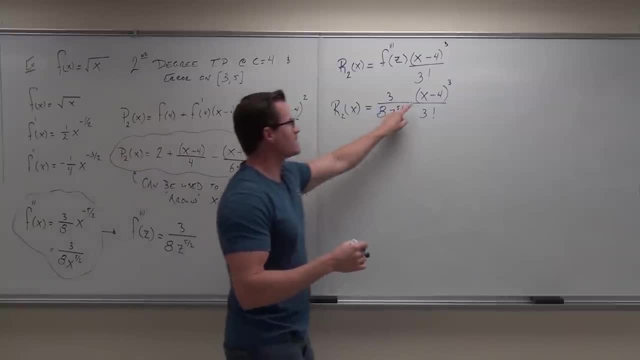 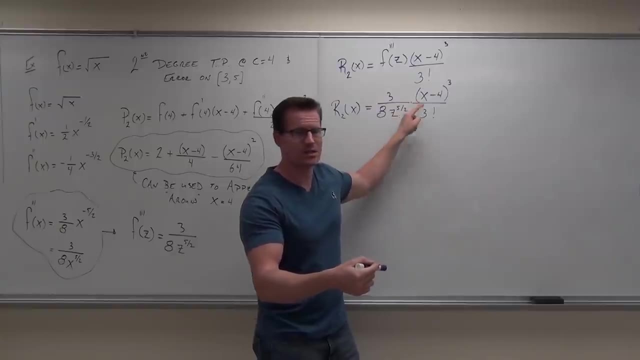 That's right in the center of your interval. It doesn't matter what your x is. Your x can be 3 or your x can be 5. You don't pick anything between there, because that's going to give you a smaller difference. 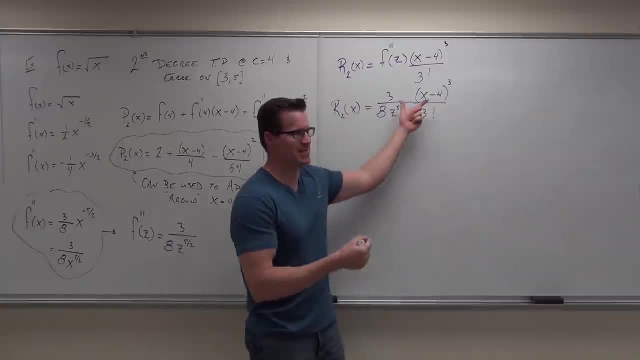 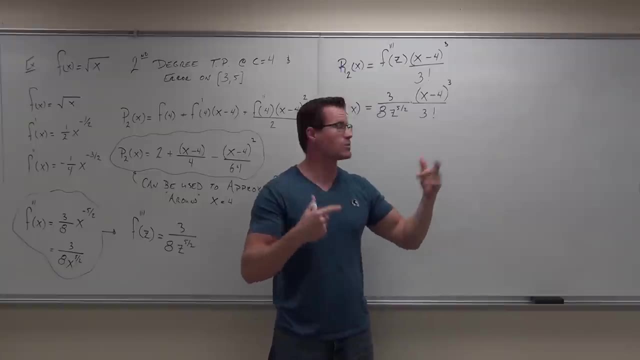 Does that make sense to you? You picked 4.01.. I mean, yeah, your error's going to be very little because it's only going to be .01.. Pick your end point, either 3 or 5.. Pick it so that this difference is the largest, okay. 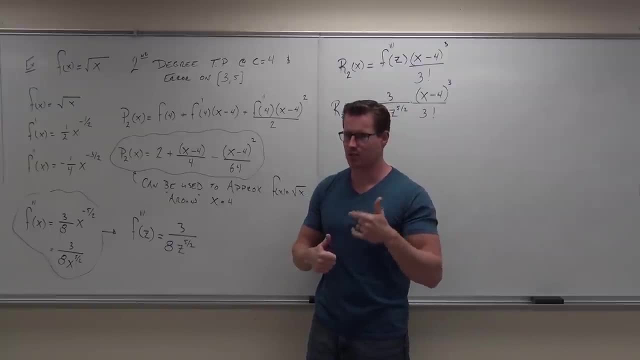 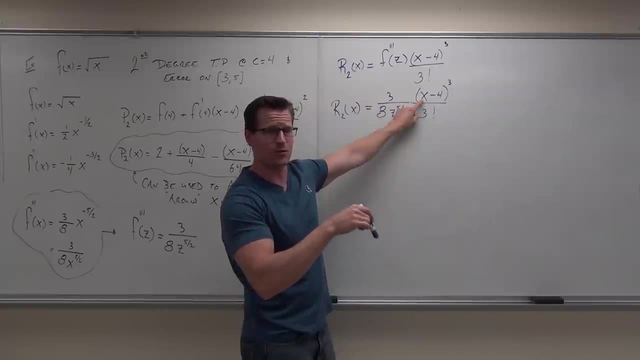 You can pick z between 3 and 5.. Pick them so that your error becomes the biggest. Here's what I mean by that: Your x in order to make this the biggest. because, hey, this is centered at 4, right. 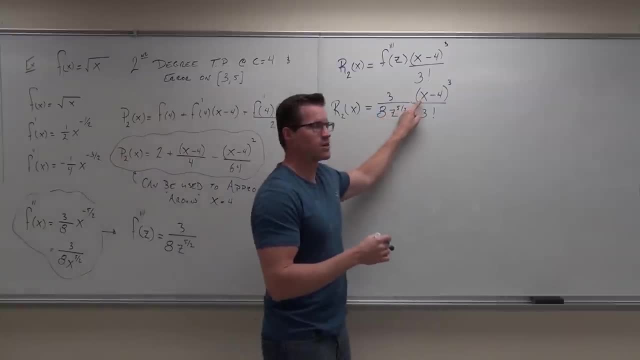 That's right in the center of your interval. It doesn't matter what your x is. Your x can be 3 or your x can be 5.. Don't pick anything between there, because that's going to give you a smaller difference. Does that make sense to you? 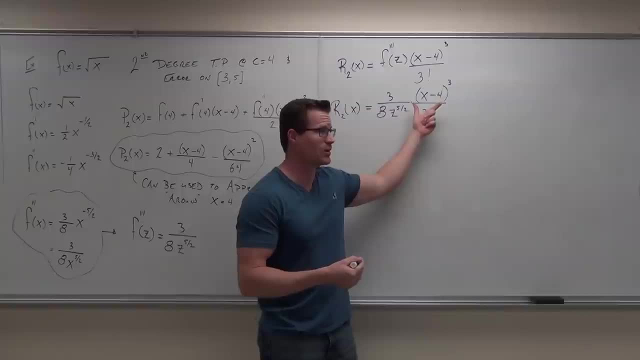 You picked 4.01.. Yeah, I mean, yeah, your error's going to be very little because it's only going to be 0.01.. Pick your end point: either 3 or 5.. Pick it so that this difference is the largest, OK. 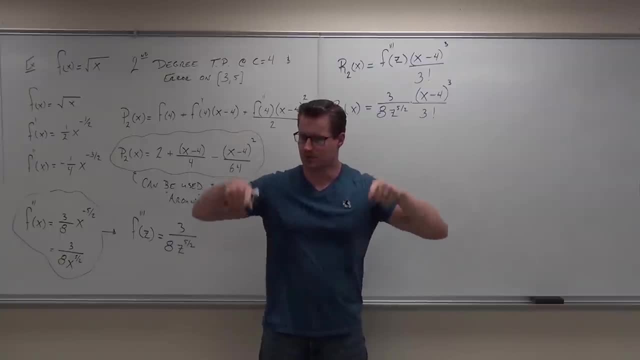 Now if you pick 3, you're going to get negative 1.. Put an absolute value around your remainder to make it positive, So you can do that. So if I pick x equals 3, that's fine, You know. say you get negative 1 out of that. 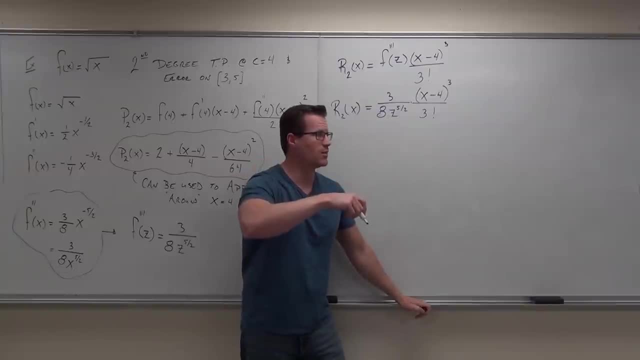 Negative 1 to the third, so it'll be negative 1.. Just take your absolute value, Your error. if you get a negative, it doesn't really matter, because all your error is saying is that your answer's going to be within this amount. 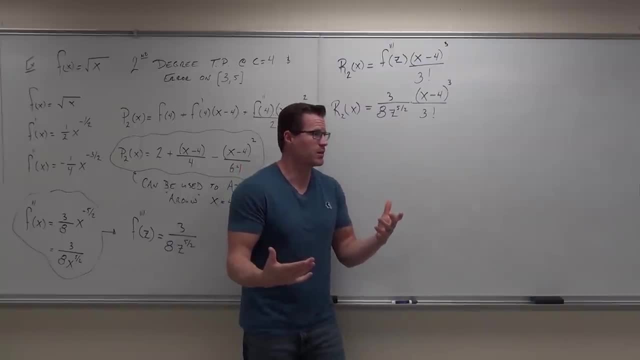 That within this amount's kind of like a measurement, It's like an absolute value anyway. So if you want to keep it positive, cool, Pick the 5.. If you want to- if you don't care about it, do absolute value, pick the 3.. 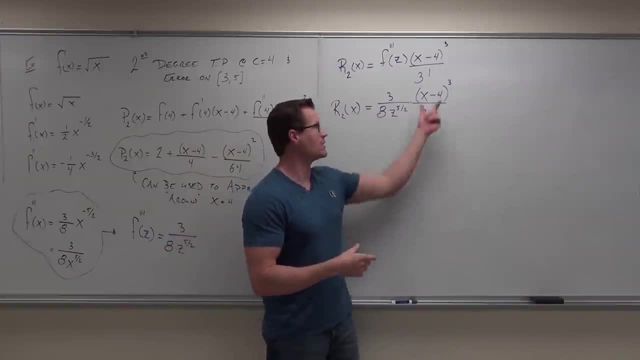 What I'm trying to tell you is that pick the end point if there exists one that gives you the maximum distance here. Not too bad, if you understand that idea. I'm going to pick the 5, just to show you that the x does not have to be the same as the. 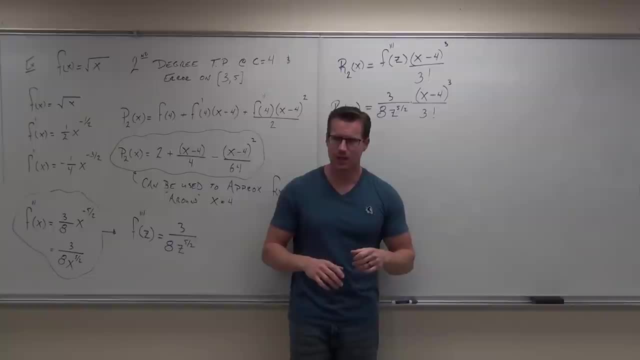 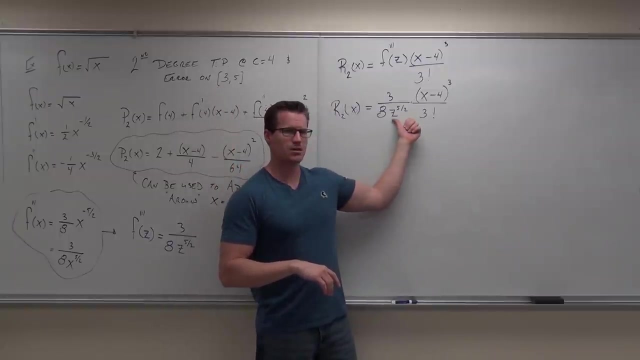 z. I'm going to pick the 5 for the x, Now the z. You need to pick one of these numbers in here that gives you the biggest, The biggest error possible. If I picked 5 for my z, would it be the biggest error or the smallest error? 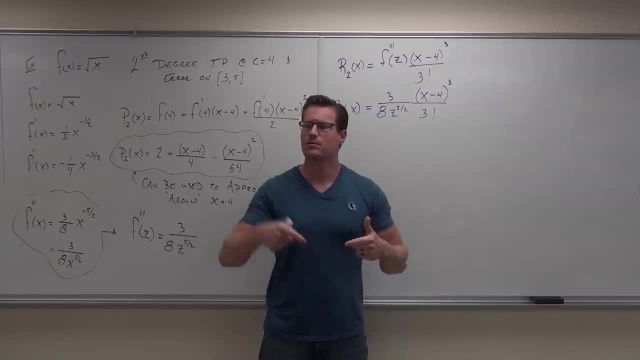 Now, if you pick 3, you're going to get negative 1.. Put an absolute value around your remainder to make it positive, So you can do that. So if I pick x equals 3, that's fine. You notice how you get negative 1 out of that. 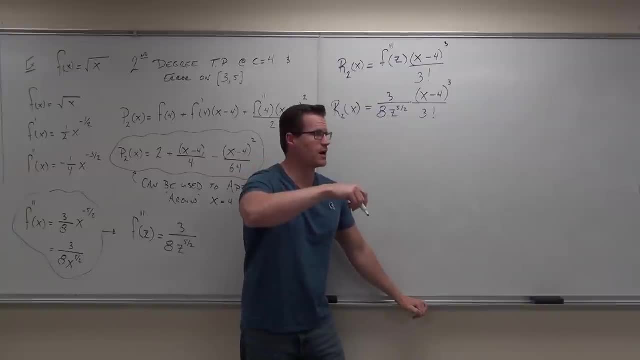 Negative 1 to the third. The third will still be negative 1.. Just take your absolute value, Your error: if you get a negative, it doesn't really matter, because all your error is saying is that your answer is going to be within this amount. 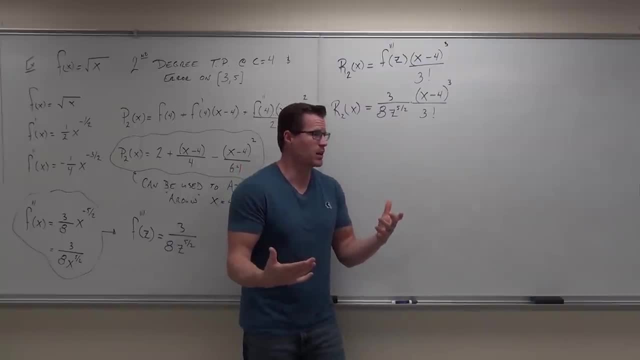 That within this amount is kind of like a measurement. It's like an absolute value anyway. So if you want to keep it positive, cool, Pick the 5.. If you don't care about it, do absolute value, Pick the 3.. 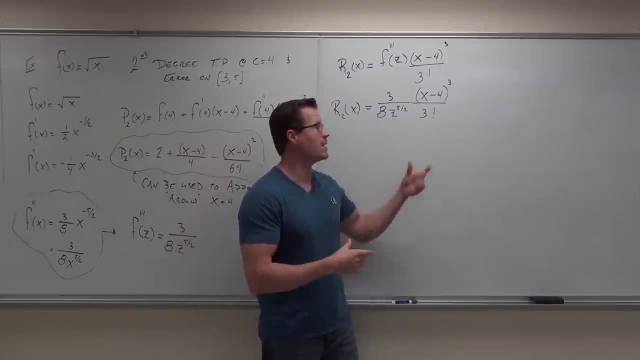 What I'm trying to tell you is that pick the end point. If there exists one, it gives you the maximum distance here. I don't know if you understand that idea. I'm going to pick the 5.. Just to show you that the x does not have to be 3.. 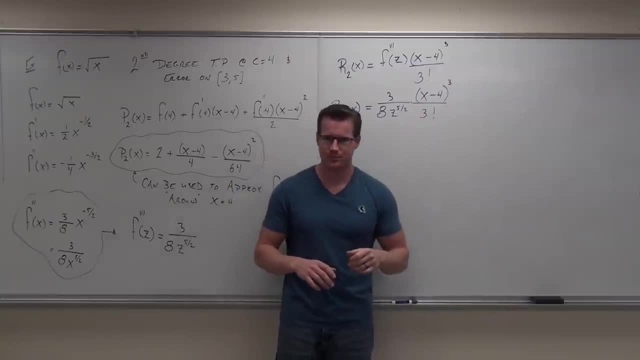 It's going to be the same as the z. I would pick the 5 for the x, Now the z. You need to pick one of these numbers in here. that gives you the biggest error possible. If I picked 5 for my z, would it be the biggest error or the smallest error? 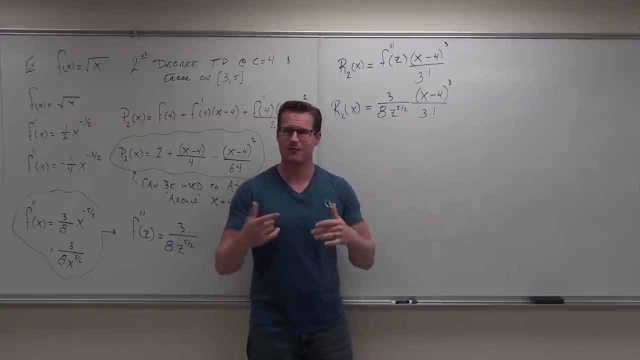 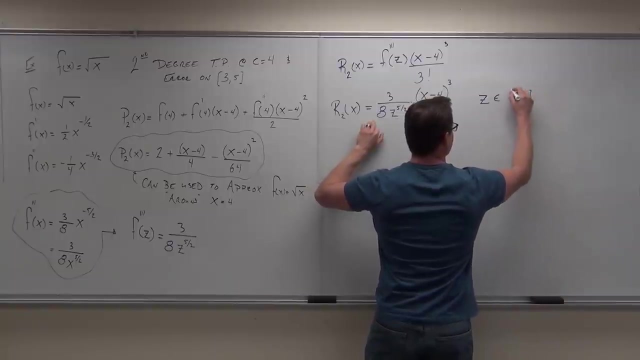 Smallest. What would be the biggest error? 3. Because if I'm dividing by a number, dividing by a smaller number gives me a larger fraction here. Does that make sense to you? So here's what we know. We know that z is somewhere on 3 to 5.. 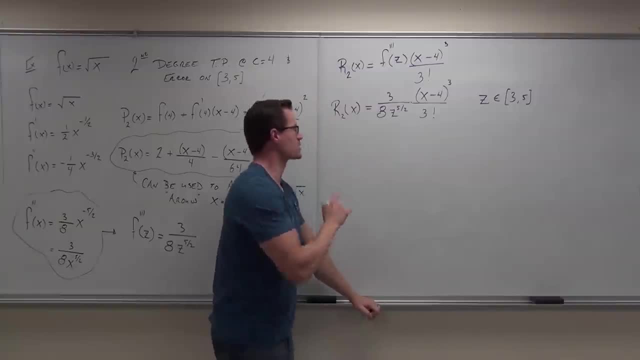 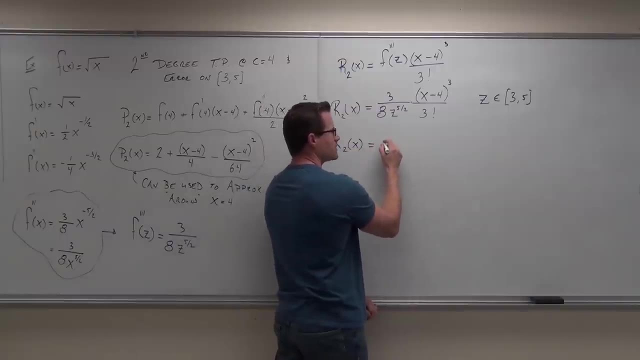 So we're going to pick the z. that gives us the largest possible error. So our error of our second degree Taylor polynomial in this case is going to be when we use 3 as our z. So if I were to approximate my function at the number 3.. 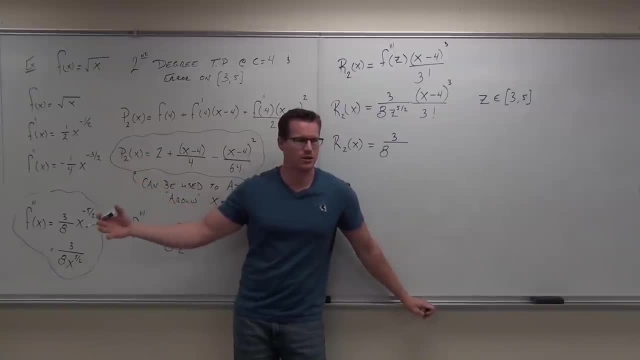 So if I were to plug in 3, that's going to give me the answer that has the most error. Make sense to you Anything more than that, like 3.01 or 4 or 5, that's going to give me a smaller error than if I were to plug in 3.. 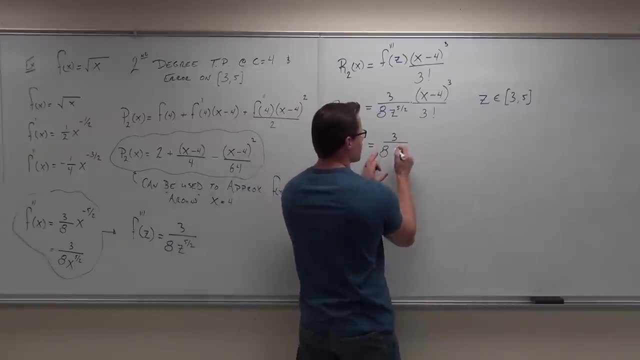 So to say: this is the maximum error that we get. we're going to use that 3.. It gives us the biggest fraction. What was I going to use for x here? 5.. Yeah, 5 or 3.. It doesn't really matter, because you're going to get 1 or negative 1.. 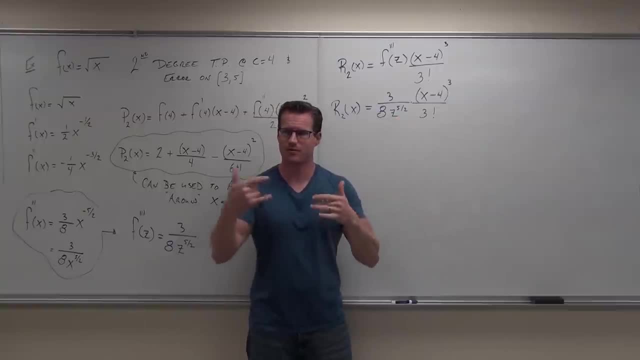 Smallest. What would be the biggest error? 3. 3. Because if I'm dividing by a number, dividing by a smaller number gives me a larger fraction here. Does that make sense to you? So here's what we know. 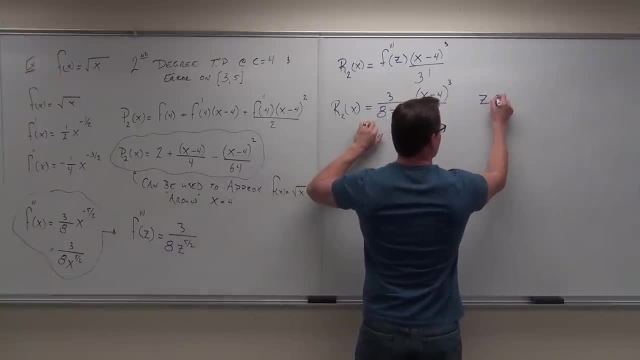 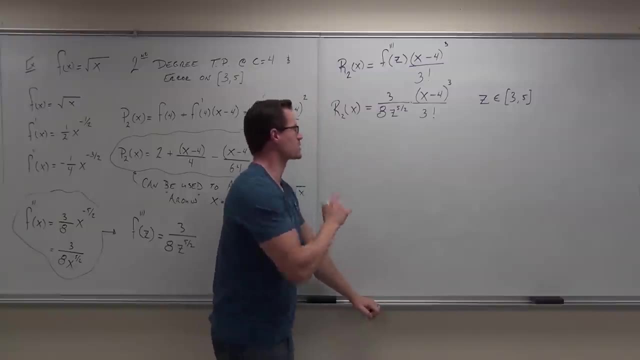 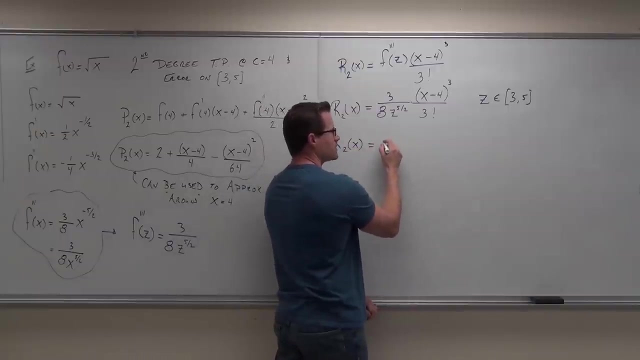 We know that z is somewhere on 3 to 5.. So we're going to pick the z. It gives us a little bit of distance. Okay, So that's the largest possible error. So our error of our second degree Taylor polynomial in this case is going to be when we use 3 as 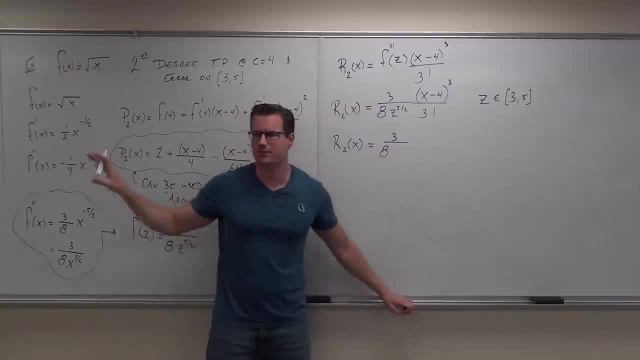 our z. So if I were to approximate my function at the number 3.. So if I were to plug in 3, that's going to give me the answer that has the most error. Make sense to you? Anything more than that, like 3.01 or 4 or 5, that's going to be a smaller error than 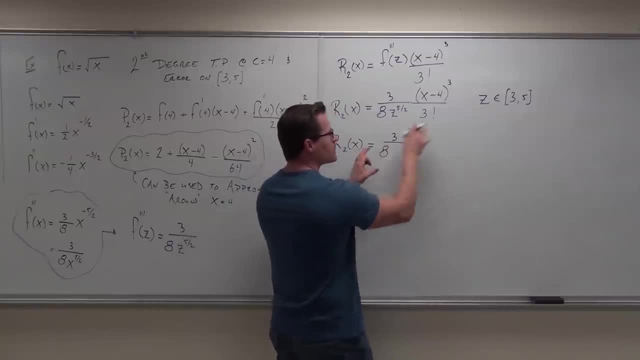 if I were to plug in 3.. So to say, this is the maximum error that we get. we're going to use that 3. It gives us the biggest fraction. What was I going to use for x here? 5. Yeah, 5 or 3.. 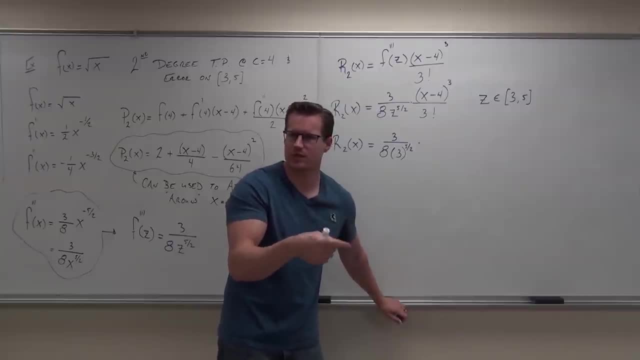 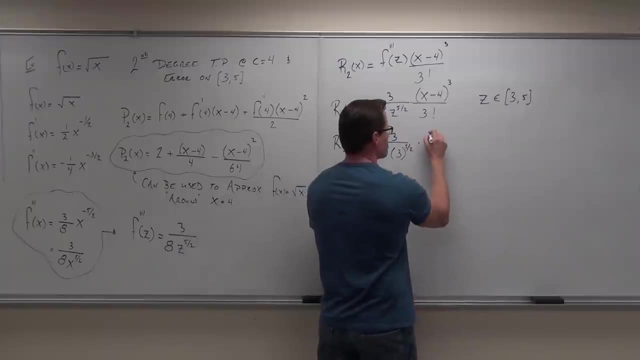 It doesn't really matter, because you're going to get 1 or negative 1.. You just want to pick one of those n points that gives you at least the biggest value in terms of absolute value. So I picked 5 to keep it positive. 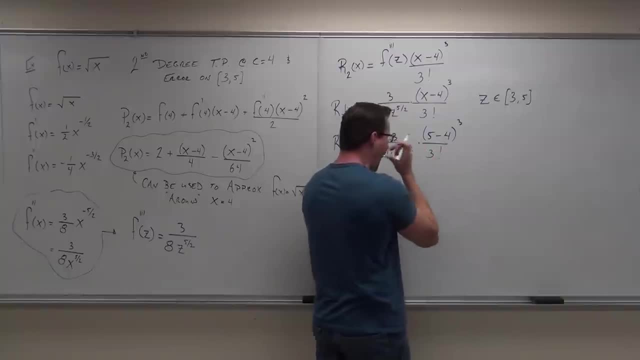 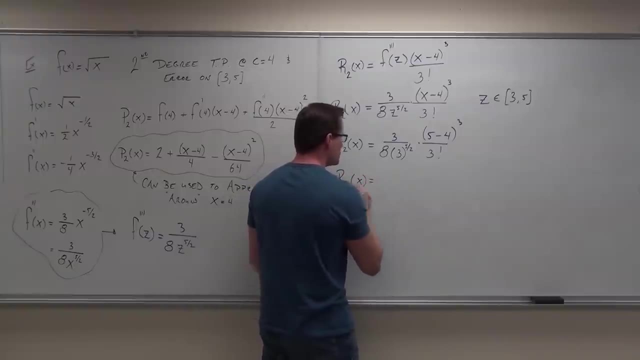 It's all good. So what this all works out to well. the 3 and the 3, factorial again. to simplify, you're going to get 2, let's see, here's 1 to the 3rd, that's 1.. 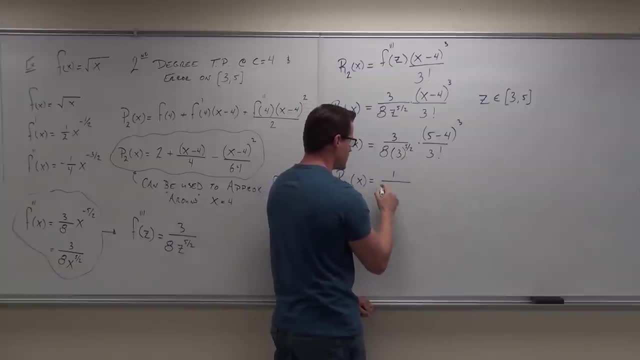 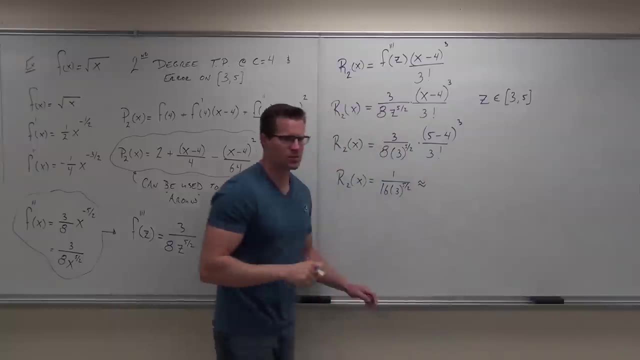 That gives you 2 times 1, so that's 2 times 8, that would be our 16, times 3 to the 5 halves, And that's roughly. can you, can someone do that for me, tell me what that is roughly? 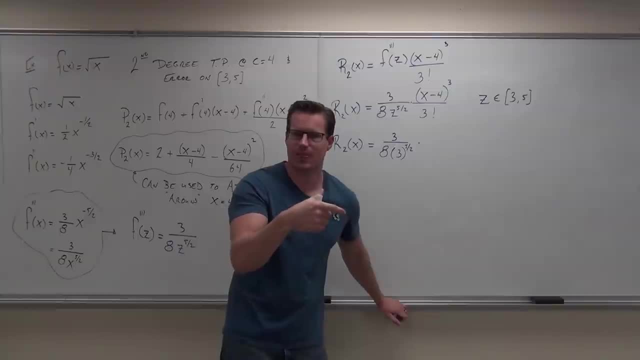 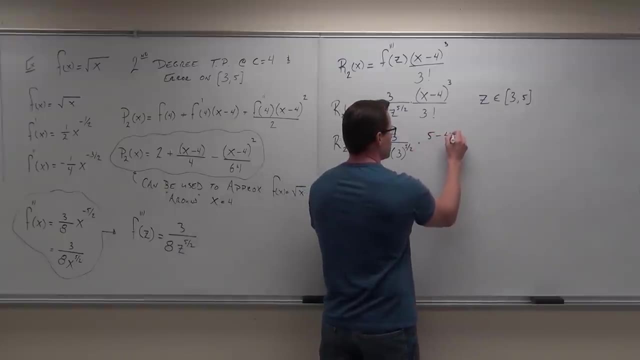 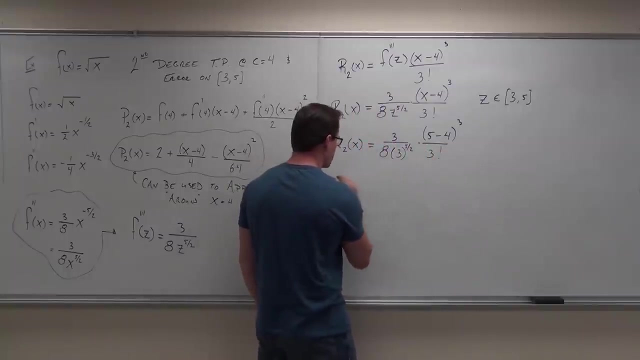 You just want to pick one of those endpoints that gives you the least. It gives you at least the biggest value in terms of absolute value. So I picked 5 to keep it positive. It's all good. So what this all works out to. 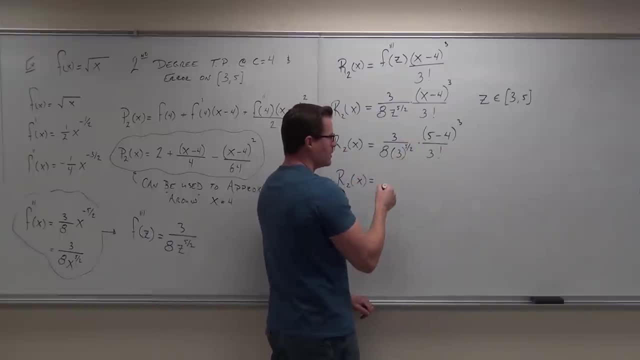 Well, the 3 and the 3, factorial again, to simplify, you're going to get 2.. Let's see Here's: 1 to the third, That's 1.. That gives you 2 times 1.. So that's 2 times 8.. 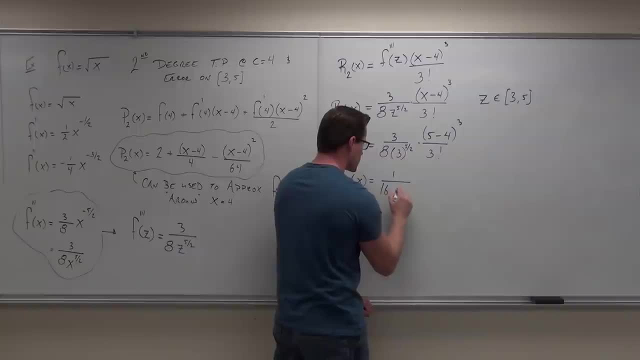 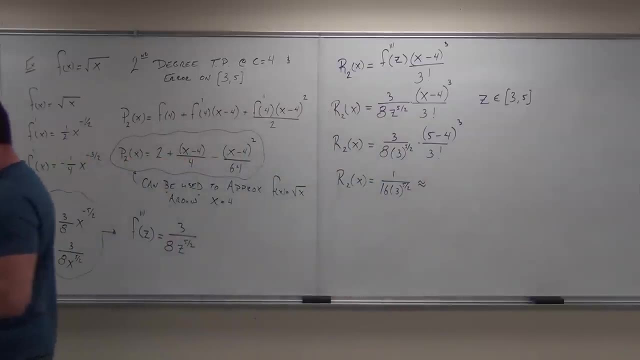 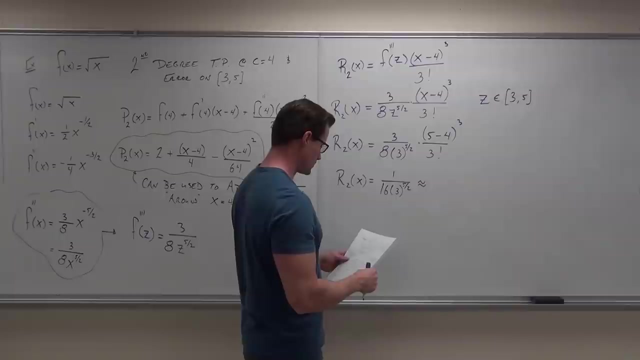 That would be our 16. Times 3 to the 5 halves And that's roughly. Can someone do that for me? Tell me what that is? roughly About 249.4.. Yeah, Say what now? 249.4.. 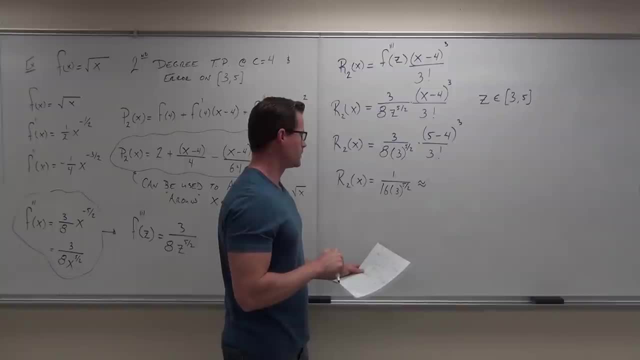 2. It's got to be a decimal: .004.. .004.. Let me get a double check on that. .004.. I agree. Well, if Rob agrees, it must be right. So Hopefully I did my math right. 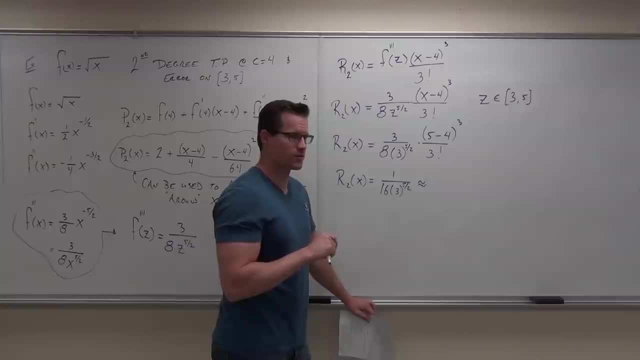 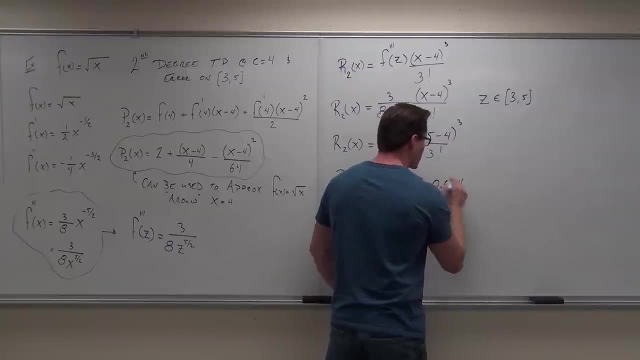 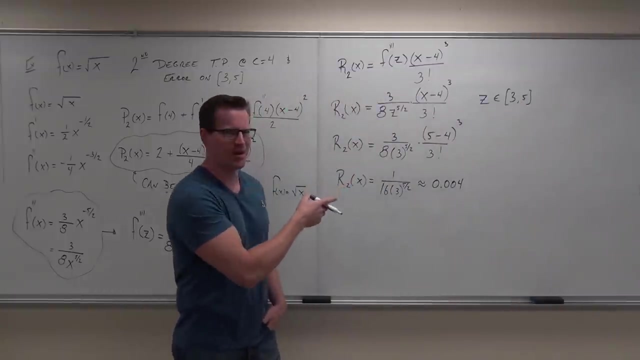 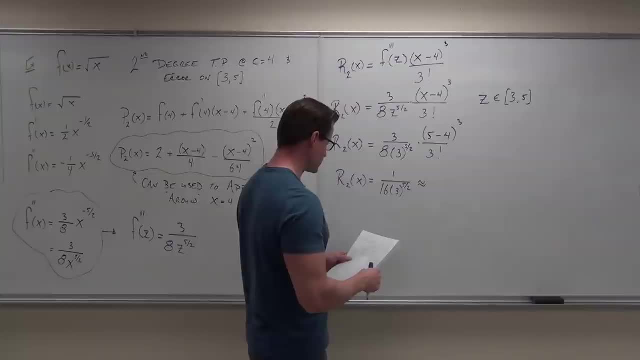 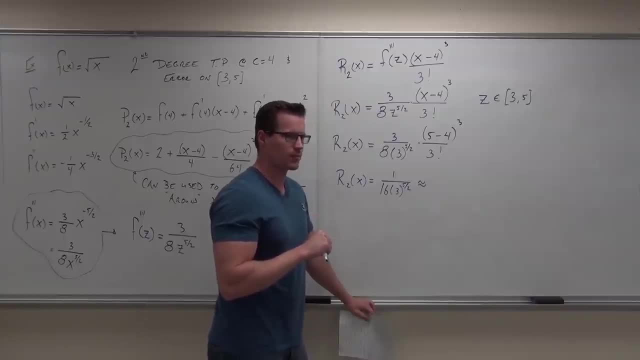 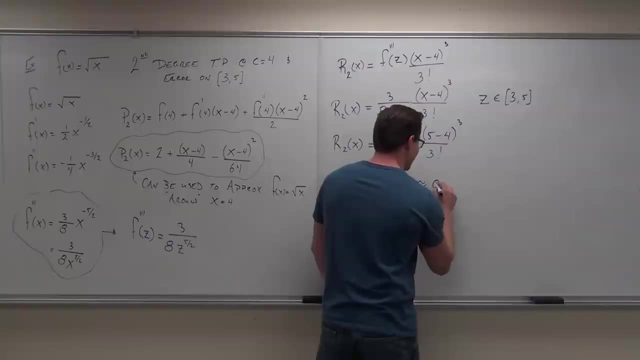 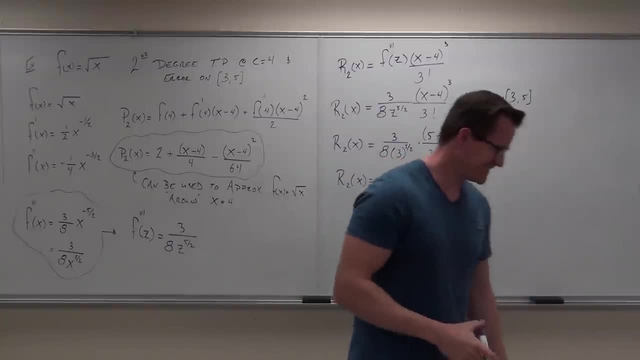 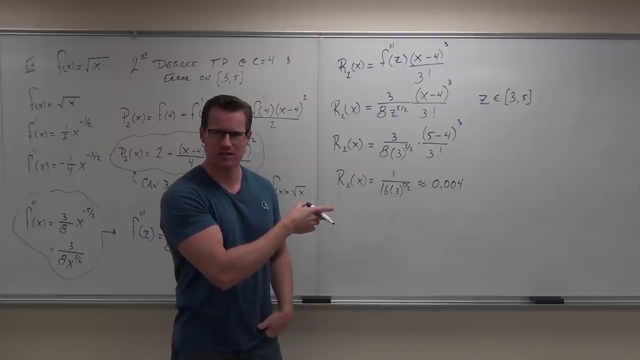 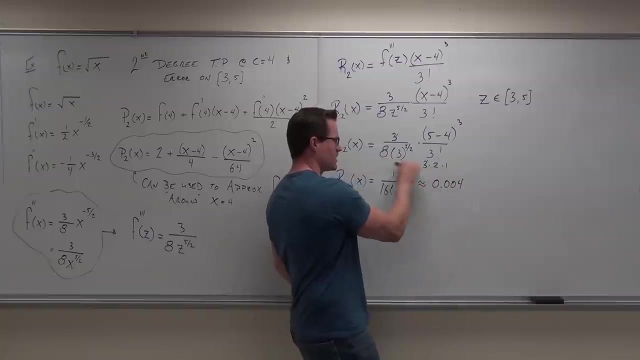 Hopefully I did my math right. Did I do my math right? Did you check it? Yeah, If this is 3 times 2 times 1, then our 3's are gone. No, No, and we get two times eight, that's 16, we have this. 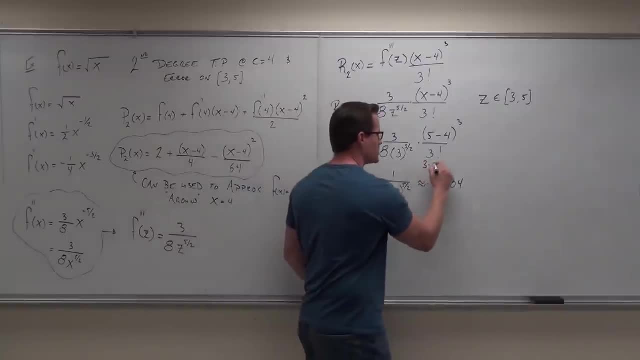 Did I do my math right? Did you check it? Yeah, Yeah, If this is 3 times 2 times 1,, then our 3s are gone And we get 2 times 8,, that's 16.. 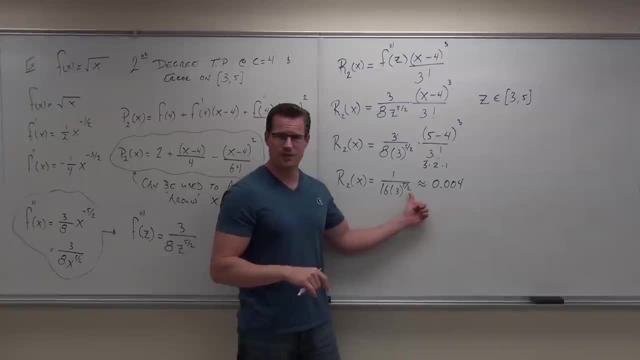 And we get this. And you did on your calculator, make sure you did this right. You did 3 to the 5th house power, Right? And then you multiplied by 16, after that Correct, Yes, And you got .004.. 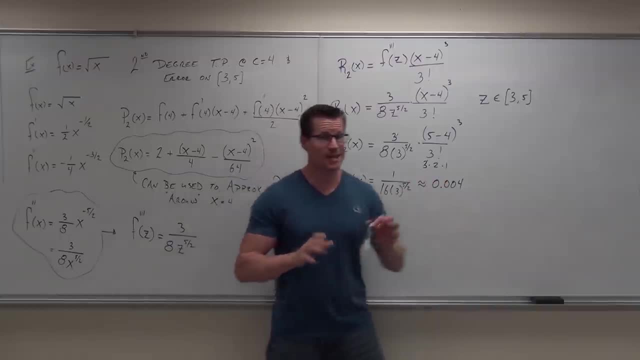 Okay, So here's what this says, Assuming that the math is correct. Here's what it says. It says All of this put together. it says this: It says that this is your secondary Taylor Point of Role, three-tailed polynomial. 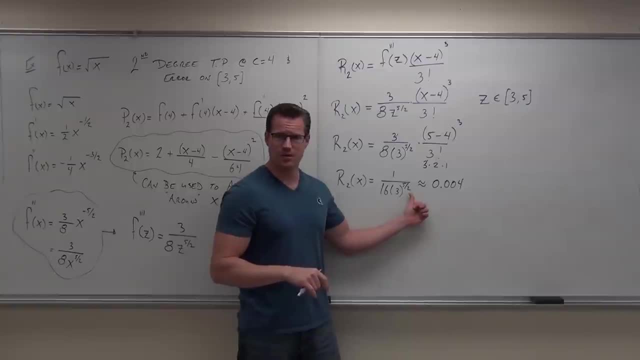 And you did on your- I wanna make sure you did this right. You did three to the five-tenths power, right? And then you multiplied by 16, after that correct, And you got .004, okay. so here's what this says. 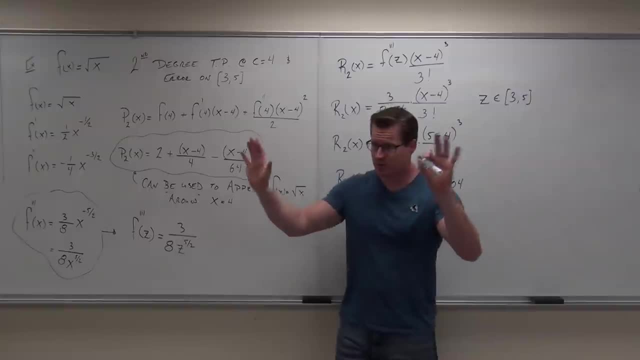 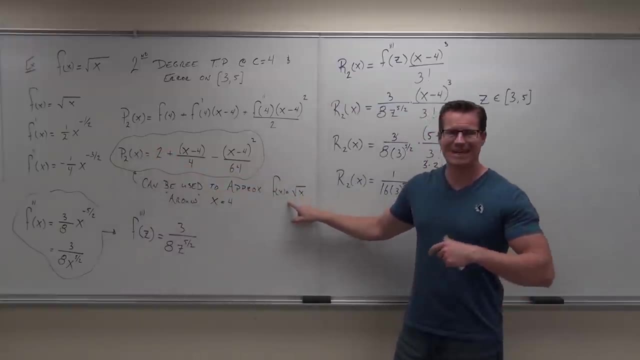 Assuming that the math is correct, here's what it says. It says all of this put together says this: It says that this is your secondary Taylor polynomial. This can be used to approximate this function at any numbers around four, In fact, if you pick numbers between three and five. 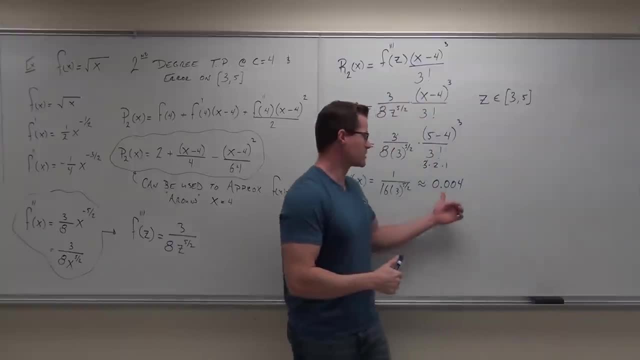 inclusive. the maximum error that you will get is .004.. That says that any answer that you get using this, any answer you get using this, is within four-thousandths of the actual value of this function, at whatever point you plugged in. Show me if you feel okay with that one. 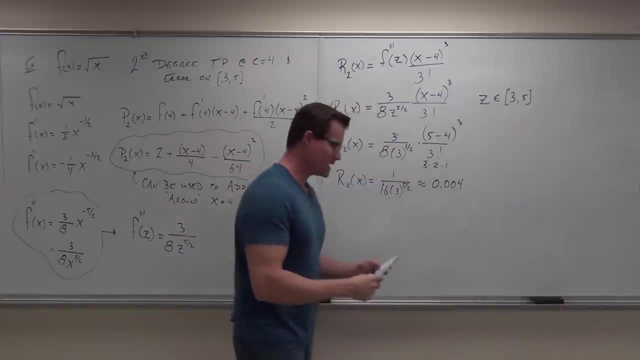 That's the idea. Now, what I'd like you to do is, since you guys are working out of a calculus textbook, read the other examples. I obviously can't go over all of them in class, but this is basically the idea. 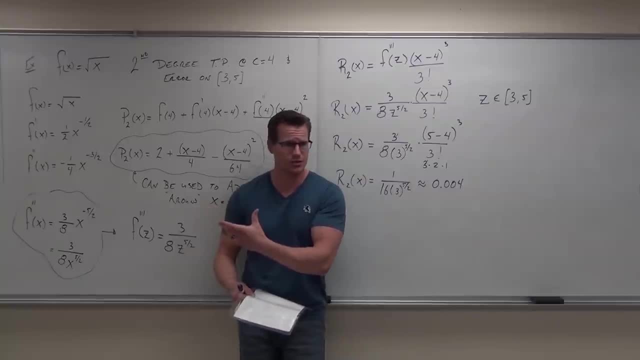 and I think, hopefully I've explained this well enough for you to understand the idea. Do you guys get it? The basic idea is: well, take a Taylor series, take part of it. It's called Taylor polynomial. It will have an error because you're not taking. 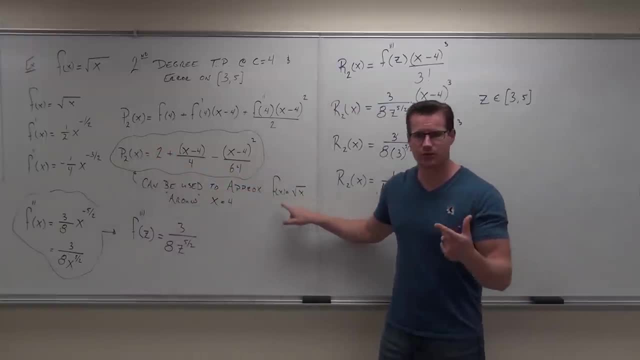 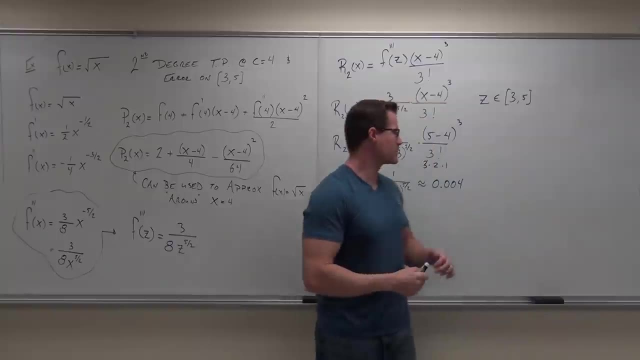 This can be used to approximate this function at any numbers around four. In fact, if you pick numbers between three and five inclusive, the maximum error that you will get is .004,. that says that any answer that you get using this, any answer you get using this, is within four thousandths. 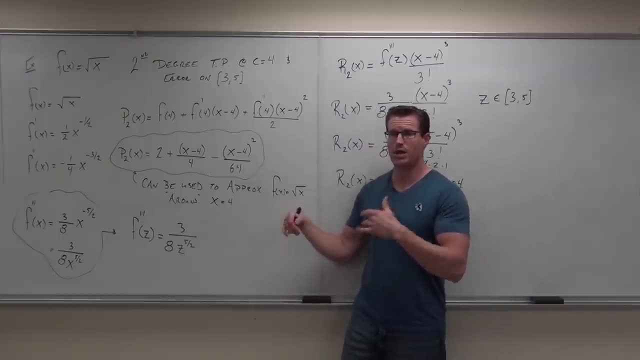 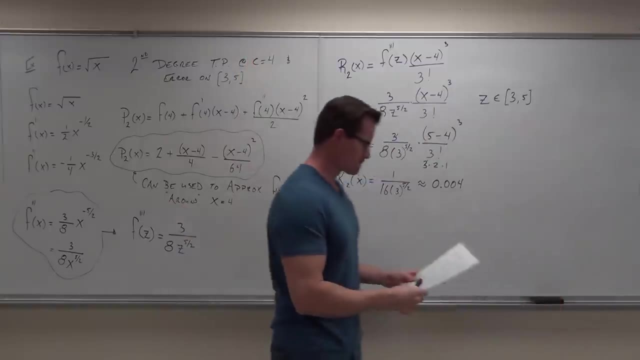 of the actual value of this function at whatever point you plugged in. Show me if you feel okay with that one. That's the idea. Now what I'd like you to do is- since you guys are working out of a calculus textbook, 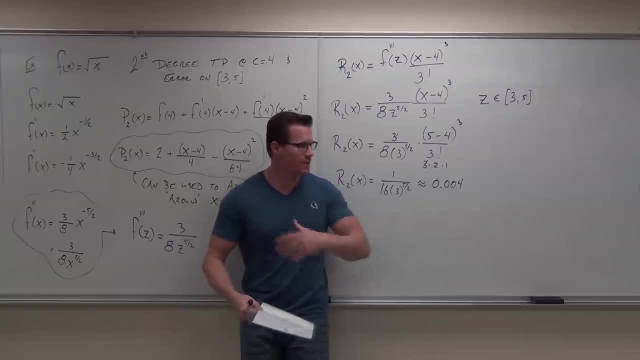 read the other examples. I obviously can't go over all of them in class, but this is basically the idea and I think hopefully I've explained this well enough for you to understand the idea. Do you guys get it? The basic idea is: well, take a Taylor series. 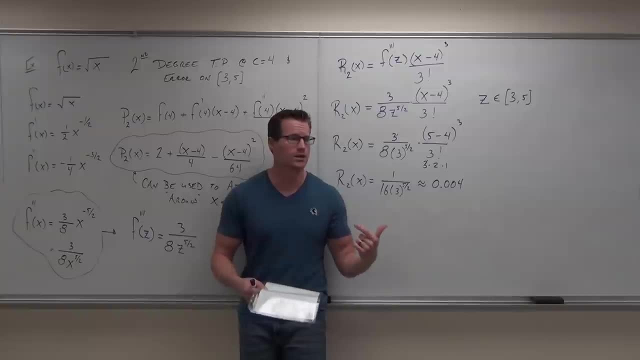 take part of it. It's called a Taylor polynomial. It will have an error because you're not taking the whole Taylor series. that error's really easy to find. It's just the next term after you stop at whatever degree I've told you. 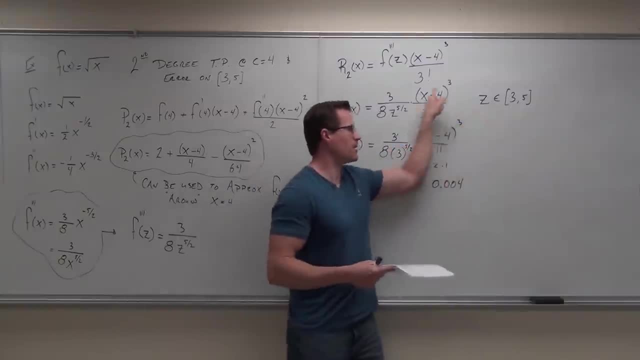 You can find that by making it the biggest possible error- and that's the maximum error you can get- from a Taylor polynomial when using it to approximate your function. Okey-dokey, Now I want to talk about something else. I want to talk about how to determine. 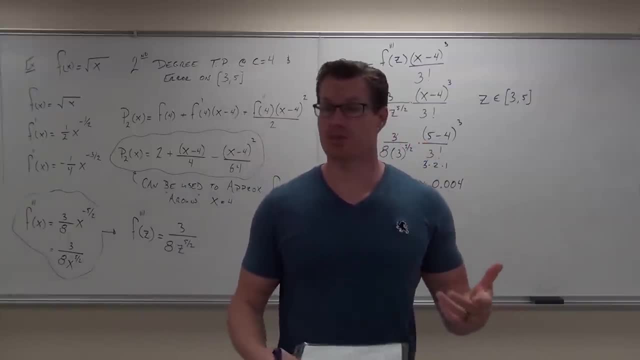 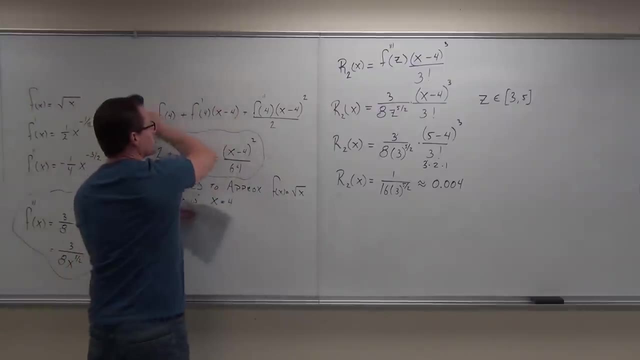 when a function can be represented by a Taylor series. That's the next thing we're gonna do. It's not a super hard concept, but it's a little bit different. By the way, are there any questions on this one, as I'm erasing the board? 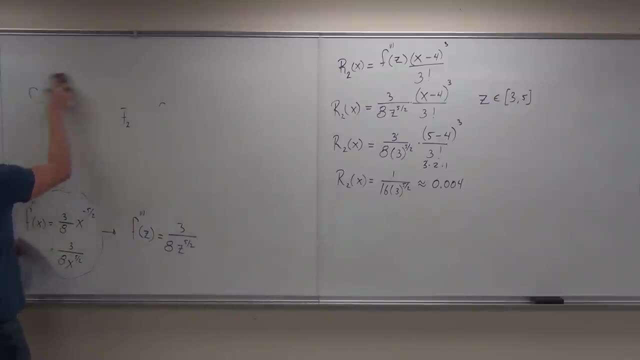 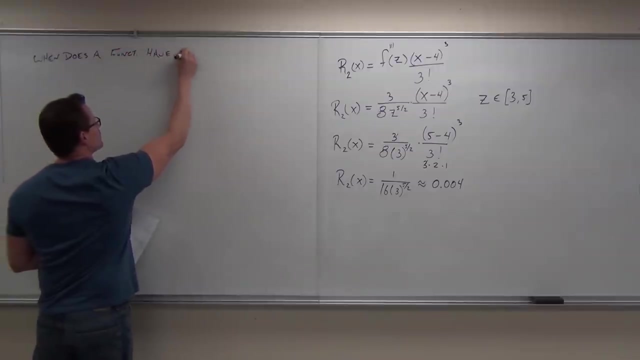 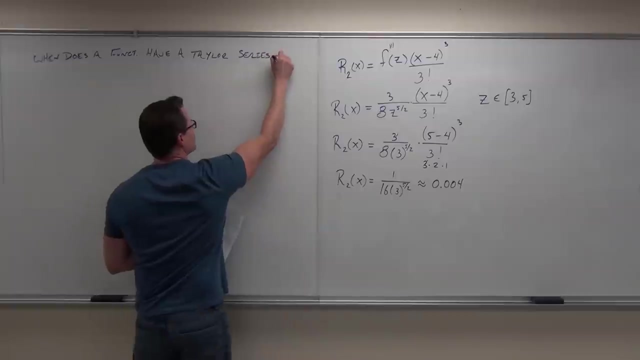 Mm-hmm. Okay, Rewind, Yeah, just rewind it. That'd be so cool if I could actually do that in real life. So when does a function have a Taylor series representation? When does a function have a Taylor series representation? 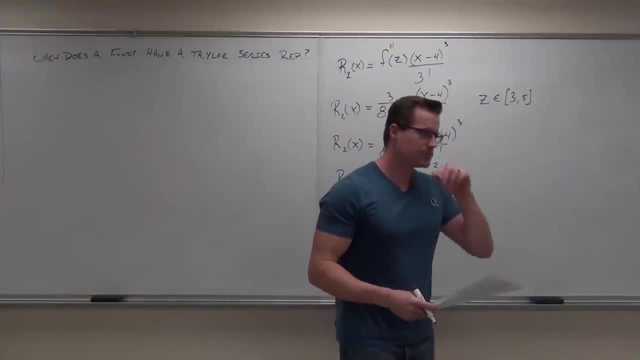 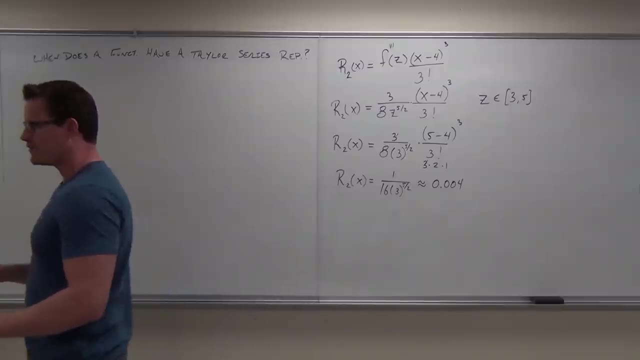 Well, let's think about it this way. Let's use what we know about Taylor polynomials. If we have a Taylor polynomial, then that Taylor polynomial is going to have a remainder, isn't it? So if the remainder is going to be a remainder, isn't it? 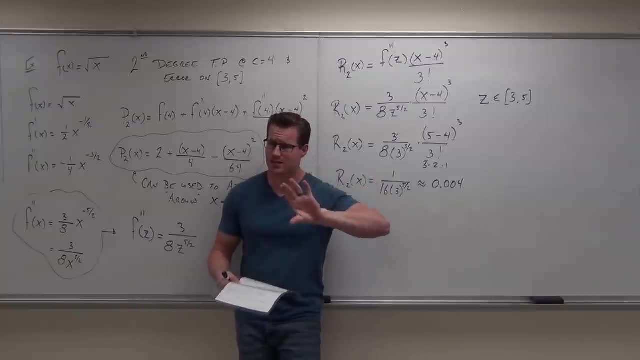 the whole Taylor series. That error's really easy to find. It's just the next term. after you stop at whatever degree I've told you to, You can find that by making it the biggest possible error and that's the maximum error you can get. 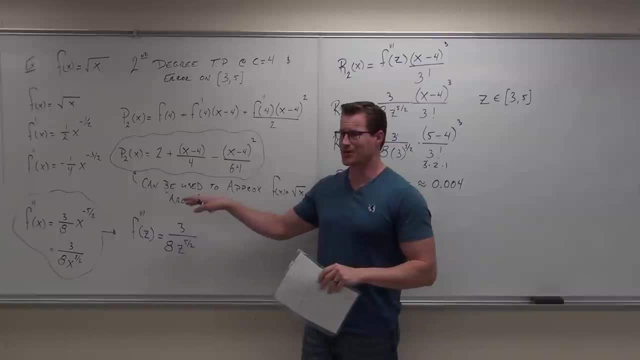 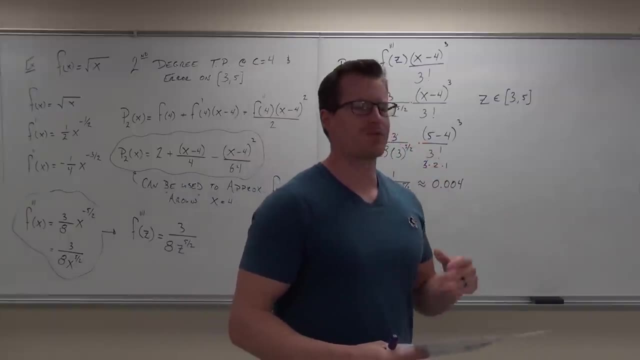 from a Taylor polynomial when using it to approximate your function. Okie dokie. Now I want to talk about something else. I want to talk about how to determine when a function can be represented by a Taylor series. That's the next thing we're going to do. 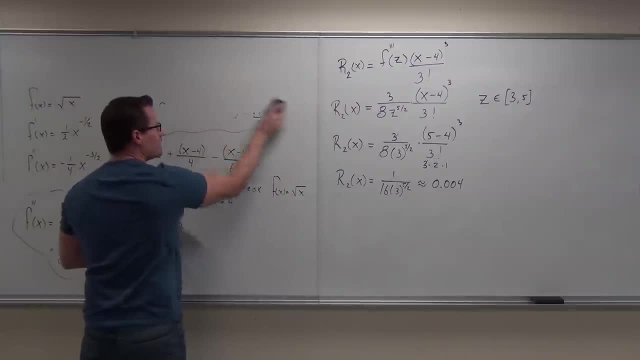 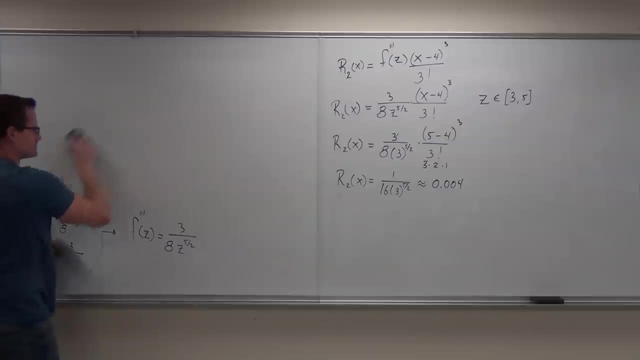 It's not a super hard concept, but it's a little bit different. By the way, are there any questions on this one, as I'm erasing the board? Okay, Rewind, Yeah, just rewind it. That would be so cool if I could actually do that. 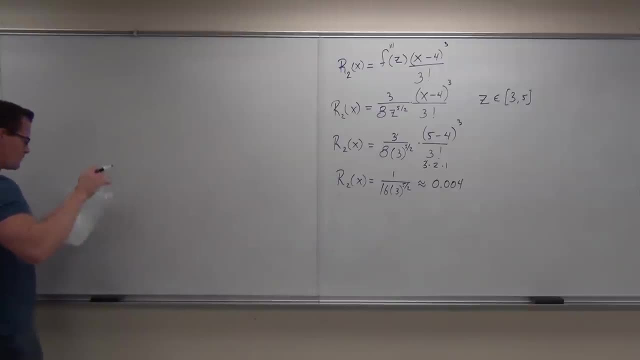 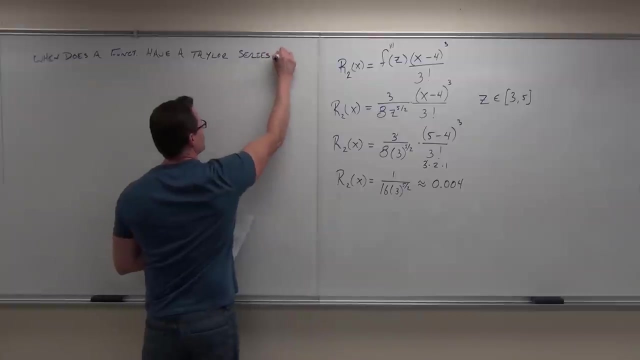 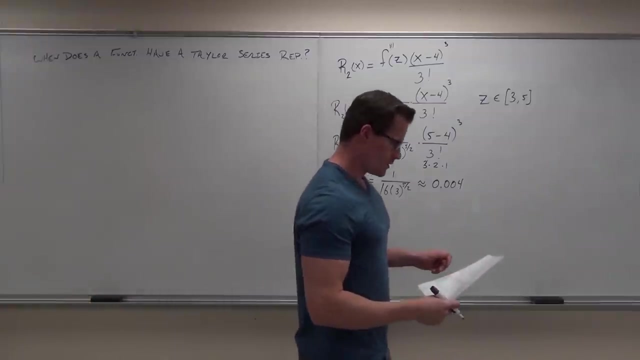 in real life, wouldn't it? Mm-hmm. So when does a function have a Taylor series representation? Where does a function have a Taylor series representation? Well, let's think about it this way: 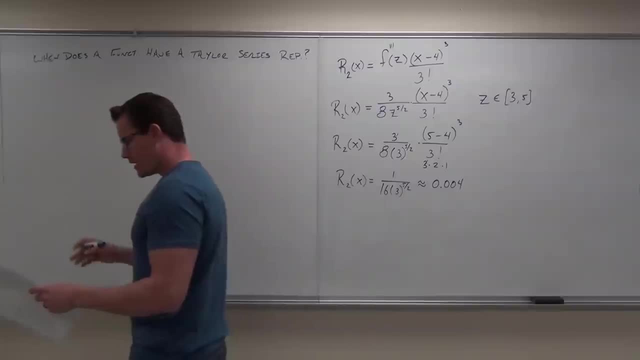 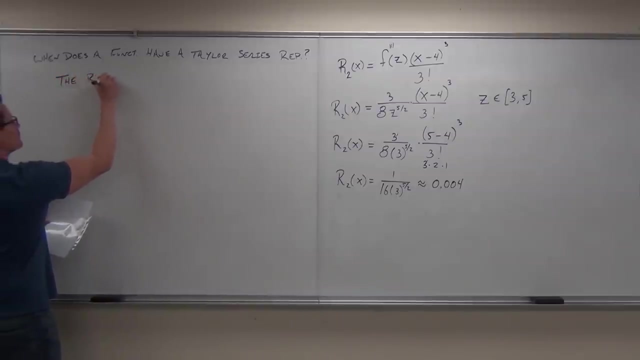 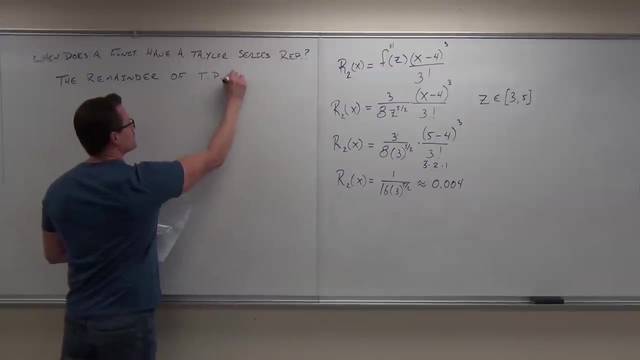 Let's use what we know about Taylor polynomials. If we have a Taylor polynomial, then that Taylor polynomial is going to have a remainder, isn't it? So if the remainder of a Taylor polynomial, so the remainder of a Taylor polynomial is this: 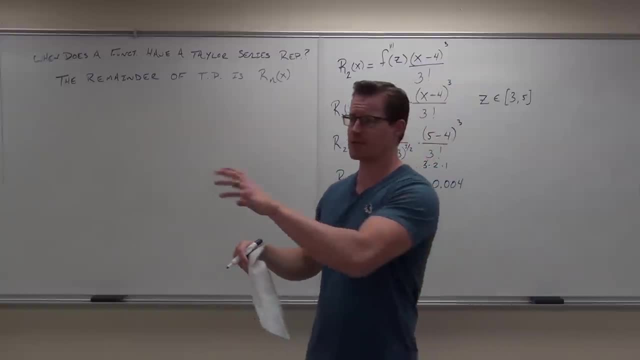 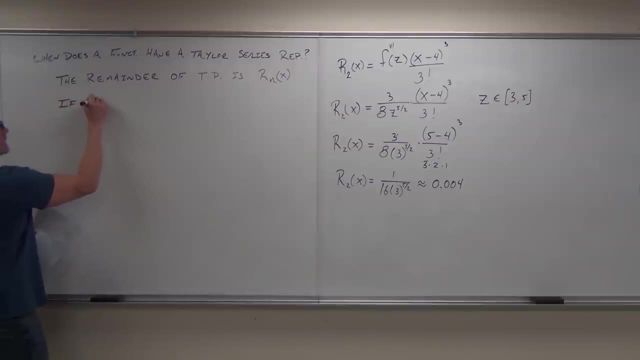 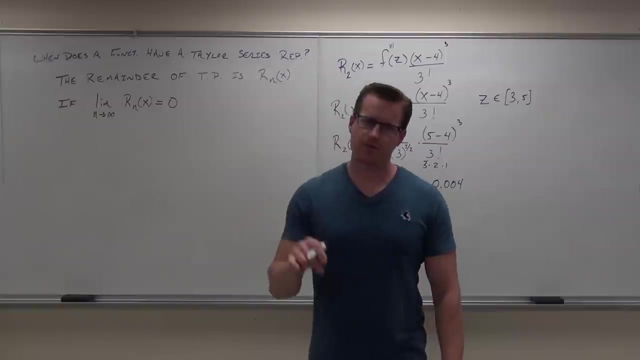 It's the remainder of whatever degree Taylor polynomial we have given a Taylor series. So we have this r sub n of x. Here's the idea. If the limit of your remainder goes to 0,, if the limit of your remainder from your Taylor polynomial goes to 0,, then our function can be. 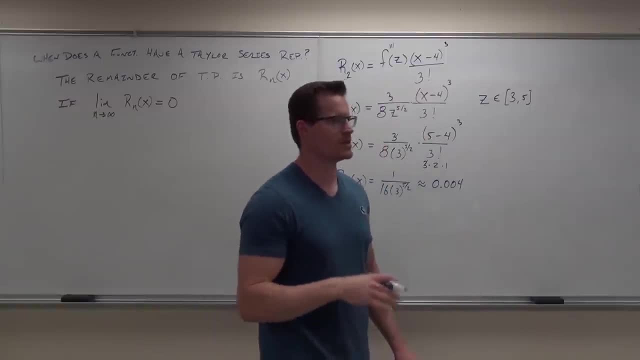 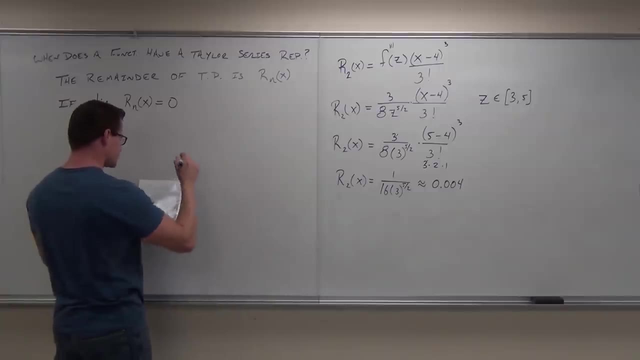 represented by a Taylor series, And I'm not going to prove it. I'll give you the idea of the proof. It's not a really hard proof, but I'll show you the idea. So if the limit of your remainder goes to 0,, then your 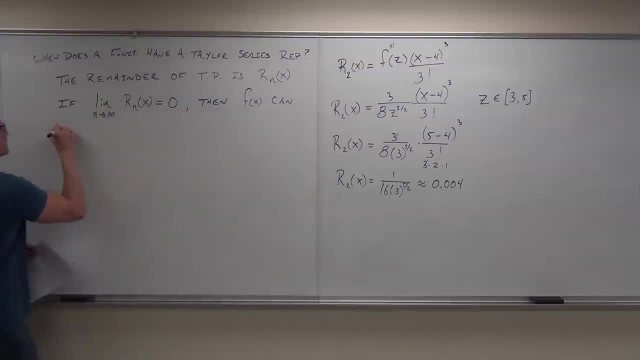 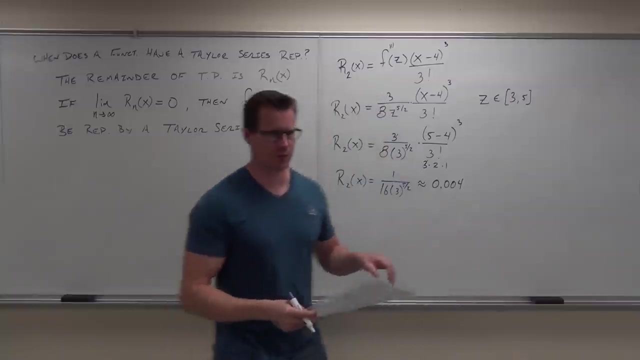 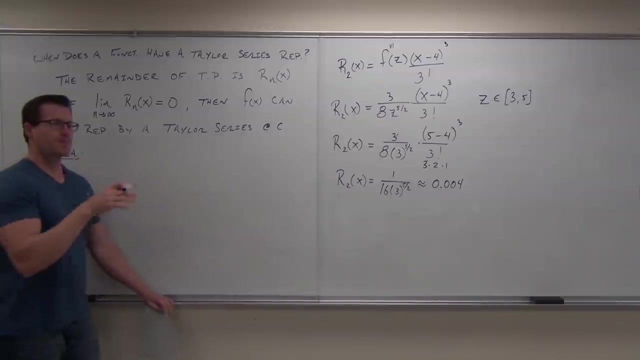 function. It can be represented by a Taylor series at some point C. Let me give you the idea of the proof. OK, Here's the idea. So, idea of the proof, kind of a skeleton proof. Here's the thing, What we just learned about all this stuff- Taylor series and 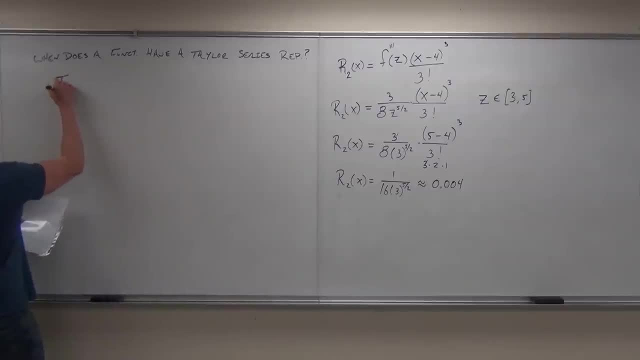 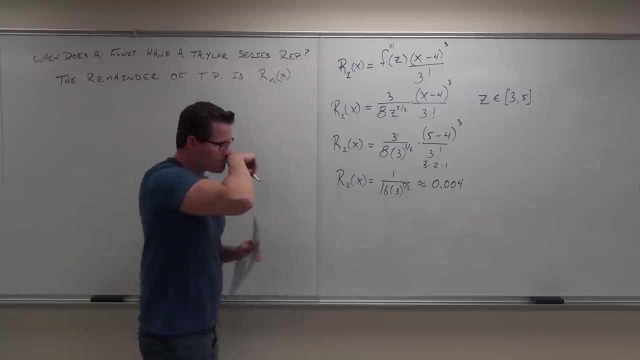 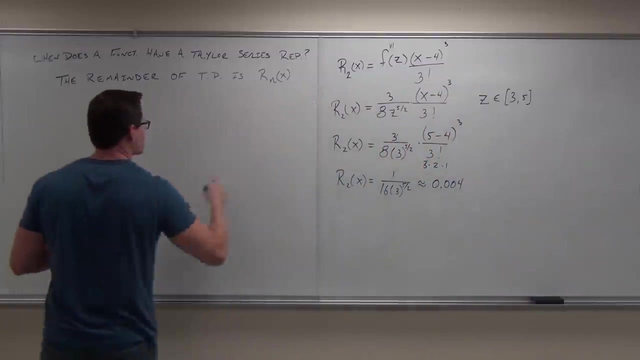 So if the remainder of a Taylor polynomial is this, So the remainder of a Taylor polynomial is this: It's the remainder of whatever degree Taylor polynomial we have given a Taylor series. So we have this r sub n of x. Here's the idea. 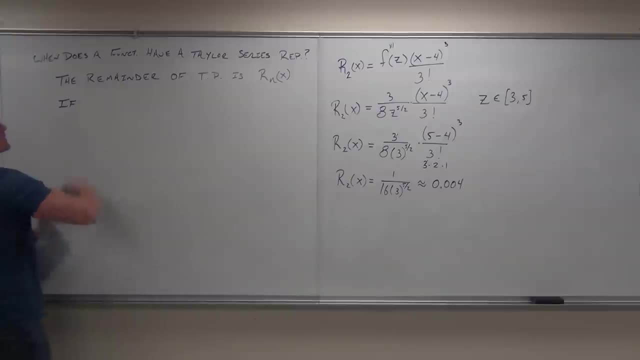 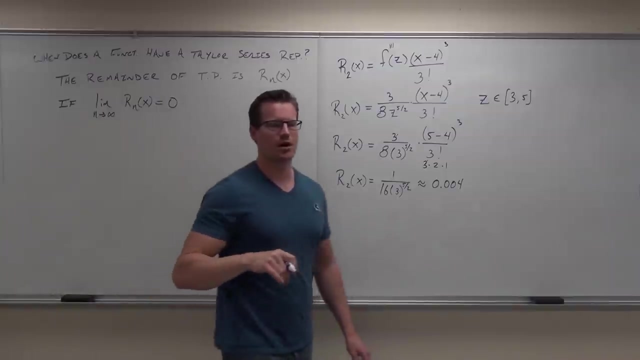 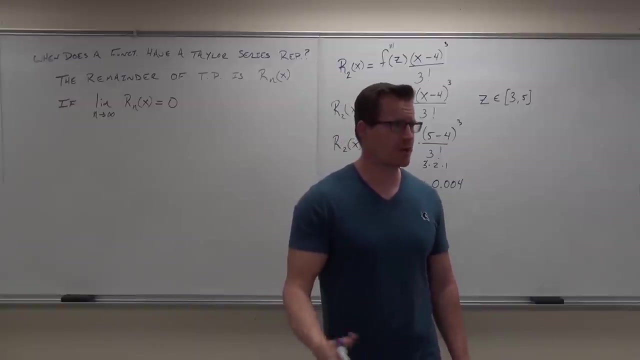 If the limit of your remainder goes to 0,, if the limit of your remainder from your Taylor polynomial goes to 0,, then our function can be represented by a Taylor series. And I'll give you- I'm not going to prove it- 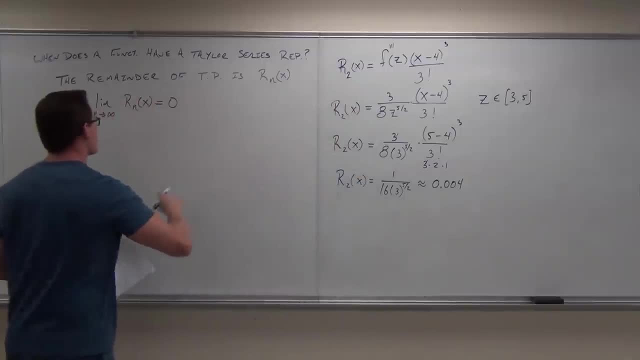 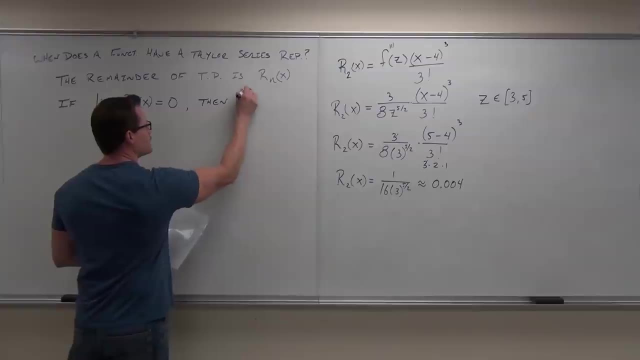 I'll give you the idea of the proof. It's not a really hard proof, but I'll show you the idea. So if a limit of the remainder goes to 0, it'll be easy to follow this idea. So, if a limit of your remainder goes to 0,, 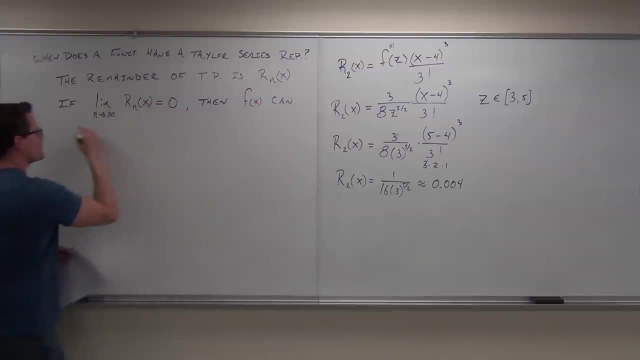 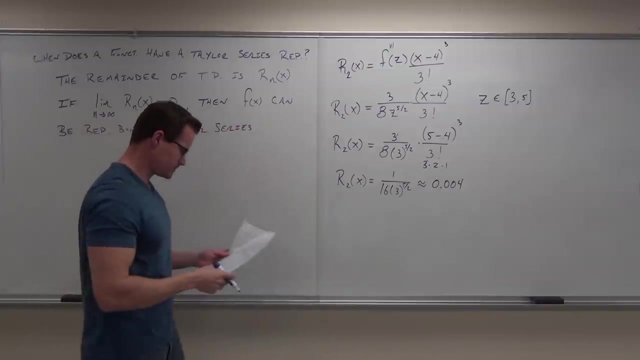 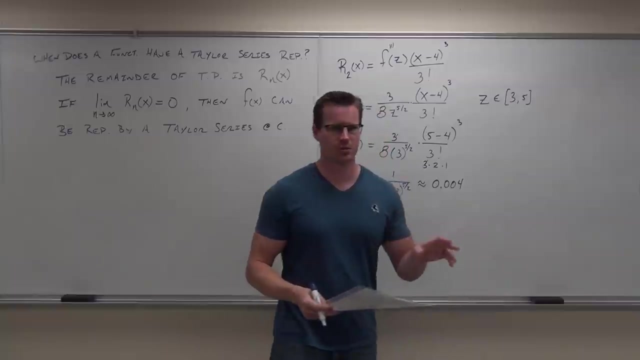 then your function can be represented by a Taylor series. Then your function can be represented by a Taylor series At some point, see, At some point, see. Let me give you the idea of the proof. okay, Here's the idea. 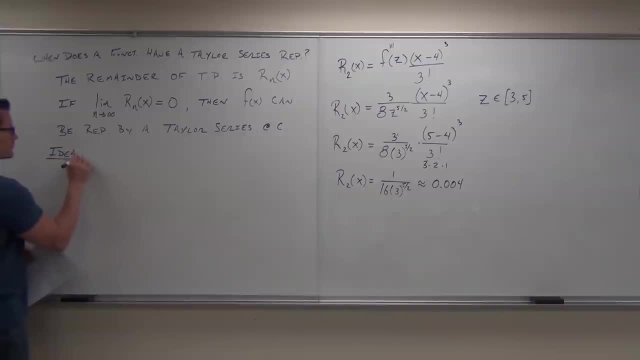 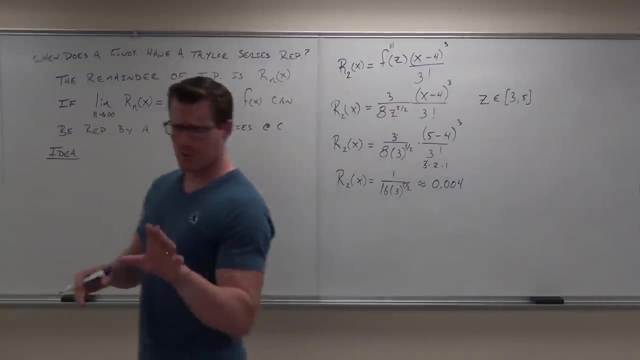 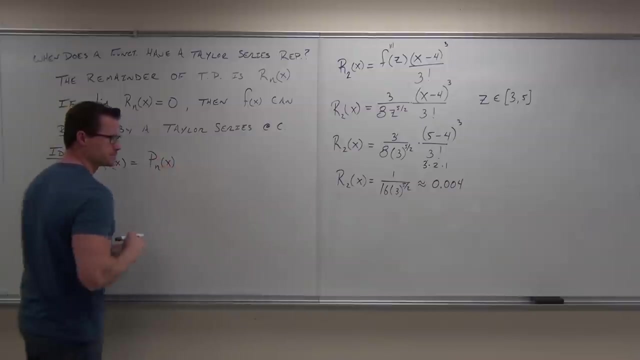 It's an idea of the proof, kind of a skeleton proof. Here's the thing: What we just learned about all this stuff- Taylor series and Taylor polynomials- is that if we represent a function by a Taylor polynomial, if we represent a function by a Taylor polynomial, 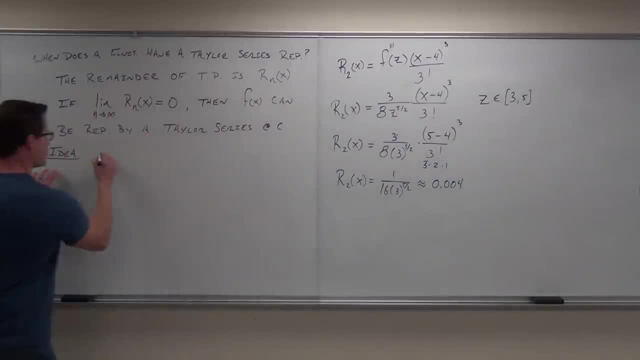 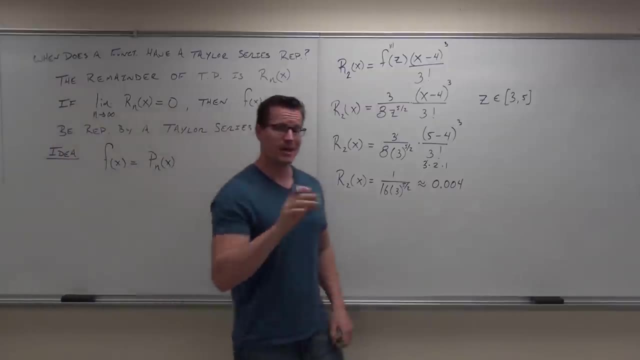 Taylor polynomials is that if we represent a function by a Taylor polynomial, if we represent a function by a Taylor polynomial, well, this is not exactly right. In fact, if I represent a function with a Taylor polynomial, it's only an approximation. 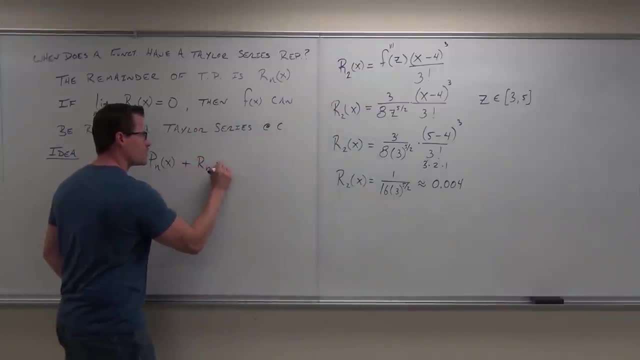 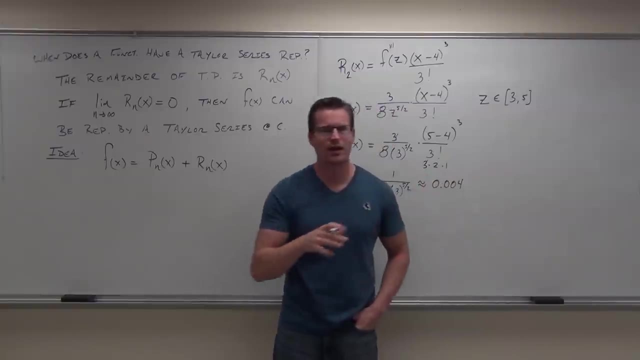 There's going to be some remainder. The rest, basically the rest of your Taylor series, gets lumped into that remainder. You guys remember doing that. Hopefully, because we just did it. OK, It says, yeah, this is true. 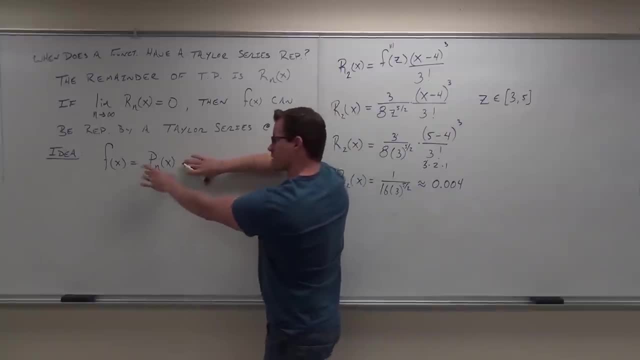 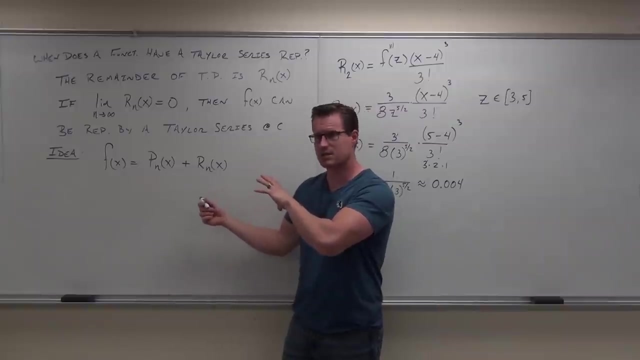 It's not really that a function gets represented by a Taylor polynomial. This is an approximation. The Taylor series is what would represent the function. So if it's possible to represent a function with a Taylor series, it's possible to represent the function with the polynomial plus a little bit more the remainder of that Taylor series. 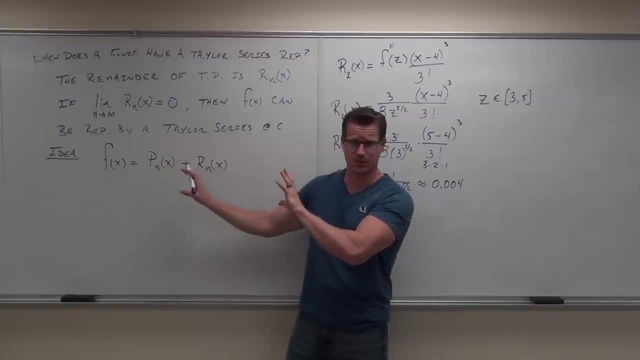 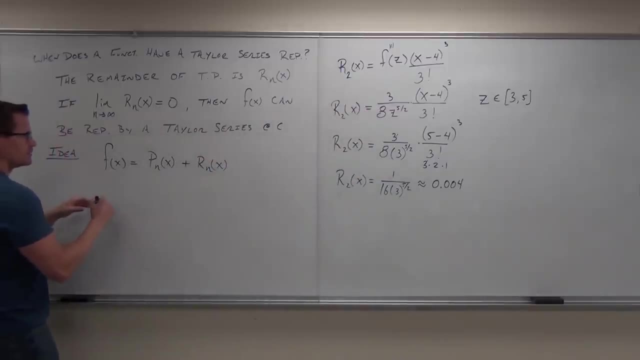 Quick head nod, please. I don't know if you understand the idea. This is how we got Taylor polynomials to begin with. OK, Well, if this is true, then if I just do a little bit of algebra here, then a Taylor. 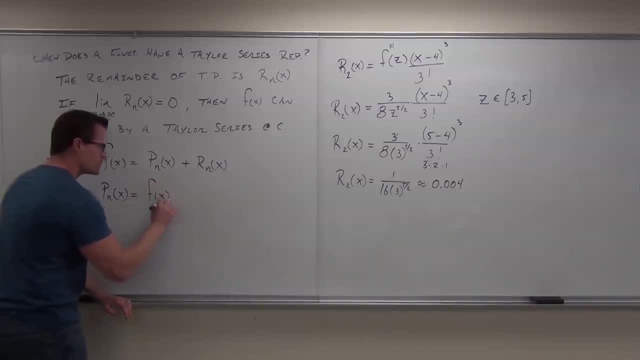 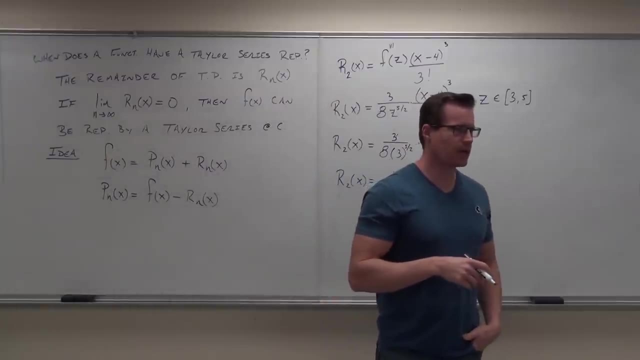 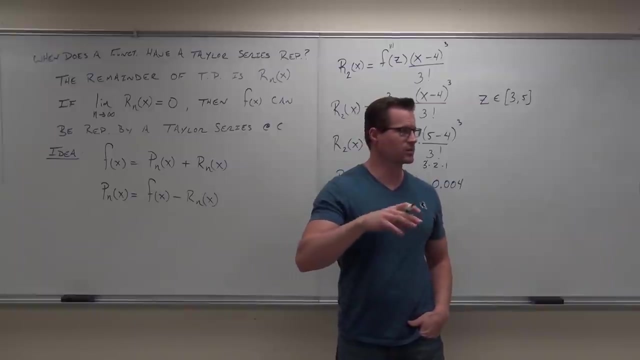 polynomial should be equal to the function minus the remainder, Shouldn't it? OK, The only time that this is ever going to work, so that the Taylor polynomial is going to be that the Taylor polynomial represents is equal to the function, is if this goes. 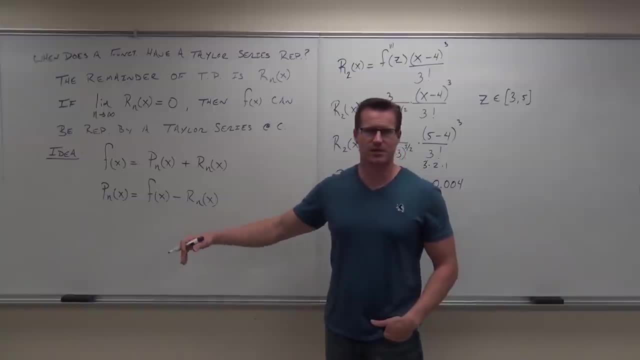 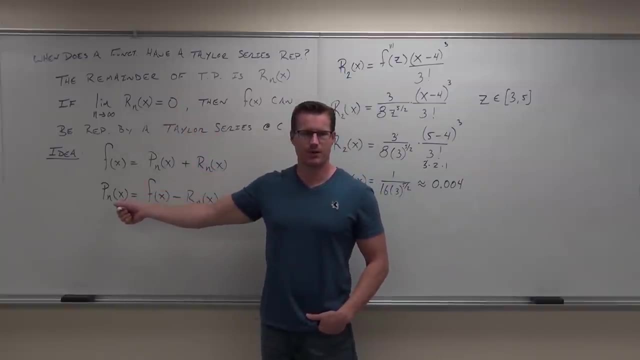 to what The second row: Yeah. So what the idea of the proof says is: you know what? If this goes to 0, ultimately, then the Taylor polynomial goes to the function. But keep in mind, here's what I'm trying to say. 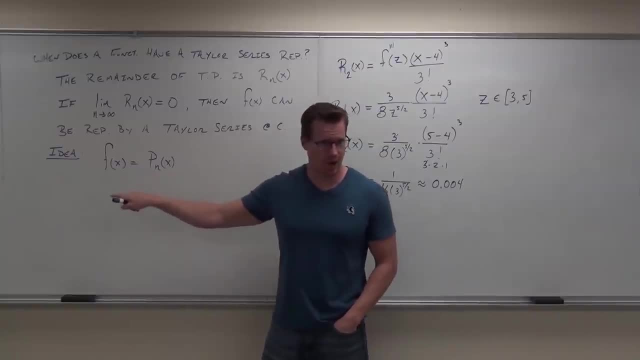 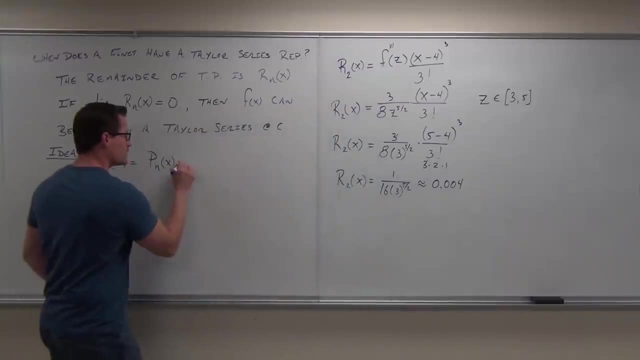 well, this is not exactly right. In fact, if I represent a function of a Taylor polynomial, it's only an approximation. There's going to be some remainder. The rest, basically the rest of your Taylor series, gets lumped into that remainder. 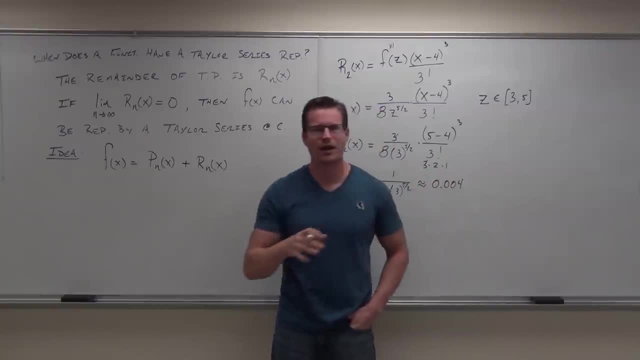 You guys remember doing that. Hopefully, because we just did it okay. It says: yeah, this is true, It's not really that a function gets represented by a Taylor polynomial. This is an approximation. The Taylor series is what would represent the function. 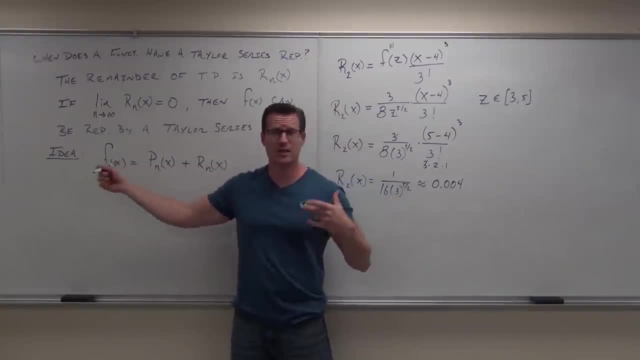 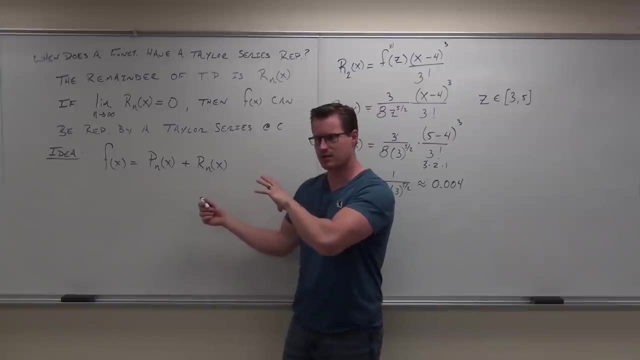 So if it's possible to represent a function with a Taylor series, it's possible to represent the function with the polynomial plus a little bit more the remainder of that Taylor series. Quick head nod if you understand the idea. This is how we got Taylor polynomials to begin with. okay. 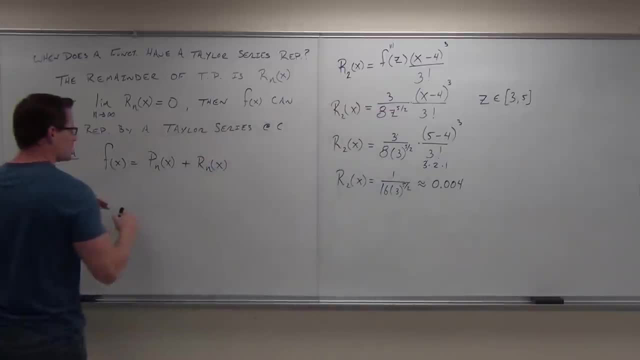 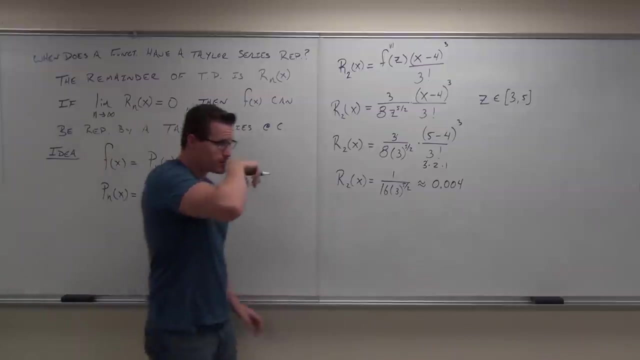 Well, if this is true, then if I just do a little bit of algebra here, then a Taylor polynomial should be equal to the function minus the remainder, Shouldn't it? Okay, The only time that this is ever going to work. 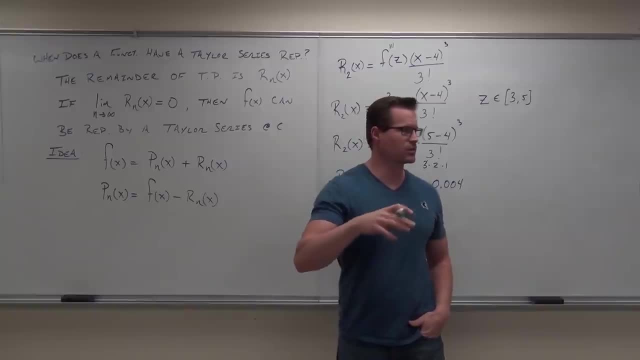 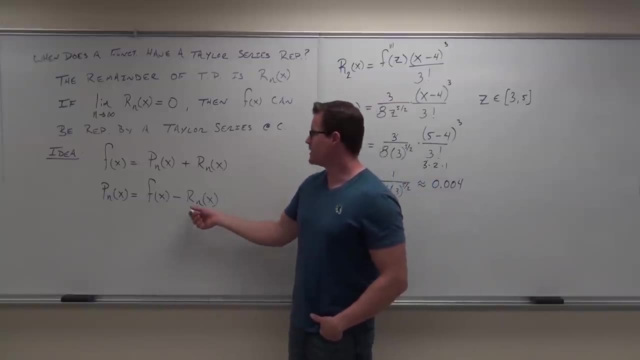 so that the Taylor polynomial represents is equal to the function, is: if this goes to what? Zero. So what the idea of the proof says is: you know what? If this goes to zero, ultimately, then the Taylor polynomial goes to the function. 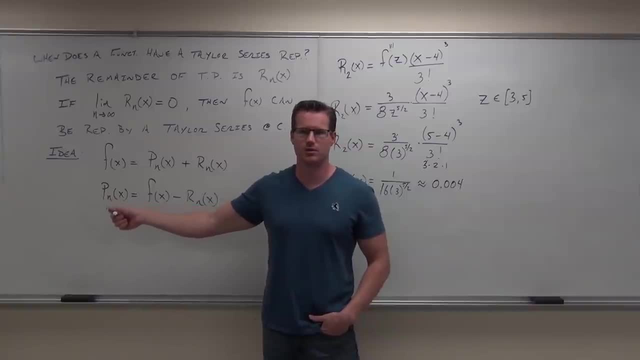 But keep in mind. here's what I'm trying to say. I'm not saying that the function is going to be equal to zero. I'm not saying that the polynomial. I'm not saying that the polynomial equals the function. What I'm saying is that as n approaches infinity, as n approaches infinity. 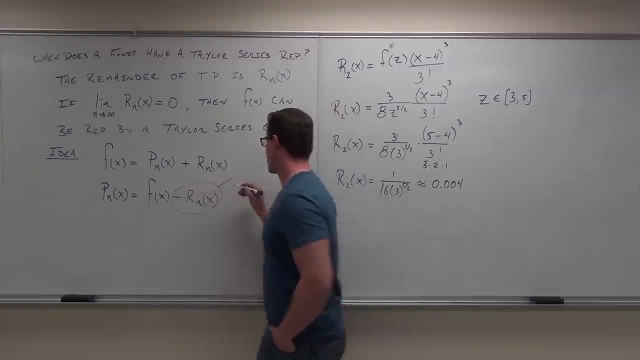 this thing has to go to where? Zero, Zero. Yeah, this has to go to zero, as n approaches infinity. What that means, though, please, please, notice this: What that means: if n goes to infinity, your Taylor polynomial becomes a Taylor series, because it's going to infinity. 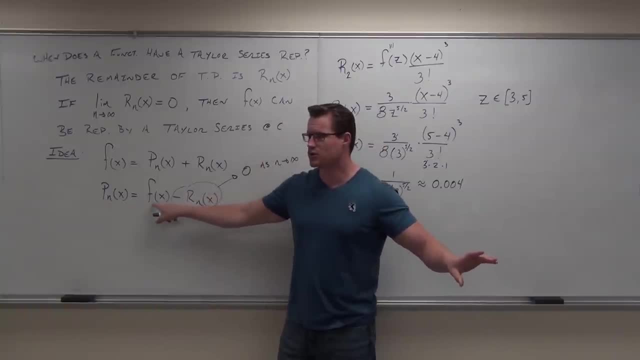 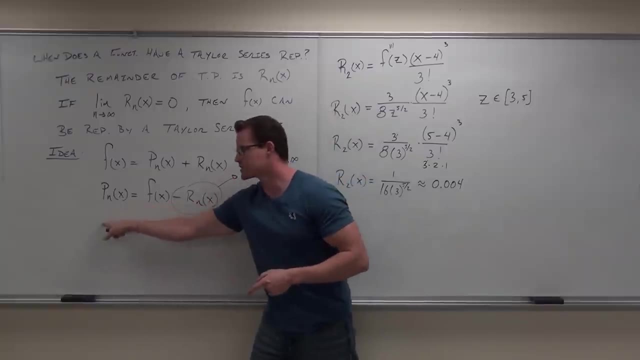 I'm not saying a Taylor polynomial equals the function. What I'm saying is that if I go to infinity, the Taylor polynomial goes to a Taylor series, and if this goes to zero, the Taylor series equals the function. And that's what I'm trying to say. 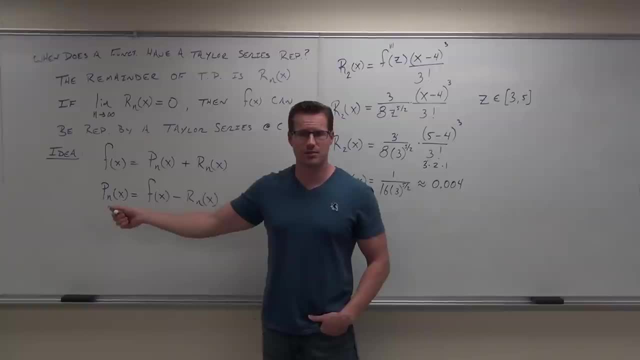 I'm not saying that the polynomial. I'm not saying that the polynomial equals the function. What I'm saying is that as n approaches infinity, as n approaches infinity, the function will be zero. This thing has to go to where Zero. 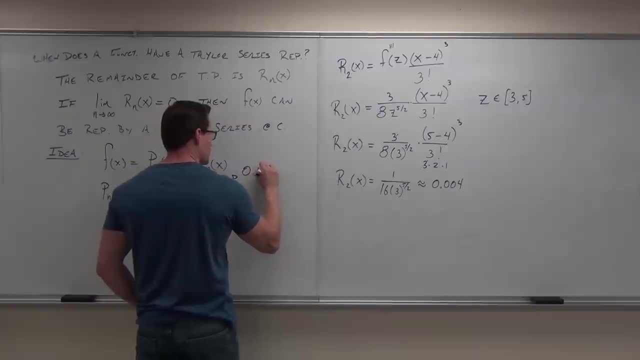 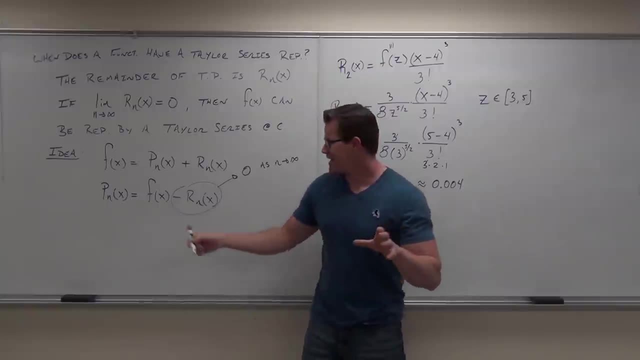 Yeah, this has to go to zero, as n approaches infinity. What that means, though, please, please, notice this. What that means: if n goes to infinity, your Taylor polynomial becomes a Taylor series, because it's going to infinity. I'm not saying a Taylor polynomial equals the function. 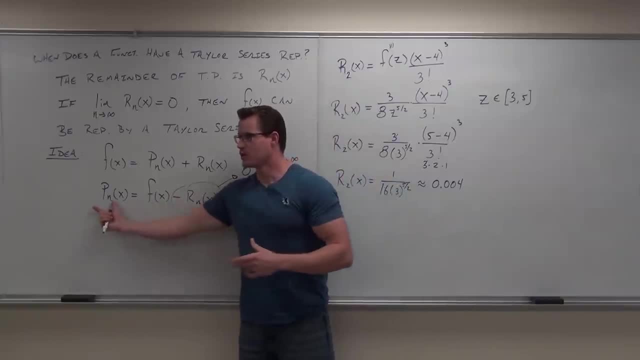 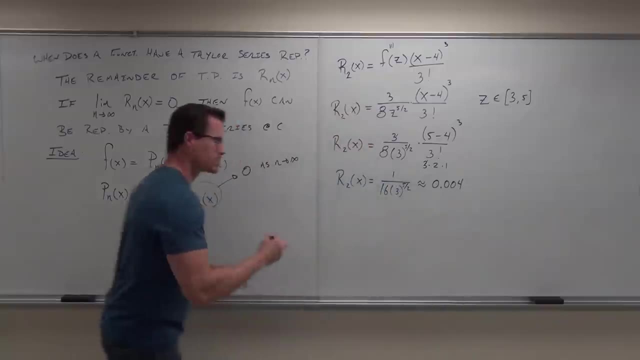 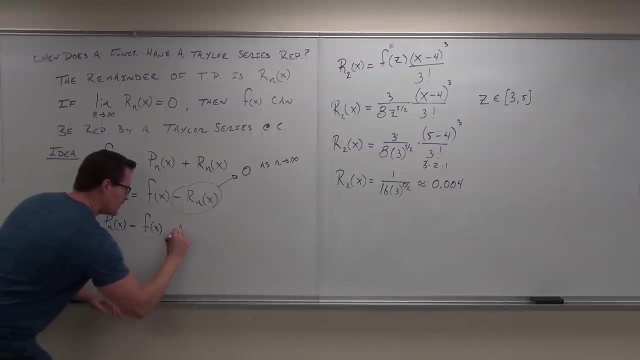 What I'm saying is that if I go to infinity, the Taylor polynomial goes to a Taylor series and if this goes to zero, the Taylor series equals the function, And that's what I'm trying to say. So this right here says that the Taylor polynomial equals our function as n goes to infinity, making this a Taylor series, which would represent perfectly our function. 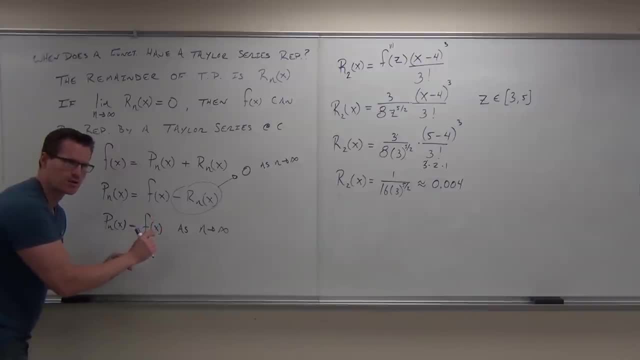 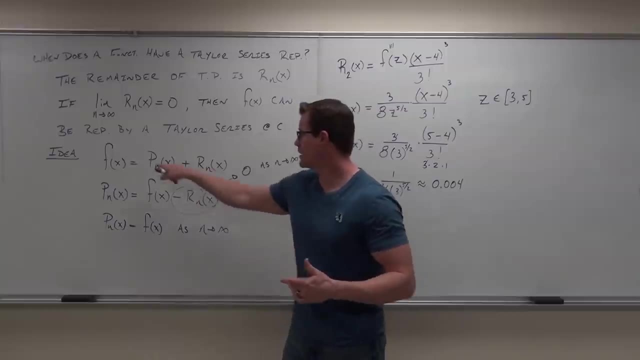 Do you guys see the minute detail I'm talking about here? So this right here, It's obviously not a complete proof, but this idea of the proof, The idea of the proof is: hey, you know what? This is for sure true. 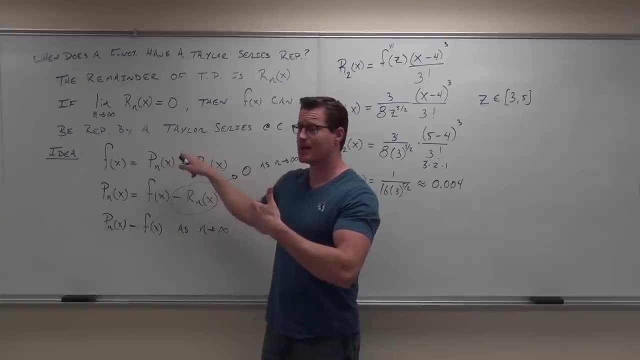 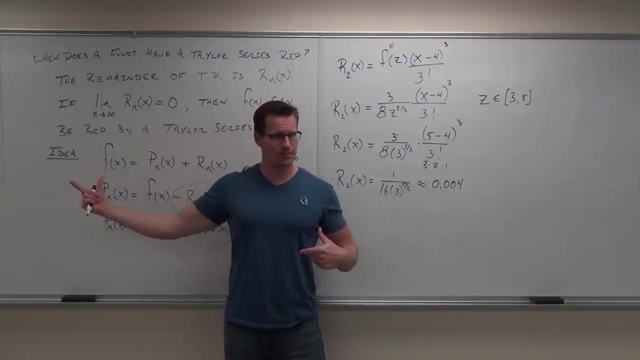 We can represent a function by a Taylor polynomial. If this remainder goes to zero, well then the Taylor polynomial equals the function as n approaches infinity. So if this goes to zero as n approaches infinity, it means n goes to infinity here as well. 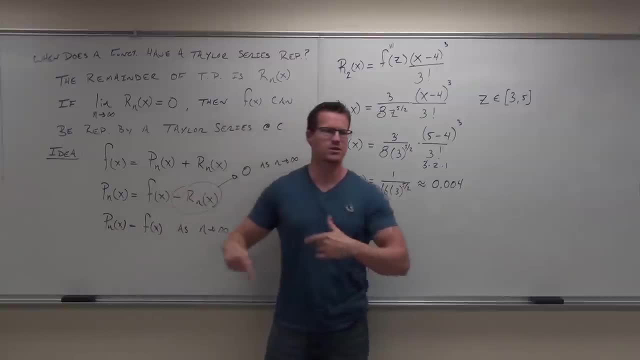 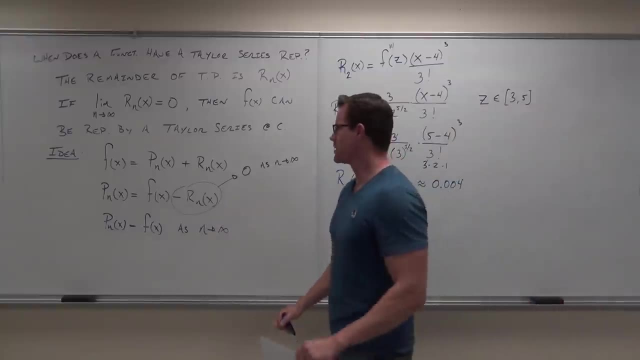 The Taylor polynomial becomes a Taylor series, and the Taylor series represents our function perfectly if the remainder goes to zero. So if you guys feel okay with the proof, Okay, that's the idea. Now there's one more thing that we're going to talk about, which we need here. 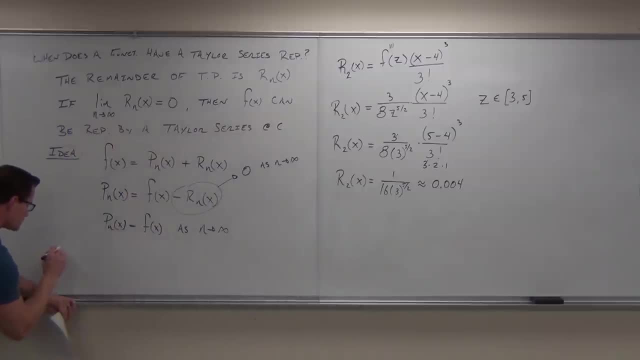 Just a little note. It's this note. You need to know that the limit- because we're going to use this at least twice in the next couple examples- the limit of this thing equals zero. Keep that in your memory banks, because we're going to use it for a little while. 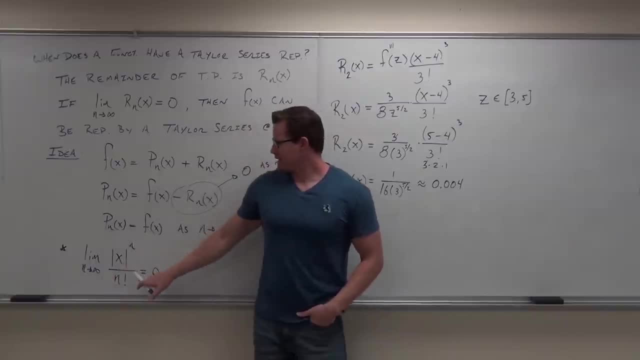 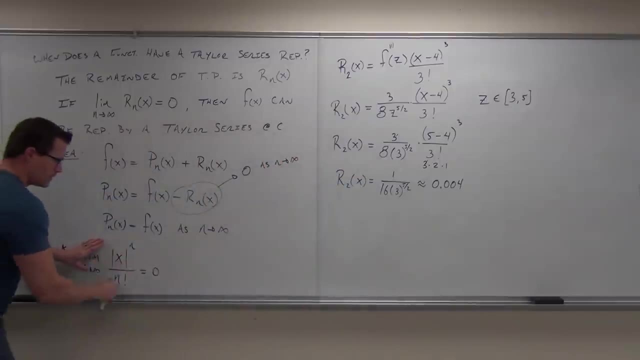 I'll give you kind of the idea here. The idea is- and we've actually seen it before in section 9.8,. the idea is this thing: right here, if you ignore the limit, the series of this converges by stuff in 9.8.. 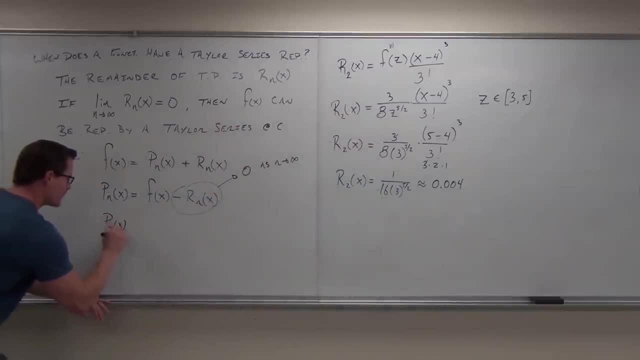 So this right here says that the Taylor polynomial equals our function, as n goes to infinity, making this a Taylor series which would represent perfectly our function. Do you guys see the minute detail I'm talking about here? So this right here is the. it's obviously not a complete proof, but this idea of the proof 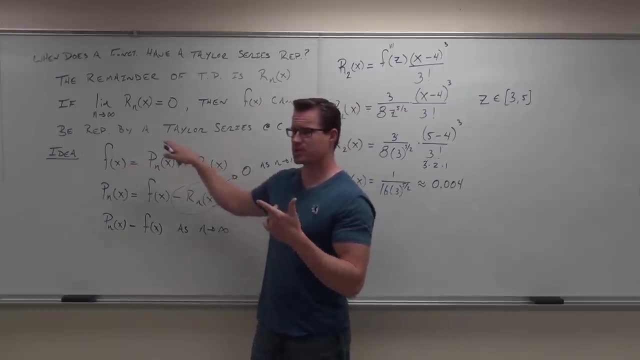 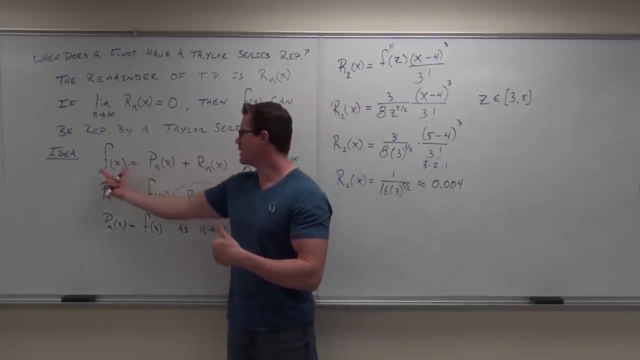 The idea of the proof is: hey, you know what this is for sure. true, We can represent a function by a Taylor polynomial. If this remainder goes to zero, well then the Taylor polynomial equals the function as n approaches infinity. So, if this goes to zero, as n approaches infinity, it means n goes to infinity. 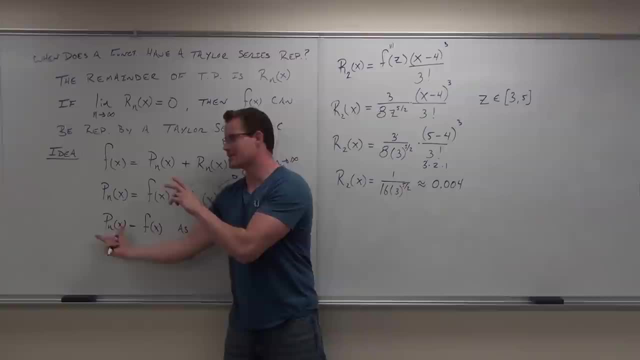 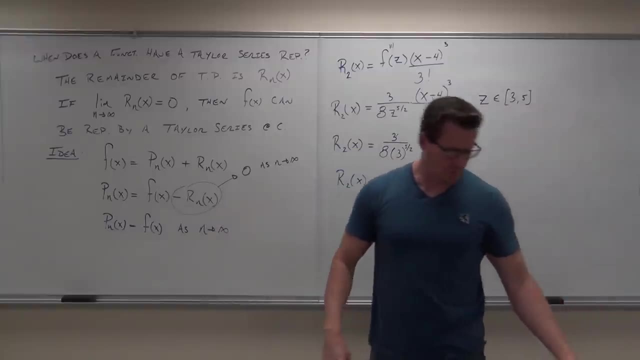 Here as well, the Taylor polynomial becomes a Taylor series, and the Taylor series represents our function perfectly if the remainder goes to zero. So you guys feel okay with the proof. Okay, That's the idea. Now there's one more thing that we're going to talk about, which we need here. 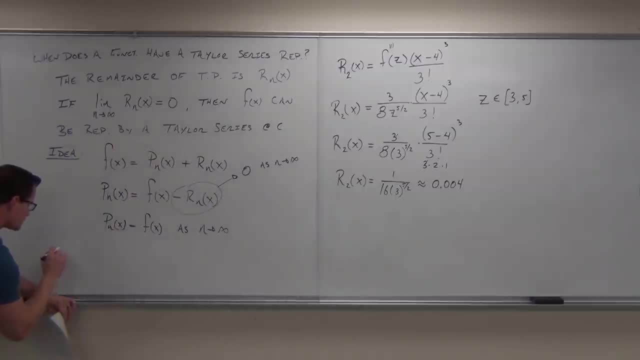 Just a little note. It's this note. You need to know that the limit- because we're going to use this at least twice in the next couple examples- the limit of this thing equals zero. Keep that in your memory banks, because we're going to use it for a little while. 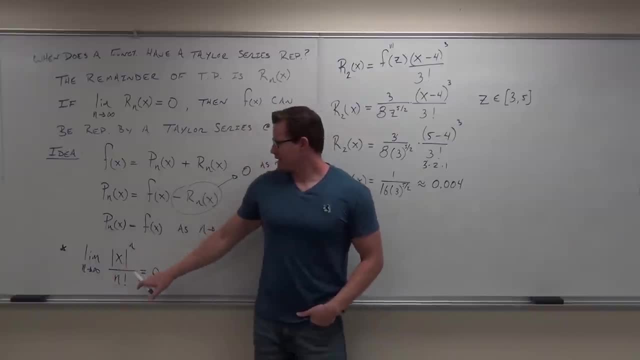 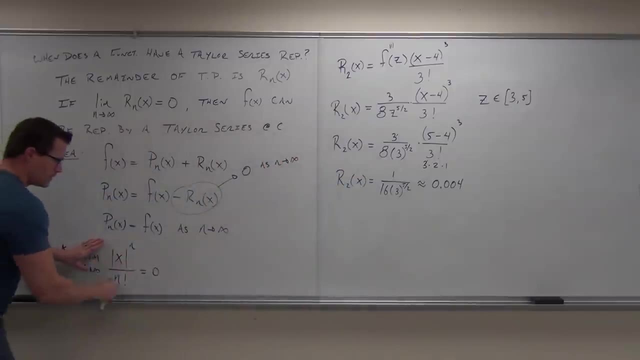 I'll give you kind of the idea here. The idea is- and we've actually seen it before in section 9.8.. The idea is this thing: right here, if you ignore the limit, the series of this converges By stuff in 9.8, you can prove that okay. 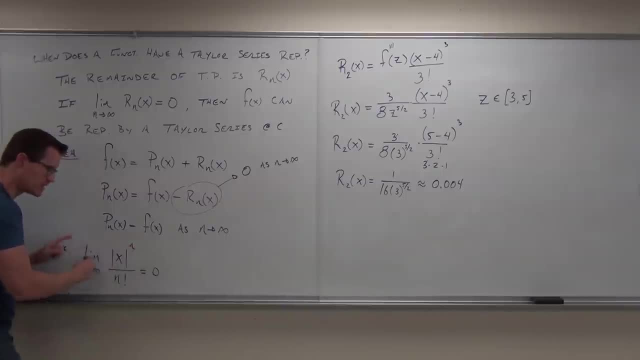 Series of this converges. If the series converges, the limit of the terms of your sequence has to equal zero. That was the divergence test. You remember doing that. If a series converges, the limit of this goes to zero. We actually used it in reverse. 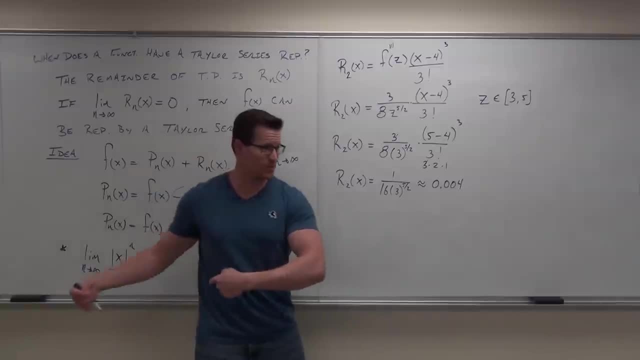 We said: if the limit is zero, well it might converge, Because if it doesn't equal zero, there's no way it converges. You remember that one. You probably used that in some of your homework. So basically it's from section 9.8.. 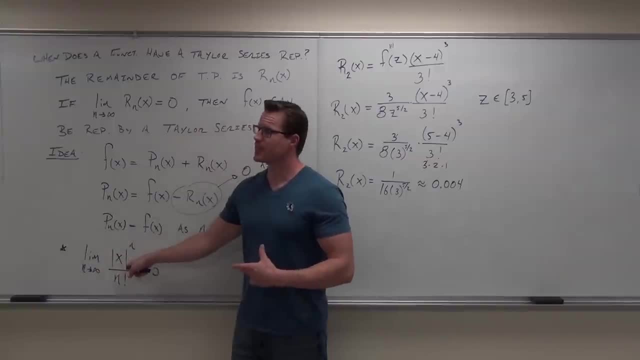 Since this is a convergent series, the limit of the terms of the sequence from which that series is built has to give you zero. We're going to use that in a little bit. Would you guys like to see some examples of why we just learned all this stuff? 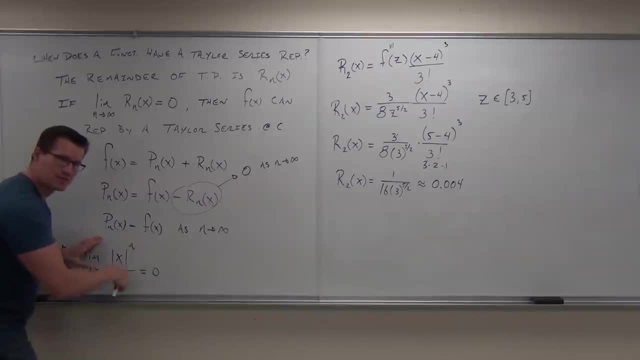 You can prove that. okay. Series of this converges. If the series converges, the limit of the terms of your sequence has to equal zero. That was the divergence test. Remember doing that. If a series converges, the limit of this goes to zero. 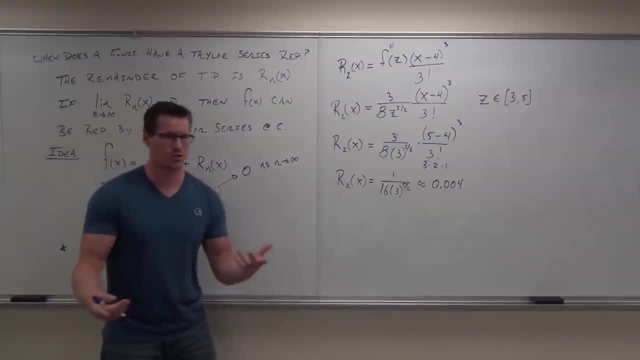 We actually used it in reverse. We said, if the limit is zero, well, it might converge, Because if it doesn't, it doesn't. If it doesn't equal zero, there's no way it converges. Remember that one. You probably used that in some of your homework. 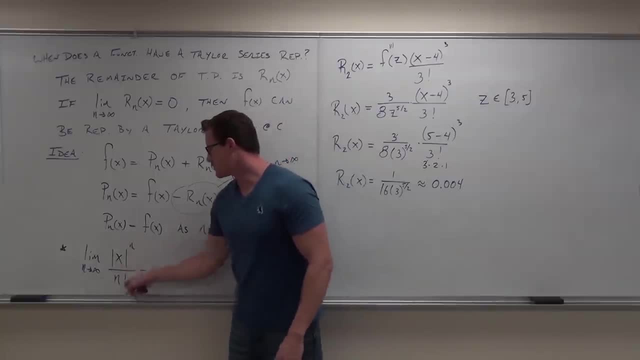 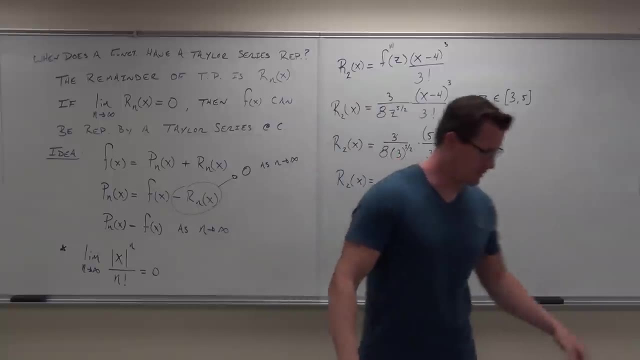 So basically it's from section 9.8.. Since this is a convergent series, the limit of the terms of the sequence from which that series is built has to give you zero. We're going to use that in a little bit. 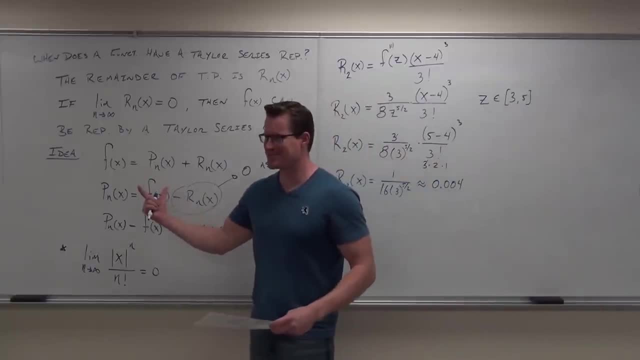 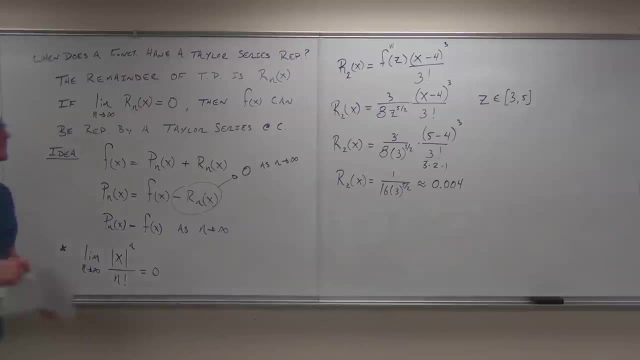 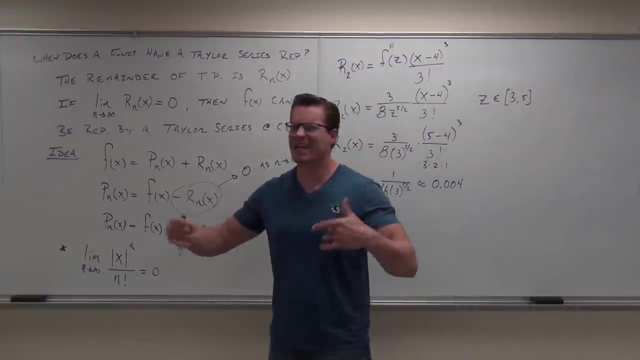 Would you guys like to see some examples of why we just learned all this stuff? Okay, so the idea is now that we know, now that we know when a function can be represented by a Taylor series, when can it, when can. let's see if you, if you even were paying attention, 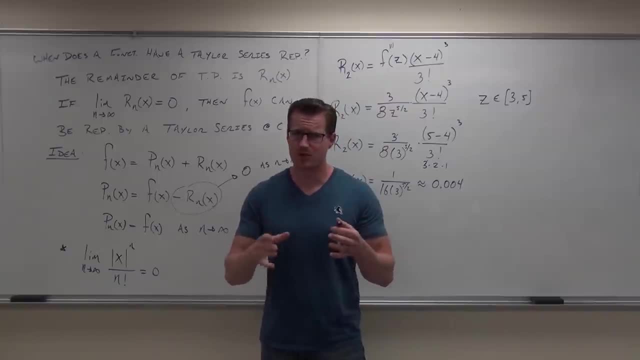 if you even kind of grasped this, when can a function be represented by a Taylor series? When the remainder, when the limit of the remainder. there you go, that's when. So if we can prove that, then we can prove that a function can be represented by a Taylor. 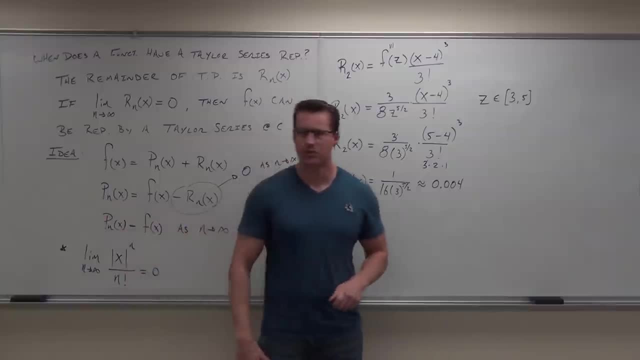 series, And that's what we're going to be doing right now. We're going to be using this in some of the examples, So let's, let's do a couple of them, just to get our brains wrapped around it. Are there any questions? 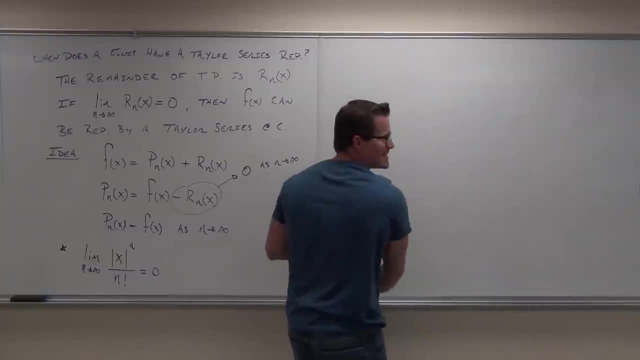 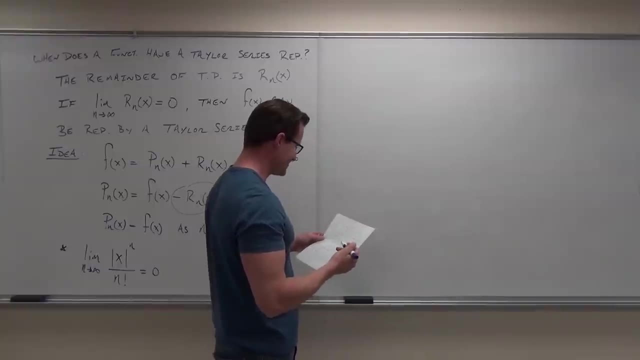 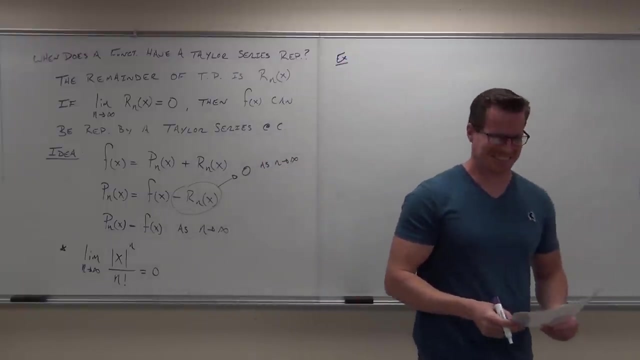 Any questions before I continue? Before we continue, We're like a team, like a math team, but I'm the quarterback, like Peyton Manning, except not during the Super Bowl, Not this Super Bowl, the one from. was it 2006 or 2008?? 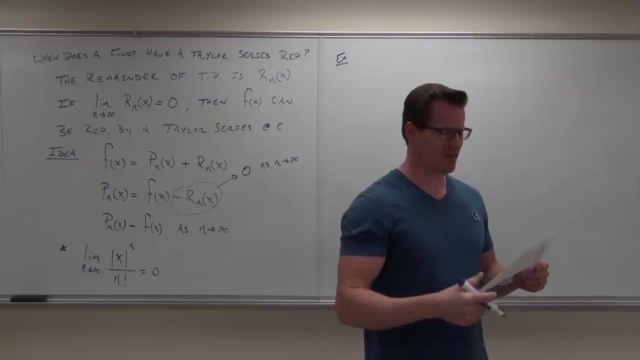 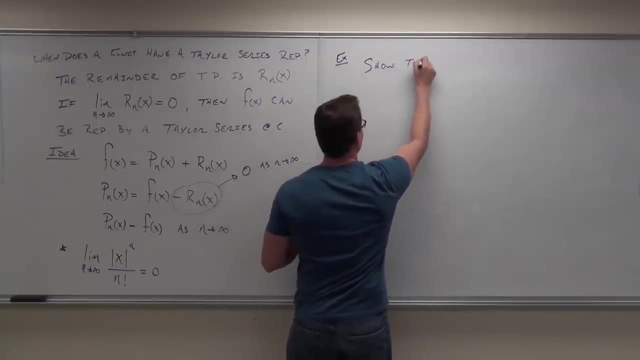 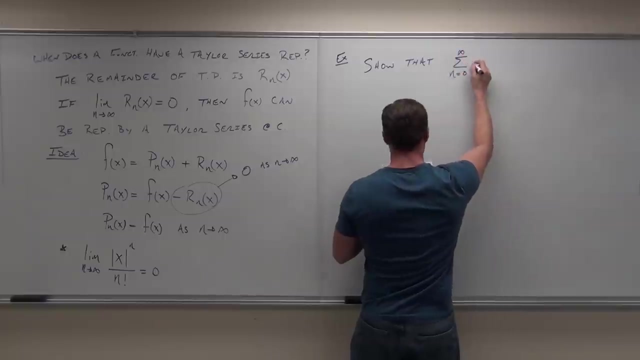 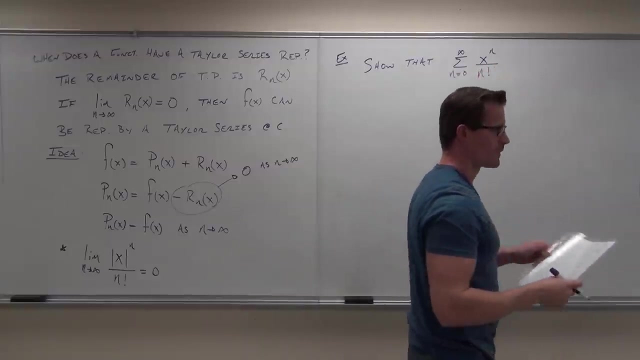 Which one did he win? The sixth. The sixth Was that long ago, That poor man. Okay, So here's what we're going to do. I want to show that this. What is that? Zero, No, No. What is this? 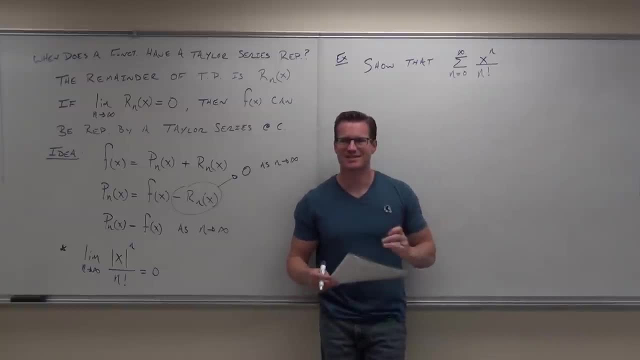 Series, Series. What kind of series? Yeah, Power series, Yeah, Yeah, Yeah, It is Specifically. I can tell you what test we can use. What series? is it Taylor series or Maclaurin series? Oh, Maclaurin. 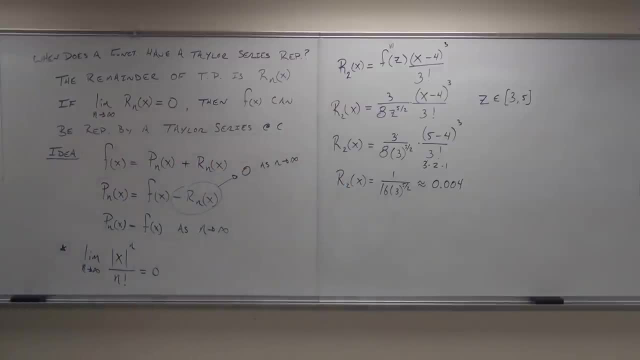 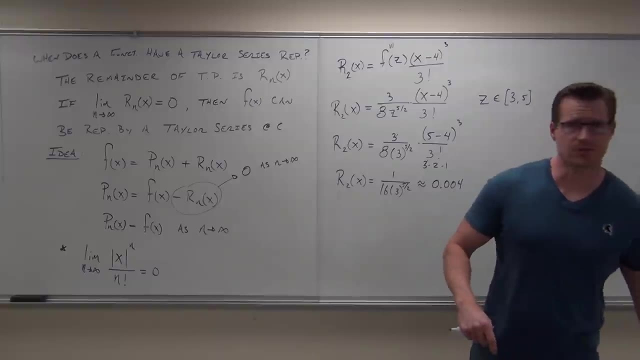 Okay, So the idea is this. The idea is this. The idea is this. The idea is now that we know, now that we know when a function can be represented by a Taylor series, when can it, when can? let's see if you even were paying attention. 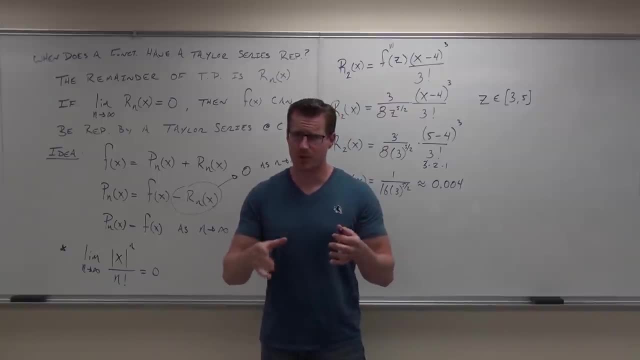 or, if you even kind of grasped this, When can a function be represented by a Taylor series? When the remainder, When the limit of the remainder. There you go, That's when. So if we can prove that, then we can prove that a function can be represented by a Taylor series. 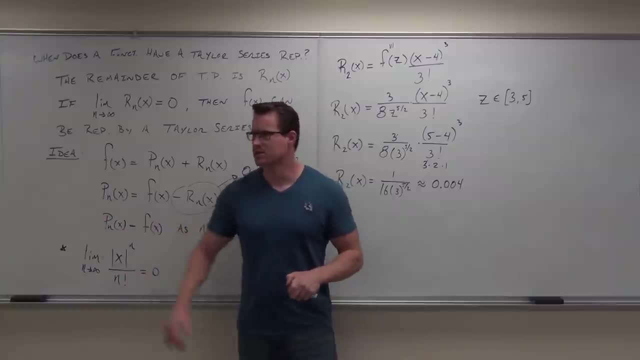 And that's what we're going to be doing right now. We're going to be using this as some of the examples, So let's do a couple of them, just to get our brains wrapped around it. Are there any questions? before I continue? 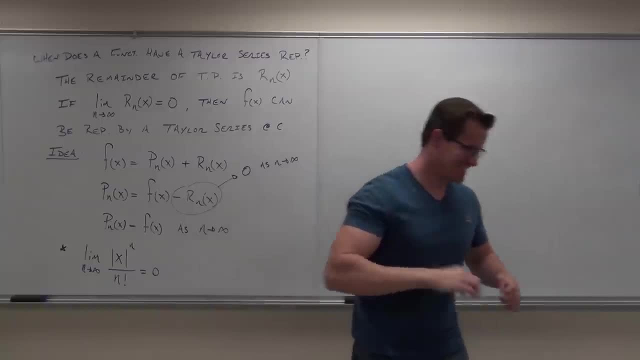 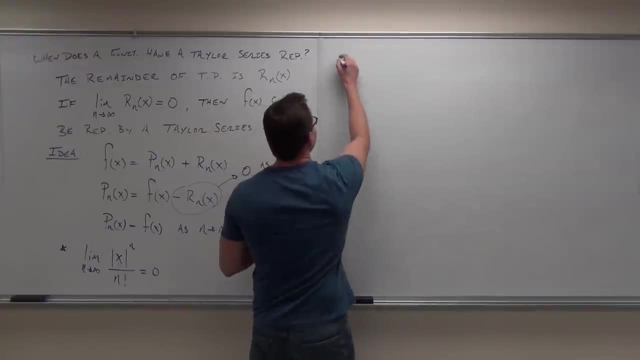 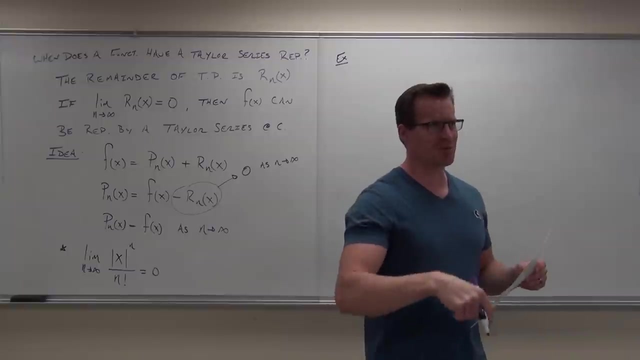 Before we continue, We're like a team, like a math team, But I'm the quarterback, Like Peyton Manning, Except not during the Super Bowl, Not this Super Bowl, The one from. was it 2006? Or 2008?? 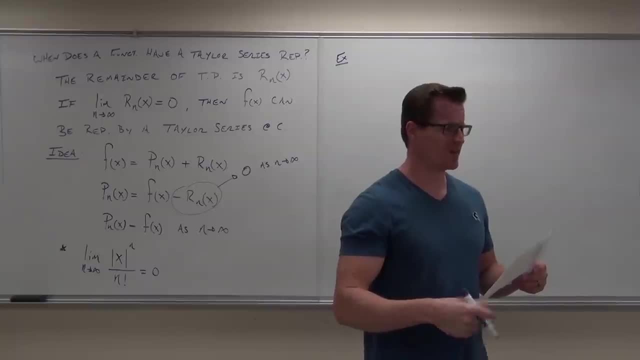 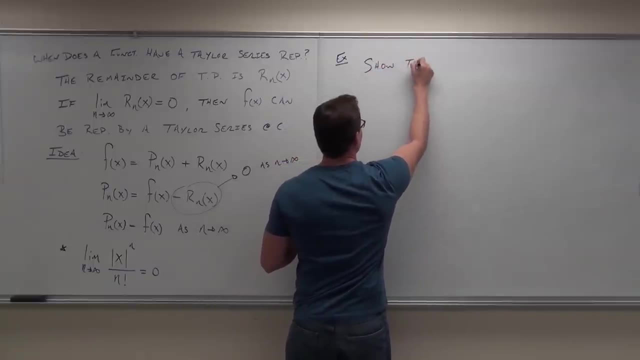 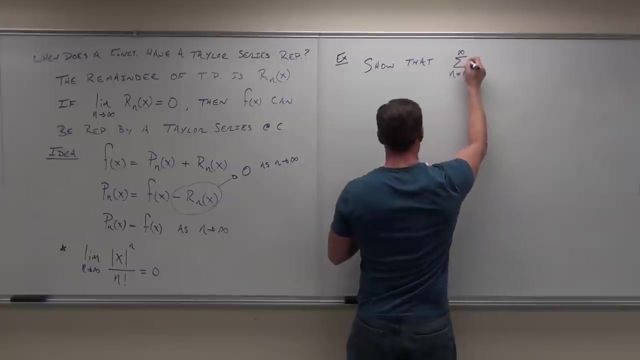 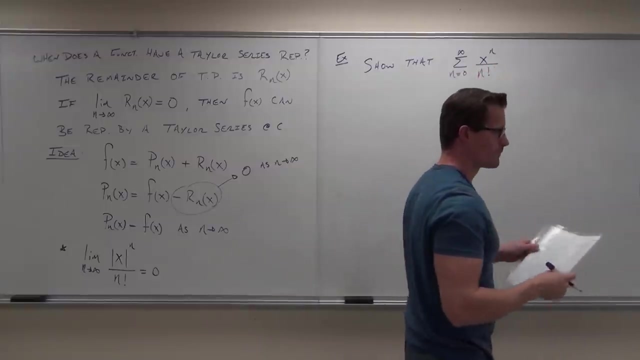 Which one did he win? I don't remember. It was six, Was that long ago? That poor man. Okay, So here's what we're going to do. I want to show that this. what is that? Zero, Zero. 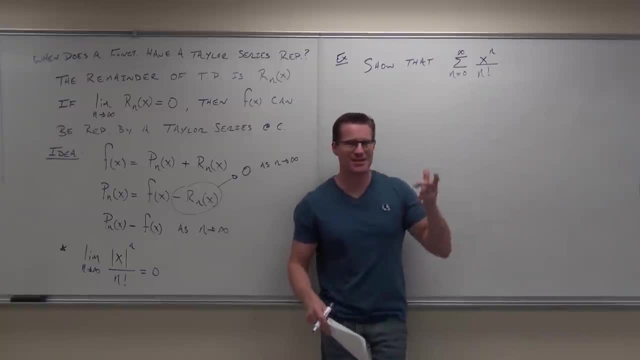 Zero. No, what is this? It's a series, A series. What kind of series? A Kind of- yeah it is specifically. I can tell you what test we do. I wouldn't want that. What series is it? 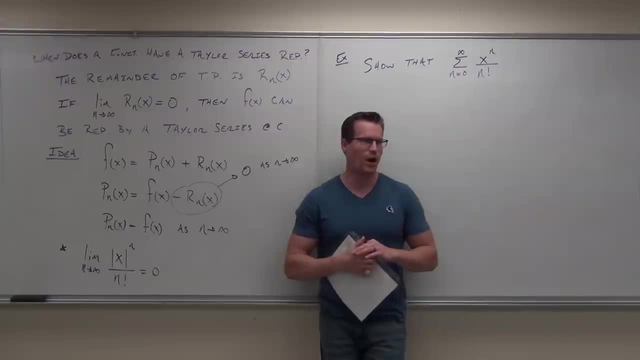 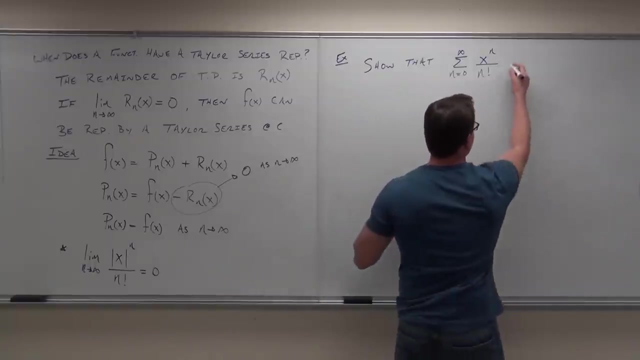 Taylor series or McLaurin series. Oh, McLaurin, Why McLaurin series? Is that also a Taylor Series? Yes, Yes, a Taylor Series. So Taylor series. OK, What I want to show is that this Maclaurin series of this, this Taylor series of the function e to the x. 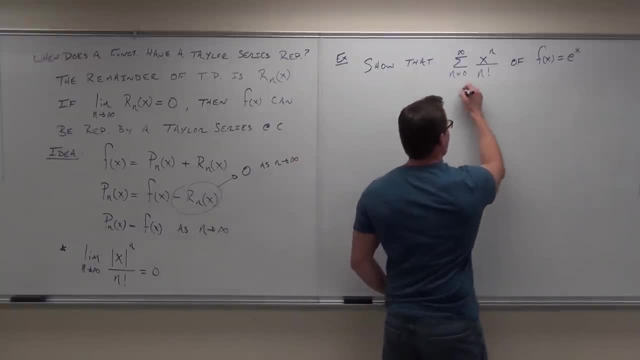 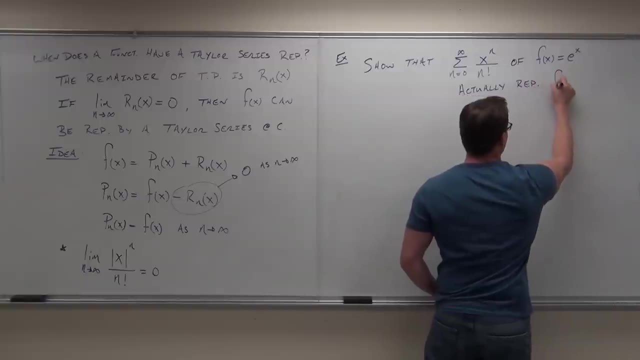 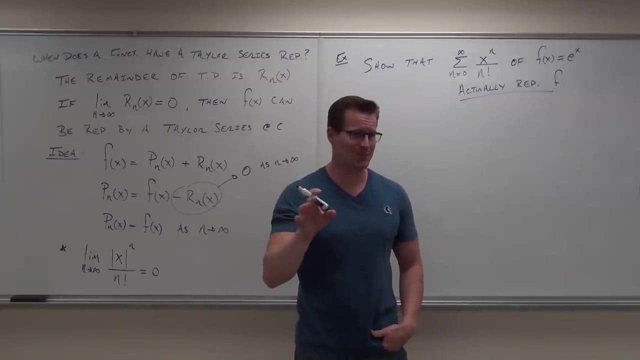 I want to show that the Taylor series, or Maclaurin series, of this function actually represents the function. I know that sounds weird because some of you said what? What are you talking about? I know it's weird, it's a weirded word, it's worded weird, but what it means is prove it. 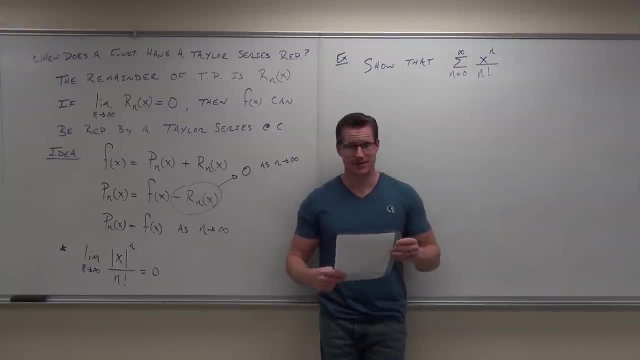 Why The incisors? Ah, good, Maclaurin series. Is that also a Taylor series? Yes, Yes, Taylor series. So Taylor series, Maclaurin series. What I want to show is that this Maclaurin series actually represents. sorry of this. 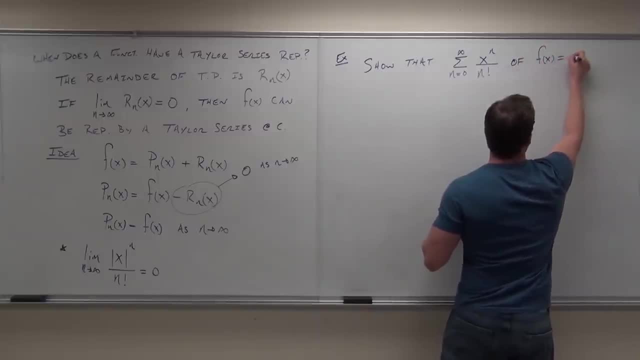 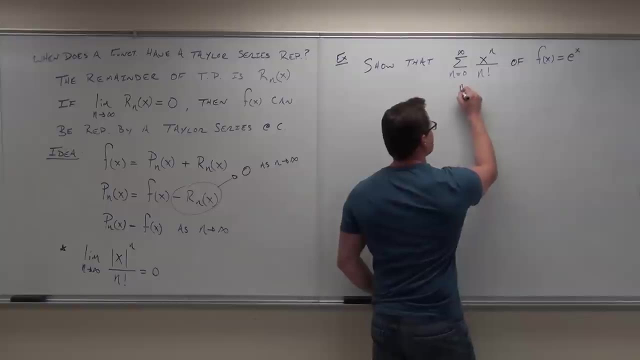 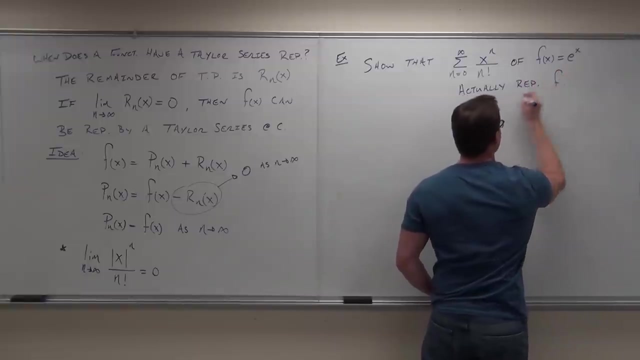 this Taylor series of the function e to the x. I want to show that the Taylor series or Maclaurin series of this function actually represents the function. I know that sounds weird because some of you said what? Yeah, Oh, it's weirded. 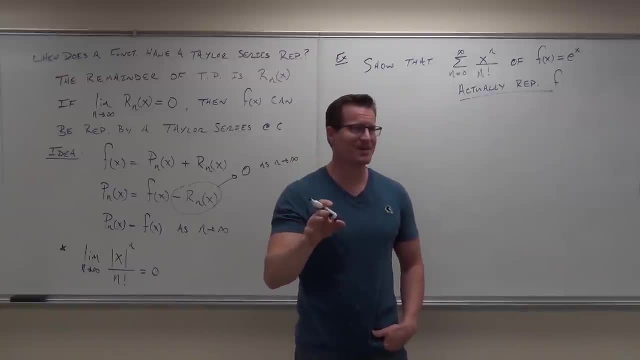 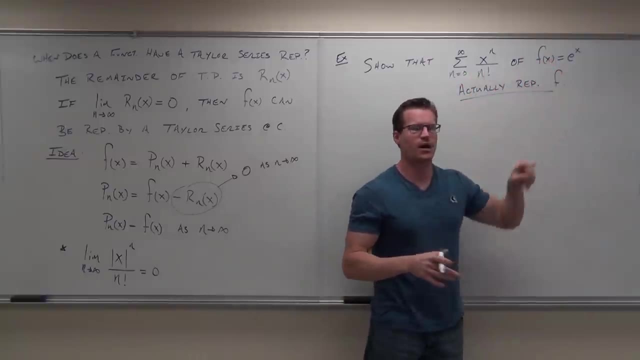 What are we talking about? I know it's weird, It's a weirded word, It's worded weird, But what it means is: prove it, Prove that this, Prove that this actually represents this. Now, please do not reinvent the wheel on these problems. 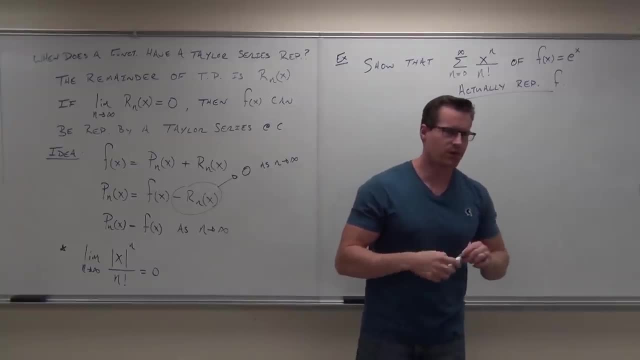 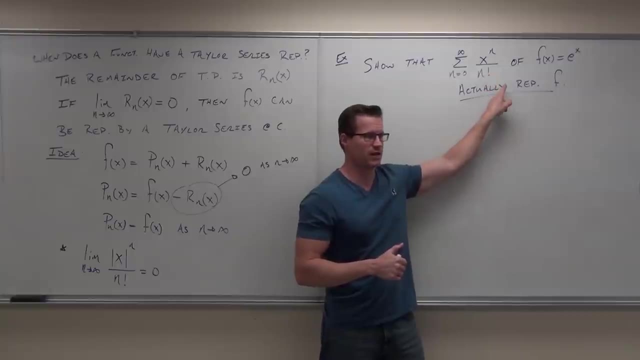 Here's what this is saying. Let me kind of break it down to you. Remember that this thing, if you look back in your notes, you're going to see this. In fact, you're going to see that this equals this back in your section. whatever you did, 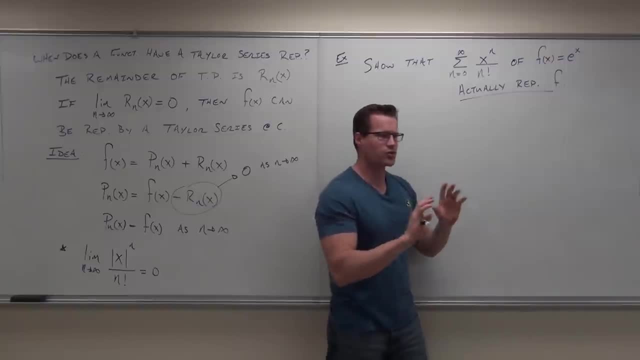 with your Taylor series. Maclaurin series- with your Maclaurin series. We're not trying to prove that this is this again, It's already shown that this is this. What we're trying to do is Prove that it actually represents it on your Taylor series. 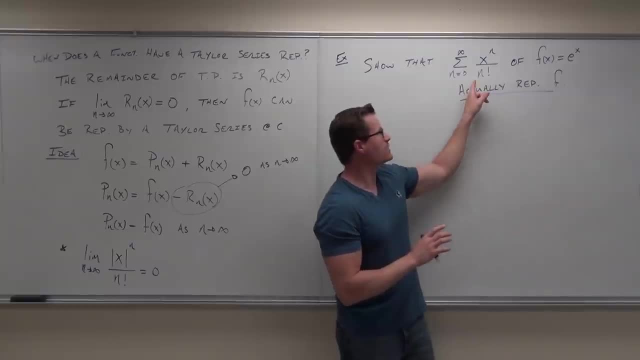 So let me say that one more time. It's already been determined that these two things are equal. What we're trying to do is prove it by showing that the remainder, the limit of the remainder, is what Zero. It's all you're trying to show here. 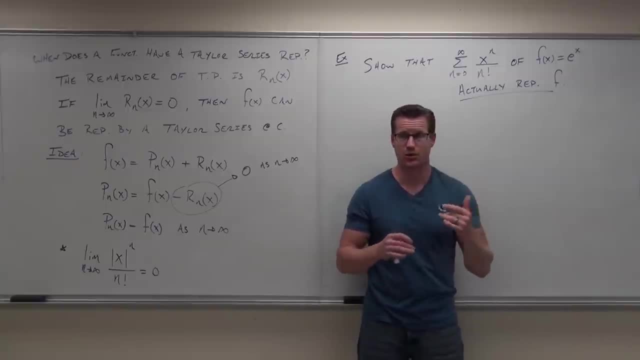 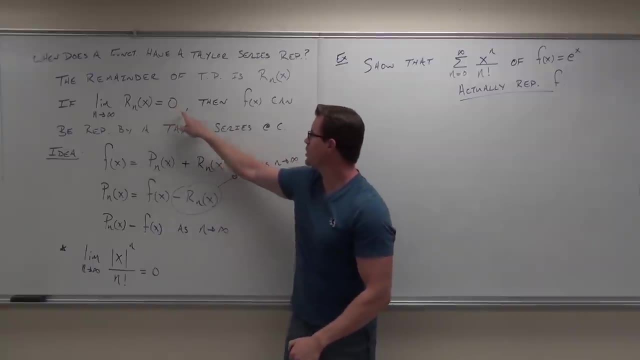 You're trying to show that the limit of the remainder is equal to zero. If you do that, If you show that the limit of the remainder is equal to zero, then you show that your function can be represented by the Taylor series That you were given at C, which happens to be zero here for a Maclaurin series. 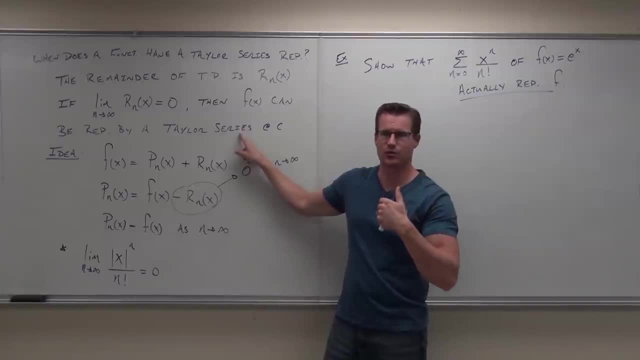 Do you want me to say that one more time? You sure You can rewind it, So it's going to be the exact same words. Okay, so ultimately, again, the idea is: look it, you're not trying to prove that this equals. 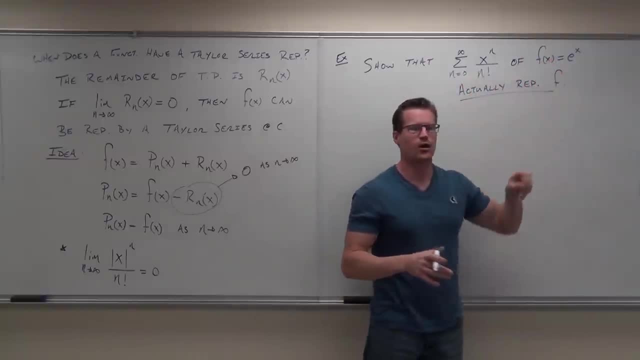 Prove that this actually represents this. Now, please do not reinvent the wheel on these problems. Here's what this is saying. let me kind of break it down to you. Remember that this thing. if you look back in your notes, you're going to see this. 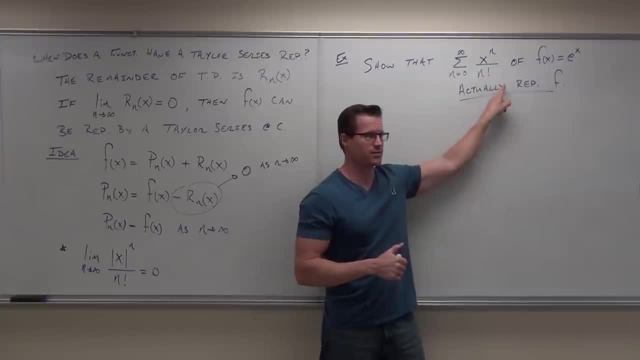 In fact, you're going to see that this equals this back in your section, whatever you did with your Taylor series, Maclaurin series. We're not trying to prove that this is this again. it's already shown that this is this. 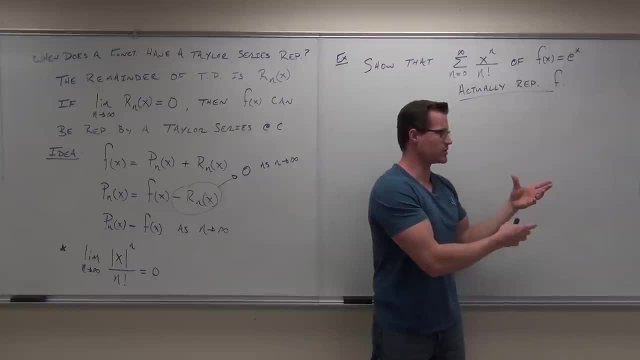 What we're trying to do is prove that it actually represents it on your Taylor series. So let me say that one more time. It's already been determined that these two things are equal. What we're trying to do is prove it by showing that the remainder, the limit of the remainder, is what 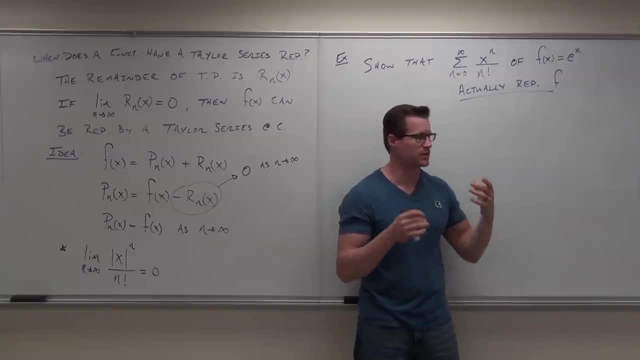 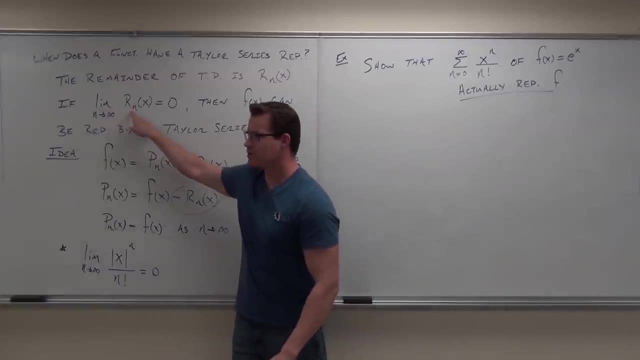 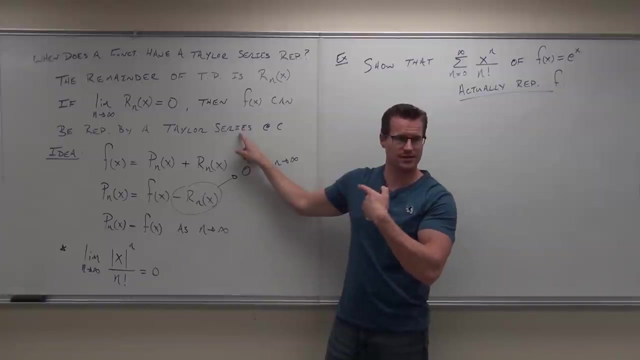 Zero. It's all you're trying to show here. You're trying to show that the limit of the remainder is equal to zero. If you do that, If you show that the limit of the remainder is equal to zero, then you show that your function can be represented by the Taylor series that you were given at C, which happens to be zero here for a Maclaurin series. 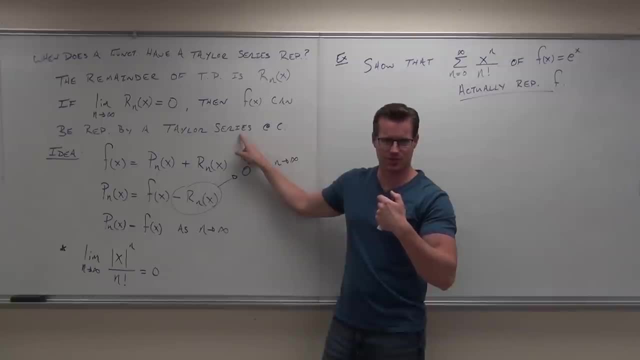 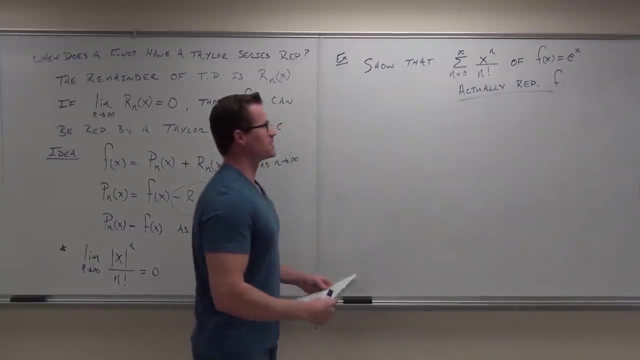 Do I need to say that one more time? You sure You can rewind it, So it's going to be the exact same words. Okay, so ultimately, again, the idea is: look, you're not trying to prove that this equals this by reinventing it. you're trying to prove this equals this by just simply showing that this is what this is. 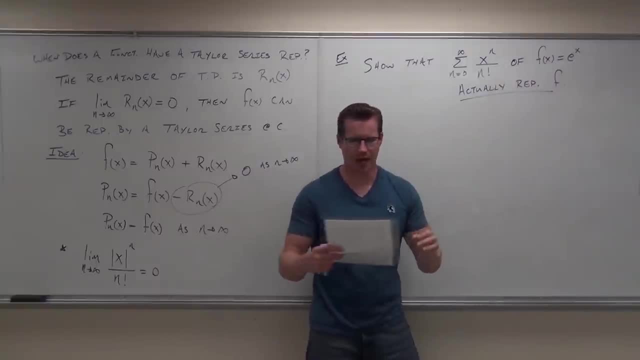 You're trying to prove that this equals this by reinventing it. You're trying to prove this equals this by just simply showing that this is what this is. You're just showing that the remainder equals zero. That's it okay. So how we go about doing that is very similar to building the Taylor series again. 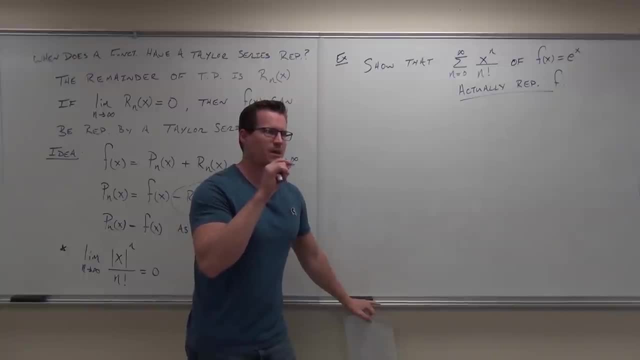 It's just you're trying to find out what the remainder is going to look like in terms of the function itself. So let me show you what I'm talking about. What we're trying to do is this: I want you to show me what this. 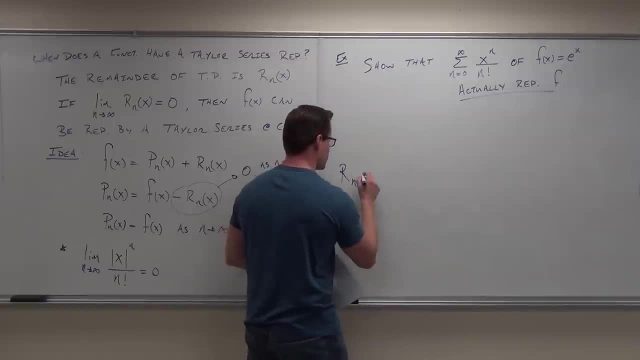 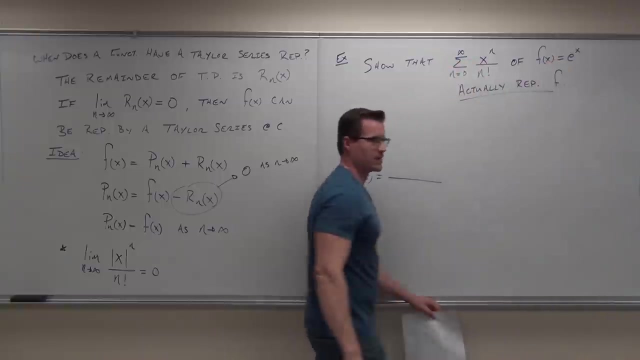 I want you to show me what this piece is. If we can prove that the limit of this piece goes to zero, then we prove that this representation is representing that function perfectly. That's what we're trying to show. Okay, now here's how we do it. 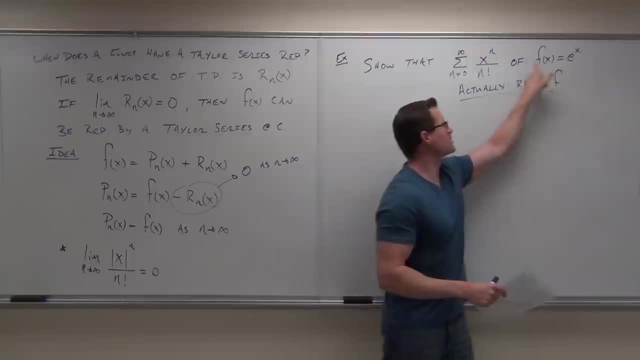 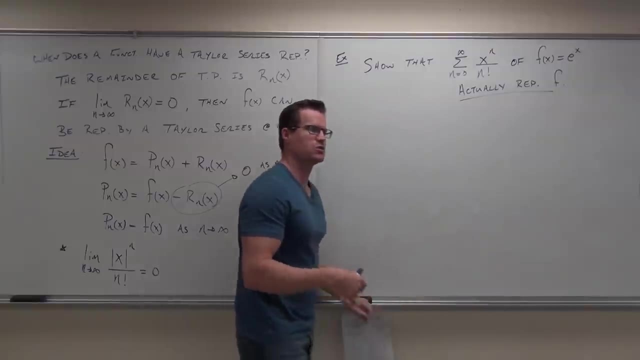 this by reinventing it. You're trying to prove this equals this by just simply showing that the remainder equals zero. That's it Okay. So how we go about doing that is very similar to building the Taylor series. You're trying to prove this equals this by just simply showing that the remainder equals. 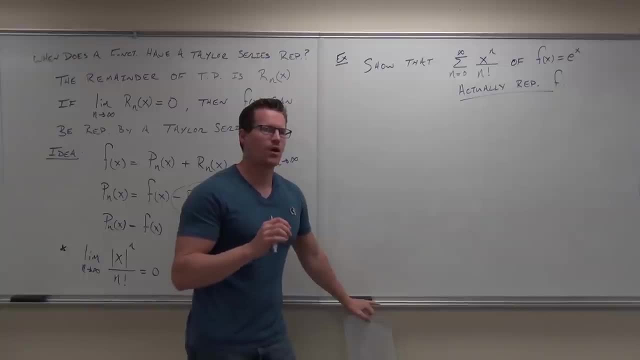 zero, Okay. So how we go about doing that is very similar to building the Taylor series. Again, it's just you're trying to find out what the remainder is going to look like in terms of the function itself. So let me show you what I'm talking about. 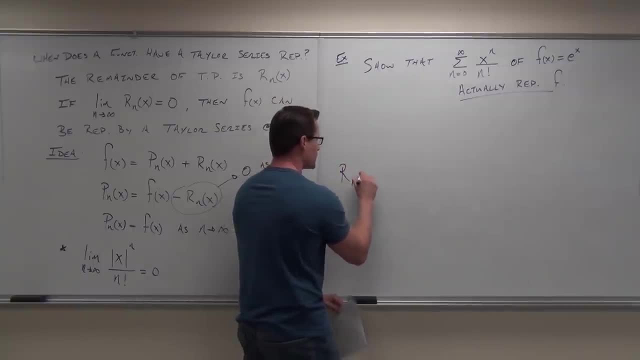 What we're trying to do is this: I want you to show me what this, I want you to show me what this piece is. If we can prove that the limit of this piece goes to zero, Then we prove that this representation is representing that function perfectly. 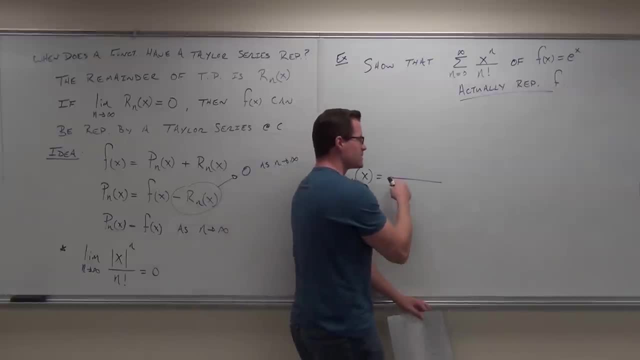 That's what we're trying to show. Okay, now here's how we do it. We, piece by piece, fill this formula out. Now some of it's really really easy. Some of it says: okay, well, remember that our remainder is always like this: 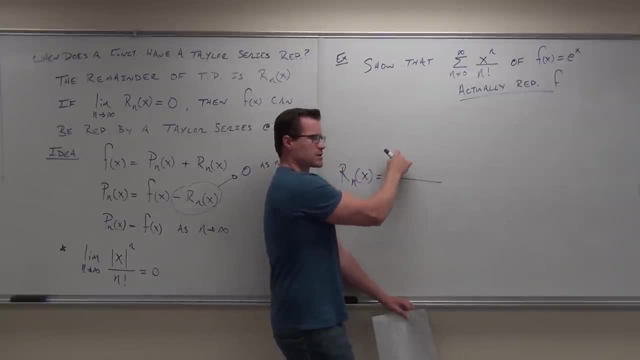 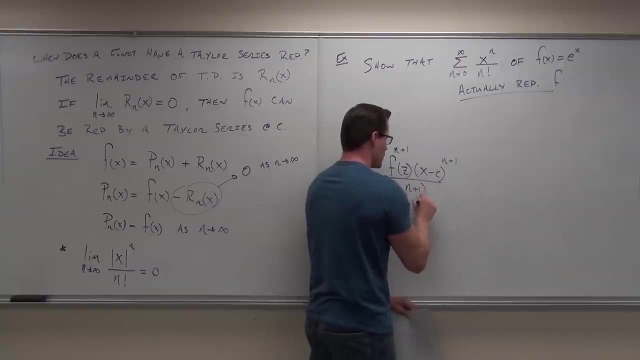 It's always the. if that's n, what's this No, for our remainder, that's n, And this is z, And this is x minus c to the n plus 1, and this is n plus 1 factorial. 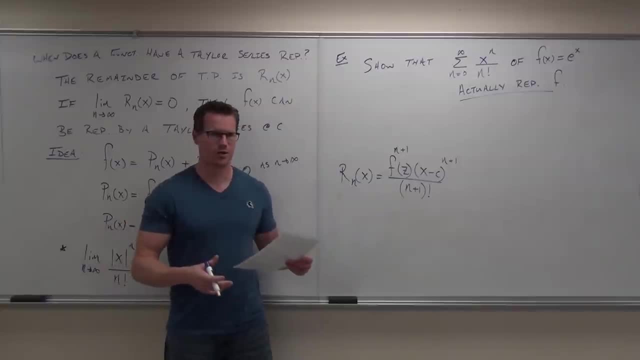 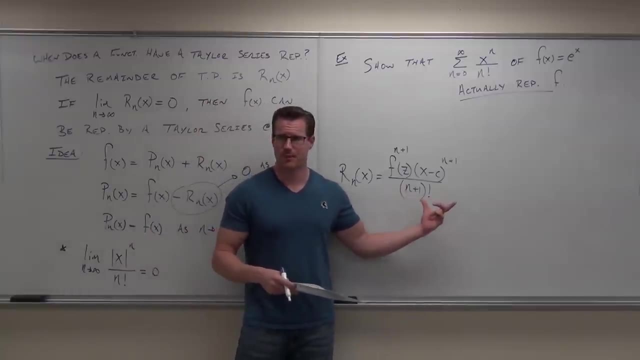 This should be no surprise. This is the definition of what the remainder of a Taylor polynomial is. You guys with me on this one? I can't afford to lose you now. okay, This should be old stuff for us, Are you okay with it? 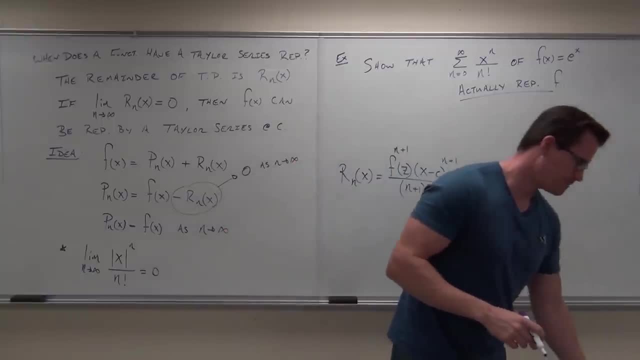 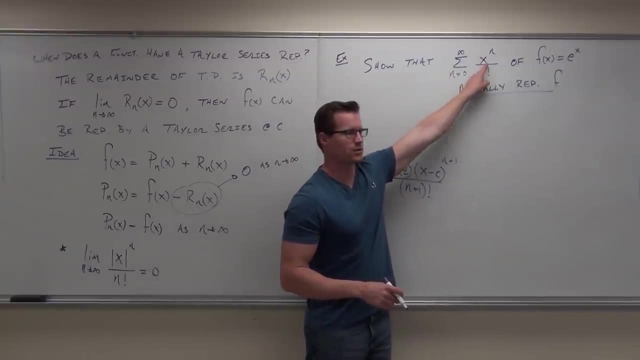 Mm-hmm. Now, some of this stuff's going to be really easy. You see, some of this stuff is well. look up here: What's your center? Good, What's your c? So this piece we can take care of. 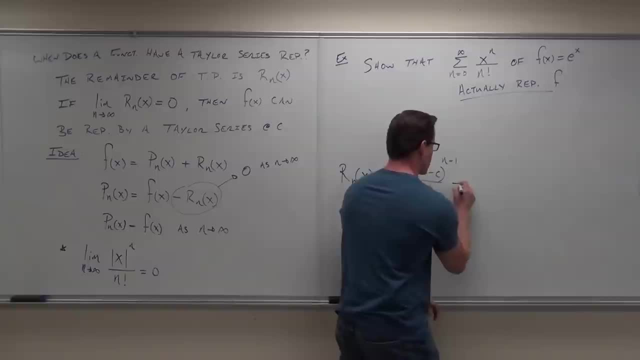 So this goes okay. well, this is the same thing as something. This will be x to the n plus 1.. Do you understand why I got rid of my c here? Yes, The center's 0. Therefore, I don't even need a c. 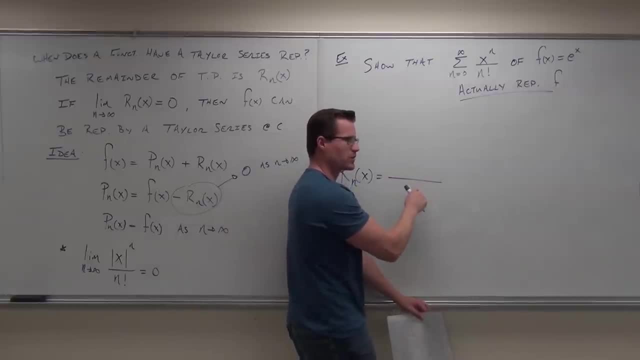 We, piece by piece, fill this formula out. Now some of it's really really easy. Some of it says: okay, well, remember that our remainder is always like this: It's always the if that's n, what's this? 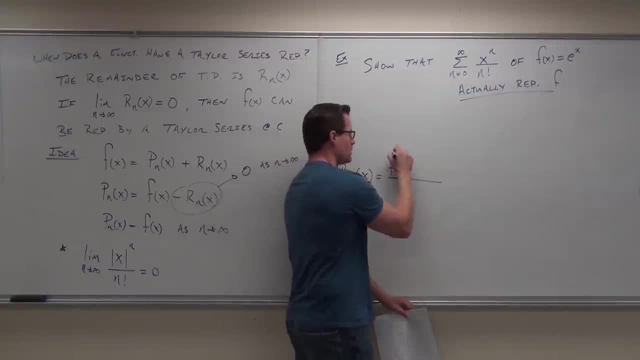 No for remainders. that's n, This is and this is z, And this is x minus c to the n plus 1, and this is n plus 1 factorial. This should be no surprise. This is the definition of what the remainder of a Taylor polynomial is. 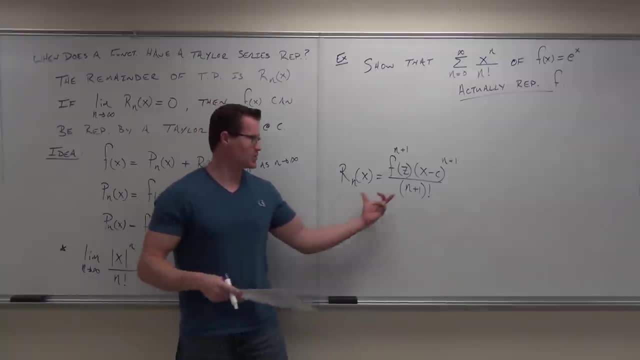 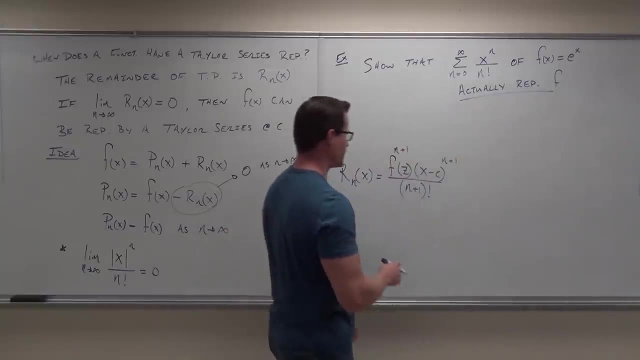 You guys with me on this one. I can't afford to lose you now. okay, This should be old stuff for us, Are you okay with it? Now, some of this stuff's going to be really easy. You see, some of this stuff is well. look up here. 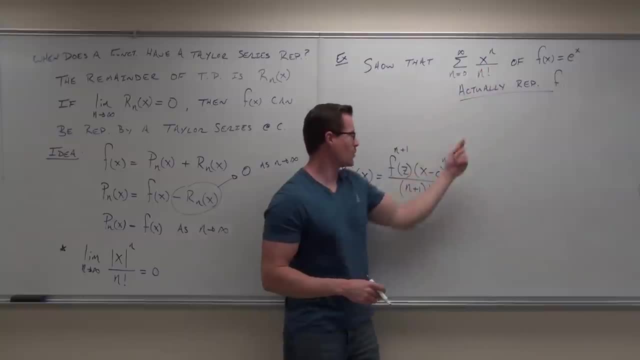 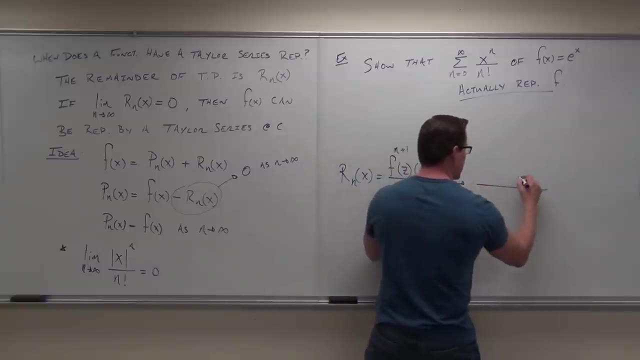 What's your center? Good, What's your c? So this piece we can take care of. So this goes okay. well, this is the same thing as something. This will be x to the n plus 1.. Do you understand why I got rid of my c here? 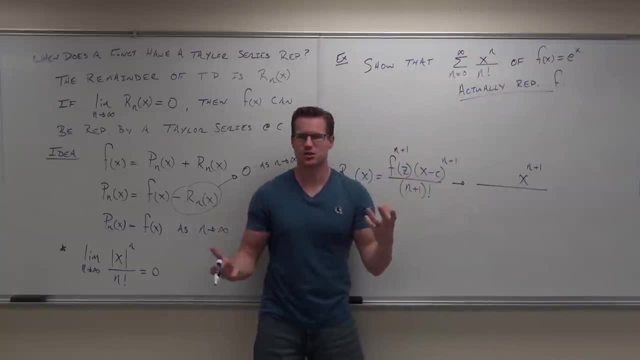 The center is zero. Therefore I don't even need a c, It's just x. Not sure you have to be okay with that one n plus 1 factorial. well, that's going to be there, no matter what. n plus 1 factorial. 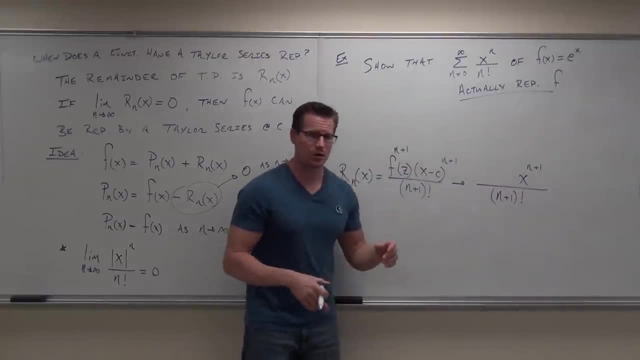 We don't need to change that Now. our goal is to find out how much this is, to find out what the n plus 1 derivative of f at z is. So we're going to do that, But when we start with it is, we start taking derivatives and find the pattern for it. 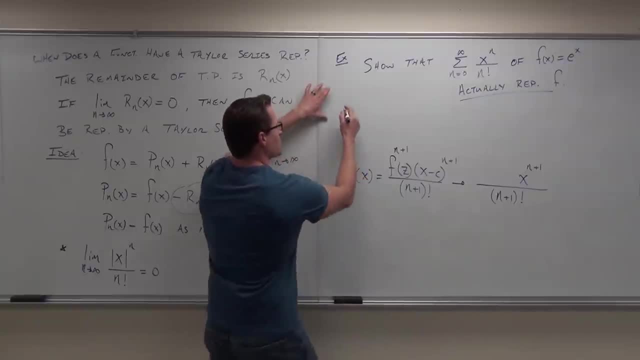 Hey, that sounds familiar, doesn't it? You've done stuff like that before, So let's start with the function f. f of x equals e to the x is going to be an easy one. You're going to like this. 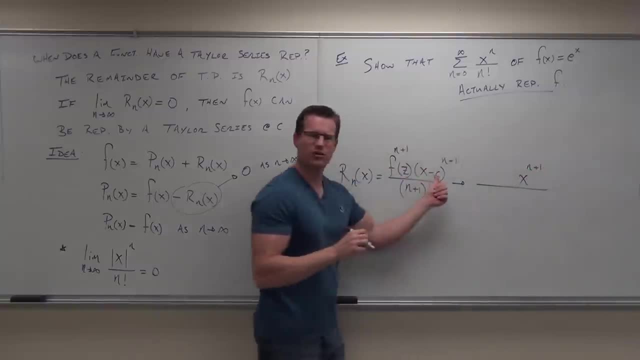 It's just x. Now you have to be okay with that one. n plus 1 factorial. well, that's going to be there, no matter what. n plus 1 factorial. We don't need to change that Now. our goal is to find the denominator. 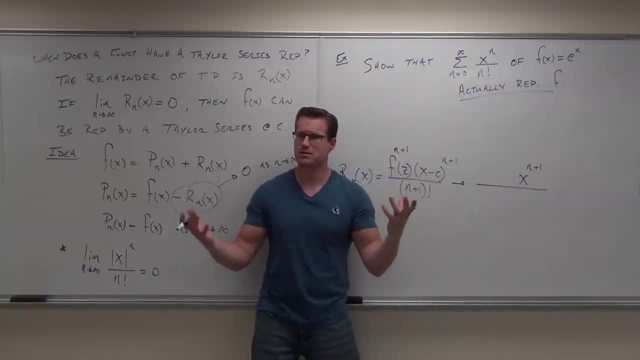 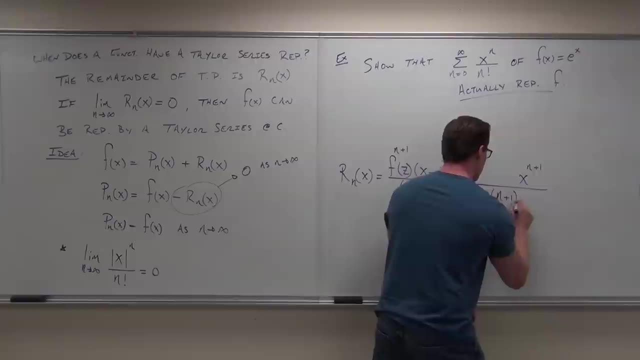 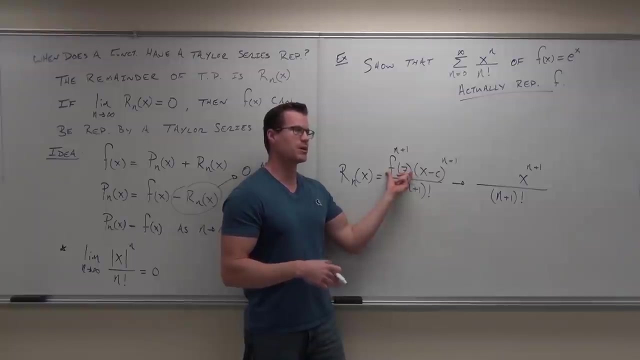 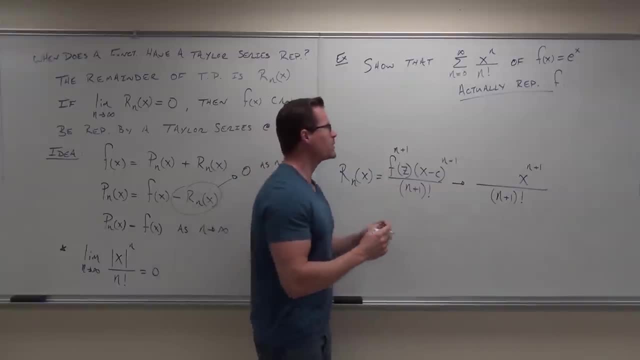 of f at z is. So we're going to do that, And where we start with it is we start taking derivatives and find the pattern for it. Hey, that sounds familiar, doesn't it? We've done stuff like that before, So let's start with the function f. f of x equals e to the x is going to be an easy one. 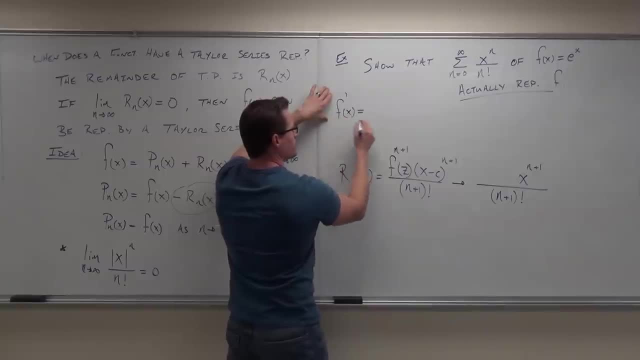 You're going to like this Sort of black and red. What's the first derivative of f? e to the x? What's the second derivative of f? e to the x? What's the nth derivative, e to the x, e to the x. 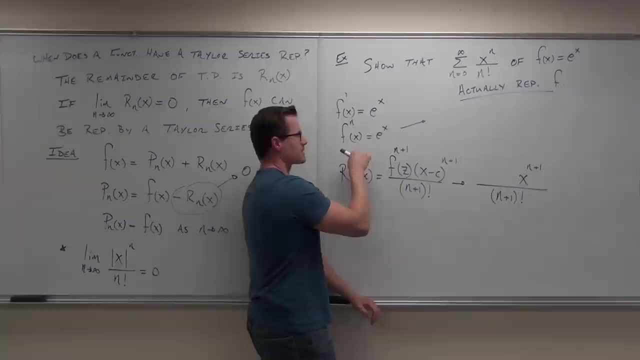 OK, now here's the jump. If the nth derivative f, is e to the x, what's the m plus 1 derivative of x? e to the x? What's the first derivative of f? e to the x, e to the x. 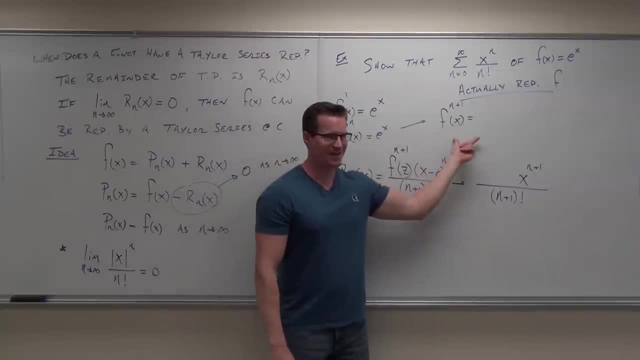 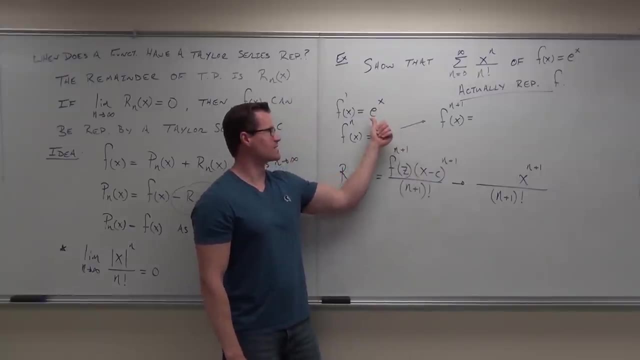 What's the nth derivative of x? What's the next derivative after that? Don't be adding ones to that. Did you add a one here? No, don't do nothing. So if this is the first derivative, and this is the second derivative, 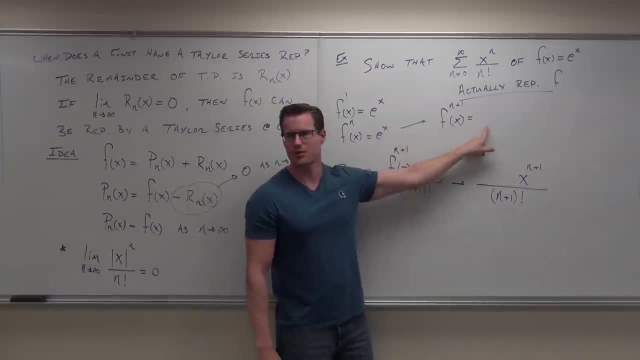 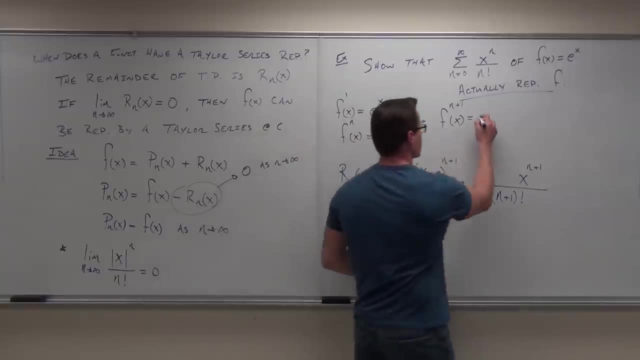 and the third derivative and the fourth derivative and nth derivative. what makes you think it's a mean derivative for the n plus one derivative? Should it be the same? Yes, Have I lost you guys? No, So we go. okay, well, tell you what. 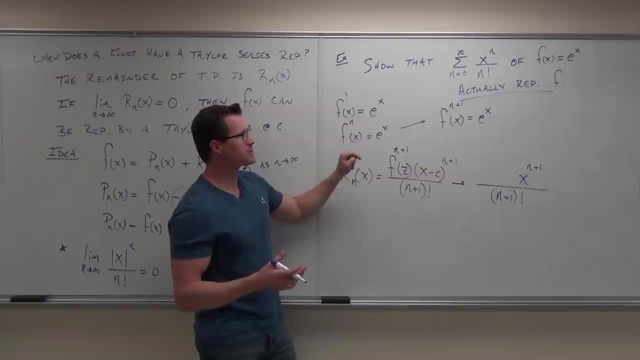 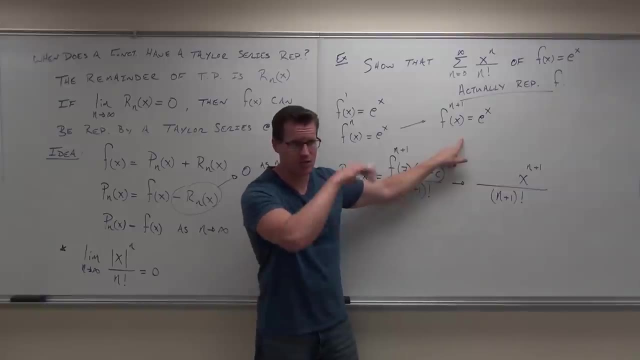 We wanna find out what the n plus one derivative of f is at z. We just found out what the n plus one derivative of f is at x. What must you do now? Change the x to the z. Change the x to the z. 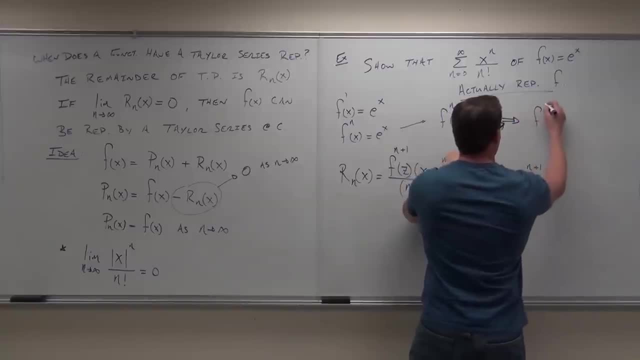 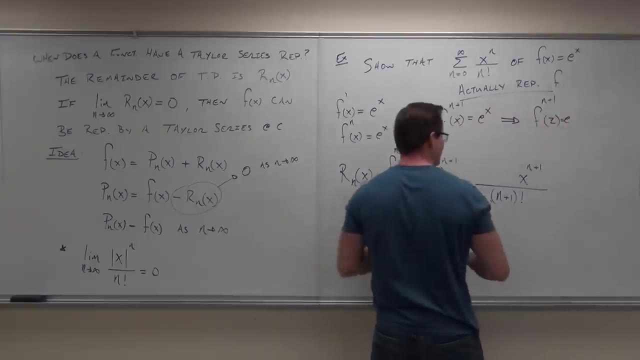 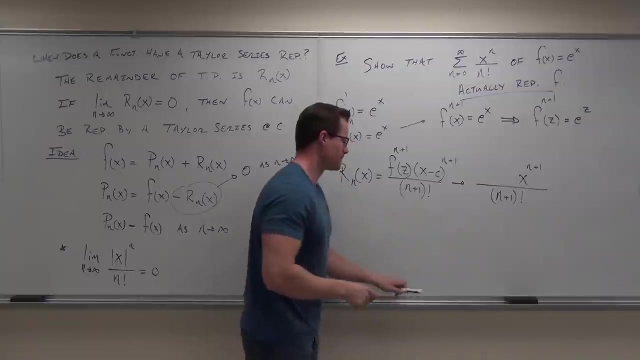 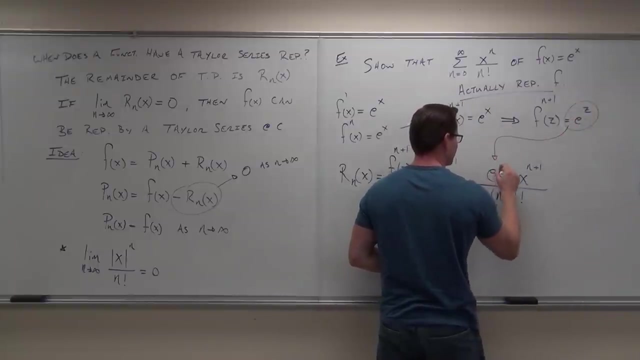 So just plug in z. Therefore the n plus one derivative of f at z is simply e to the z. It's easy, right, That's great. Then you have to bring a broom in. Find you a be noisy, 어머ny. 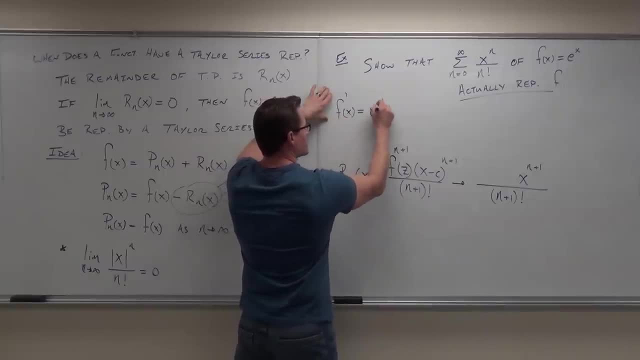 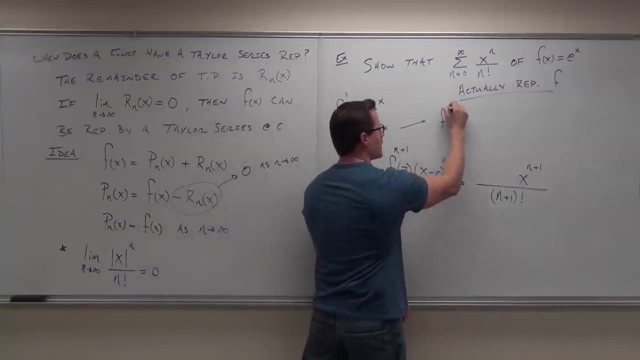 What's the first derivative of f? e to the x. What's the second derivative of f? e to the x. What's the nth derivative? e to the x, e to the x. Okay, now here's the jump. If the nth derivative of x is e to the x, what's the n plus 1 derivative of x? 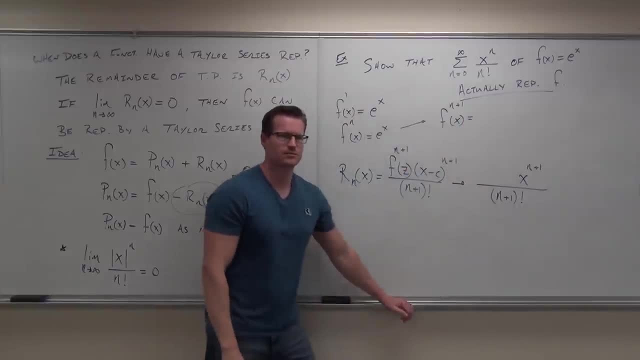 e to the x 1.. What's the first derivative of f? e to the x. What's the nth derivative of x? e to the x? What's the next derivative after that e to the x? Don't be adding 1's to that. 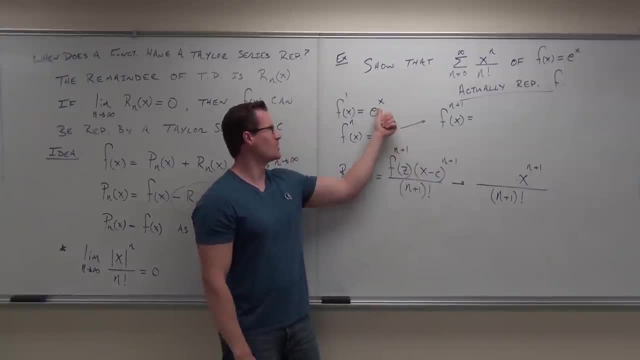 Did you add a 1 here? No, No, don't do nothing. So if this is the first derivative, and this is the second derivative, and the third derivative, and the fourth derivative and nth derivative, what makes you think it's going to be different? 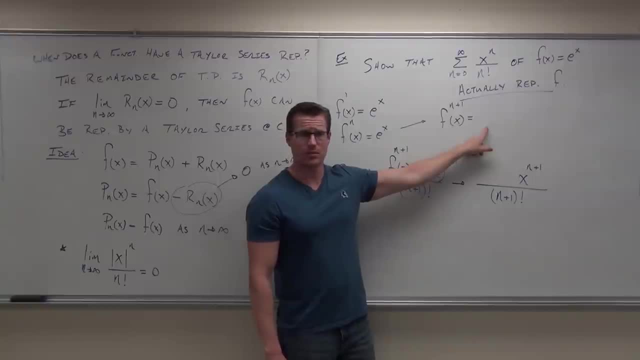 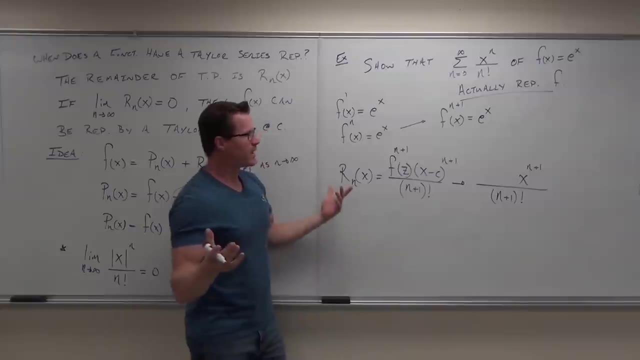 for the n plus 1 derivative. Should it be the same? Yes, Have I lost you guys? No, So you're okay. Well, I'll tell you what We want: to find out, what the n plus 1 derivative of f is at z. 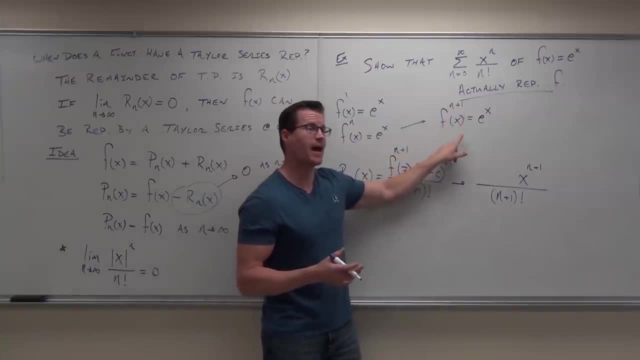 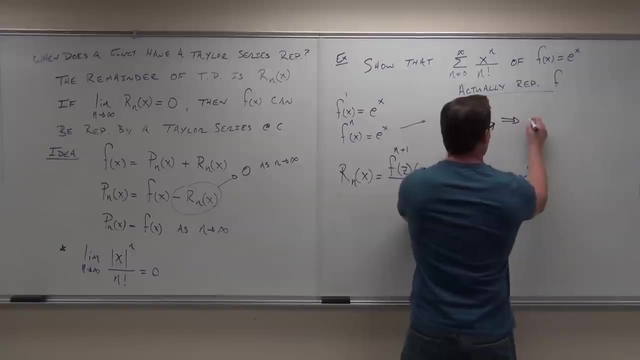 We just found out what the n plus 1 derivative of f is at x. What must you do now? Change the x to the z, Change the x to the z, So just plug in z. Therefore, the n plus 1 derivative of f at z is simply e to the z. 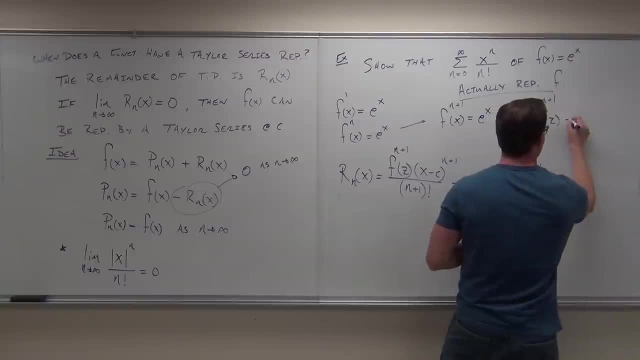 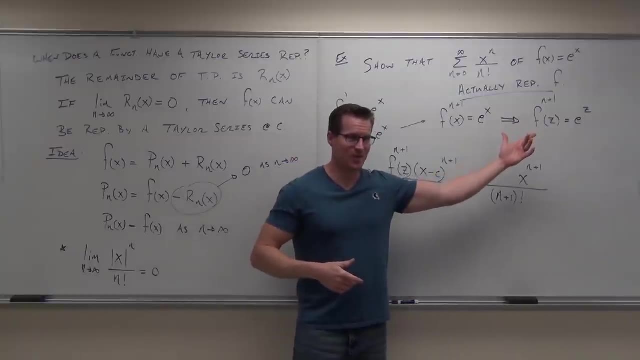 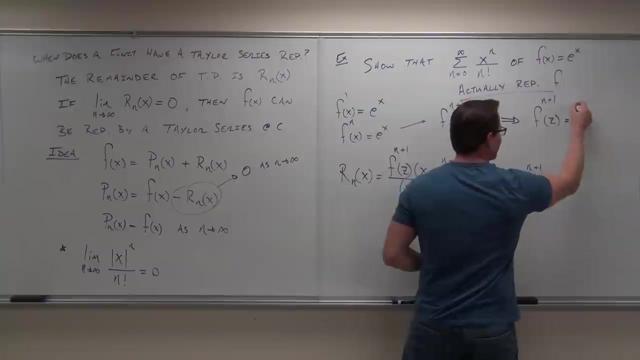 It's e to the z. On the z, It's easy Right? Wow, You didn't have to bring a broom in, I only need to buy you an EC. It's either ball or corn. That's even worse. 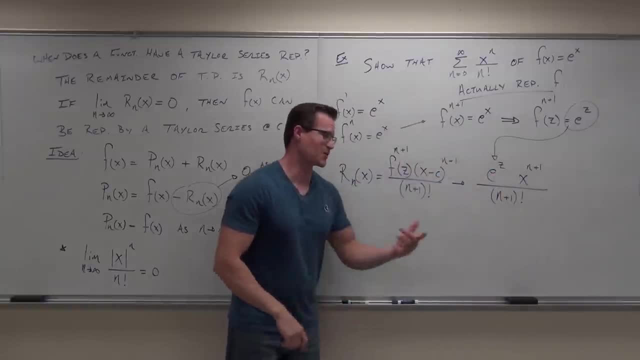 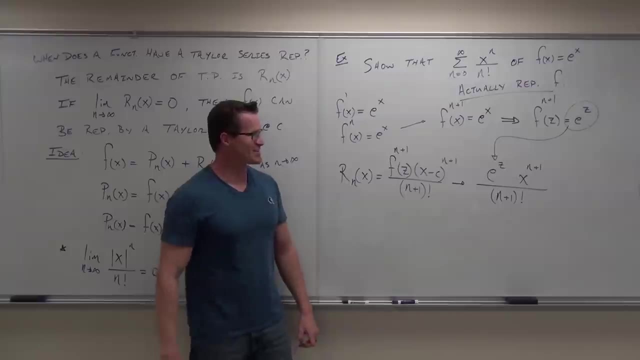 I'm at some videotape now. I'm not going to edit that. it's a good one. So what are we trying to do? We're not trying to reinvent the wheel. We don't need to reinvent that. this represents this. 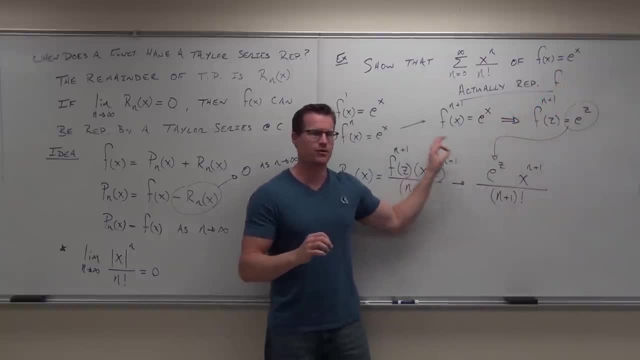 we're trying to prove it. Prove it by showing that the limit of your remainder is zero as n approaches infinity. Do that by trying to fill this piece out. This is always where you start for these problems, always where you start when trying to prove them. 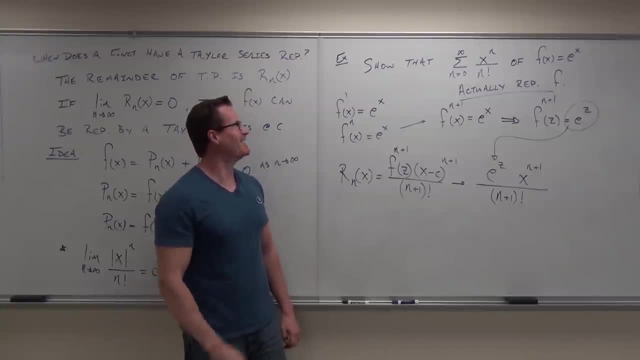 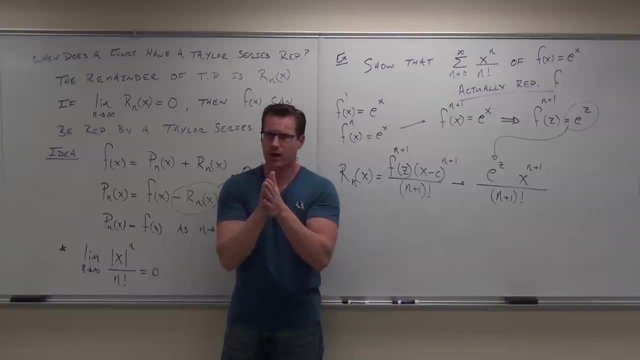 Now it's a video tape. now I'm not even gonna edit that. It's a good one. So what are we trying to do? We're not trying to reinvent the wheel. We don't need to reinvent. this represents this. We're trying to prove it. Prove it by showing that the limit of 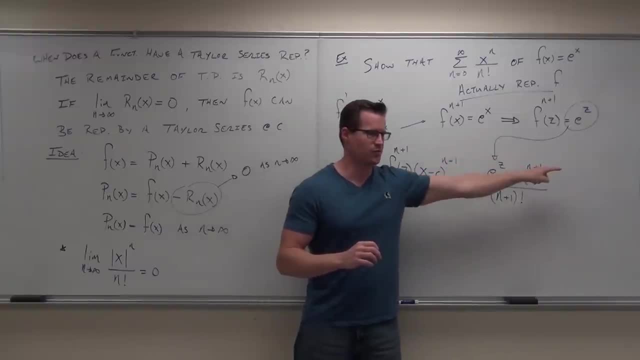 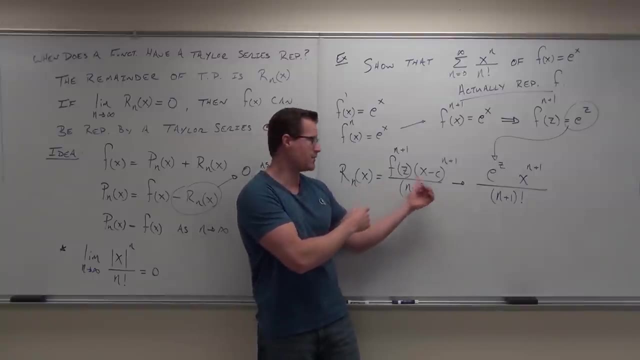 your remainder is zero as n approaches infinity. Do that by trying to fill this piece out. This is always where you start for these problems, Always where you start when trying to prove them. You have x minus c. Hey, it's a Taylor polynomial right, So you're going to have 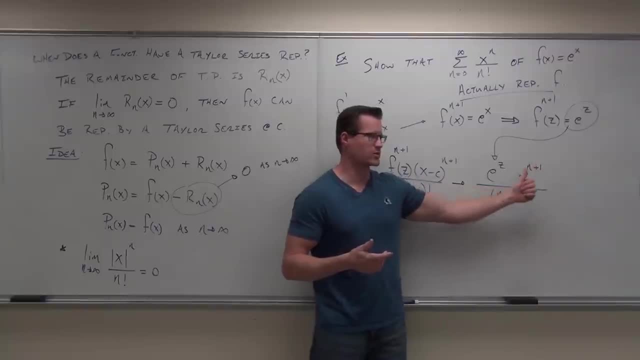 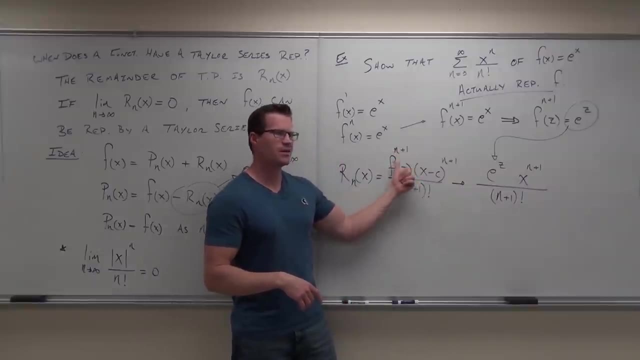 x minus c. c happens to be zero. x minus zero, no problem. x to the n plus one Over. n plus one factorial. that's your next term, Got it? And then we have the n plus one derivative of f at z. This is what you got to work on, So start with the first derivative, do the 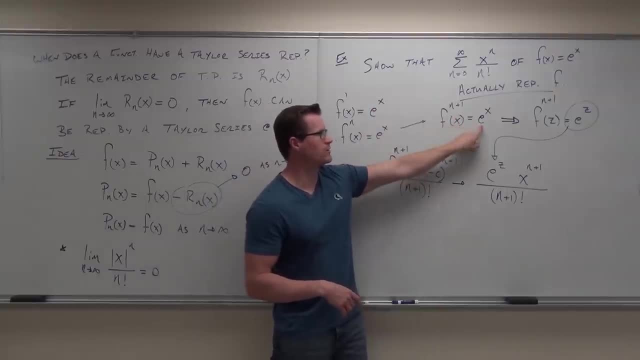 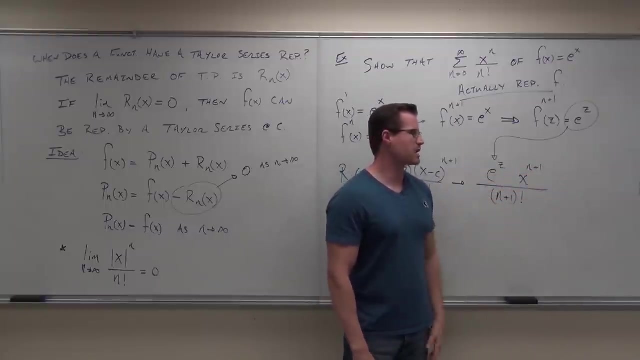 second one, do the third one, do the nth one, do the n plus one derivative and then simply plug in z. So far, so good. Now, after that, what we're trying to show is that the limit of this thing goes to zero. This is the idea. Now, you might have some cases here, You see. 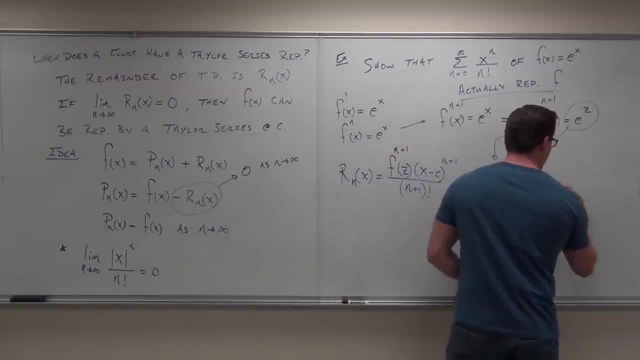 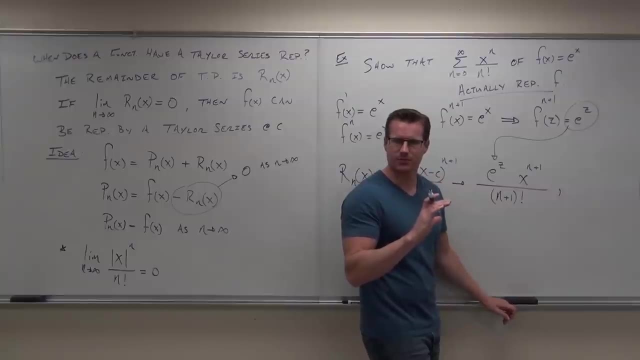 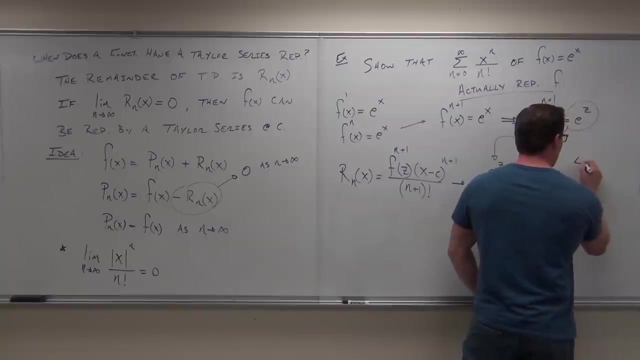 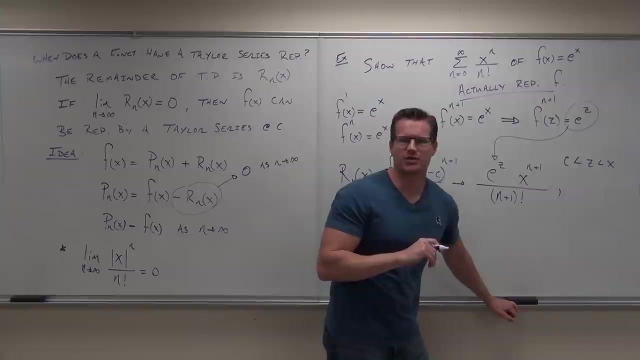 the thing is is that z is always equal to infinity. So what we're trying to show is that z is always between c and x. You follow: z is always between c and x. So if z is always between c and x, how much is our c? again, Everybody. how much is our c? 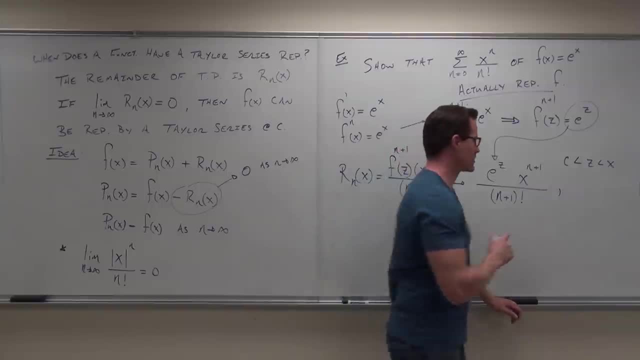 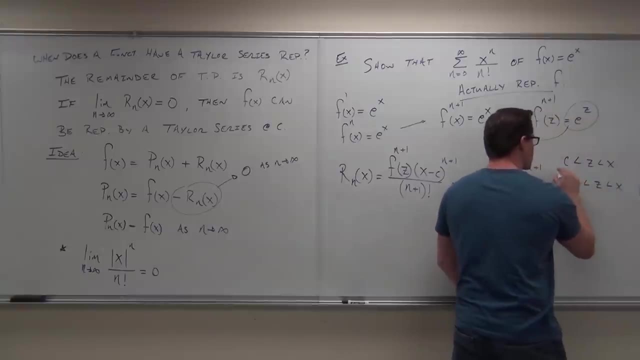 Zero. Very good, Why is it zero? Because I've learned before, Because I've learned before, So there's zero. So we basically have two cases. So this is: let's see, let's see, let's see. So this is zero. We have the case where x is positive and we have the case where 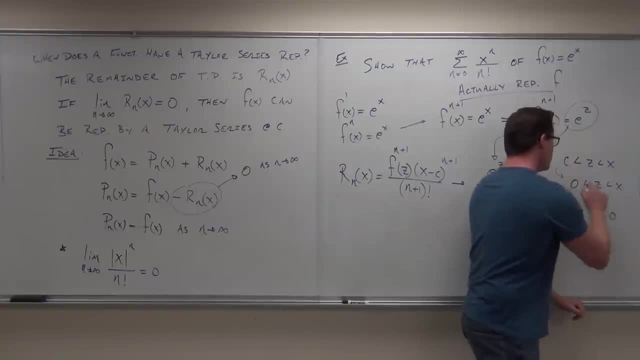 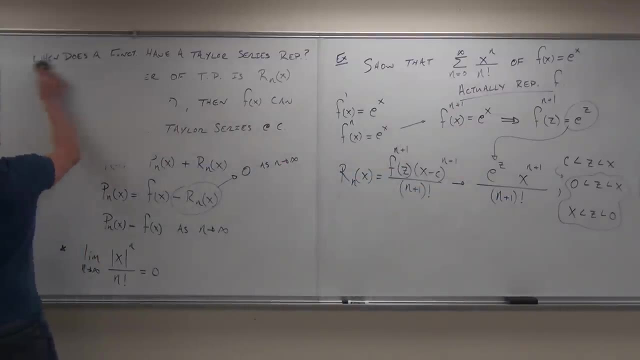 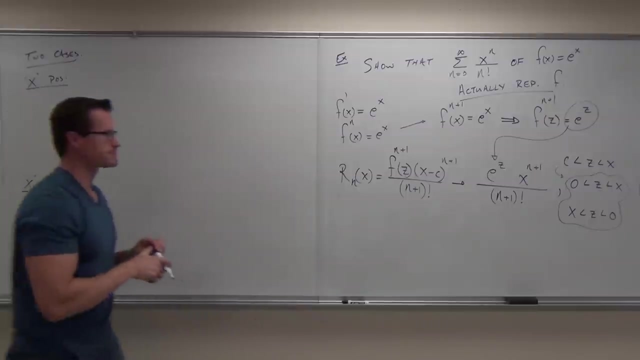 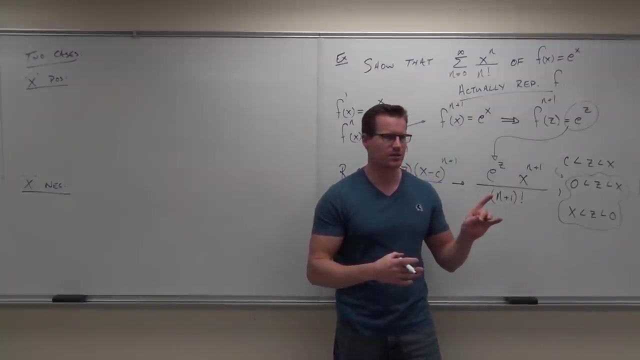 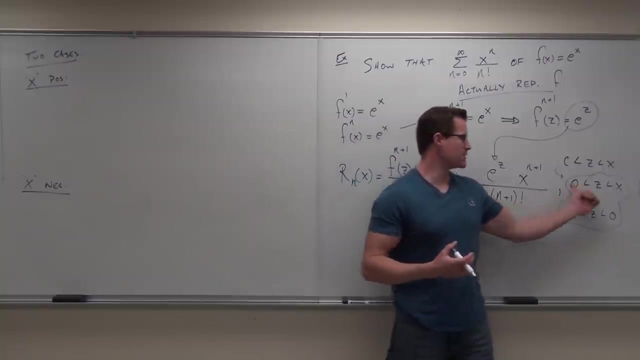 x is negative. You've got to show both those cases. Okay, let's start with the. do you guys understand the idea that z is always between c and x? You with me? Yeah, C is zero in this case. So either x is positive, in which case z is between zero and x, But 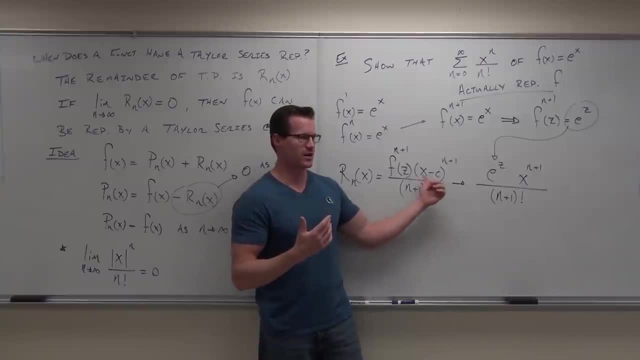 You have x minus c. hey, it's a Taylor polynomial, right, You're gonna have x minus c. c happens to be zero. x minus zero, no problem. x to the n plus one Over n plus one factorial. that's your next term, got it? 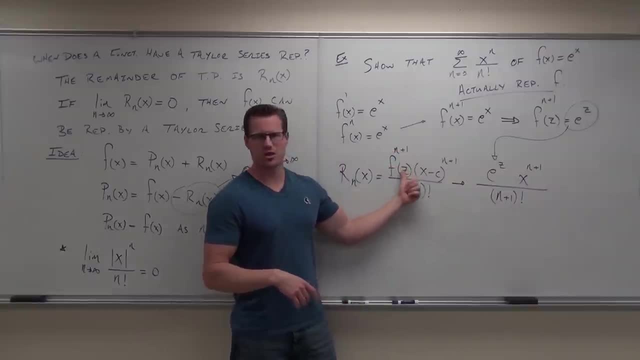 And then we have the n plus one derivative of f at z. This is what you gotta work on. So start with the first derivative, do the second one, do the third one, do the nth one, do the n plus one derivative. 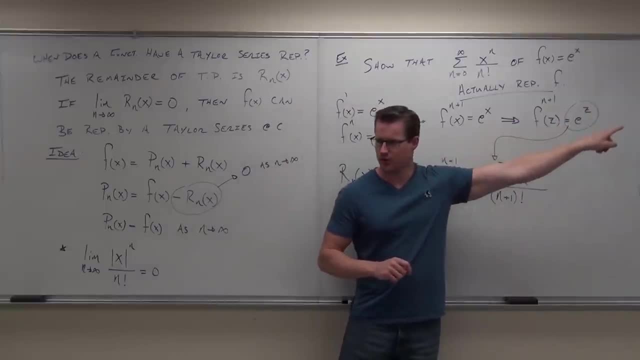 and then simply plug in: z. So far, so good. Now, after that, what we're trying to show is that the limit of this thing goes to zero. This is the idea. Now, you might have some cases here. You see, the thing is. 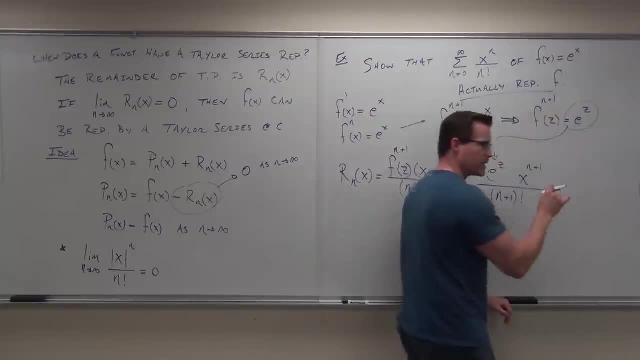 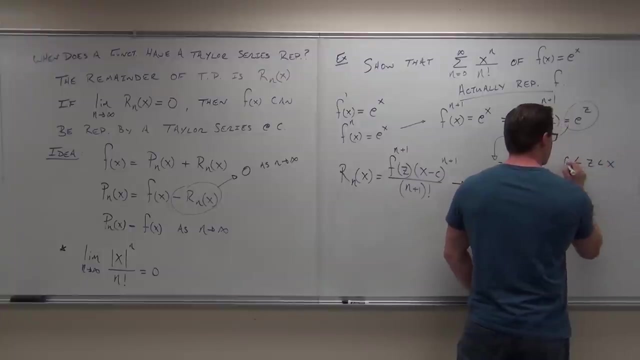 is that z is always between c and x. You follow, Yes, Z is always between c and x. So if z is always between c and x, how much is our c? again, Everybody. how much is our c? Zero. 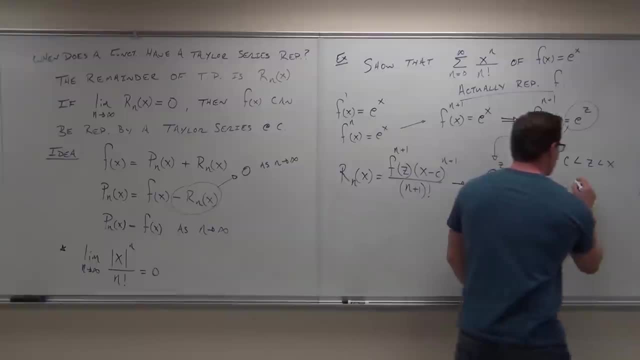 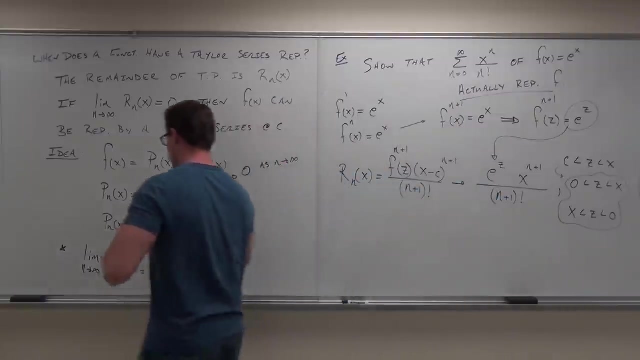 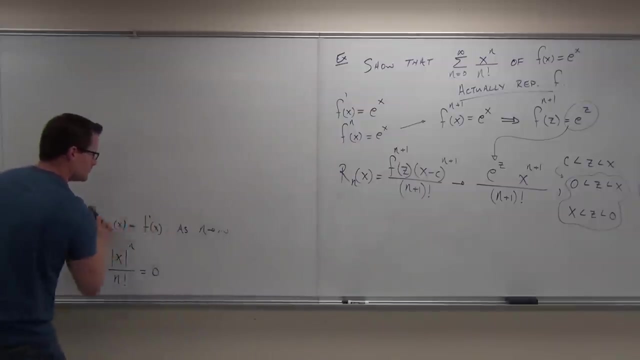 Very good. Why is it zero? Because I've learned before Senator: zero. So we basically have two cases. So this is zero. We have the case where x is positive and we have the case where x is negative. So we have z is always between z and x. 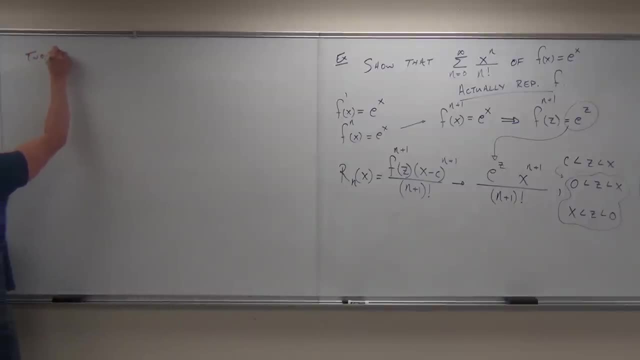 So this is zero. Now we've got to show both those cases. You've got to show both those cases. You've got to show both those cases. Okay, let's start with the. if you guys understand the idea that z is always between z and x, 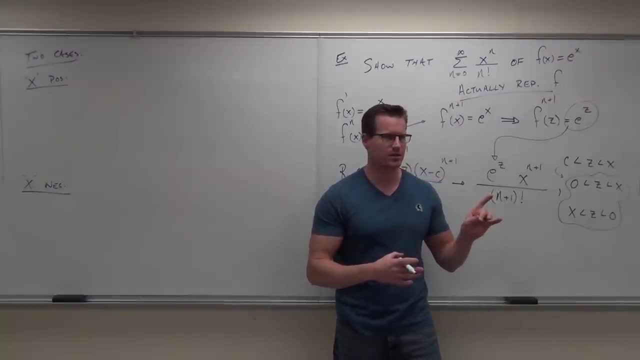 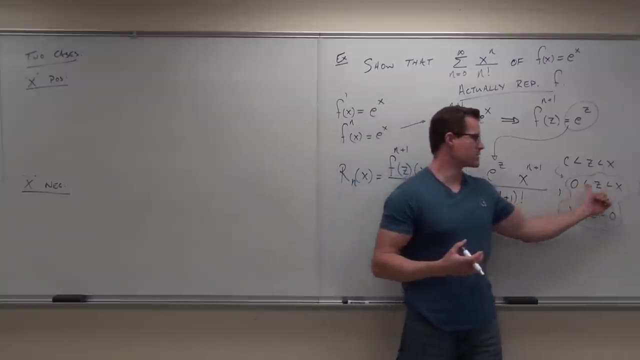 You've got to show both those cases that z is always between c and x. You with me? Yeah, C is zero in this case. So either x is positive, in which case z is between zero and x, or x is negative, in which case c is between x and zero. 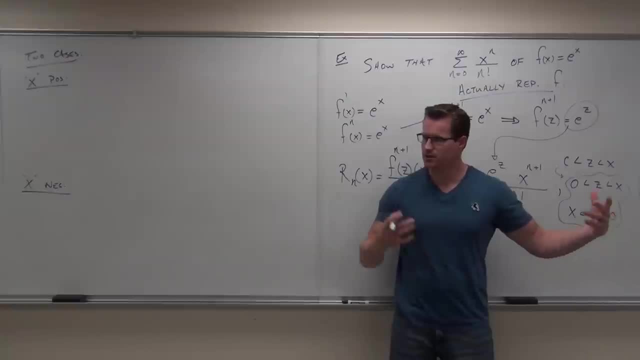 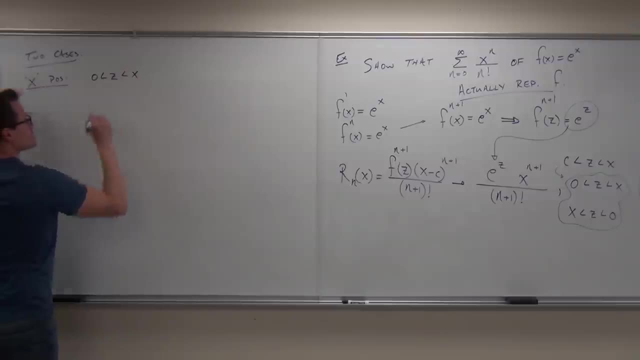 because x would be negative in this case. Not sure if you understand that idea. So, if z is positive, what we know is that zero is less than z, which is less than x. Z's gotta be somewhere between zero and x. 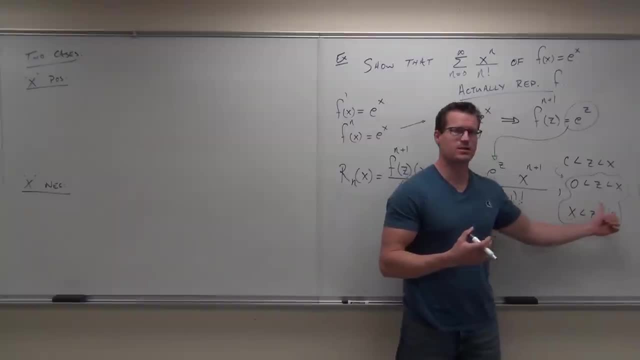 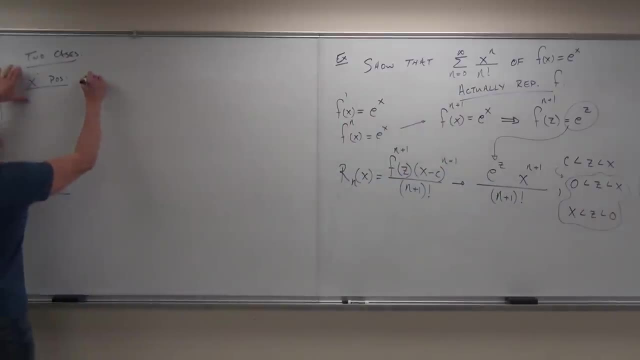 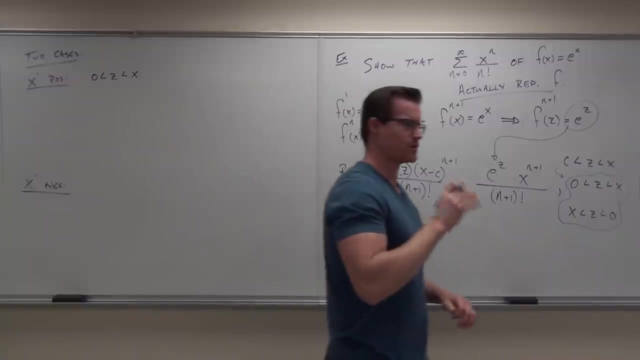 or x is negative, in which case c is between x and zero, because x would be negative in this case. Not sure if you understand that idea. So, if z is positive, what we know is that zero is less than z, which is less than x. z's got to be somewhere between zero and. 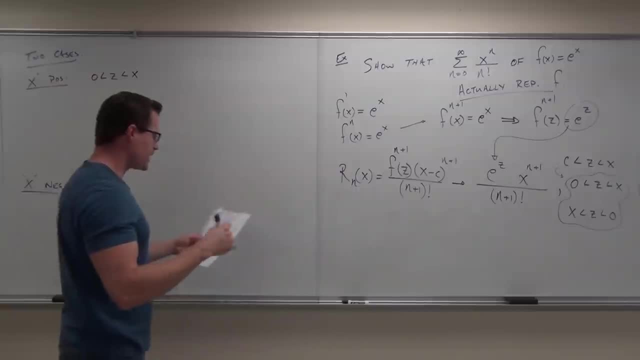 x. Now, if that's true, if z is somewhere between zero and x, stick with me here. we know a couple things. We know, firstly, that zero is going to be less than or equal to the remainder. Look at our remainder. Look over here. Is it true that that's always positive? 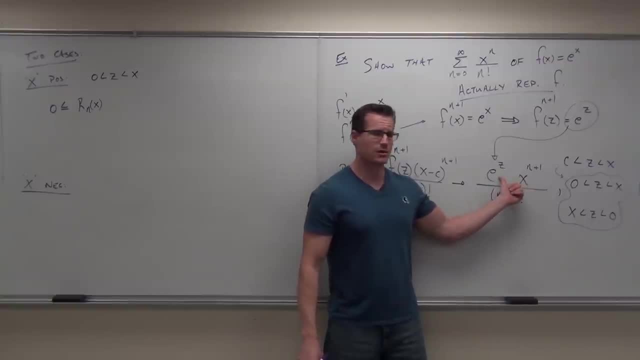 Yes. Is this always positive? Yes, Is this always positive? Yes? Well, no, But if x is greater than zero, yes, because that's in our case right now. Does that make sense to you? Yes, I don't want to lose you guys here. I'm getting some weird looks, So do you get that this? 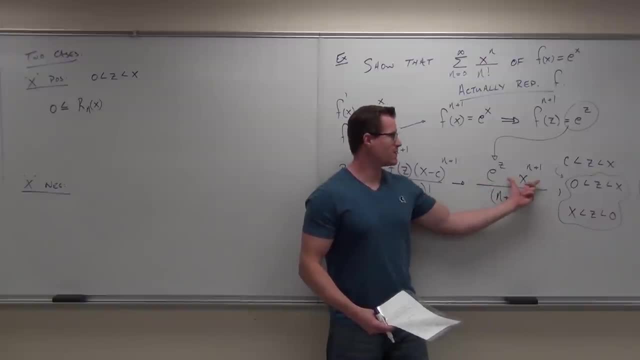 is always positive. Yes, Do you get that this is always positive? Yes, Do you get that? if x is greater than zero, if x is positive, then this is always positive. Yes, Therefore, this remainder is always positive. right now Has to be Now, since this equals. 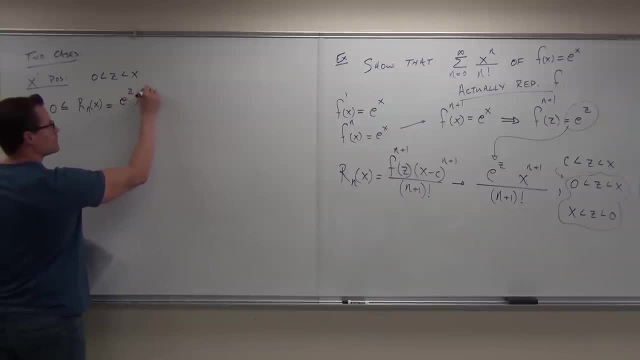 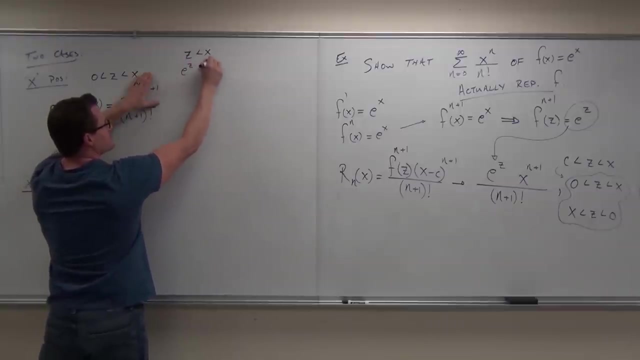 this thing. here's where we, here's where this comes in. If z is less than x, do you agree that e to the z is less than e to the x? Do you agree with that? Then this piece is less than e to the x: x n plus 1 over n plus. 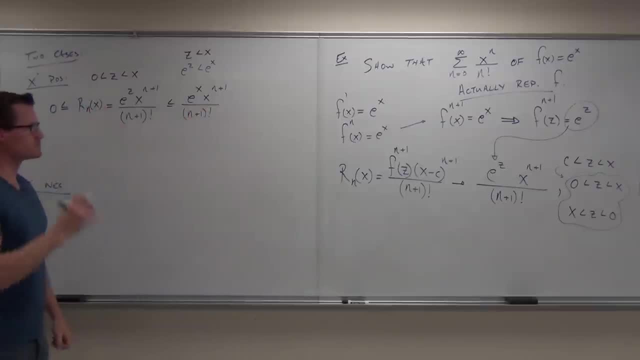 1, back to order. What Lost you? I just heard a lot of e to the v's and x's. Sure, Well, look at the board. Okay, This is what we're basing this on, correct? Yeah? 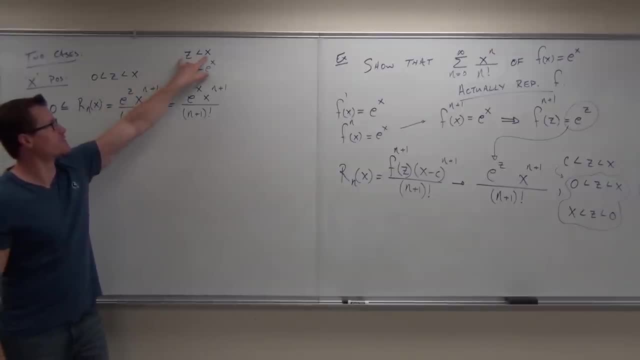 If this is true, same here, right. If this is true, this is true. If this is true, that's all I'm doing. Exactly the same crap, except this is now less than e to the x. If that's the only thing that's changing- and this is bigger than this- then this statement: 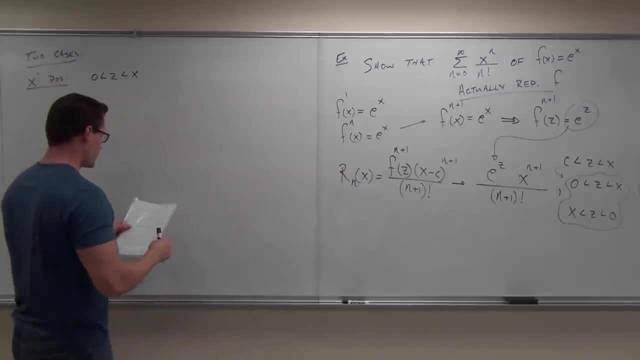 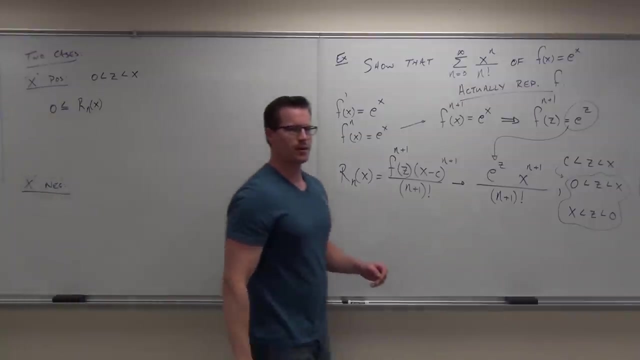 Now, if that's true, if z is somewhere between zero and x, stick with me here. we know a couple things. We know, firstly, that zero is going to be less than or equal to the remainder. Look at our remainder. 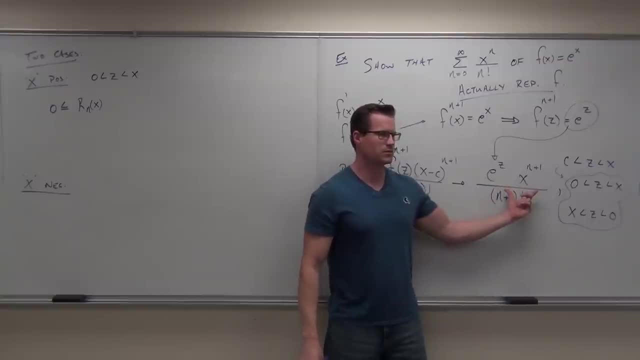 Look over here. Is it true that that's always positive? Yes, Is this always positive? Yes, Is this always positive? Yes, Well, no, but if x is greater than zero, yes, because that's in our case right now. 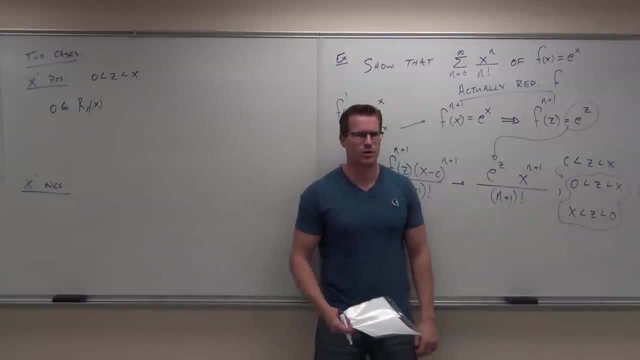 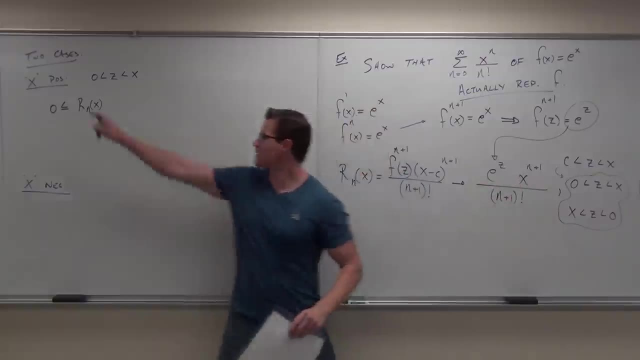 Does that make sense to you? I don't want to lose you guys here. I'm getting some weird looks. So do you get that this is always positive? Yes, Do you get that this is always positive? Yes, Do you get that if x is greater than zero, 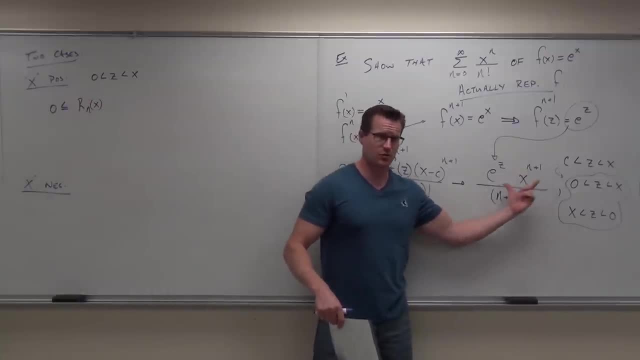 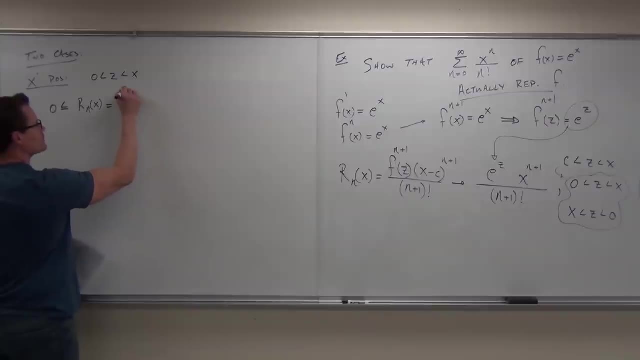 if x is positive, then this is always positive. Yes, Therefore, this remainder is always positive. right now Has to be Now, since this equals this thing. here's where this comes in. If z is less than x, do you agree that e to the z is less than e to the x? 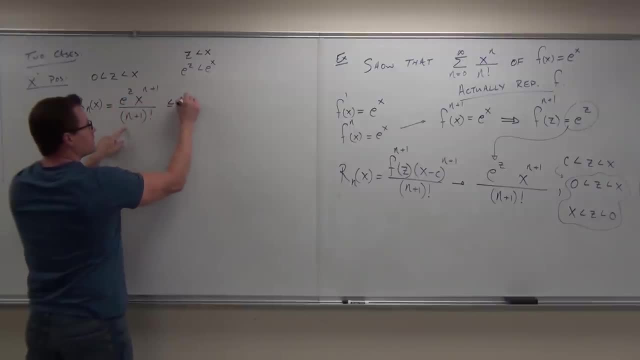 Do you agree with that? Then this piece is less than e to the x, x, n plus one over n plus one. Back to order. Lost you. I just heard a lot of e to the v's and x's. Sure well, look at the board. 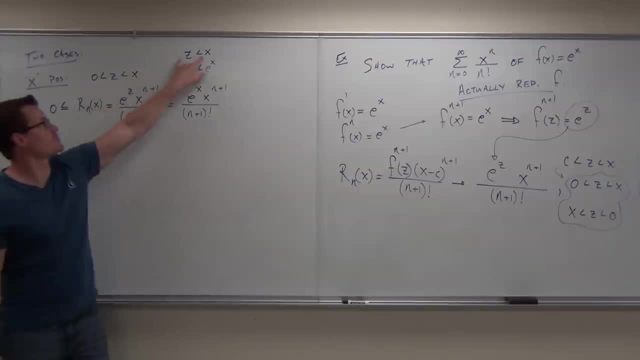 This is what we're basing this on, correct? Yeah, If this is true, same here, right? If this is true, this is true. If this is true, that's all I'm doing. Exactly the same crap, except this is now. 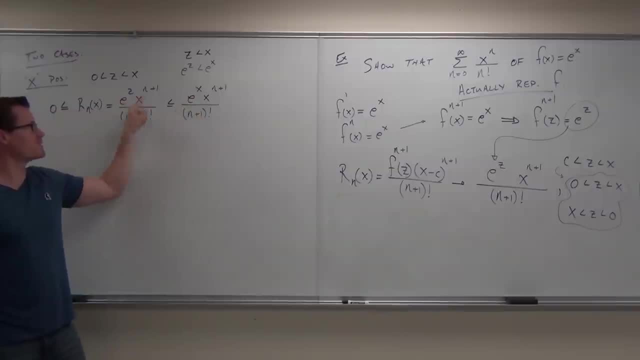 less than e to the x. If that's the only thing that's changing and this is bigger than this, then this stays Okay. If it's less than this, then this statement's true. Does that make sense to you? Yeah? 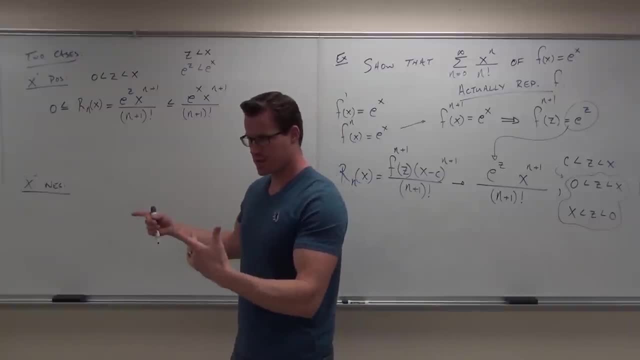 Now here's the idea: If I take the limit of all this stuff, what's the limit of zero? So I'm taking the limit of this as n approaches infinity. What's the limit of zero? Zero, Less than this stuff. 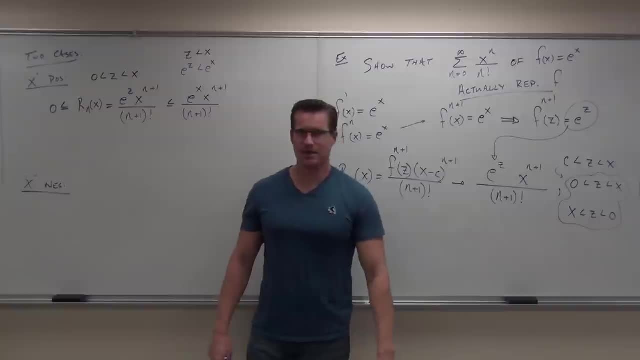 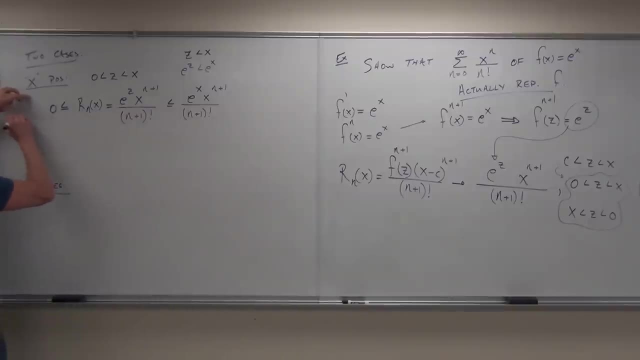 is true. Does that make sense to you? Yeah, Now here's the idea. If I take the limit of all this stuff, what's the limit of zero? so I'm taking the limit of this. as n approaches infinity, What's the limit of zero? 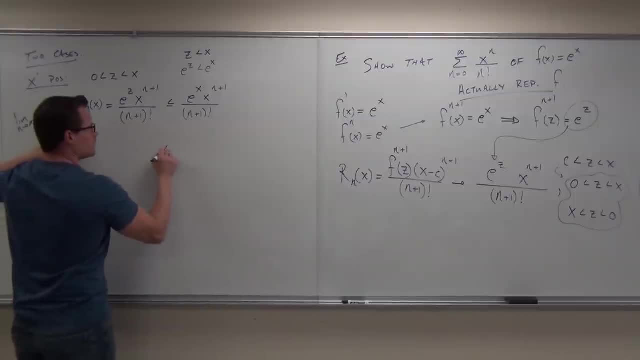 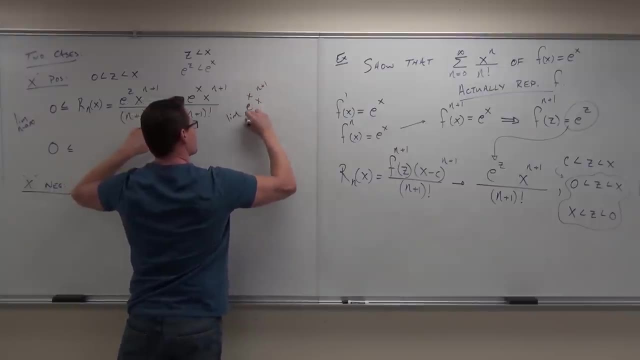 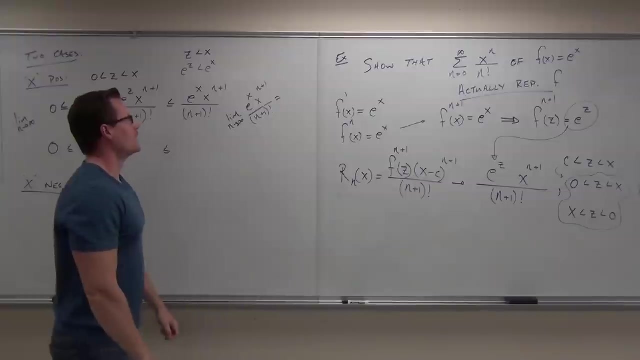 Zero, Less than this stuff. What's the limit of e to the x? x? n plus 1, all over n plus 1- factorial. This is why I gave you that statement just a little while ago. Ignore the e to the x right now, because that's not based on n. Here's what this says. Please listen carefully. 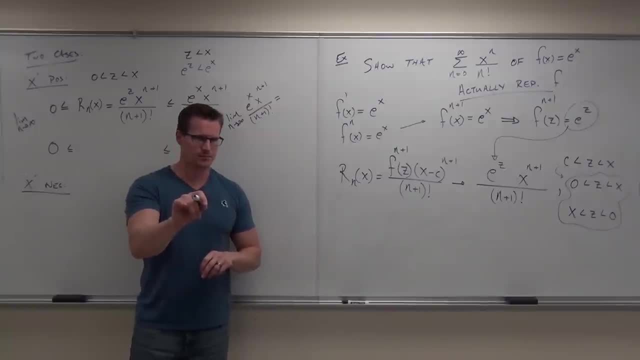 Pick an x for me, Anything. Two In your head, Whatever you want. Four billion, I don't care. okay, E to the four billion is going to be a constant. Do you get me? Yeah, X to the n plus 1.. Well, it's going to be four billion to the n plus 1.. That's true. 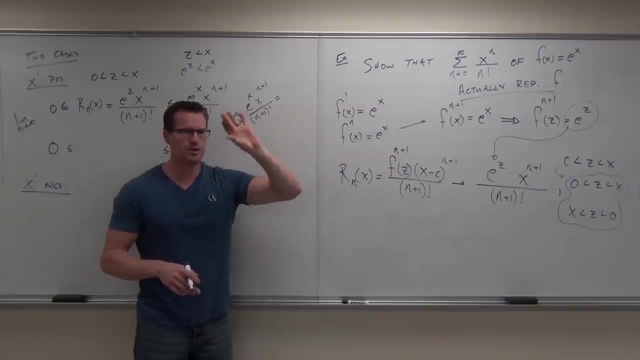 So you're going to have four billion times four billion times four billion, But it will be a constant for every single one of those fractions. Do you get that? Is that ever a constant? No, No. So the idea is this thing goes forever. 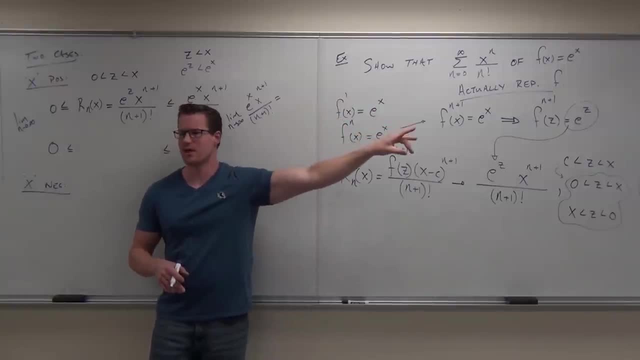 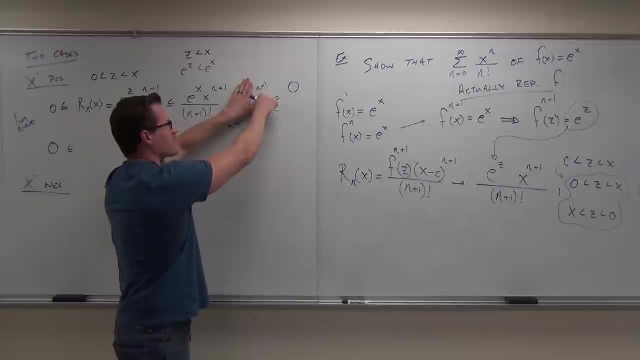 Forever. So it gets four billion and then it goes way bigger than that. Does that make sense? Ultimately, this limit is going to be zero. That's why I gave you this. Remember doing this? X to the n over n was equal to zero. I had it on the board. rewind the tape or 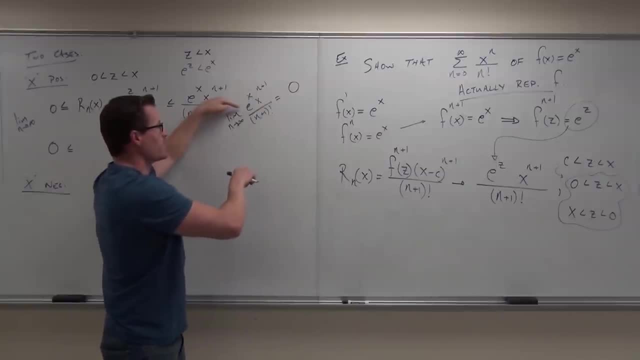 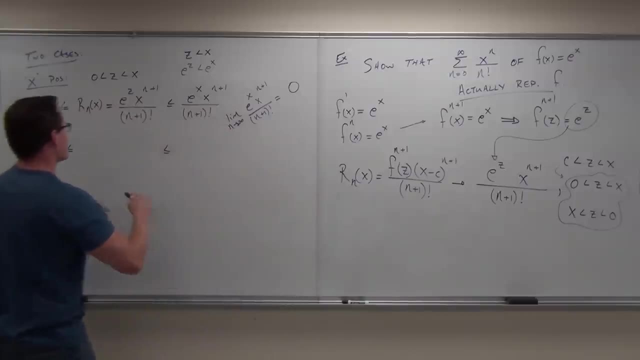 look back at your notes. This was zero. If I multiply it by something, that's going to be a constant, it does not change that It's still going to be zero. Do you buy into that? Okay, Therefore, if this limit gives you zero and the limit of this thing is zero, oh tell. 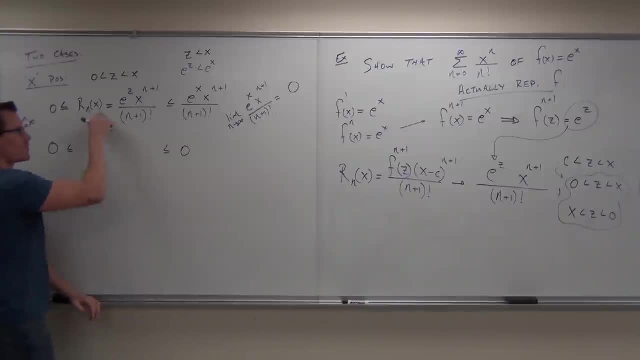 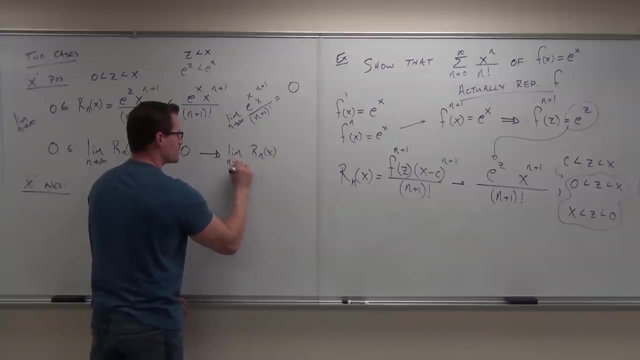 me what this is going to be: Zero, Zero. Therefore, the limit of the remainder as n approaches infinity by the squeeze theorem. this says the limit of the remainder of our Taylor polynomial as n approaches infinity must also be zero. Why is that important? 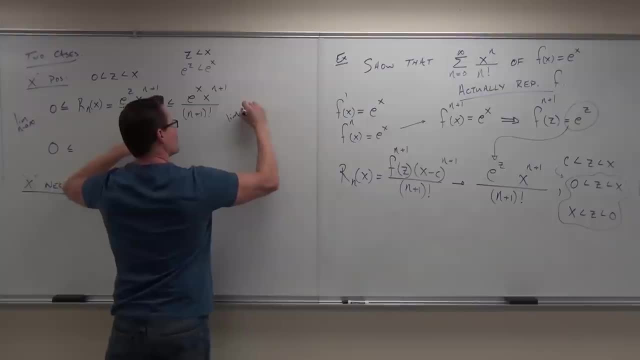 What's the limit of e to the x? x, n plus one, all over n plus one factorial. this is why I gave you that statement just a little while ago. Ignore the e to the x right now, because that's not based on n. 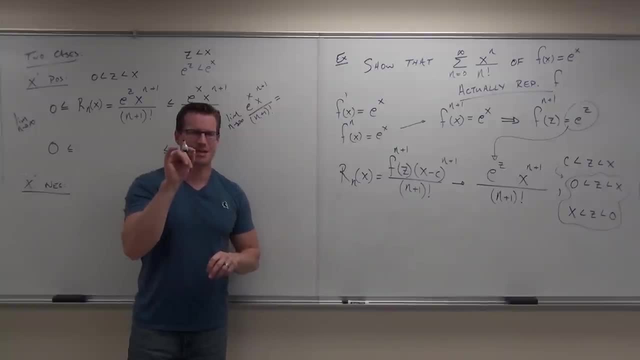 Here's what this says. Please listen carefully. Pick an x for me, Anything, Two In your head. Whatever you want, Four billion, I don't care. okay, E to the four billion is gonna be a constant. Do you get me? 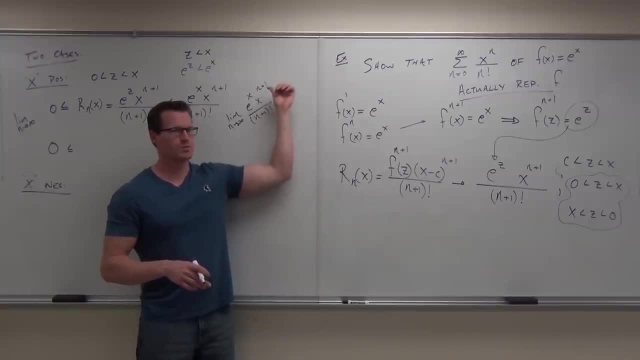 Yeah, X to the n plus one. well, it's gonna be four billion to the n plus one, that's true. so you're gonna, you're gonna have four billion times four billion times four billion, but it will be a constant for every single one. 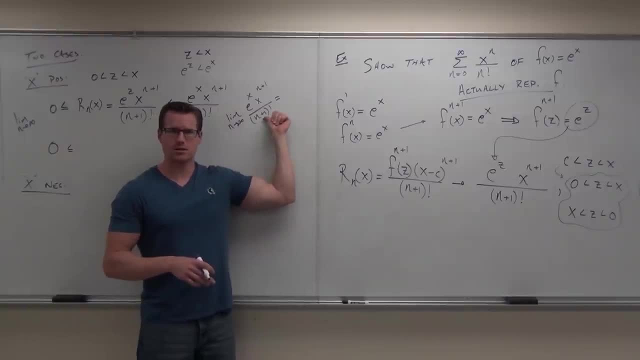 of those fractions? do you get that? Is that ever a constant? No, No. so the idea is: this thing goes forever, so it gets four billion, and then it goes way bigger than that. Does that make sense? Ultimately, this limit is going to be zero. 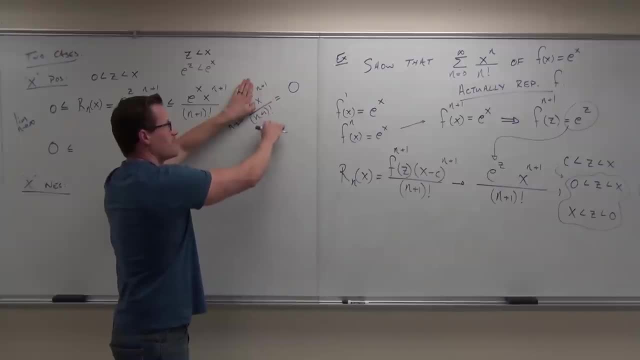 That's why I gave you this. Remember doing this: X over x to the n over n was equal to zero. I had it on the board. rewind the tape or look back at your notes. This was zero If you multiply by something that's going to be a constant. 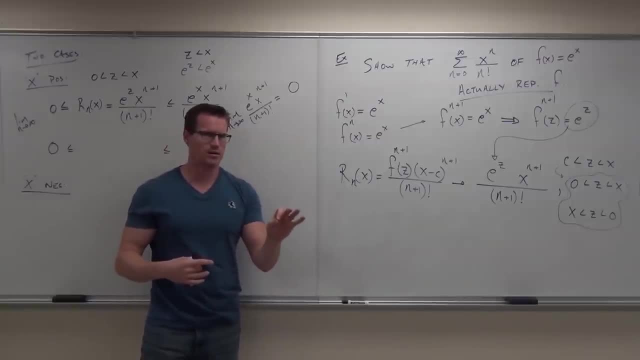 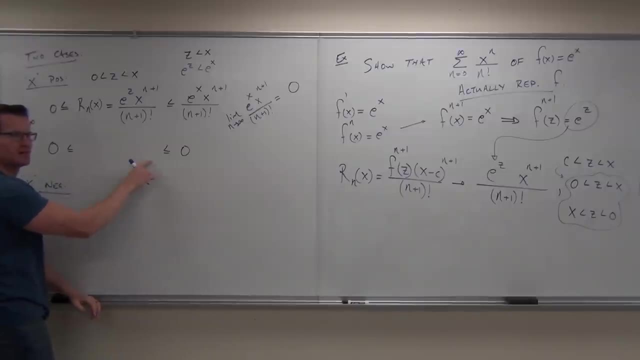 it does not change that, it's still gonna be zero. Do you buy into that? Okay, therefore, if this limit gives you zero and the limit of this thing is zero, oh, tell me what. this is gonna be Zero. 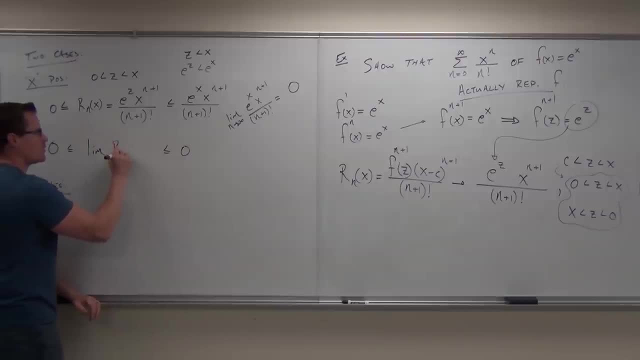 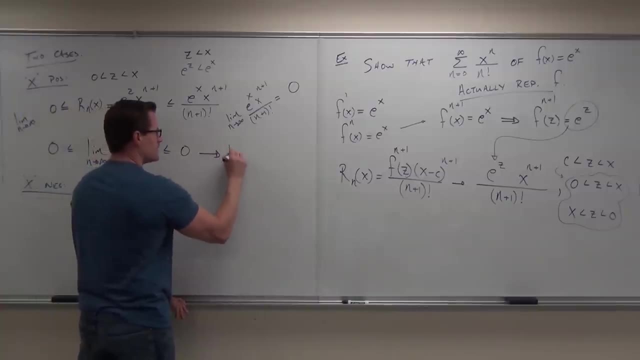 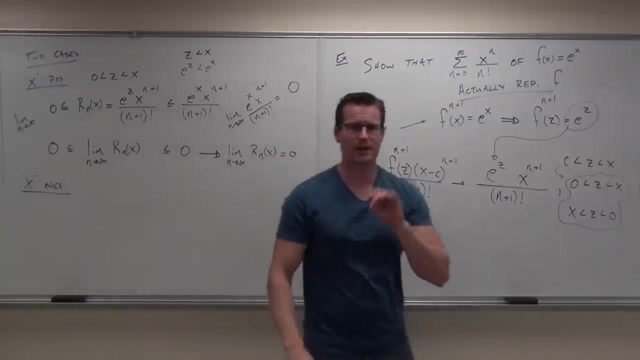 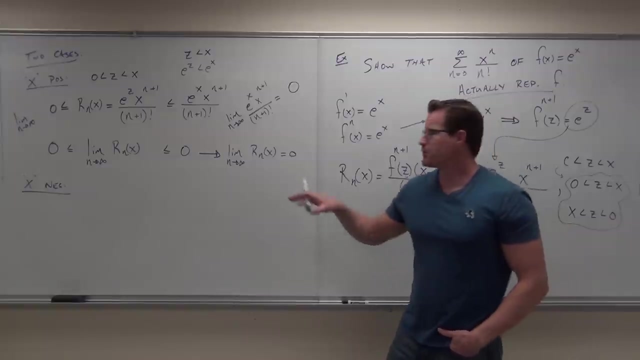 Therefore the limit of the remainder as n approaches infinity by the squeeze theorem, this says the limit of the remainder of our Taylor polynomial as n approaches infinity, must also be zero. Why is that important? That proves it right there, If the limit of our remainder gives you zero. 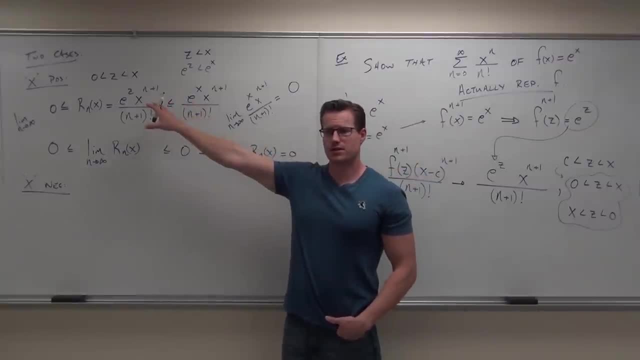 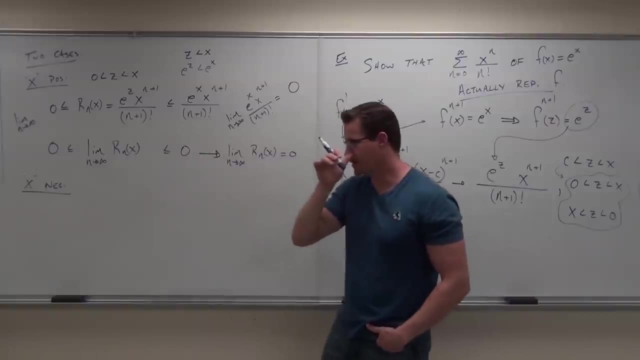 what that says is that for this case, for this case, the Taylor series represents our function. That's what it says, because the remainder gives us zero. We showed that earlier. that was the idea of our proof. Now I gotta go through this one a little bit quickly. 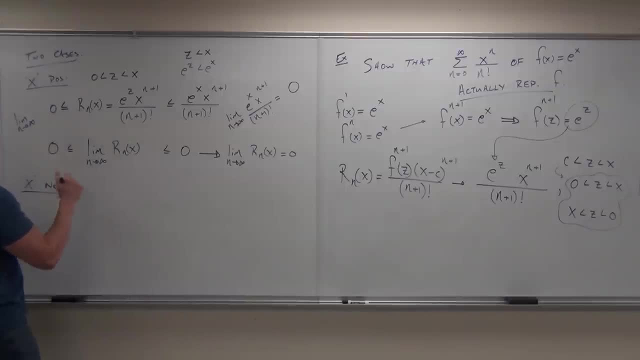 because I wanna do one more example before I let you go. So if x is negative, then x is less than zero, but z's gotta be somewhere between there. Well, if that's true, this one's actually a little bit easier, okay. 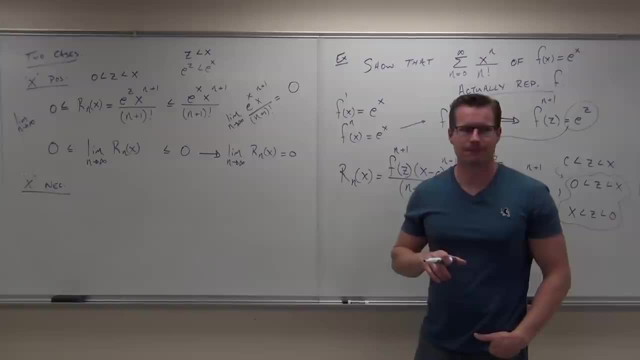 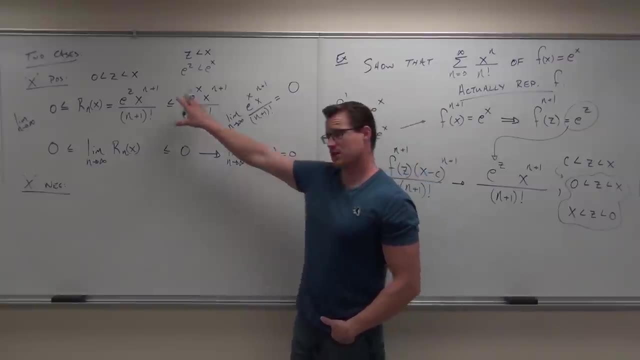 To show that the remainder of our polynomial is zero. That proves it right there. If the limit of our remainder gives you zero, that means that for this case, the Taylor series represents our function. That's what it says, because the remainder gives us zero. We showed that earlier. That was the idea of our proof. 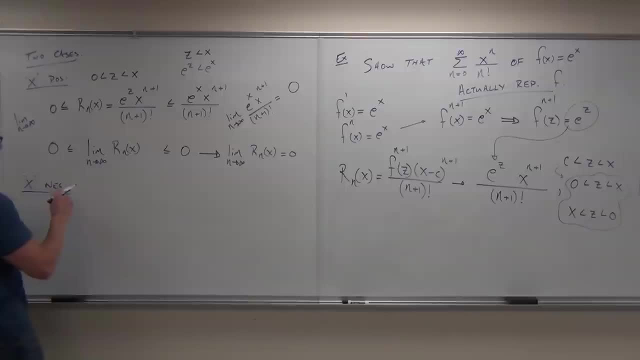 Now I've got to go through this one a little bit quickly because I want to do one more example before I let you go. If x is negative, then x is less than zero, but z has got to be somewhere between there. If that's true, this one is actually a little bit easier. 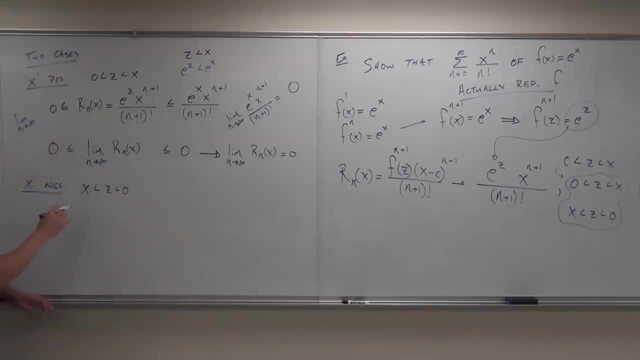 Okay, so check it out. If that's true, well then, what we're going to do is we're going to use a little trick here. Remember that if things are convergent in absolute value, then they're convergent regularly as well. You remember doing that. 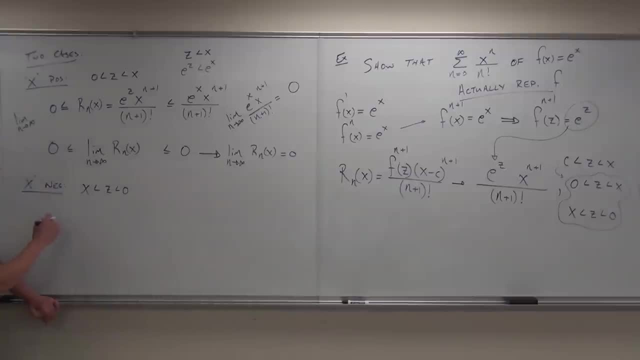 Yes, Okay, we're going to do this, We're going to say okay. well then, let's just consider the absolute value of our remainder. Is it true that the absolute value is going to be greater than zero? Yes, Okay, and this would be the absolute value of e to the z, x to the n, plus one all over. 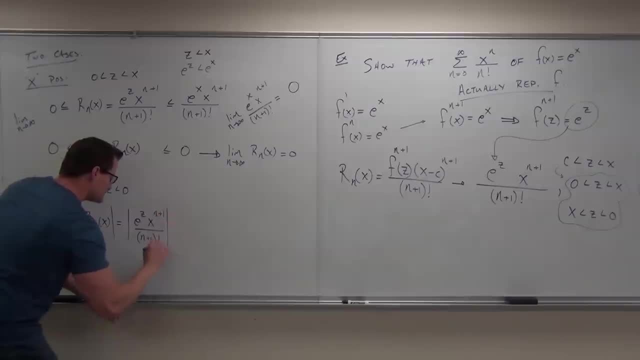 n plus one factorial, But this would be less than check this out. See if you can stick with me here. In this case, z is less than zero. Does that make sense to you? Well, if that's true, then e to the z would be less than zero. 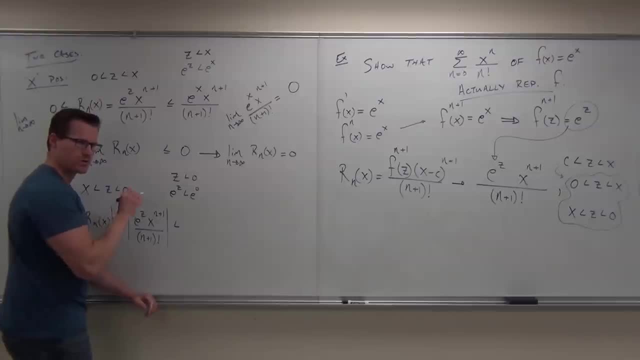 It would be less than e to the zero. You with me on that one? Yeah, Therefore, e to the z would be less than one. Does that make sense? Mm-hmm, If e to the z is less than one, then what we have is well, instead of e to the z, we. 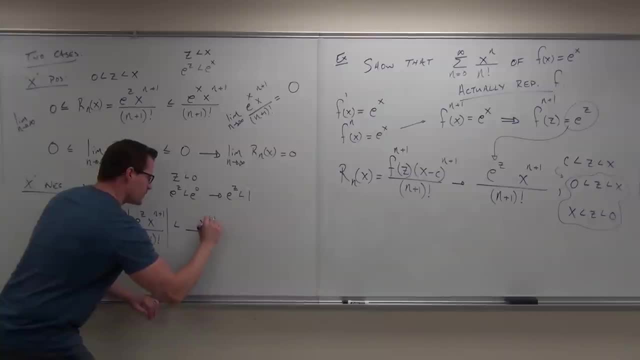 could have the same stuff, but instead of e to the z, we could have what? One? One Very good. Hey, look at this. What's the limit, as n approaches infinity, of zero, Zero, Oh, come on everybody. 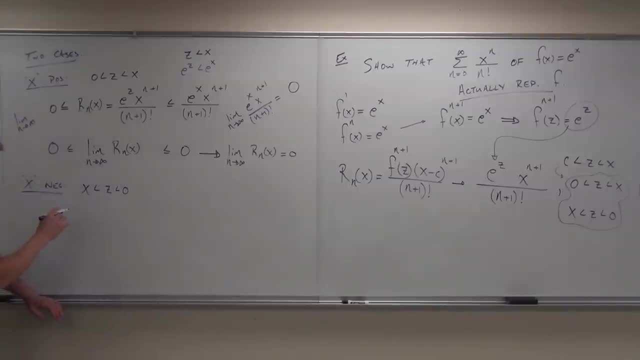 So check it out. If that's true, well then what we're gonna do is we're gonna use a little trick here. Remember that if things are convergent in absolute value, then they're convergent regularly as well. You remember doing that. 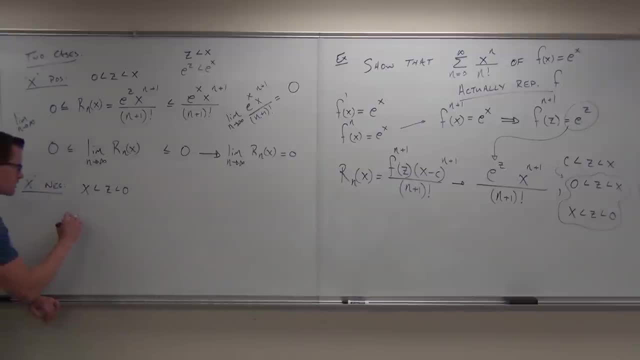 Yeah, Okay, we're gonna do this, We're gonna say okay. well then, let's just consider the absolute value out of our remainder here. Is it true that the absolute value is gonna be greater than zero? Yes, Okay, and this would be the absolute value of. 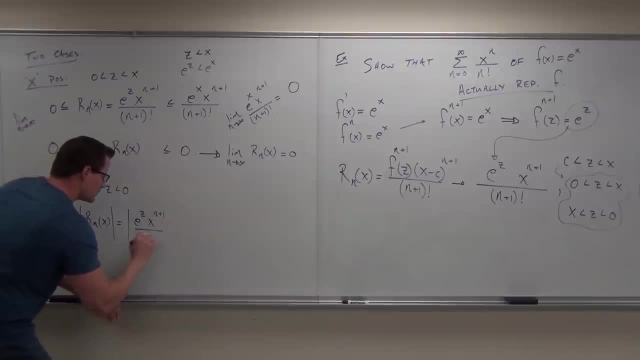 e to the z, x to the n plus one, all over n plus one factorial. But this would be less than check this out. See if you can stick with me here. In this case, z is less than zero. Does that make sense to you? 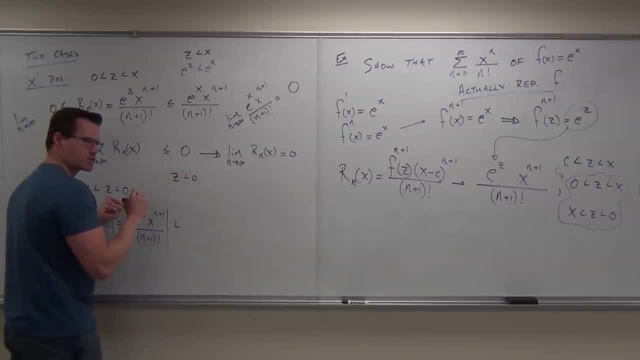 Mm Hm. Well, if that's true, then e to the z would be less than e to the zero. You're with me on that one? Yeah, Therefore, e to the z would be less than one. Does that make sense? 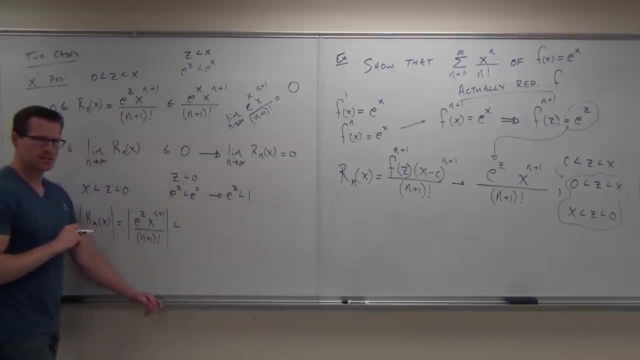 Mm Hm, If e to the z is less than one, then what we have is: well, instead of e to the z, we could have the same amount ofJustin. Oh, Oh, Exactly, Oh, It's true. 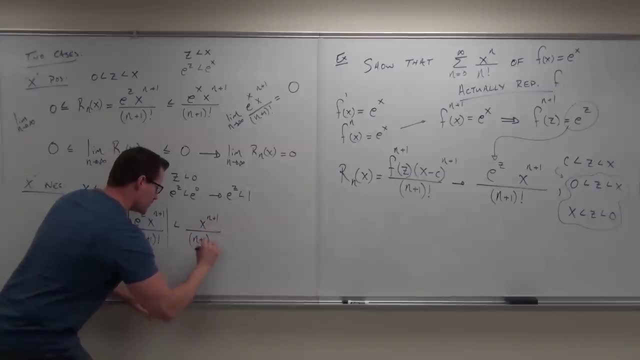 stuff. but instead of e to the z, we can have what One? Very good. Hey, look at this. What's the limit as n approaches infinity of zero? Oh, come on everybody, Zero. What's the limit as n approaches infinity of x to the n plus 1, over n plus 1 factorial. 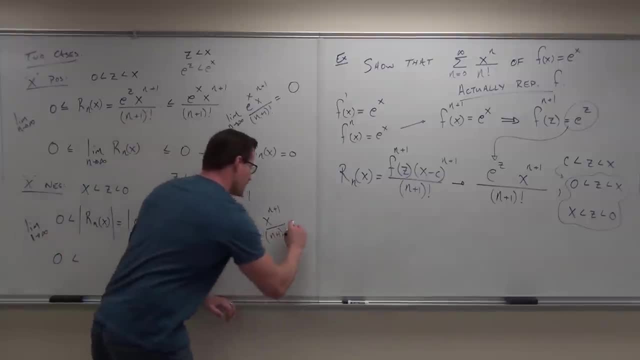 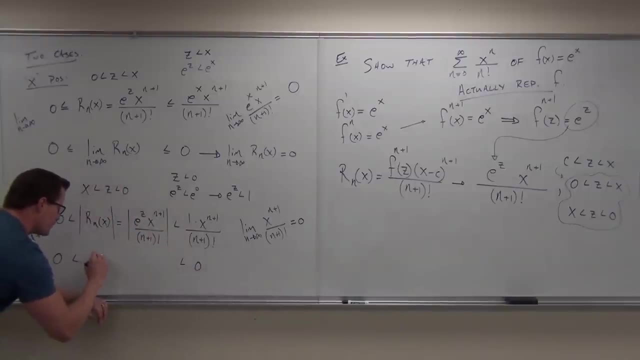 Think back to what we did, the opening of class. This is zero, So the limit of this thing is zero. The limit of this thing is zero, Therefore, and when we do, the limit of the remainder of our Taylor polynomial on this case, 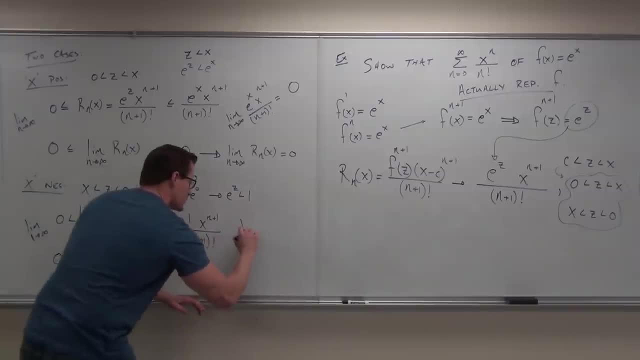 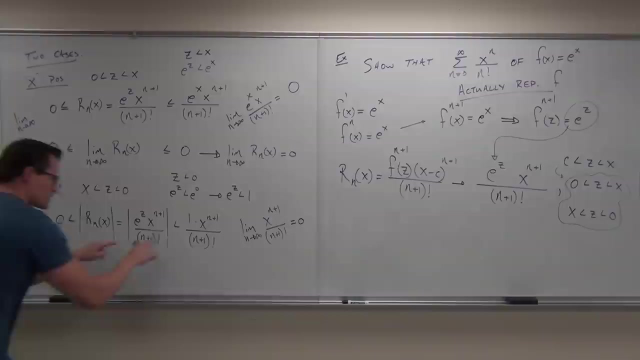 Zero, Zero. What's the limit, as n approaches infinity, of x to the n plus one over n plus one factorial. Think back to what we did: the opening of class Zero. This is zero. So the limit of this thing is zero. The limit of this thing is zero. 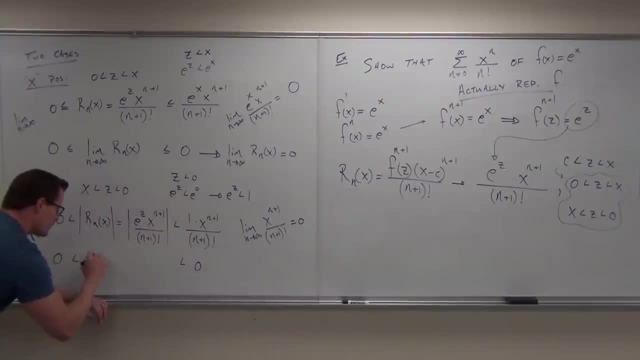 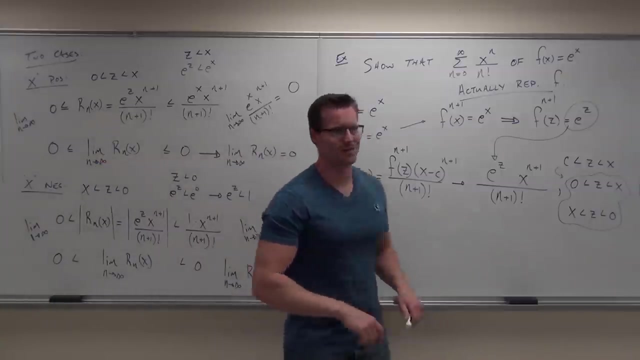 Therefore, and when we do the limit of the remainder of our Taylor polynomial on this case, we get that this is also zero. Whew, That's a lot of abstract stuff, right? That's proving some stuff. That was what we just did. 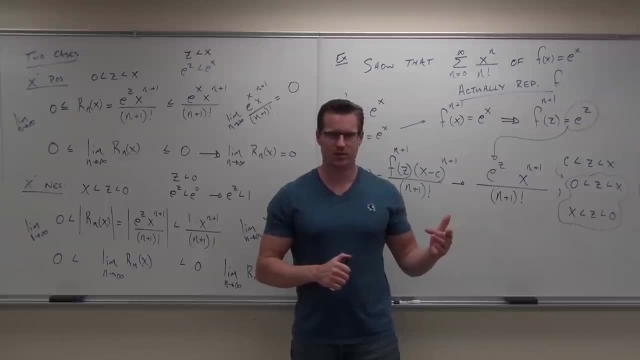 All right, Do you need me to go back through it for a few seconds? 10 second little recap here. Okay, 10 second, 20 second recap: Here it is The idea of this whole idea is: don't reinvent the wheel, You're trying to prove that the 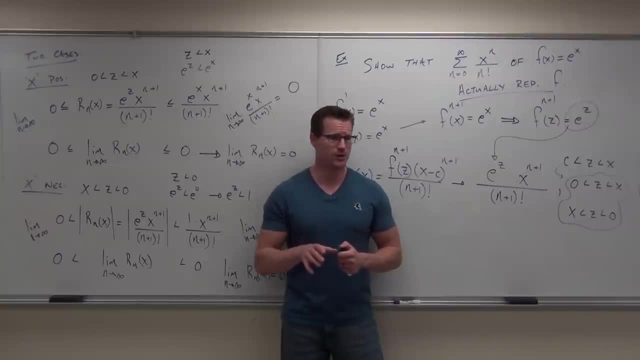 remainder equals zero when you take a limit of it as n approaches infinity. If you do that, what that says is that the remainder goes to zero. Therefore, if I go to infinity, the Taylor polynomial actually represents a function. that's a Taylor series. 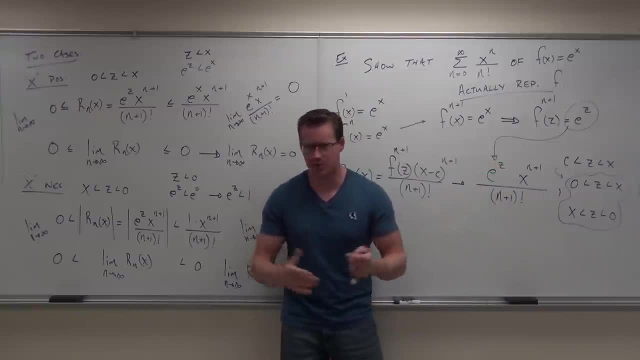 So just prove the remainder equals zero. All right, The way we do that is we try to build the remainder into something in z's and x's, Not f's. You've got to get z's and x's, So e to the z, x to the n plus 1, no problem. 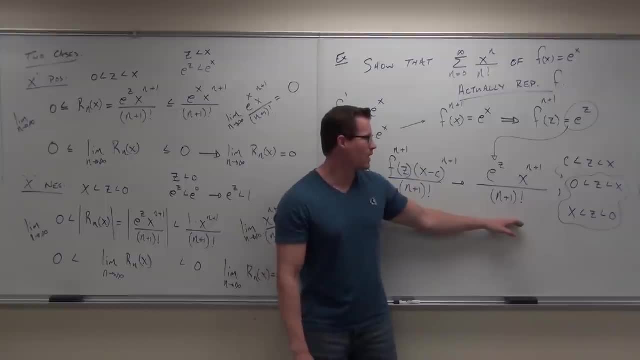 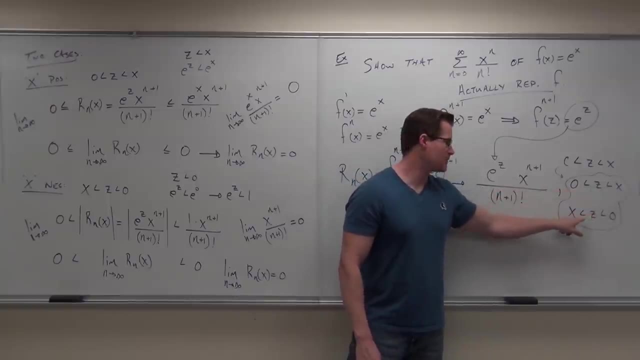 Sometimes you're going to have some cases here. In our case, well, x could be positive and x could be negative. We have two cases. If x is positive, z is between zero and x. If x is negative, then z is between x and zero. 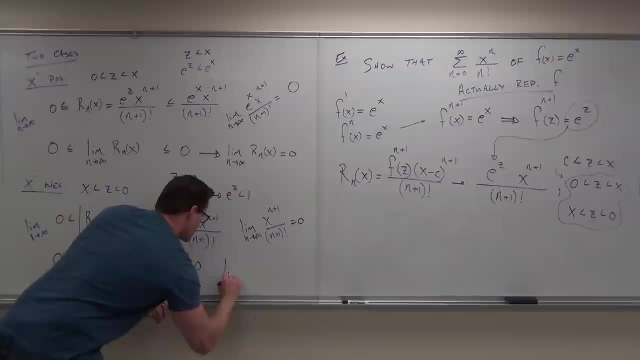 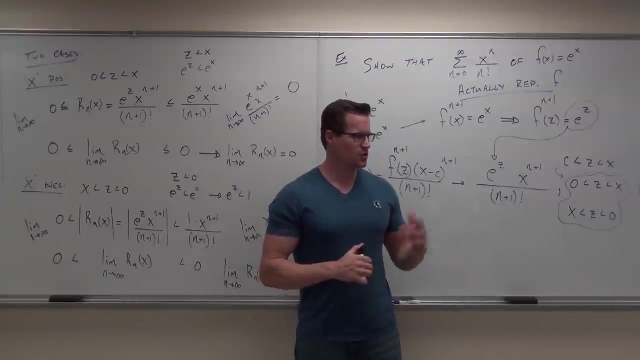 we get that. this is also zero. That's a lot of abstract stuff, right? That's proving some stuff. that was what we just did. Do you need me to go back through it for a few seconds? 10-second little recap here. 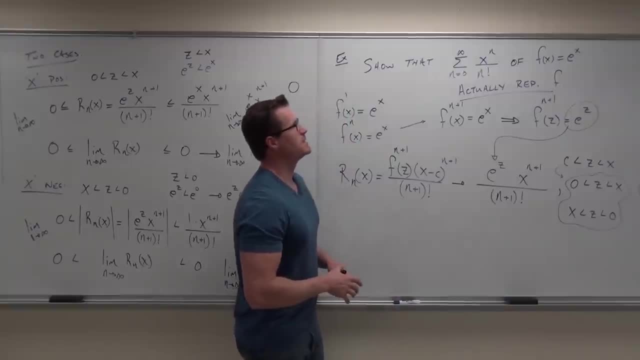 Okay, 10-second, 20-second recap Here. it is The idea of this whole idea is: don't reinvent the wheel. You're trying to prove that the remainder equals zero when you take a limit of it as n approaches infinity. 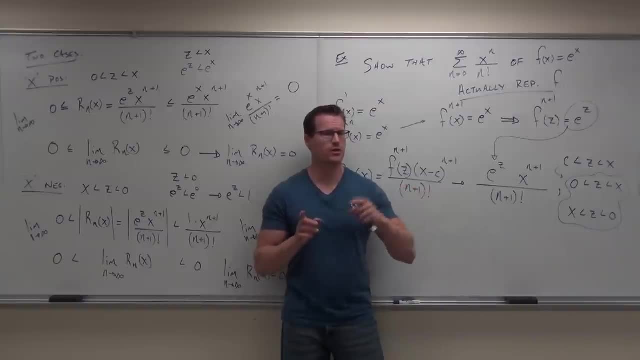 If you do that, what that says is that the remainder goes to zero. Therefore, if I go to infinity, the Taylor polynomial actually represents a function, That's a Taylor series. So just prove: the remainder equals zero. All right, The way we do that is we try to build the remainder into something in z's and x's, not f's. 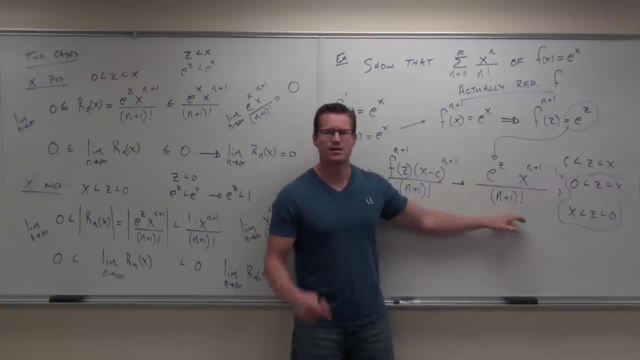 You've got to get z's and x's. So e to the z, x to the n plus 1, no problem, Sometimes you're going to have some cases here. In our case, well, x could be positive and x could be negative. 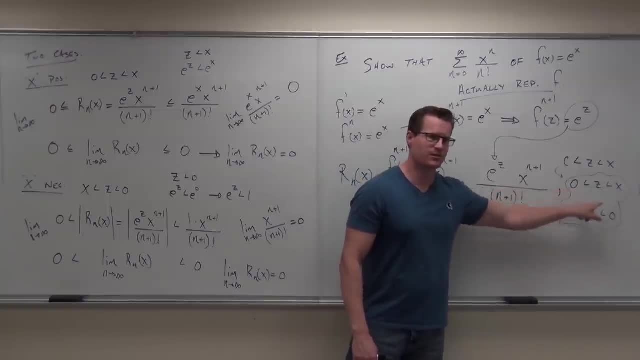 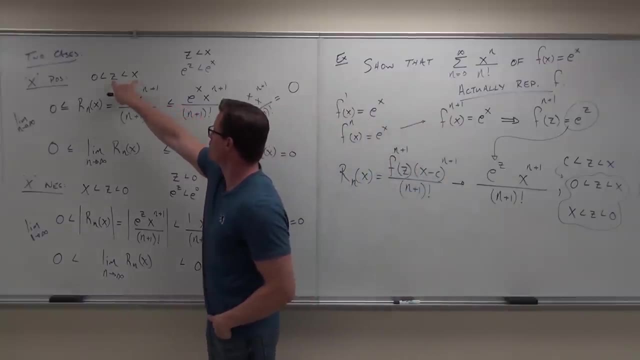 We have two cases. If x is positive, z is between zero and x. If x is negative, then z is between x and zero. Show for both. So you're going to have to use some inequalities here. If z is less than x, e to the z is less than e to the x. 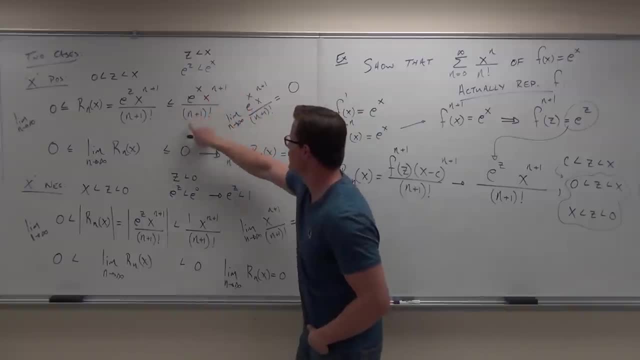 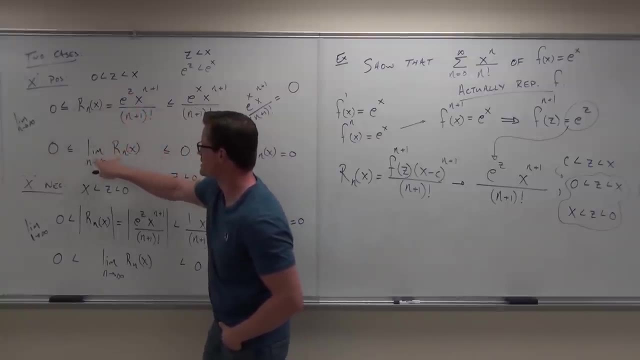 Okay, we got that. This limit, the limit of this thing goes to zero. The limit of zero is, of course, zero, We know this is positive because z is greater than zero. Therefore, because this limit is mashed or squeezed between these two zeros. 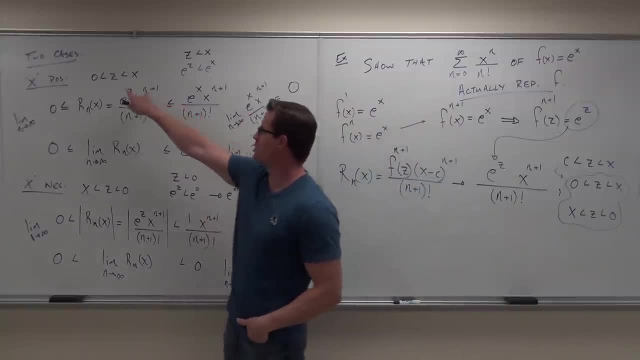 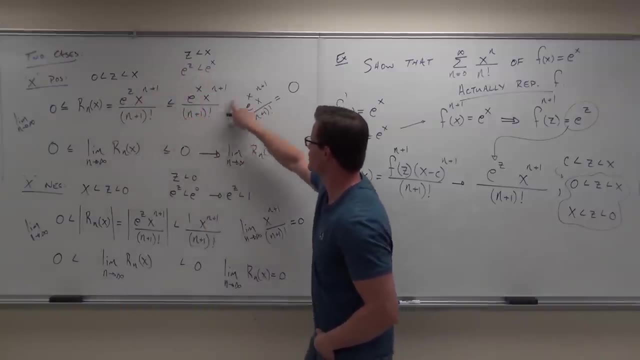 Show for both. So you're going to have to use some inequalities here. If z is less than x, e to the z is less than e to the x. Okay, We got that. This limit, the limit of this thing, goes to zero. 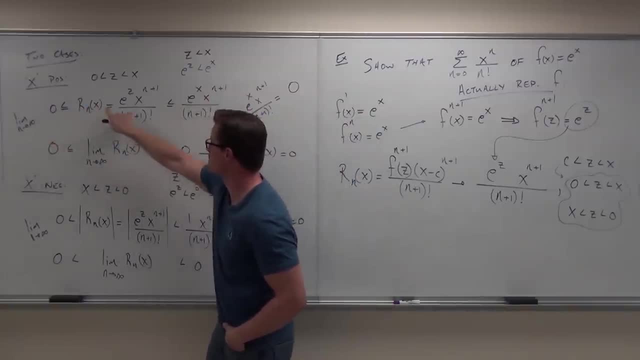 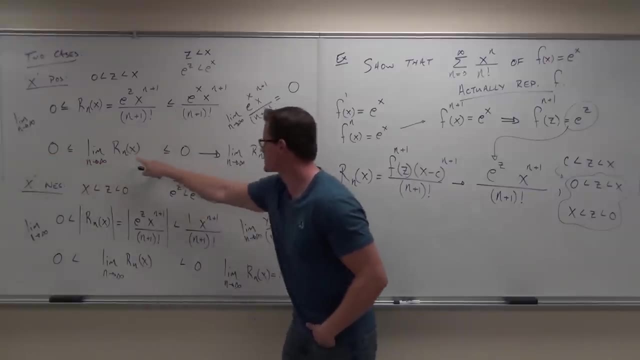 The limit of zero goes to zero. The limit of zero is, of course, zero. We know this is positive because z is greater than zero. Therefore, because this limit is mashed or squeezed between these two zeros, the limit of this remainder is also zero. 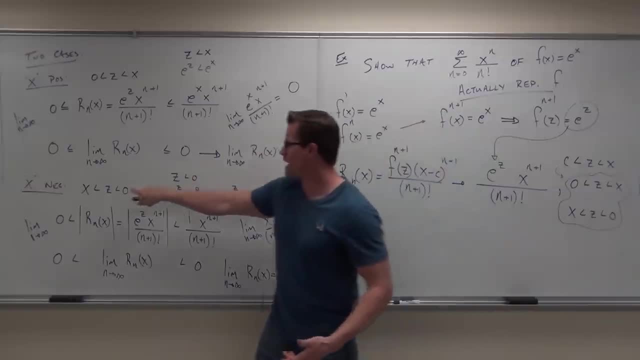 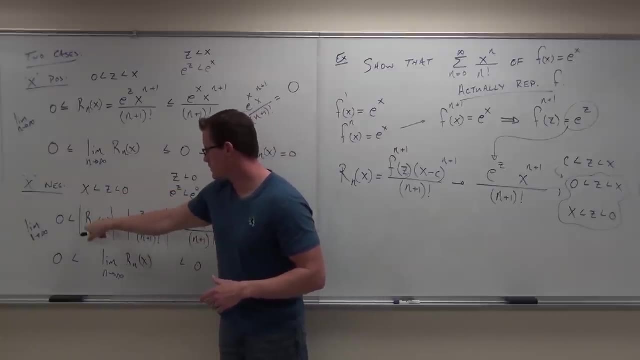 That's what we want, right? We want to show the remainder is zero. Cool, Now if it's backwards? if z is between x and zero, well, take the absolute value. The absolute value of the remainder is greater than zero. 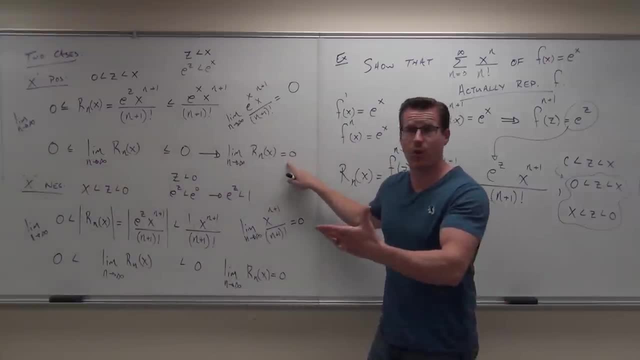 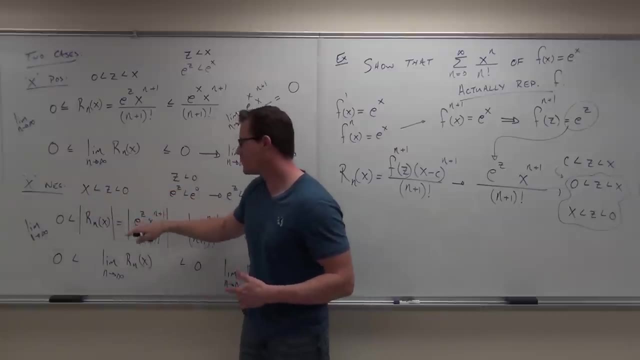 the limit of this remainder is also zero. That's what we want, right? We want to show the remainder is zero. Cool. Now if it's backwards. if z is between x and zero, well, take the absolute value. The absolute value of the remainder is greater than zero. 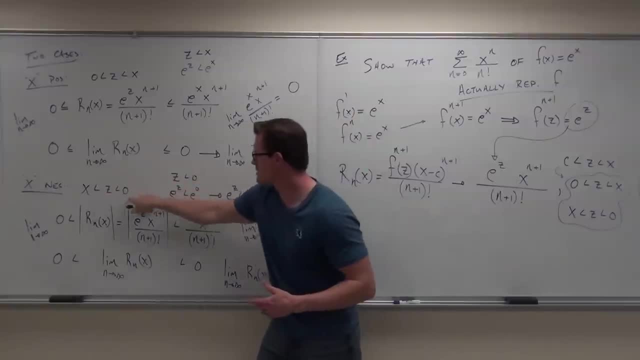 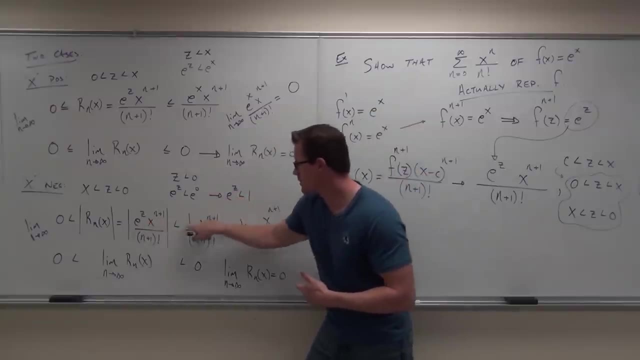 Well, it's positive. Also, less than one, because if z is less than zero, e to the z is less than e to the zero. So e to the z is less than one, e to the zero is one. Make this jump. 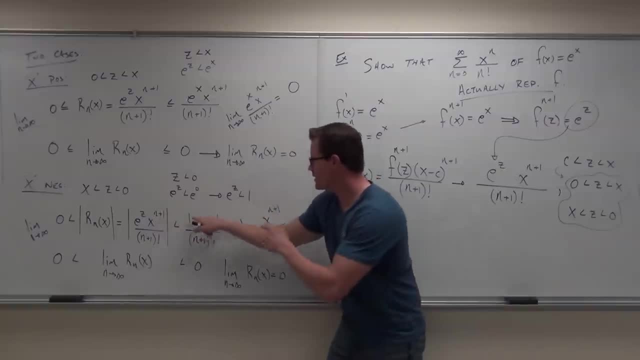 Therefore, e to the z is less than one, No problem, These things are all the same. The limit of this goes to zero. Again, we get the squeeze theorem Zero. we get zero. Our limit goes to zero and this proves it case by case. 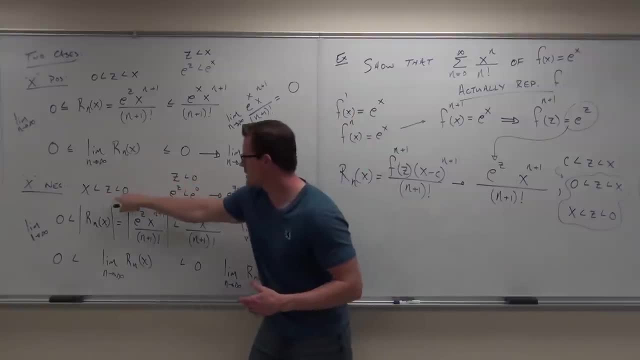 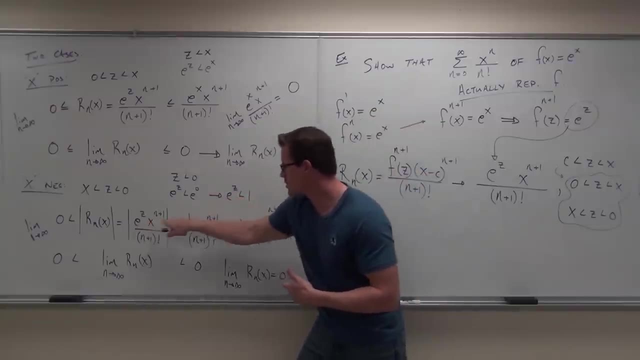 Well, it's also less than 1, because if z is less than zero, e to the z is less than e to the zero. So e to the z is less than 1.. e to the zero is 1.. Make this jump. 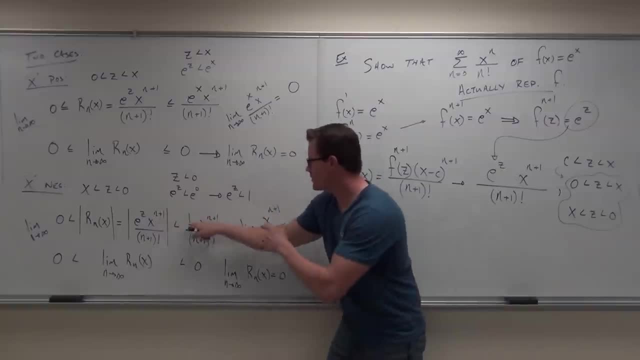 Therefore, e to the z is less than 1.. No problem, These things are all the same. The limit of this goes to zero. Again, we get the squeeze theorem. We get zero, We get zero, Our limit goes to zero. 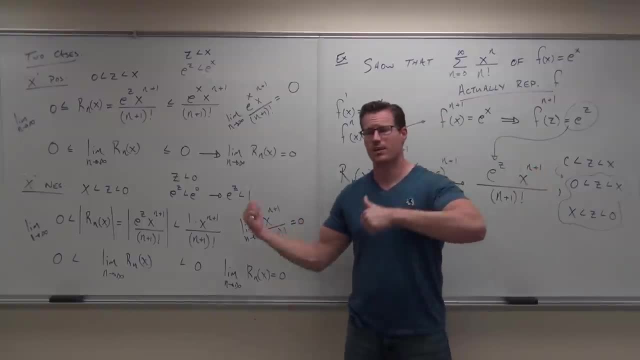 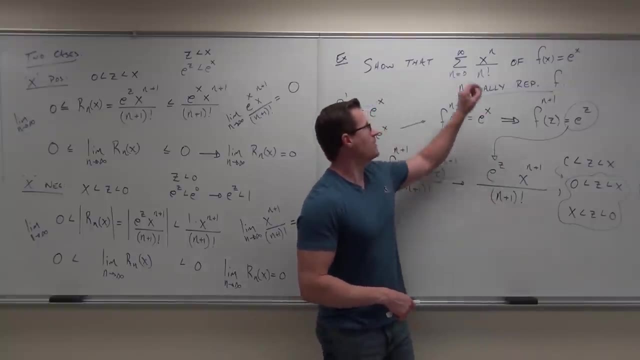 And this proves it case by case. So, no matter what, if x is positive, we got remainder zero. If x is negative, we got remainder zero. Therefore, since the remainder is zero, this proves. this, proves that this Maclaurin series. 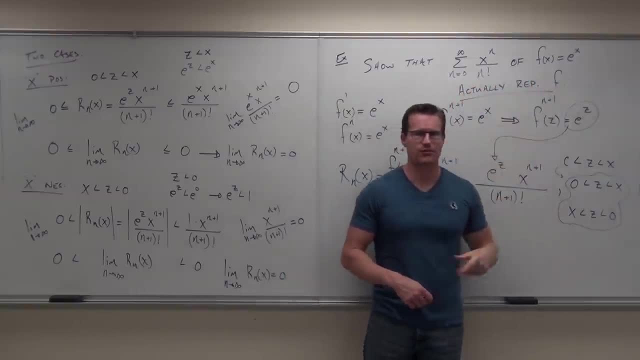 representation actually does represent the function f. That's the idea. It's a long way to show something that we didn't do very much. for What if we have a function that is derivative, like we can't find it? Then you get a problem. 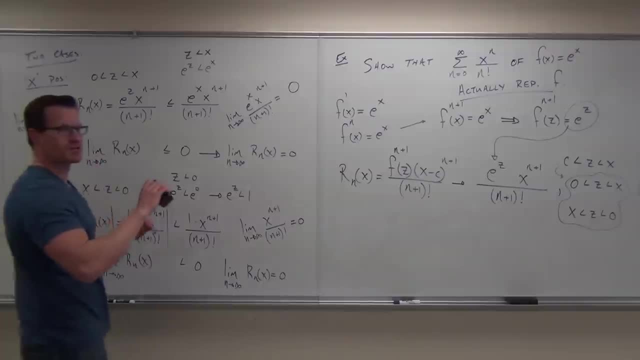 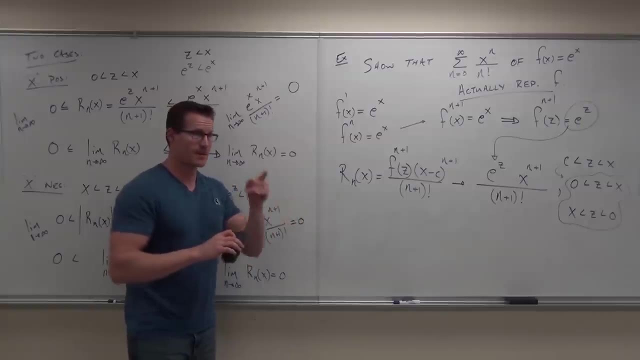 I'm going to show you one right now. Any more questions. I got to erase it to show you the last one. No Good, That's a good question. It's going to be hard to actually do that. You got to find some relationship for it. 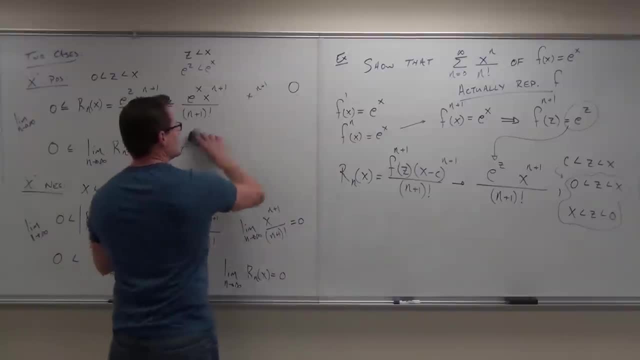 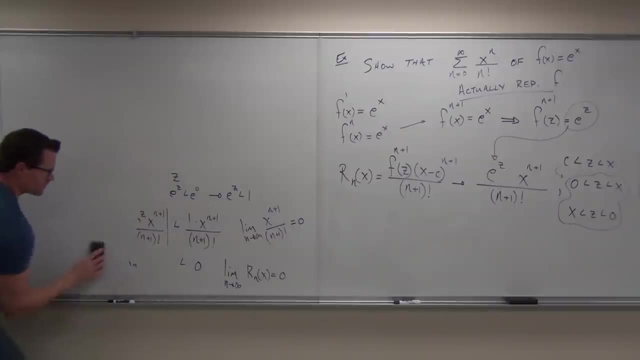 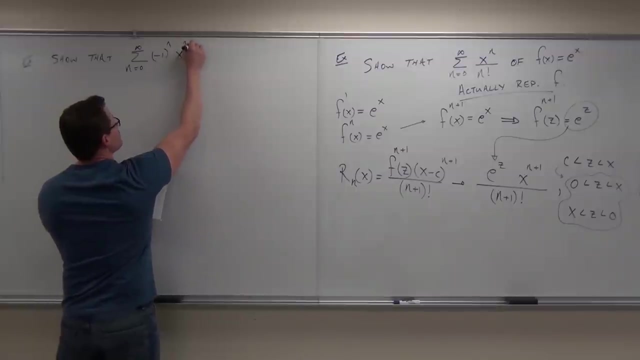 I'm going to show you an example like that right now. I didn't mean to just not answer your question there, but I'd like to answer it with this: OK, Don't worry, This one's quicker. It doesn't look like it's going to be quicker, but it is. 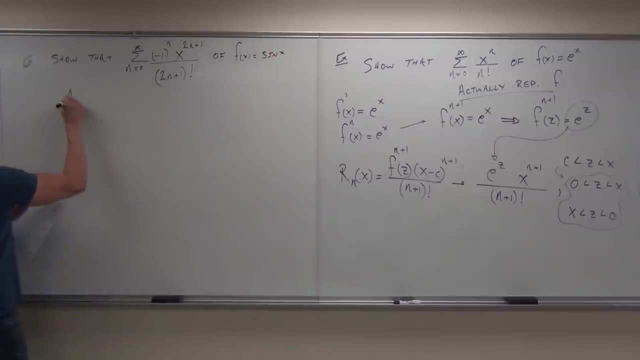 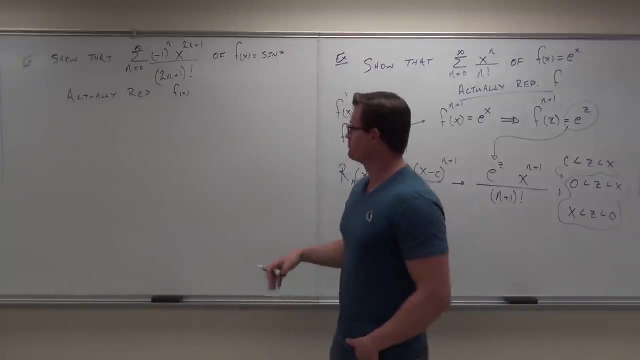 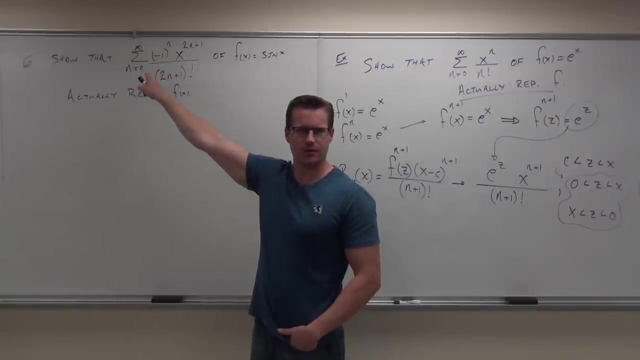 Show that that piece of junk actually represents the function. So show that this. whoa, what is that McLaurin-Taylor? Does it look familiar to you? This was given to you earlier, So in the last couple sections that we've done, 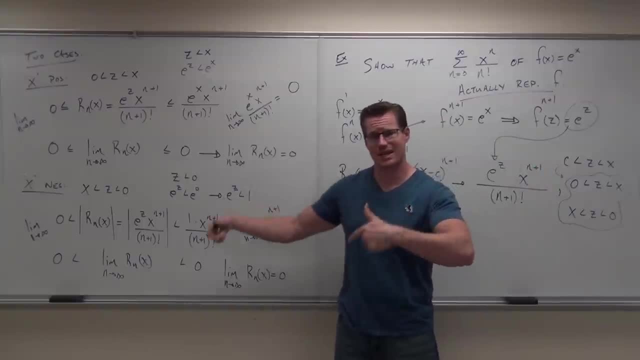 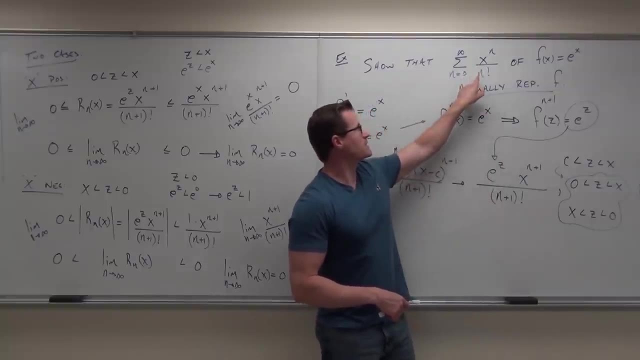 So, no matter what, if x is positive, we got a remainder of zero, If x is negative, we got a remainder of zero. Therefore, since the remainder is zero, this proves. this proves that this Maclaurin series representation actually does represent the function f. 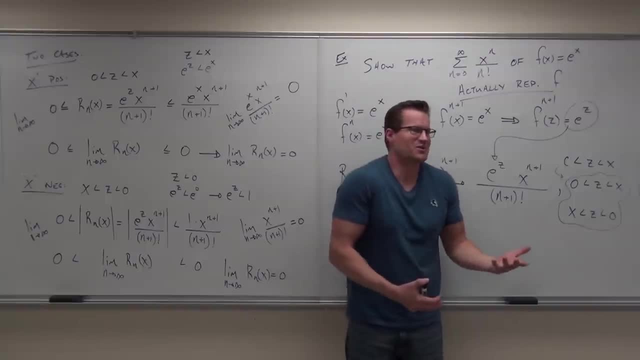 That's the idea. It's a long way to show something that we didn't do very much. for What if we have a function that is derivative? like we can't find it? Then you get a problem. I'm going to show you one right now. 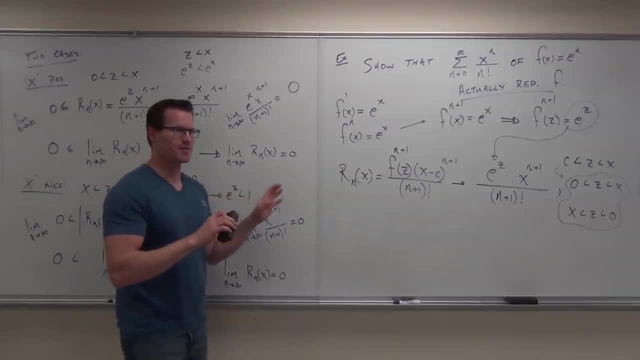 Any more questions, I got to erase it to show you the last one. No Good, That's a good question, because it'd be hard to actually do that. You got to find some relationship for it. I'm going to show you an example like that right now. okay, 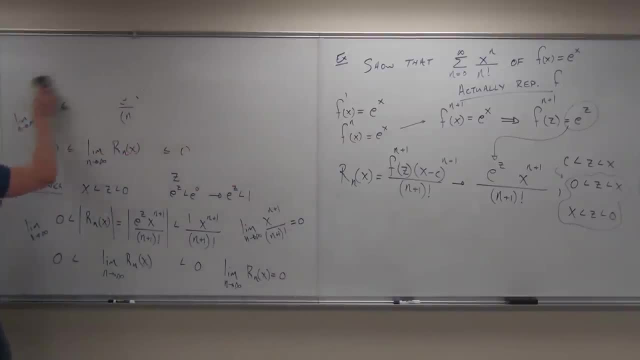 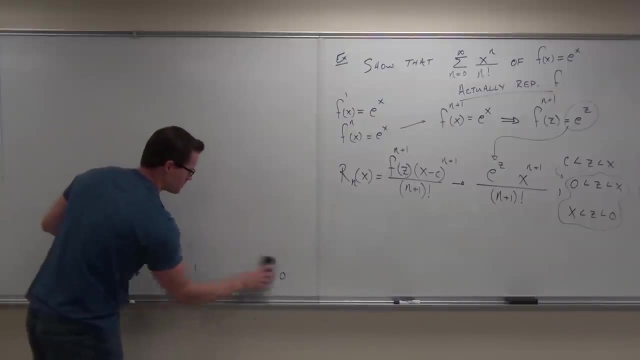 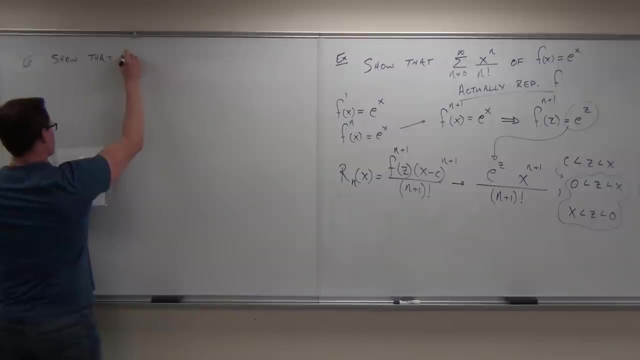 I didn't mean to just not answer your question there, but I'd like to answer it with this: Okay, Don't worry, this one's quicker. It doesn't look like it's going to be quicker, but it is Okay. 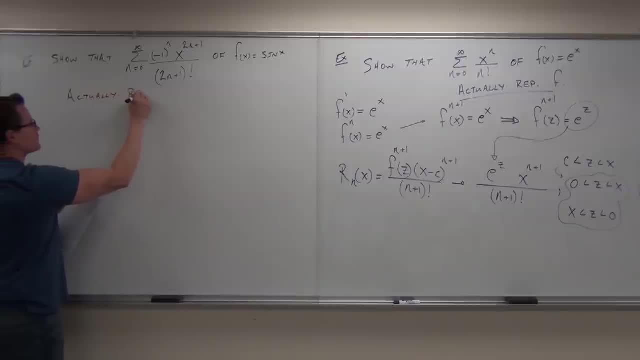 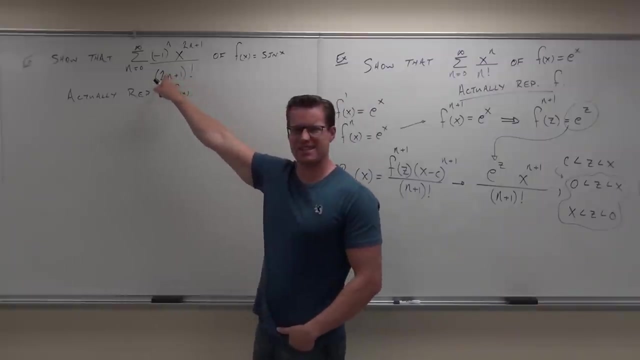 Show that that piece of junk actually represents the function. So show that this. whoa, what is that, Maclaurin-Taylor? Does it look familiar to you? This was given to you earlier, so in the last couple sections that we've done, 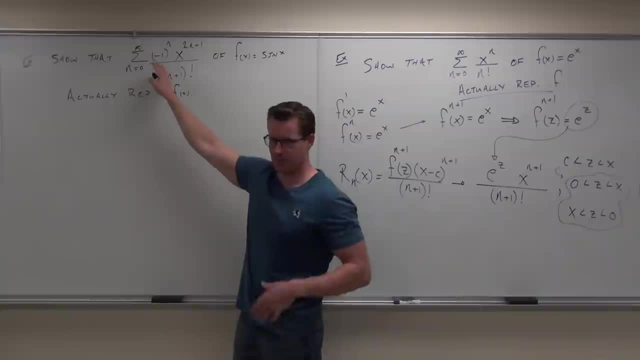 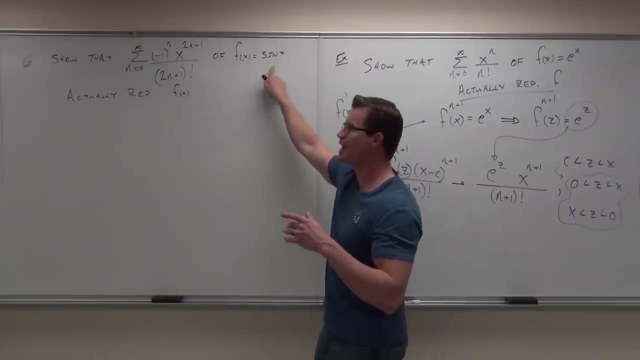 So here's what this says: Show that the Maclaurin-Taylor, Show that the Maclaurin-Taylor, The Maclaurin series, word for word in English, not math, speak. show that the Maclaurin series, which was developed from this function sine of x. 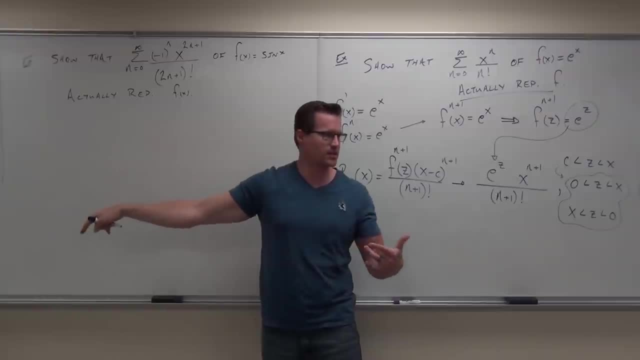 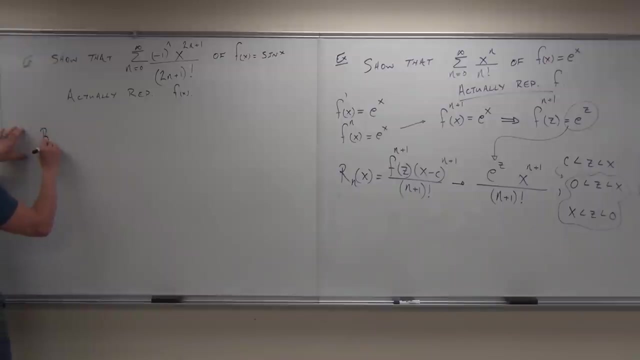 actually represents the function sine of x. That's what that says. So show that it's true. The way that we show that this is true is showing that the limit of the remainder of our Taylor polynomial goes to what? Zero. Okay. so what we want to do is we want to somehow find what this thing is. 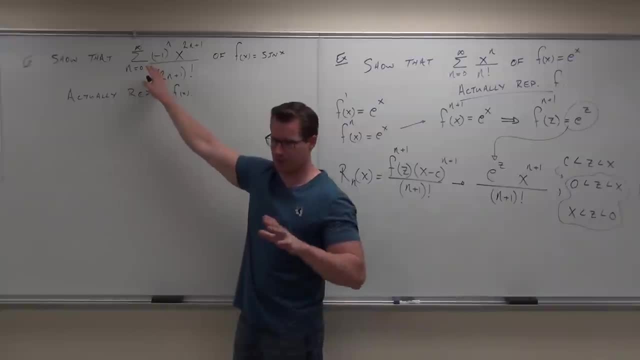 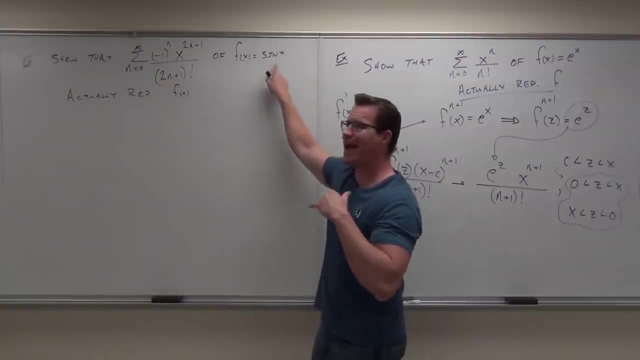 So here's what this says: Show that the McLaurin series, word for word in English, not math speak. Show that the McLaurin series, which was developed from this function sine of x, actually represents the function sine of x. 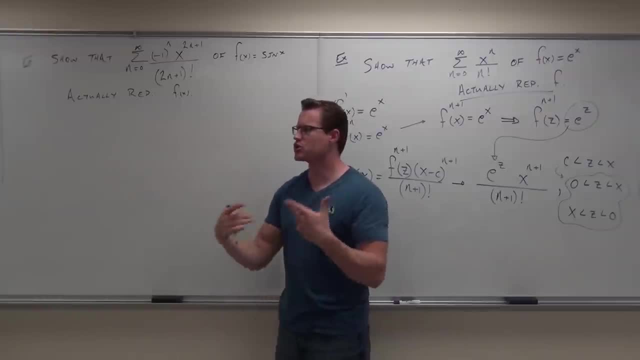 That's what that says, So show that it's true. The way that we show that this is true is showing that the limit of the remainder of our Taylor polynomial goes to what? Zero, Okay. so what we want to do is we want to somehow find what this thing is. 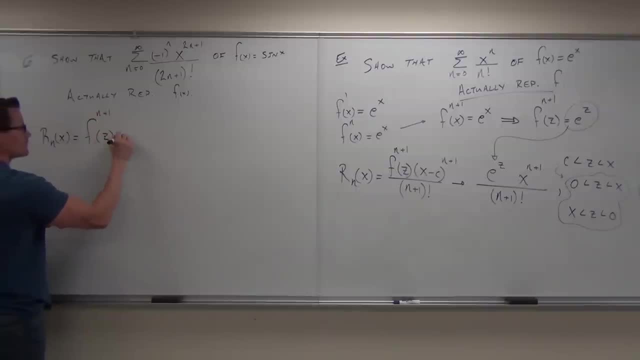 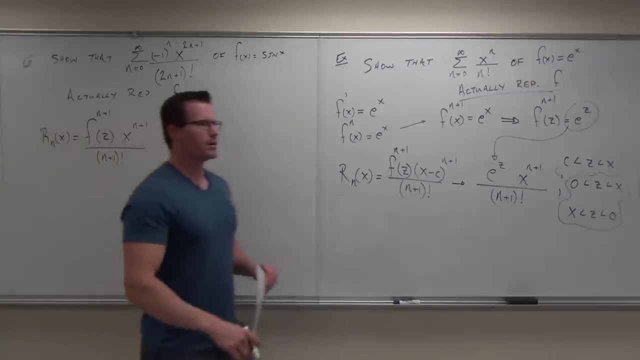 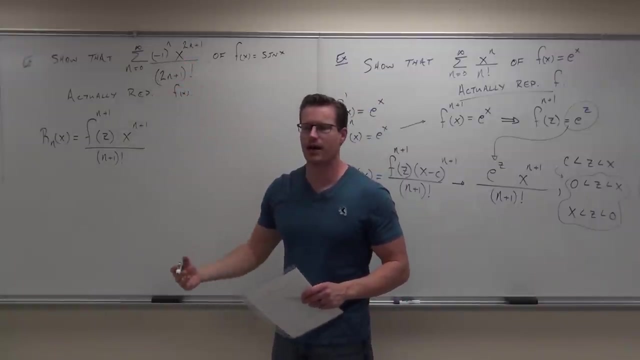 And then show that that goes to zero. Notice something: I don't have to have a 2n plus 1 up here. I don't really care about that. All I'm trying to show is that the remember the remainder of the Taylor polynomial is going to look like this: 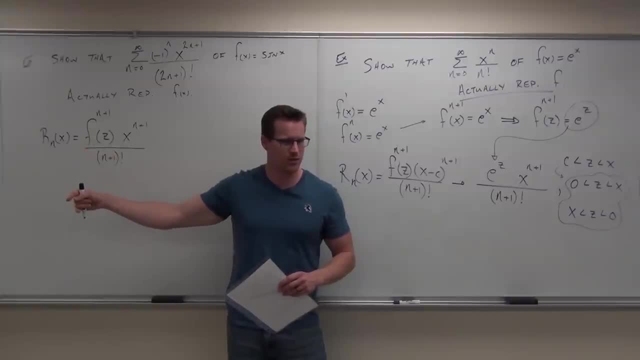 It's going to be x to the nth, It's going to be x to the n plus 1 over n plus 1 vectorial. You guys with me on that one? Uh-huh, That's what it's going to be. 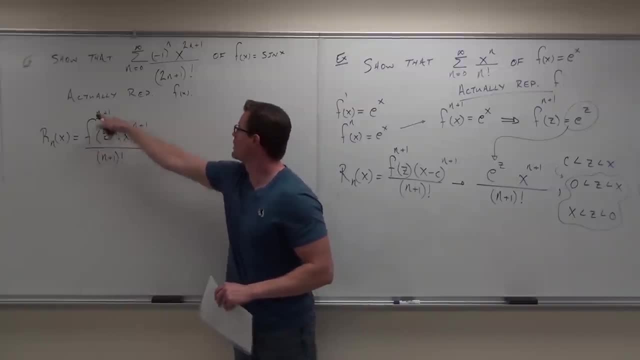 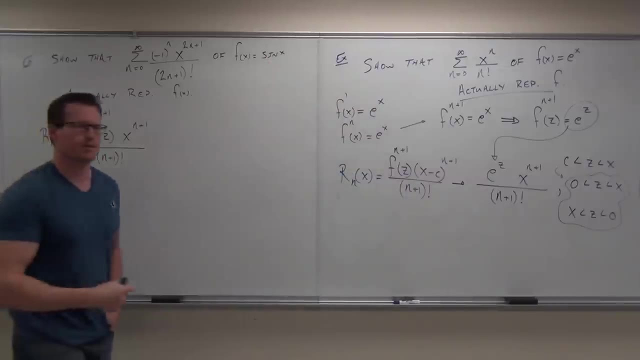 That's going to have an f to the n plus 1 over z. This is where we use- sorry, this idea. So that's where we get the function coming into it. Now, let's think about this for a second. This thing, that's going to be there. 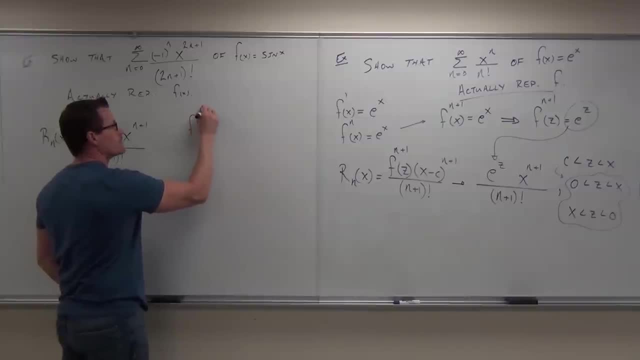 This is going to be there. We've got to find an expression for this. Well, let's start with a little bit different of an idea. Let's start with Just x. Let's start taking some. let's start taking some derivatives. 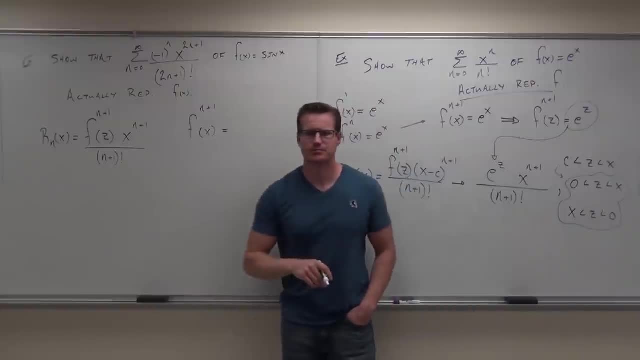 Just in our head: What are you going to get for your derivatives? And then, And then, And then. So this is going to either be sine cosine, negative sine or negative cosine, No matter what we get, no matter what we always know. 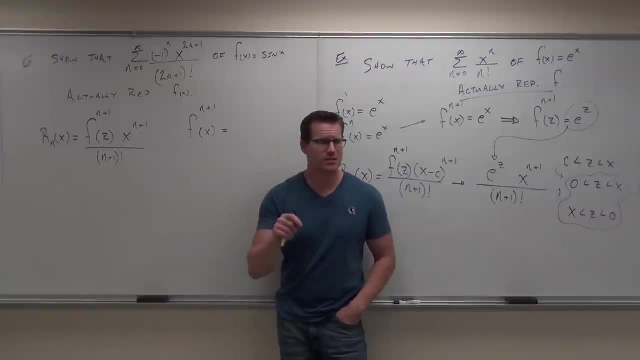 that if I plug in any number, I'm always going to get something. that's between what two numbers? Let's try that again, because I heard like 15 different answers right now. Okay, do you get that? this is always either plus or minus sine? 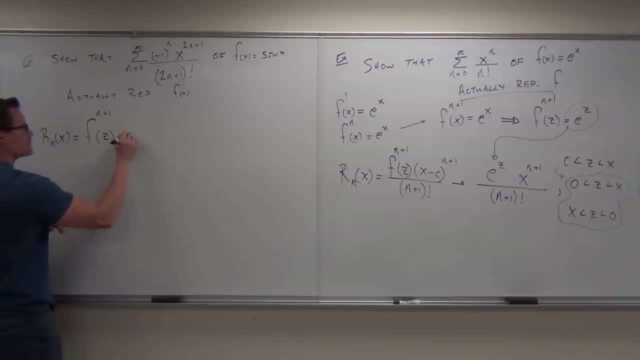 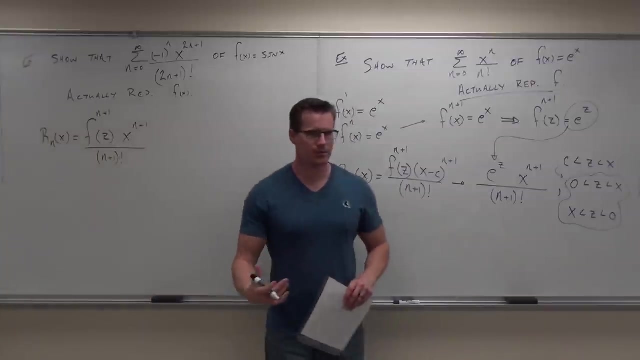 And then show that that goes to zero. Notice something: I don't have to have a 2N plus 1 up here. I don't really care about that. All I'm trying to show is that the remainder of the Taylor polynomial is going to look like this: 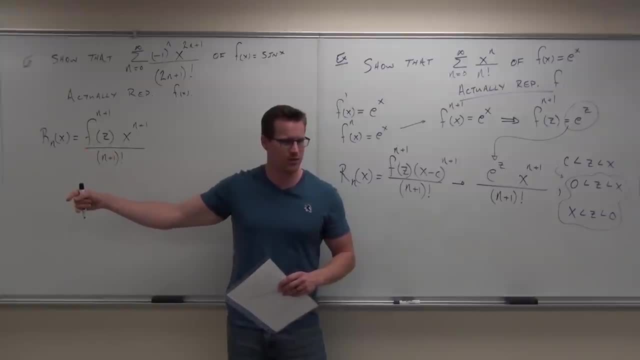 It's going to be extra than plus 1 over M plus 1.. factorial- You guys with me on that one. So it's going to be that's going to have an f to the n, plus 1 over z. This is where we use- sorry, this idea. So that's where we get the function coming. 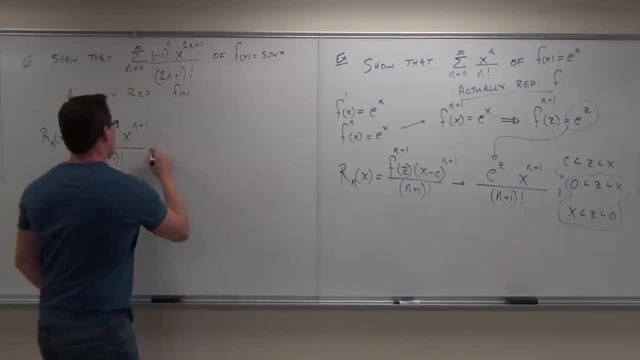 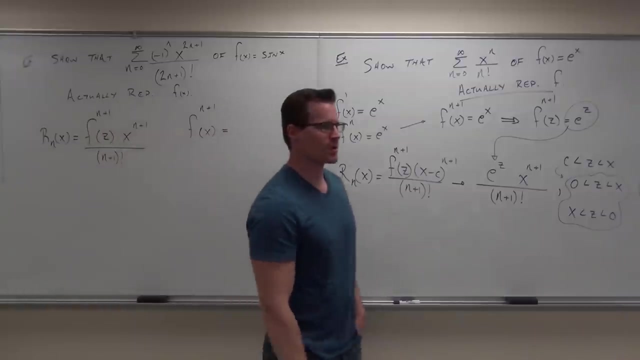 into it. Now, let's think about this for a second. This thing that's going to be there, This is going to be there. We've got to find an expression for this. Well, let's start with a little bit different of an idea. Let's start with just x. Let's start taking some derivatives, just in our 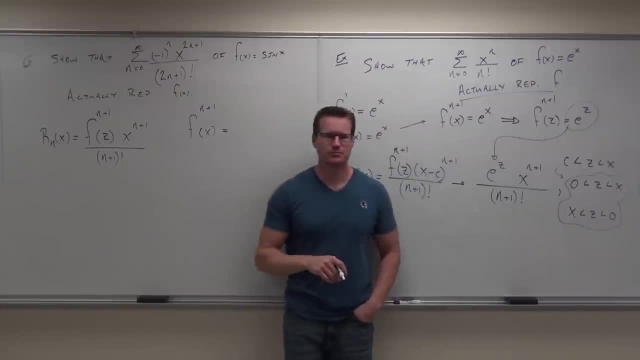 head: What are you going to get for your derivatives? And then, And then, And then. So this is going to either be sine cosine, negative sine or negative cosine. No matter what we get, no matter what. we always know that if I plug in any number, I'm always going to get something. 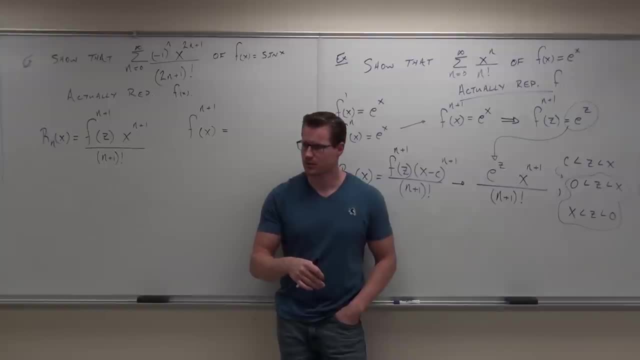 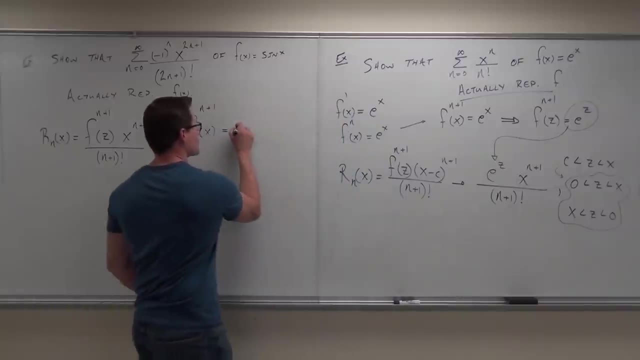 that's between what two numbers. Let's try that again, because I heard like 15 different answers right now. Okay, do you get that? this is always either plus or minus sine or plus or minus cosine, Do you guys get that? Yeah, Okay, therefore, if I start plugging in, remember z means you're. 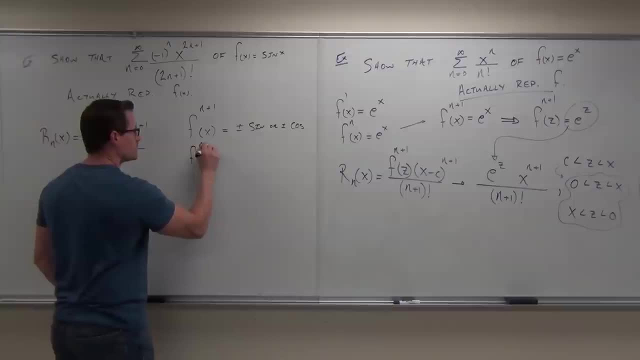 plugging in numbers. okay, If I plug in numbers here, if I plug in numbers, then what's going to happen is: this is going to be a maximum of what number? What's the biggest thing you can get out of this? What's the smallest thing? 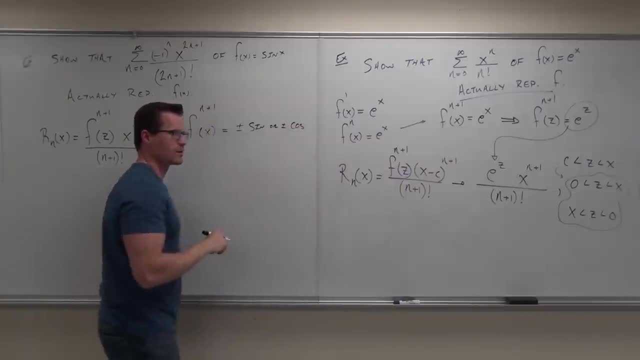 Or plus or minus cosine. Do you guys get that? Yeah, Okay, therefore, if I start plugging it, remember z means you're plugging in numbers. okay, If I plug in numbers here, If I plug in numbers, then what's going to happen is this is going. 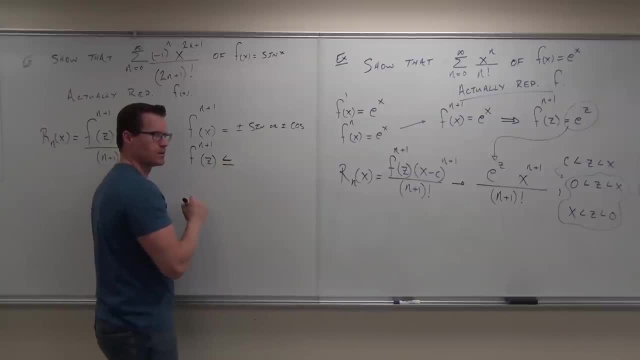 to be a maximum. of what number? What's the biggest thing you can get out of this One? What's the smallest thing you can get out of this One? So somewhere when I plug in numbers, I know that remember. 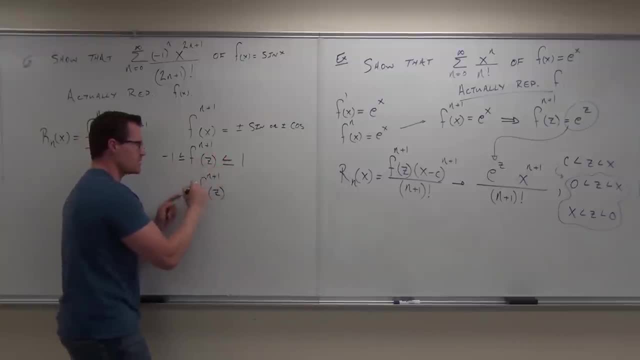 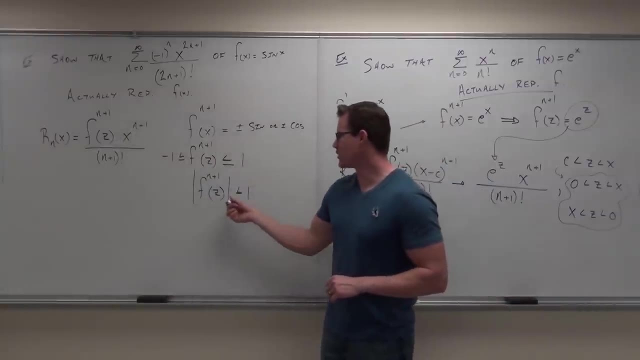 double inequalities like this negative one is less than this, is less than this. you can make this an absolute value and do this is less than one. That's, by definition, what an absolute value is. It says, hey, an absolute value, inequality is a double inequality. 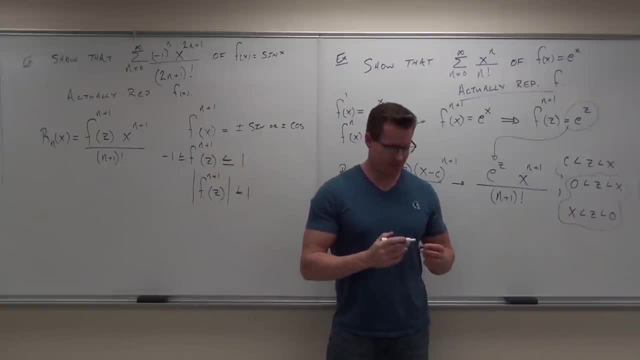 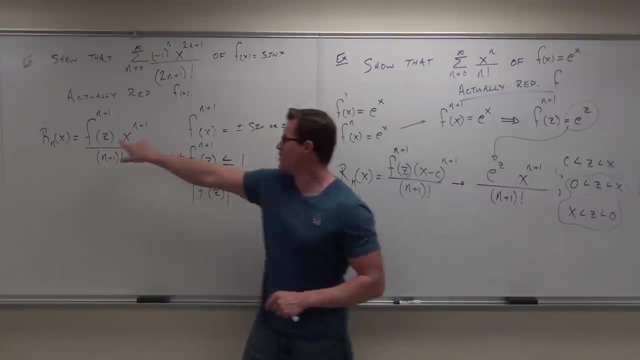 That's what that means. So here's what I'm trying to say. It's: we did a lot of math to show something quite simple. Here's the whole point. Do you understand that, no matter what my derivative is, this value right here will always be, in terms of absolute value, less than one? 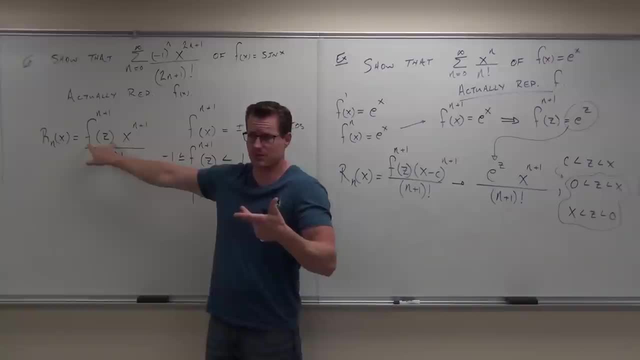 Do you guys get that idea? Yeah, The biggest thing it can be is one. The smallest thing it can be is negative one. So an absolute value: it's got to be less than one. Well, let's go ahead and do this thing. 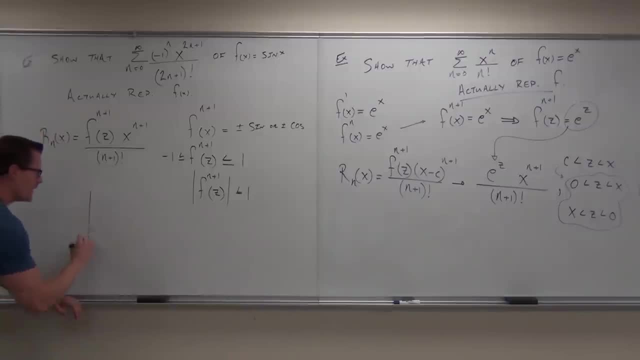 Let's set up an inequality. So, if I do my absolute value, which is what I'm going to do, what's this always greater than in terms of absolute value? Sun Zero, Yeah for sure. Now, this equals this Absolute value. 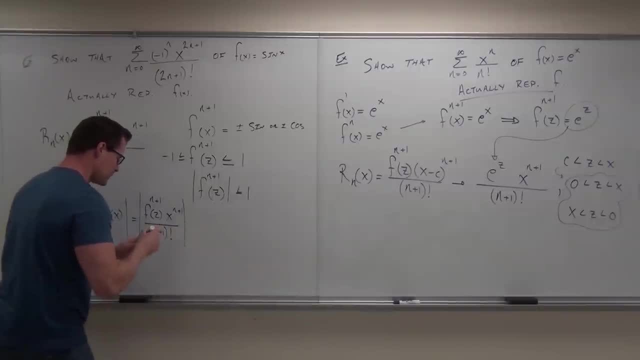 But this thing, okay, here it is one more time. Check it out. There you go, Watch, watch, watch. So if the absolute value of the n plus 1 derivative of f at z is less than or equal to one, 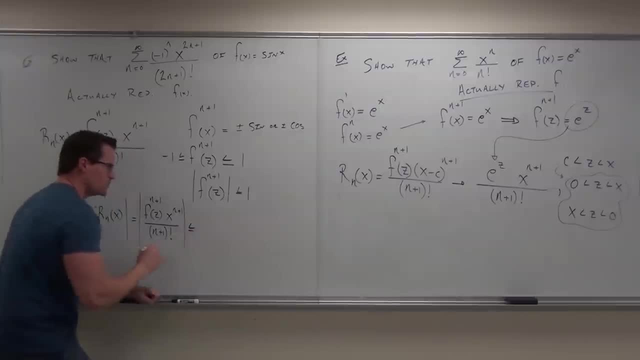 the absolute value of this whole thing is less than or equal to what's going to change here. Is the x to the n plus 1 going to change? No, we didn't say anything about that. Is this going to change? No, 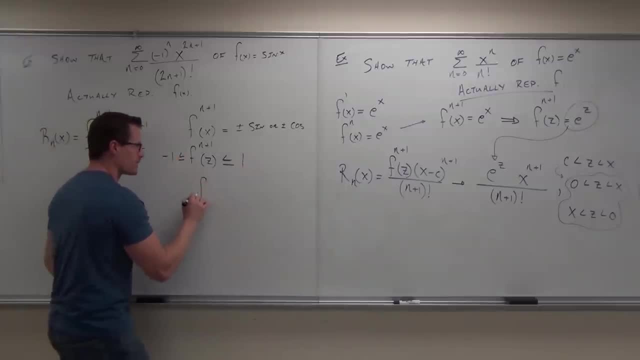 you can get out of this. So somewhere when I plug in numbers, I know that remember. double inequalities like this: negative one is less than this, is less than this. you can make it an absolute value and do this is less than one. That's by definition. what an absolute value is It? 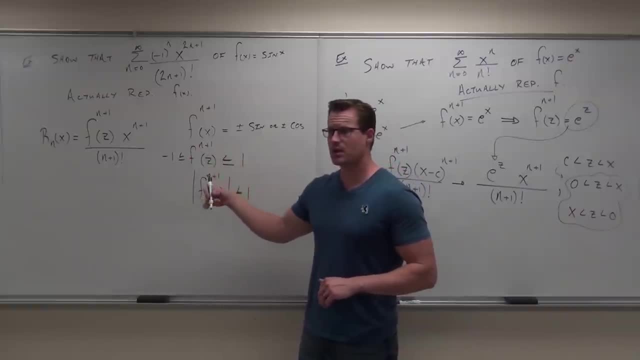 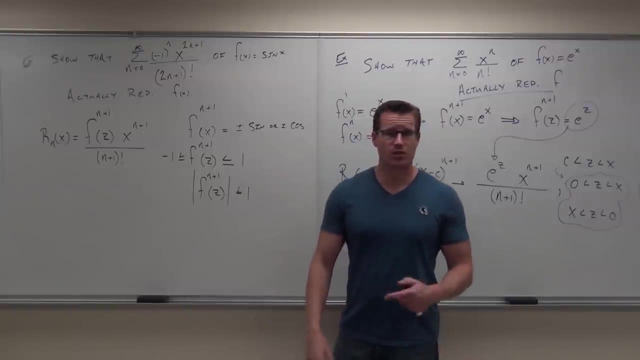 says: hey, absolute value inequality is a double inequality. That's what that means. So here's what I'm trying to say. It's we did a lot of math to show something quite simple. Here's the whole point. Do you understand that, no matter what my derivative is, this value right here will always be? 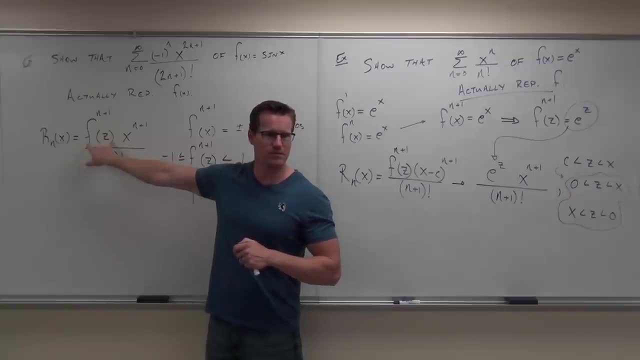 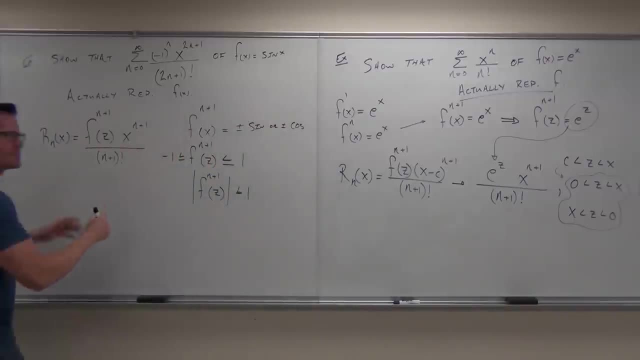 in terms of absolute value less than one. Did you guys get that idea? Yeah, The biggest thing can be is one small thing can be as negative one. so an absolute value it's got to be less than one. Let's go ahead and do this. then Let's set up an inequality. So, if I do, my absolute value. 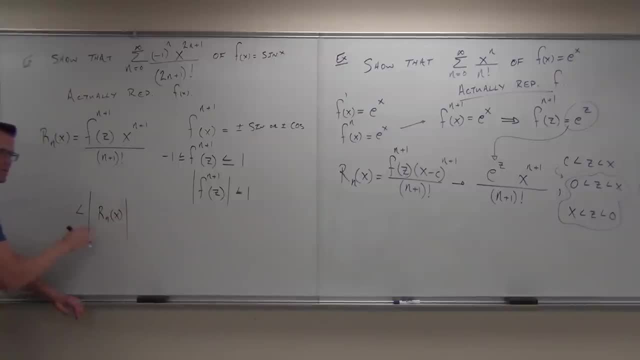 which is what I'm going to do. what's this always greater than in terms of absolute value? Yeah, for sure. Now, this equals this And this is my absolute value. But this thing, okay, here it is one more time. Take it out. There you go. 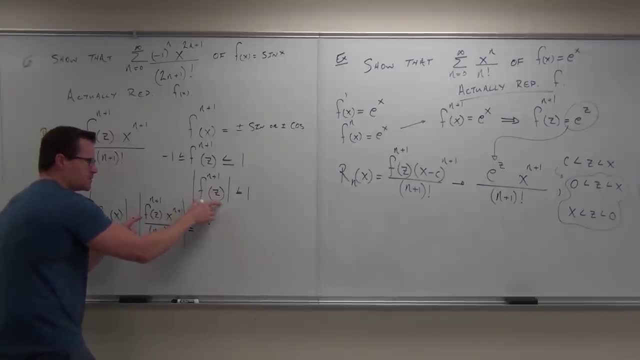 Watch, watch, watch. So if the absolute value of the n plus one derivative of f at z is less than or equal to one, the absolute value of this whole thing is less than or equal to. what's going to change here? Is the x to the n plus one going to change? No, we didn't say anything about that. 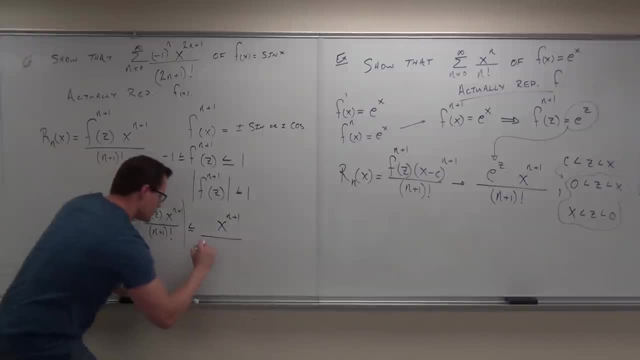 Is this going to change? No, Is this going to change? Yes, How much is this less than One In terms of absolute value? we have that. In terms of absolute value, this is less than one. Does that make sense to you? Now? now we get to take the limit. What's the limit? Zero Of zero. 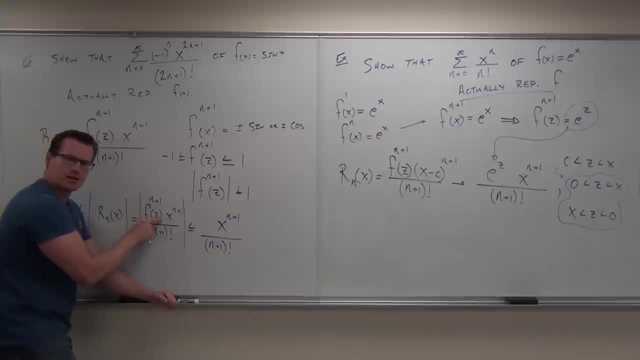 Is this going to change? Yes, How much is this? less than One In terms of absolute value? we have that. In terms of absolute value, this is less than one. Does that make sense to you Now? now we can take the limit. 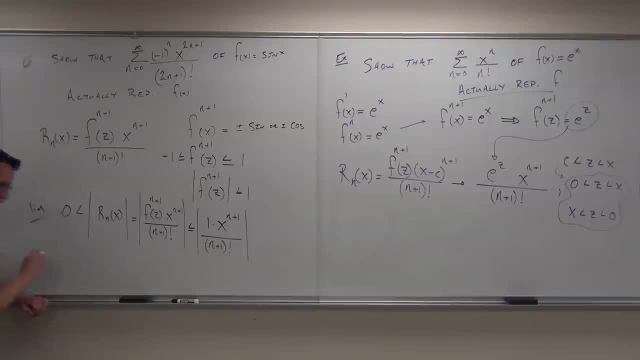 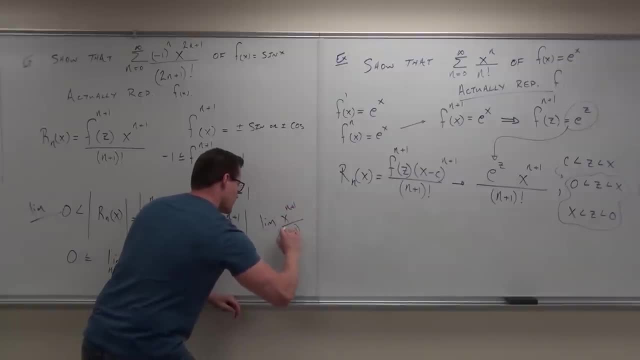 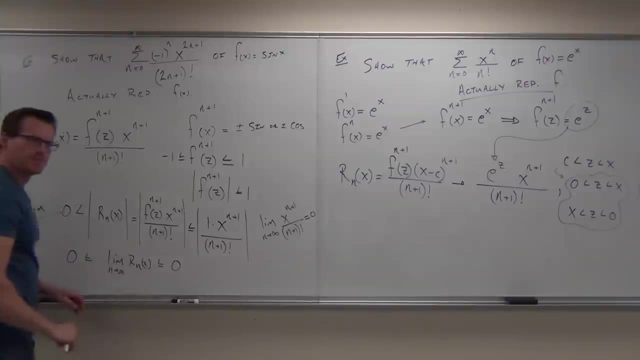 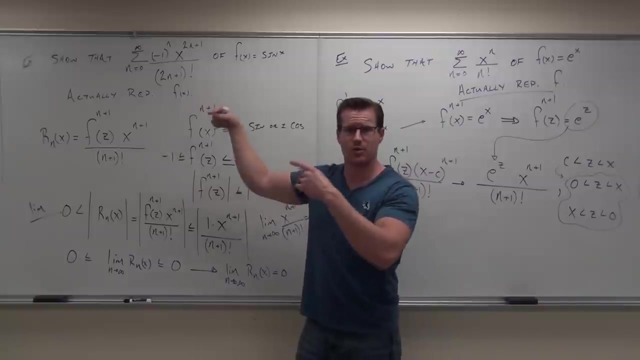 Zero. I told you we're going to do this several times. What's that say about this limit? Zero, Zero, Zero. What does that say about this limit? What's that say about this? Does this actually represent our function? Yes, 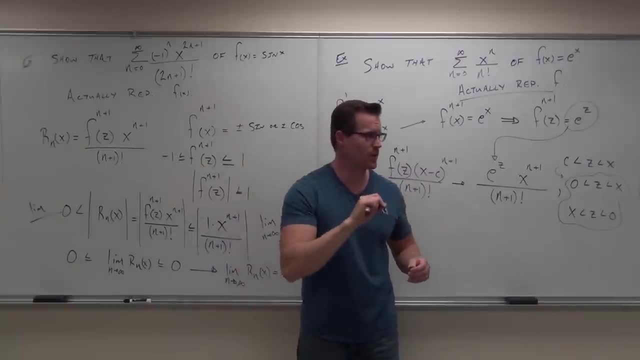 If the remainder of our Taylor polynomial, as n, approaches infinity, goes to zero, that means that the Taylor polynomial itself, as it goes to infinity, is a Taylor series which actually represents our function. And that's how you prove it. You've just got to prove that the remainder goes to zero, and we've done that here. 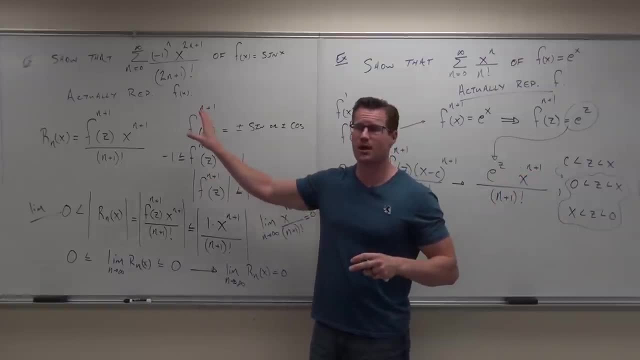 You find out- and hopefully Michael answered your question- you find out some relationship. Not necessarily can you find a pattern. there is no pattern. well, there's a pattern, but not that we can represent mathematically. We go: okay, this is either plus or minus sine or plus or minus cosine. 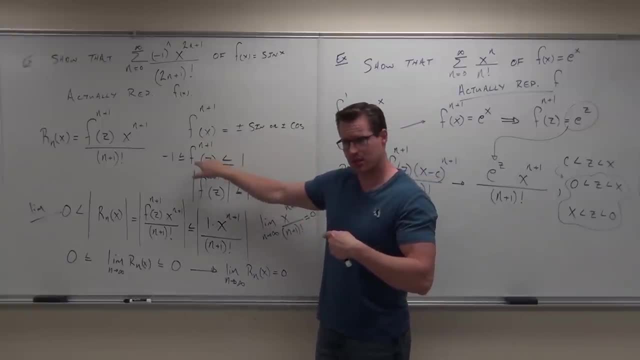 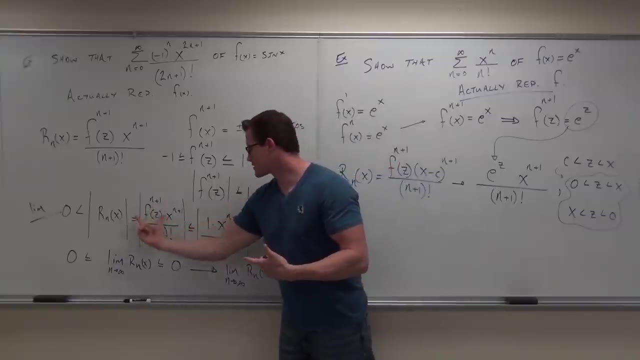 No matter what if I plug in numbers to it. that's what a z is. it's got to be between negative one and one. If it is, then the absolute value of that is always less than one. Use that: Say this is always less than one and then show that this goes to zero. 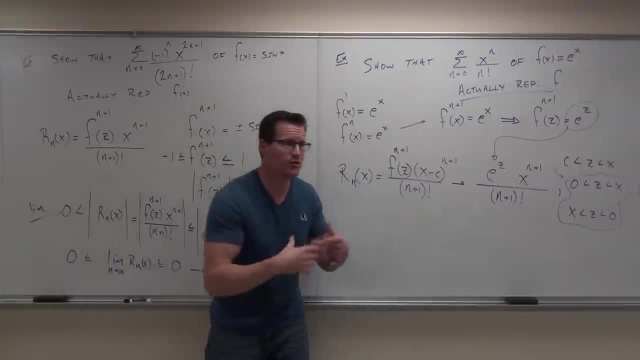 Show that well, it's bigger than zero. if it's absolute value, no problem. Remember, you're always trying to prove it's zero, right? So use the squeeze theorem, but it's always going to be the same number: Zero and zero. 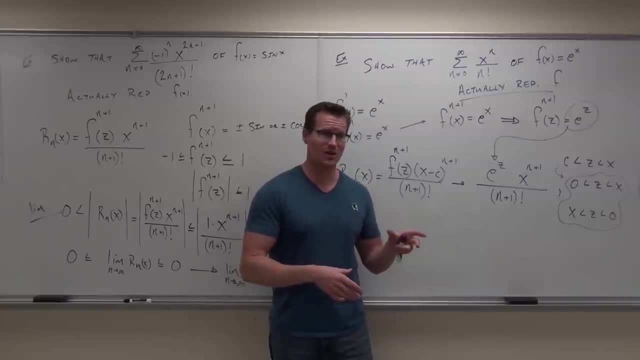 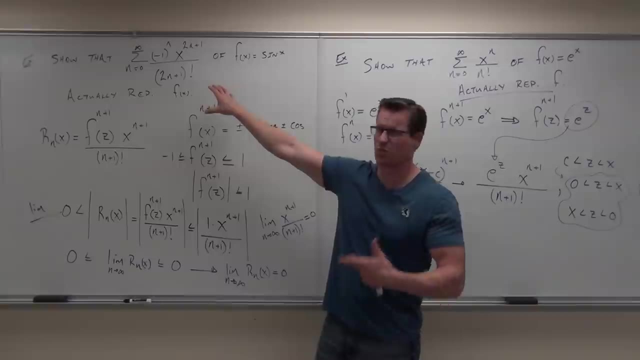 Show that that limit of your remainder is somewhere between zero and zero, And you've proven that the limit of your remainder is n equals infinity, is zero. therefore, your Taylor series or your Perforin series or whatever you have actually does, represent the function.